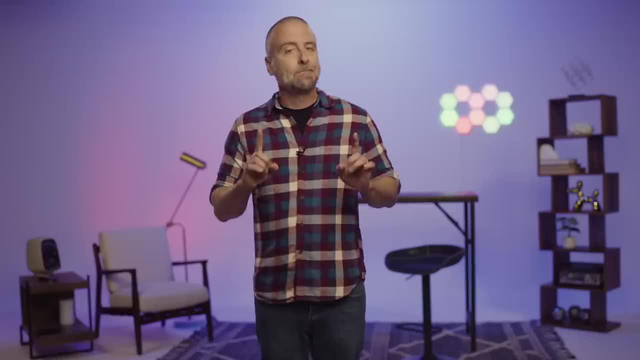 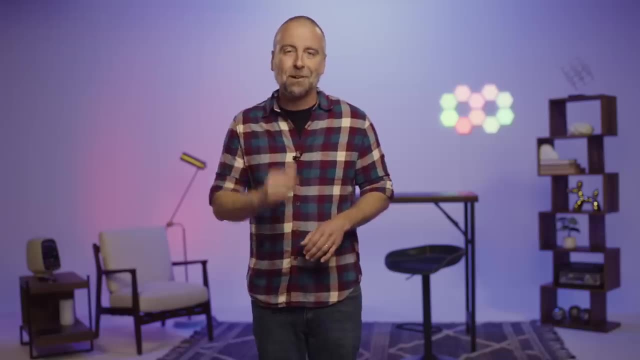 language, you'll pretty much be ready for this course. It will be helpful if you have a basic understanding of how the web works with web servers and browsers. but don't sweat it, we'll touch on that too. Now, if you haven't met these requirements, please check the notes attached to. 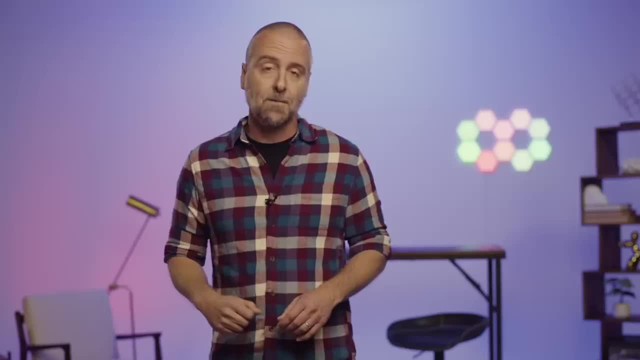 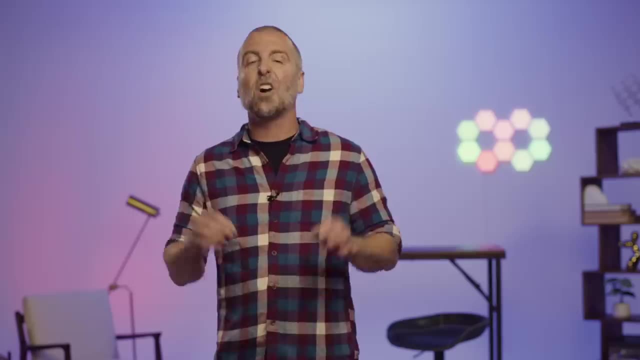 this video for where to get started with some beginning web and programming concepts. That reminds me you should take some time to get used to your learning environment. The notes are attached to this video and I'll also drop more information into that section to keep you updated. 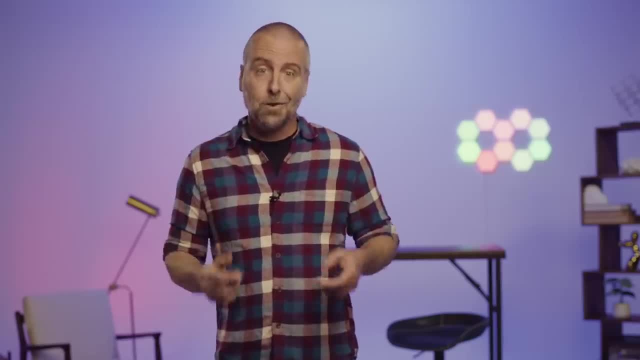 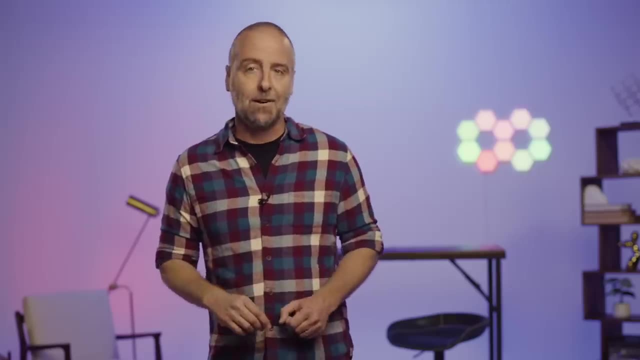 on what might have changed from my right now to your right now, And I'll do my best to remind you to look in there when there's something I think you just have to see. but you really should get in the habit of checking that area out. There'll be tons of juicy information there. 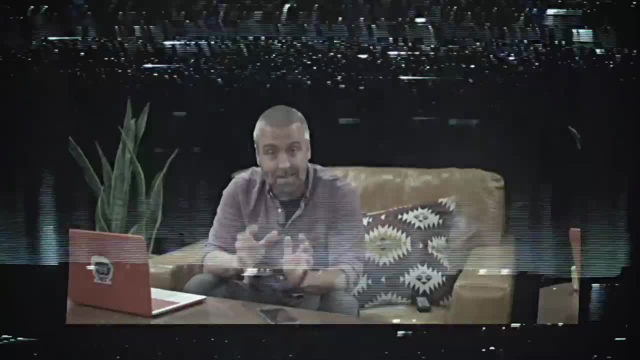 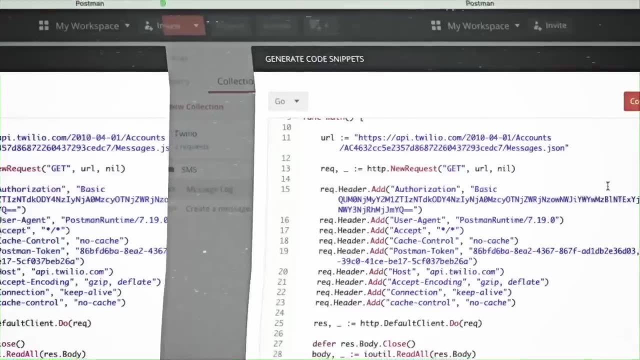 You might be getting a real bad case of deja vu right now. This is a refresh of a course from 2019, which these days seems like about 30 years ago or something. If you saw that version, welcome back. Technology is constantly evolving. 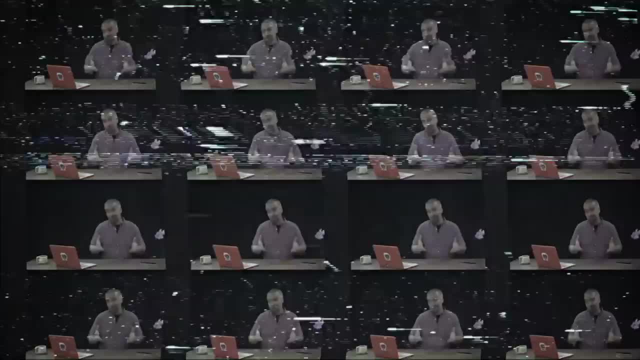 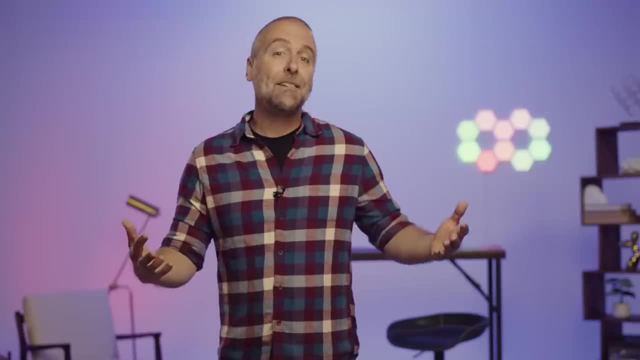 and just updating the notes wasn't cutting it, so this is version two. Thanks for all the feedback. by the way, A lot of yours and your fellow learners' suggestions are implemented in this new, updated version. All that to say, we got you. These videos have captions, so if you feel like you. 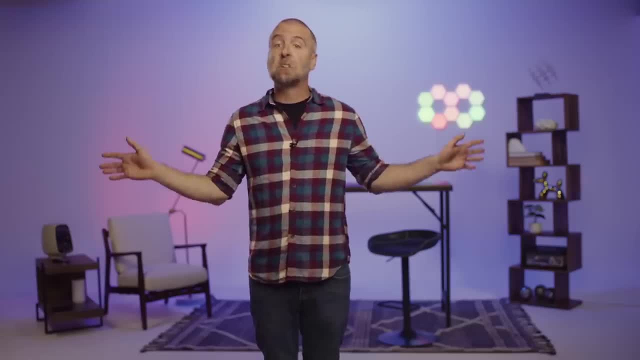 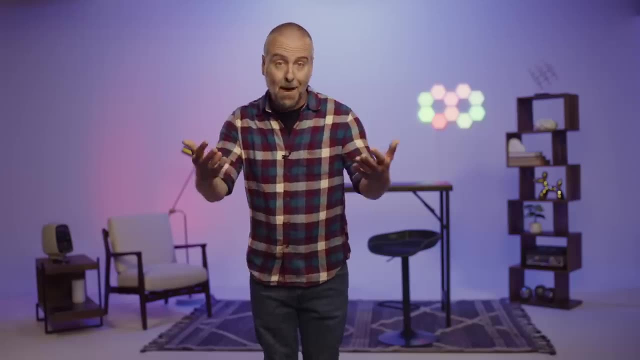 might benefit from having those on. please use them. This space is all yours. If you want me to speak slower, please use the speed controllers to slow me down And if I'm taking a long time, speed me up. I make a pretty good chipmunk. And last but certainly not least, 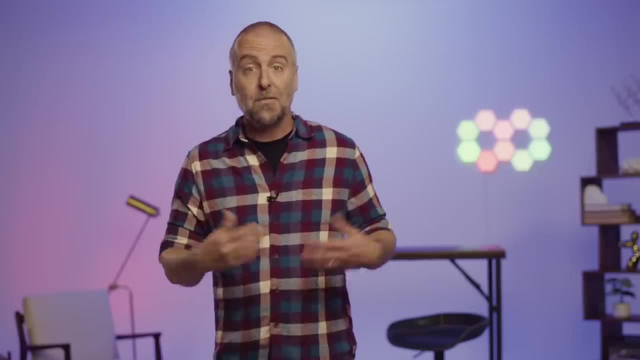 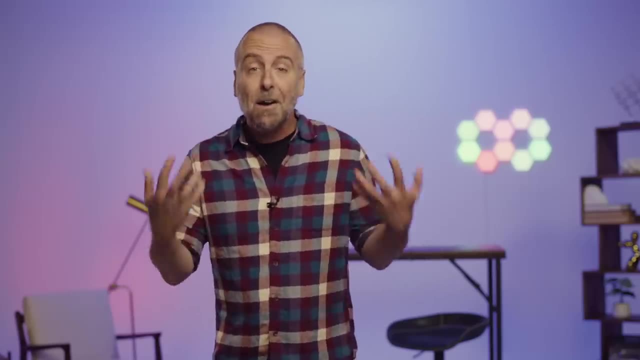 take advantage of the fact that you are in a video-based course. If you need me to repeat myself, use the video controls to rewind me. If you feel like you need to take a break to let something in seek in, by all means please pause me. I'll be right here waiting for you. 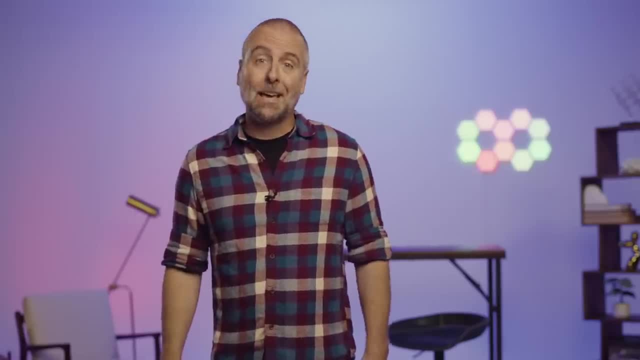 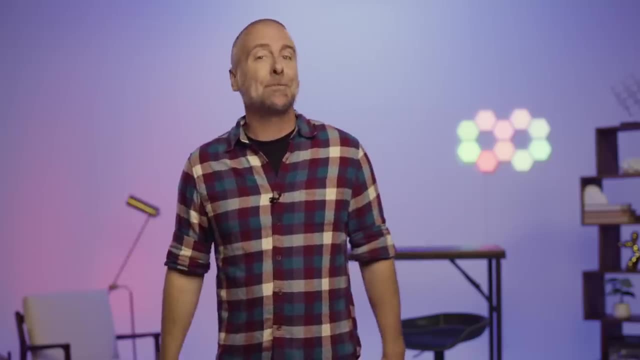 I know that I've gotten into some pretty bad viewing habits with all this streaming media. Now, while binging might be a great way to consume an entire season of your favorite show, it's not the best way to learn something new. Education isn't meant to be binged, And because 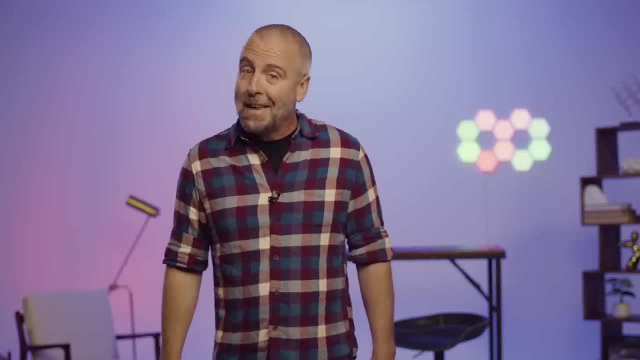 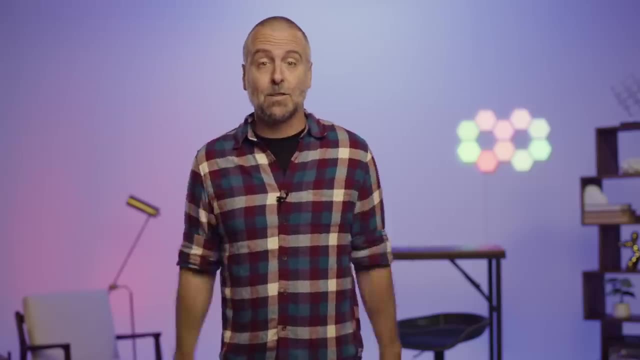 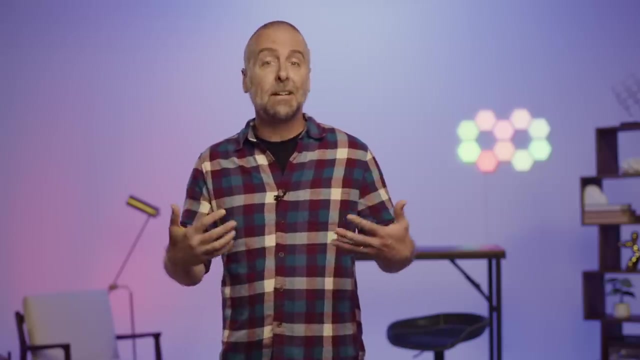 of this. I'll probably remind you quite a bit to take breaks and encourage you to let what you just learned marinate. All right, let's get to it. API: Those three little letters generate quite the buzz, don't they? First, I'd like to take some time up front here and clearly break down what is. 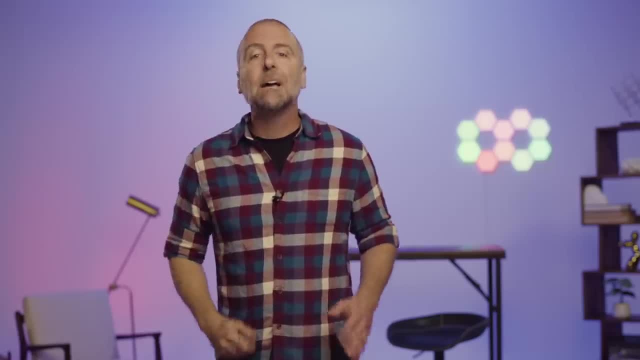 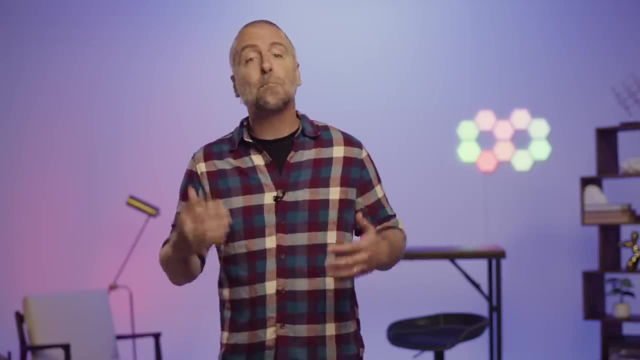 meant by application programming interface. By understanding its purpose and a touch of its history, I think you'll understand why it's important to use it. think you'll start to see its importance and begin to understand why this term keeps popping up in your life. After we get a good grasp on the what and the why of APIs, we'll go and learn how to 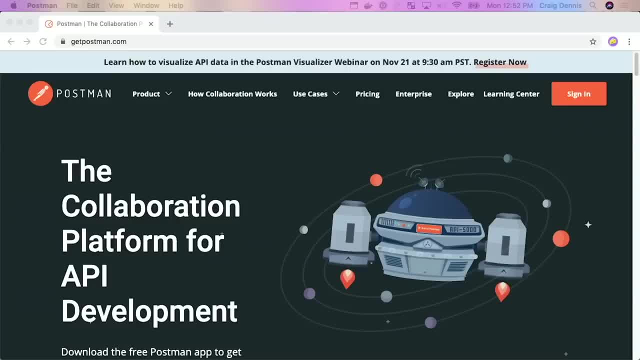 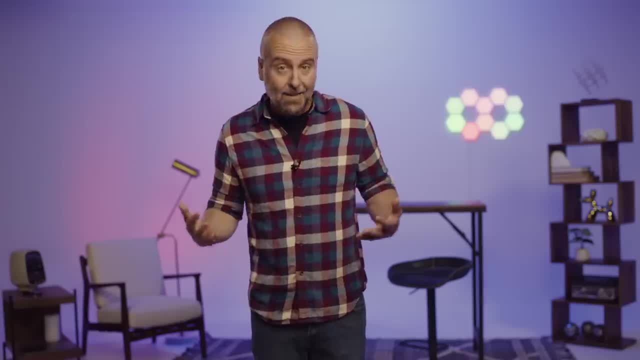 explore two existing ones. We'll get familiar with several handy tools that you can use to interact with web-based APIs. We'll use those tools to hit an external web API to send actual text messages, and we'll get some interesting data back from a streaming music service API Once we get some. 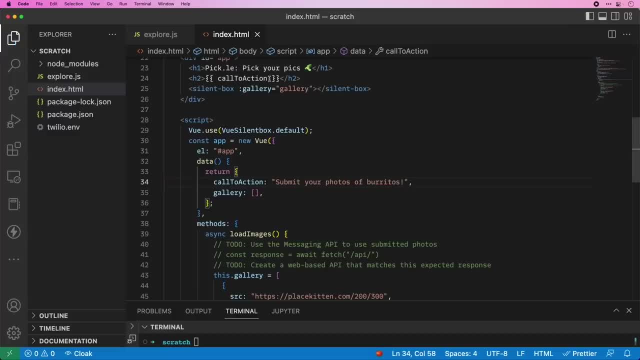 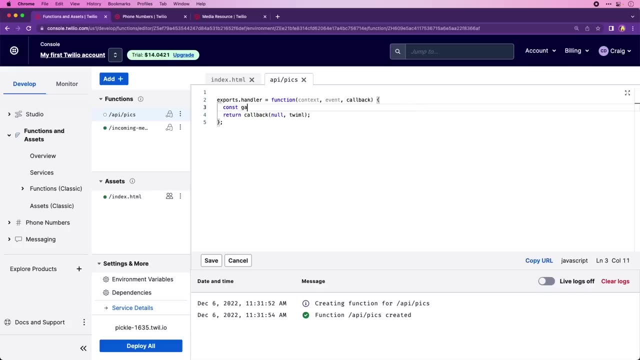 practice. using the APIs. we'll use them in a web application that you'll actually publish. The application that we're going to be building is going to receive user-submitted photos via a text message, and then we'll use an API to display a collection of all these photos And you get. 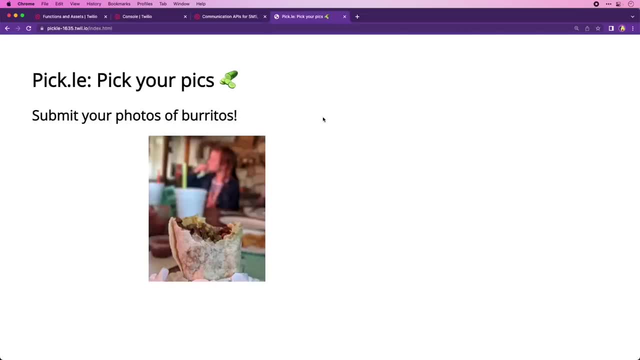 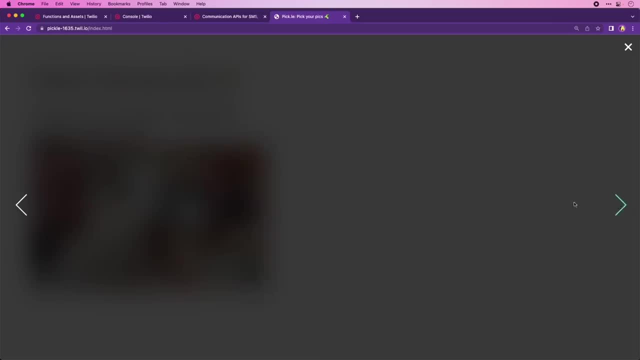 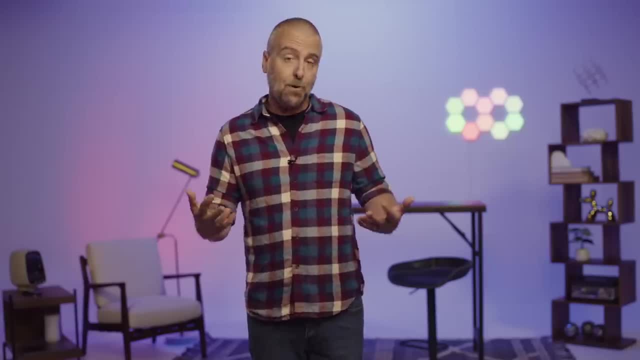 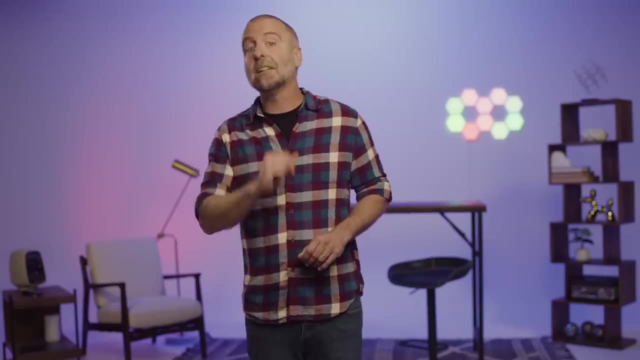 writing our own, While you most likely are going to end up learning some best practices in ABI design. we won't be covering that specifically. There are many great courses available that show the creation thought process, and I've linked to some of my faves in the notes attached to this. 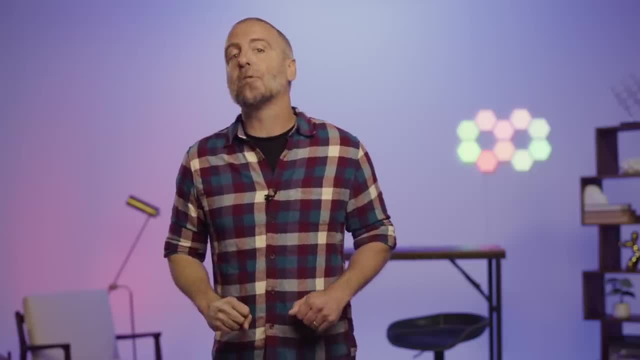 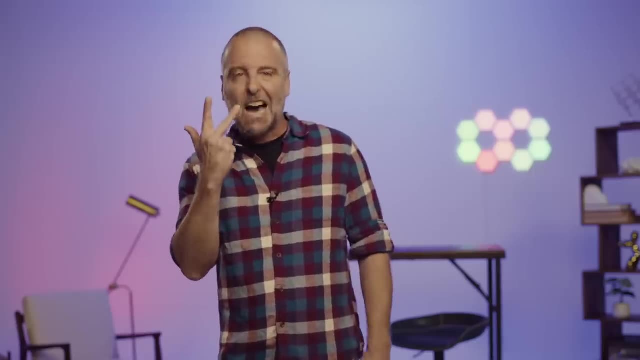 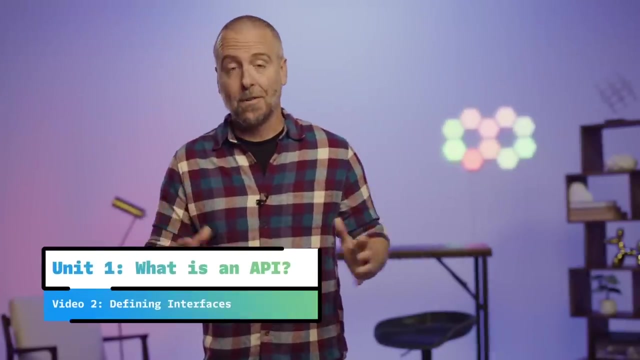 video. In my opinion, the best way to start learning about any acronym is to focus on each individual letter For A, P, I. I think we should start on that last character, the I- interface. Let's talk a bit about the interfaces that you've seen already. Interfaces are all around us. 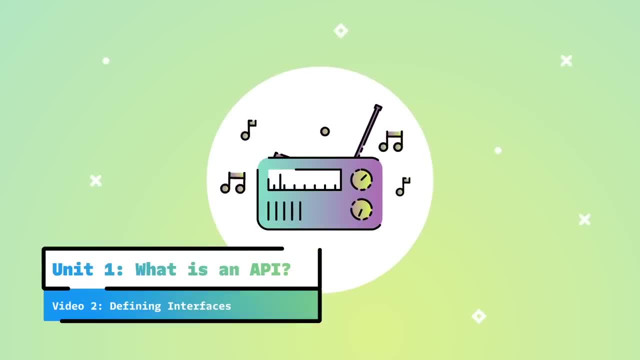 For instance, this radio. here it has a familiar interface. The interface allows me to do things like change the volume, change the station. I can turn it off and on. I literally have no idea how anything inside this thing works, But still the interface allows me to control the way that it. 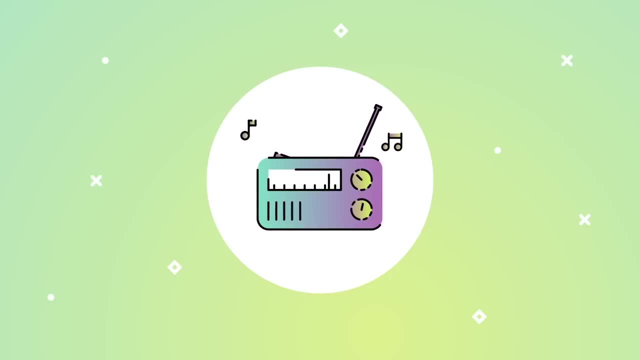 works through the options that are exposed, And that's pretty great, isn't it? The magic that is happening is completely abstracted away from me. I'm still in control of what has been determined that I, a user, can handle. Interfaces usually evolve over time. 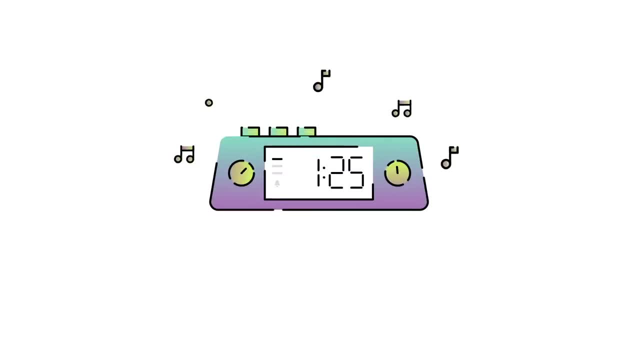 Like an alarm clock radio, for example. It has my familiar volume and station controls, and it also adds some new features like changing the time and setting the alarm. I still have no idea how this works implementation-wise, but the interface is something that I can understand Usually. 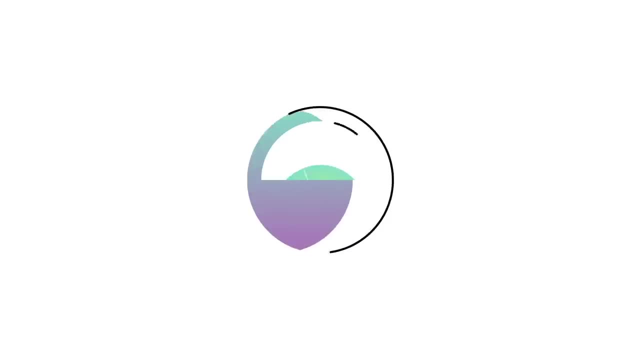 And as technology evolves and new options come into existence, they make their way into the new versions of the interface, still abstracting away things for us, but enabling us to be in control of the new features. Sometimes these physical interfaces get so recognizable they even make it into GUIs. 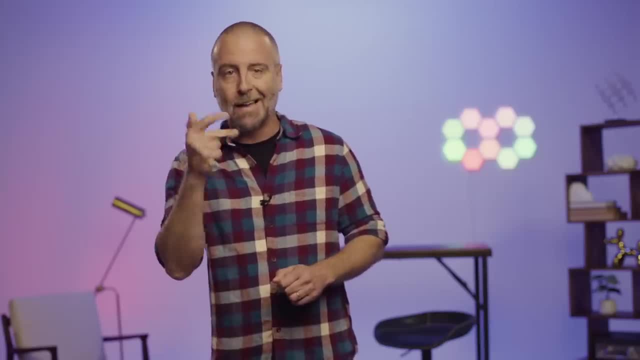 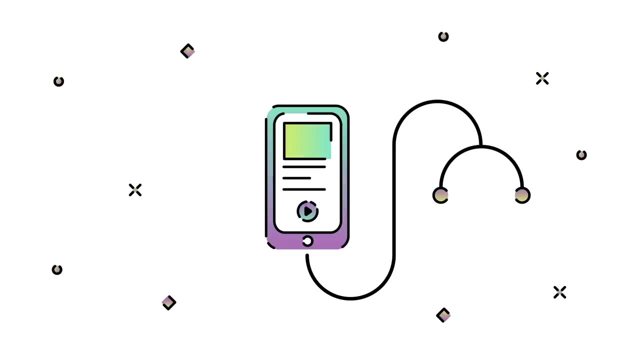 Hey, did you hear that? There it is again GUI G-U-I Graphical User Interface. This is my streaming music app on my phone. There's my familiar play button in the user interface or UI, And I know what the play button does when I press it. but I have 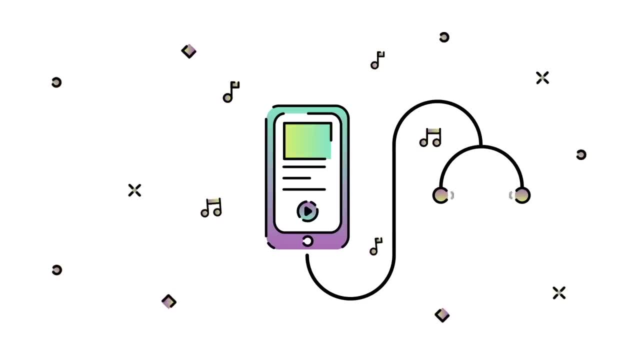 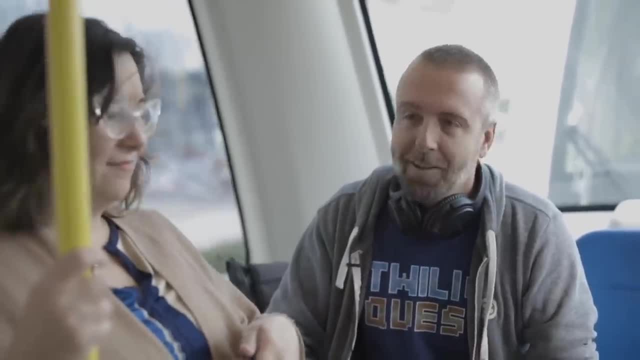 no idea how it does it, And I'm okay with that level of abstraction. What would I do in public transit without music, Like talk to people: Hi, How's it going Now? the developer who wrote this streaming music application of course understands how. 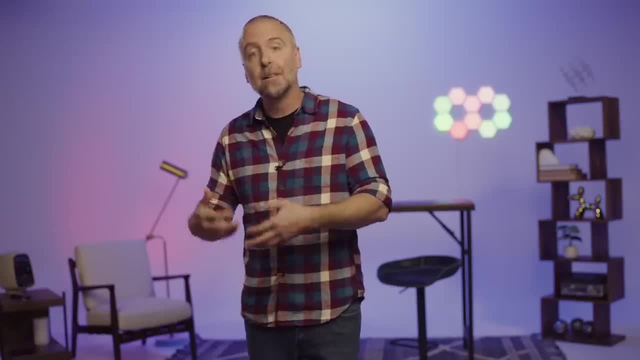 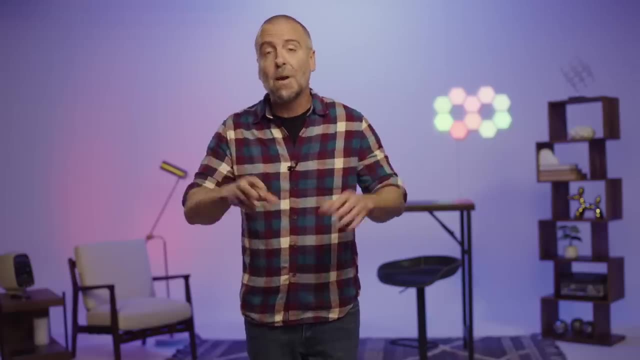 the play button works. She coded the button so that, when it gets clicked, the music starts playing. Here's the thing, though. Our developer is also working with quite a few interfaces that are abstracting away some of the details for her, For instance, she wrote code that happens when the 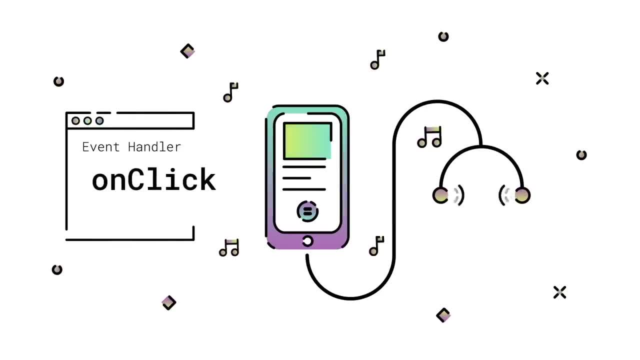 button is clicked. She probably did that using an event handler on the button, like onClick. What she didn't have to do, however, was write the code that makes the button interact and change with the press. She didn't have to write the code that makes that familiar clicking noise. 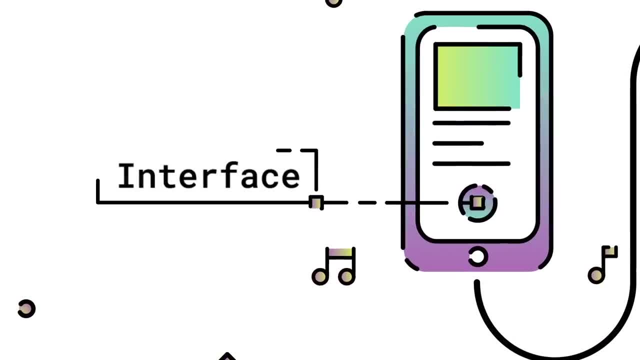 It was already there for her. Buttons are, in fact, an interface. They provide the developer the means of controlling its interactions while abstracting away how that actually works implementation-wise. This button is part of the API or Application Programming Interface, and 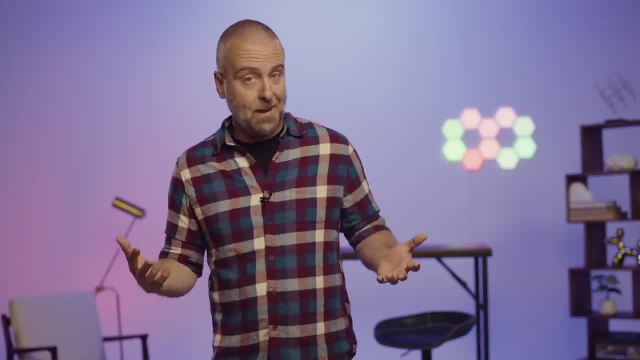 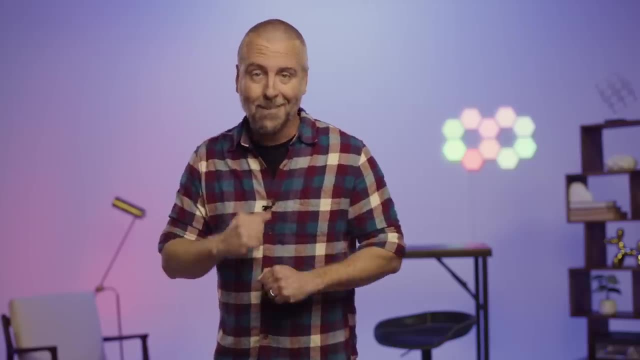 it's available from the application framework that was used to create the app. Because most apps need buttons, this interface has been used to control the app's interactions. This interface has been created and provided to our developer or Application Programmer to use By implementing. 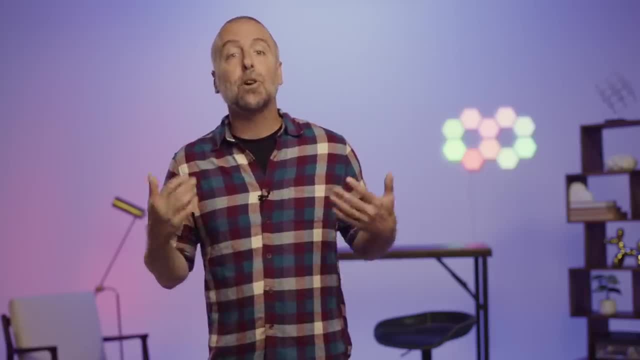 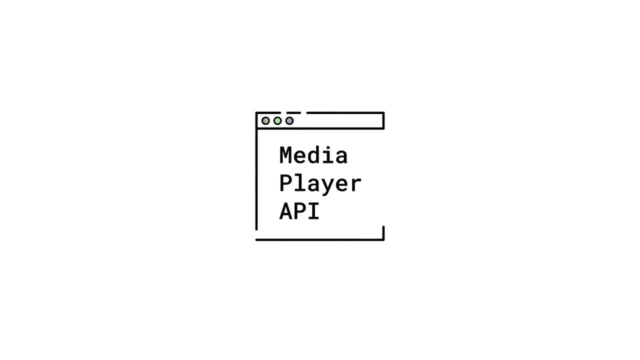 the button interface. our developer was able to make her code run when the button was clicked. It's worth noting that the code probably also uses a MediaPlayer API that is provided with the operating system of the device, like Android or iOS. This MediaPlayer API abstracts away, needing 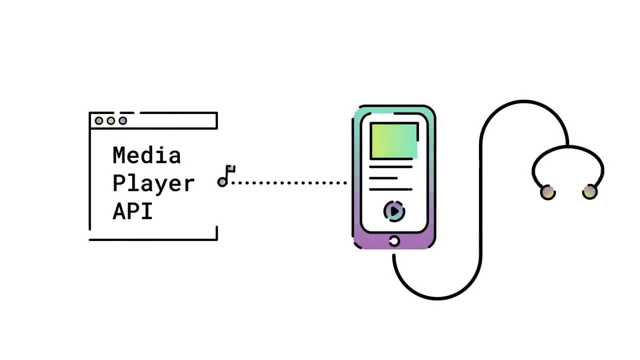 to understand details of how to send audio data to hardware. The developer knows they just want to call the play method on the MediaPlayer API. They just can't take the audio data they're making on a media player API. I suppose too, the song isn't stored on the device, It's being streamed over. 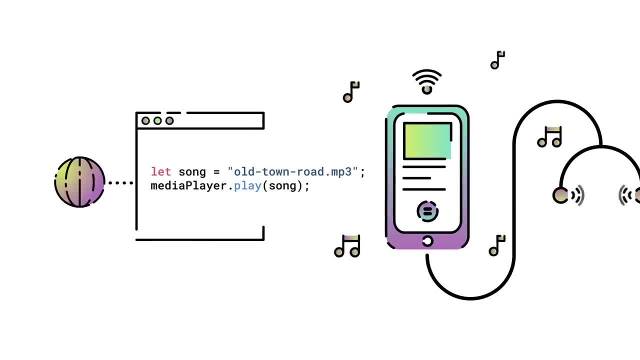 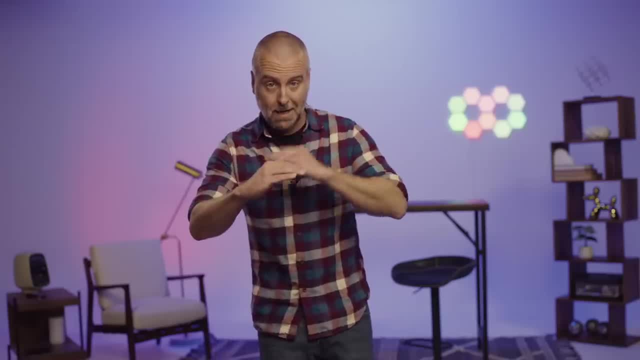 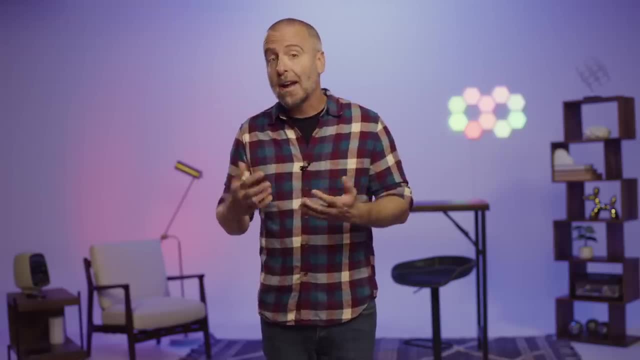 the network, So a web-based API call has been made over the internet to get that data. It's actually APIs all the way down to the ones and zeros preventing abstractions at many levels. So let's take a look at what all of these interfaces have in common: They all define ways for us to interact. 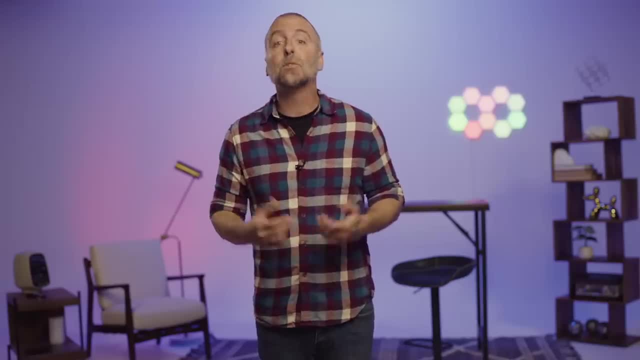 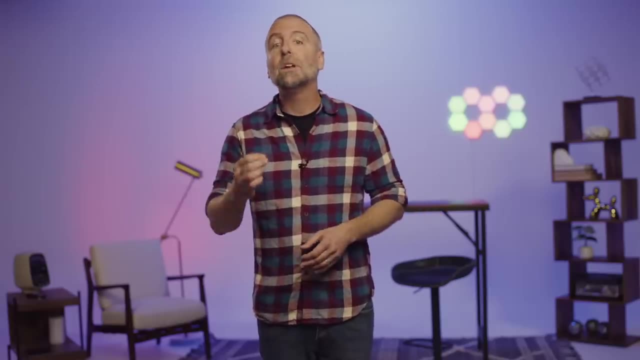 or communicate with an object, whether that object be physical or software, And as a user of the interface, we don't need to understand the implementation, We don't need to know how it works. We just need to know what we've been allowed to change or see Interfaces abstract away the 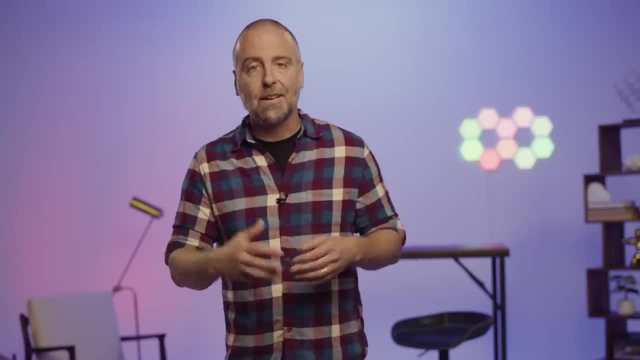 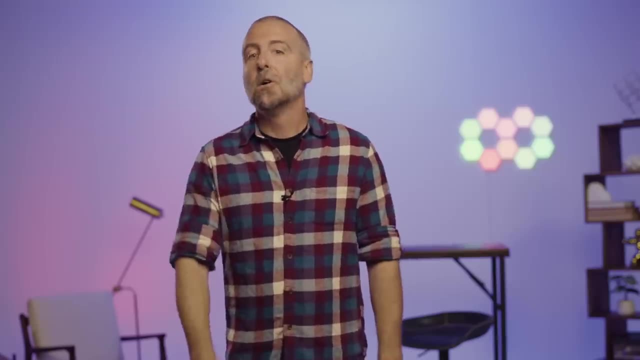 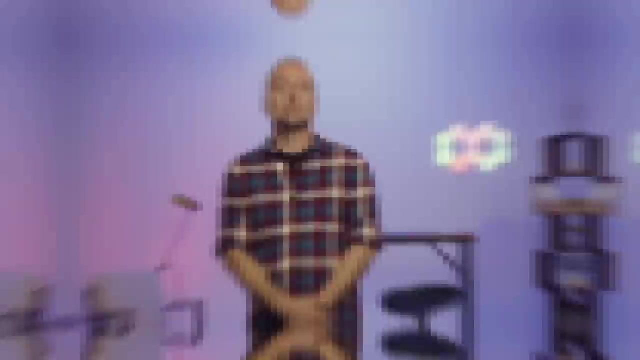 implementation. Now, while the UI or user interface is made for the user of the application, the API is made for the application programmer to use and extend in their applications. With the I covered in our API, let's take a deeper look at the rest of the API acronym. An API is a contract. 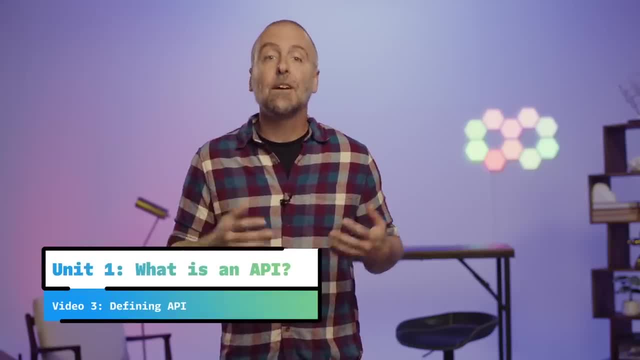 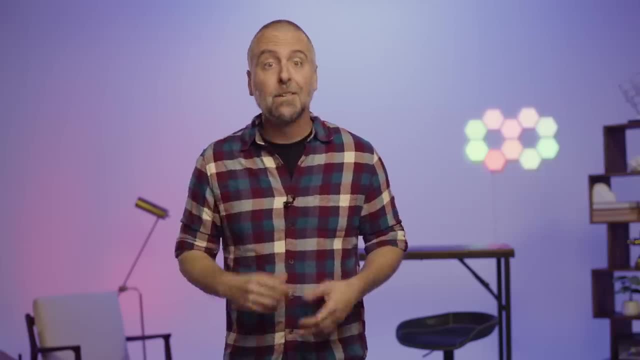 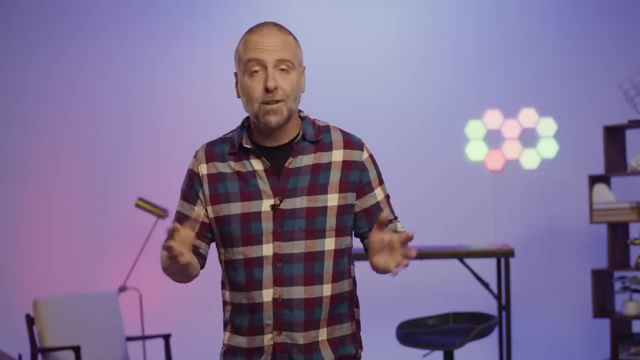 It defines how it is expected to be used and it defines what you can expect to receive by using it. Think of it as a set of tools designed for software developers like yourself to use. An API is created to help make your life easier by giving you access to data and by providing you with an abstraction. 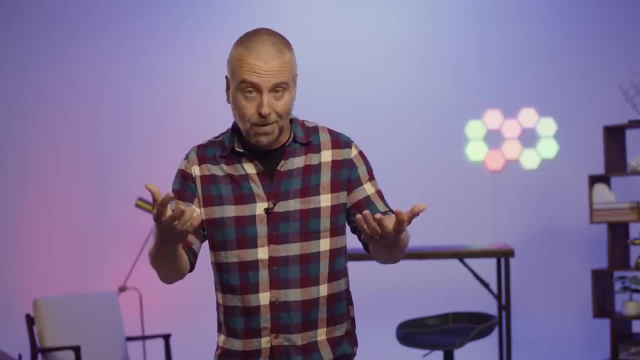 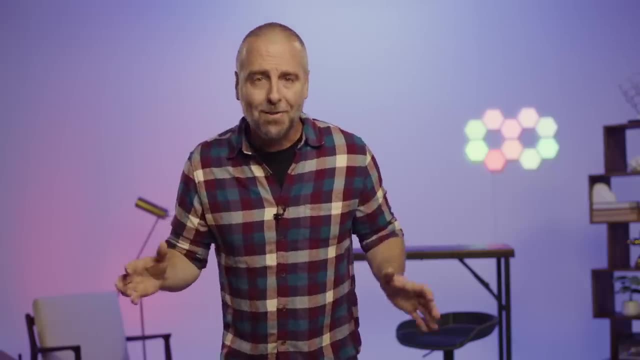 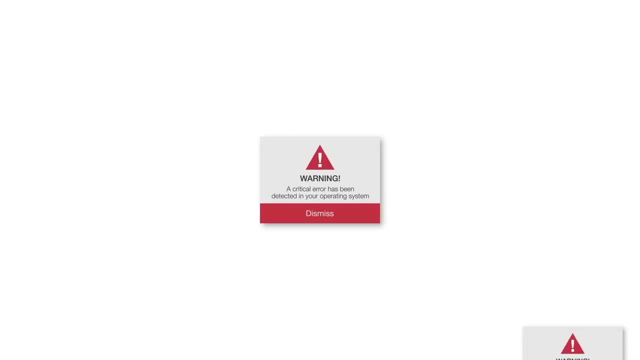 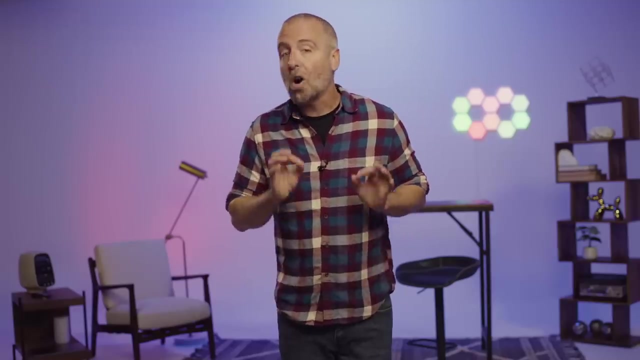 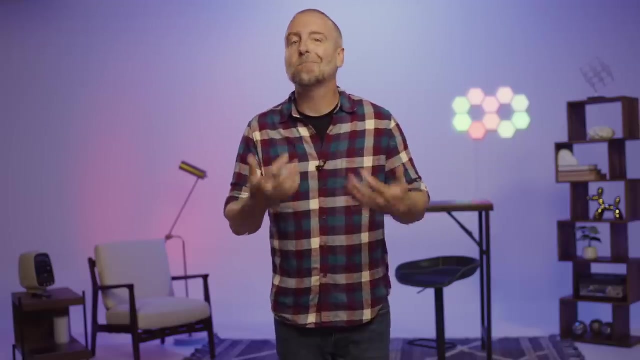 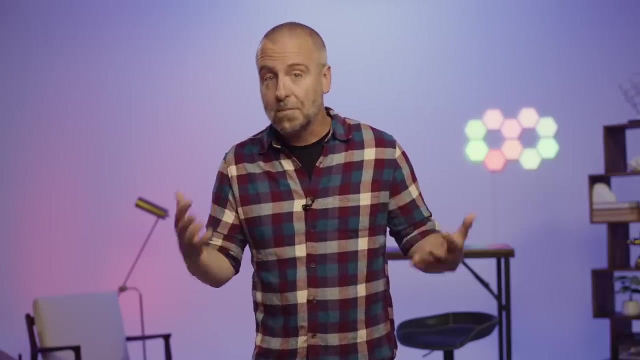 of the implementation. You know, not needing to know how it's doing whatever it's doing. They save you from needing to create everything yourself, Like when designed well, they make nearly impossible things happen with just a few lines of code. Now you're probably starting to see why it's important to get familiar with them, right? I want to do a quick word of warning here about some naming issues that you'll probably run into. These days, the term API is almost always used as a way to explain web-based APIs. In fact, it's probably safe to assume that when you hear API in the wild, it's most likely that people are talking about a web-based API. We'll explore those here in a few. However, if we focus on all types of APIs instead of just the web-based subset, we'll get a better look into why web-based APIs are so important. 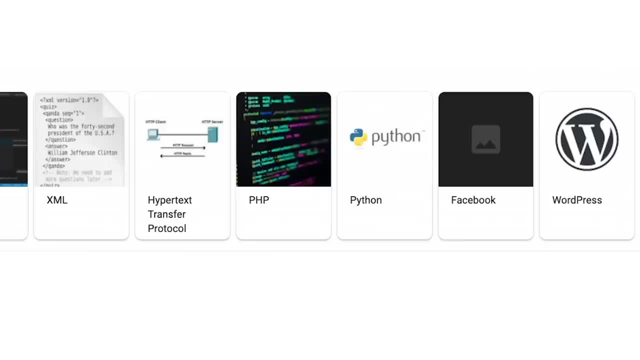 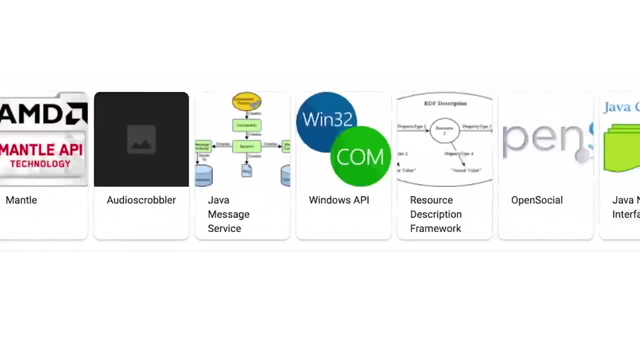 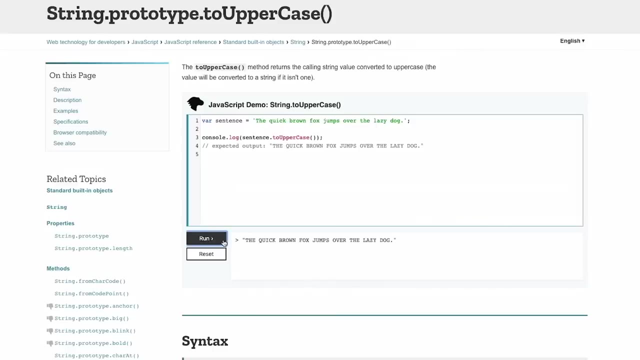 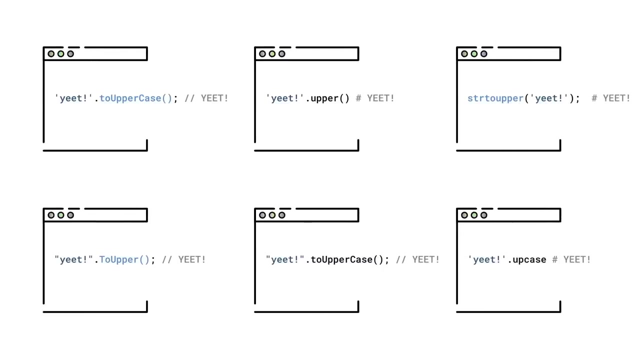 web-based APIs are so popular. So hang tight, we're getting there. APIs are everywhere in your software journey, just about everywhere you look. Your programming language, whichever one that might be, provides many APIs. Let's take a look at one that is common in all of them. They all provide some way of working with strings. you know, like a series of characters Want to make your text all uppercase, Just call the API method and voila, You could probably create the uppercase string all by yourself by doing some sort of low-level bit math on each character. 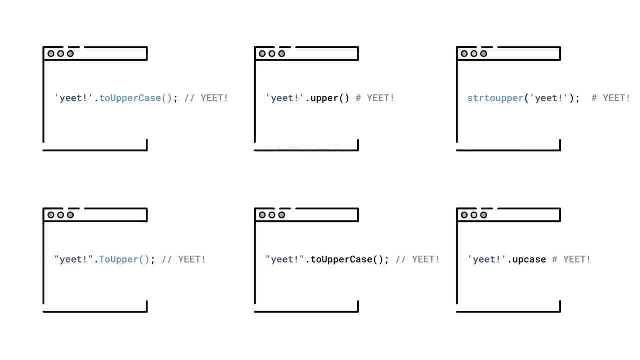 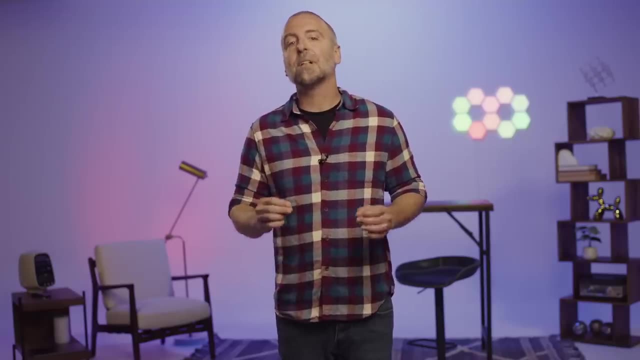 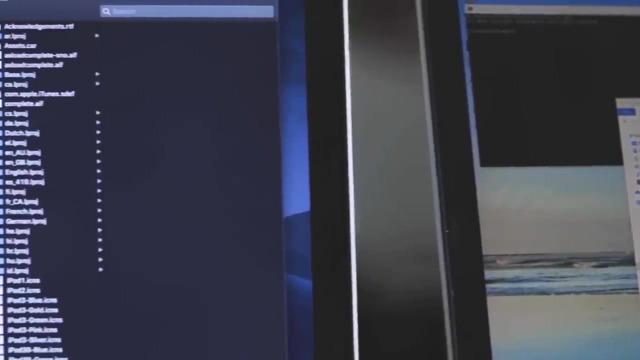 But you don't need to because your programming language has abstracted away that for you and provided a handy string API. It exists because this is a common enough problem that developers run into, Because these programming language specifications are just interfaces. different operating systems can supply their own implementation so that the code works properly in their environment. I think an easy way of picturing this is to think about how different operating systems like Windows or Mac OS maintain their files. They're totally different. 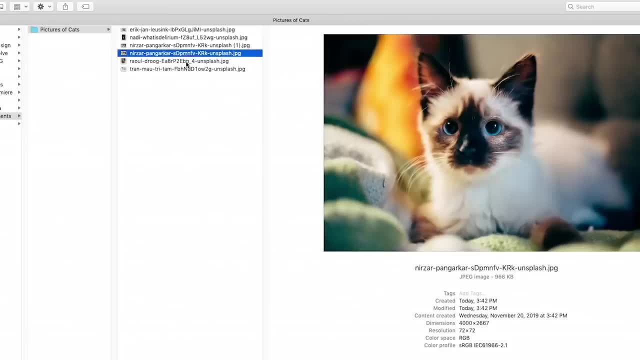 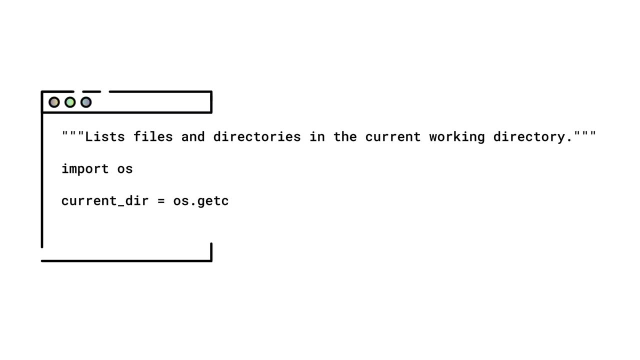 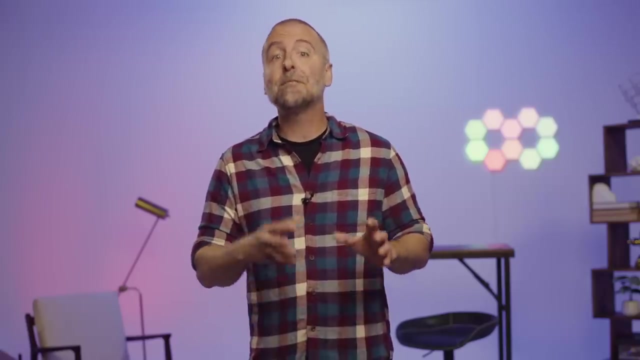 Yet your programming language provides a single API for working with the file system. You can write one script and it works both in Mac and Windows. It's the implementation that takes care of all of the details for you. Pretty cool, right. Definitely something to be thankful for. It makes our lives so much easier not having to worry about what operating system is being used, And the importance of an API to a language cannot be understated. There have been some fascinating legal cases where it's been questioned if the language API itself- again, not the implementation, but the code itself- can be used. 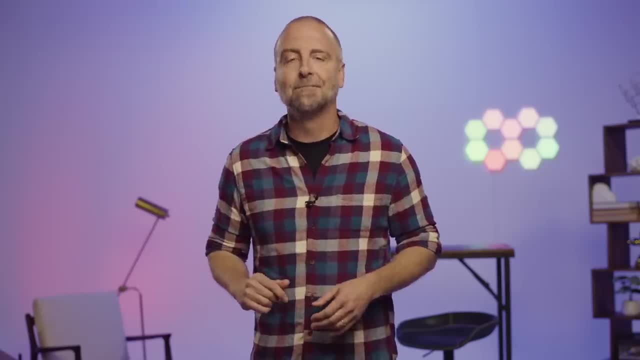 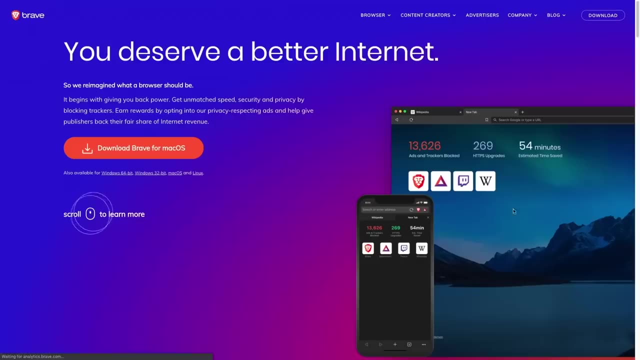 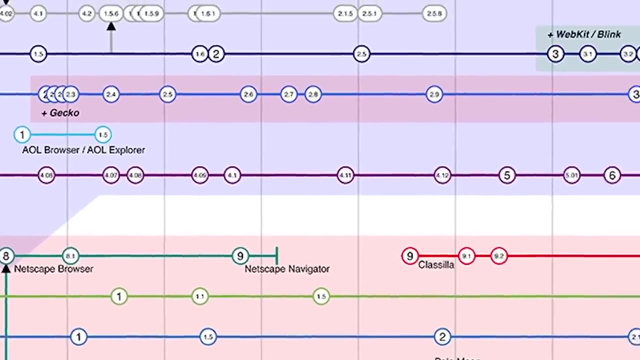 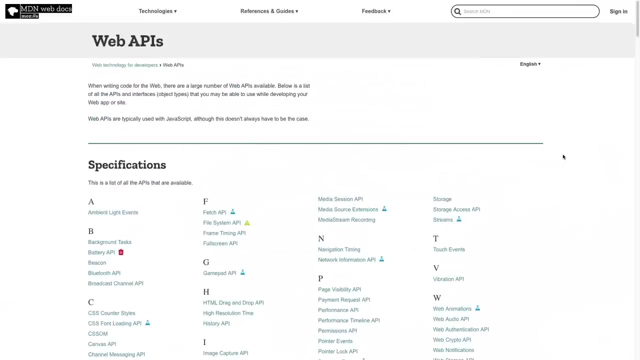 The implementation can be copyrighted. Check out the notes for more on that. Along similar lines, there are different web browsers, you know, like Google Chrome, Microsoft Edge, Safari, Firefox. Brave, Now, you might not have pondered this before, but isn't it amazing that you can write code for the web and it will work in any of them? This works because there's a set of web APIs that web browsers all must implement in order to make that magic happen for you. We're standing on the shoulders of giants, folks, and we really should thank those giants more often. 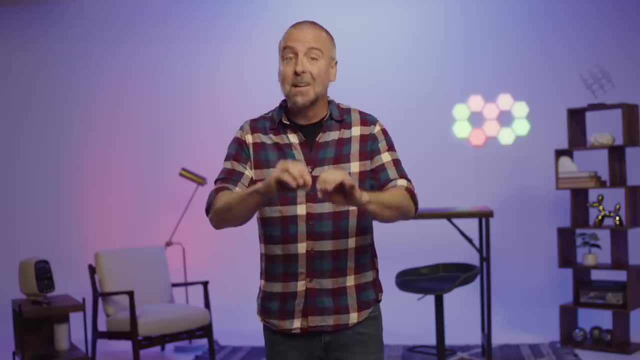 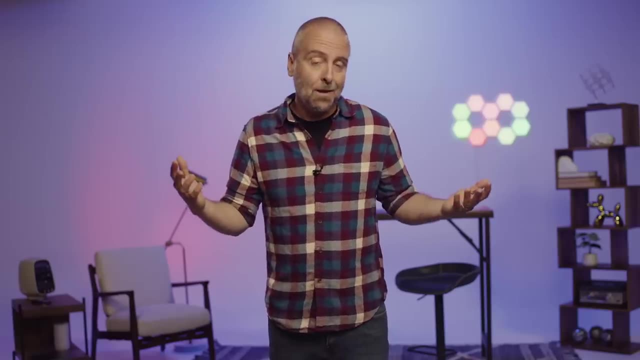 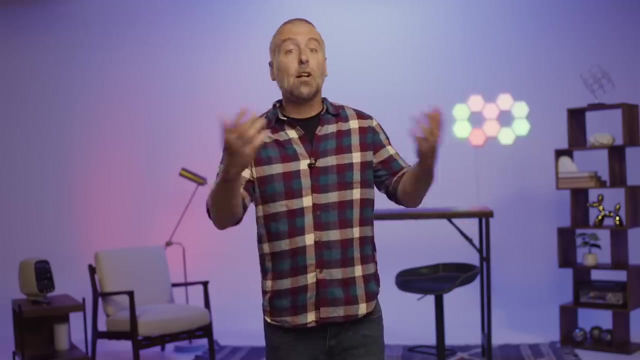 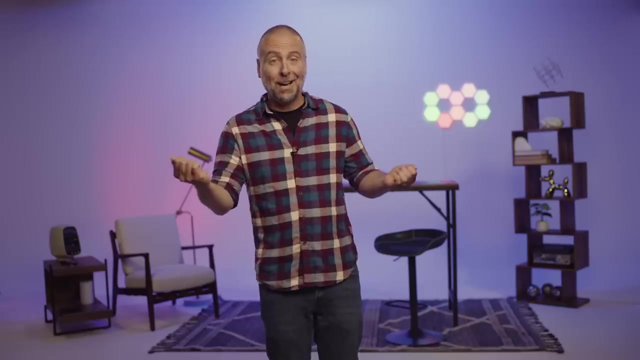 Thank you Authors and maintainers of libraries that package up code to solve common problems so that you don't need to do it yourself. For instance, do you know how to programmatically make a photo black and white? Me neither, but I can download and import an image package into my application and suddenly I can. I just call a method and boom. I wish real life skills worked this way. I'd import dancing so it could be more fun at weddings. Cha-cha-cha. 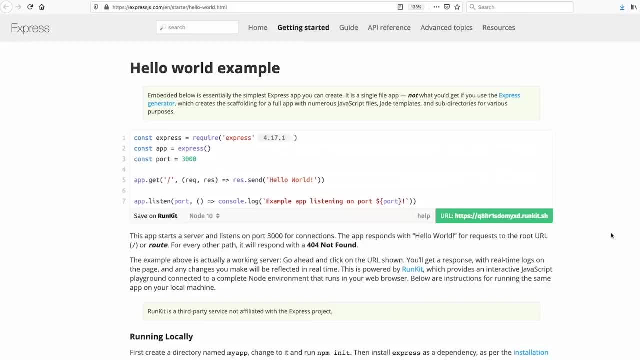 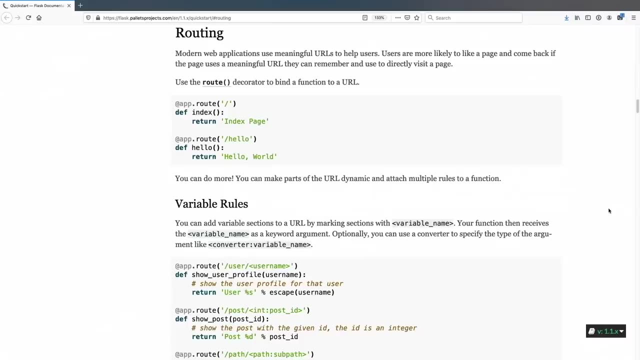 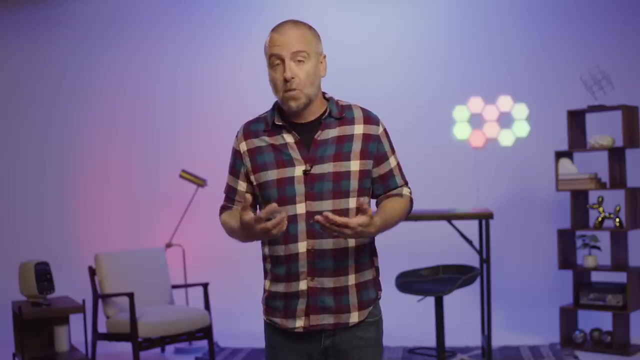 Frameworks provide an API that allow you to extend what has been provided to make it your own Like, for example, most web frameworks provide you with the ability to add a new route to your web application. It allows you to write out dynamic data to a template that you specify, And you do all of this with just a handful of lines of code. You don't need to understand how it's doing things, but you do need to know how to write an implementation to what the framework is expecting. In this case, you're using the API, the contract- to write a valid implementation. 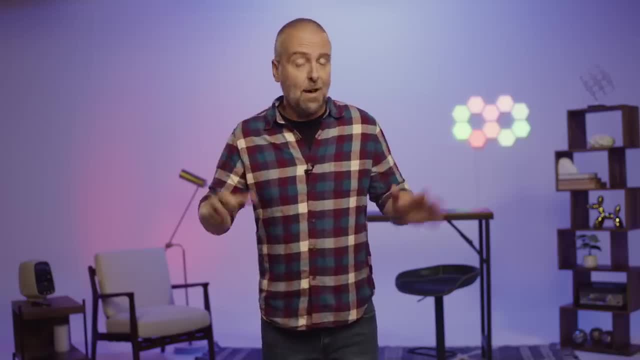 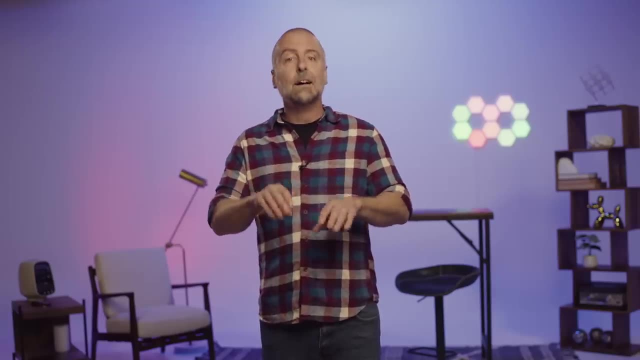 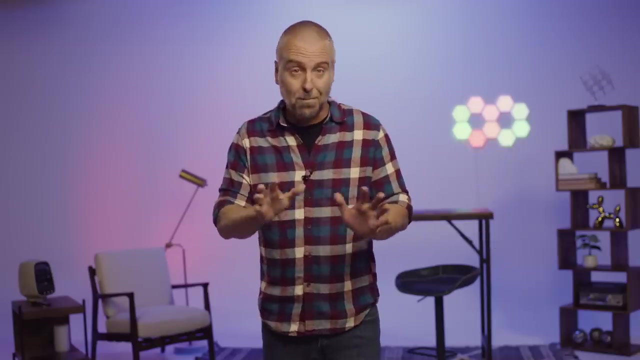 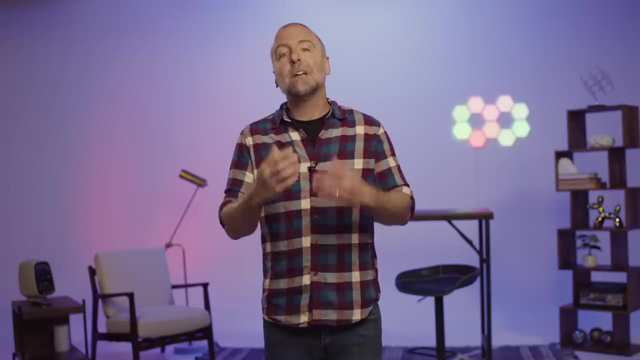 That meets the requirement. Now, all these APIs that we just talked about: they're local to our code base. They exist within our code. We use them to avoid recreating the wheel, That is to say, they assist us in accomplishing tasks that we need to perform by abstracting away a ton of the work for us, The stuff that we developers shouldn't be worrying about. We should be focusing on the business problem at hand, And that means a big part of your job is figuring out how to leverage these APIs to your advantage. Now, I think this is an excellent time for you to take a break. 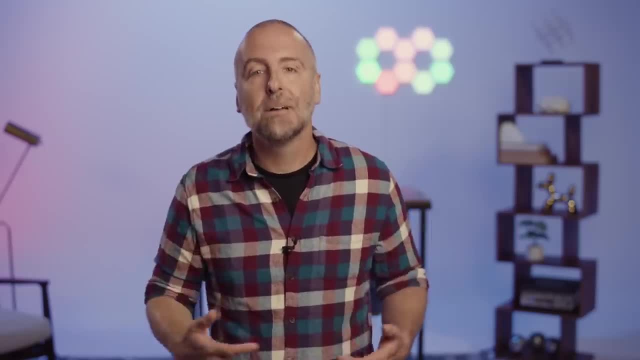 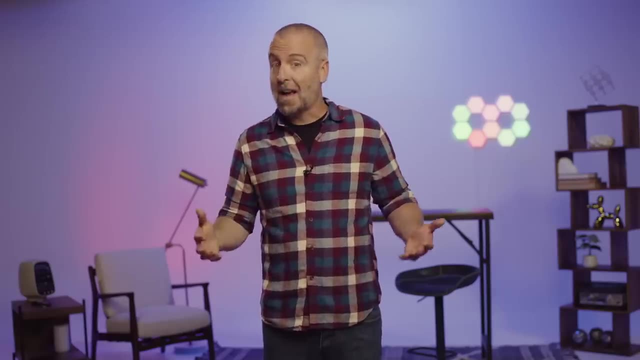 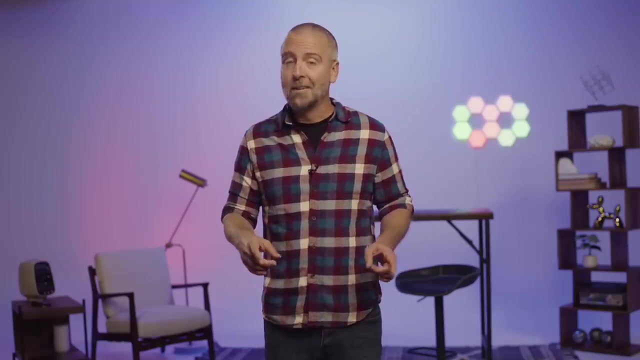 I just gave you a lot to think about, and I'd like you to take some time and breathe. Why don't you jot down some APIs that you've used today, Even if you weren't coding? I know that you've seen some in action. If you're having a hard time thinking of some, I'll give you a hint. You're watching a video right now inside of a web browser. 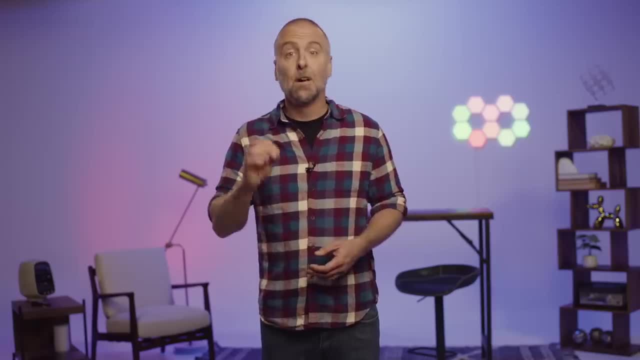 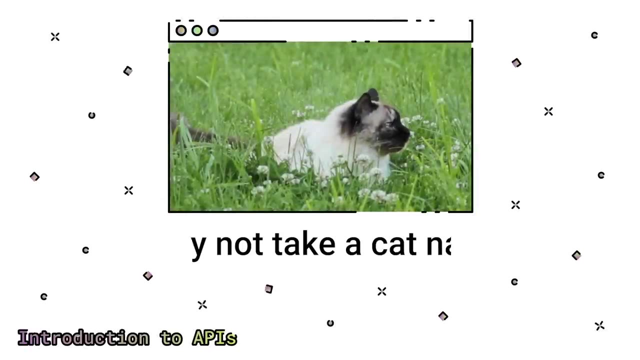 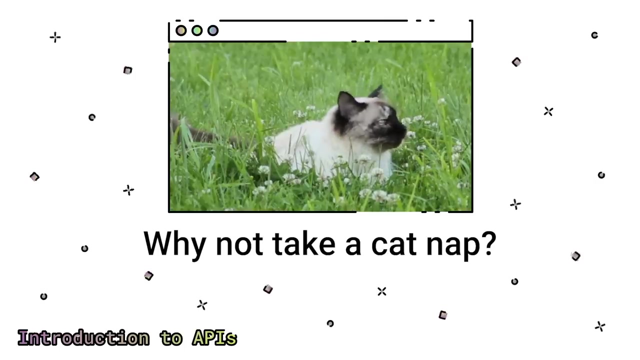 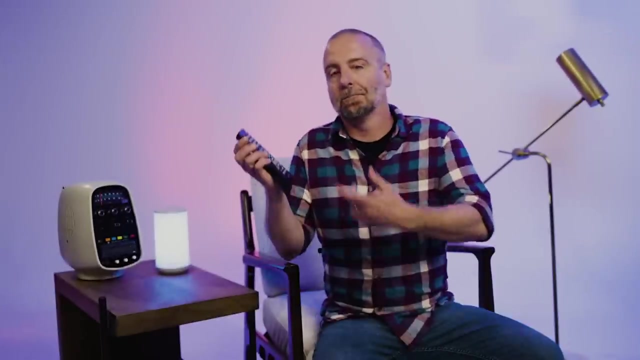 When we return, we'll explore the concept of remote APIs, ones that aren't executing locally in our code base, and why that is such a powerful concept. It took me a while to find this remote control. It was in the couch. It's always in the couch. 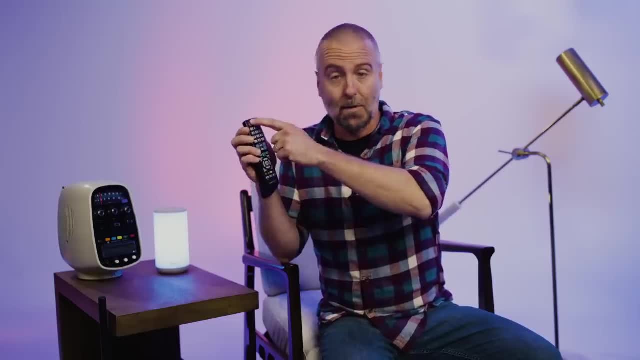 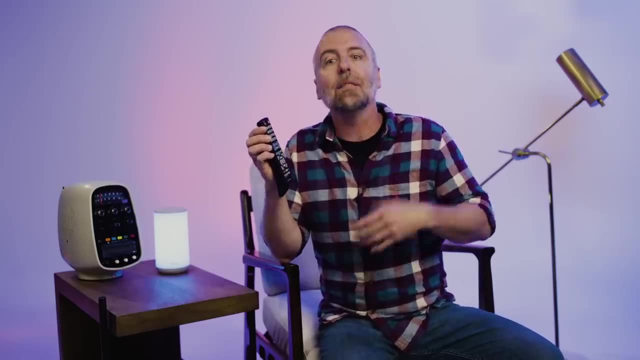 Anyways, this remote has an interface. on it right There's a power button And when I press the channel button it changes the channel. And when I press the volume button it sends the request to my radio And the volume changes, as if I turn the volume up using the interface on the device itself. 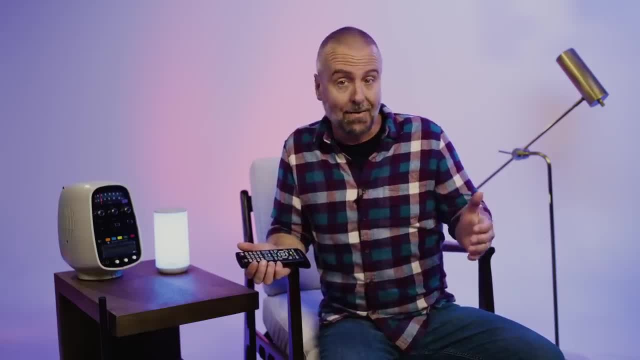 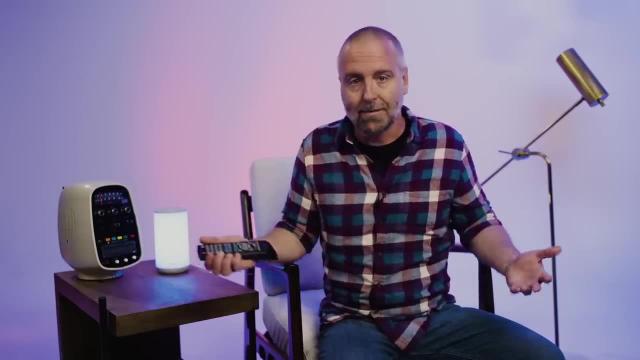 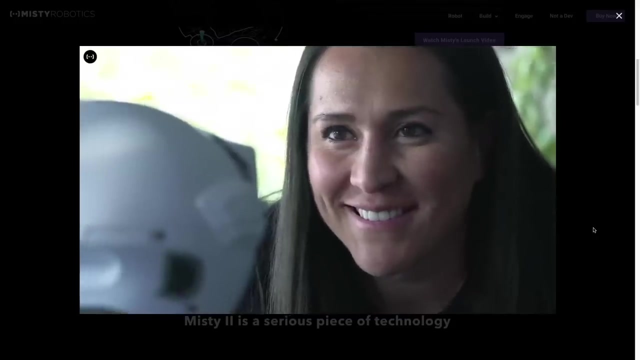 And we know why that's important. I want to remotely control my device. I don't want to get up from my chair. There are, of course, more, less lazy reasons as to why we'd want to remotely control objects. This cute little robot, for instance, has a remote API. You can send commands to it and it responds, and it even sends back sensor information. 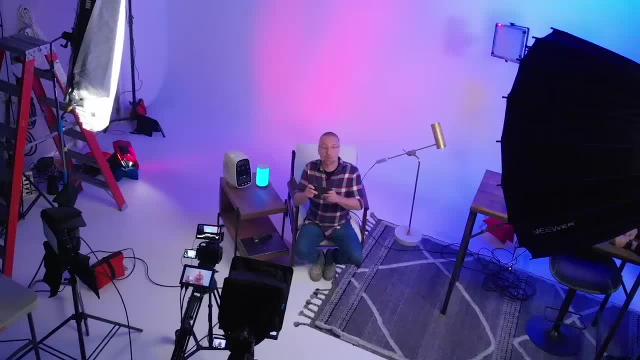 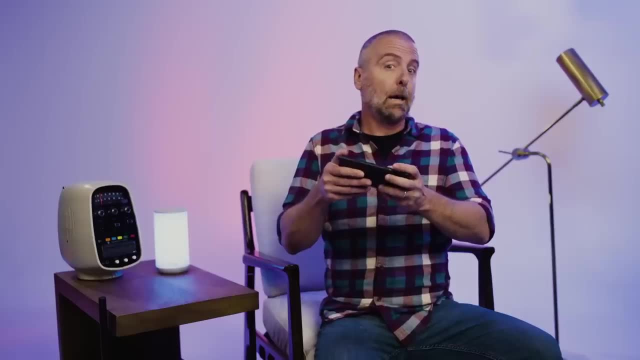 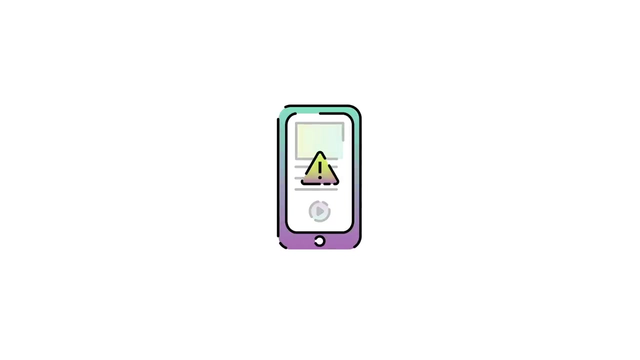 These traffic signs can change based on an API call. This drone here is remotely controlled by an app on my phone, See. And it's not just physical objects that benefit from remote APIs. Oftentimes we don't have space on our local machines for all the data that's available. 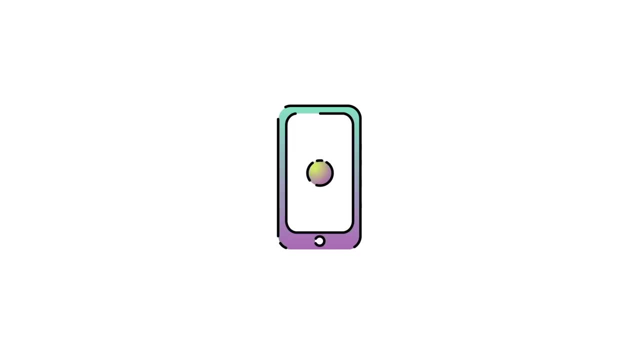 Like. for example, have you ever used one of those apps that helps you figure out what song is playing? You send up a snippet of a song that you heard playing at a grocery store using your microphone and it sends back exactly what song it is. 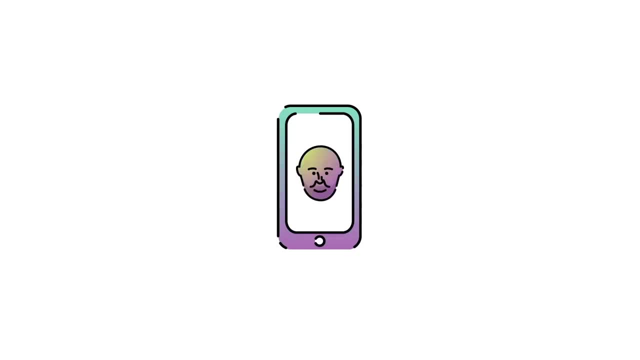 It's usually Phil Collins. It turns out that both grocery stores and yours truly love Phil Collins. You don't have rules. You have room for all the songs in the world on your phone and with this remote API, you don't need to have all of them. 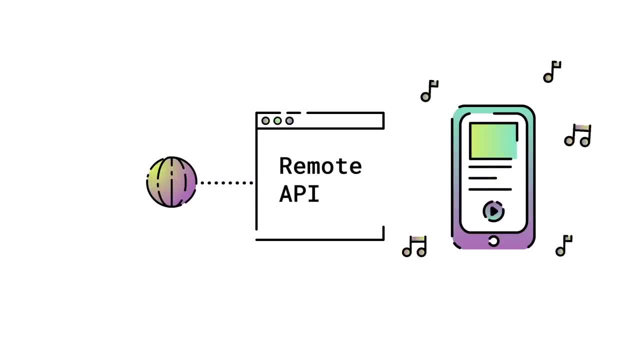 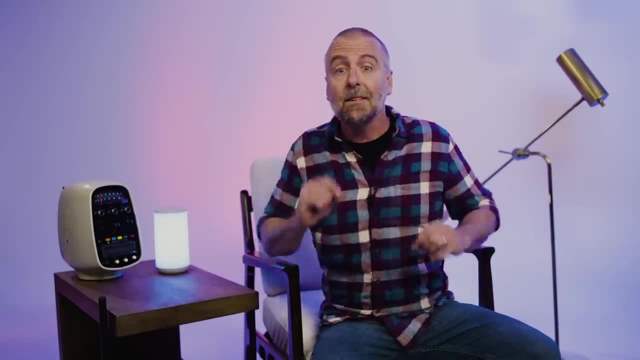 It does all the searching and processing and it's surprisingly quick. How can it possibly do that? I don't know, but I love the interface. It's so fast. Ooh, that's another benefit of remote APIs. Computational power. Because an API removes the limitations of your local device, you can gain access to seemingly infinite amounts of power. A good example of this is the AR app of Google Translate. You can use the camera on your phone and in near real time it's able to translate directly to your screen, like instantaneously. 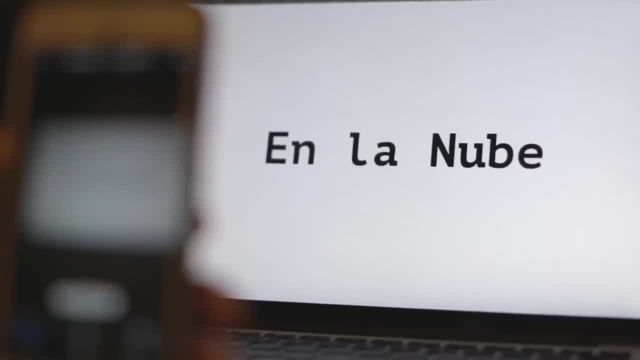 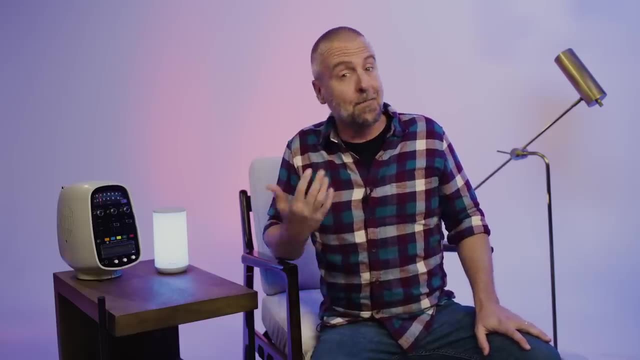 It's using a ton of processing power to make that magic happen. and that processing is happening elsewhere in la nube. It took quite a bit of experimentation and some evolution of ideas, but over time we finally turned this remote API dream into a reality. 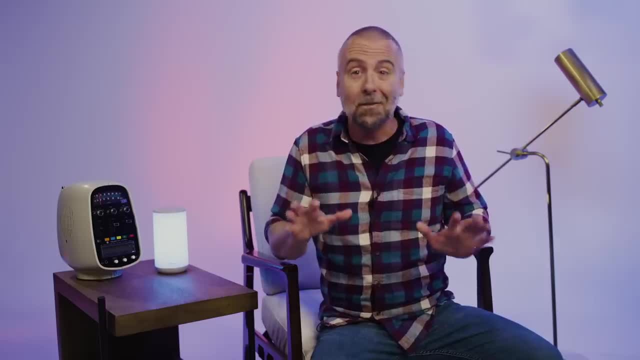 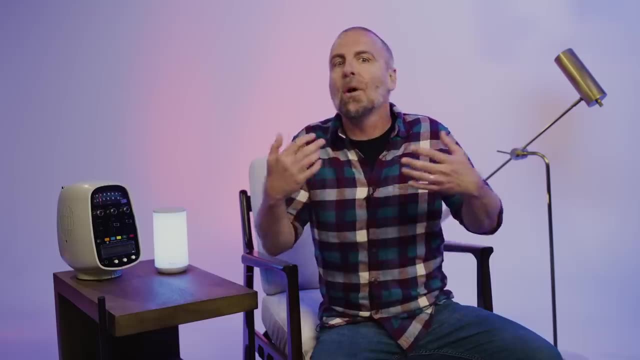 Now I'm going to drop some history into the teacher's notes, but I just want you to know that the struggle to achieve this concept of remote API is a lot of work. The idea of remote APIs was very real. Now, most of the problem was that there wasn't a standard that everyone loved. Things were pretty clunky for a while as these ideas were sussed out, but then it happened. A new architectural style appeared that was clear and allowed us developers to interact with specific resources over the web, and it quite literally changed everything. This style rapidly emerged as a winner, and just about everyone began offering and consuming external APIs over the internet. 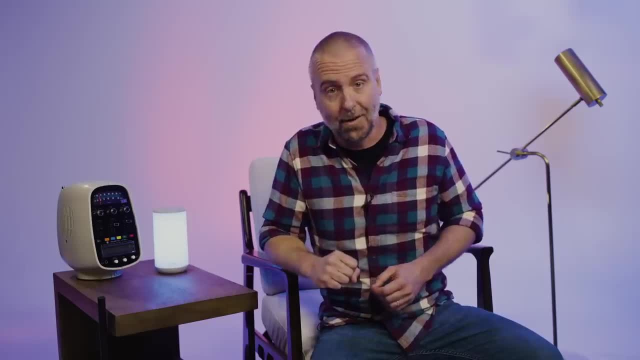 Now, what I'm talking about is the idea of remote APIs. The idea of remote APIs is a little bit different than the idea of remote APIs. The idea of remote APIs is a little bit different than the idea of remote APIs. What I'm talking about here is REST, or Representational State Transfer. 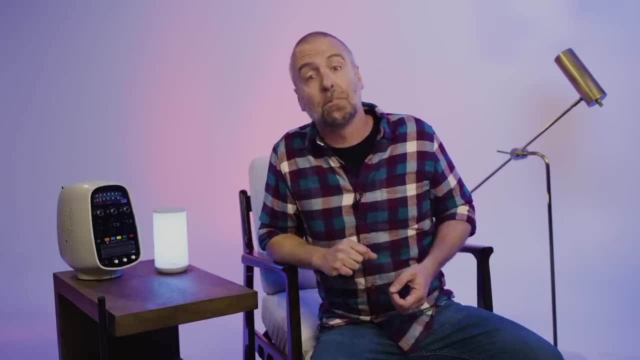 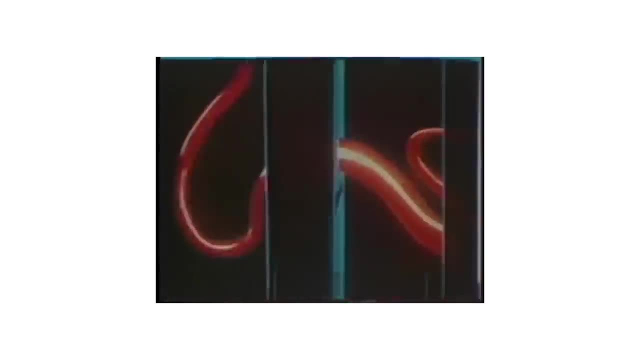 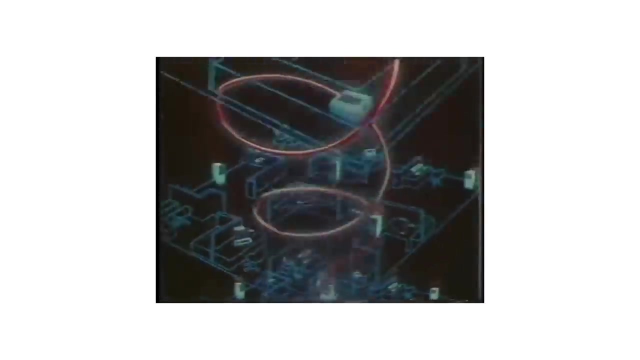 It was the approach that we needed and, honestly, it's the abstraction that we developers deserve. Like we talked about already, the popularity of REST spread so rapidly that it nearly completely overtook the term API. It's like how we use the word Xerox to mean photocopy, even though Xerox is just a brand of photocopier. 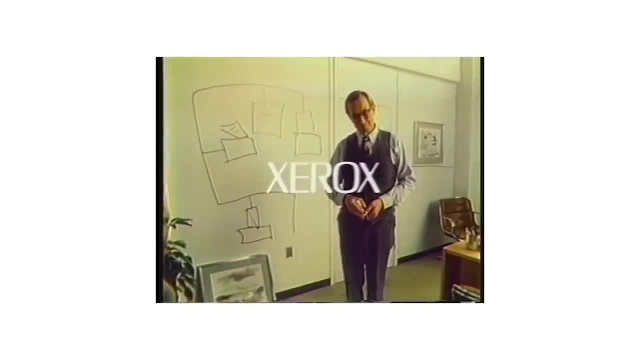 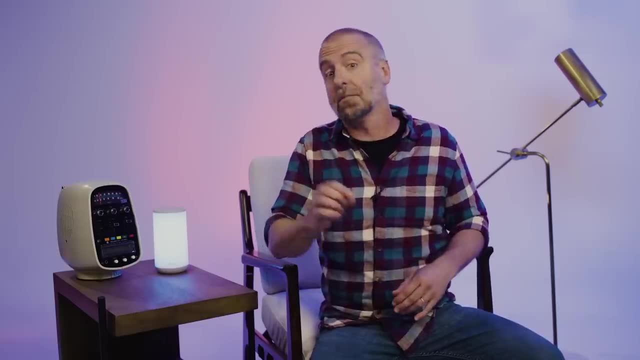 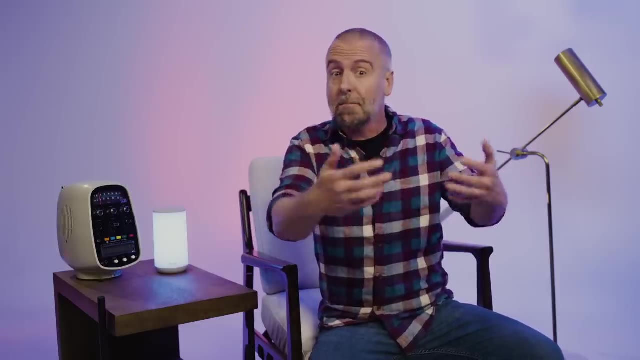 Xerox does other stuff too. I think That's how pervasive REST is. REST is for sure not the end-all be-all. There are definitely some limitations, which we'll discuss here in a bit. Technology is ever-evolving and of course there's movements that are still advancing the concept of the best remote APIs. 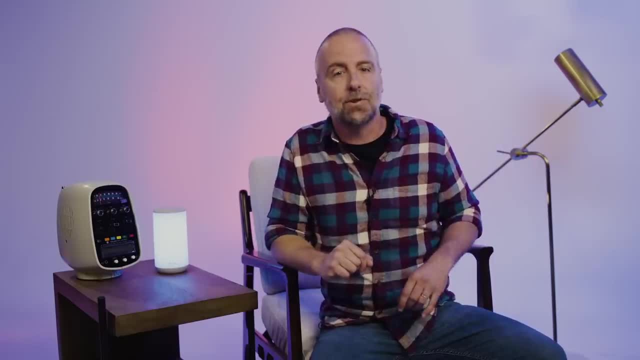 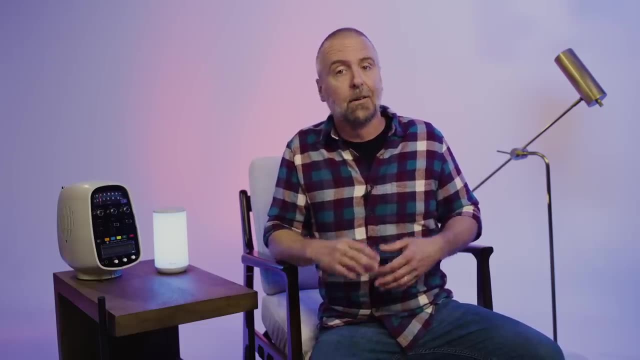 Some terms you might even have heard, like GraphQL. More on this in the teacher's notes. Now for the rest of this course, we are going to do a deep dive into APIs that are written using the REST style. When APIs embrace the style and constraints of REST, they are said to be RESTful. 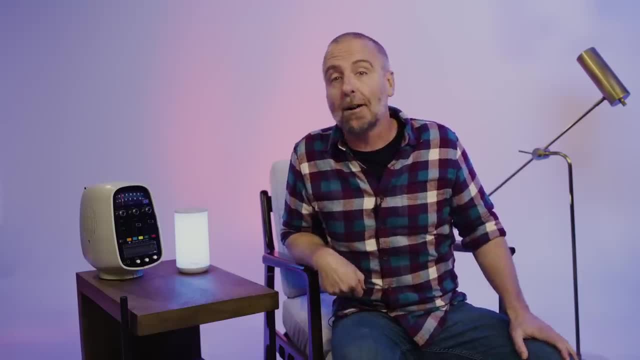 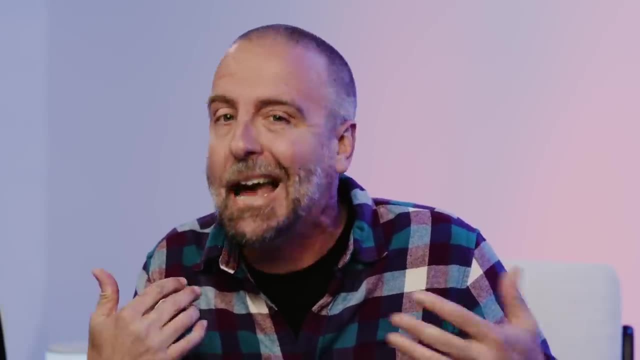 Cute right. If you feel like you need a little REST, go ahead and pop. Pause me before we do a deeper dive into what it means to be RESTful. Sorry, that was a bad and obvious joke, but as a developer you kind of have to make it. You don't really have an option, Because REST sits on top of web technologies like a really nice hat. we should probably do a whirlwind refresher of how the web works. It might have been a while since you thought about how the web works. 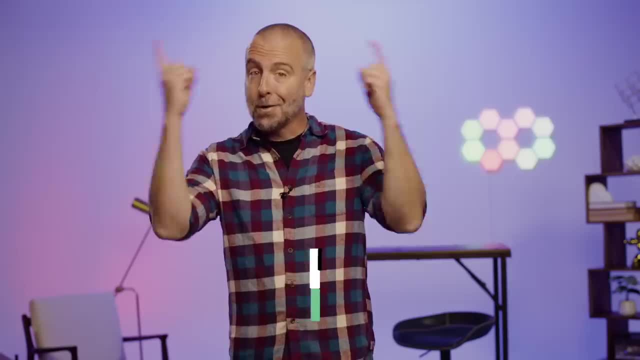 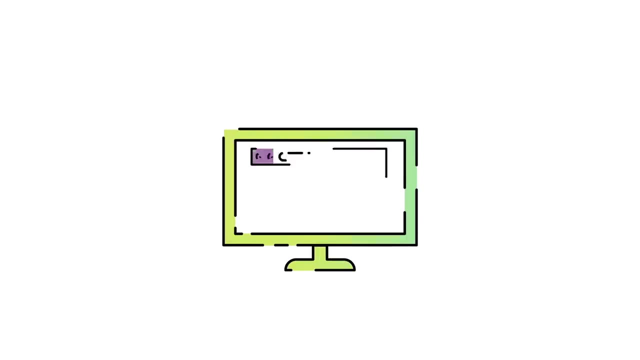 There are a smattering of terms that I'd like to reload into your working memory before we talk more about how REST uses them. So let's use the web. I've got my computer here and on. it is an internet browser. The browser is a web client and I'm going to use it to connect to a server. 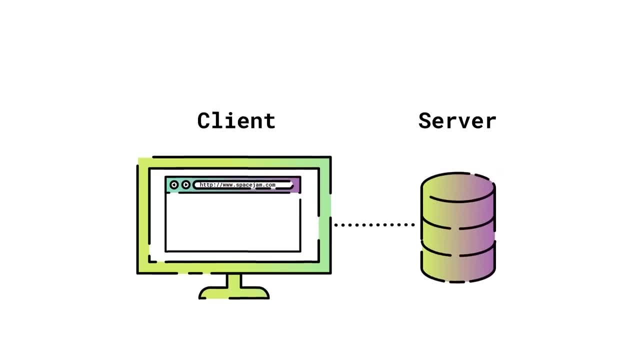 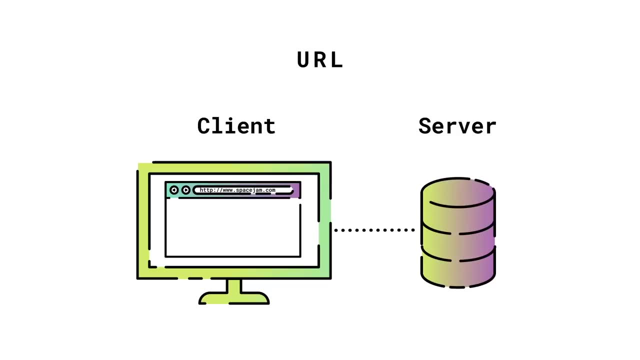 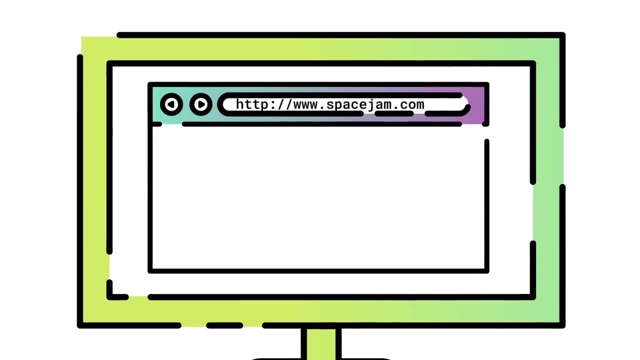 I'm going to do this by putting a location in the address bar: A user Universal Resource Locator, or URL to be exact. You might also hear this referred to by its superset term, URI: Universal Resource Identifier. Now, our URL here has a scheme portion, and this one happens to be HTTP. 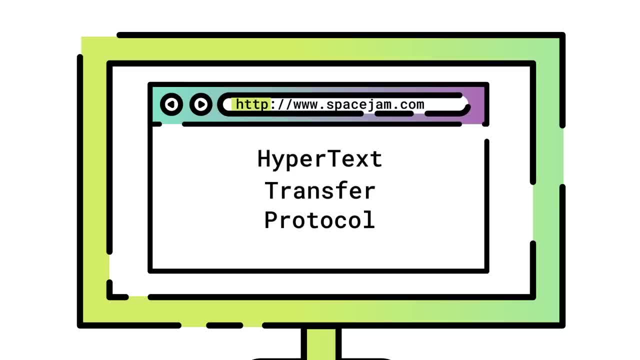 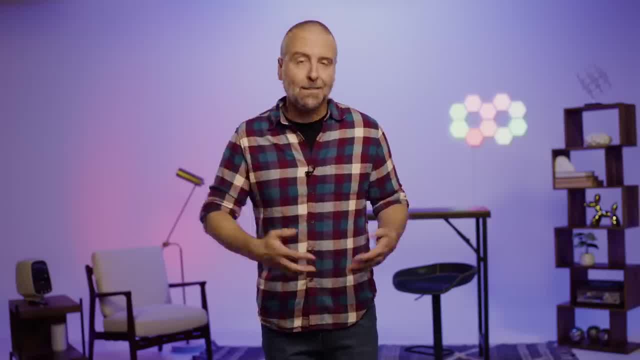 HTTP stands for Hypertext Transfer Protocol. Let's break that down a bit. Let's grab that last part: protocol. A protocol is also often likened to a contract. It's a little lower level than an API, but it's similar in concept. 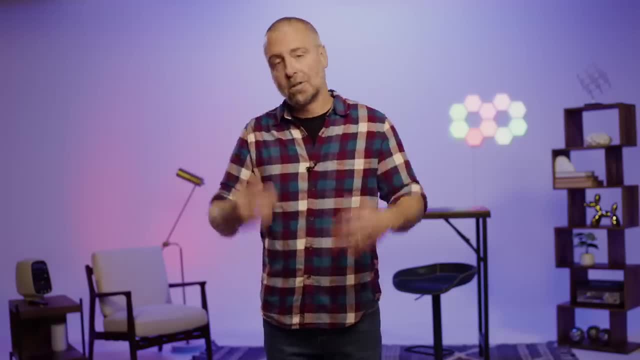 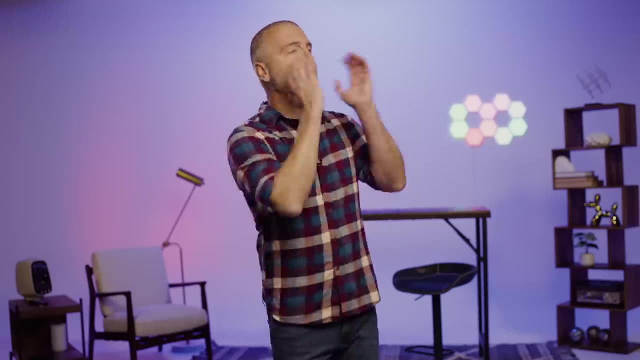 You can think of it as defining the expectations of how to communicate, Like an example that I think really sticks with me is if you've ever been to a rally and someone does one of those chants where they're like, When I say foo, you say bar. 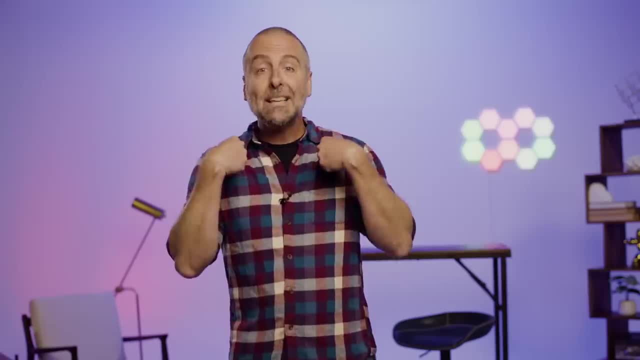 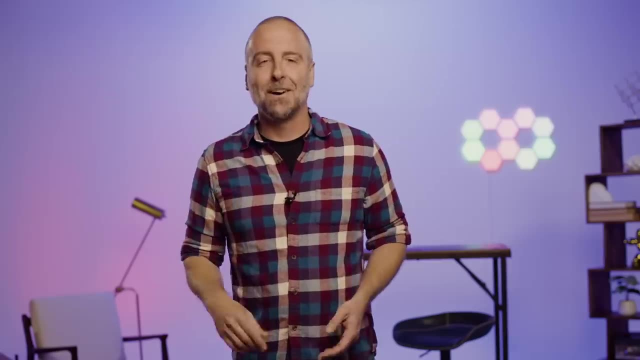 Foo Bar, One of those Here. let's do one. When I say HTT, you say P, HTT, HTT. Oh, I just realized I might have made you yell P out loud. Hope you aren't in a coffee shop. 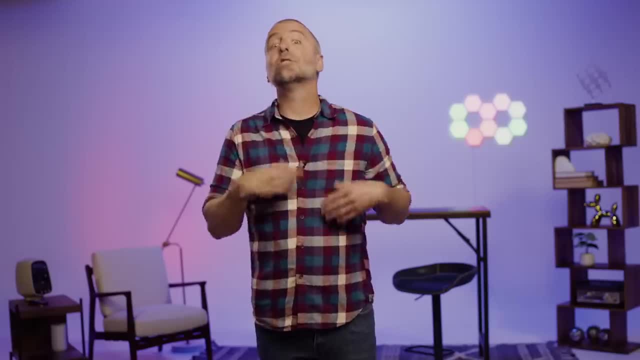 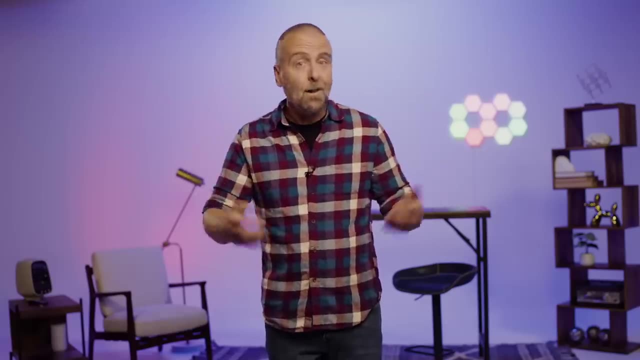 Awkward Anyways. We- You and I- Just set up a real quick protocol. I told you how to respond to my specific request and you would have been breaking our agreed-upon protocol if you yelled anything else but P. 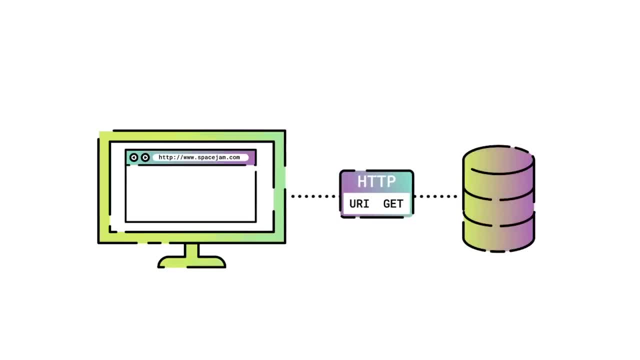 So the browser creates an HTTP request for you. Along with the URI, it also specifies a particular HTTP verb. In this case, it is using the GET verb, which is used to clarify that this request will only receive data, That is, it won't be making any changes. 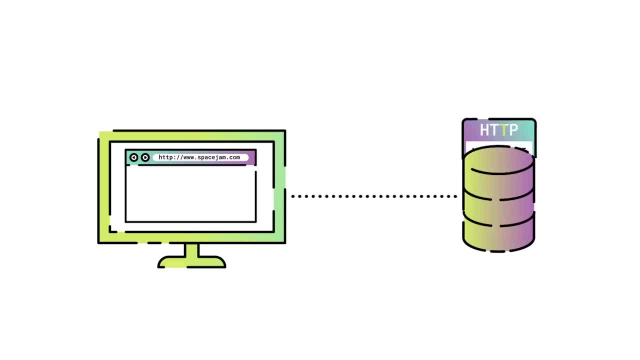 The server receives the request That was transferred From the client. There's that second T. The server then does the work that it needs to do. Finally, it generates the resulting web page and sends back a response to the client- My browser in this case. 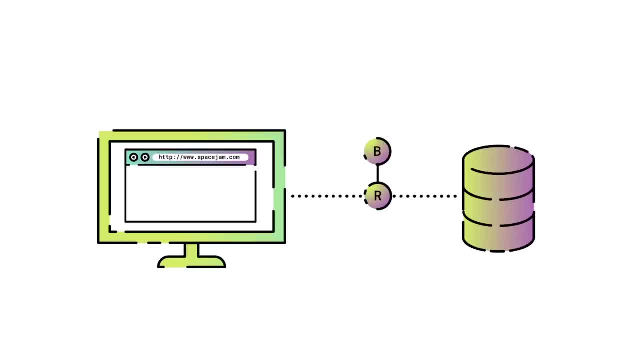 The most important part of the response is the body For a web page that contains the HTML Hyper Text Markup Language, Which gives us the remaining parts. The HT of our acronym, Hyper Text, is text that can link to other text In HTML. we perform that linking with anchor tags. 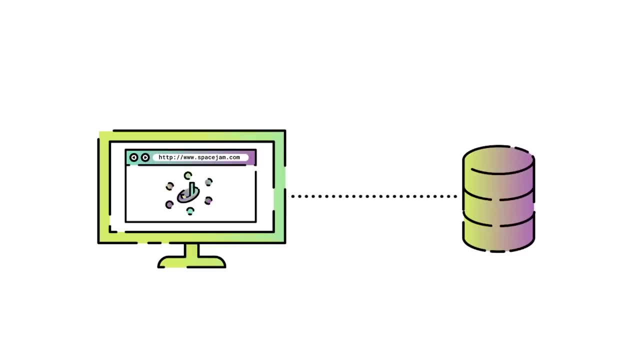 So with that response, the browser renders the picture. So with that response, the browser renders the picture. That's the page. When one of those links are clicked, they kick off a brand new HTTP GET request and the process repeats itself. 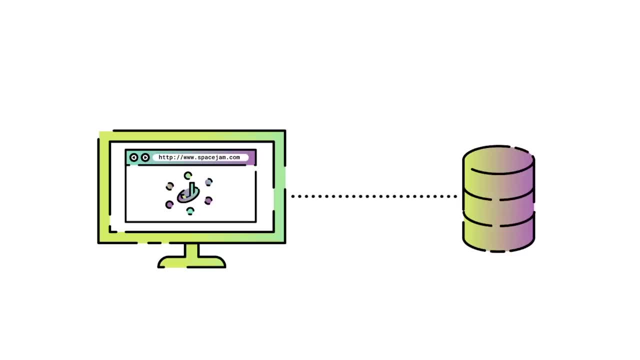 Over and over. In between those clicks, though, the protocol's done. We've made the request. We've got the response. HTTP, as it was originally designed, is a stateless protocol. Once that request receives a response, it's all done. 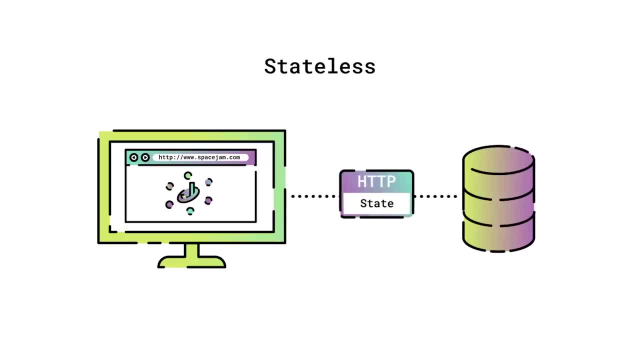 If you want to keep some sort of state, your client will have to manage that itself And send it up with each new request. Check out the notes for more on this. There are more HTTP verbs, also known as request methods, besides GET. 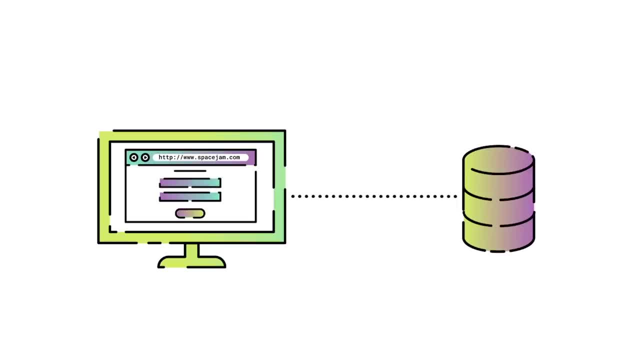 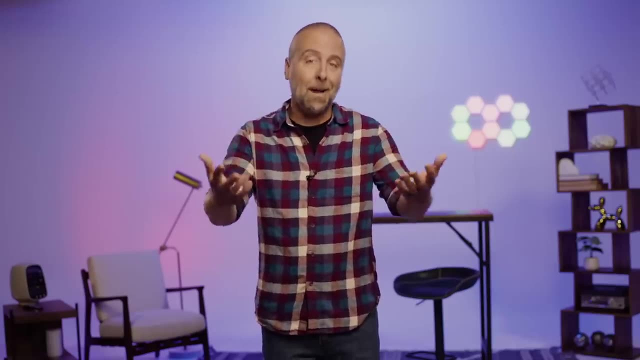 Most common scenario, you see, is when you encounter a form that is used to take information from you. Typically, you'll see the verb POST used to explain that you are submitting or posting data to the server. Okay, so our protocol that's used to transfer this hypertext is, admittedly, a little more complex than our rally chant was. 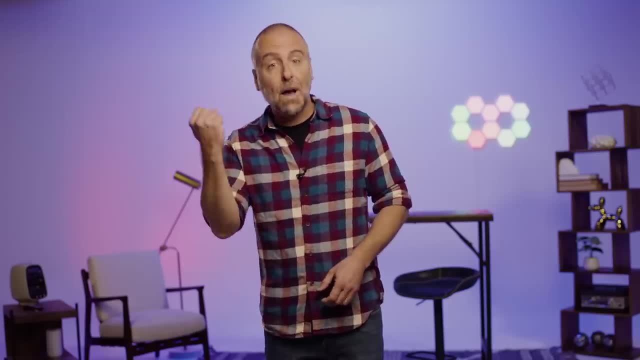 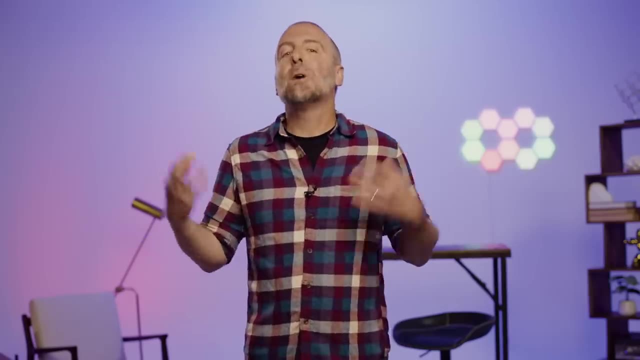 There's quite a bit of important information in there that is included in the request and the response. You've probably seen query string parameters in URLs and you know the stuff after the question mark. This is one way to pass information about the request. 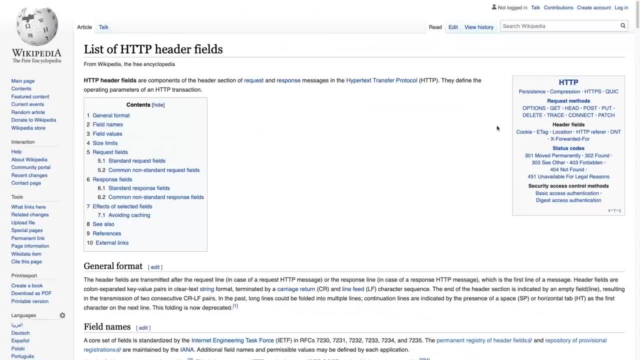 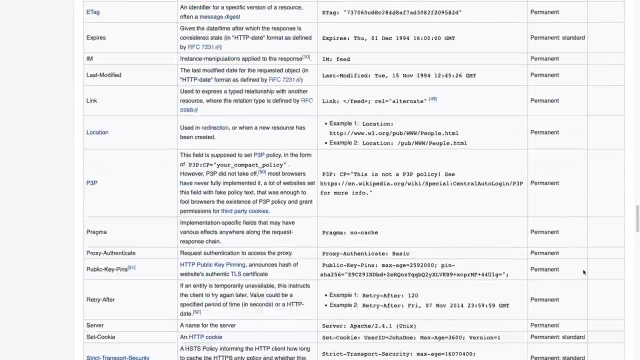 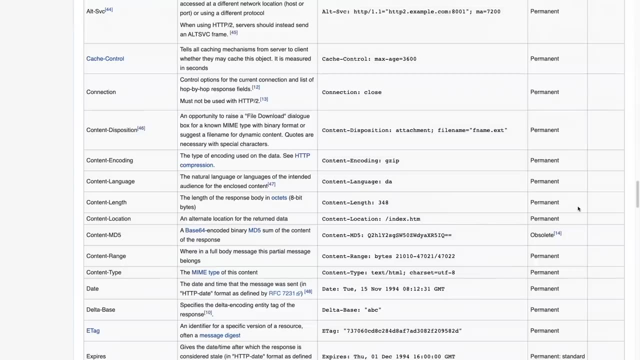 Another common way this information is passed around is through specific key and value pairs called headers. Both requests and responses have headers, and they're used to help further communicate what is wanted as well as what has been sent back. Some of the popular request headers allow you to specify information about the content that you expect back, like the language or the type of content. 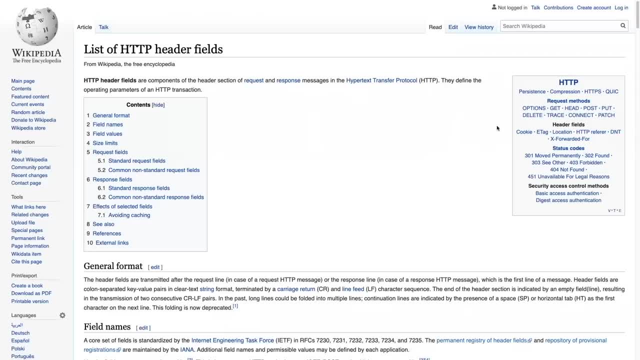 You can also specify the type of content that you expect back. You can also specify the type of content that you expect back. You can also state that you want the page if it has changed since a certain time. This technique allows for caching, which is a powerful concept. 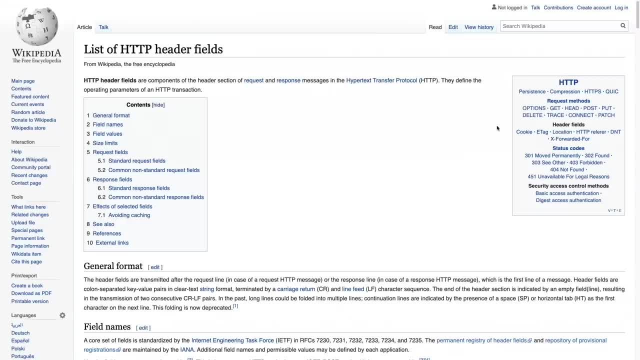 Why get the whole page if you already have it in your local cache? You can embed authentication information in each request using a header. In this way, you're essentially keeping your client logged in across requests. This response also contains headers. A super important one is the status code. 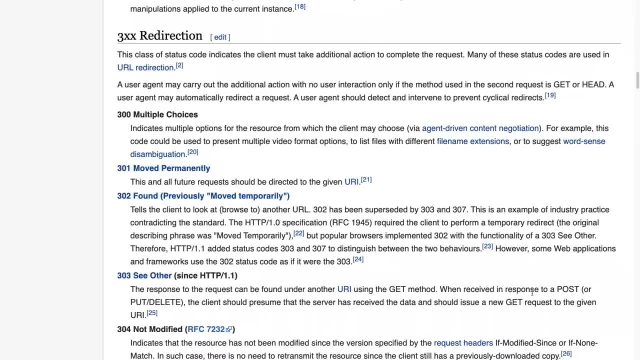 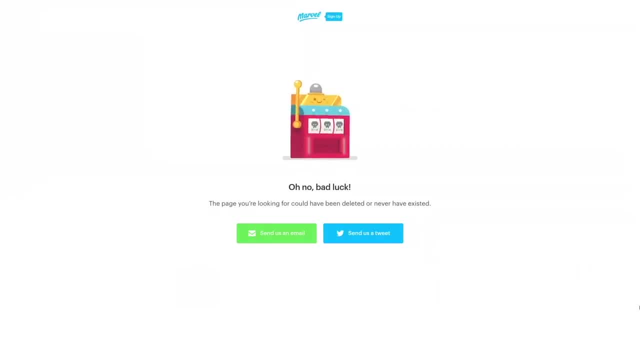 This lets you know what happened on the server side and can convey things like missing documents. I'm sure you've seen the old 404, or maybe I'm sure you've seen the old 404, or maybe The page has moved, but hopefully everything is A200 okay. 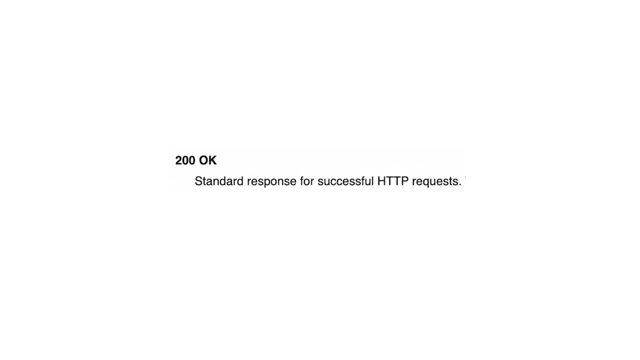 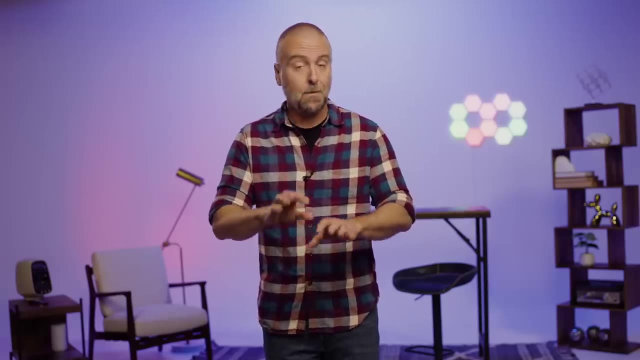 It can also explain the content type, how large the data returned is, and many more things. Okay, got it. Are you feeling good about that little whirlwind tour, Remember? feel free to make me repeat myself if that was too much. 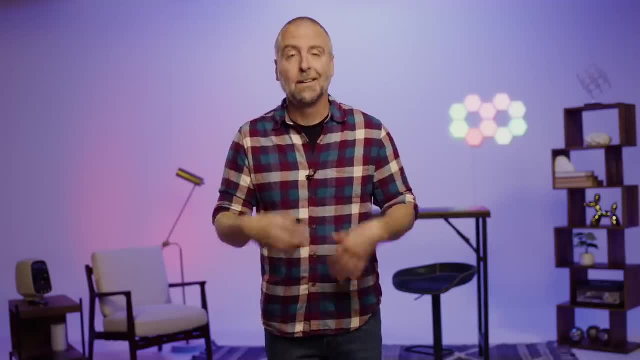 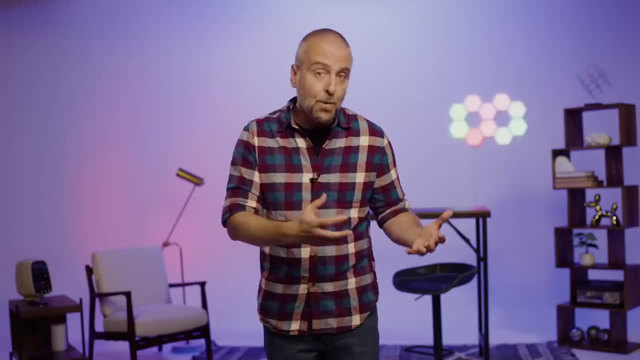 I totally get it. That was a lot of information. It's important to have a basic understanding of these things, because REST sits on top of them. It uses the concepts that were introduced with the web to expose resources that can be accessed and manipulated. 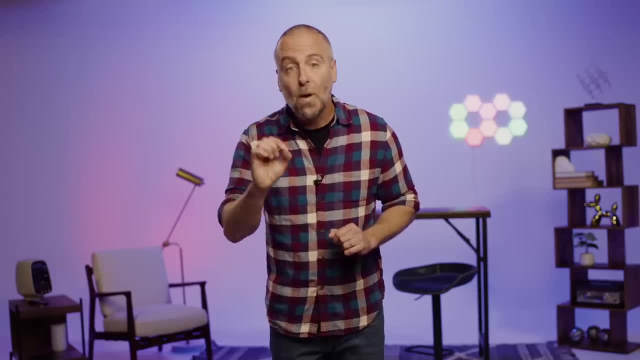 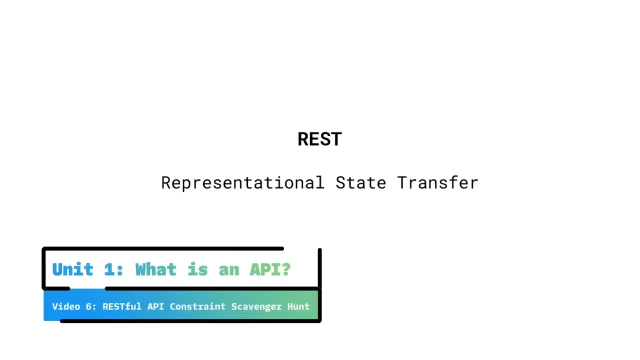 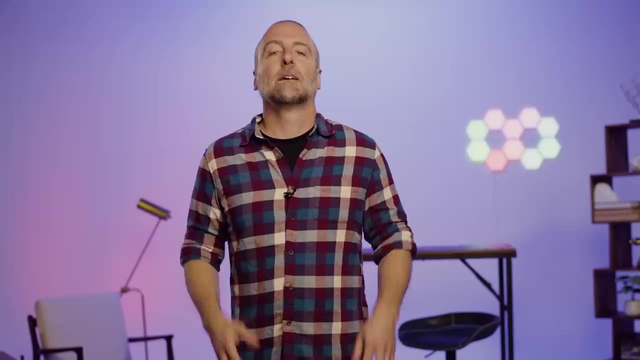 Let's take a look at how the RESTful approach takes advantage of the web and its tooling for your benefit And profit. REST stands for Representational State Transfer. APIs that meet the REST architectural style constraints are considered to be RESTful. Now, a typical way to teach about RESTful APIs is to cover the constraints that define it. 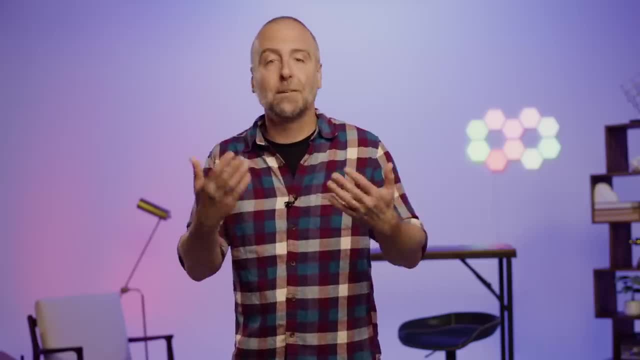 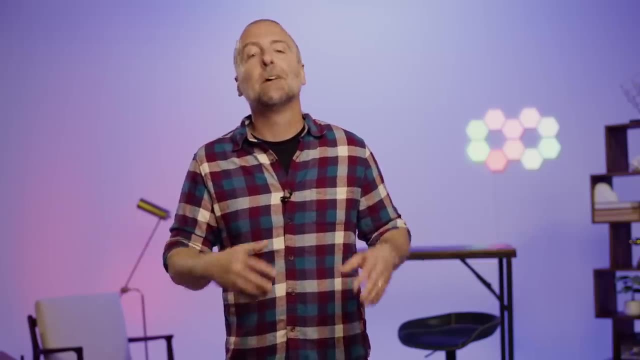 All up front. Now, I don't know about you, but personally I find approaching learning that way pretty overwhelming, Especially from the beginning. I mean, we haven't even looked at an API yet. On top of that, most of the REST APIs that you'll use will meet all of these constraints. 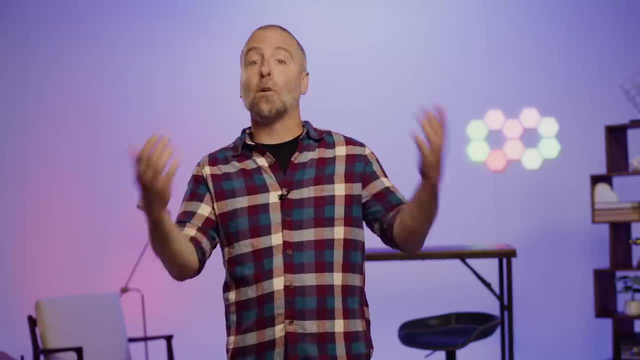 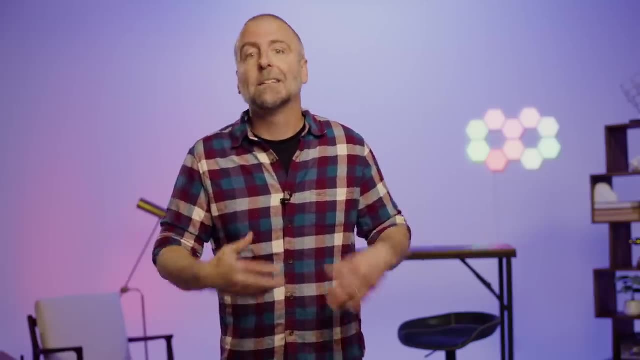 So here's the thing: I promise that we'll go over all the constraints, but let's do it on our own time, Like don't learn them all right this instant. We could even make it a fun journey Like a RESTful constraint scavenger hunt. 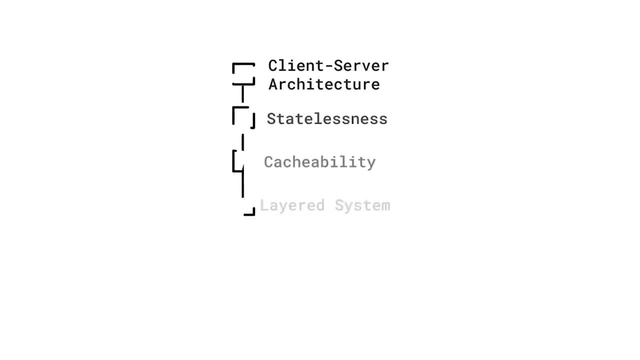 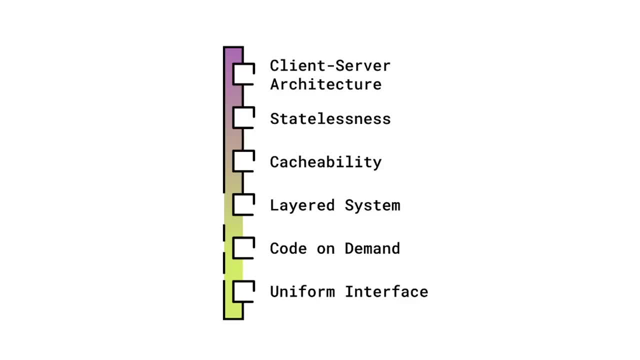 Here are the guiding architectural constraints required for an API to be used. Here are the guiding architectural constraints required for an API to be used. We'll check them off when we discuss them and then we'll loop back once more at the end to review. 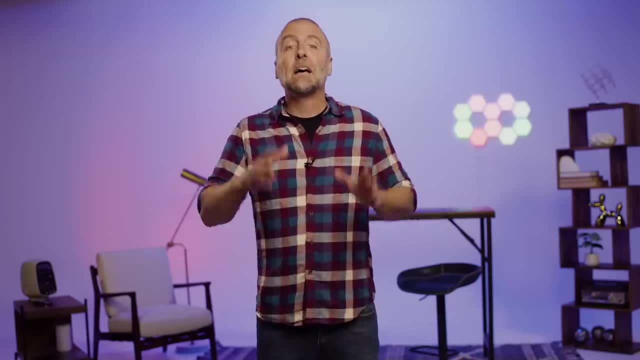 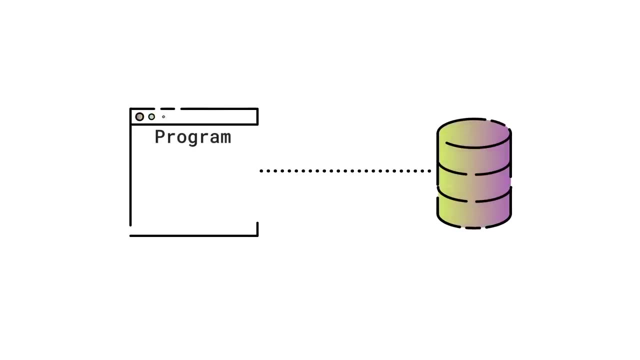 Gotta collect them all. Sound fun. Good, Let's get started talking about how REST API sits on top of web technology. Like a little hat, Much like the web. the client makes a request to a server. The client, in this case, is typically going to be your program. 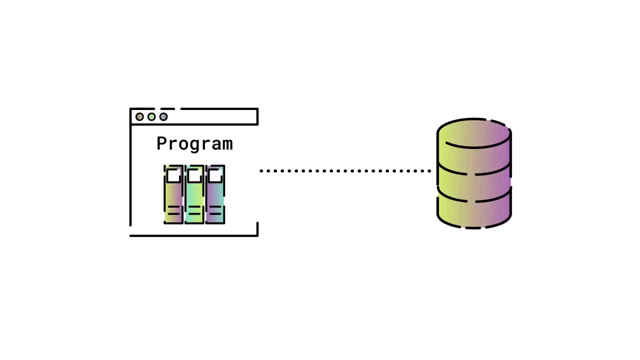 and you'll probably be using some sort of library to create the request to the server. The protocol used- You guessed it, guessed it- it's HTTP And it's stateless. The server won't remember anything about the particular client. If you want to maintain state, like your login details, you must send it with each and. 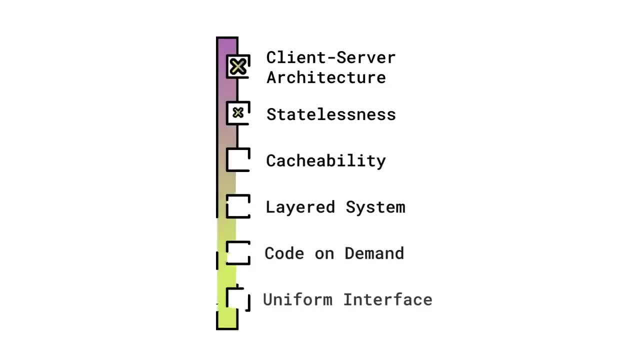 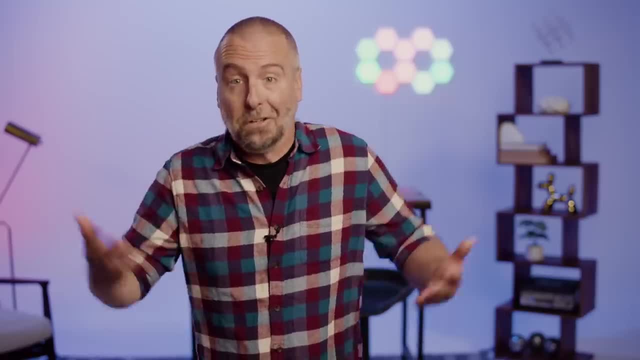 every request. You'll do this using headers And just like that. we talked about two of our rest constraints: client-server architecture and stateless. You got two knocked off already. You're on a roll. Now we should probably talk about what that request was requesting, right? 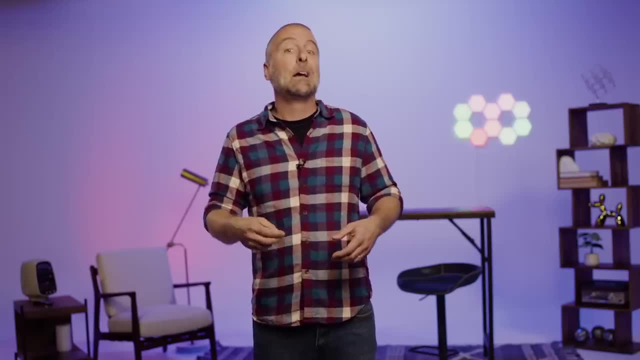 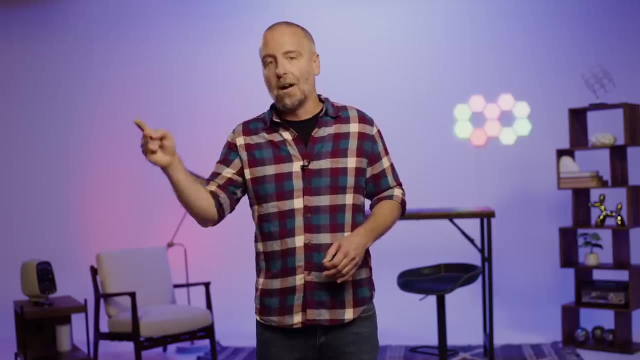 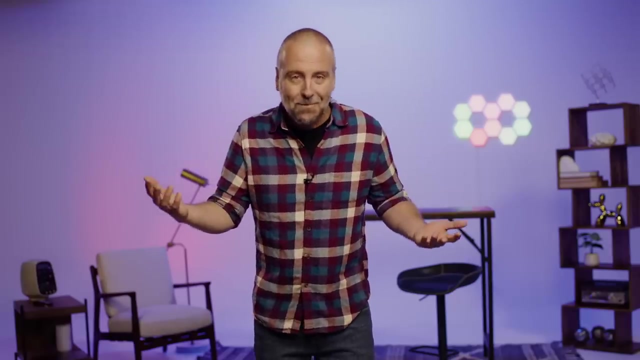 Well, it most certainly was requesting information about a resource. Now, a resource is a little abstract and that's intentional. It's the R in the URL or URI. We use the term resource to reference an object. Also happens to be pretty abstract, right, And this is because we can use. 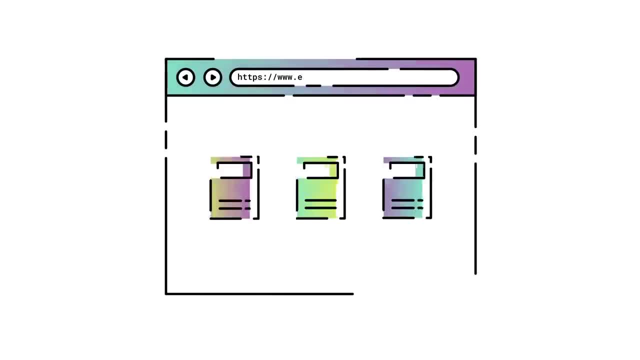 resources to describe just about anything that we build. For instance, let's imagine an e-bookstore website. On the homepage there's a list or collection of new books. Each of these books is a resource. We click in to take a closer look at that book resource. 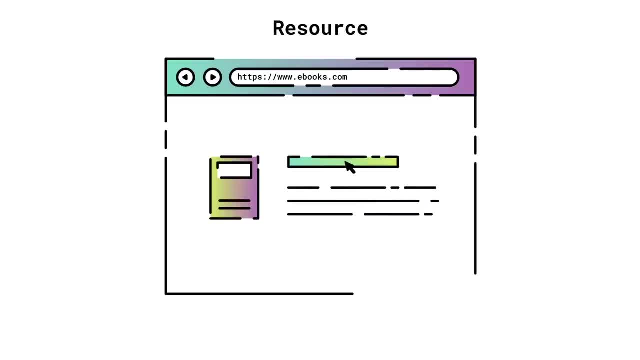 and we see a link to the author, which is also a resource. We click into the author resource and we see a collection of all the other books they've written. Maybe we even see a group of fans- Again another collection- And each of those fans are a resource. Clicking into a fan resource. 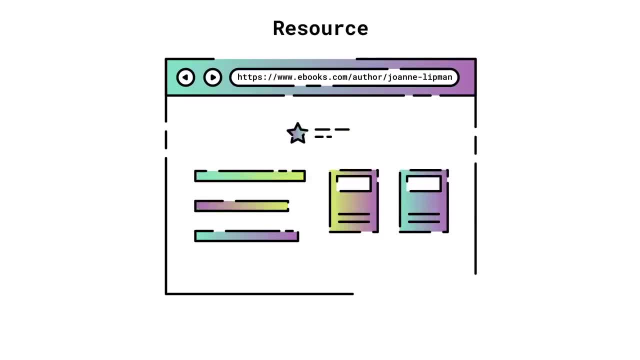 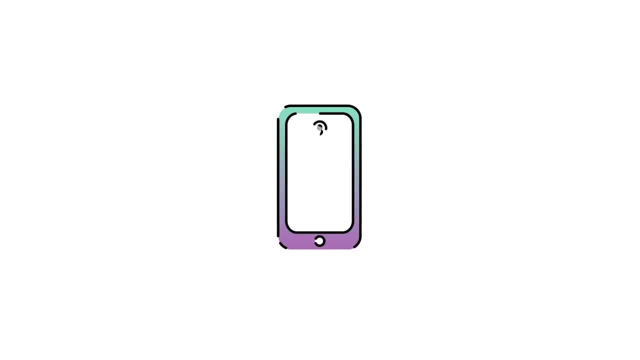 we see a collection of their favorite authors and books. Everything is a resource. Let's change gears. How about an image-sharing application on your phone? So we have user resources and those users post photos, which are resources, and those photos can be loved. So there's a lover resource. Maybe there's an album that could be created. There's an 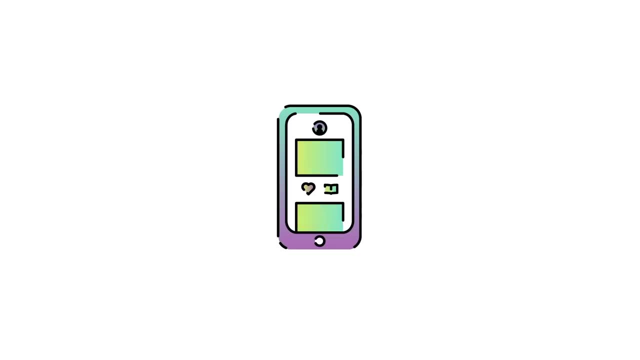 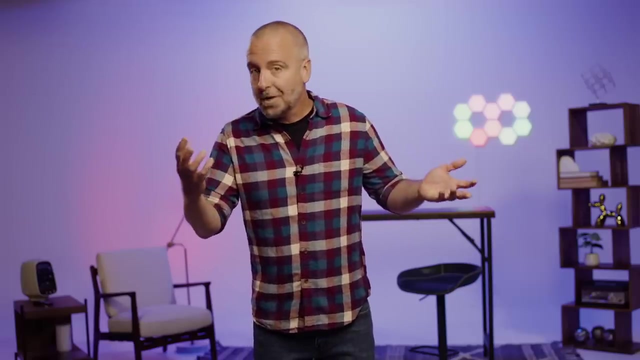 album resource that contains photos and albums, have a collection of contributor resources, Turns out, almost everything we ever want to build can be expressed in terms of resources and collection. Most of what we want our applications to be able to do to the resources can be expressed through the unfortunate-sounding acronym. 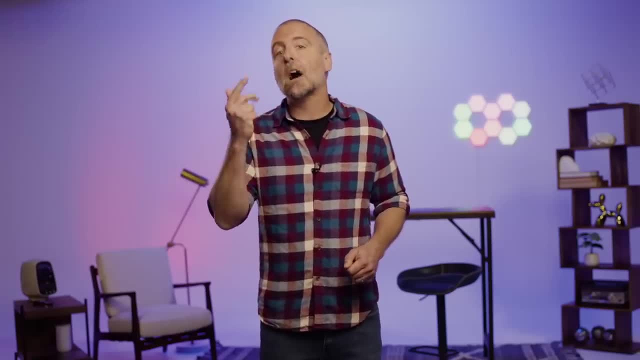 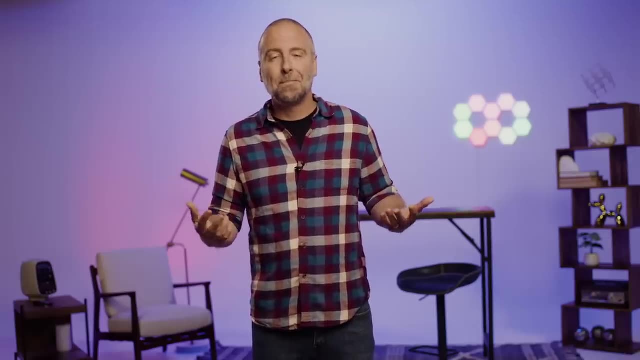 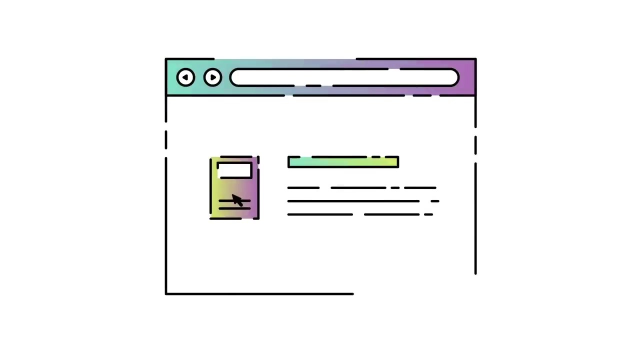 CRUD, And that stands for Creating, Reading, Updating and Deleting. Now, as a user of the ebook site, all we did was a bunch of reading. No pun intended, I actually did intend that one. We were reading right, Just getting information to display it Like we retrieved the author page. 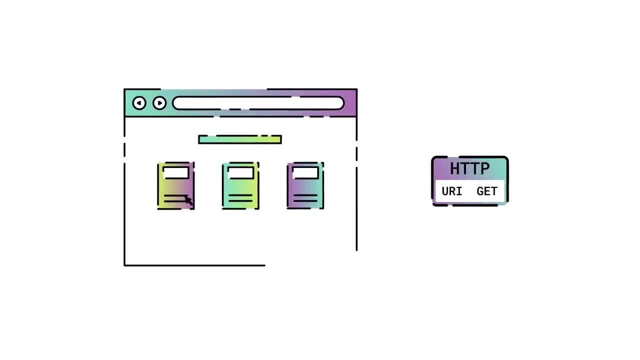 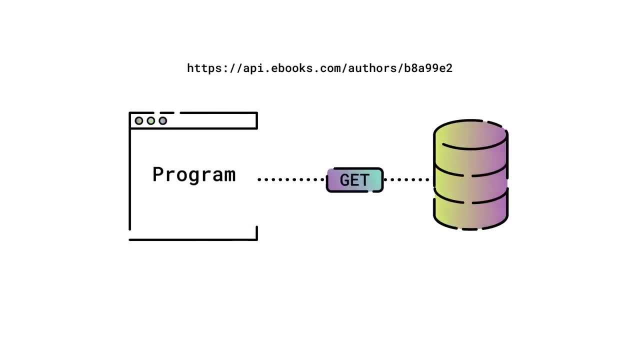 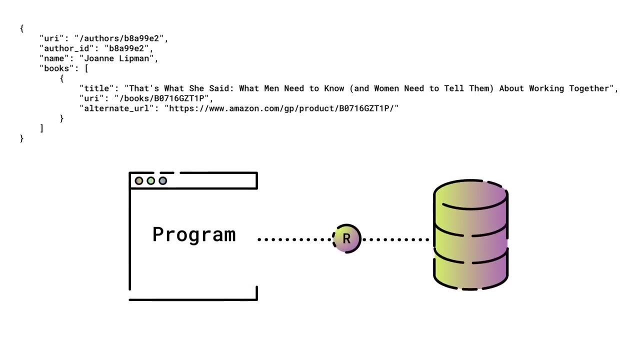 We made a read request. The web browser used a get request to the specific author page. The RESTful API follows the same logic. The program sends a get request to a URI, Then the server responds with data and, of course, all the HTTP headers you've come to know and love. The body is typically represented these days as 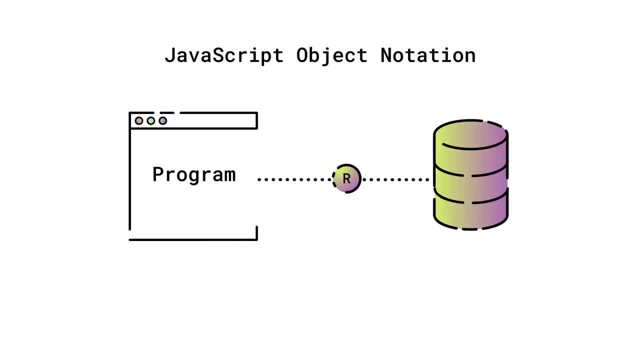 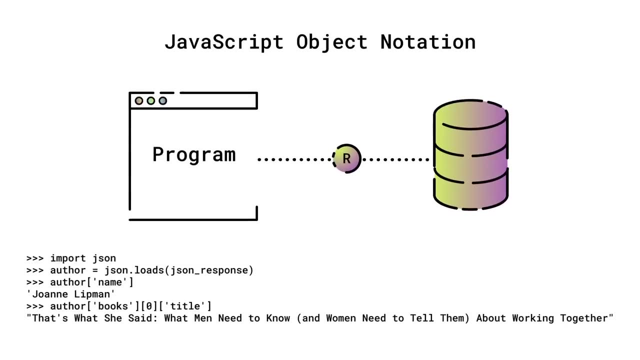 JSON or JavaScript, Object Notation. JSON provides a great way to structure and nest your data. Every programming language that I can think of provides some means of turning a JSON string into a native object. The content type is typically something that you can specify in your request. 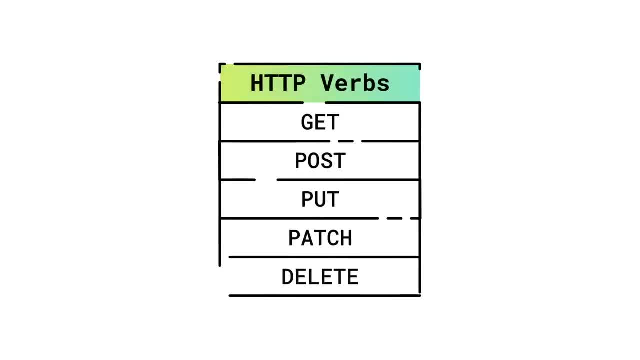 if JSON isn't your thing. If you recall, there are other HTTP verbs available. These verbs are used in REST APIs to clearly state the intention of your request. Want to add an author Post to the slash authors endpoint and send the data that you want to update in the body of your request. 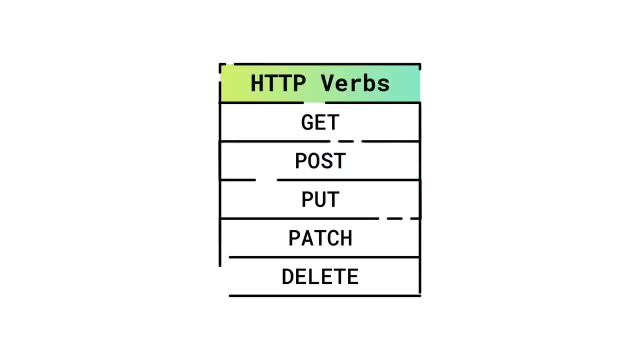 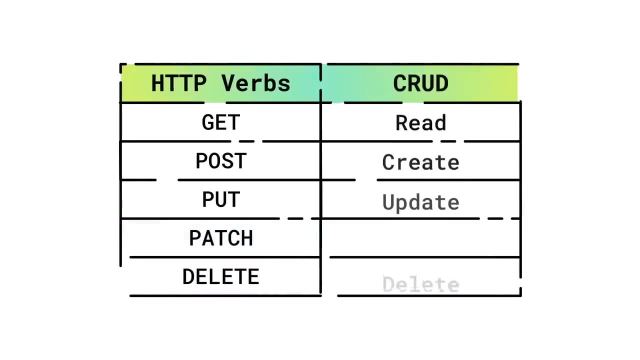 At least fields will be defined for you somewhere. Want to remove an author? Send a delete to that specific author. resource Updates typically support the patch verb and you'll see we're able to represent our CRUD needs: The create request, update and delete. 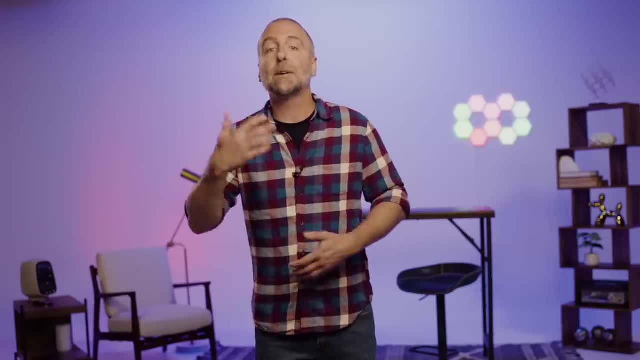 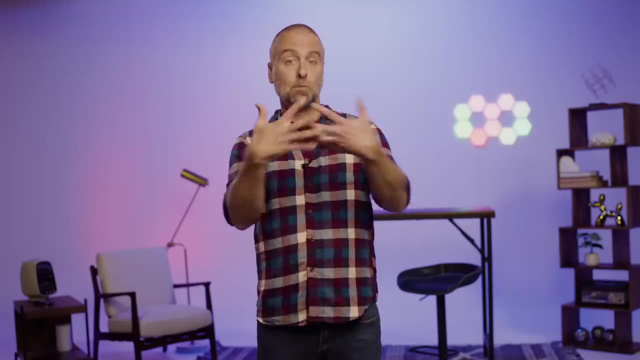 are all in the HTTP method. Pretty cool, right. What this means is that you can interact with any application out there that's exposed their REST API. You could grab data remotely, automate tasks and even smoosh together different services. This is called a mashup, And here's the thing. 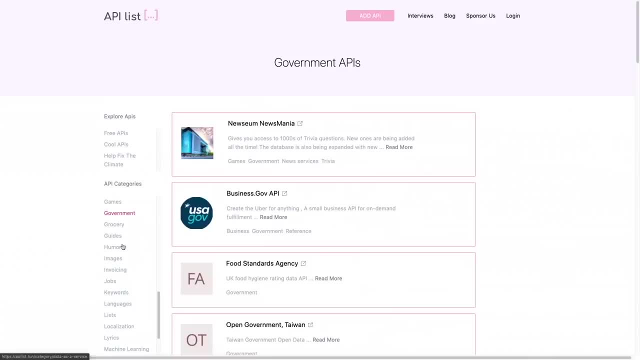 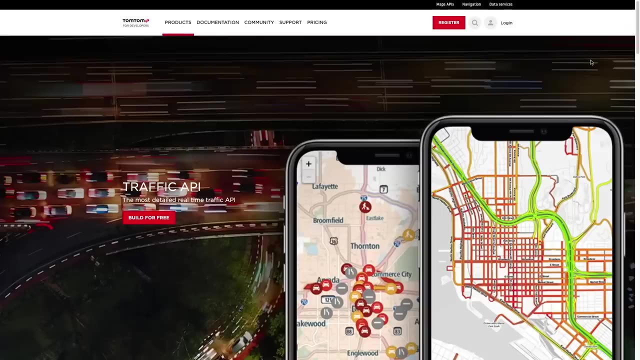 There are a ton of APIs available- just about anything that you could imagine, And if they're truly RESTful, they'll all feel pretty much the same. You can build anything. There are services that allow you to do incredible things with just a few simple API calls. 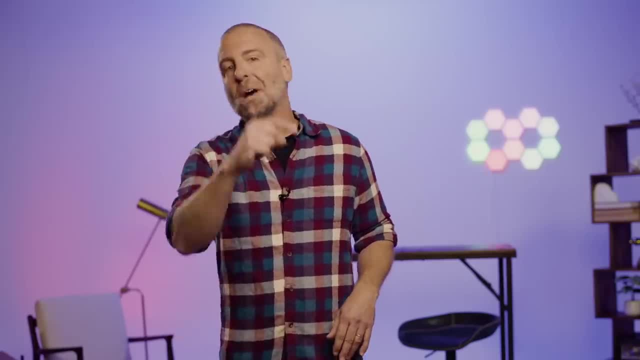 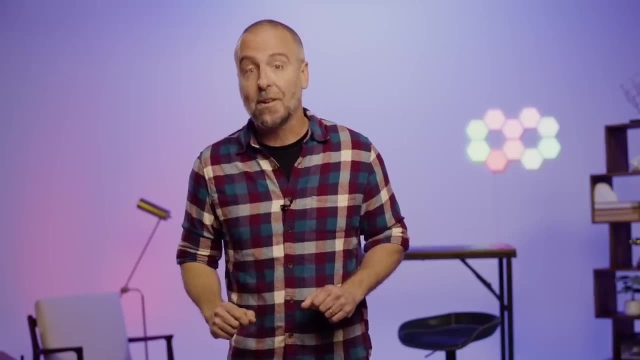 So now the question becomes: what are you going to build? So why don't you take a quick break and when you come back, let's explore a RESTful API together? We'll take a peek at how to use the music streaming service Spotify. 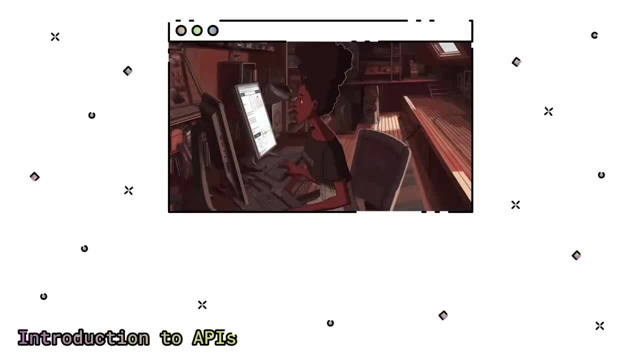 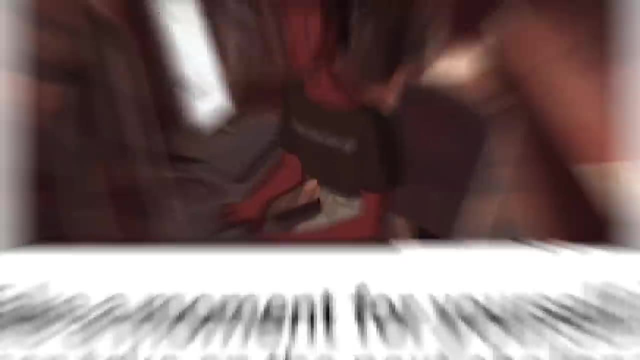 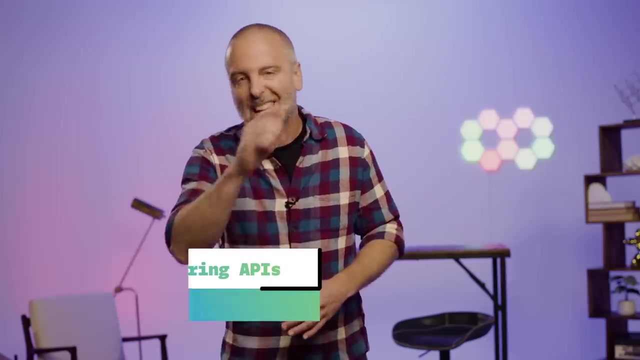 and their excellent RESTful API. You have some newfound understanding of the RESTful API. This is the first time you've seen a RESTful API of how web-based APIs work. I walked you quickly through some imaginary REST APIs and now I'm thinking it's time. 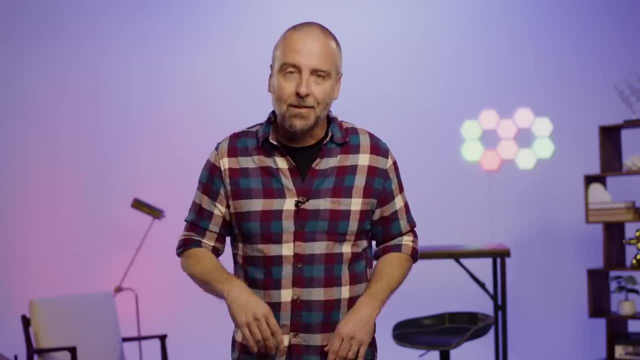 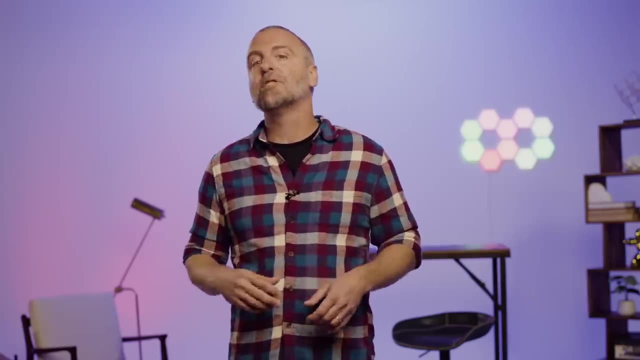 that we get a little more specific. Why don't we go exploring together? Some of these REST APIs allow you to give it a try from the comfort of your very own web browser. One of my personal favorites that allows for exploration is the streaming music service Spotify. 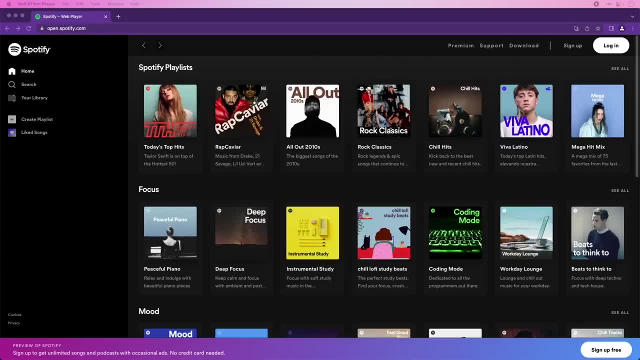 So here I am at Spotifycom, And now a quick word of warning: it is going to look different. I guarantee you, this site is gonna look different because they're always making things better for us, For us Spotify users, us lovers of music. 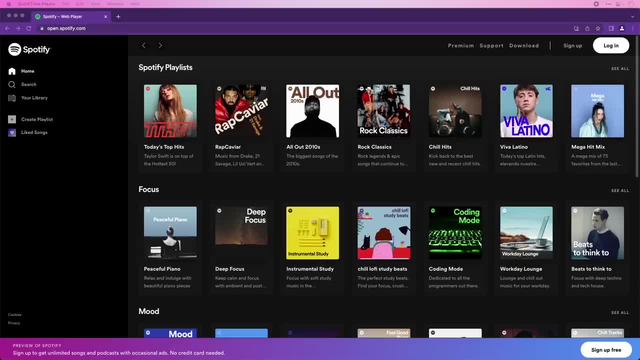 and as well, us developers. So I want you to try this When you go to a site- any site that you want to. you'll see here that this is really nice: Spotify's letting us kind of test out what it feels like in the web, on the webpage. 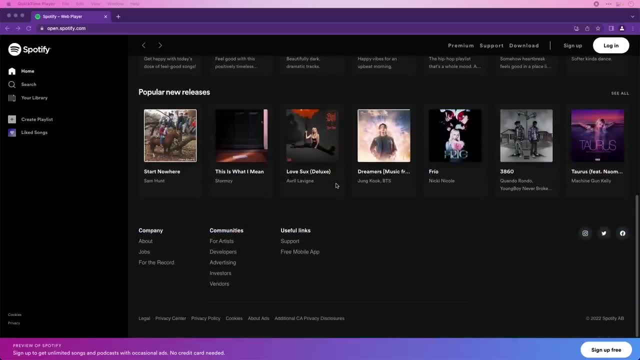 But if I scroll down to the bottom, that's typically where they hide nerdy stuff. Now, I knew this was here, but if I didn't, I would look around for something like this. this developers And I'm going to click into here. 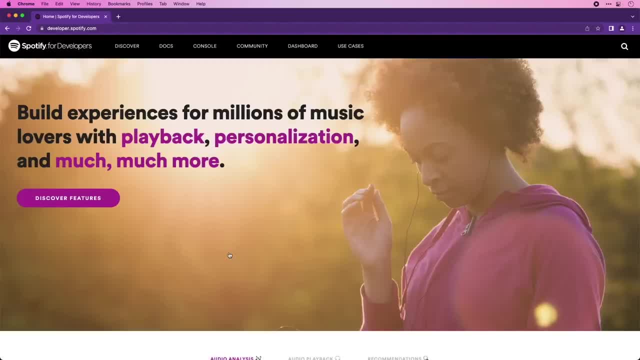 Oh, I cannot tell you how good it feels as a developer to end up in a place where it feels like you're being taken care of right. This is so nice, this Spotify for developers. It looks like it was thoughtful And I can tell you that it is very nice. 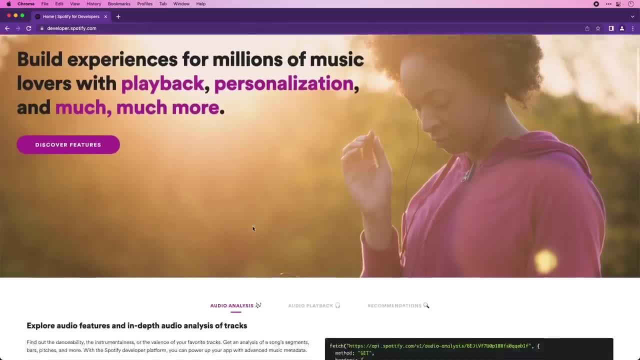 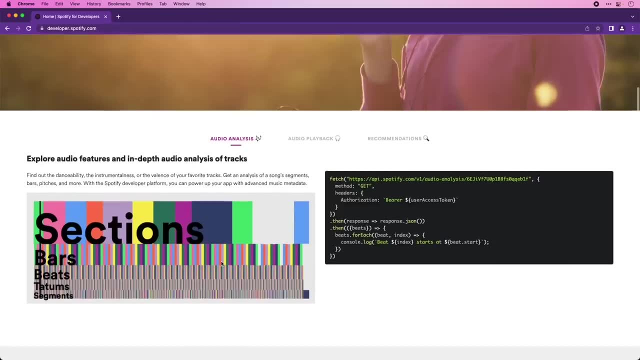 It's a very nice tool. We can scroll down. you can see all sorts of stuff. They give you some examples of what you might want to do. right, What could you build with this? So you could find out like different things. 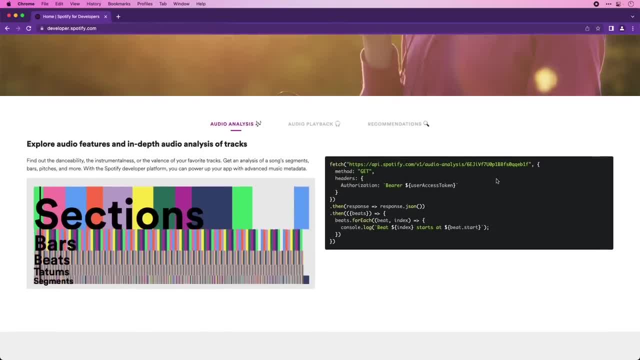 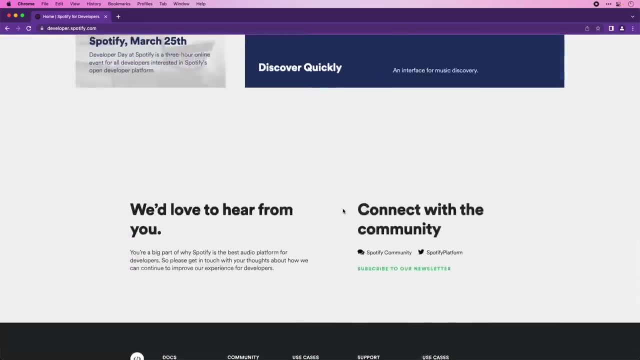 Like you could use an API to see the beats and the sections and the bars. I think that there's a way to figure out if a song is danceable or not. So maybe I could import dancing. we'll see. And if I scroll back up to the top here, 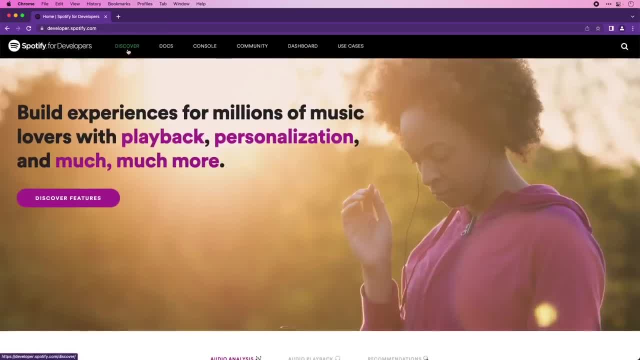 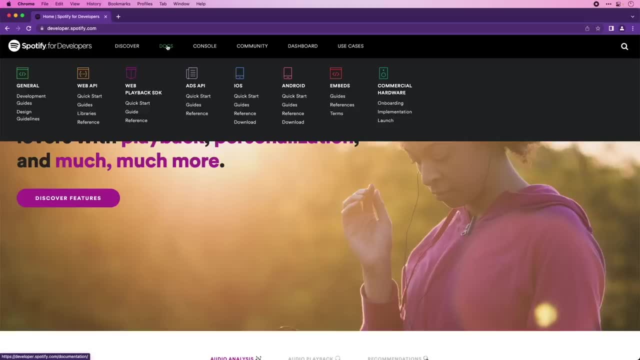 you'll see that there's these different headings. We've got this discover. I think this is great. if you're going to explore things, We have this docs- You'll see that there's all types of different actually APIs and SDKs, software development kits. 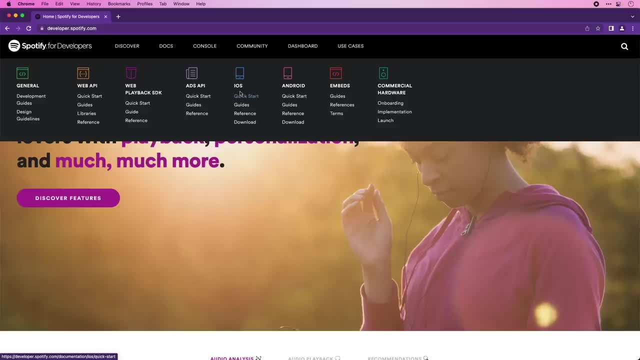 which are APIs which allow you to do different things. You'll see that there's ones for iOS, There's ones for Android. What we're going to be focusing on is the one for the web API. So if I click into that, 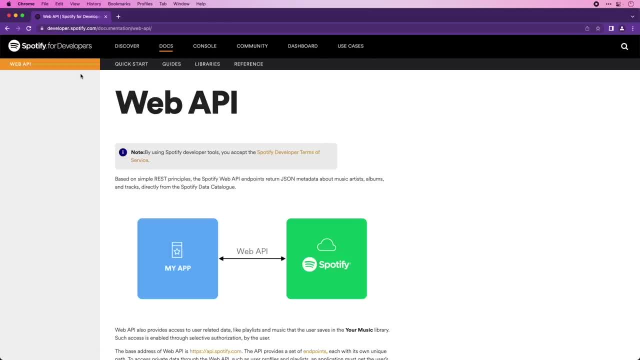 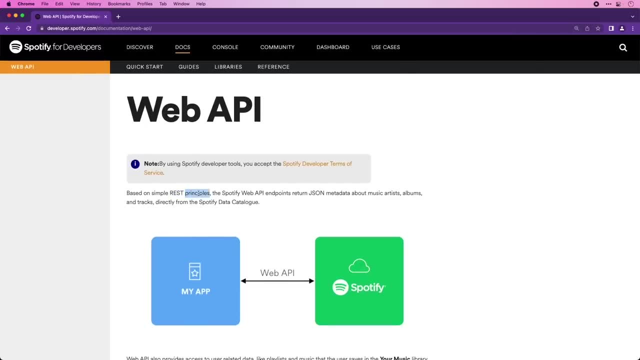 we'll get a nice overview of what this is. I'm going to blow this up just a little bit So you'll see, based on some simple rest, representational state transfer principles, That's our, that's what we're doing, That's what we're going through. 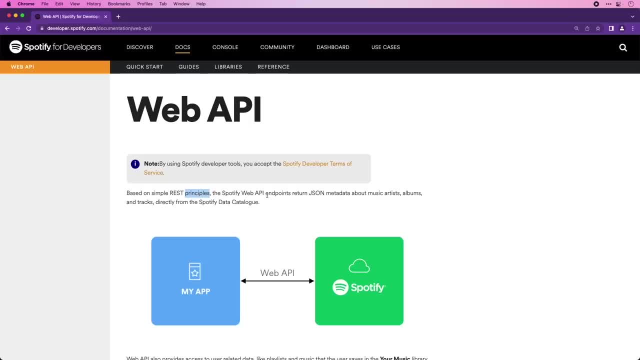 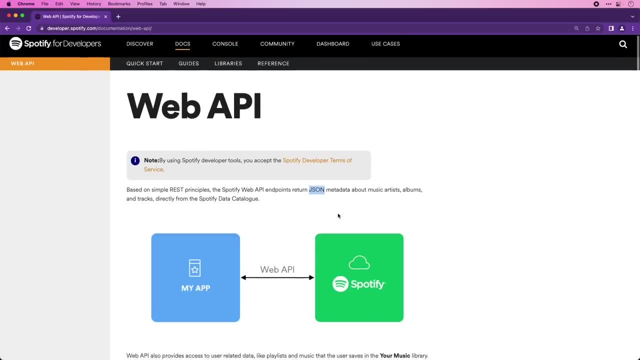 We're going through our scavenger hunt. We're going through that. There's a Spotify web API that returns JSON JavaScript object notation about music, artists, albums and tracks- right, so that's awesome. that's great. uh, so we can see all sorts of 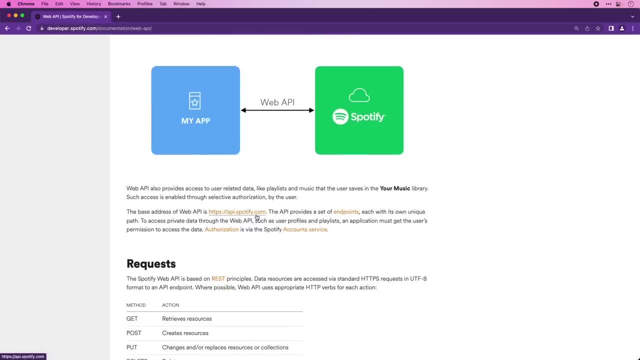 different stuff. it uh, it opens up at this: apispotifycom is the specific url, and then it has a set of endpoints with each unique path, right, each of those urls that we were looking at before. there is a way to get um specific data so you could do this thing for you where you authorize. 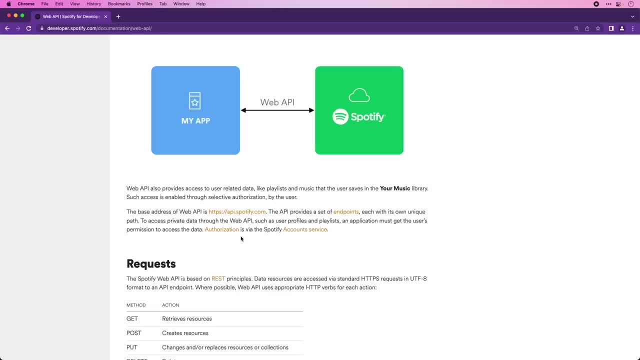 so i could, uh, i could- be a user. you could see what i recently listened to. i could have a playlist i can add to it, but in order to do that, you need to have uh authorization to be able to do that. you don't want to be able to just add to anybody's playlist, right? so, um, there is some authorization. 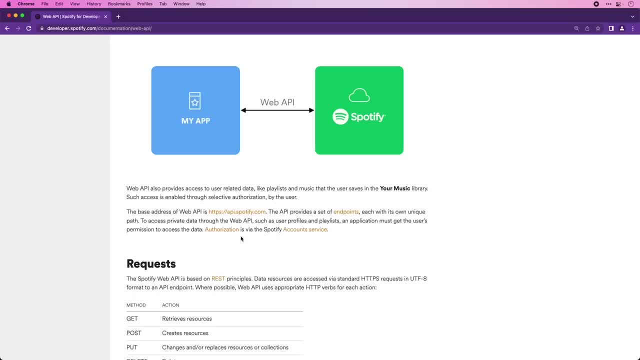 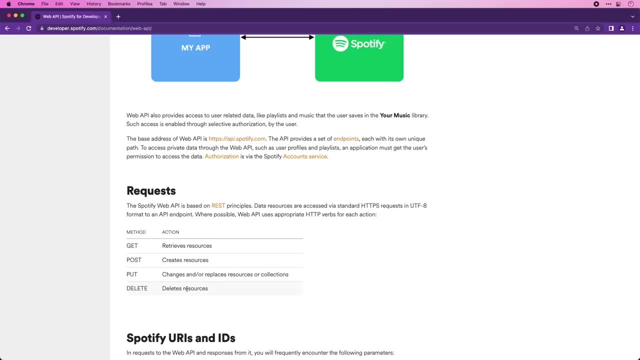 that's available and uh, we're not going to do anything that requires that here. so, uh, if you keep on looking down here, you'll see that there's, uh, it's, it's based on those rest principles, um, and uh, you'll see that it does, uh, get to retrieve resources, right, and there's the post to create. 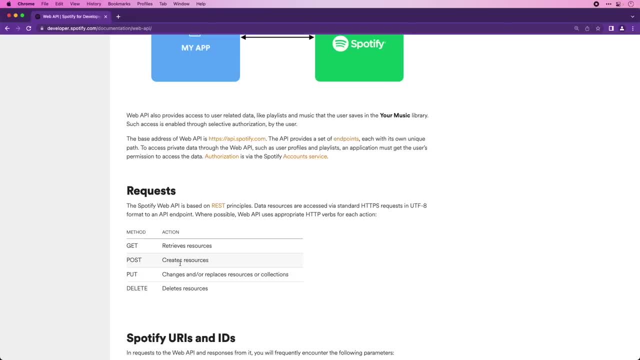 resources and again resources. here are uh, songs and artists and tracks. maybe maybe the resource you're creating here is one of those playlists that we talked about. uh, you can change using a put and a delete will delete the resource. so awesome, right, so it's using rest. uh, like we saw, 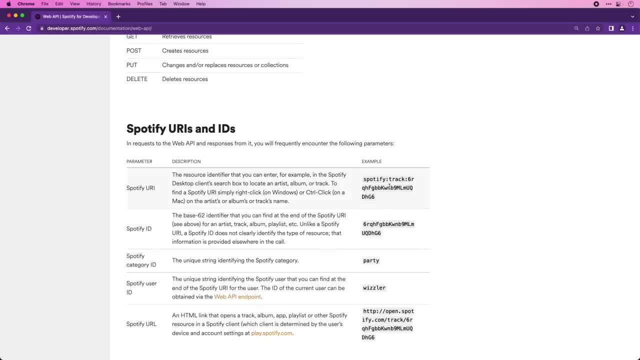 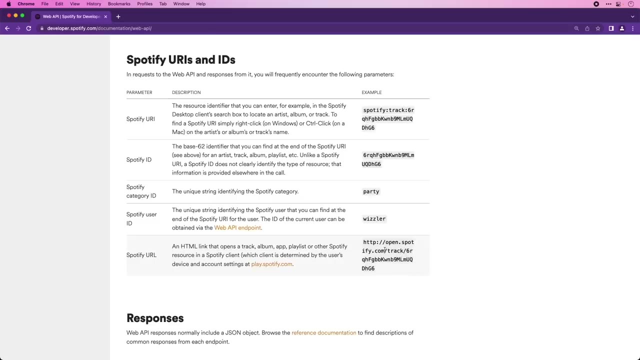 you'll see that spotify uses this uri uh style, so it's a spotify track, and then, uh, it has this unique id, this spotify id. this will make more sense as we we uh dig into it a little bit more, and then you'll see that there's always this uh spotify url that allows you. 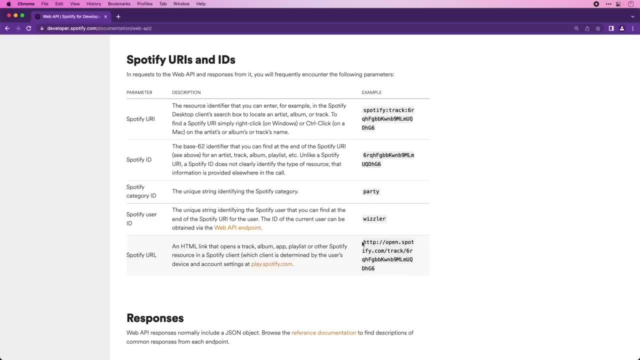 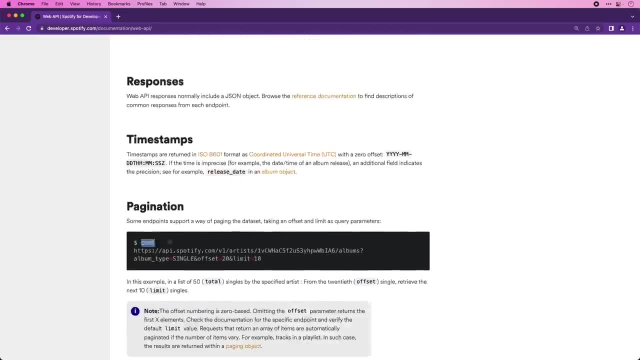 to see what it was. it will show you this. um, as well as we said, uh, the responses come back and they are a json object. uh, and we're going to be looking here at a tool, uh, in in the future, called curl, which you can use from your command. 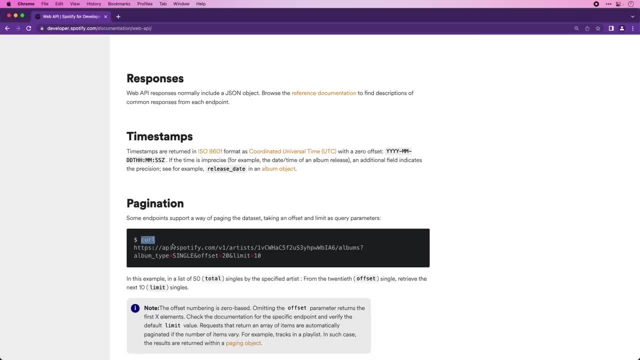 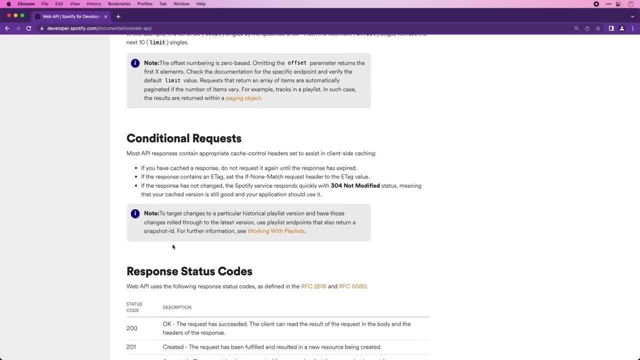 line. that's what this dollar sign here is talking about. i'll show you all this, but basically it's saying that there's a lot of artists that come back. you don't want all the artists and it will come back paginated, uh, and of course, um, you can use caching. we'll take a look at that here you can. 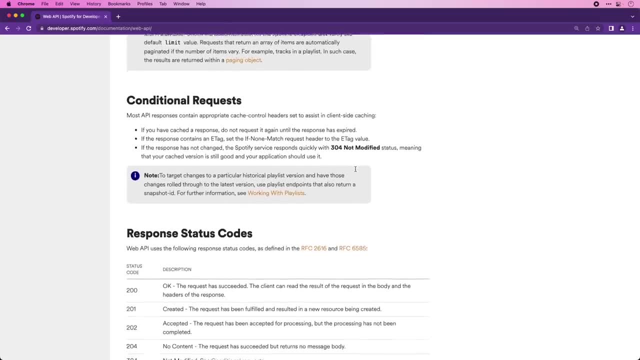 you can uh see if, uh, the thing has changed or not. so we'll take a look at that and then we'll talk about the rest of this as well. at that, and basically the response that comes back: if everything's good, it's going to say a 200. 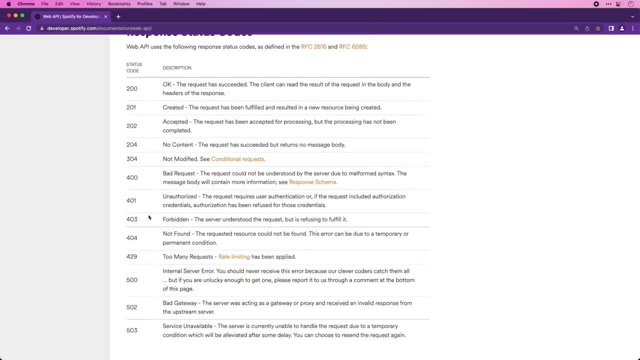 or these, these 200 level uh accounts, and then there's uh bad requests. so if, uh, if you ask wrong or maybe maybe it wasn't found, that's the 404, or unauthorized. if we try to do one of those playlists, uh, we get an unauthorized. and there's also if you're a developer, uh, you never want to. 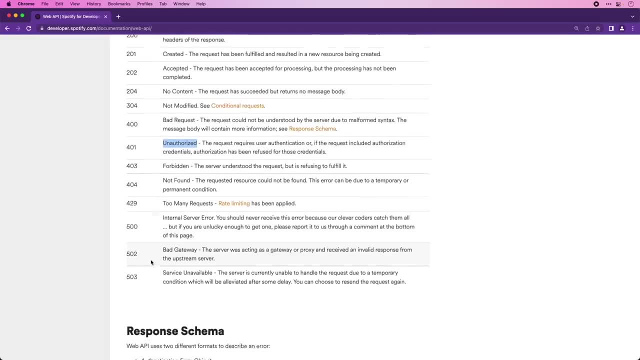 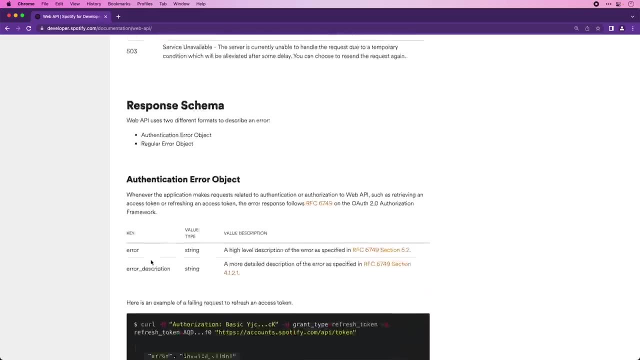 see this one. it's the 500. it means you made an error. um, uh, on the server side. uh, we won't be be doing any of those because we're just going to be hitting somebody else's code. cool, all right. so, um, spotify offers the ability to: uh, you can look at this and you can build your. 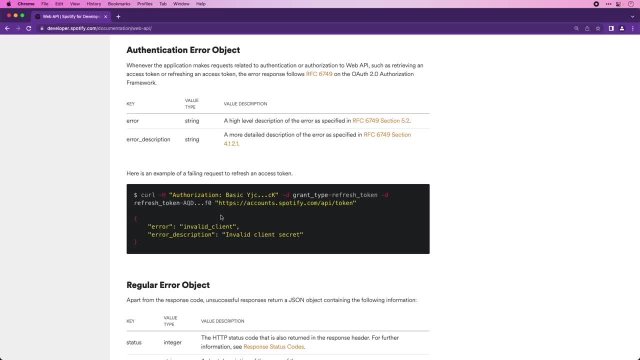 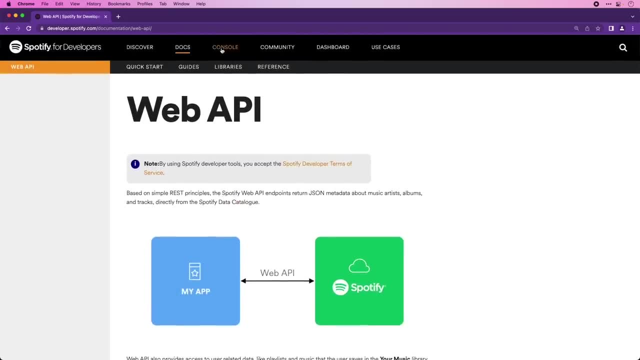 own curl requests. but one of the really nice things that i love about their api- and you'll find this happens often if we scroll back up here to the top- sorry if i'm making you sick there and we're going to jump in here- to what's known as the console. over on the left are the things 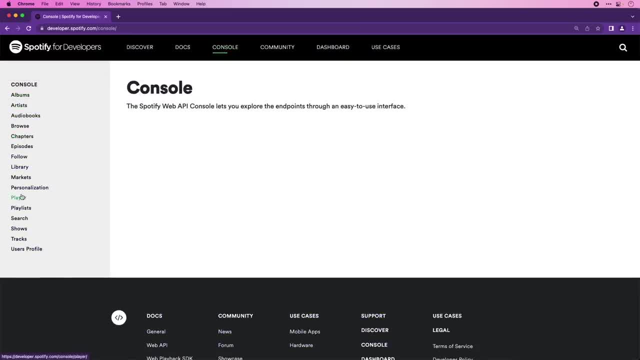 that we can do with their api, and one of the things i want to do first is i want to search. you can see it's making a git to the search endpoint, so i'm going to go into there. and what's really nice is it's set it up so that we can kind of build the query that we're looking for. so now we need to. 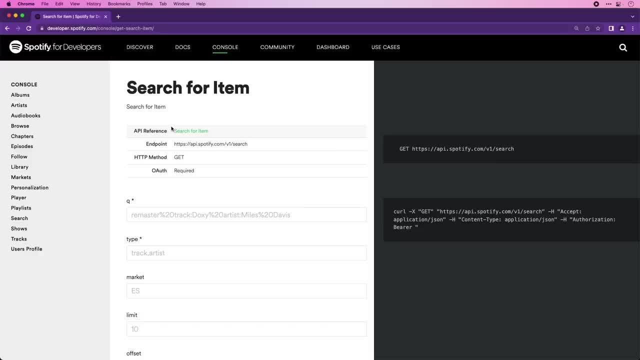 decide what we're going to do. i think probably the first uh person that i would ever search for. the first artist i would search for- and you can see that here it's showing the different values of what that is i would- i would probably search for beyonce. i mean, right, wouldn't you? and i could 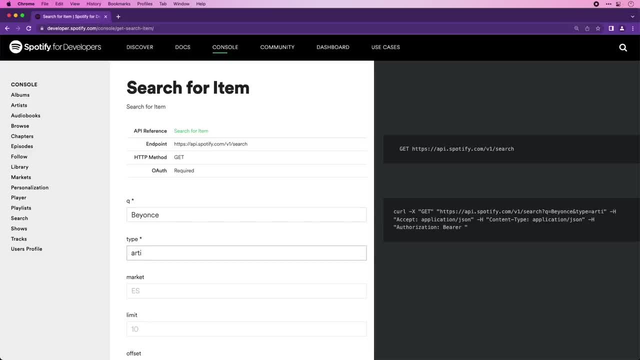 choose? is that a track or an artist? so the type there is important. if i type artist, you'll see that what's happening is i'm going to search for beyonce, i'm going to type artist and i'm going to see. that's where the gist of it is. you'll see the curl here is changing. it's changing the. it says. 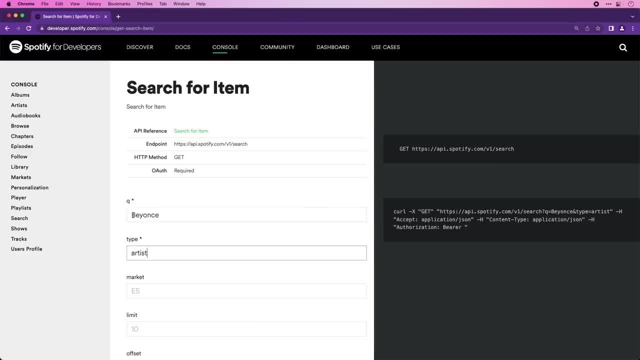 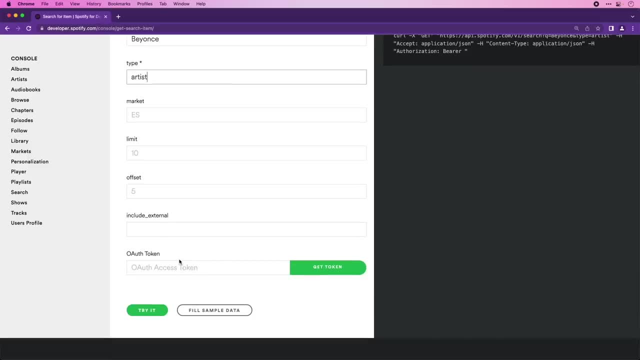 the q is the beyonce, so that's one of the parameters that we're passing into the api and artist is here and you can see there's different, uh, things that we could do here. what's really important is that it needs to have this oauth token. now, what's nice is we can build one of. 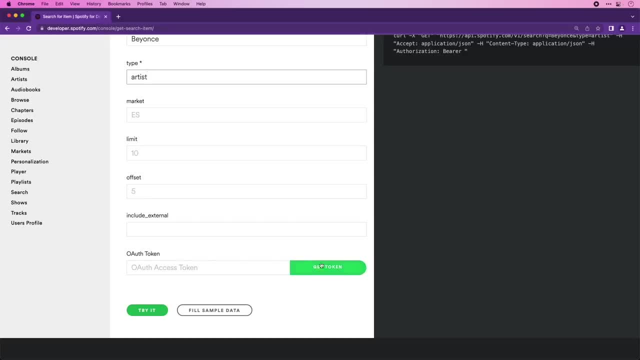 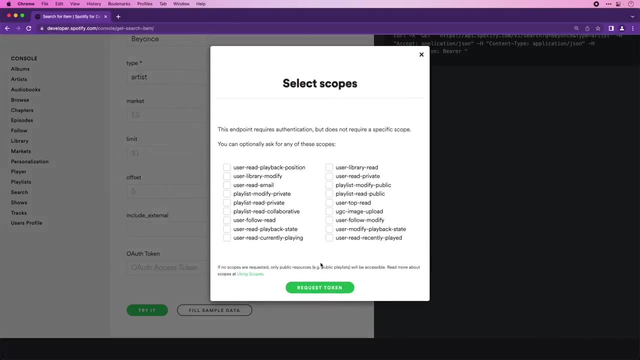 those, even if we don't have a spotify account. so i'm going to do that. i'm going to click this get token. i am not currently logged in, um, and i actually don't have a spotify account yet. in this, uh, in this user, i do have a spotify account. i love spotify. 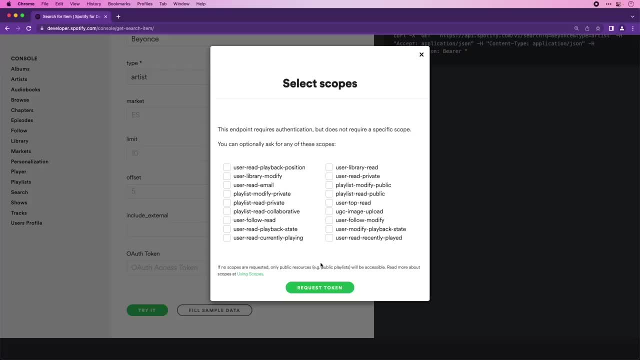 And this is asking basically, what you would do is you would create a specific OAuth token. If you were ever to use this API outside of where we're doing this right now, you would create one of these tokens so that you could log in later. 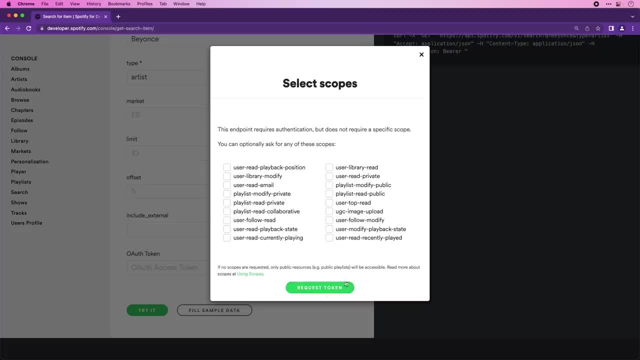 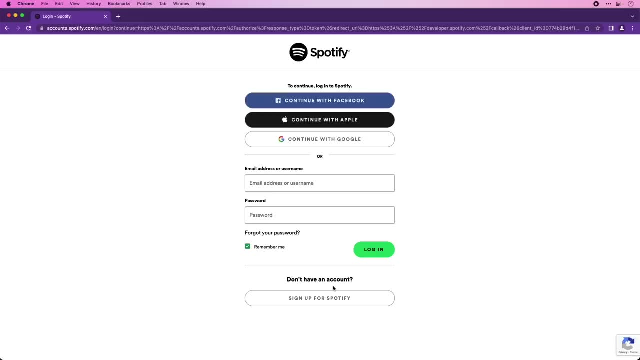 and you say what it is that you want. So here's the playlist, right? We're not gonna do any of the playlist stuff, We're just gonna do a search. Maybe we'll look up some of Beyonce's tunes. So I'm gonna go and I'm gonna click this request token. 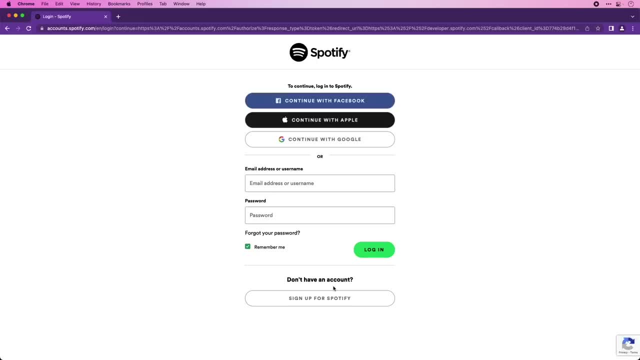 So now it's asking me to either log in with my Spotify account, which I can, or I can create a new one, And let's walk through that. And just in case you don't have a Spotify account already, let's create a new one. 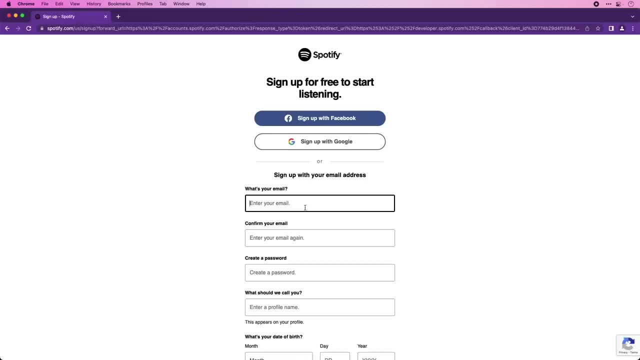 And this will be at my developer account here. So I'm gonna put in my email. So my email. I don't know if you know about this, but if you use Gmail you can do a little plus sign and it will still send to the left side of your Gmail. 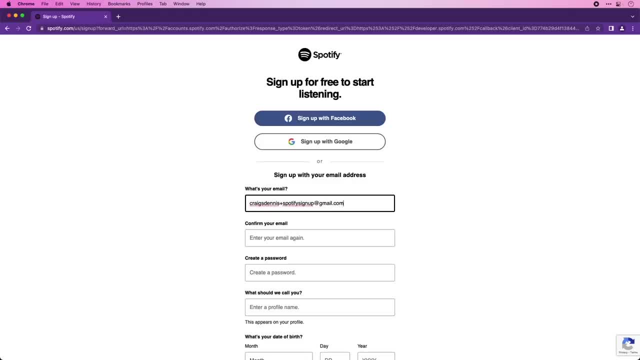 So I'm gonna do at Spotify, sign up And that way any emails I get from here it will have that, And it's a kind of a way to let you have multiple accounts and a thing. So again, my Gmail is craigsdennis at gmailcom. 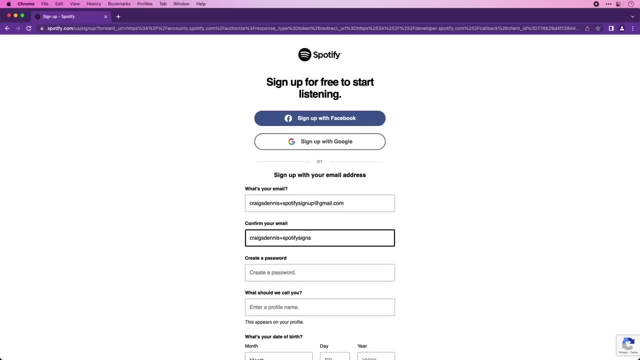 but I'm gonna do Spotify, sign up at gmailcom And it will go to my Gmail. It will just kind of ignore this Gmail does that for you. It's pretty nice, right? So I'm gonna put in the same password as my luggage. 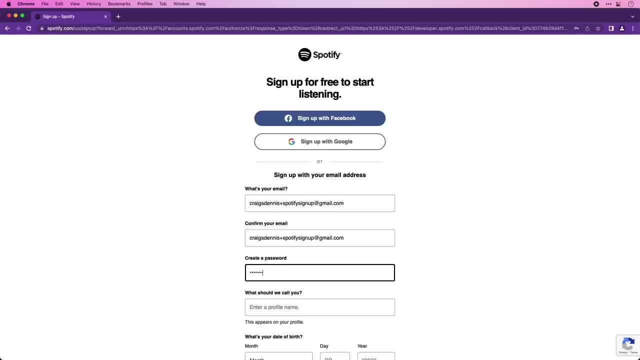 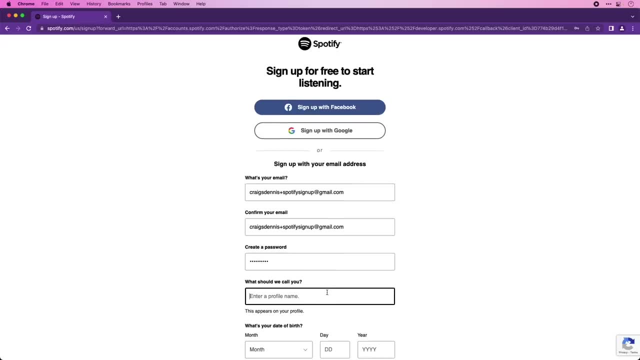 which is one, two, three, four, five, six, Just kidding. And what should we call you? Oh, you know what I love it when you call me Big Papa. That will appear on my profile. I am ready for it. 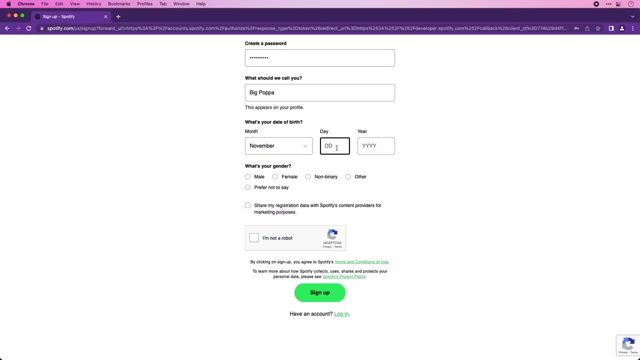 And let's see, it is my birthday on November 19th, 19,. let's see, what do I? I think it would be nice if I was born in 1999.. What is your gender? This is nice, How nice. 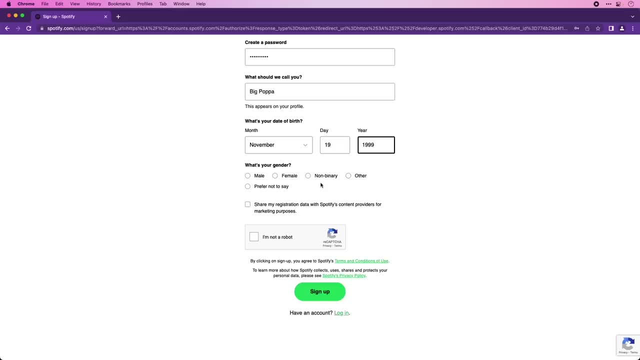 This is like super inclusive. I love that this is so inclusive. It's like somebody at Spotify went and talked to their people and listened to what people wanted, And they included people who identify as non-binary or other or prefer not to say. 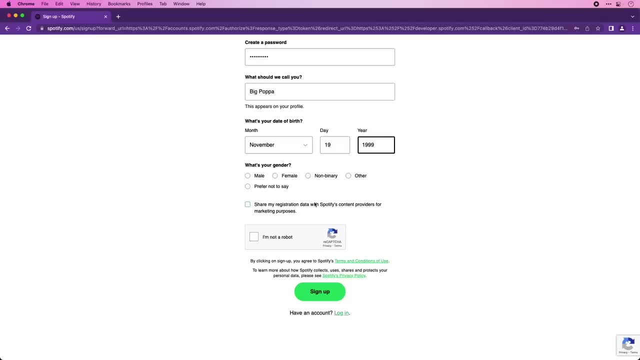 So, like wherever you sit, in that I love, and hats off to you, Spotify, for being inclusive, because inclusivity matters. Share my registration data? Sure, why not? I am not a robot. I don't think I am. Oh, oh no. 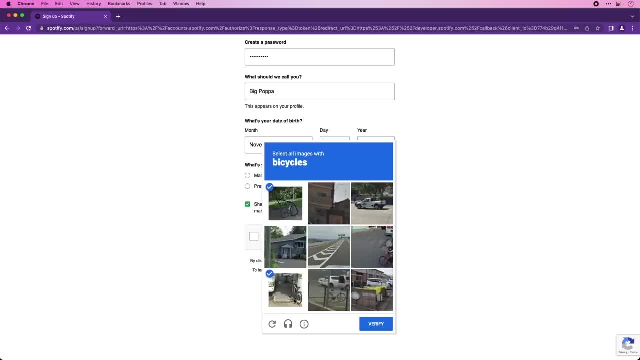 The images with bicycles: That one's got a bike. That one's got a bike. That one has a bike. What is that garbage there Is that bike. This is a bike lane. This is a bike. Okay, here we go. 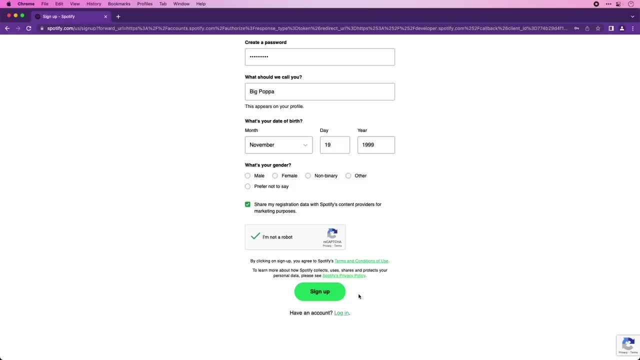 Please, I am not a robot, Thank you, All right, so I'm gonna click sign up. Oh, I am male, I am male, So here we go. That is how I identify. All right, I'm gonna save that log in. 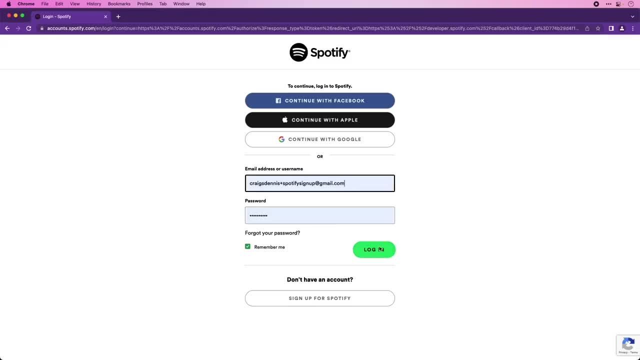 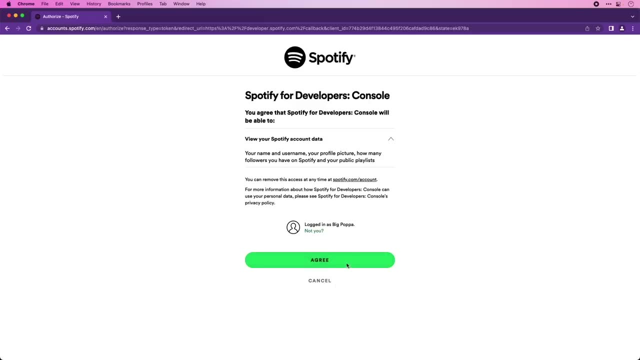 And I am going to log in with it. So here we go, All right. so it's asking me if I have access to this developer console and it will see my logged in as big papa, Here we go. And now you'll notice here that there is this token here. 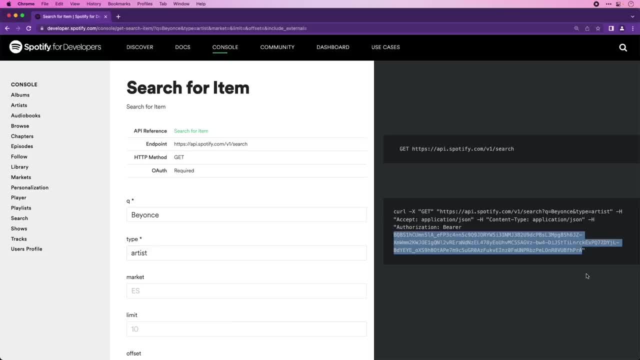 Right, This is this OAuth token that got created for me by Spotify and it's putting it into this console for me so it can share it Now. you never wanna let your token out. If you get ahold of somebody gets ahold of your token. 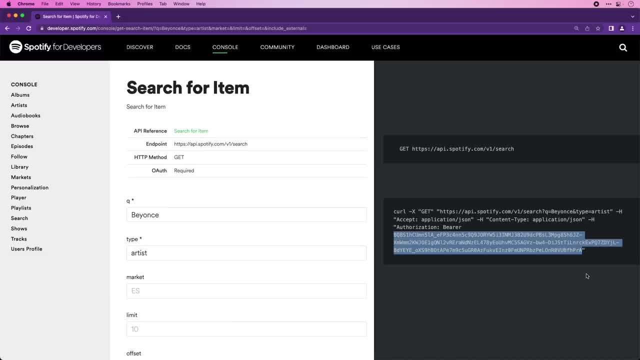 they can do stuff on your behalf, And I realized that this is on a screen being recorded And I am going to get rid of that. Okay, I'm gonna get rid of this token here in a bit, So you will not be able to have it. 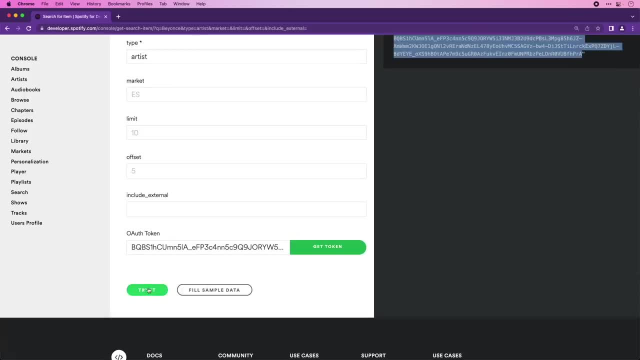 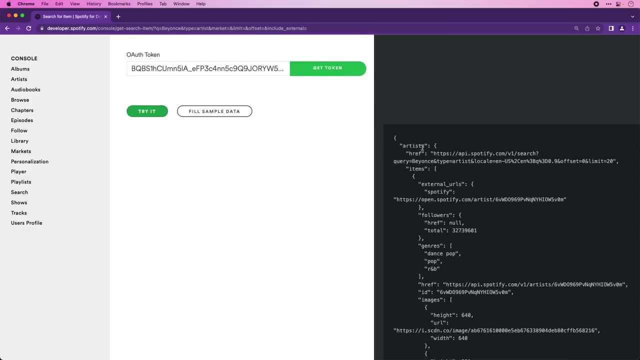 So I've got this token, it's filled out here, I'm gonna click, try it And we're gonna do a search for Beyonce. Let's see what happens. So you will see that we got some information back. So we got a list of artists. 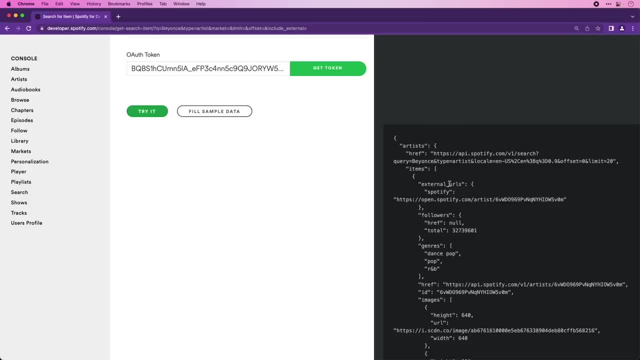 cause. that's the type that I searched for And this is the search that we did. I will see some external URLs And we think that this is probably her. I'm gonna see, I'm gonna grab this really quick, but you can kind of see how things are laid out here. 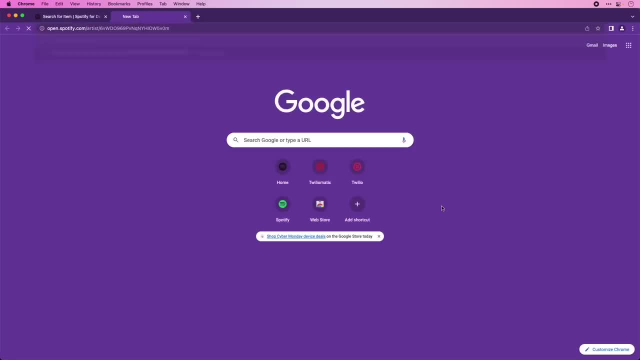 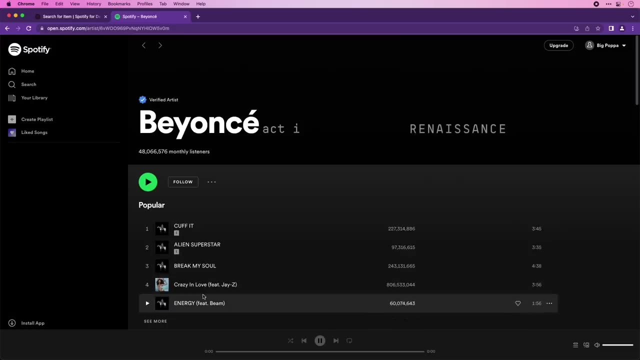 Right, So this is my Spotify URL for that. All right, So let's see if this is. is her? This looks like her. Yeah, yeah, definitely So so great, Crazy in love, cuff it. I haven't heard that one yet. 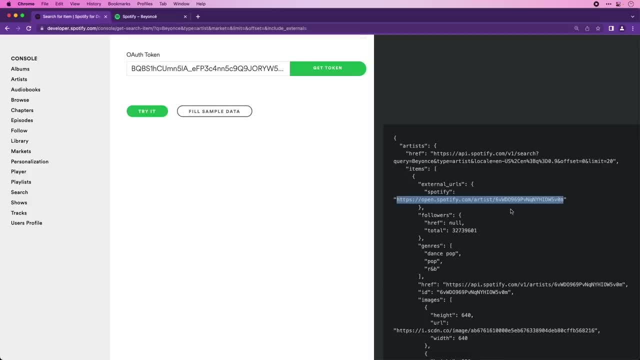 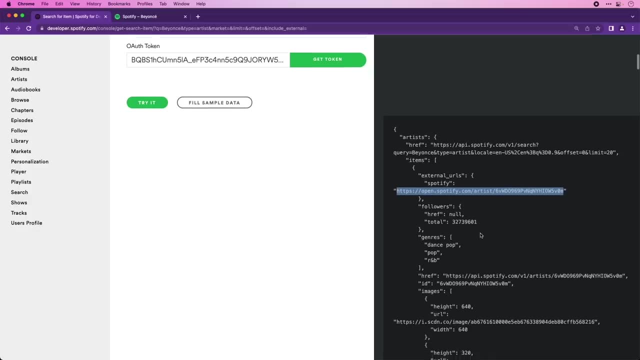 Awesome. So this is Beyonce, Great. So we got her. we found her. We use this search. It has shows how many followers she has- Wow, 32 million. Good job. It tells the genre, So we can do all sorts of really cool stuff with this. 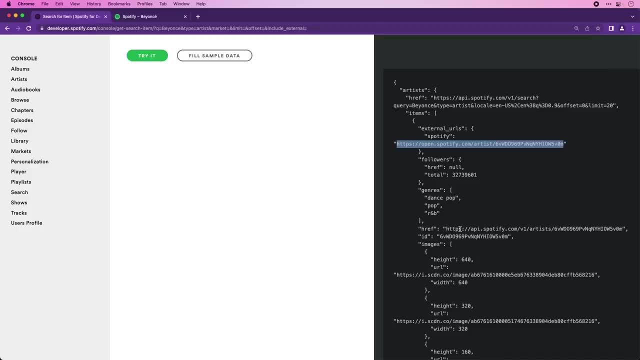 And here you'll see that I'm getting a URL, I'm getting a link that will open up her specific artist page, Right? So so here is is her ID. So if I take her ID, I'm gonna grab this ID. 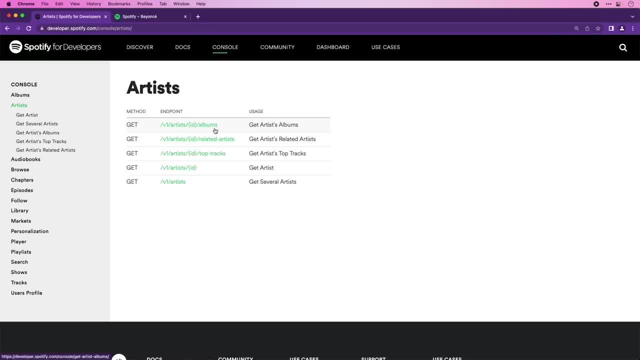 I'm gonna come over here to artists and I can come in here and I can show all of the artists albums. So you'll see it will be artists, slash ID, slash albums. Let's see all of the albums that she did. but let's look at that in JSON format. 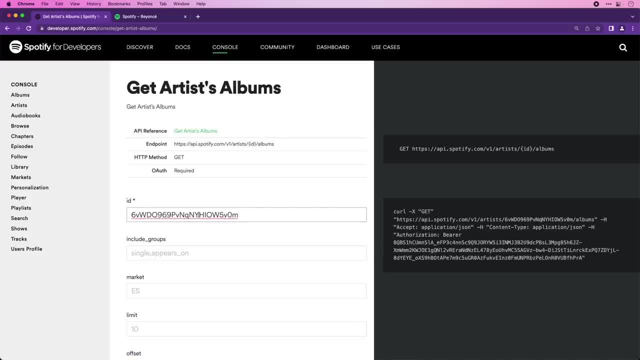 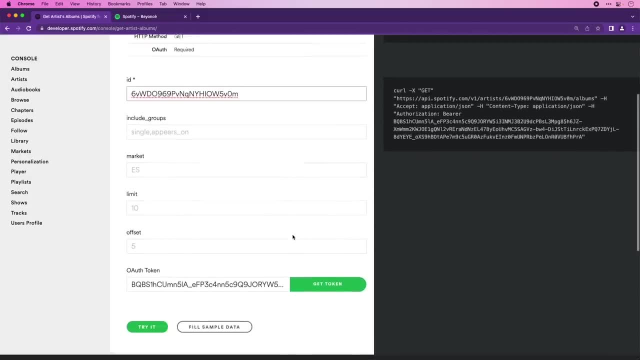 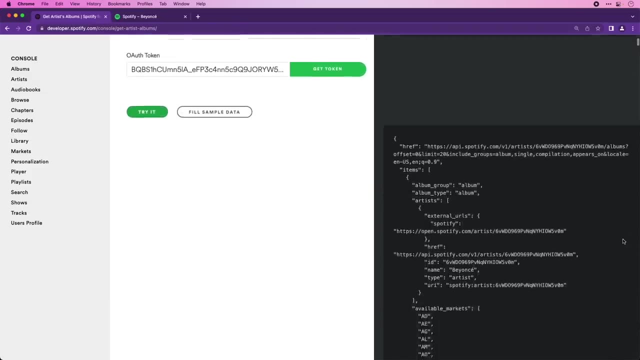 So the artists that I want, I'm just gonna pipe pipe that ID in there from before, Right, Right, Right. my bearer token, the console has done that for me and i can go ahead and do try it, and we should see that now it's going to return back albums, right? so we've made a get request to the albums. 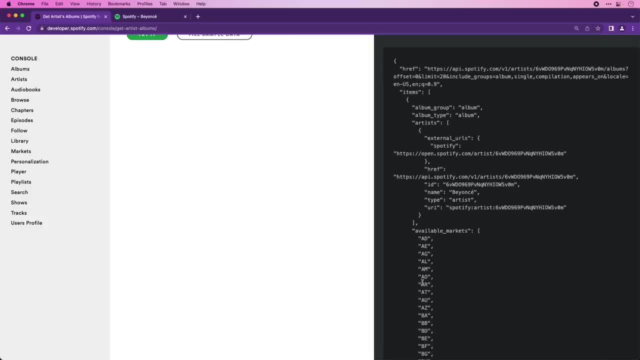 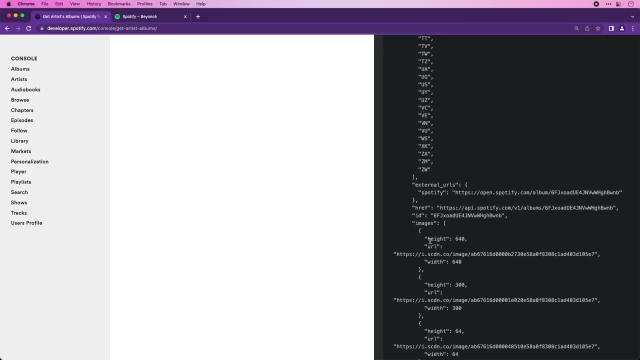 and i can see all of the albums, uh, that she's had here, and we can see, uh, where they're available in different markets as well. looks like she's available in lots of markets all over the world. uh, who runs the world? all right, so here we go, uh, we're going to look, let's see, uh, these are. 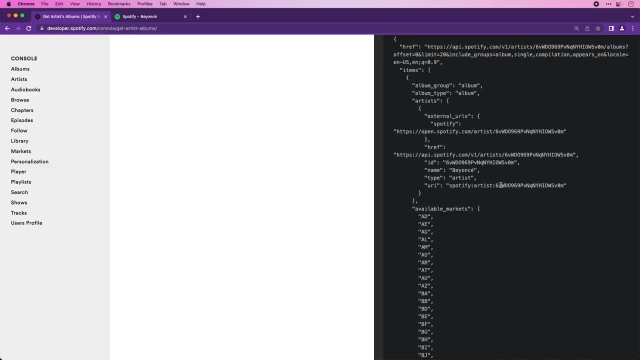 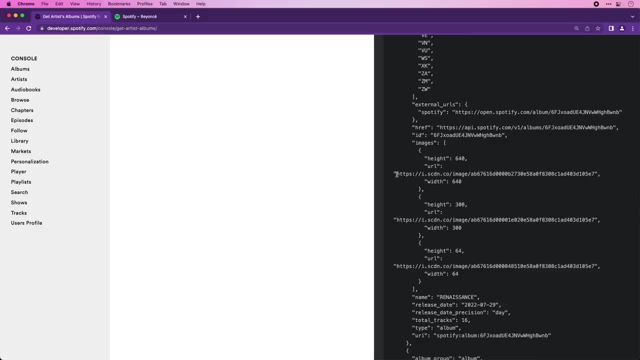 these are albums. that's the artist there. that's the type of the artist. let's get one of the albums here. let's make sure that we got it. so, uh, you see that it's got different things like i could get access to, maybe the image of what this album is. so let's do that. i'm going to post that here. open. 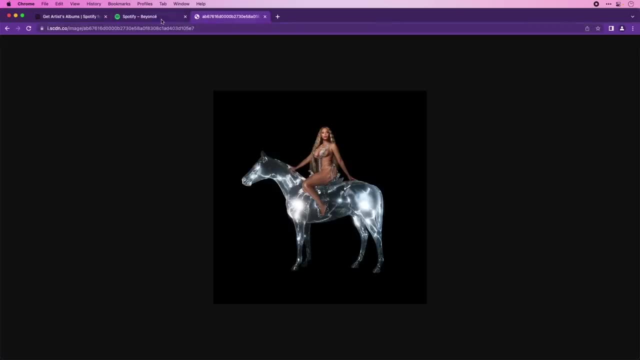 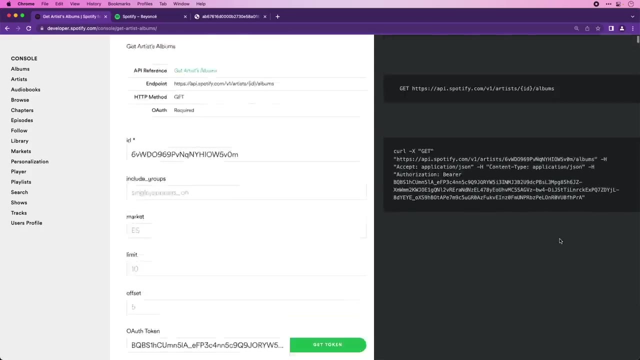 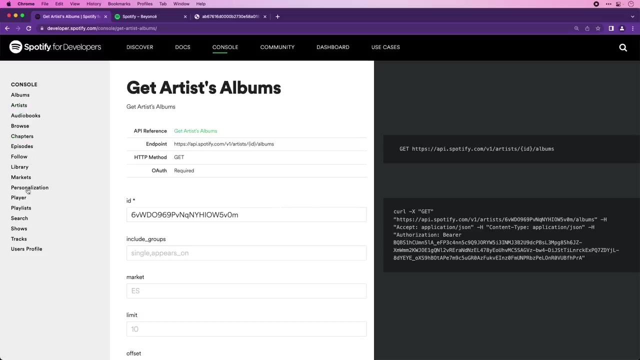 that up and let's see, there she is on her horse, her, her magical horse, there. so that's pretty cool, right? this is. this is awesome. i can get access to all sorts of information about an artist. i can get by their id. i can go and find all sorts of different things that i wanted to do, right, so, so, um, uh, if i knew. 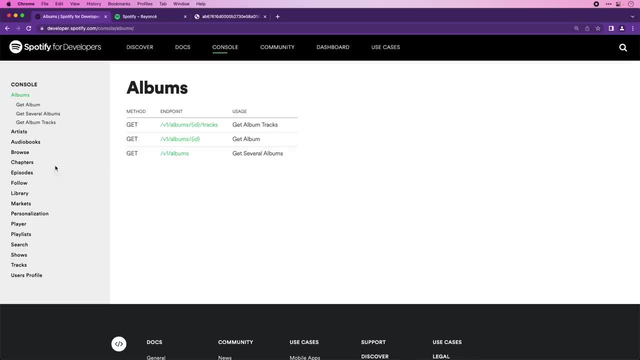 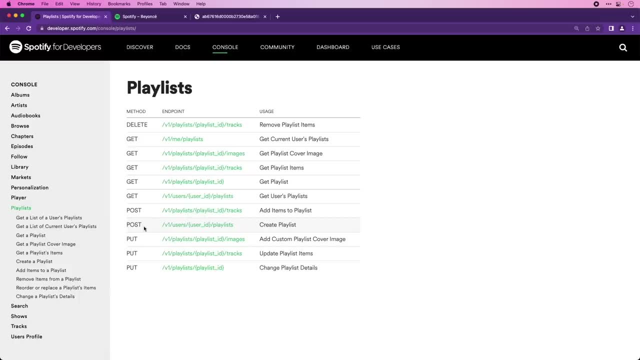 an album too. once i have the id, i could get the id. i could get the tracks, um, all sorts of amazing things. and then there's these playlists, right, so you can add a playlist. if i wanted to, i could post to create a playlist. now, of course, i need to authenticate to do that. that's a little bit. 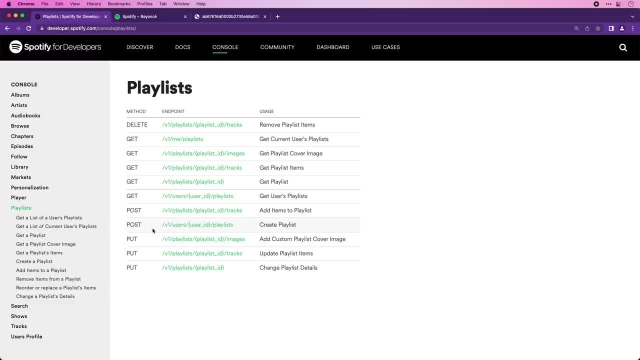 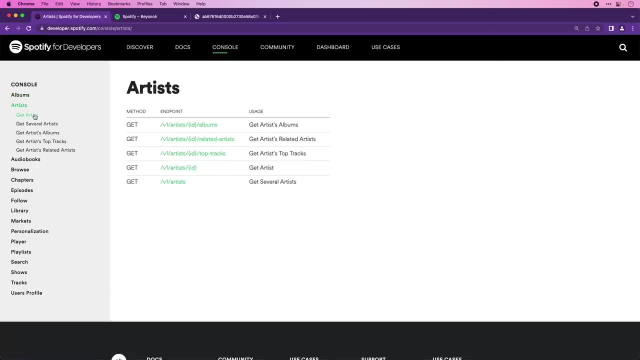 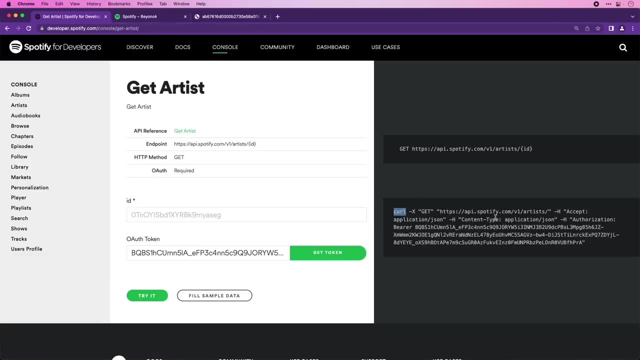 outside of what we're doing here, but i could add: um, put together a playlist for for everybody to do using this api. uh and uh again. when we are looking at the artists, um, when we're looking at this get artist, it's showing this curl command and we're going to take a look at that here in a bit. but i just want to take a little. 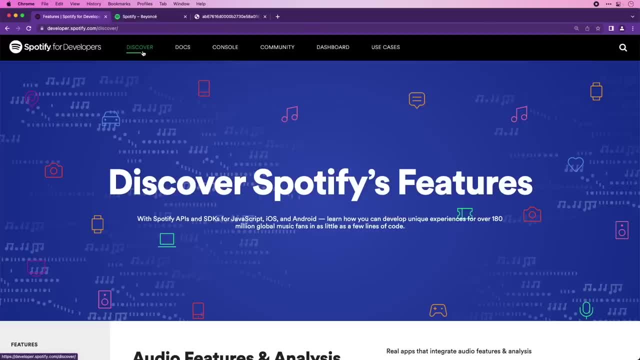 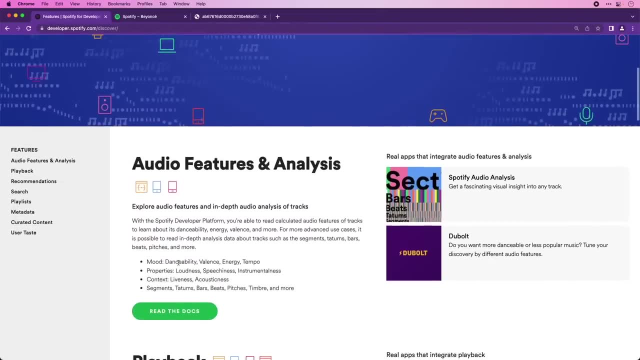 bit of time. i want you to go and take a look, go back to this discover section and kind of get inspired by what's what's available, right, so so you can look at- um, there's these different things where you can. you can- i was right- you can check and see if there's danceability of a song. you can. 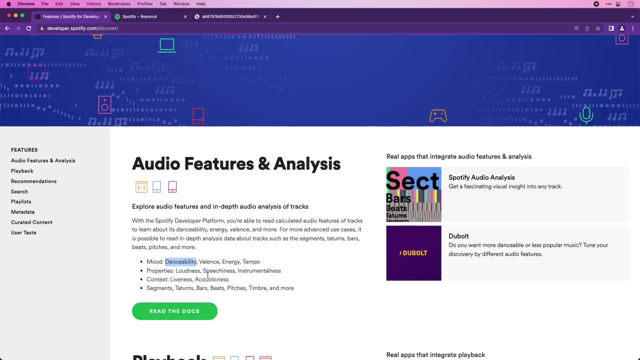 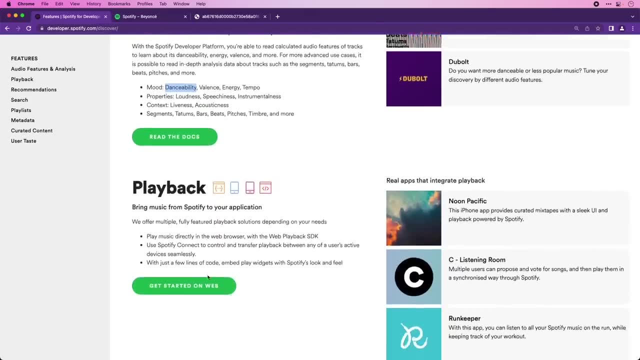 go and find a track and it is danceable. and you know that beyonce's songs are going to come back very hot and you can check and see if there's danceability of a song. you can go and find a track and the danceability, uh thing there. but lots of powerful things and there's lots of cool examples. 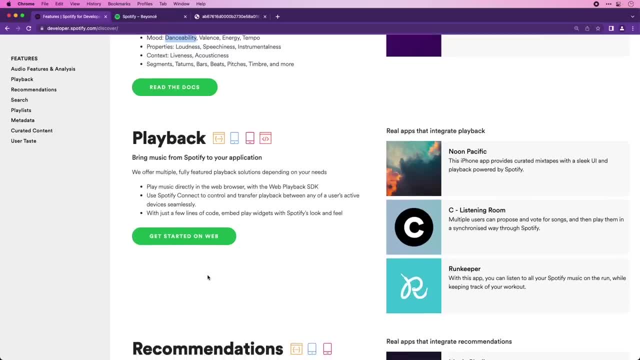 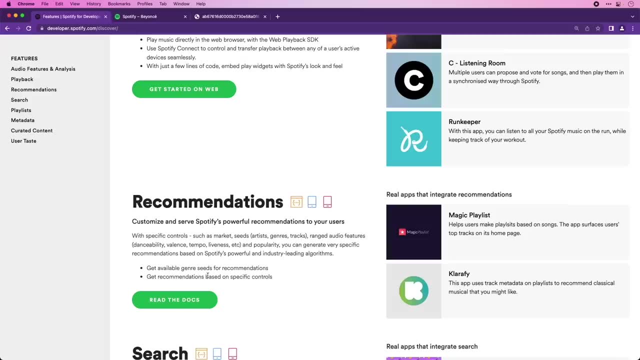 that you can do that. people have already gone and built and you can take a look at how they built it and how they use the api. uh, recommendations, this is awesome really. this is like super wide open to you and, uh, you can do all of this because of the apis that they provide. pretty cool, right, you can. 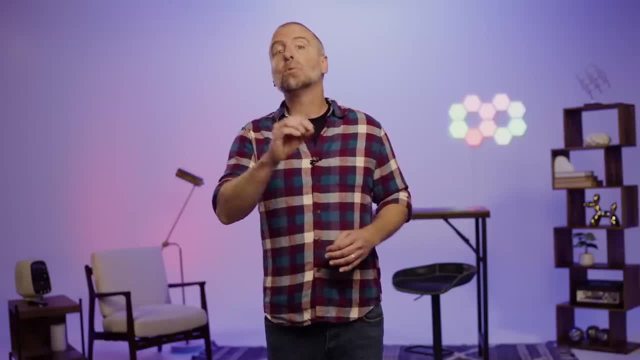 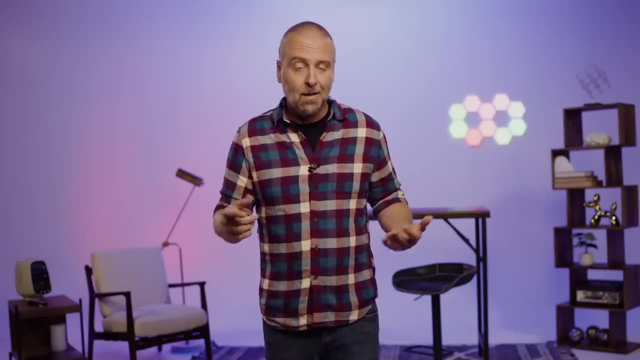 get access to all of spotify's music library and you can build tools that extend their platform. i highly recommend that you go and take a look at what i've done and i'll see you in the next video other people have built using these apis. it's super impressive. did you notice how fast those 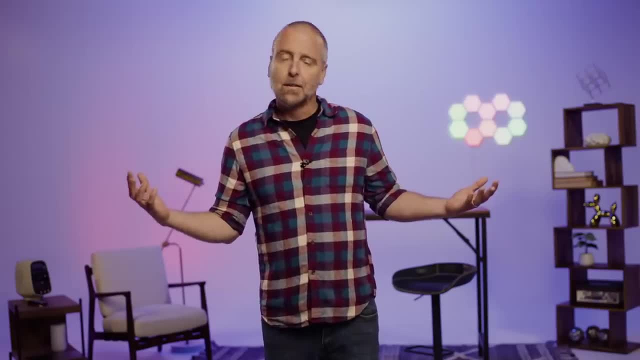 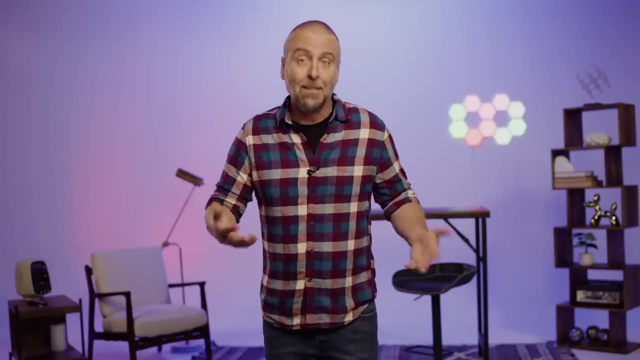 results came back. how could it do that search so quick? oh wait a second. does it even need to? those results don't change all the time. it's not like beyonce is dropping a new song every minute, though i wish she would. those results are definitely cashable. ding, ding, ding. 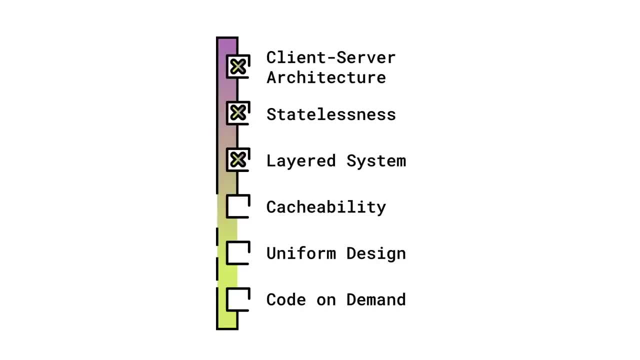 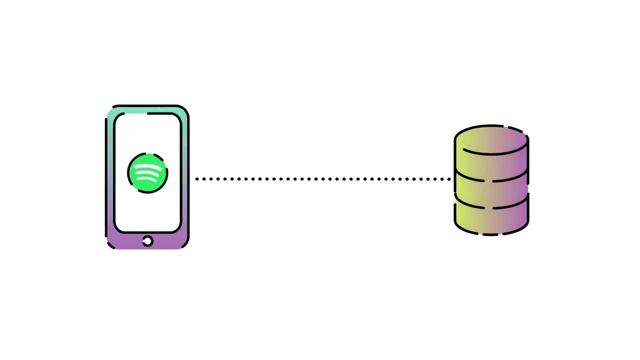 cashability is also available on the client, and we'll get to that here in a bit, but this is a great example of a layered system. i'm almost positive that spotify has set up things so that it returns the same json from its own server-side caching mechanism. 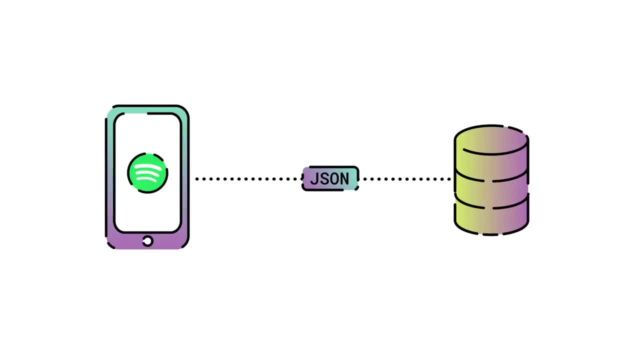 it's not rendered that on every single request as a user of the api. i don't know how it's doing that and, frankly, i don't care. i want it to be available and fast, when i hit that specific url. beyonce definitely appreciates how fast the results are returned. she might even take that. 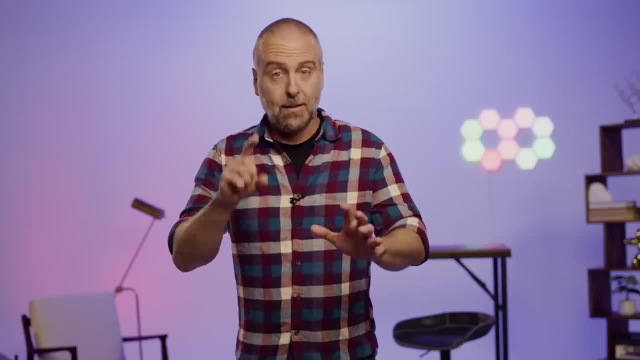 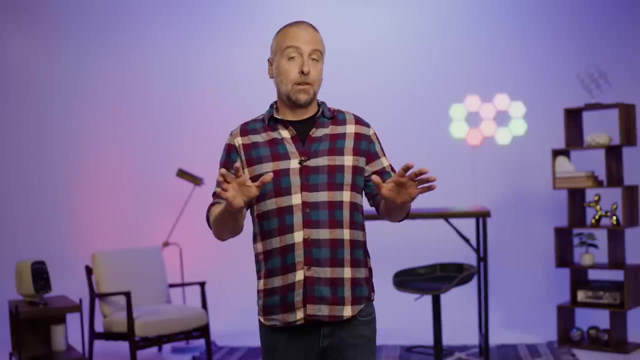 api dev to red lobster. let's go ahead and take a quick break. during this break, i'd love for you to move around and think about what you might be able to build with that spotify api, for instance. while i was using this api, i had this idea pop up when i'm at a music festival. 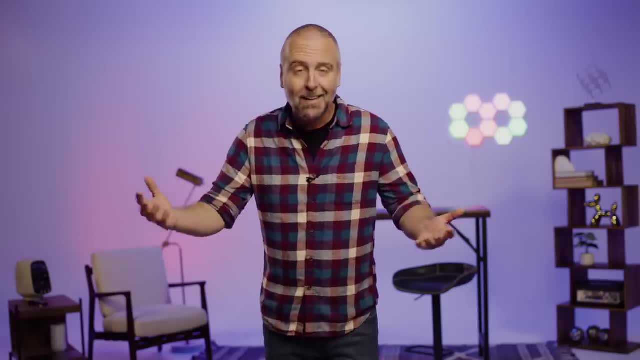 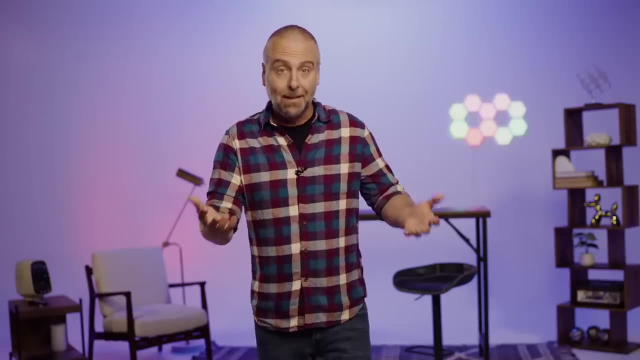 i often have a hard time deciding which band i should go see. there's so many. now i would love to have an app suggesting me which of the bands that are currently playing i would most likely enjoy. you know, based on my listening habit, i'm pretty sure that you could build that just with 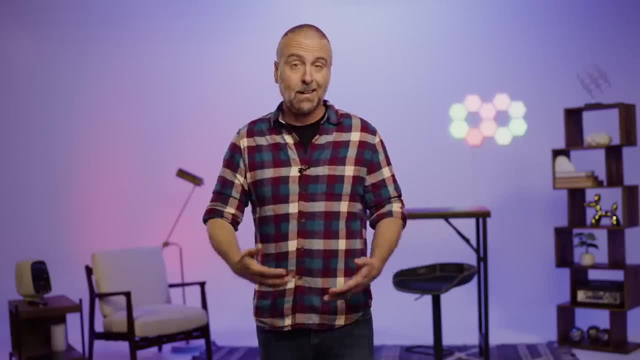 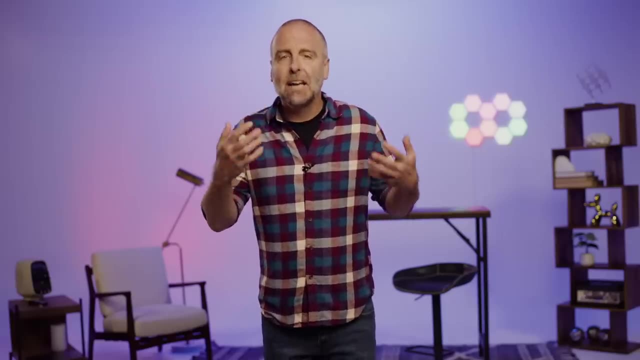 the spotify api and using a list of events of the bands that are performing. and if you do end up building that, share it with me because i need it. what other interests do you have that provided api that you can use? check the notes for more ideas now, after you come back from your break. 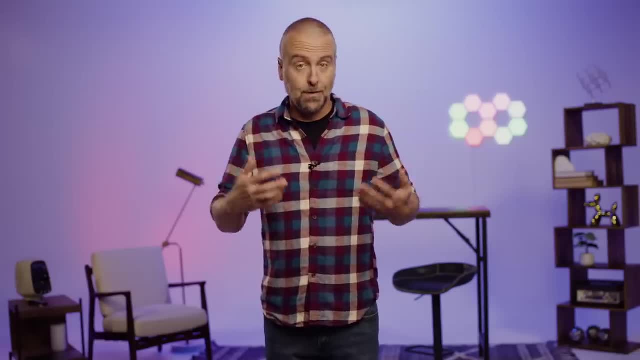 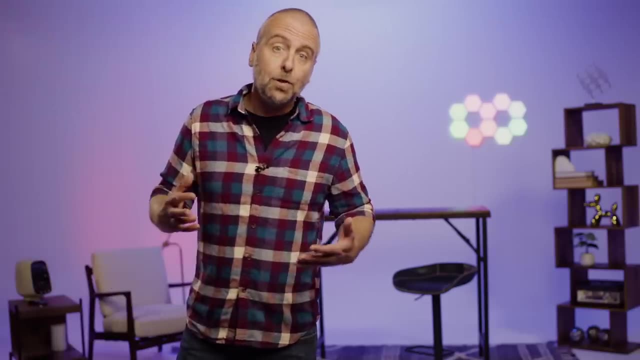 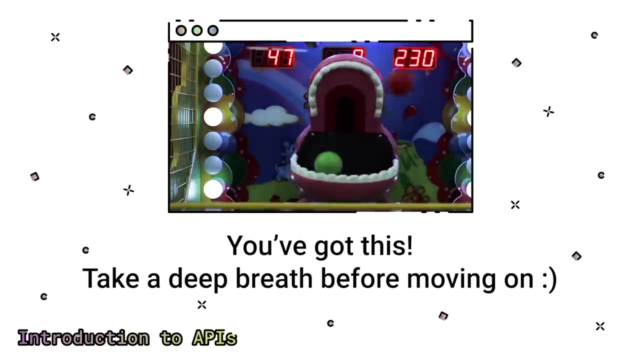 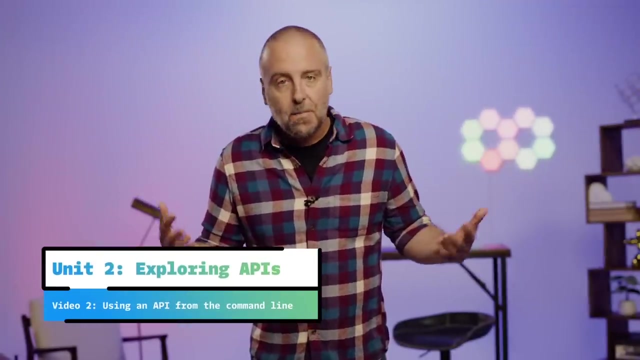 let's dive a little deeper and make use of an api using our own tools. see you soon. no, really, take a quick break seriously. it'll do you good. no binging. well, i realize that exploring an api on a website is informative. it might not feel like you're. 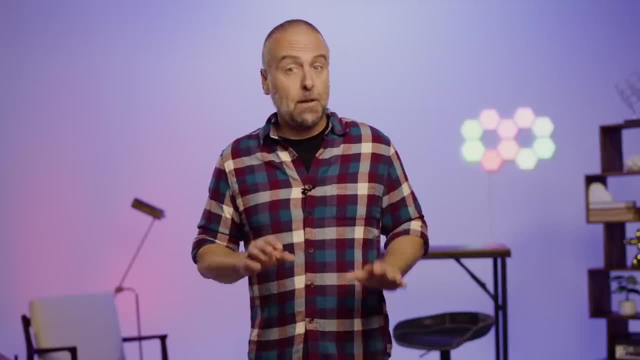 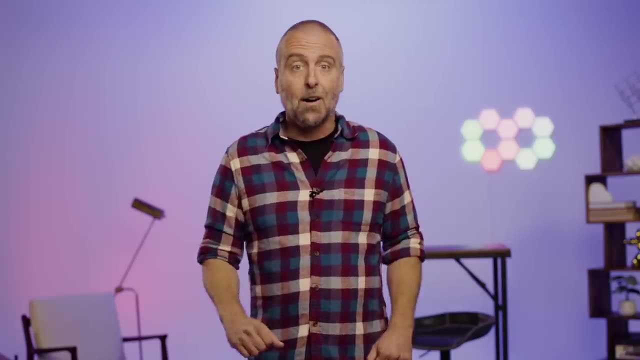 actually using that api. i think the next logical step in exploring is actually making that request yourself from your computer, not from a website. now, as i pointed out in the spotify docs, there were examples that were using a command called curl. curl is an open source tool that is used. 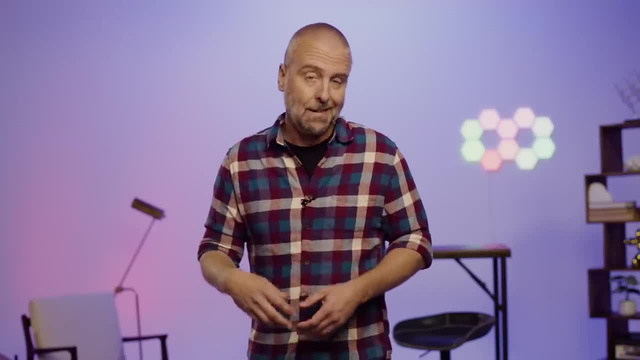 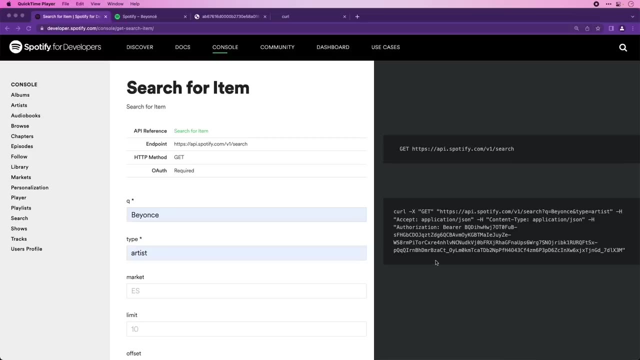 to send data back and forth and it runs locally on your computer. it's awesome for poking around at apis. what do you say? we explore it a bit. okay, so we are back here on our spotify page and we say that there is a command here that says curl. curl is a command that we can run from our terminal. now, if both of those terms are, 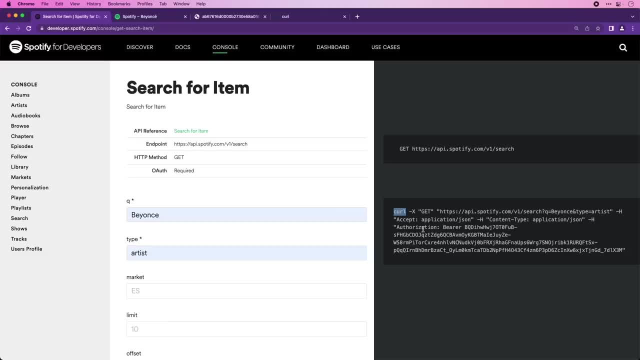 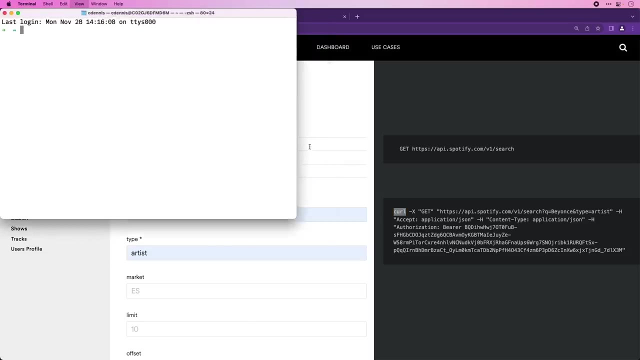 new to you: command and terminal. this is a great time to head over the notes and learn about what the terminal is. so my operating system is a mac and it has an application on it, uh, called terminal. so i'm gonna open that up, terminal and in fact i'm gonna make this a little bit bigger. let's go. 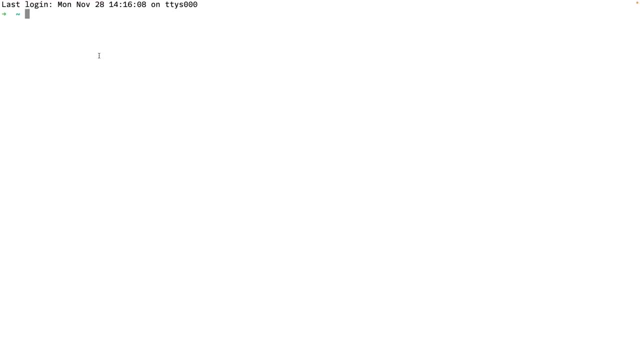 ahead, let's. let's let it take up the whole screen. we're gonna be in here for a little bit, so i'm gonna type clear and clear my window, all right. so, um, uh, this terminal allows me to perform actions on my computer like i can make it do text to speech, i can do say, and i can say: hi, mom, hi, mom and it. 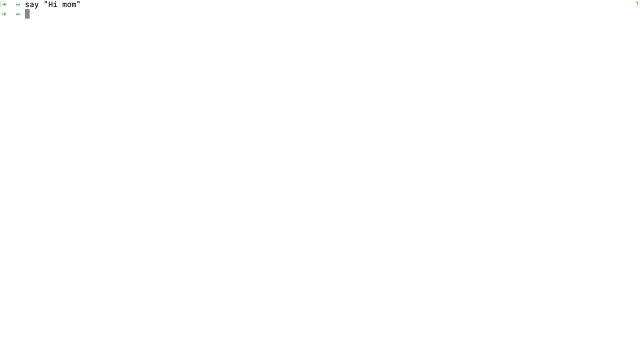 says hi, mom, um, uh. and the windows operating system has a terminal as well, and while it's a little bit different from what it's supposed to be, it's a little bit different from what it's supposed to be, but check the notes for more on this. so what happens is i write the command. 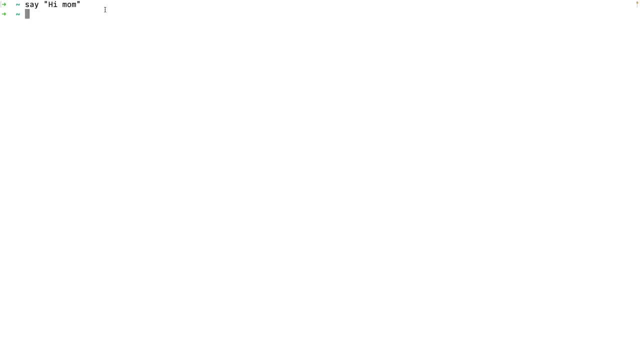 and then i pass in values for the parameter. in this case it's hi, mom. now note that i used quotes there because i want to pass one value even though there's a space. if there was a space, that's kind of how you separate things, but with the quotes it's saying: this is one. 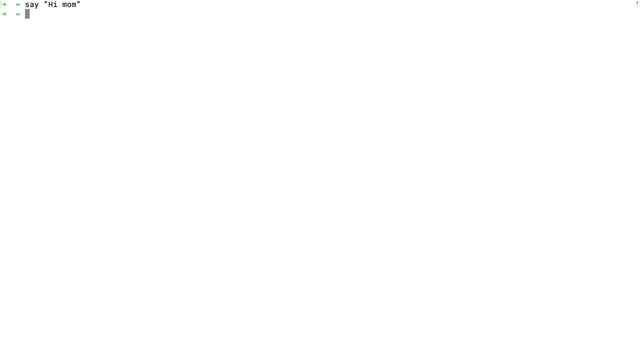 value that i'm passing in. we developers spend a lot of time in our terminals, so if this is new to you, i want you to remember that it was new to everyone at one time. so please take your time and don't let this get you too frustrated. you've got this. 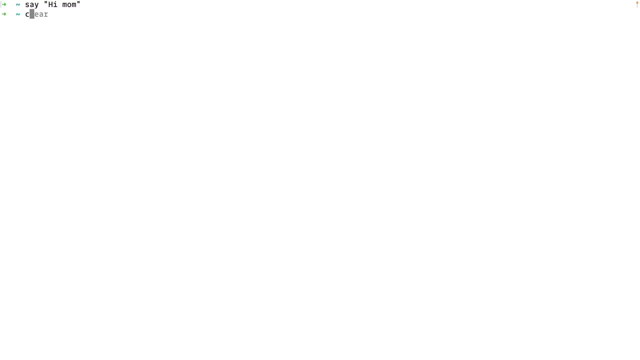 so i already have curl installed. i'm going to just go ahead and make sure that i do by typing the word curl, and if i see this, i can see that i can type curl and then the command dash, dash. help now, if i didn't have this installed, if this came back with like i don't know what you're. 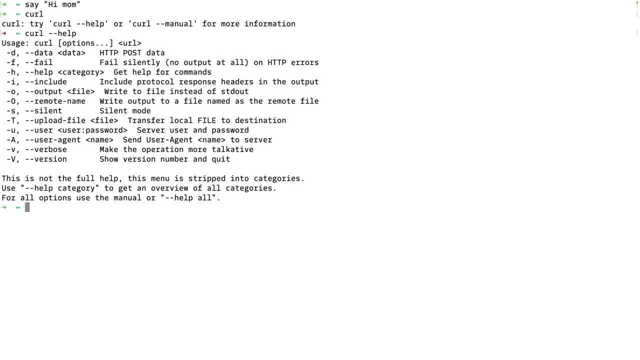 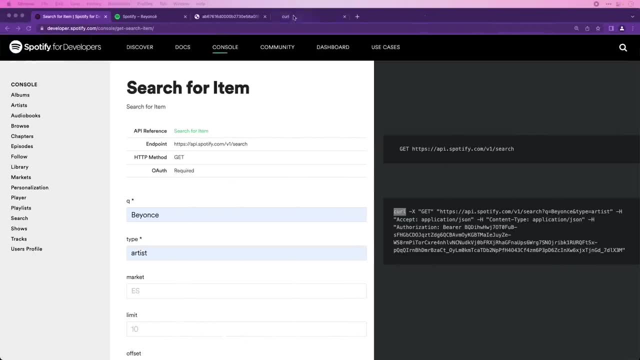 talking about when you type curl, the word curl, uh, that's okay. so, um, uh, we're gonna head over to the notes, uh, and you'll get sorted there, but the starting point- we're why i want you to go- is curlse, so you'll come to this page. you'll see, this is a command line. 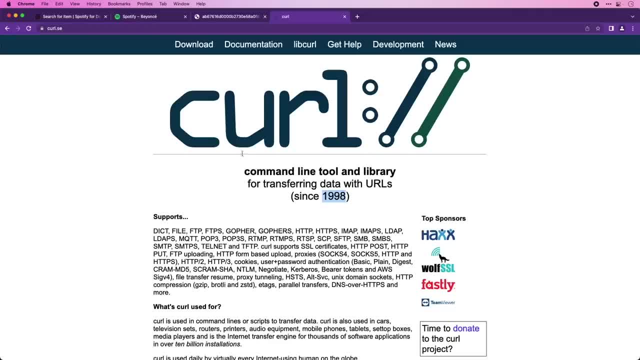 tool in library for transferring data since 1998.. that logo sure feels like that, doesn't it? uh, it does all sorts of things. what we're really concerned about is this http right. we're going to use this from the command line to get access to a url. so if you don't have a curl on your command, 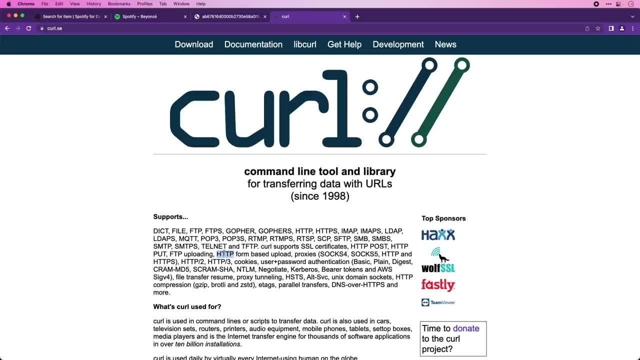 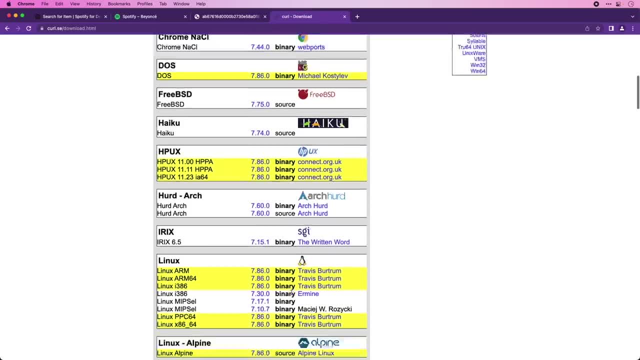 go ahead and pause me and check out the notes for the best way to get this installed on your computer. you'll see that there's different- uh uh- operating systems. so you've got your linux and you've got your mac os and if you come down here, you've got your windows. so there's different ways of getting. 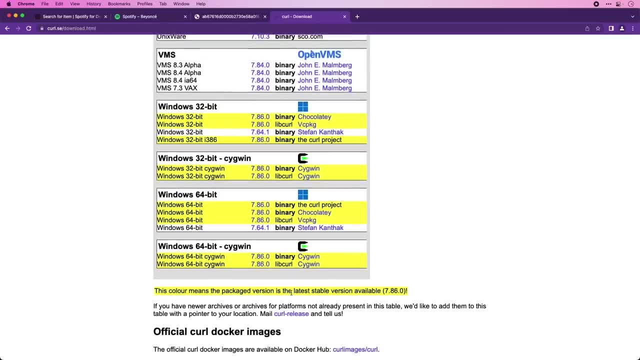 things uh installed. so go ahead, take your time, get that installed and when you come back, um, i want you to try this. i want you to do this thing with me. so i'm going to go back to my terminal and i'm going to make sure that it works. uh, the way that i always like to test is: i like to go to 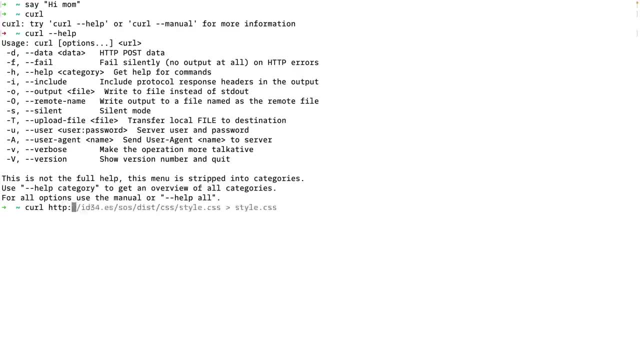 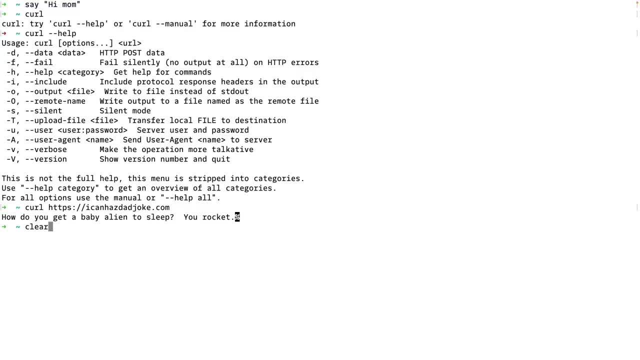 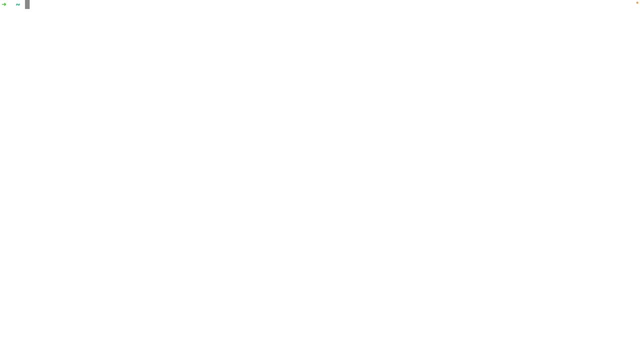 you do that, um, that'll let you go and it's going to hit that website and it's going to give you back a joke when you're ready. so now that we've got our curl up and running, we've got our successful dad joke, let's go ahead and run that command from spotify. so i'm going to come back over to my 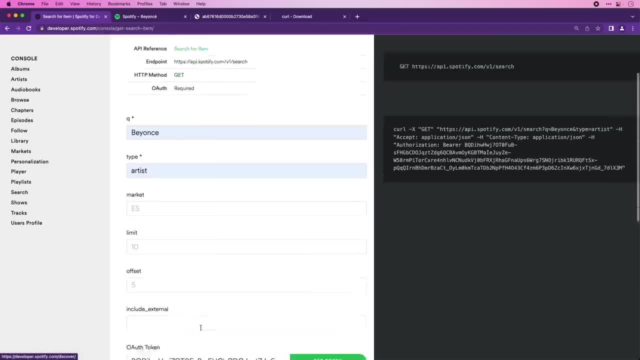 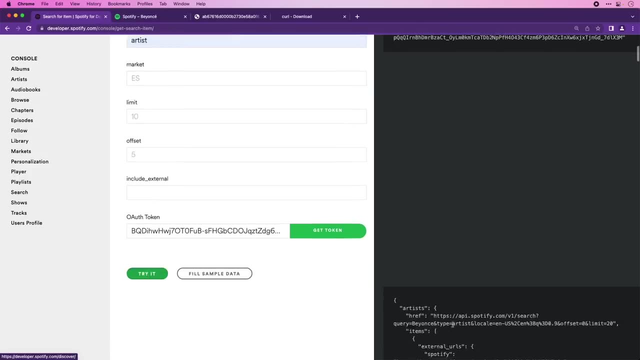 spotify thing where i was running the search. i'm going to make sure that it's still working, actually get started, because these, these tokens can expire and, depending how long your break was, i might have expired, but mine is still working, so i got this back here and i should be able to. 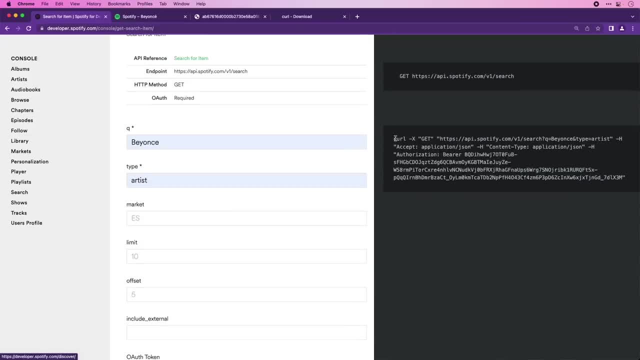 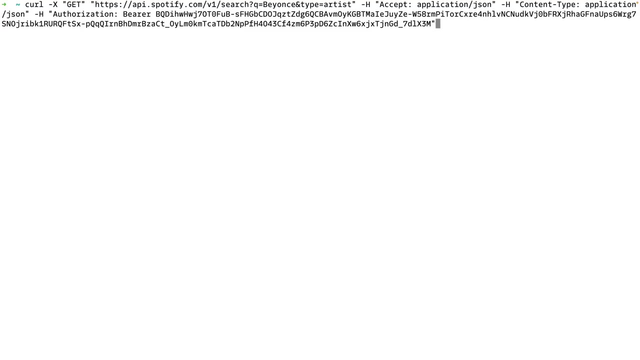 get this from my command line and what i'm going to do is i'm going to copy this and i'll highlight this. this is a uh development practice known by us developers, known as copy pasta. so i'm going to copy this and i am going to go back to my terminal and i'm going to paste um in this long 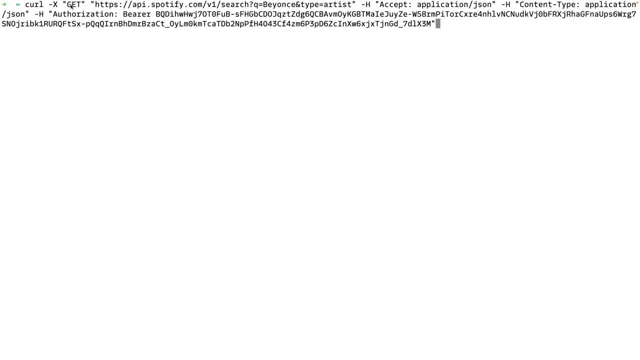 list of things here. what this is doing is saying: hey, i want to make a get request to the apispotifycom forward slash v1 search. remember that's where we were at. we were searching and we're passing the query string of beyonce and the type of artist and uh, we're. 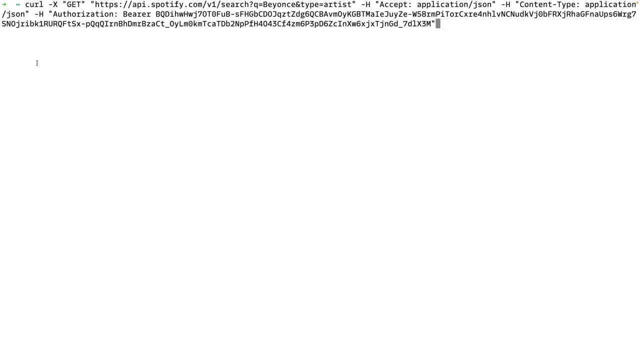 telling it: hey, i would like to get back. uh, json, and i am sending you json, even though we're not actually sending json. the default has that there and this is the important one. this is sending you a header, right, the dash h is a header and authorization, and this is that long token. 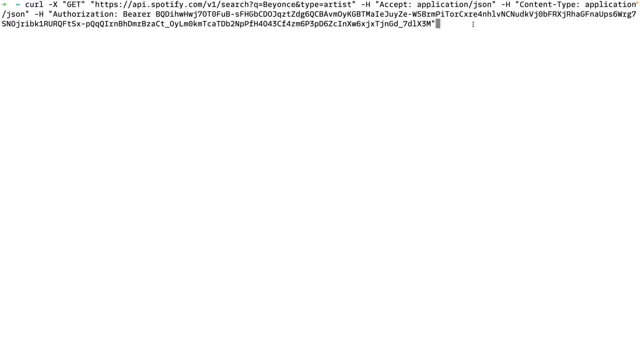 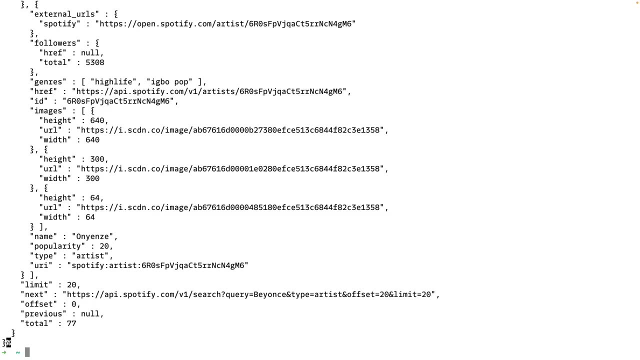 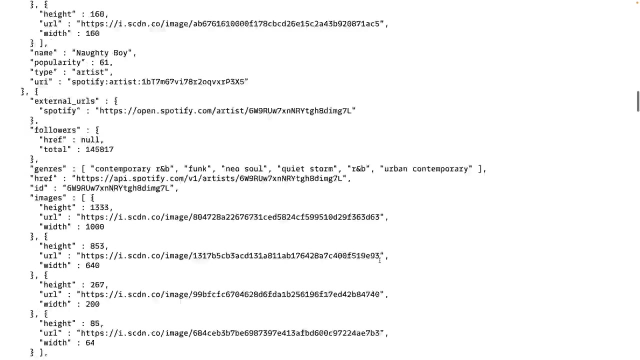 that we had there. now, if all is working, when i press enter, i should get here locally on my machine that uh same list of data that we did, and i did check that out. so what i'm going to do is i'm going to come back up here and i am going to grab: wow, there's a lot of information here, right when. 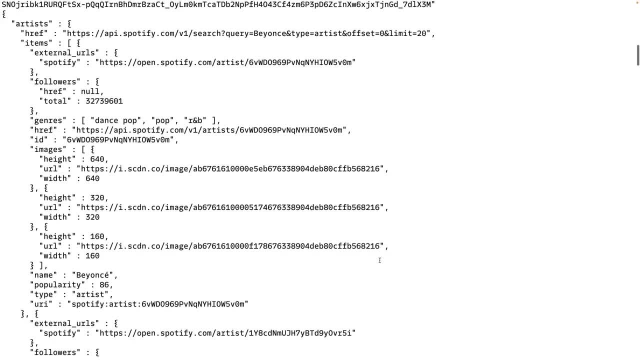 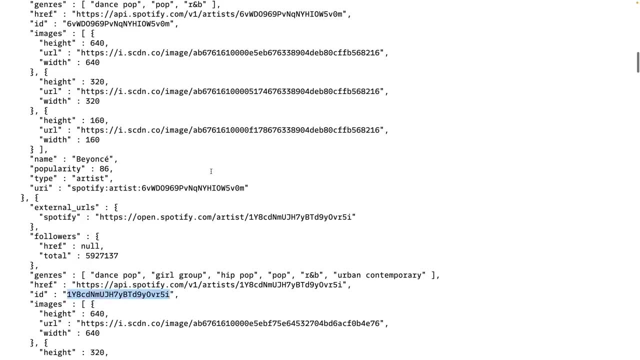 this comes back. i'm going to grab uh her id, and so i remember that when we were looking at it it was down in here. this id, is this the right one? is that the first one? so we got items? uh, no, this is her id here. this is her idea. it starts with a six. 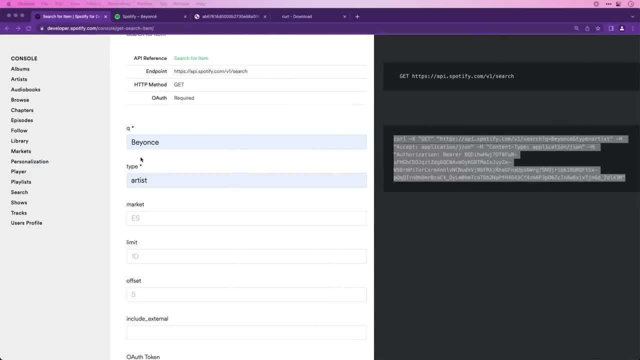 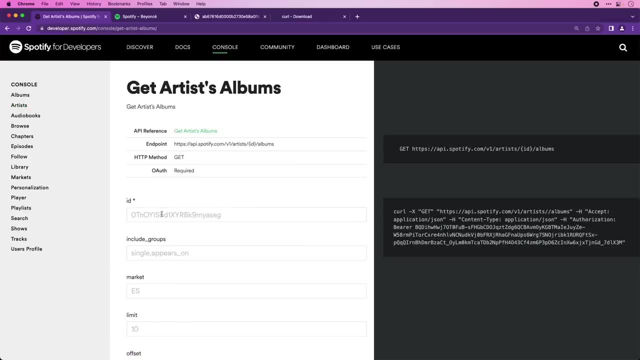 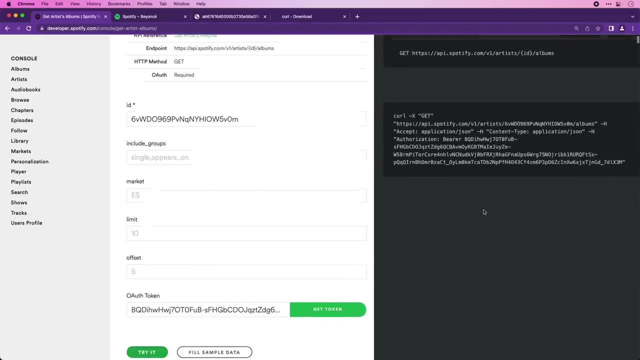 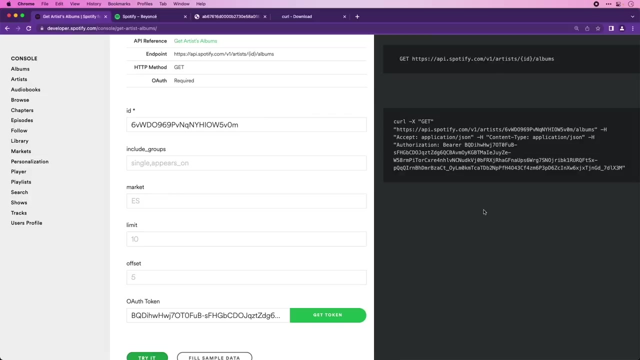 double comma: zero. beyonce is head. uh, another little need, a little bit inside o. so now that we have the data here, i'm going to go ahead and copy that and i'm going to use that. i'm going to go back and remember. i'm going to go and i'm going to look. i want to see what, um, what albums. 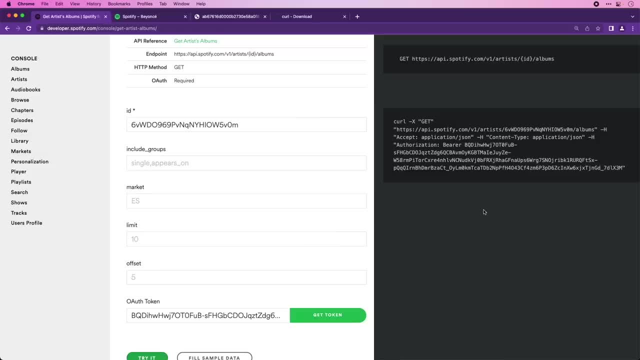 albums on your local machine. So here's what we'll do: You give it a try And if you, once you get it, once you get it printing locally on your machine, you can let me know And then unpause me and I'll show you how I did it. Okay, Are you ready? You got this, Pause me. 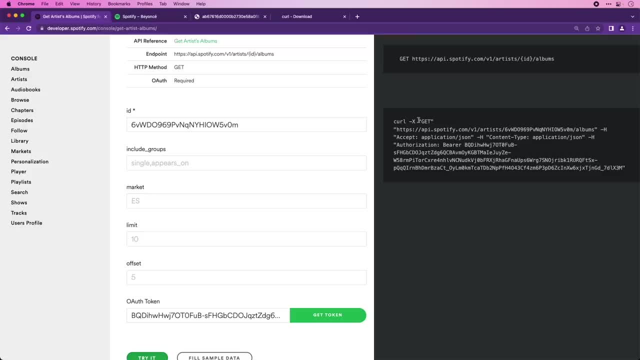 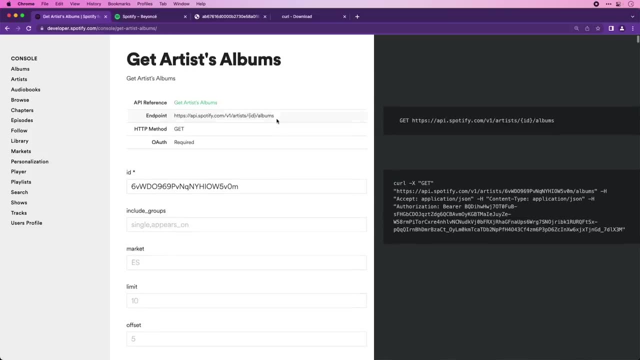 Cool. So how'd you do So? here's probably one way that you could have done. it is just copied that right, Copy this whole thing and pasted it. But what I want to show you is that we have access to, we know what these, these, these URLs are right, So we know that there's this V1. 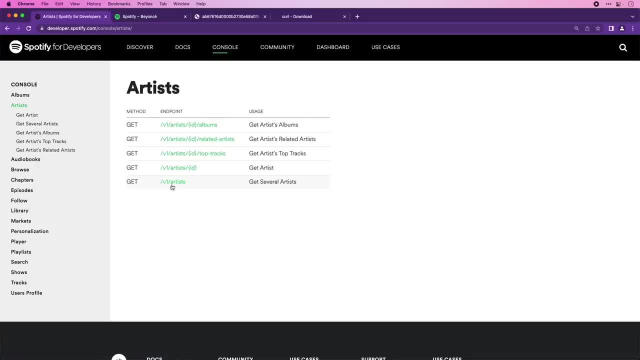 artists And in fact, we can see that there is a get of slash V1 artists and then you can actually pass their ID in the in the URL there. right, That's what this ID is here. So let's, let's just. 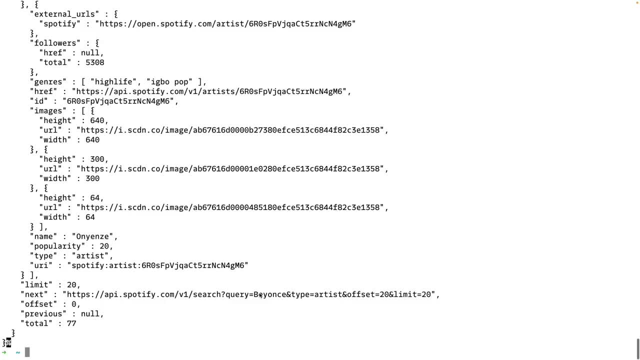 go back. I'm going to show you a little trick too. So I've I've got her ID copied still, So I could have just just ran that query and copied the curl and pasted it here, And if you did that, you did. 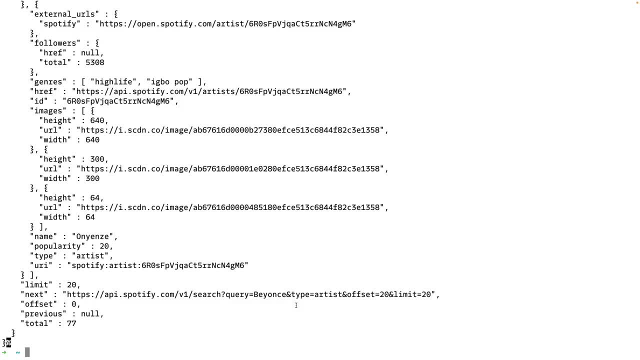 it right. I just want to show you a little bit more of what else, how else we could explore. So I'm going to press the up arrow and you'll see. um, my cursor is moving here. Um, I'm going to press. 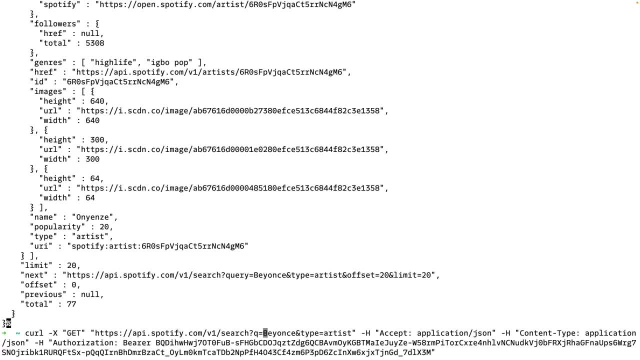 the option key on Mac. I think you can press the alt key on windows. You can jump around like this and I'm going to get rid of what's here and I'm going to say V1 artists- right? So that's the collection of artists and I have that specific ID, right? So there's the ID, Uh, and I'm going. 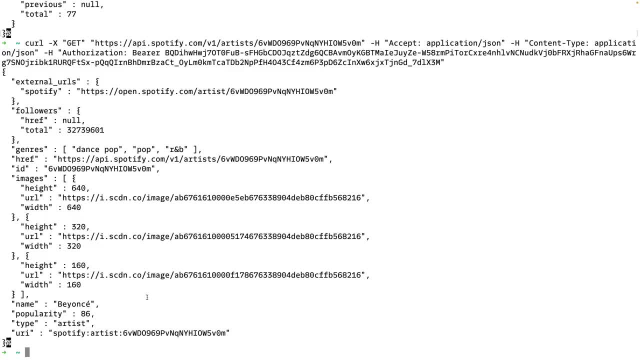 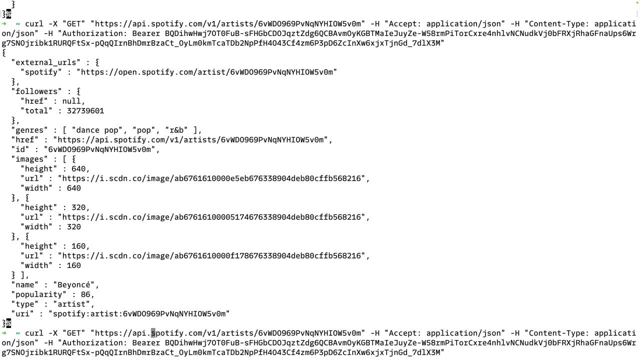 to press enter here and you'll see that I got back Beyonce, which is awesome. That's what I did. And then remember the artists have. I'm going to go to the front of the line. That's control a on a Mac, Uh, and I'm. 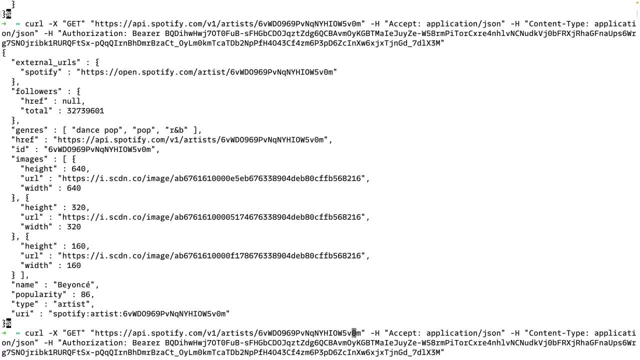 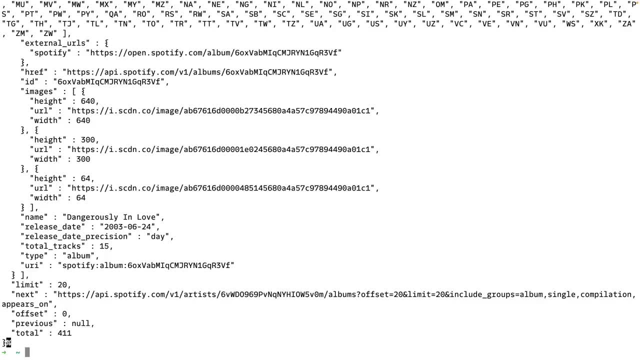 going to switch this. So artists have- uh, this is specific artists, So Beyonce, and we want to see Beyonce's slash albums, which is what the console would have generated for you. But I just wanted to show you that you can kind of navigate and move through and you'll see that there's a, there's a. 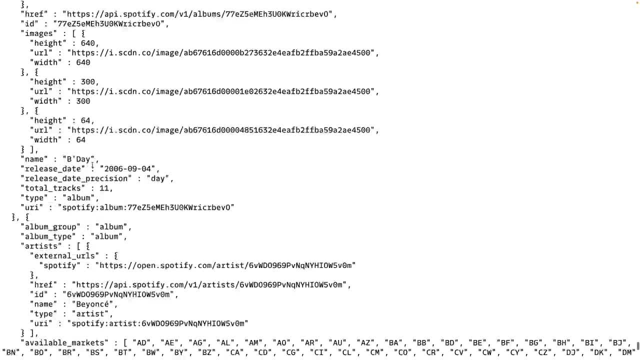 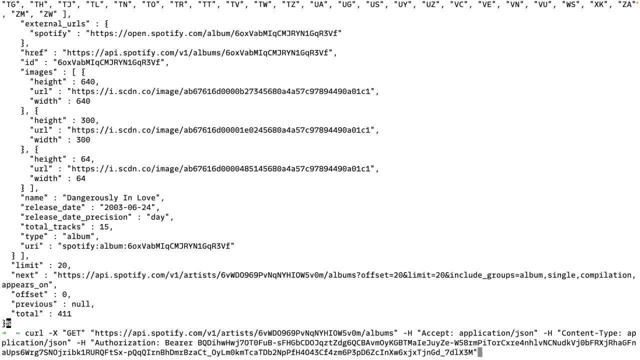 bunch of different information that comes through here. Um, it's kind of hard to see, right, So so, um, kind of hard to parse, And this is something, optionally, that you can do: Press the up arrow and I'm going to press, pipe that into a tool called J Q And, uh, you'll see. 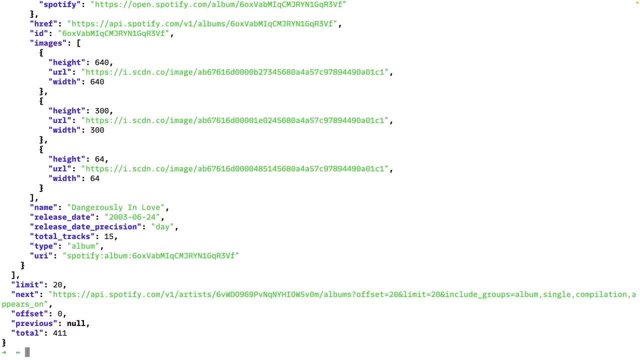 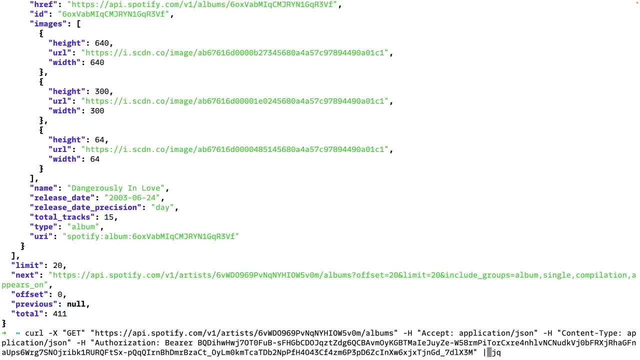 that it comes back very nice and pretty right. So, um, this is something that that is very nice to have. Uh, and I piped that, that's this, this, uh, the symbol above, uh, the, the enter key is: 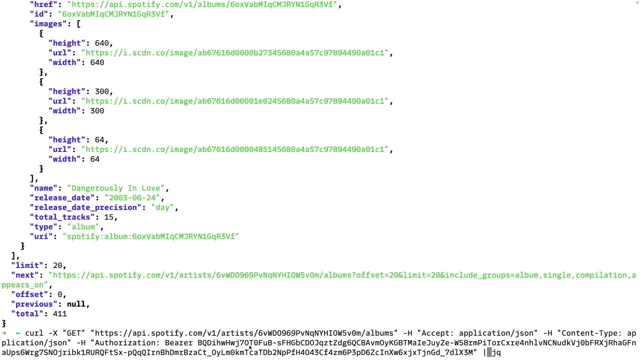 this pipe symbol and it allows you to take whatever happened in this first part of the command and take its results and put it in this part of the command, which is super cool. Um and again, this is in the notes. You don't need to. you don't need to worry about this, but I know. 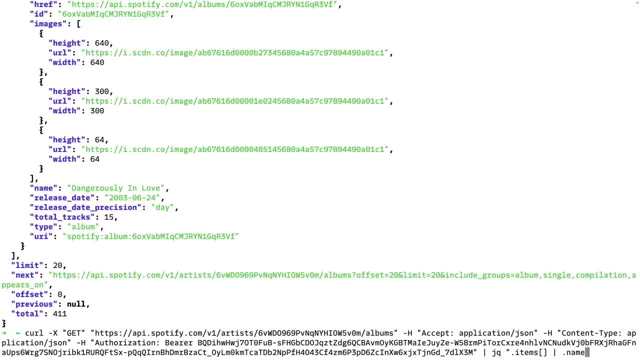 I can query things, So I can say that of the items I'm only interested in the name, uh, the dot name from each one of the items, And this is a little query language that's attached to this JQ uh program. You don't need to do this, This is just something. if you're doing it from the 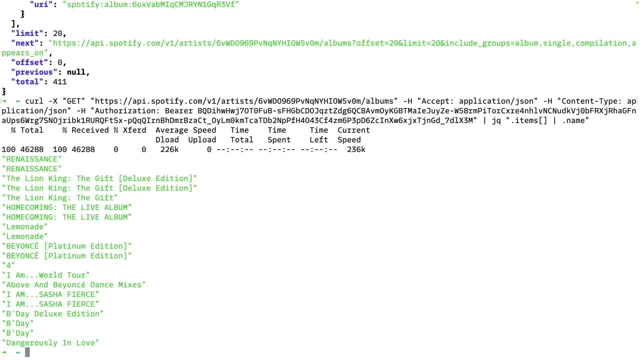 command line. it's something that we do that we could kind of hack around with a little bit And you'll see, I can get all the the lists of her albums And that's pretty cool right. That's powerful. And if you are going to just start poking around and moving around with the URLs, 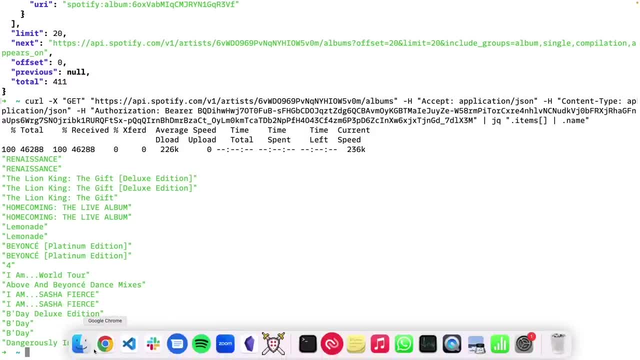 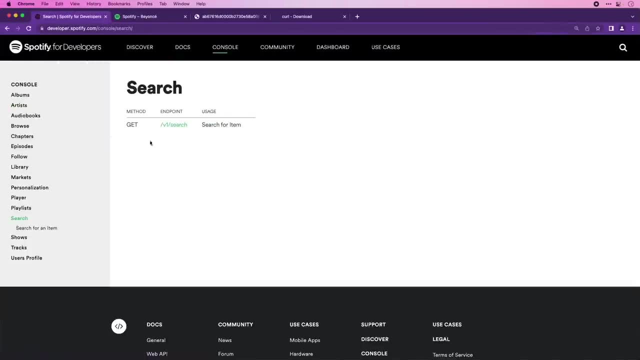 one thing I wanted to make sure that you're cautious of is, if we come back a look at, uh, the the console page here, they do a nice trick for you for back here in search, Like one of the things that I want to make sure. uh, I know that Beyonce has this song, That's. 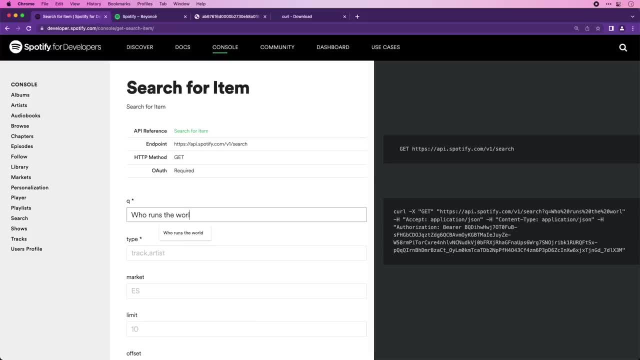 like something like: who runs the world, right, Who runs the world girls, but I don't remember where, what album it's on, So I'm going to search for a type track And now note that my query has spaces here. Now, what's happened here is it's done this uh URL encoding, So like if you were trying to. 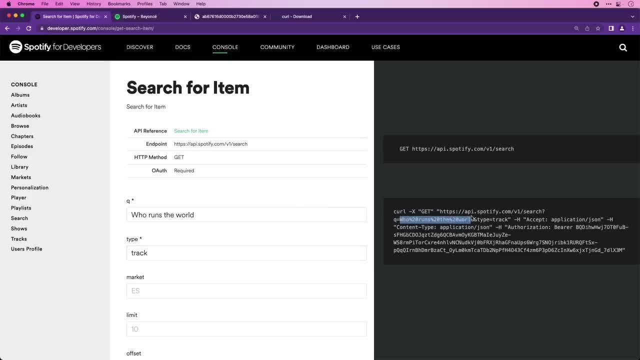 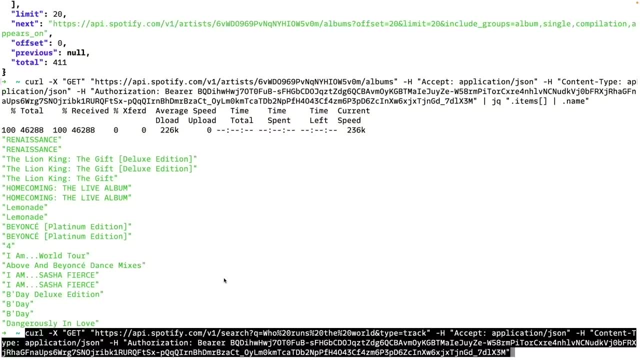 to mess around and work with the search. you'd want to make sure that, whatever you did, you passed that uh with those, those plus signs there. So I'm going to run that curl command and we'll see who runs the world girls, And I am going to- uh, I see there's. 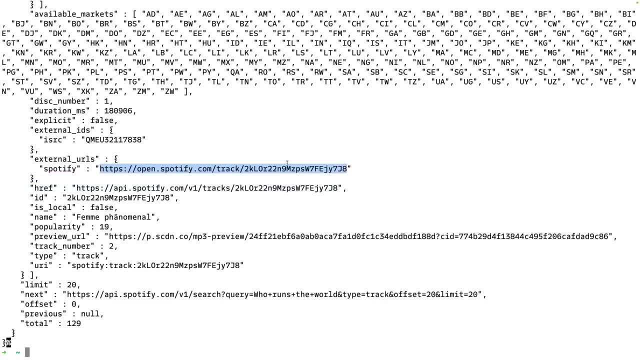 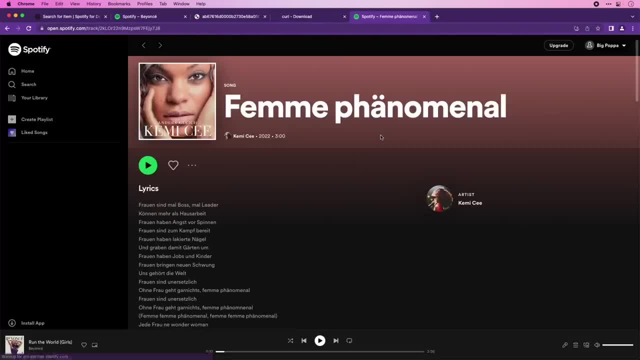 this, uh, this open link here. So I'm going to go ahead, I'm going to open that. Let's take a look, Uh, and make sure this is the right track. I'm pretty sure it is. It is not the right track. 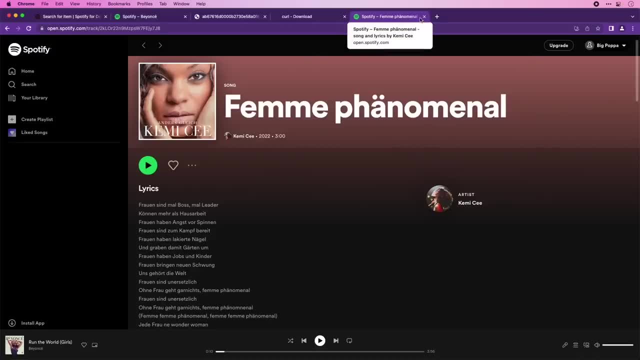 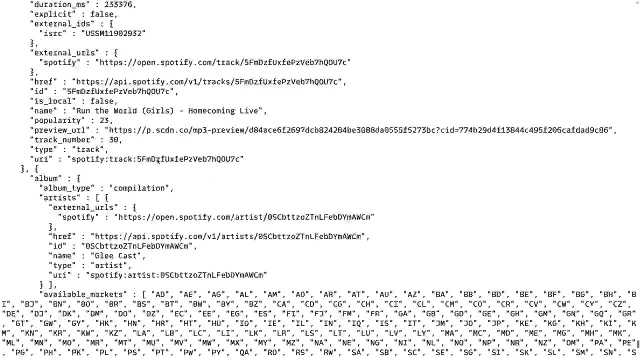 What is this? Maybe it, maybe it's some other, some others, So let's take a look. Well, that that's interesting. So, uh oh, I just went to the bottom instead of going to the top, So I should have went to the very top of these results. 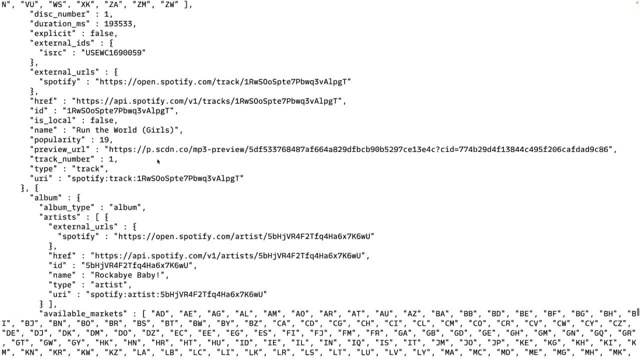 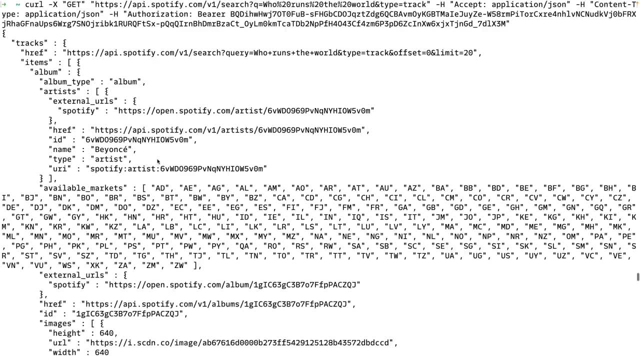 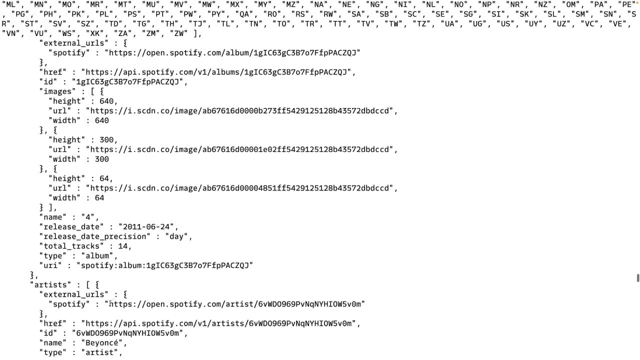 or I should have pulled- probably pulled- the name out: Rockabye baby. There's a rockabye baby version of this Whoop. Okay, So when the color stops if you're not getting sick all the scrolling. So Beyonce is the artist that we want, So this is the one. we want to hear this song, Let's see. 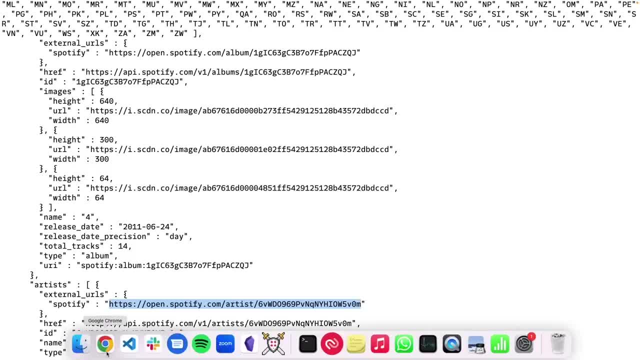 if I got the right one this time. That's just something. you know. there's a lot of data coming back here, So let's see if I got the right one this time. So let's see if I got the right one this. 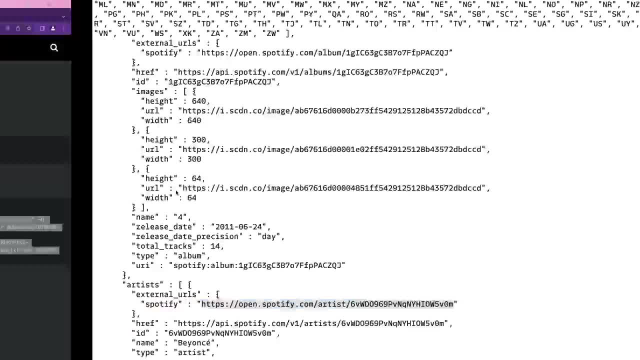 time So you can start your song on an advanced version of the start. It's, it's really easy. It's kind of hard to do to use on the command line. Sometimes I'm a little klutzy, like you just saw. Here we go. Let's, let's see what happens, Let's make sure this is it. 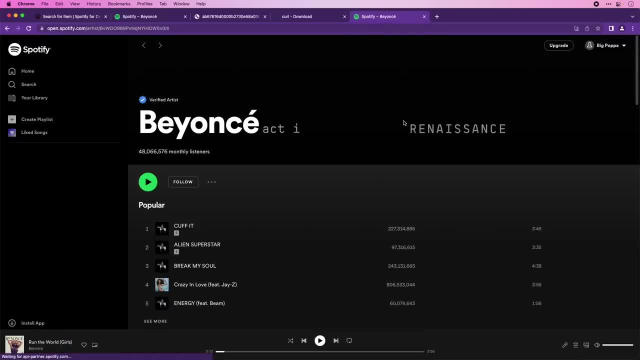 There it is. There's Beyonce. not the song I was looking for. Oh yeah, it is Who runs the world girls And now I can listen to that. So it's like who runs the world girls. It's kind of like who runs the terminal curl Boy. that was a. that was a big setup just to make that. 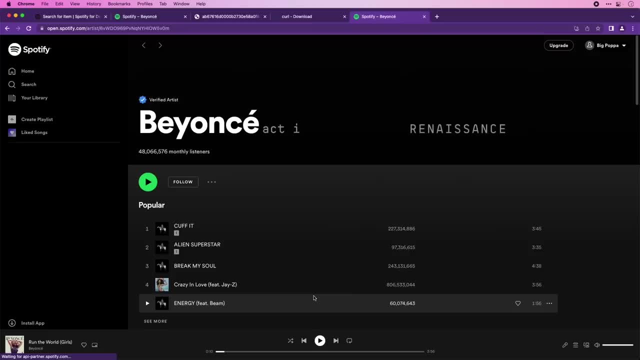 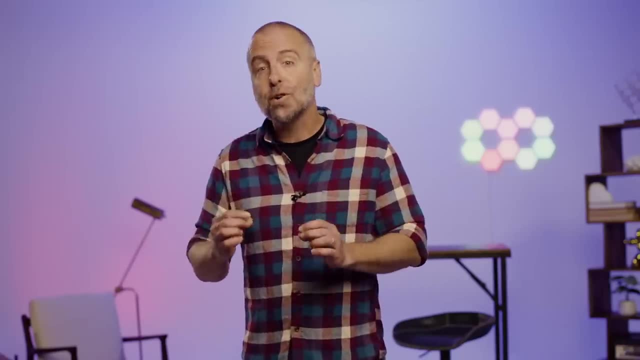 joke. I hope that you enjoyed it. You can have dad jokes. curl is an awesome way to explore apis and you'll find that often, just like we saw with spotify, apis will use curl in their docs to show you how they work. spotify is just one api and there are 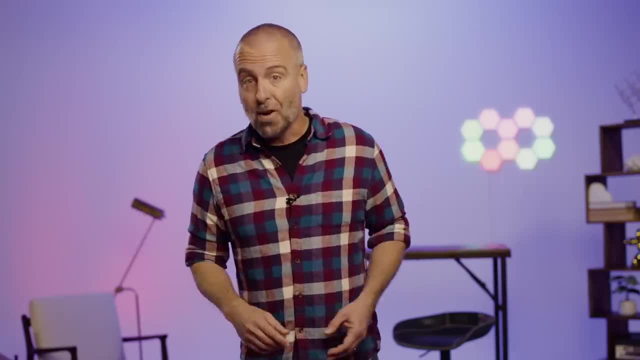 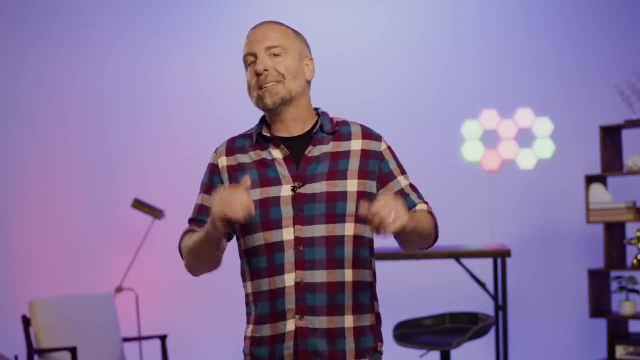 so many companies and services out there. in fact, some apis are the product like. that's what the company's selling to us developers. so now that we've been building up those muscles, why don't we take a swing at another api? let's use a different api this time. let's use twilio- twilio. 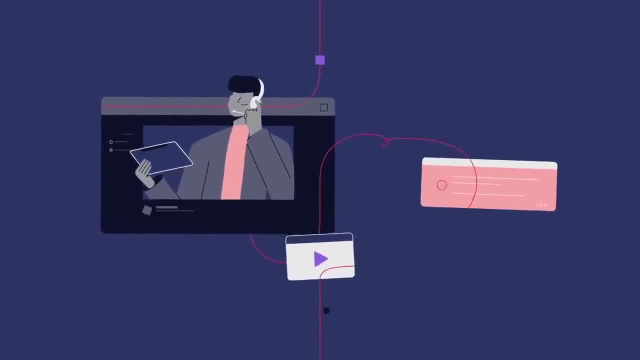 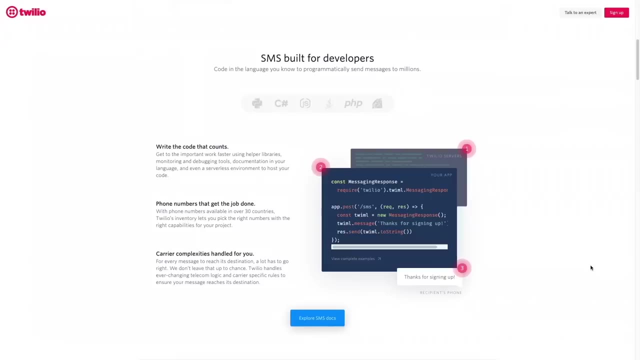 is a company that loves apis. in fact, that's what the company started as more than a decade ago: just a set of apis. it started as abstracting away communication channels, and by that i mean any way you'd ever possibly want to communicate with your users. want to send a text message? 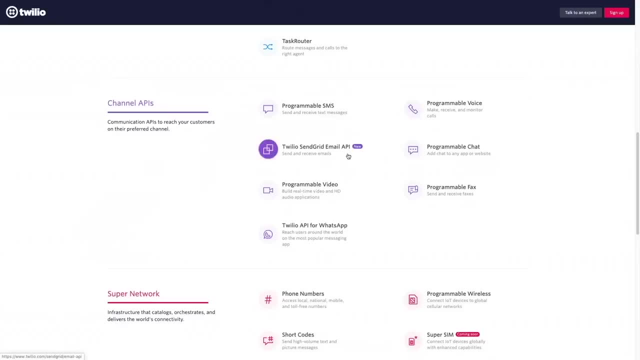 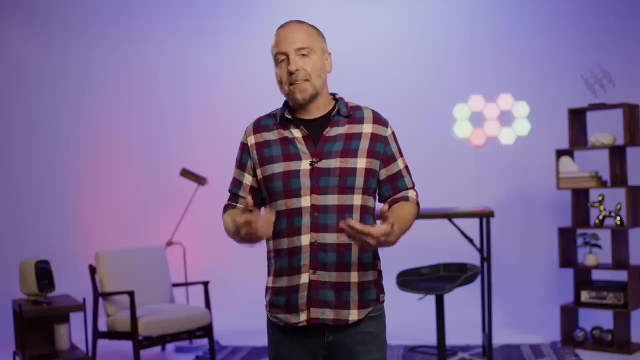 there's an api. call for that. want to make a phone call? there's an api: send an email, a whatsapp message, literally whichever way you want to communicate. there's an api for all of them. developers embed these apis into their apps and i'm pretty sure that you've probably used it. 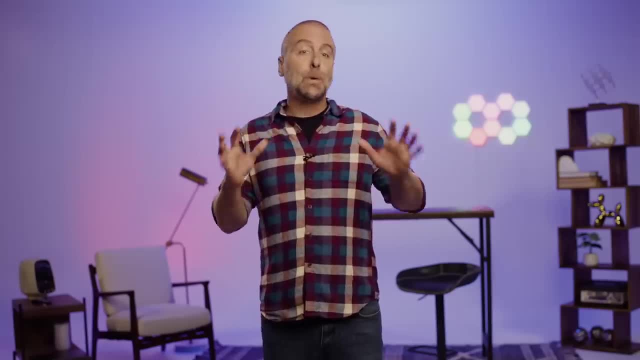 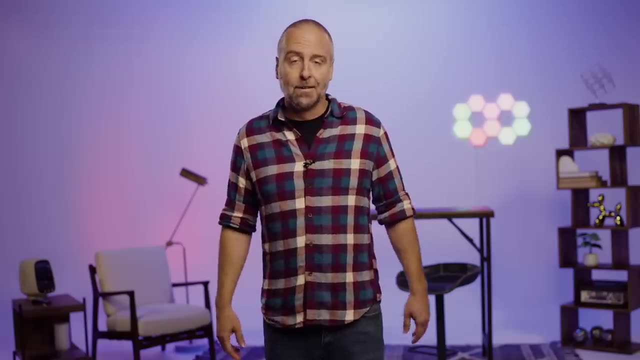 without even knowing it, you were. now nowadays there's a whole suite of products that twilio offers that they saw their customers needing, but under the covers it's still these apis that are powering everything. i need to be a little up front here with you. i love twilio. i mean, i love it so much i even 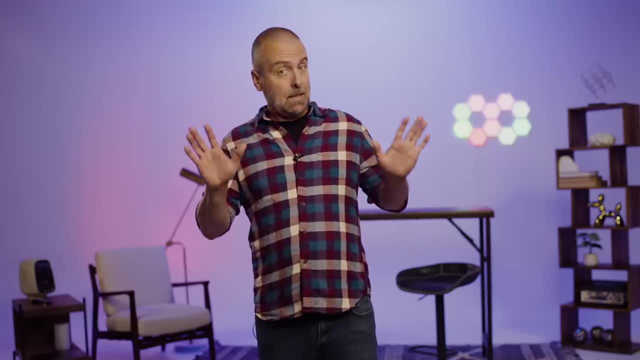 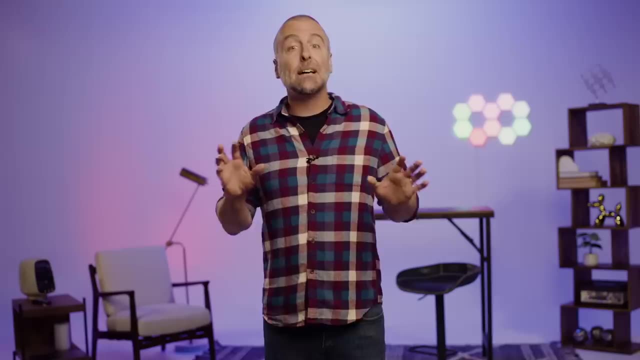 applied for a job with them and i got it. but even if they didn't hire me, i know that i'd still show off how powerful their apis are. i mean, with a single command you can send a text message. i remember when i first did that i was like wow. 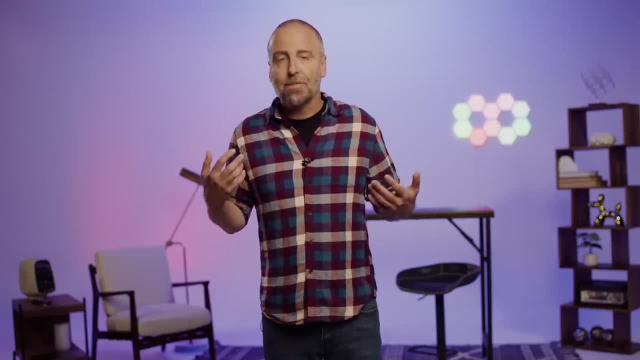 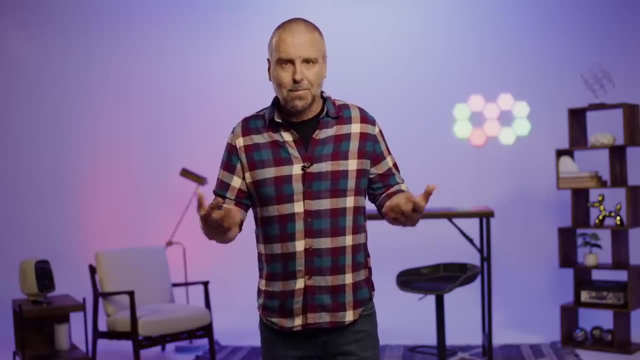 like that level of abstraction is amazing. i mean, if you've never thought about it before, what even is a text message? i mean, i know i have an app on my phone and i can use it to communicate with literally anyone else, but how does that work? like there's all those different cell carriers and 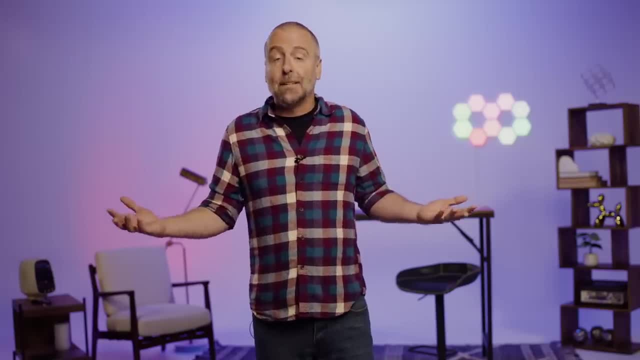 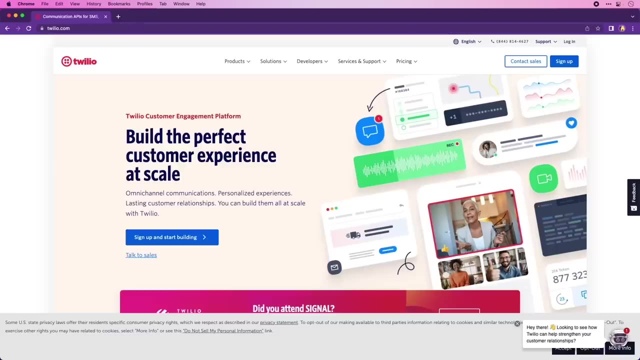 standards and phone numbers. i mean, i, i have no idea. and with twilio i don't need to know. that's the beauty of this api, it just works here. let me show you all right. so here we are at twiliocom. and again, a word of warning. this is going to look. 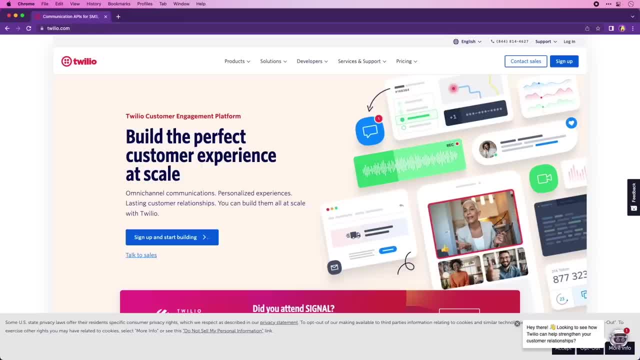 completely different from my right now to your right now, uh, so please make sure that you check the notes for anything that might have changed. and it's specifically about this flow that we're about ready to do is we're going to sign up for a trial account, so i'm going to click this sign. 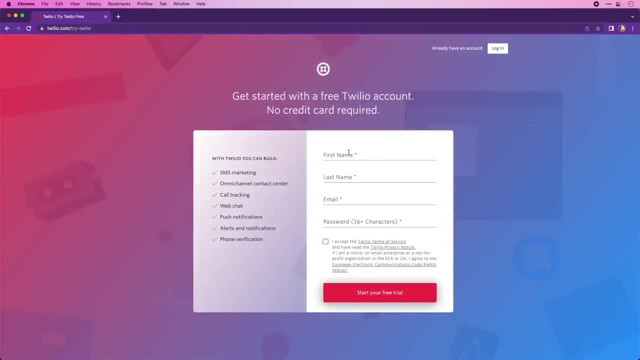 up button here and this is going to look completely different. i know, because our team is constantly making this better, but the one thing that i want to make sure that you know right now is that you see that there is no credit card required and it is a free twilio account. so i'm going to put my 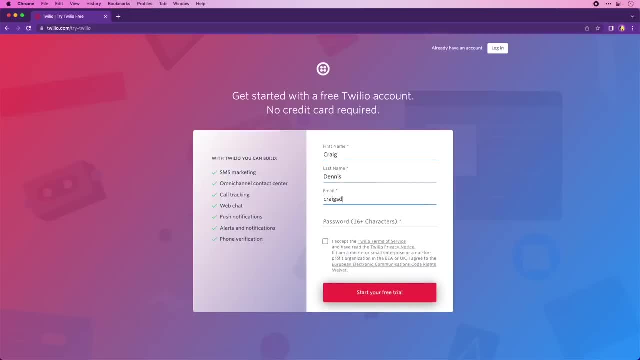 information in here and i'm going to use the same thing that i did earlier and i'm going to put my same trick that i used uh before, uh, where i do plus, and i'm going to say, uh, api course v2 at gmailcom. so i uh the plus side. there again the little gmail trick. um, uh, we're going to go ahead. 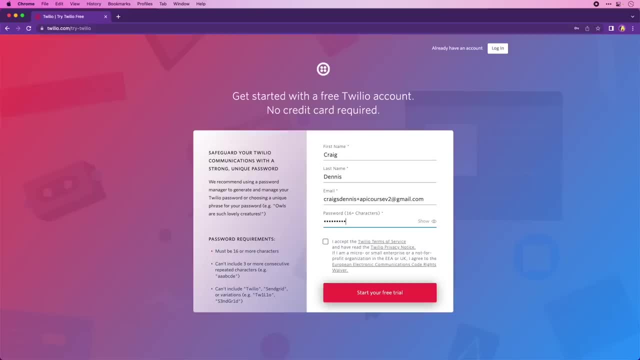 and i'm going to put in my password again: uh, one, two, three, four, five, six, my luggage, how many times can i do that joke? and then uh, would i do this, except uh must be 16 or more characters. okay, there's some password requirements over there. 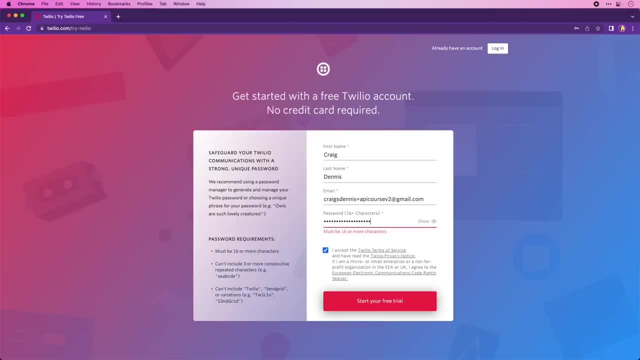 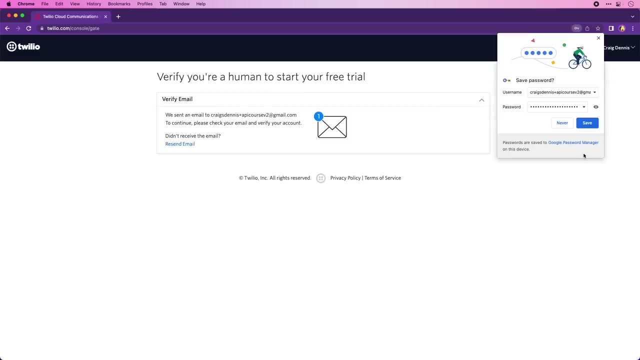 i think that's 16. all right, uh, here we go, starting my free trial. i'm ready, let's do this. i'm definitely going to save that long password because i need that for later. all right, so i have now. uh, should have been sent an email, so let me make sure that i got that email. 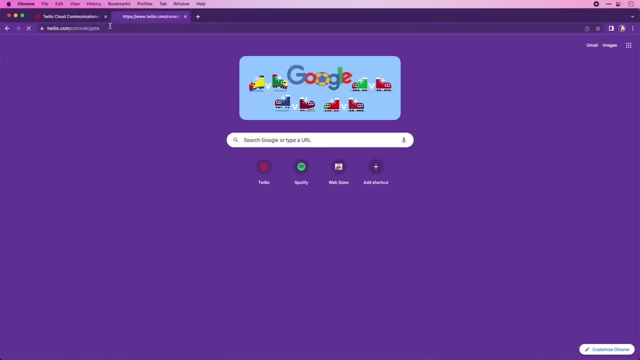 and i didn't read it right, so i'm going to save that, and then i'm going to save that, and then i'm did. I am going to click the link to verify it. And here we go. I'm going to verify my phone number. 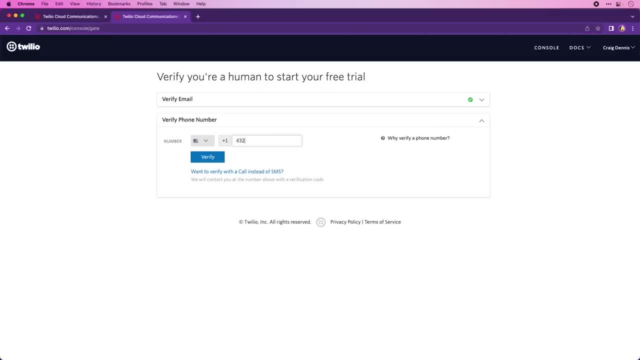 to verify. I'm human, because all humans have phones, So we're gonna do 432-527-4274.. Please don't call too late. I'm going to try that. I'm going to click verify. All right, so I got my. 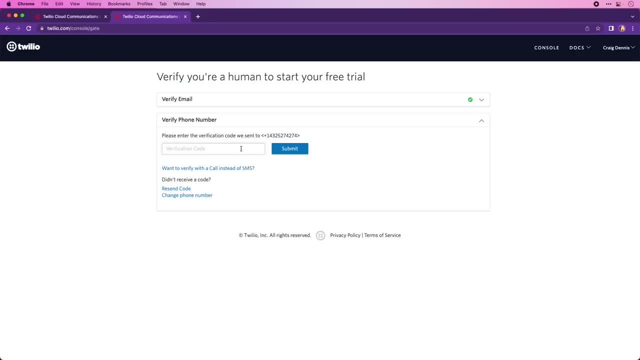 verification code. Hey, that came very quickly, What's wonderful. My verification code is 017 869.. Hopefully your code's different than that one. That'd be funny if they were all the same. All right, so here we go. So which product are we here to use? We're going to use SMS. We're 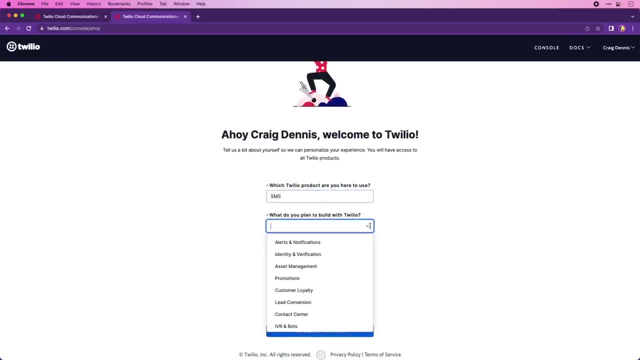 going to use the SMS messaging product And what do we plan to build? Let's see. Of course, these questions are going to be different. We're going to build something else. We're going to build something else. How do we want to build with Twilio, With code, right? So we're going to end up. 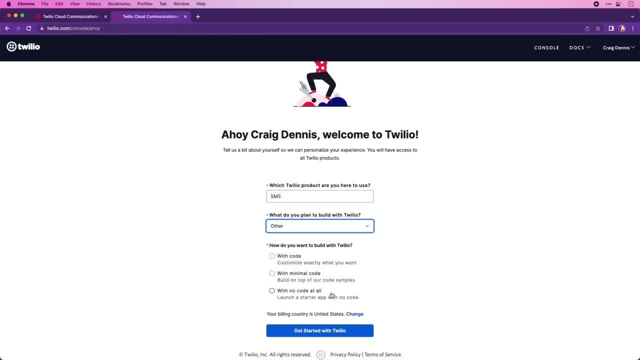 writing code if we want to, With minimal code on top of code, samples or no code at all. So definitely don't need code to build over here. But I'm going to say with code because we're we're developers here, So what is your? 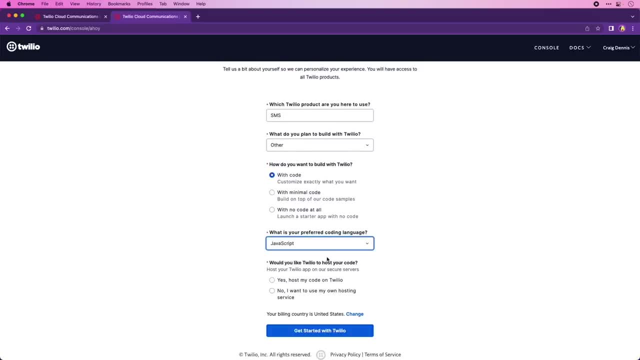 preferred coding language, we're going to do JavaScript, even if it's not. we're going to be doing JavaScript for the rest of this course And I do want to host my code on Twilio, which is nice. There's a nice serverless option. These options, like I said, are totally going to change. 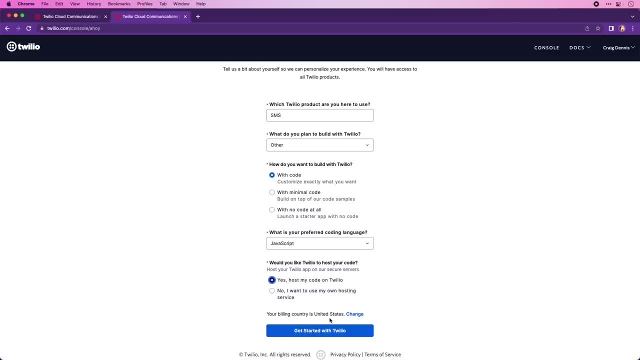 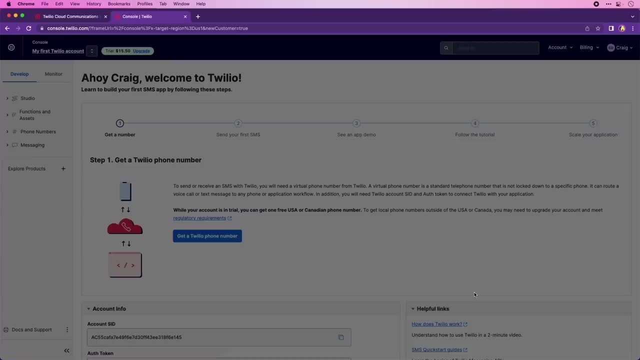 just try to answer them as truthfully as you can. So my billing country is United States, which is true, and I'm going to get started. I'm going to go ahead and walk this. I guess let's go ahead, And so we'll. I can explore. 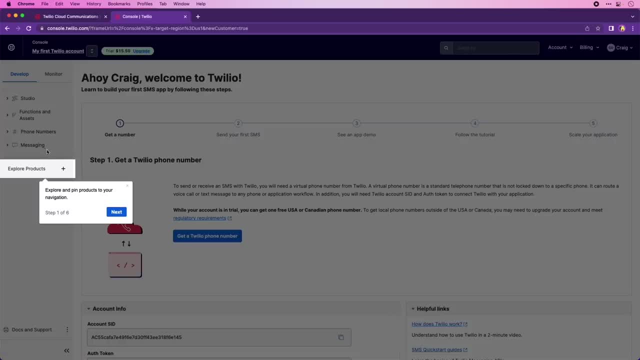 products. there's way more products that are available than you can see here. This is what got built based on the menu of what they thought, But if I ever want to, I can come to this, explore products and get more. we probably won't need to do that, because we filled out what we're going to. 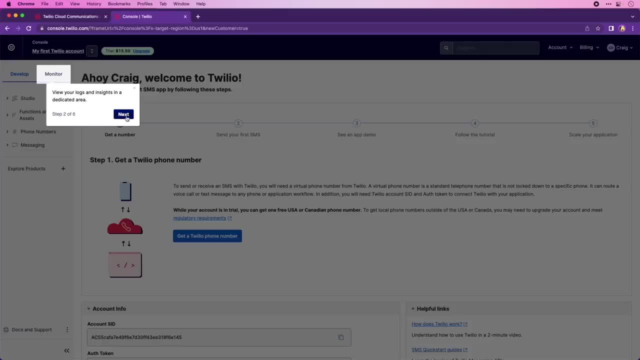 do And this is where you can get access to your logs. I'll show that off here in a bit. If there's any problems, you'll be able to find them there, Manage your account keys and build trust with your customers. Yeah, we can build all sorts of different things in here. we probably won't need. 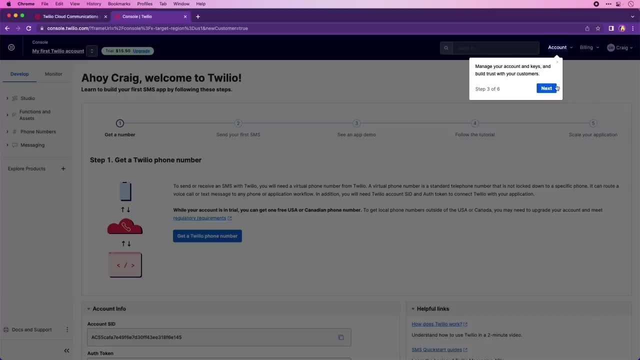 to do too much here, Because most of the keys that we have are available to us right from this page that we're on actually. So we'll keep going. And I can see the billing. And again, you're in a trial account and you think you get something like $15 to try with, So we'll be sending text messages. 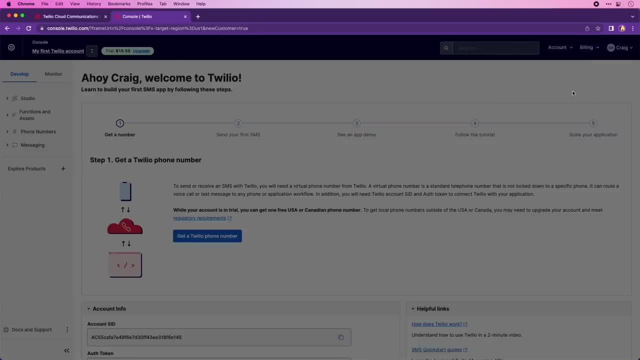 using that, that trial dollar, dollar bills, y'all. So here we go, And then we can switch between products So you can have multiple accounts, right? So if you wanted to come and like, explore a little bit, do your own personal thing, maybe do something for work later. up to you, There's a 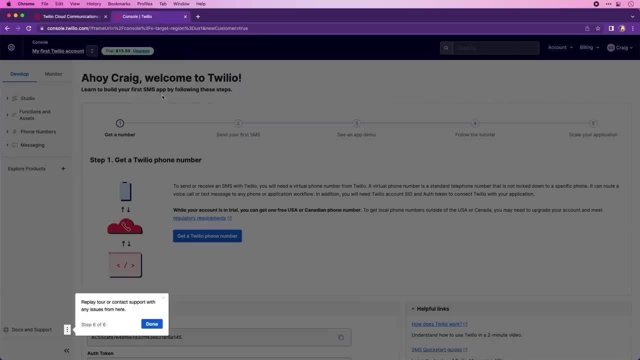 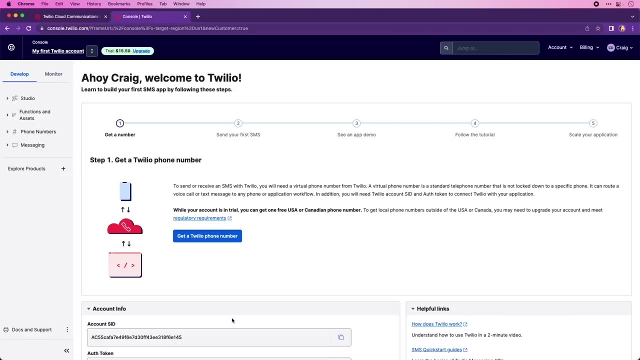 lot of different things that we can do here, So I'm going to go ahead and click next, And then I'll click next, And then I can. anytime I want to, I can look at this tour again to help navigate around, which is really nice, beautiful console. So we could definitely go ahead. And the first 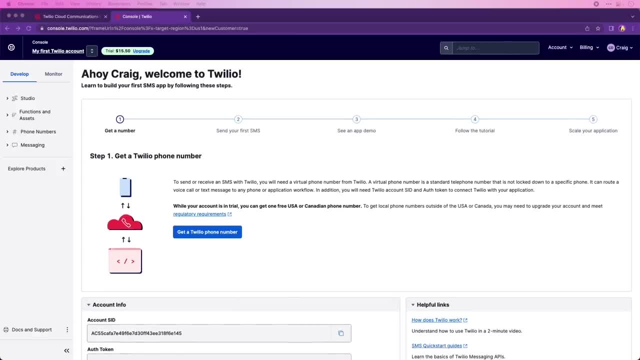 thing that we want to do is we want to get a Twilio phone number. So I'm going to do that. I'm going to click this: get Twilio phone number, And I am so glad that this happened to me. it says that: 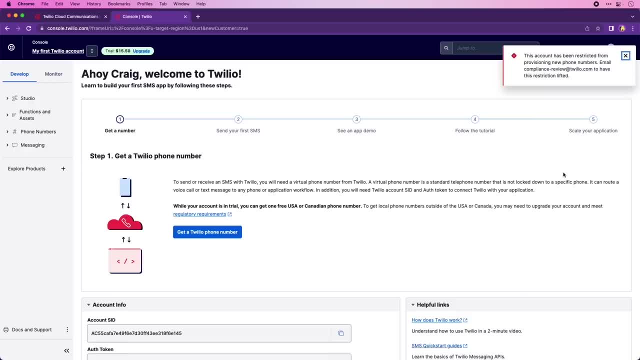 this has been restricted from provisioning new phone numbers, which means it thinks that I might be spam. And you know why it is: it's because I put that Gmail account with a little plus thing there. So if this happens to you, I don't want you to feel offended or anything like that. I want. 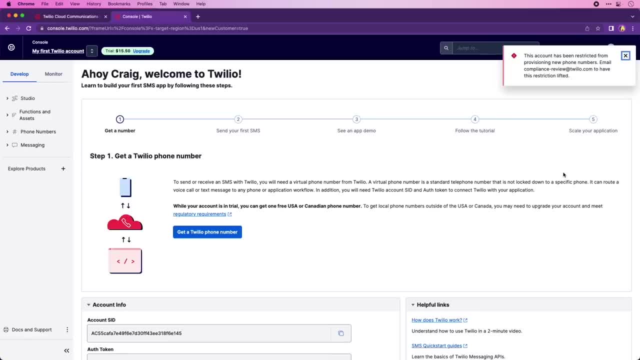 you to check the notes for the latest ways to get around this. And also, I'm going to go right now and I'm going to email compliance review at Twiliocom And I should get that up and running. If this happens to you, go ahead, press pause. check the notes here for for what to do, And I'm 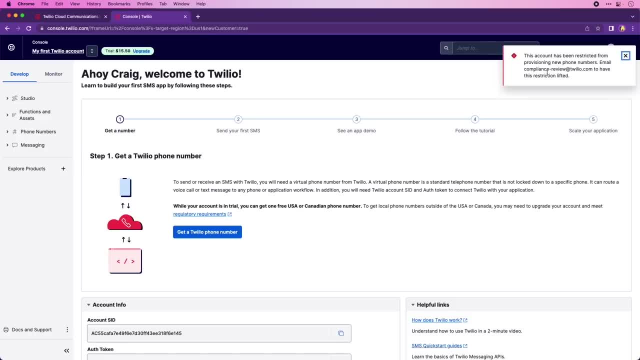 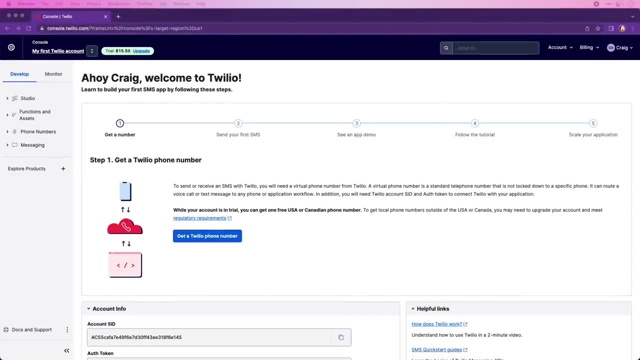 going to actually do that. I'm going to press pause here. I'm going to get my account able to get a phone number and I will see you back here in one second. Alright, so I got all sorted out. So I sent my email to the compliance folks And I was able to say that I was doing a personal account And 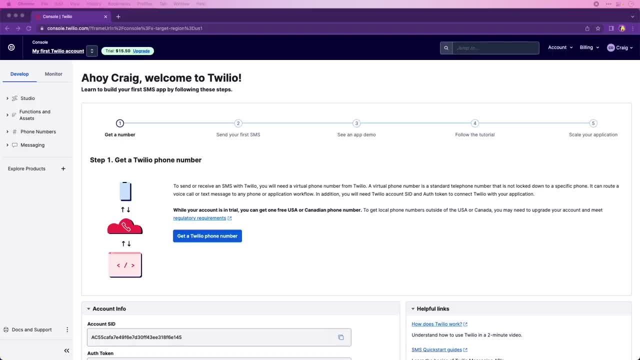 I'm learning how to use these API's And they were able to let me get in here, So what I'm going to do now is, when I click this, get a Twilio phone number. we're not going to see that message because I'm coming in. 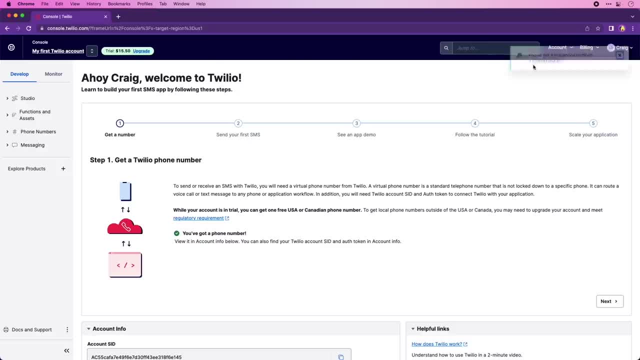 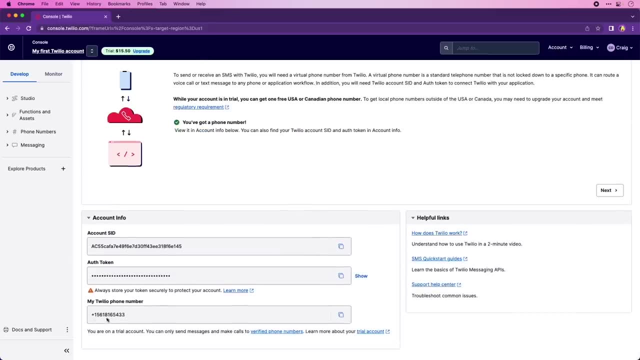 And I've got a new phone number And it automatically gave me this one, this one here, this 561.. It went away really quick, But it's down here. This is my. this is my. my Twilio phone numbers is 561-816-5433.. Now this number is mine, which is awesome. I can use this message. I can send messages, I can receive messages. I can do all sorts of things with this. I can make calls, I can receive calls. this Twilio phone number is mine. play with. I think we should do just that. we should send a text message. 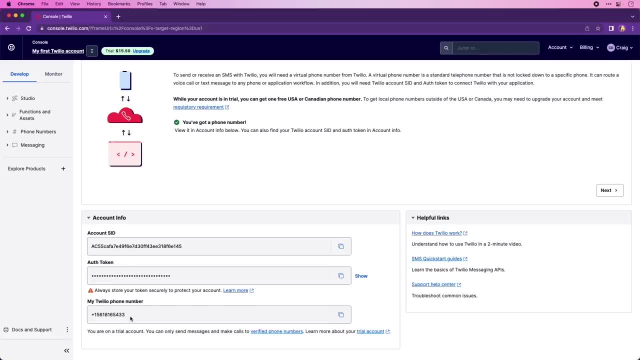 Now, before we get started, I want to make sure that you know this, this stuff. you are on a trial account, So there are some limitations. you can only send messages and make calls to verified phone numbers. So when we set things up, we verified like I'm able to send a text to myself because I verified my phone number. I mean it will say sent from my Twilio account beforehand, And there's more things about your trial account too, if you wanted to get into that. So So check the notes, because this, this very well could have changed. But check the notes for more on this. 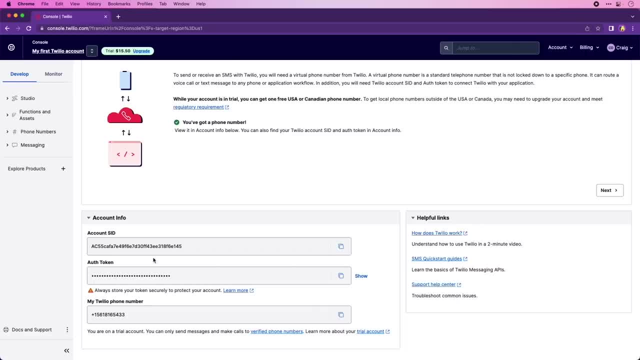 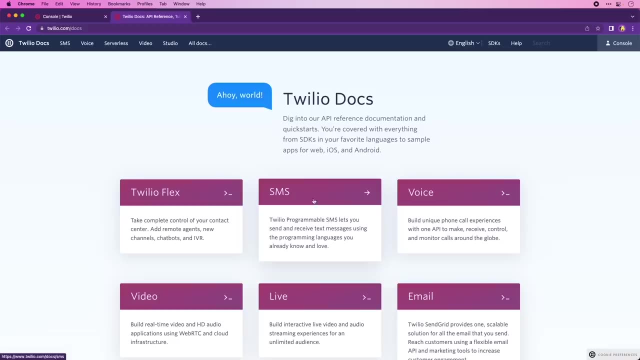 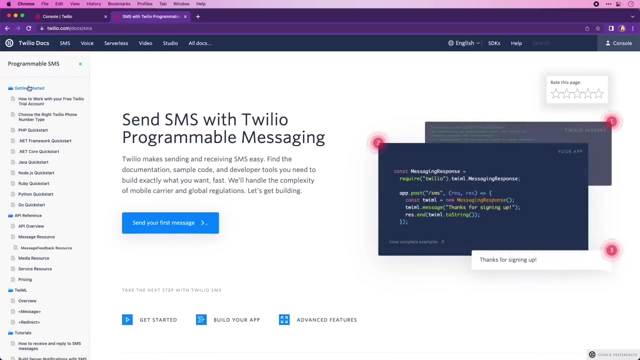 So let's do it. Let's send a short message service and SMS. So I'm going to click here on this docs and support And when I click this it's going to open up. I'm going to go: these developer docs. These developer docs are some of the best that are available out there. I want you to see these. So we're coming here under SMS- because that's what we're doing, right, short message service. And under here, under these, these sides on the docs, here you can collapse these. So I'm going to come in here under API reference. I'm going to go to this message. 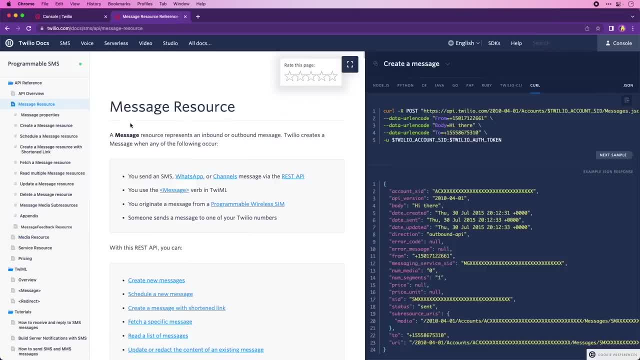 resource. Now, this is a. this is an API, right, So we're in the API reference. So the API that we want to do is we want to be able to send a from, and we want to say from the phone number that we just got, And we want to send a message to my phone number, right? So we're going to do that And you'll. you'll see that over here on the right, There are things that you can do that show you what you can do. So with this message, we can do all these different things. We'll start with create a message. we'll create a. 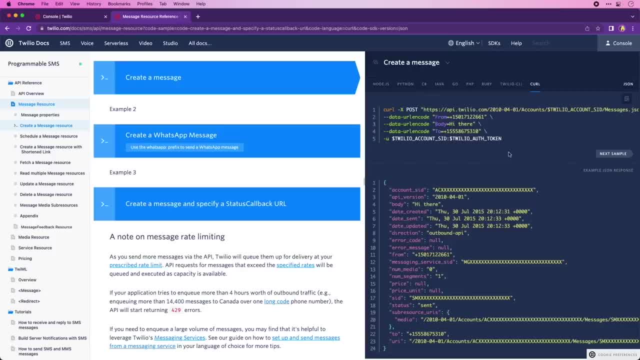 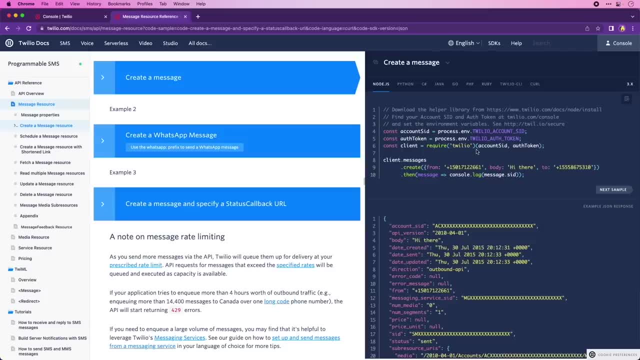 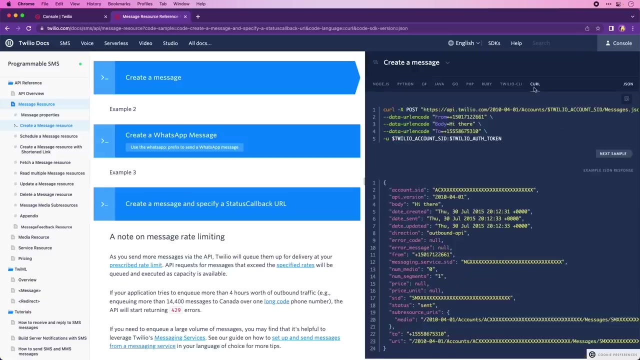 message first. So we're going to go into this, create a message, And there's these different languages here. So we have Nodejs And you can see the style that it looks like. we'll take a look at something like this here real shortly. This is a helper library that wraps around the API, So you don't need to do the sorts of things that we're about ready to have to do. You can- you can do things a little bit more cleanly, But what we're going to look at is curl, right? So here's our friend curl. we're gonna jump over here to curl, And the docs have this really nice thing where I'm able to actually copy this, So I'm going to click to. 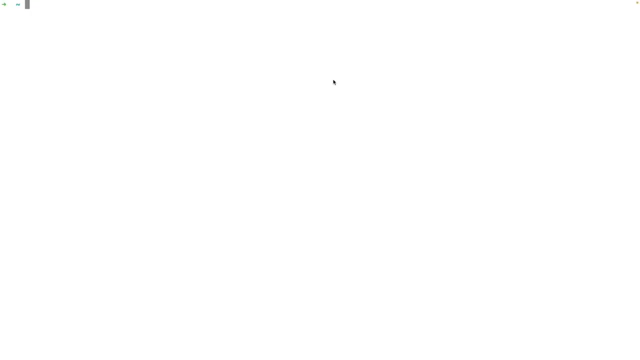 copy this. I'm going to pop over to my terminal Now. again, I'm running on a Mac, So there's a couple of things here that this is assuming that it's going to be okay because I am running on a Mac- it's going to assume that these slashes- see these slashes at the end here, these in on a Mac terminal- these show that we are in the new, we're making a new line available here, And also you'll see that there's these account SIDS and these auth tokens, this dollar sign, Twilio auth token. dollar sign. 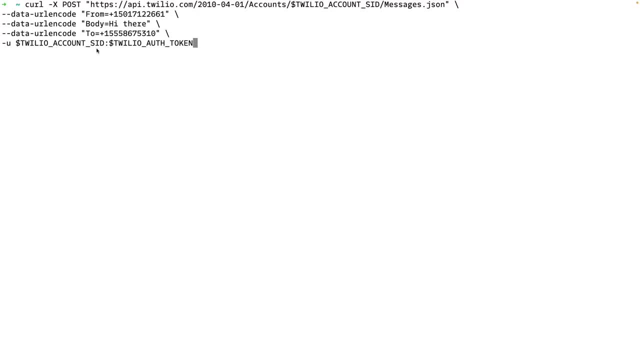 Twilio account said in my terminal on my Mac that is what's known as an environment variable, And they've been set. Now I don't have those set currently because I just built this account. So what I'm going to do is kind of bad practice. Actually, I'm going to actually put my real 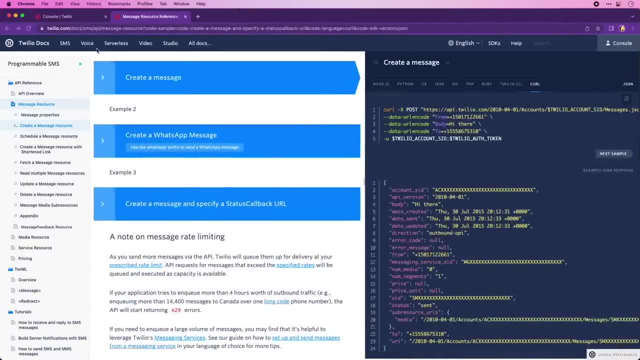 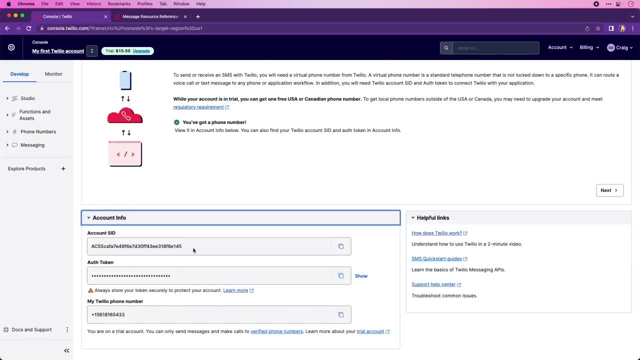 information here for us to use. So. so back back here on our console, on our Twilio console, you'll see that I have this thing here called this account SID or string identifier. So this is my ID, my unique ID for the account that I just created. So I'm going to go ahead, I'm going 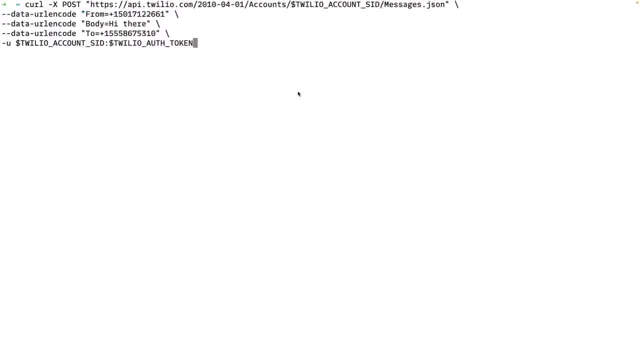 to click this copy button. So I copied that. I'm going to come back here and I'm going to move my mouse and I'm going to remove right here It says account SID. So that's string identifier. I'm going to paste this So that is the way that Twilio is identifying who I am. I'm going to go. 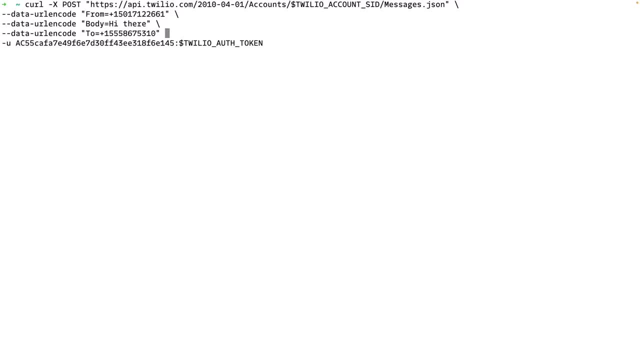 backwards through the rest of these, And so if you're watching here on windows, let's just go ahead. Let's get rid of these, these new lines here. So I'm going to just put them all on one line. We can handle that, We'll do that. So I'm going to get rid of that line And that way it. 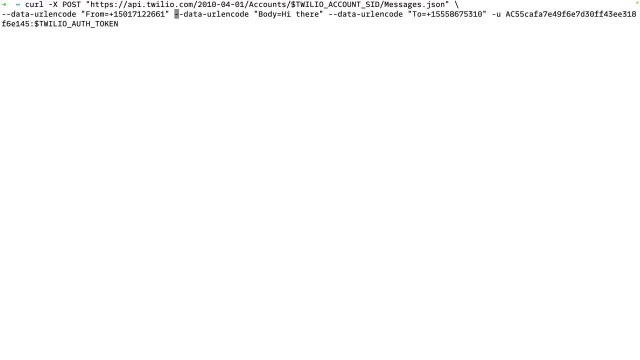 will work completely on both- both windows and Mac- for what we're trying to do. So I still have my account SID here, So I'm going to keep on backing up here And I'm going to get rid of that line. There we go. 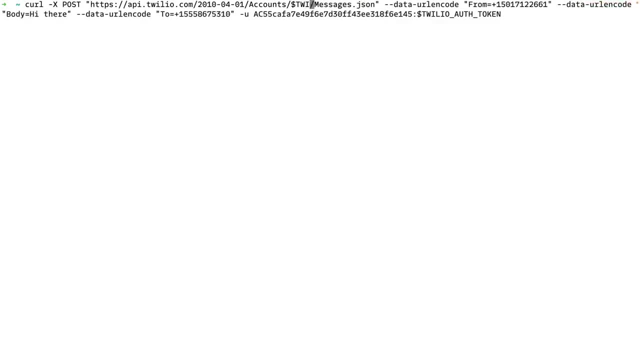 And you'll see one more time here. There's the Twilio account SID. that string identifier for my account was still present, So I'm going to paste that there. So now the API call that I'm doing is to that specific account. It's doing to this messages and you'll note that it's doing now. 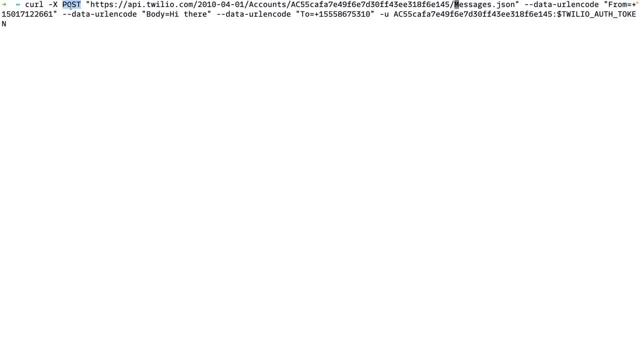 it's doing a post. So because we're creating something new, right, So we're using post to create a message and you'll see here that it says: from equals and the number actually there for the from. we want that to be the Twilio number that we just got right. 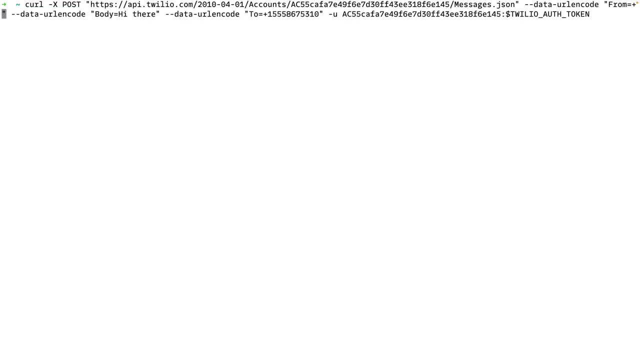 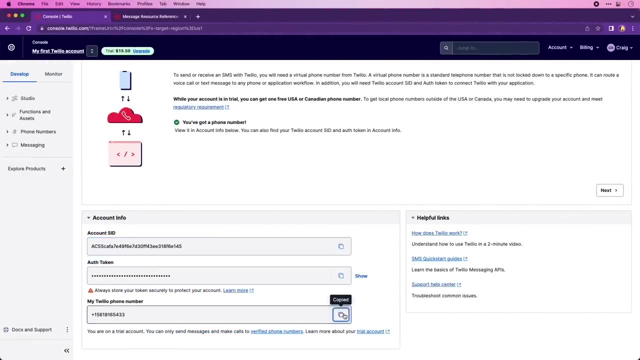 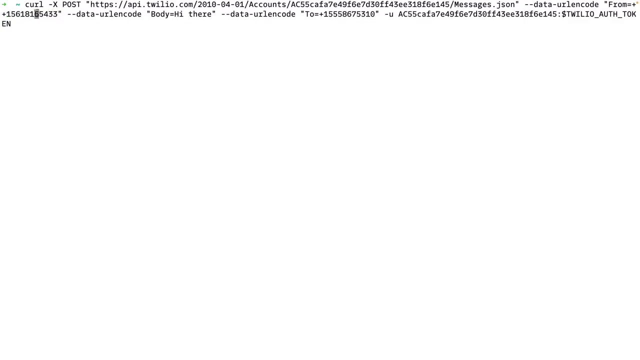 So that new one that we just got, we're going to say that is sent from. let me go back. I'm going to copy my Twilio phone number. So I've got my, my five six one number there And I'm going to paste that here. So from and this plus five six one, that's a US number. 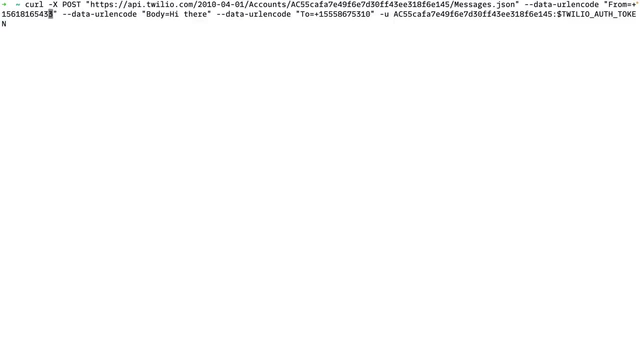 So it's got that the. it's called a 10 digit long code, 10 DLC, So it's 561811813.. six, five, four, three, three is the number that i just bought and, uh, we're gonna say by default, it said: hi there, um the body of the message, right? so instead of that, whatever we're gonna do, and 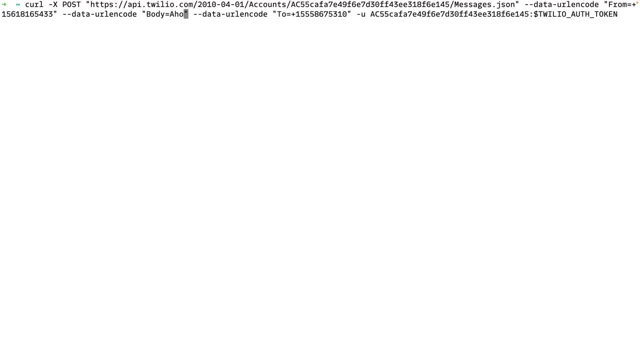 note that this is all in quotes and we're gonna say: ahoy, world. i don't know if you know this or not, but the the first word, the way that we used to answer the phone, um, was uh, we'd say the phone would ring and you'd be like ahoy, and the other side would go ahoy, hoy. so we like to do that here. 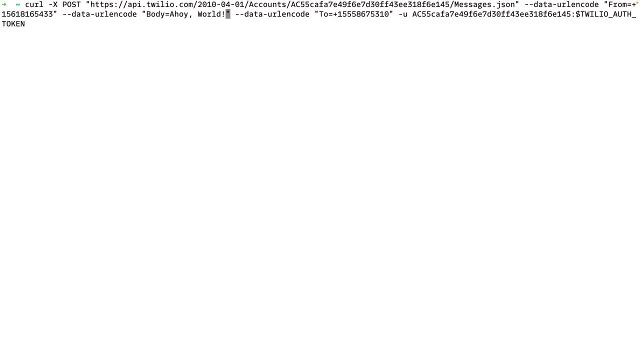 a lot at julia. we say ahoy world, uh, it's kind of like the hello world of this. so the body of the message, the text that we're going to get, uh, is going to say ahoy world, and then we're going to send it. i'm going to send it to my phone number, um, so this is, this is one of those numbers that 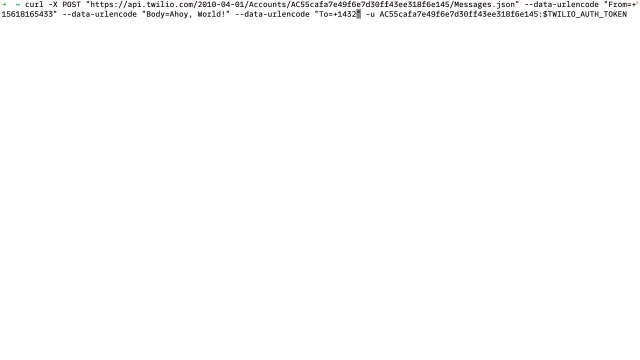 you verified right when you created your account. you verified you had a number, so my phone number is five four, three, two, five, two, seven, four, two, seven, four. don't text too late at night, please. um, and then the final thing that we have here is this auth token: now. 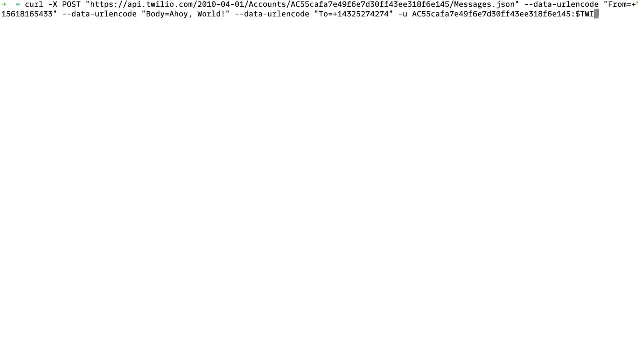 this is a very private key right. we don't ever want anybody to have access. this is like that spotify token that we had right, we don't ever want anybody to have it. i am going to, i trust you, uh, and i'm gonna go ahead and i'm gonna paste that here, uh, so that we have it. so, um, uh, that is. 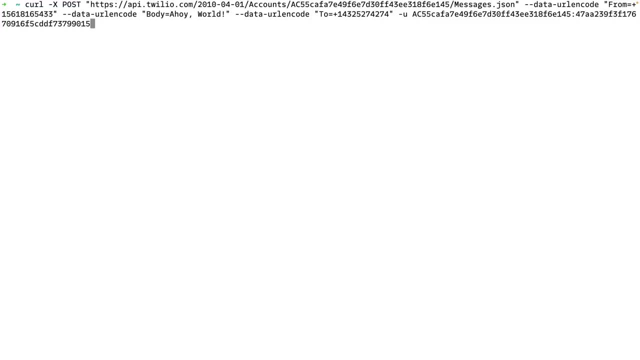 uh, something that you never want to let out, because now you could, seeing this on my screen, you could use this right, um and uh. you probably don't want anybody doing that, so you never want to actually give that number out. you want to hide that, uh, and we'll talk about how to do that uh more here in the future, but right now i just wanted to. 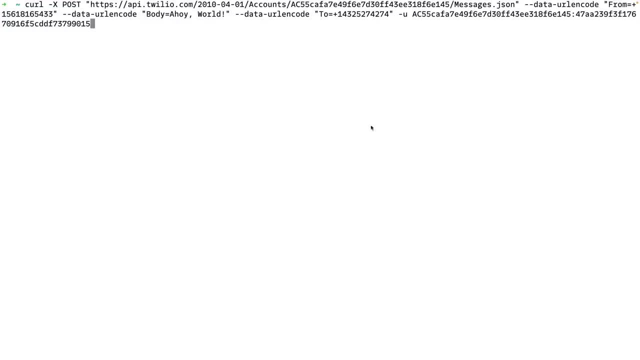 show you we're going to use curl, we're going to create, we're going to send a post to this url here and you'll notice that ends in json. so that's what we're going to get back. that's the way that that works. this is to my account. my account said: you see, it starts with this ac. 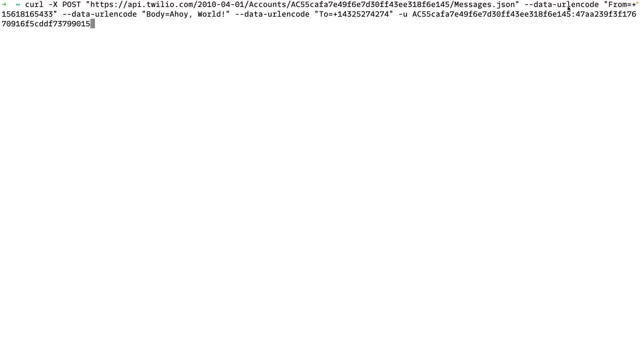 um, and, and we're going to post uh using this data url encode. so the way that the twilio api works is it takes um, some parameters, it takes from body and two, and the way that you pass those in curl is with this dash, dash data url encode and you pass what it is that you want to have uh go across here. 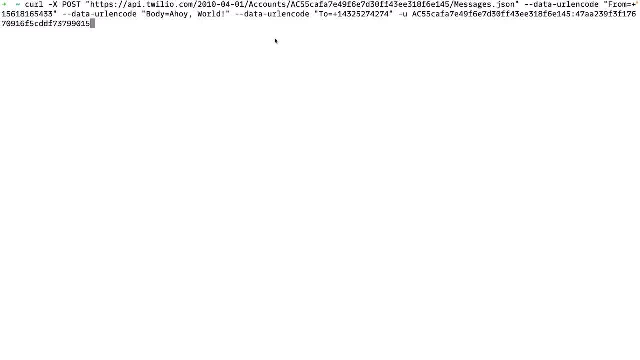 so we're gonna. if all of this works, i should get a message back, uh. i should get a text message on my actual phone, uh, that says ahoy world, let's do. and it looks like i'm missing a quote someplace, so where is the quote that i'm missing? 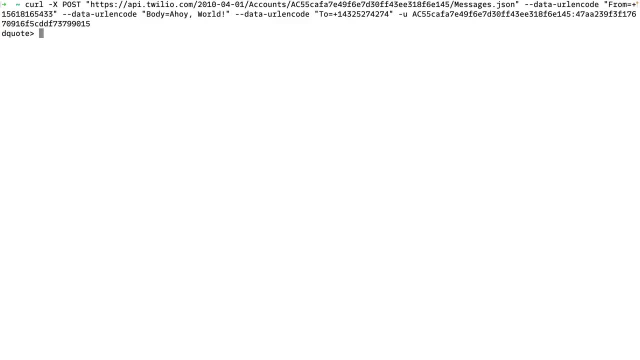 i don't see a missing quote. i can go press the up arrow, maybe it will show up. yeah, oh right. you know how many times i do that. the ahoy world. the exclamation point uh is is uh, something you need to typically escape. so i'm just. 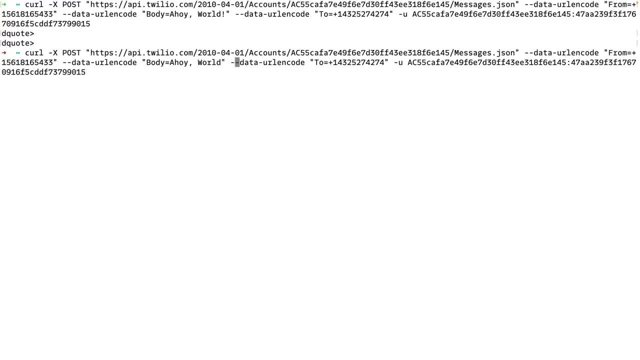 going to say ahoy world with a single quote there. so if, uh, if you're having that problem- sorry, that's what that was. so i pressed the up arrow to get my information back. uh, there, and now i'm going to see if all is going well and i press send, we should get a text. here we go. and so i got this. 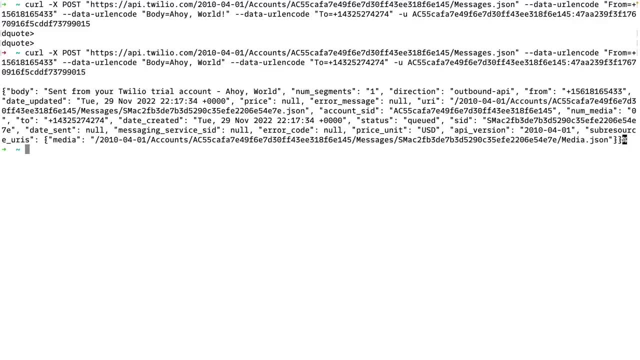 message back. i got this and, sure enough, here it is. i got it and you can see here it says at the front of the body that it sits. it says ahoy. it says uh, sent from your twilio trial account, which is fine, we're in a trial account, that's totally fine. but i did and boom, i got it on my actual. 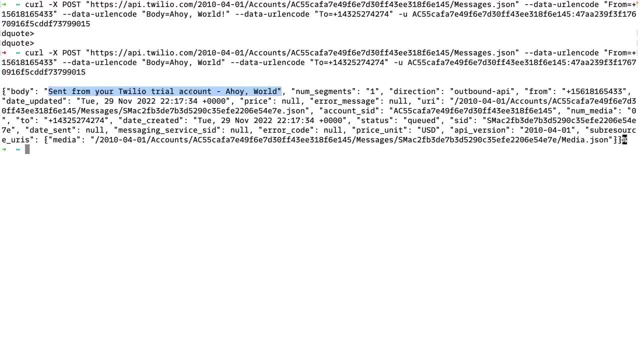 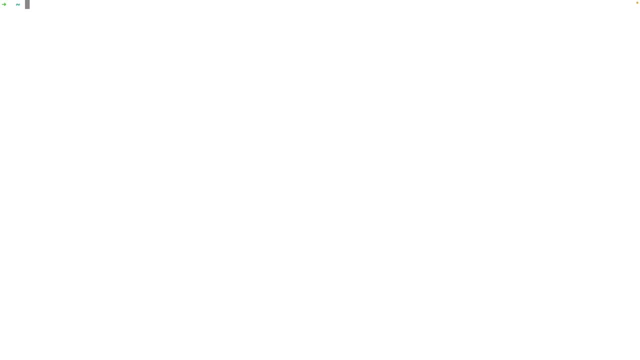 phone. i got that message, which is awesome. we now have the ability, uh, to send a text message from the command line. right, that's pretty cool. now let's take this a step farther, actually, so we know that, uh, that that api, when i did a post, i was able to uh get information back. i'm going to go ahead now and i'm going to do. 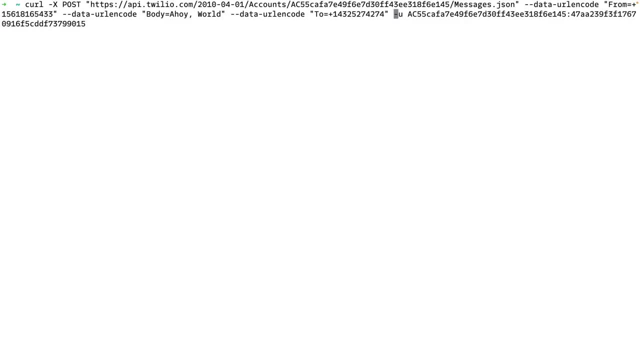 uh, just bring that back and i'm going to get rid of all of these parameters here. um, i'm going to get rid of the from the body and the two and i'm going to change. i'm going to make that, i'm going to do a get and let me show you what that looks like. so i'm going to get rid of all of those. 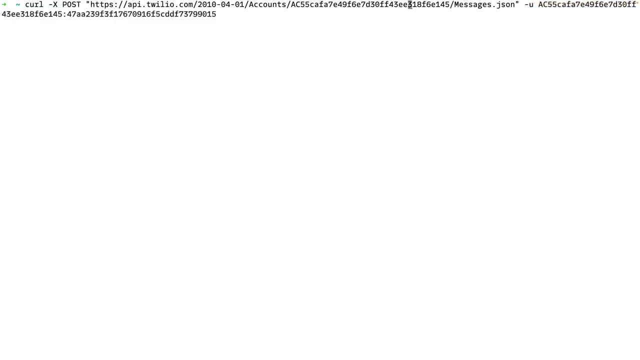 parameters. i'm going to keep that same url and it still has my account sid there, right in there, and uh, instead of a post, what we're going to do is we're going to do a get. what we should do is we should get back all of the messages that are there, so i'm going to hit this kind of like a. 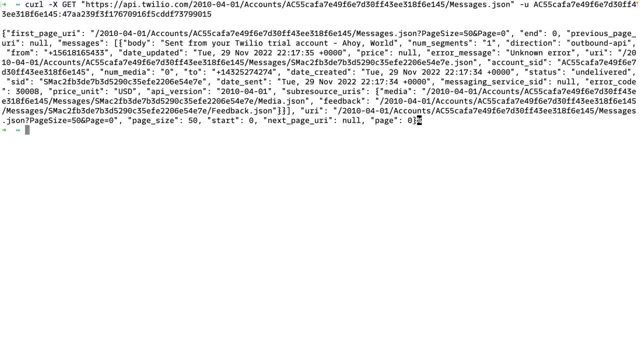 message log: right, so these are all the messages that have been sent. uh, which is awesome here, it is sent from your twilio trial account. so- and actually i can make this look a little bit prettier, like we saw with jq- again, totally optional in the notes if you want it, but yeah. 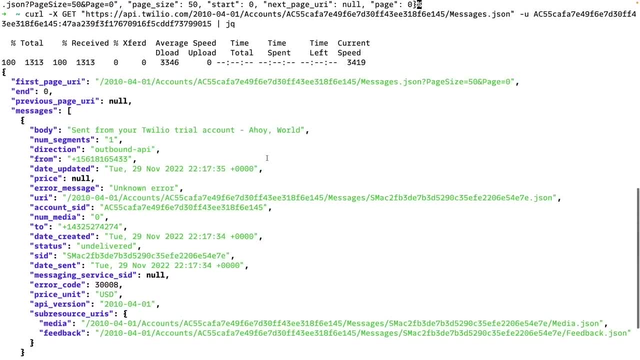 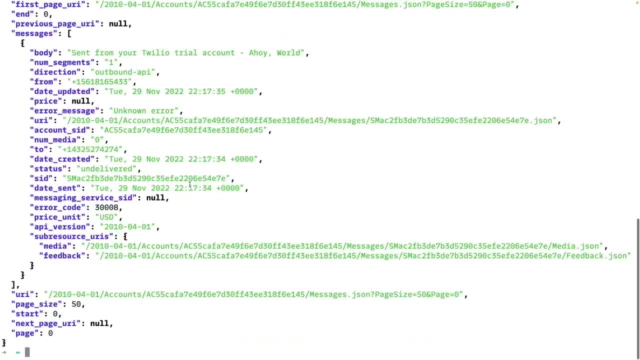 there we go, so you can see that, um, i've got some information uh that's sent back here and you can see that the the message that was sent. it was sent outbound uh to my phone number to me, uh, from that number, uh, which is awesome, right, and uh, like i said, curl's a little bit uh, challenging. 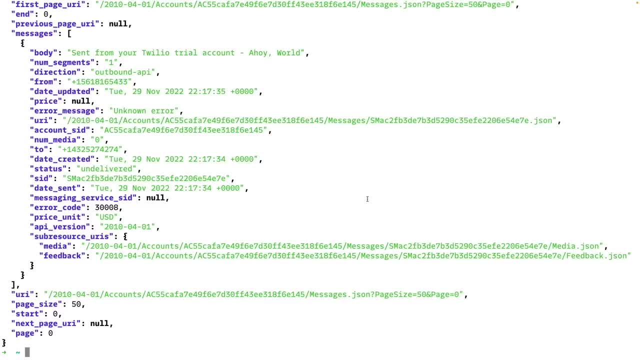 because it's going to be a little bit different if you're in, uh, microsoft windows or if you're in mac. i tried to make that as comfortable as possible, but you saw that i did run into a couple of things, like i couldn't use the exclamation point and things like that. um, it's a little clumsy, so um. 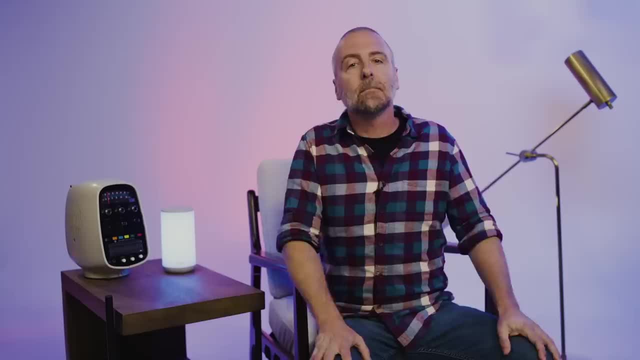 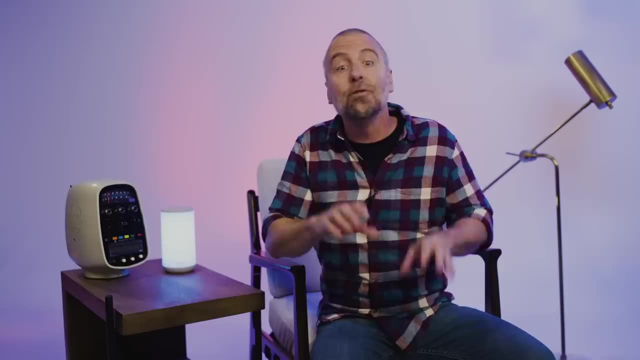 stay tuned, because there are more tools coming your way. awesome job, getting that running from your local machine. it feels pretty good, doesn't it? what a cool skill you have now you can send a text message from your machine with just a single command. now, believe me, this is just the tip of the iceberg of 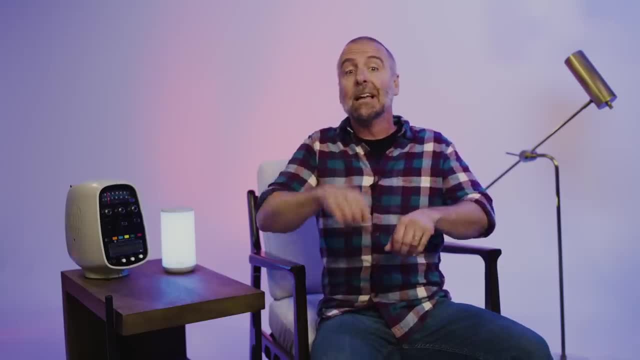 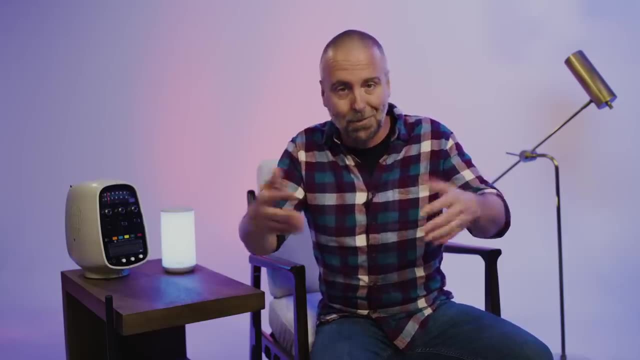 what you can do. there are so many more twilio apis available, and now i know that you can explore them with curl. for now, though, let's take things another step deeper now. i don't know about you, but i'm a little clumsy when it comes to long commands on the terminal, like we just did with curl. 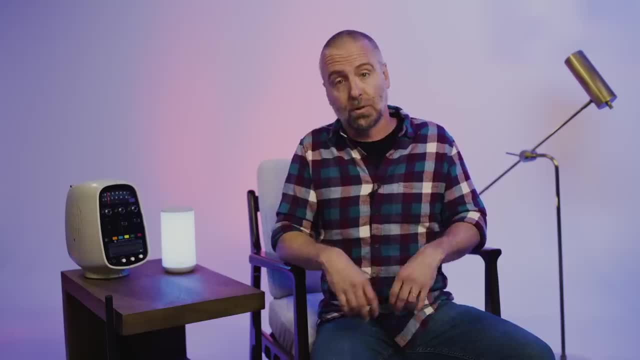 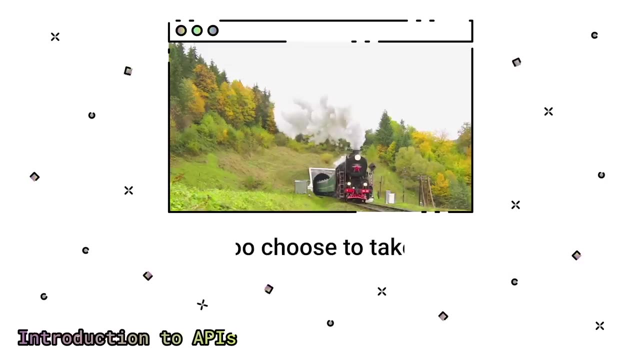 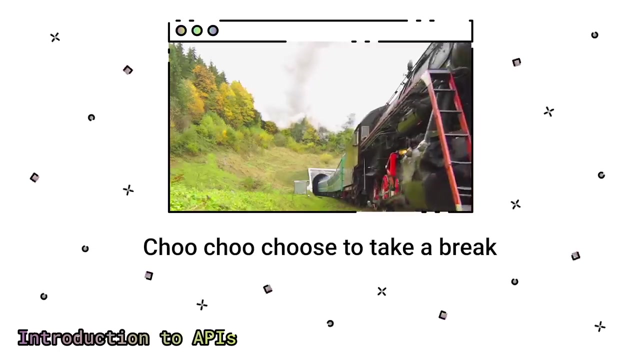 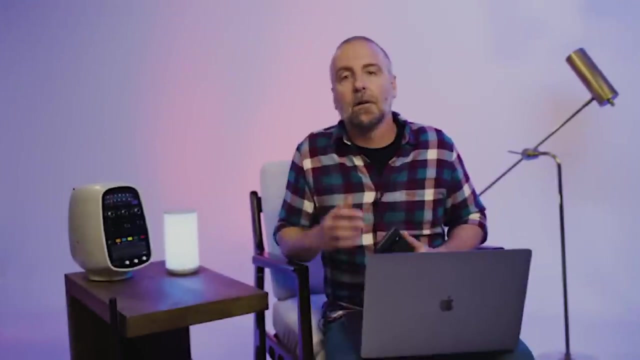 when exploring apis. i really like to lean on visual tool. if you don't mind, i'd love to show you some. that is, of course, right after you take a quick break. there are a few tools that i rely upon when it's time for me to explore new apis, and i thought i'd 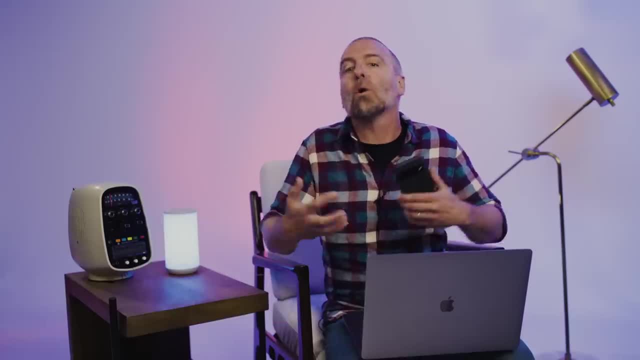 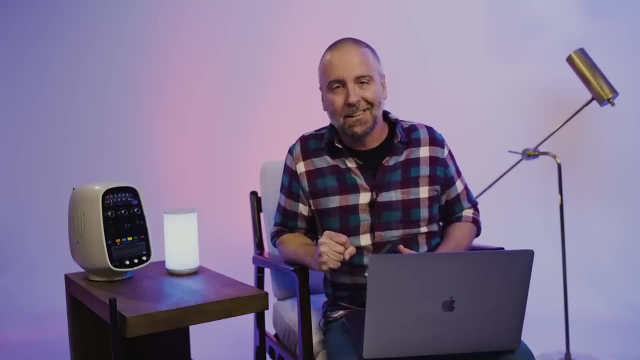 share them with you. i use these to dive in and get my hands dirty and organize my learnings. one of the most famous tools, and one that you've probably already heard of, is called postman. do you get it, postman? in addition to being a pretty good pun, it's also a powerhouse of features. 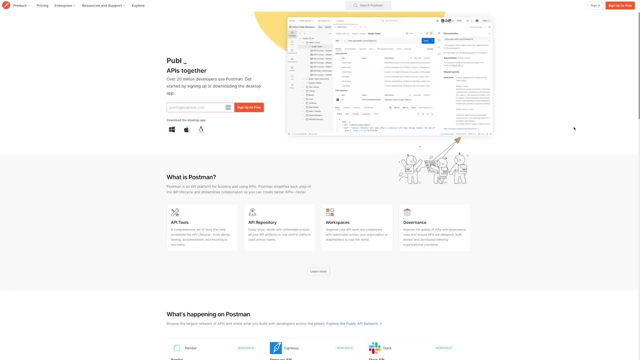 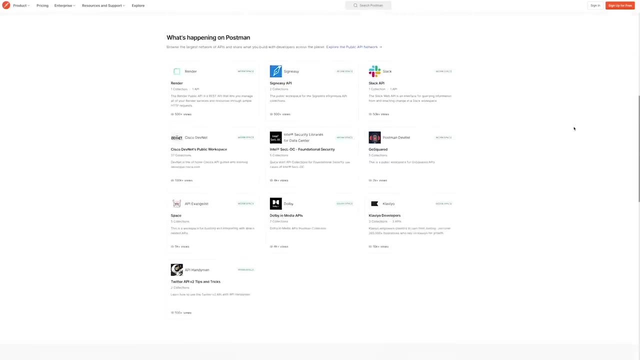 postman started as a chrome extension that let you make api calls, and what it's turned into is a powerful enterprise ready tool with all sorts of bells and whistles and even shareable collections for the most popular apis that are out there. it's jam-packed full of features and, in my humble 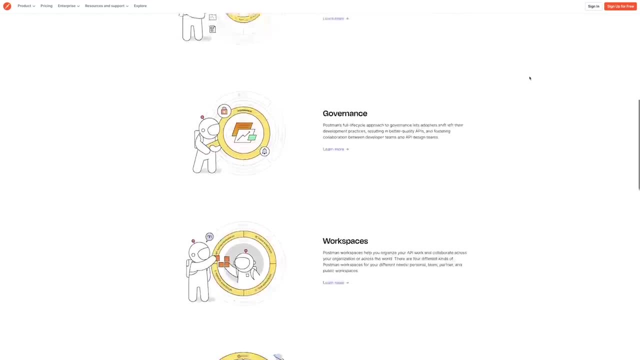 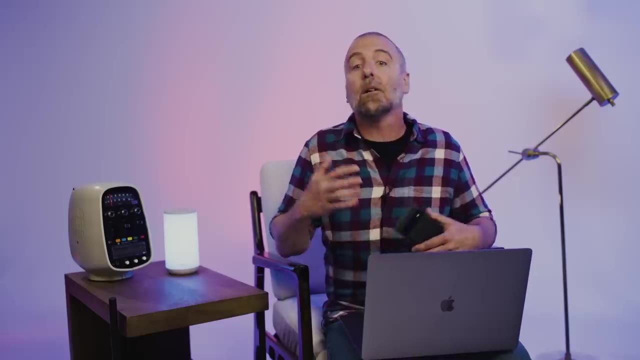 opinion, you probably don't need all that just yet in your learning journey. there are entire courses on how to properly wield its power, and i've linked to a few of those in the notes you. there are other tools popping up all the time that allow you to explore apis and store your notes. 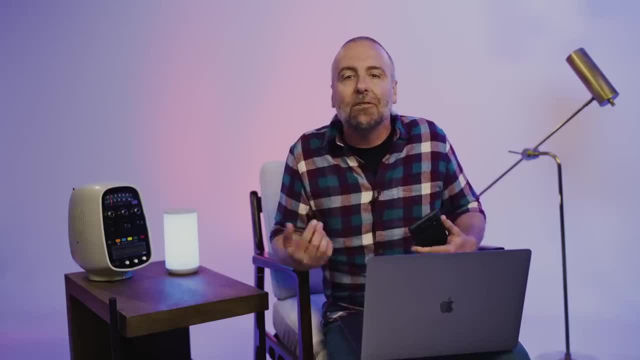 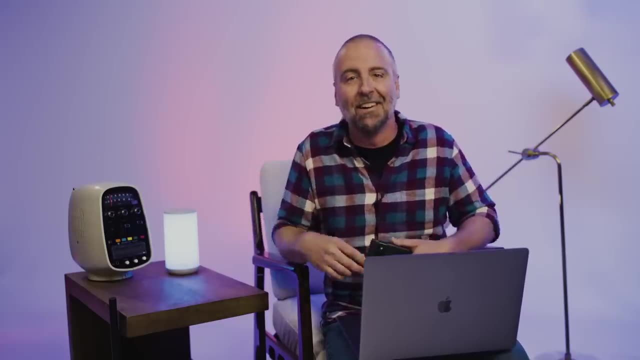 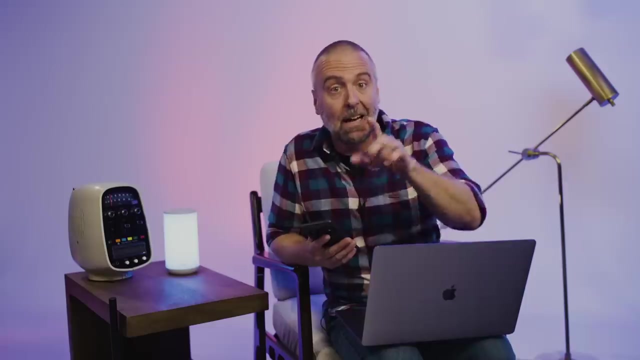 i like to think of these apps as the built in the vein of postman. there's a whole genre of video games that gets dubbed metroidvania, because they're similar to metroid and castlevania. now these apps are postmanania, postmate, postman-esque. let me show you an example. i just 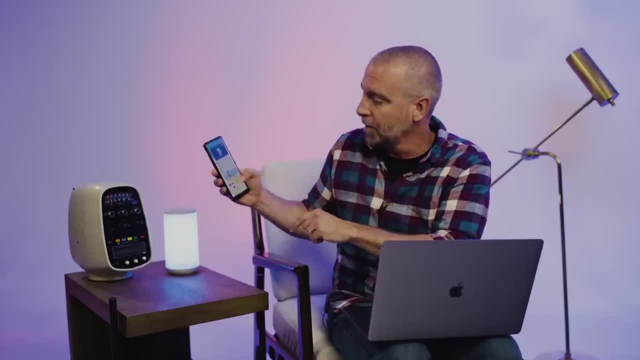 bought this lamp here. it's rad, it's from govi and it's got this app that i can use to control it on my phone. i can change the colors right, and i could even make a video on it, and it's just a simple way to make it dance to my beatbox. 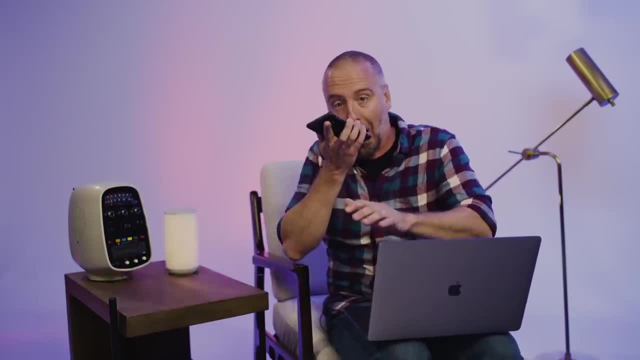 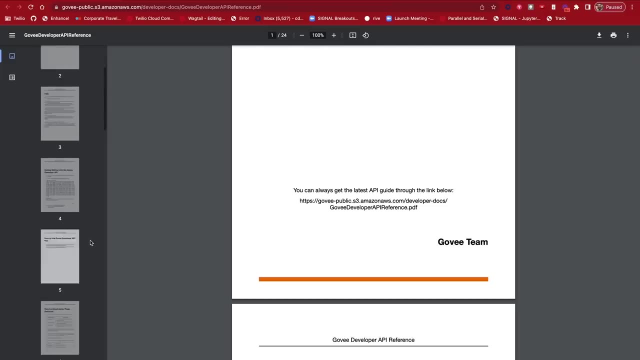 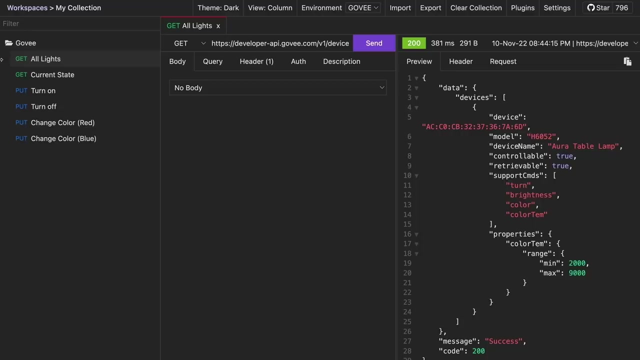 it also has an api. these are the docs here, and as i explore these docs, i'm going to save them in one of these postman-esque tools that i've been using lately, called rest fox. like here, i can see all of the devices that are associated with my govi account and i set that up. 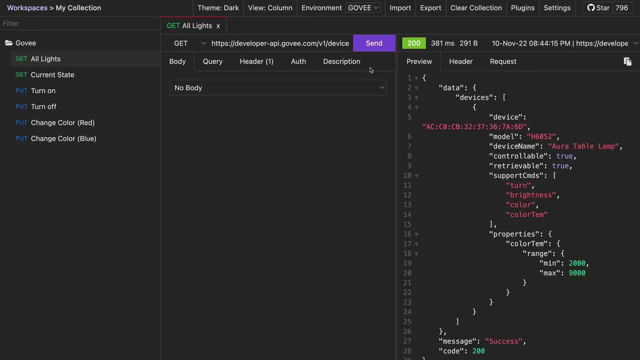 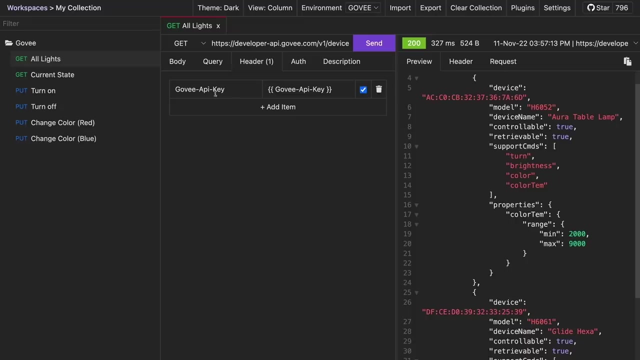 using this url here and you'll see that it is a get request and i pressed send and it sent the request and i got back the govi devices that are associated with my account. this api requires a header and it's called govi api key and you'll see these double mustaches here. 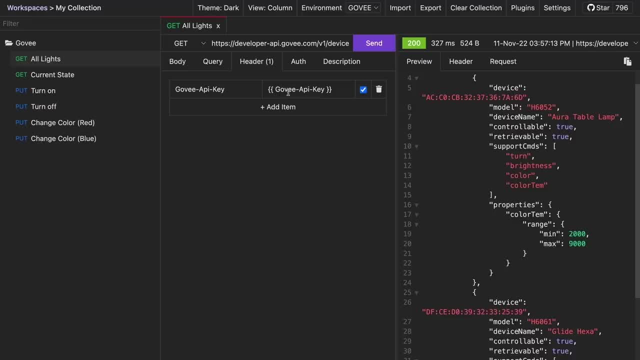 that i'm using this side. little mustache thing. this is giving things from my environment. it's a special key that i don't want anybody to see. i'll show you more of these here in a bit. now notice how this is a get, so i can send the request and you'll see that. here's my response. 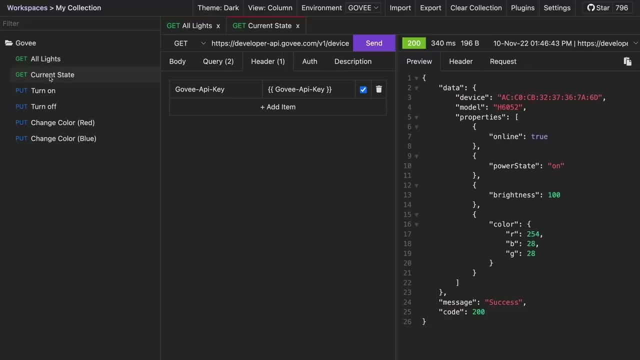 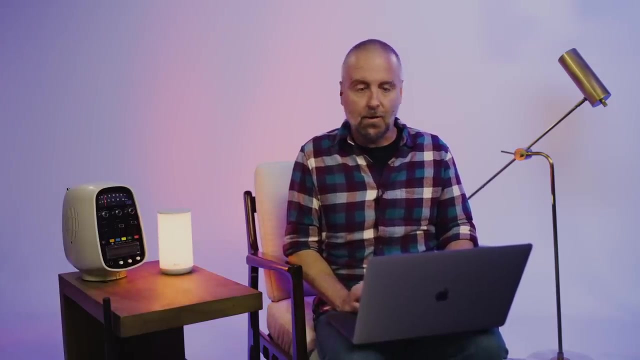 and i can also get the current state. so i have a different call here. i can get the current state and note that if i click send here, we can see that this is the color of my light currently and i can also, uh, turn it on or turn it off, and i can turn it on and i can also change the color. 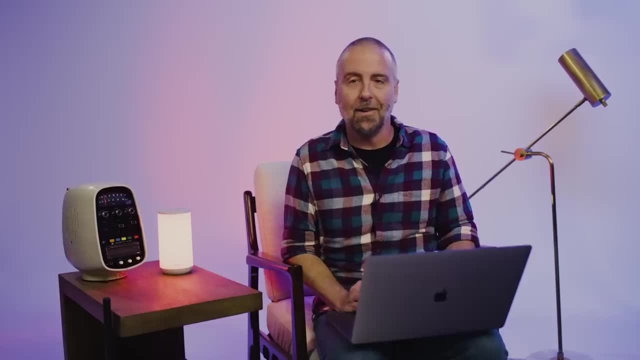 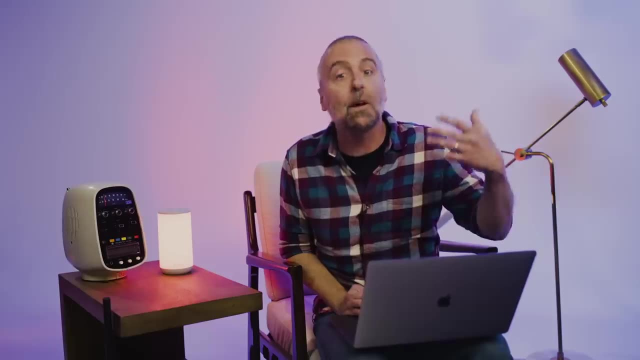 right, so i'm going to turn this to to red. you don't have to turn the red light on roxanne. pretty cool, right? and i have this here for me whenever i want to tweak things, when i want to come back later and when i want to use it in my govi account. i can also get the current state. 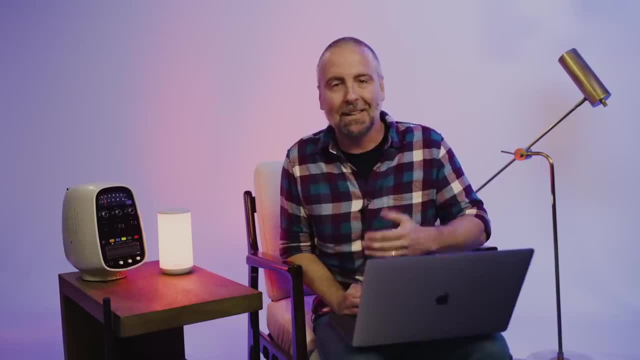 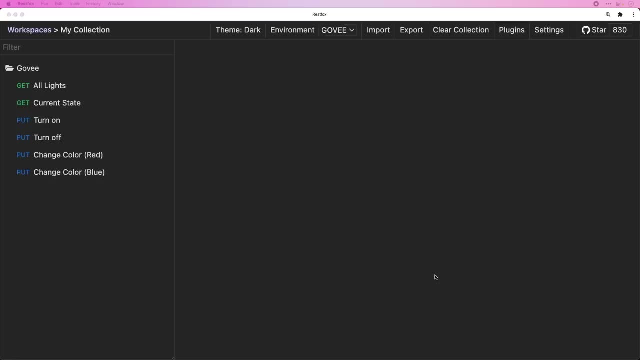 my code. did you just have a light bulb moment? i quite literally just did. let's see if we can't build one of these for the twilio apis. so if you'd like to get rest fox installed, please check the notes. this is an open source tool and it's getting better every day. now, if you love it. 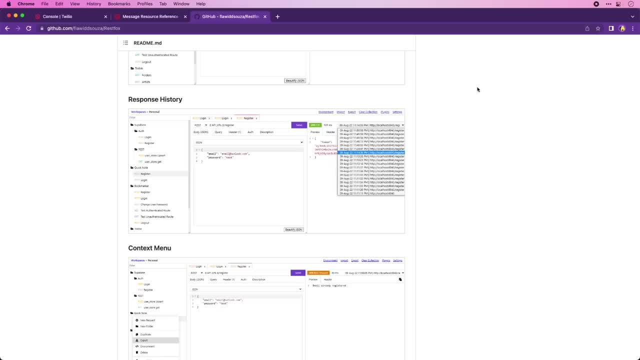 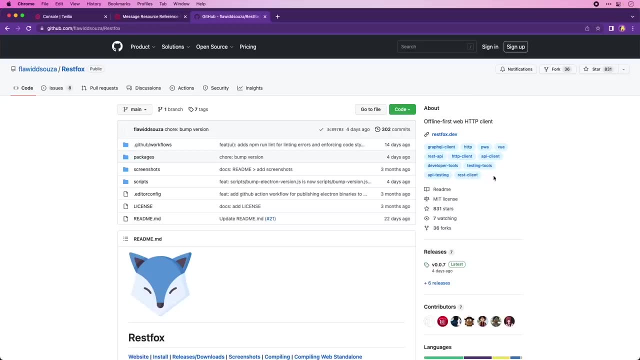 too. i highly suggest that you start. if you click up here, you could go and you can actually check out the github repo, uh, and you could see cute little fox here and you'll see uh over here how it's tagged. oh, it's tagged rest client. i guess maybe that's a little bit better than my. 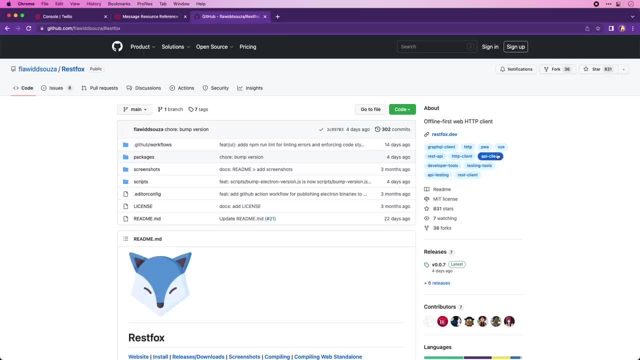 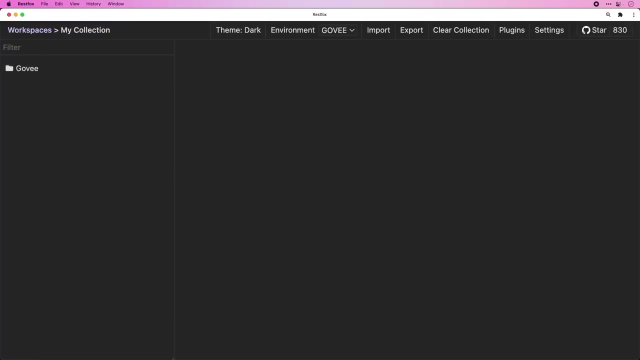 metroidvania analogy. uh, maybe rest client's a good thing, api client- that's also a good thing. there's lots of these tools, uh, that are available, but let's start using this one. so i've got rest fox running here and you'll see, i've got the govi folder, which i can collapse, and typically what i 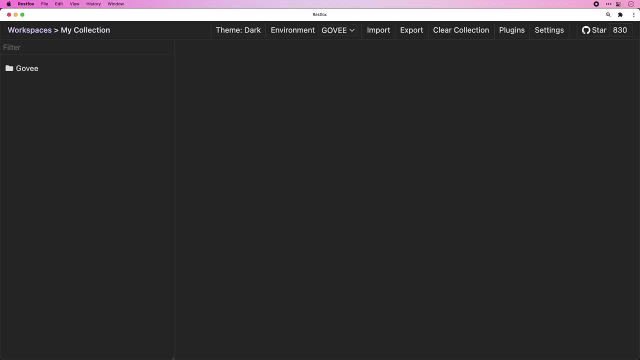 do is group these by the api that i'm exploring. so let's keep poking around a little bit with twilio. so what i'll do is i'll make a new folder called twilio. so i'm going to right click over here and make a new folder called 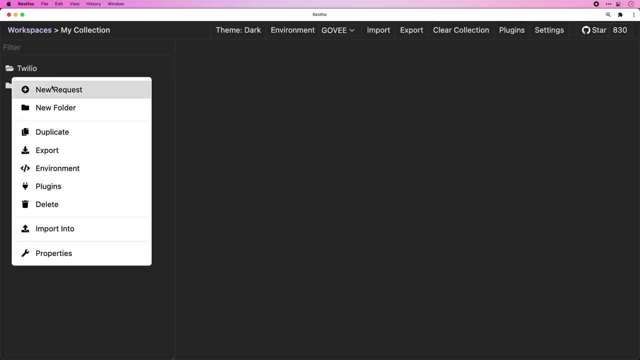 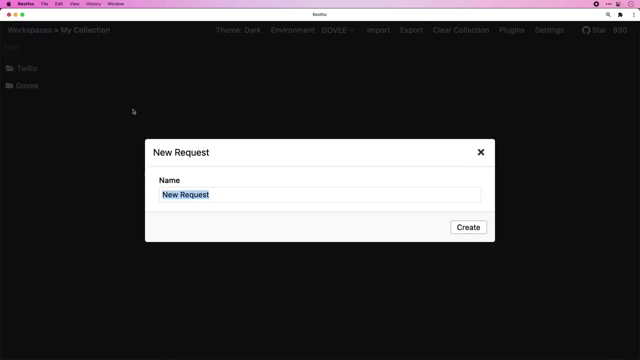 twilio, and now in here we'll create a new request. so i right clicked new request and i'd love to explore more of the sms api. so let's see- uh, oh, you know what- this new number that we just bought, this twilio number that we bought, not only can it send messages, but it can also receive them. 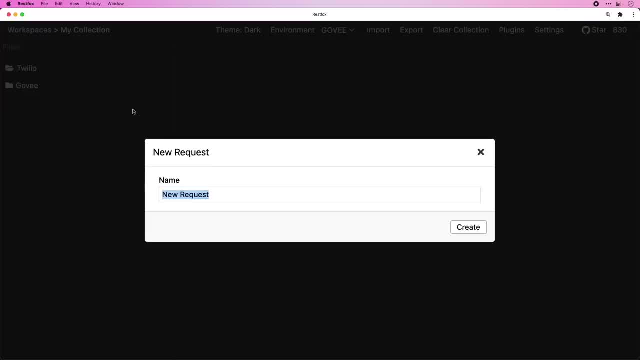 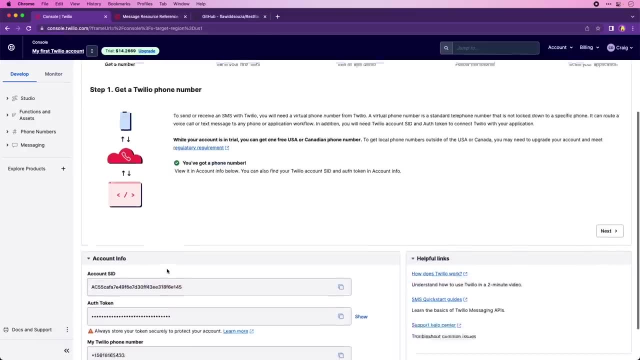 so we could send it a message. so let's do that. so let's go ahead and send a text to your number now. if you forgot your number, it's uh over in your console. so if you come to your console and scroll down a little bit here you'll see my twilio number. so go ahead and send uh a text to. 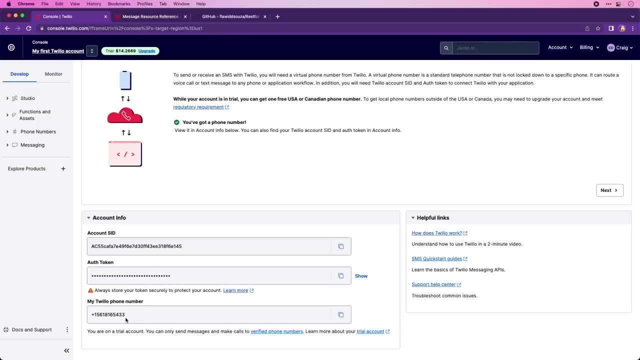 your number, now my number. i'm going to send a number. it's five, six one, eight one, six, five, four, three, three. i'm going to send it, yo, and uh, uh, there we go, it went and i ended up getting a default message back. um, and we could change this, we could make, we could program this to do whatever. 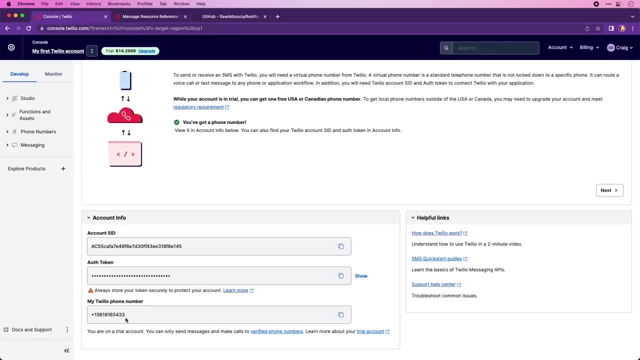 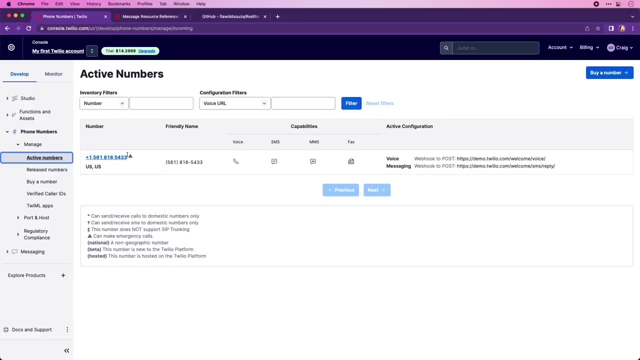 but i'll show that off later, but for now, uh, i just want you to know that we created a new message, uh, by sending to this this api, and we can actually get it. um, and you can also find your phone number later here under this phone numbers. if you go to phone numbers, manage active numbers. uh, you can see your phone number. 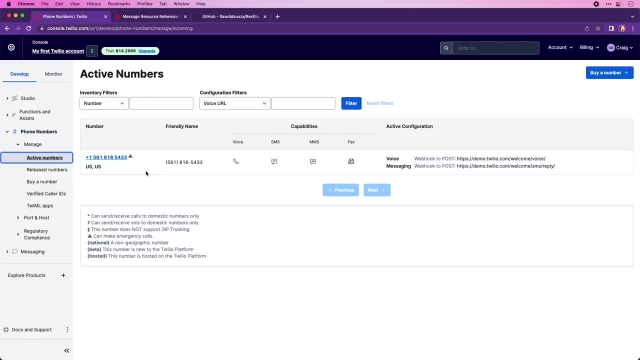 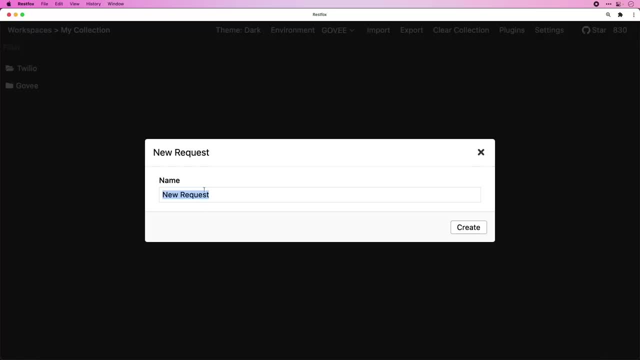 remember, outside of trial mode you could buy multiple numbers. so that's an important uh thing to know here. so, all right, so we're going to look at the incoming messages. so, uh, we should do that. we should call the request what it's going to be. we'll call this incoming message log. that sounds. 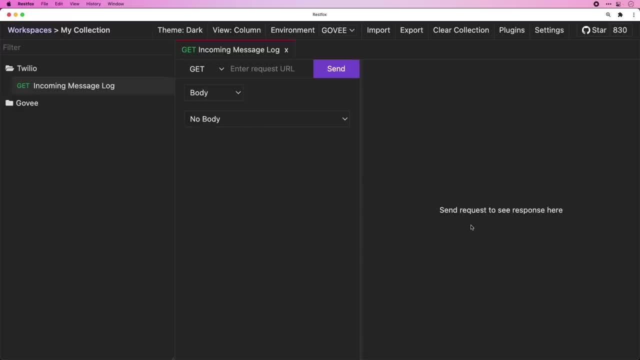 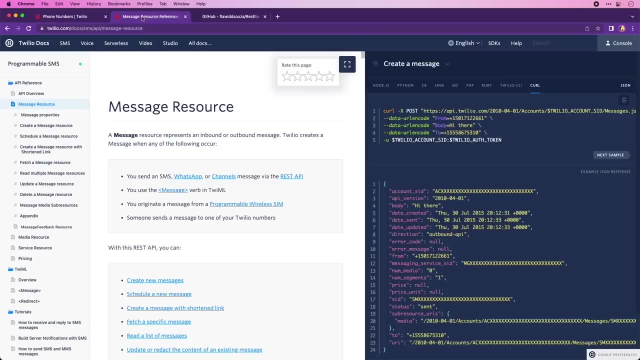 good, and we'll click create. okay, so let's head over to the docs and see how we might do this with. so back in the docs, here on the message resource- remember, this is where we did the create a message. i'm going to see if there's. 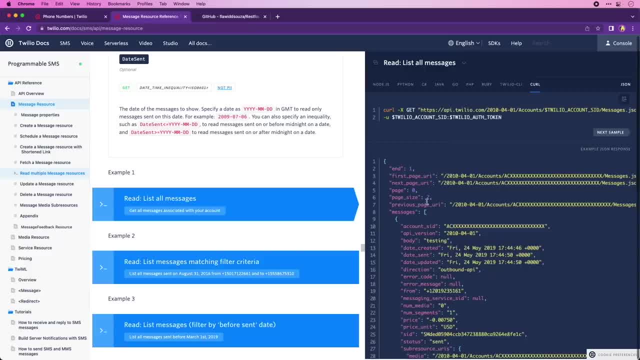 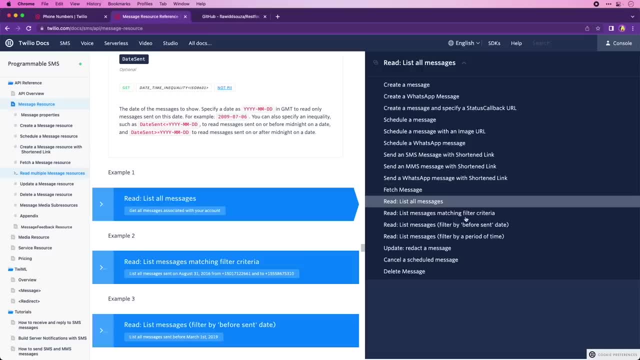 something else down in here. ah, list all messages. that's a good one, but we don't want all of the messages. we actually want to filter it a little bit. so look here we can do this by by matching filter criteria. that's great. so we're in here. i'm under the curl tab, right, i could be in these. 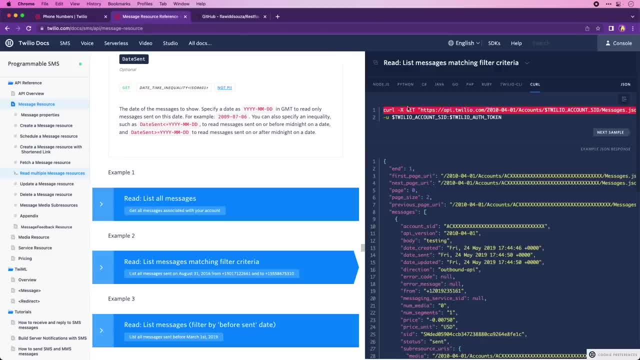 different ones, but this. this is the example that we want here. i'm going to grab this url. you're going to see all of this. so that's how they're filtering. there's some stuff here at the end. i'm going to grab all of this. i'm going to 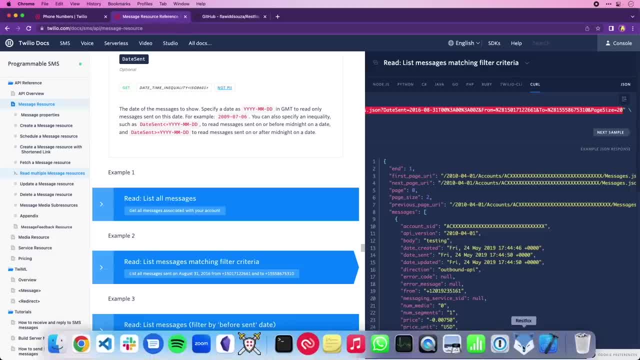 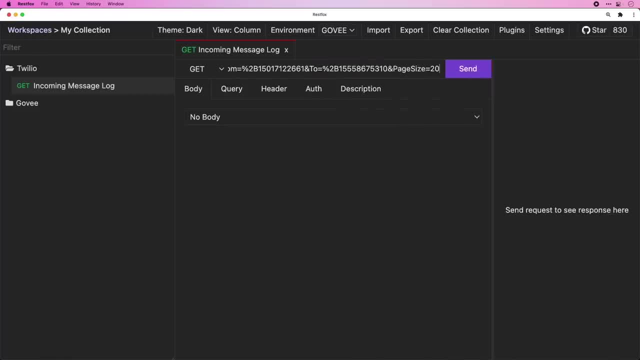 copy it. i'm going to come back over and i am going to paste it here in this enter request url. i'm going to paste the whole thing there and it was a get request and, uh, the url had some stuff in this query string that came afterwards and a query string that came afterwards and i'm going to paste. 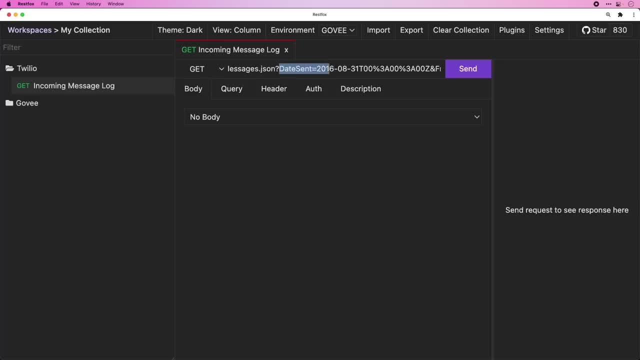 here and a URL in this place and i'm going to go back to the data st Sangha in here. ah, and i don't know if this doesn't appear on the profile, but i think i'm doing a confession. t change in the repo, because the URL here is being changed and you're going to get a. 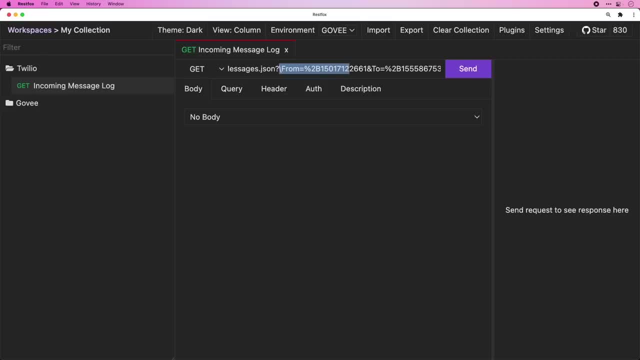 benzpwhale. we don't want from here, we don't want number, we want to look at everything that's here. but also we want, you know, i'm not evenWoah of the data, so now i have to drop this a little bit. i'm going to take this down if this literally did whatever by the like is defined by this. 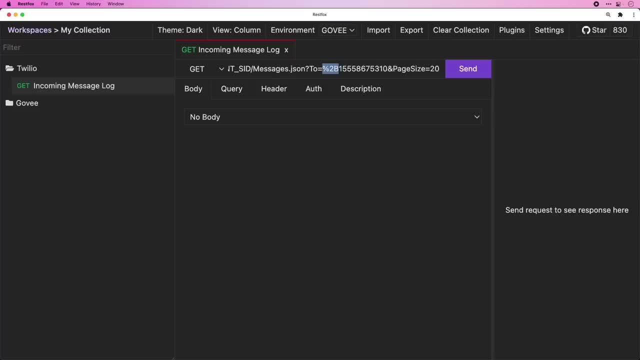 question mark. so we don't want this date sent. let's get rid of this. and what's next? we don't, we Google it, but that's a little rough to know, Like how do I make a plus sign in here? Wouldn't it be nice if this tool just did all of this URL encoding for us? 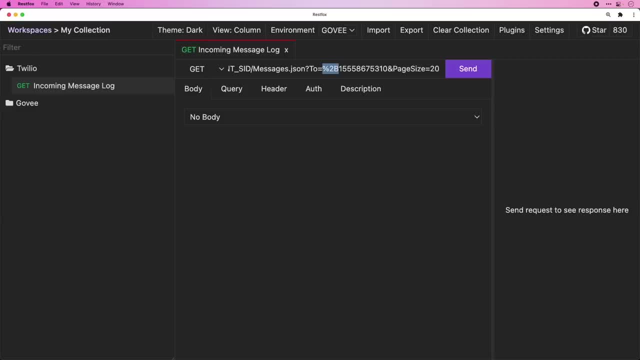 Like we didn't need to make this mess at the end. Well, check this out. Here's query right here. This is what we want, So we want to add this query. We don't want to have this whole stuff at the end here. 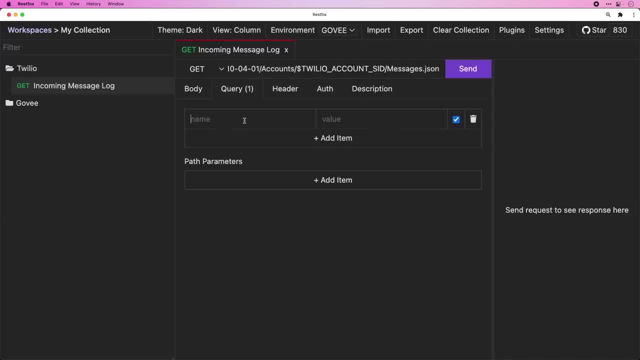 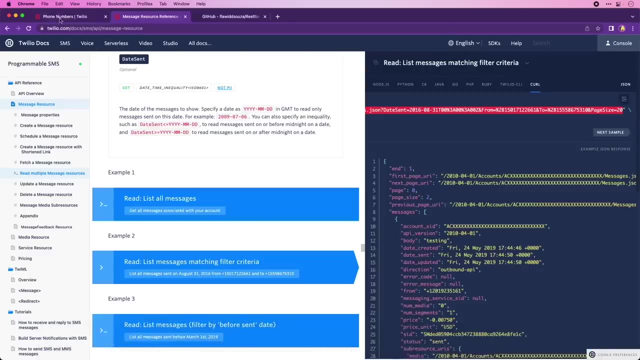 We want to put in a two. We're going to add one of those things there. We'll put in a two. So that's going to append that query string for me And I'm going to put in to my phone number, which again my Twilio phone number which is over here in my logs. 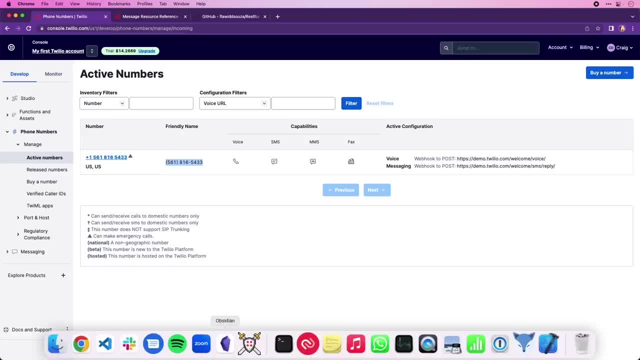 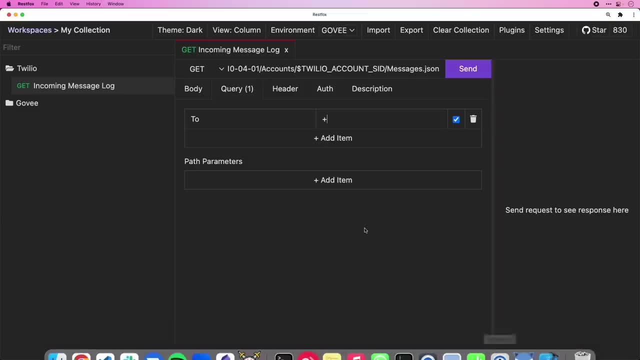 Right here. actually, I'm going to grab this number. This is my Twilio number. I'm going to put it in the format that is wanted there in my rest box. Here we go. So I'm going to use that. We're going to get rid of this. 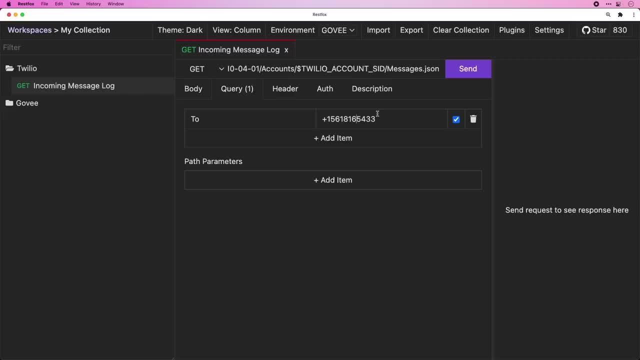 We're going to make sure that's one, Five, Six One. There we go, Got rid of all those, All right. Now also, remember that this was accounts and then it had account Sid, right. So that's the ID for my account and then it's under messages. 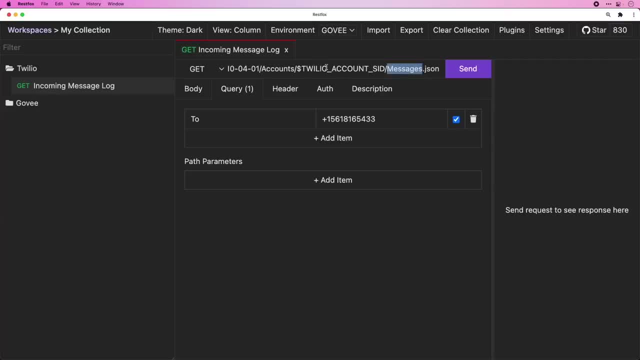 There's a collection called messages underneath this account, Sid. But what we want here is we want that was using an environment variable from curl, But this is also known as a path variable right, A path parameter. So here down here we have this path parameter. 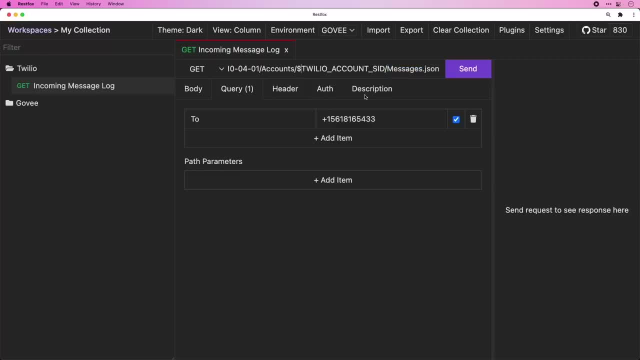 So the way that these work actually to replace them is if we go like this: if I get rid of this and I put a colon, what's going to happen is we can. anything that's down here in this path parameter will replace what's here. 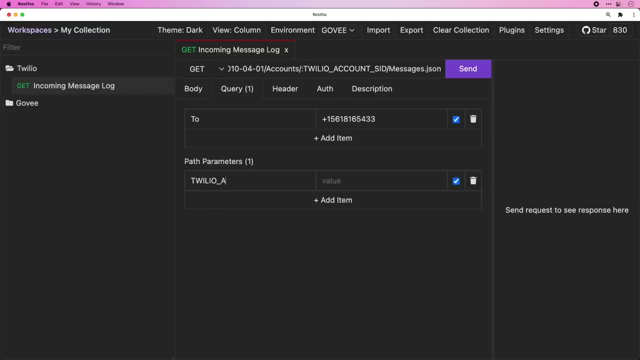 So let's do that, Let's add this item. And again, that is Twilio account, Sid. So that's the name of the variable that's up here. right, It's colon Twilio account. So that was just what's there. 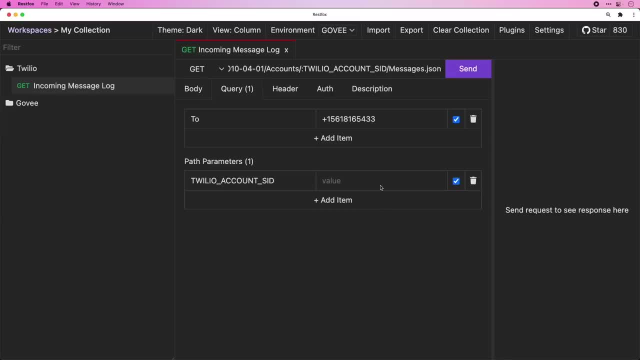 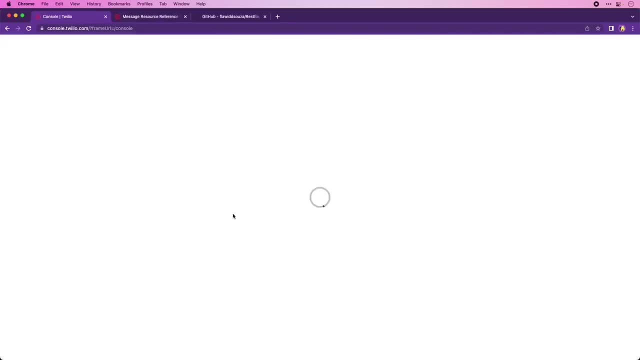 Let's keep it because that's what it is, And then we're going to put our account, Sid, there. So that also is on my console. So I'm going to flip back To my console And on the main page, here You come in. 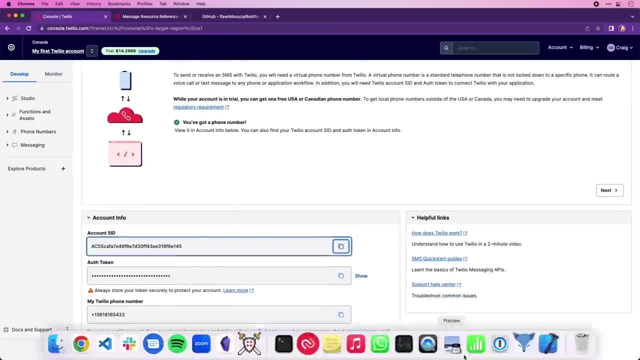 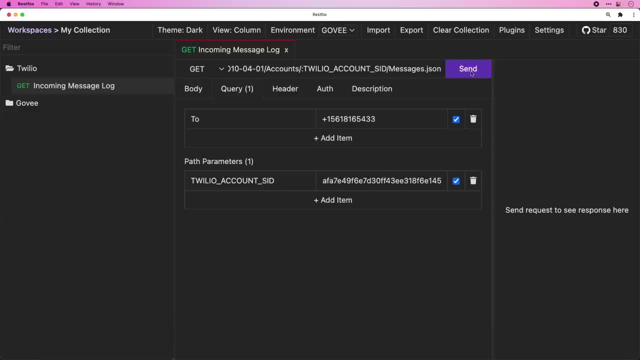 You can come down and you can grab your account Sid. So now I have my account, Sid, and I'm going to paste that there. Awesome, And I think we're ready. I'm going to press send And oh, we got an error. 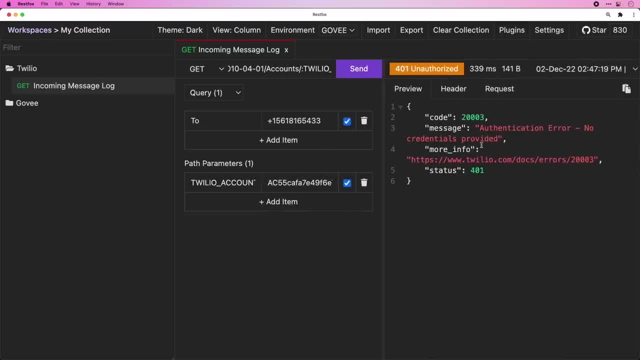 We got a 401 unauthorized, No credentials provided. Oh, that's right, Of course we want to log in. We don't want anyone just being able to see These messages, So we want to make sure that we have some authentication happening. 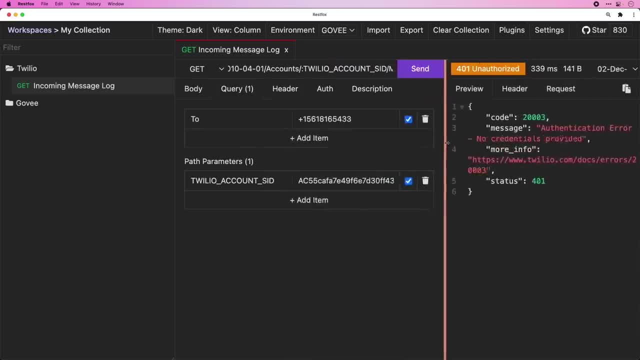 So I'm going to head over to the off tab. You'll see that if I slide this back and forth, I don't know how much screen real estate you have, but you can. you can slide these kind of around as need be. 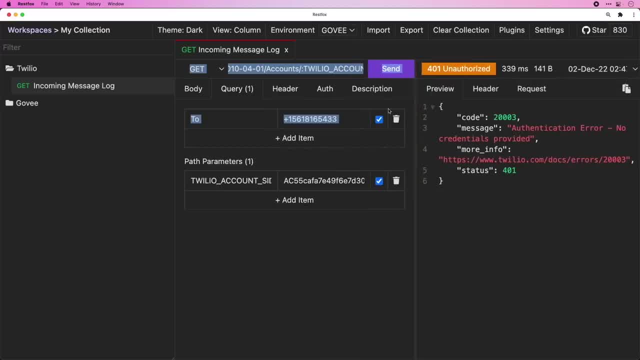 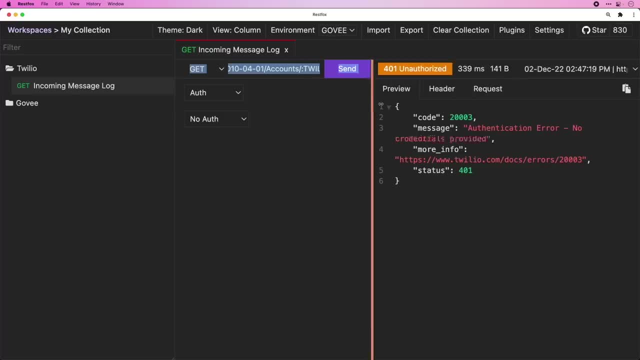 So I can. I'm going to pull this, and you'll see that when I do my, my little menu here collapses, So I'm going to choose off from here, but that that is also available in the header here, right? So like it's just a different view of it. 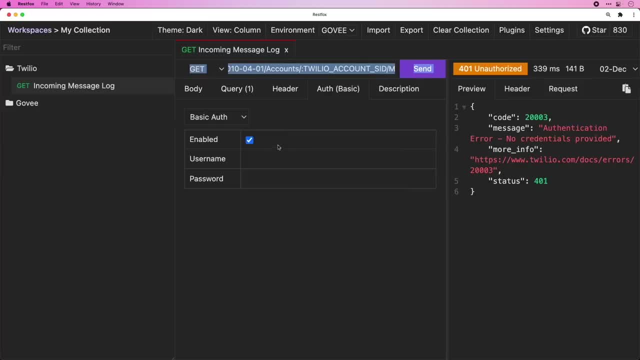 All right, So in the off I'm going to put in a basic off and I'm going to put in a username, which is my username, And then I'm also going to put in, uh, my password, which is my off token over here. 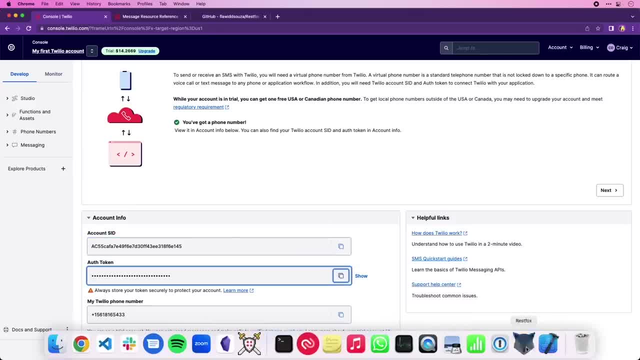 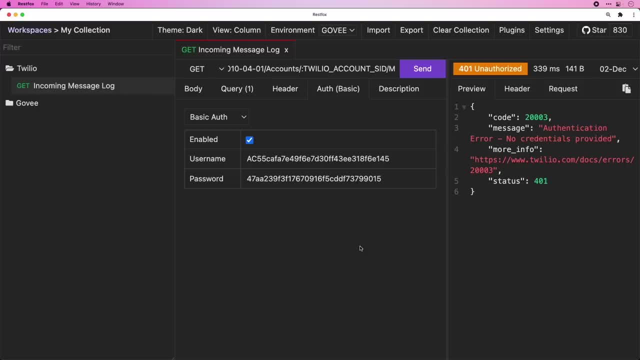 And again, this is very private and you would never, ever want to do this. Uh, you now know my off token. I don't want you to have that. um, uh, uh, because, uh, you could do exactly anything you wanted to to my account. now that we're there, 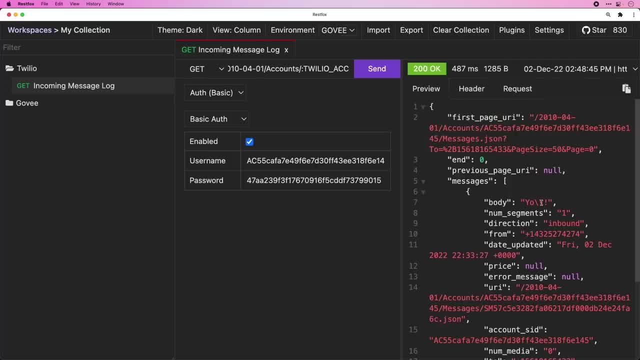 And one Of the things that you could do is see the messages that were sent in and look there's my yo. my yo message has made it in Um, awesome, So uh, also, I wanted to show you the request that happened. 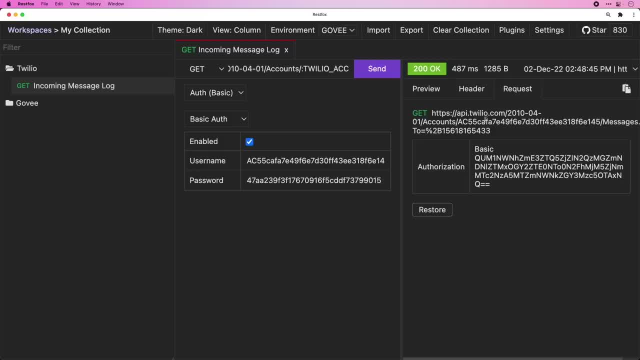 Let's take a look at that. You can see that what actually happened was it was a get that was sent, with the account said: right, And so that was the account said that we used from. if we look back at the query parameters here, the account said, uh, showed up there and then, uh, it automatically did a two URL. 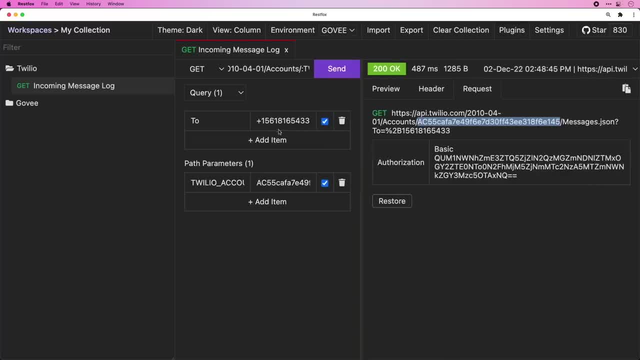 Encoded And if you look, it put the question mark in for us and it did that percent to be for us automatically URL encoded. Very nice, right, And we can see the headers that were sent and we can also take a look. 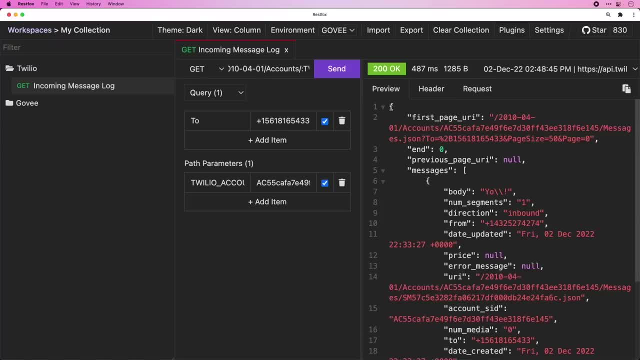 Let's look again at this preview So we see that we had, uh, the. the response came back and this is Jason, right, So we have a key called messages and this messages has this: uh, it starts out. there could be multiple messages here, right? 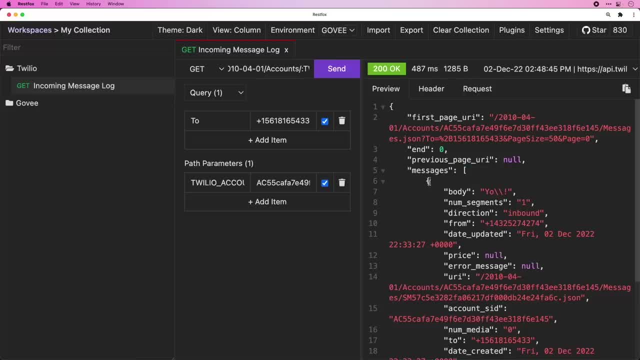 So this is a the start of what's a known as a list or an Array, and then there's an object, and the start of the object is always done with one of these mustaches. And we call those mustaches because if you kind of turn your head sideways it looks like a mustache. 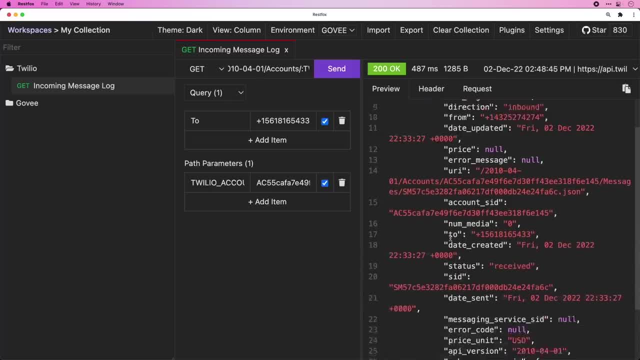 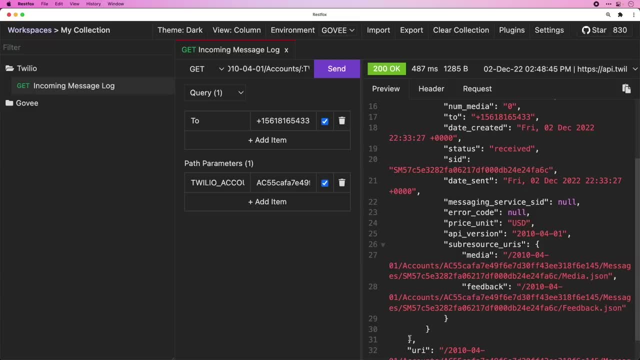 So, uh, all between the opening mustache and the closing mustache, uh is the information about um the messages right? So here's the and there's the closing uh bit of my list. There's only one. 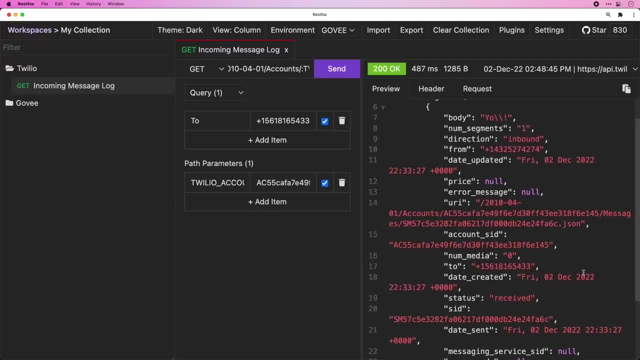 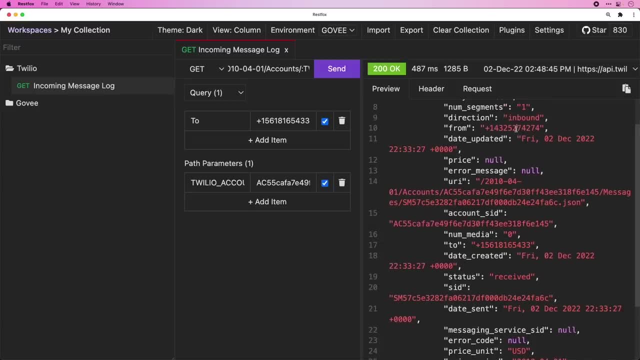 This is the closing mustache there And, uh, so part of the message that we could see. we could see who, uh, it was Two. that's that's my Twilio phone number here, And we could see the from. there's my phone number there. 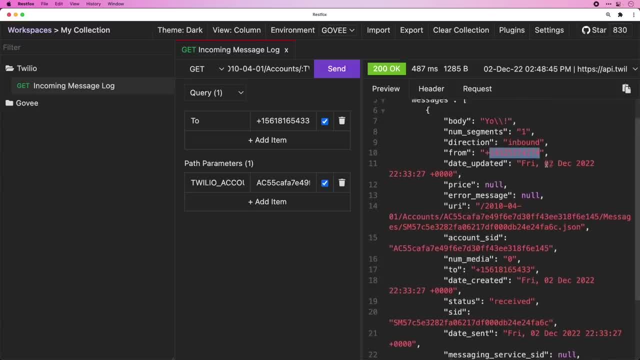 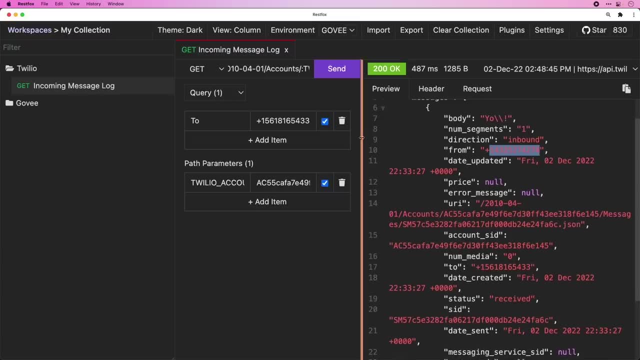 Please don't call too late. Uh, but that's my, my phone number. Uh, and I did say I said yo to it, which is awesome, So now we have this. now this step is completely optional. This is something that I like to do. 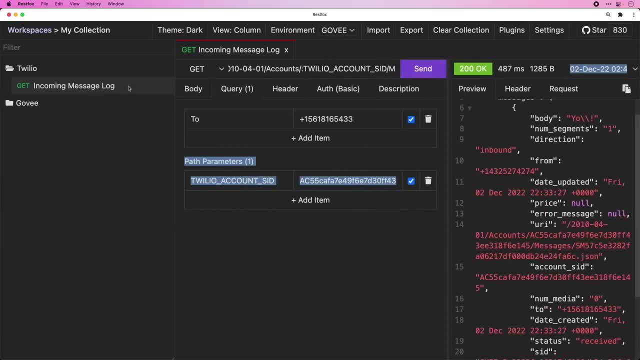 Uh is, I like to take notes, All right, So there's this incoming message log. I like to keep notes and I put those in the description over here And so, uh, uh, let's see. uh, this returns. 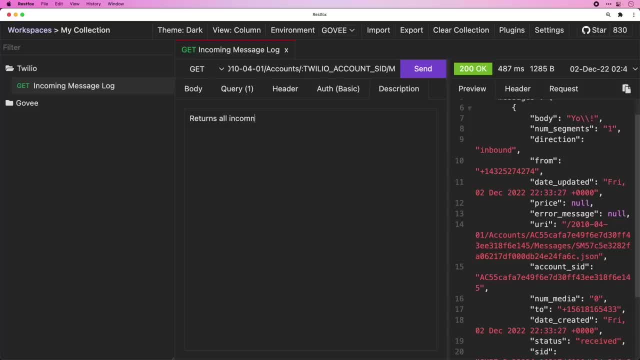 All incoming. well, let's- let's be a little more- all messages uh sent to this phone number, Right And uh. one of the things that I like to do is I like to put on, uh the docs here. 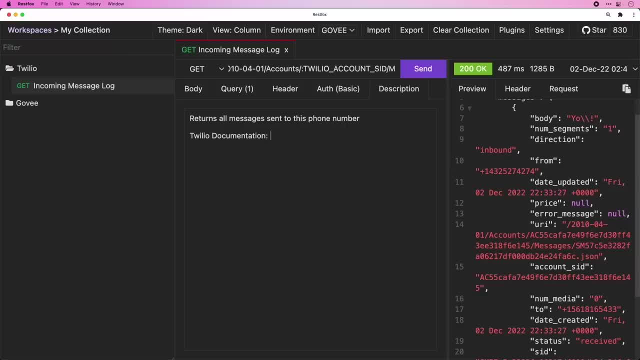 So if I ever come back and I want to find how was it that I learned how to do that, I can come go and look, uh, and put a link there. So I'm going to go flip back over to this docs real quick. 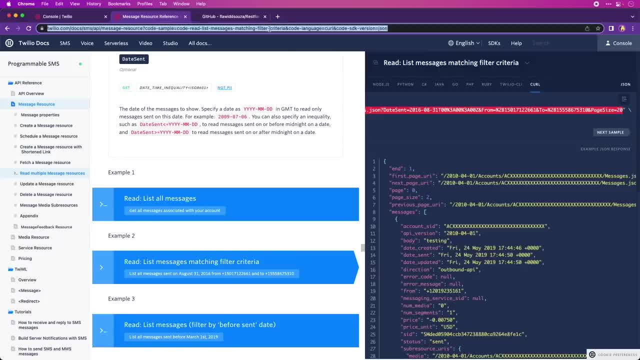 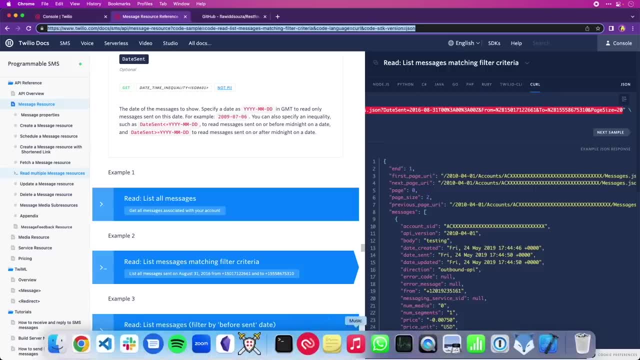 Uh, and this is read, a message with matching a filter. I'm going to copy this. I'm going to grab this or a click this here so that then it changed the URL up here When I copy this. this is what I'm going to store in my notes. 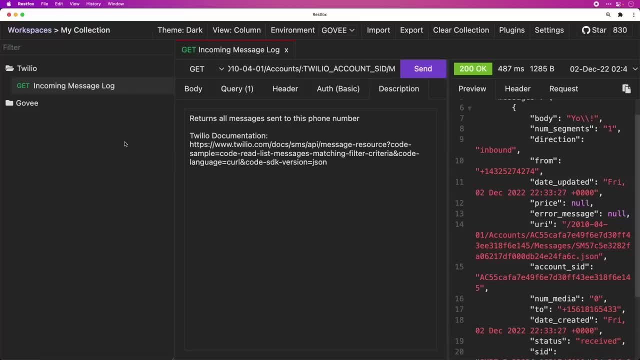 Again, this is totally optional and this is just notes for you for later, because you could end up having a whole bunch of these. You might not remember how you found how to do that. If there's something specific or strange about the API that you wanted to know, I keep the notes in there and it's a just a handy learning tool. 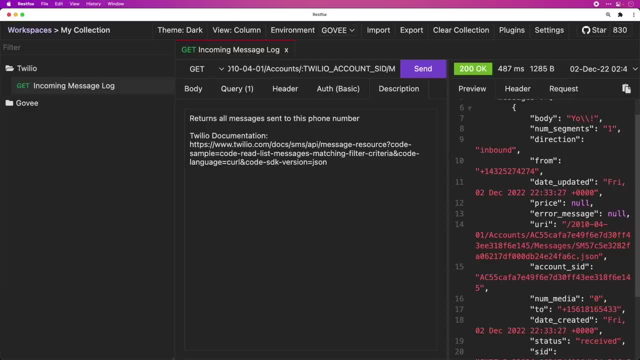 And again totally optional. So we've got our first entry all set and I think we should add another. Why don't we create the send message one, right? So the one that we did before we sent messages? let's do that. 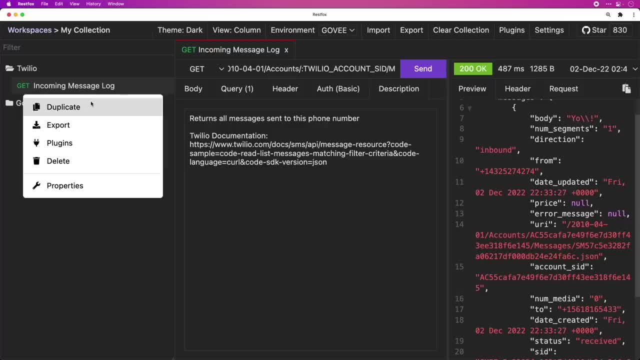 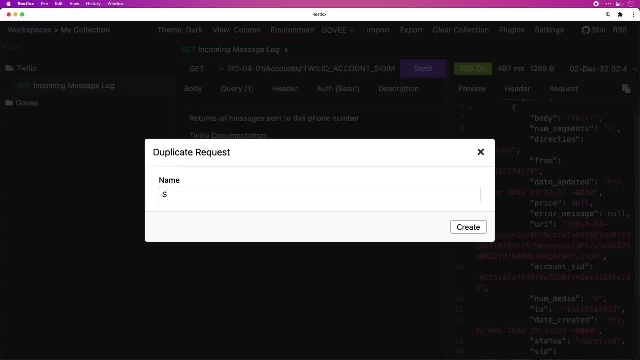 So I'm just going to duplicate this Cause it's got a bunch of the information that I already need in it, So I'm going to duplicate it. And uh, what I'm going to do here is I'm going to duplicate and I'm going to say, uh, send message, right. 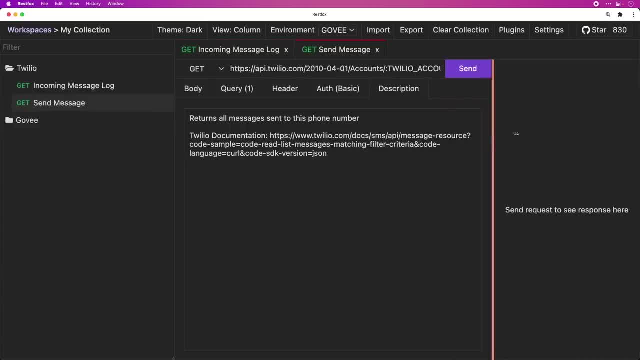 So, uh, when we sent a message before, remember it wasn't a get to post. So I'm going to change, um, I'm going to change that from uh, a get to send To a post. So now we've got this: send a message. 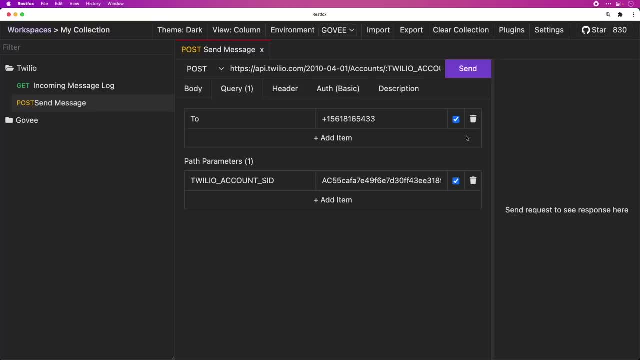 That's a post, uh and uh the query string. I don't uh want to send a query string anymore, Right? So remember, when we did this, we sent it to uh using the data URL and code. 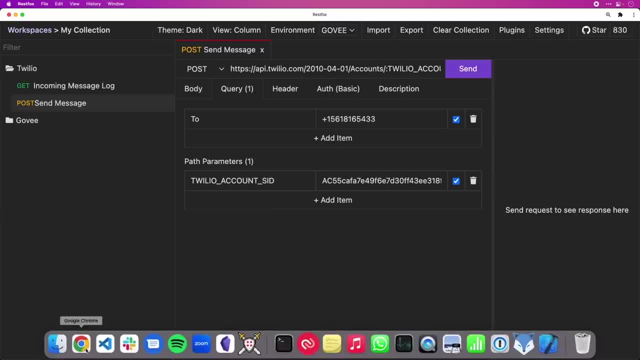 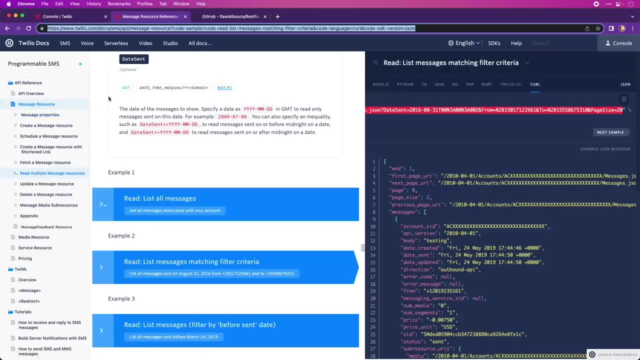 In fact, let's go, let's pop back over there and look at what it was that we did. So in the documentation, uh, over here we have this: uh, create a message resource. So so on the message resource page here we can look and we can go to this: create a message. 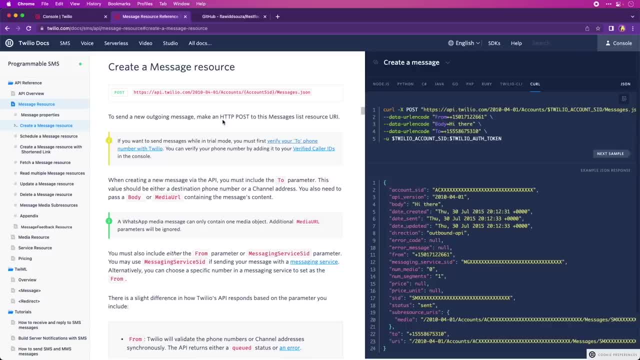 Resource and, uh, there's some information about it. So you send this HTTP post, Uh, and you can see that again. we were remember before we did this data URL and code. we were doing this uh URL encoded. 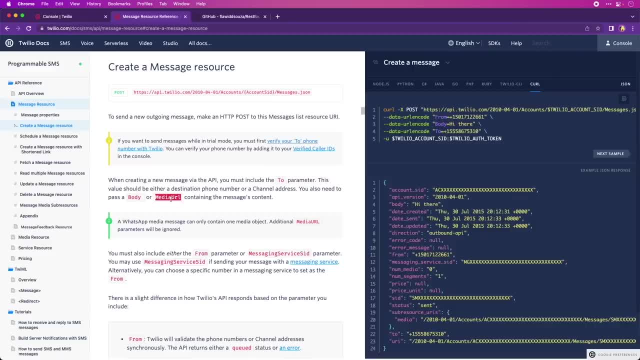 So it's this form encoding is what's happening here And oh look, uh, well, a couple of things actually. there's a nice warning here That says if you want to send messages while in trial mode, you must verify your two numbers. 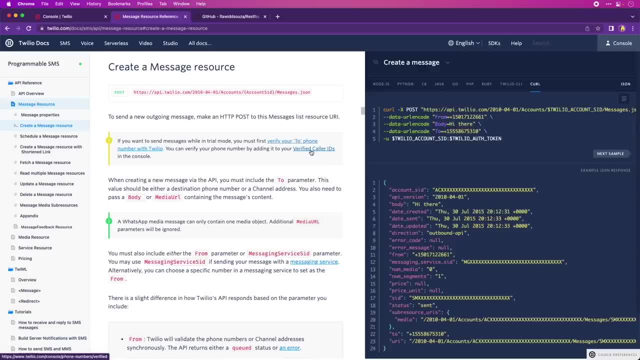 So if you wanted to send to somebody else, you could put them in this verified call caller IDs. If you want it to, you could send to somebody else as well. Um, just just there. That's how you do this. 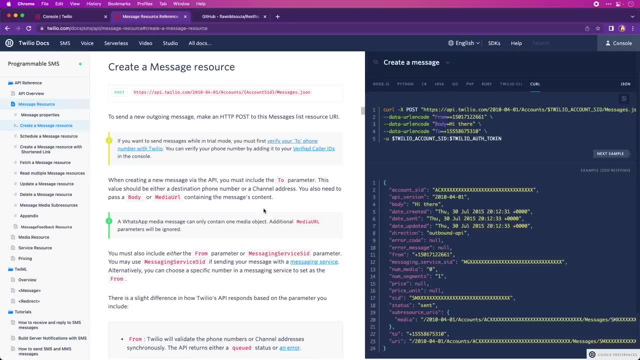 If you wanted to test or show somebody what you're building, um, that's, that's how you do that. Uh, after, of course, after you're not in trial mode, you could send it to whoever you would like to. 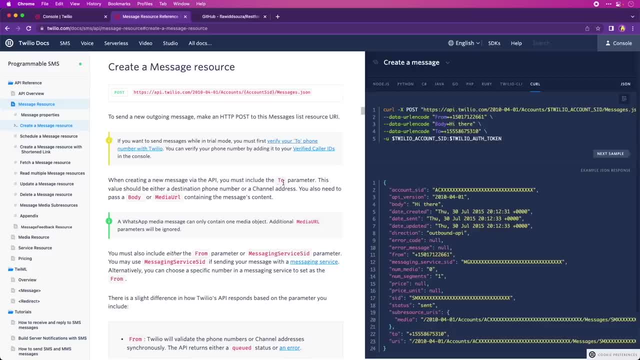 So, um, when we are creating a message, we must include the two right, We need that and we need the from. so we'll do either and we'll do body. and there's this media URL, which means I can send a picture. 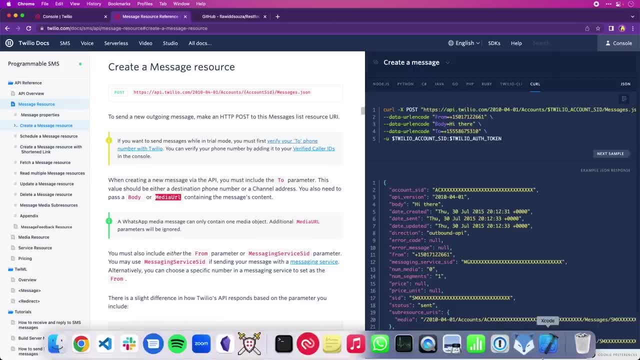 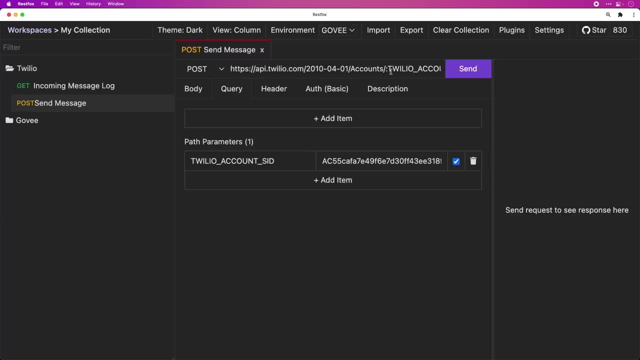 Let's, let's do that. Let's make it so that it sends a picture Now when I am in rest Fox over here. um, I don't want to use the query anymore. Uh, I'm going to keep the path because the path is the same, right? 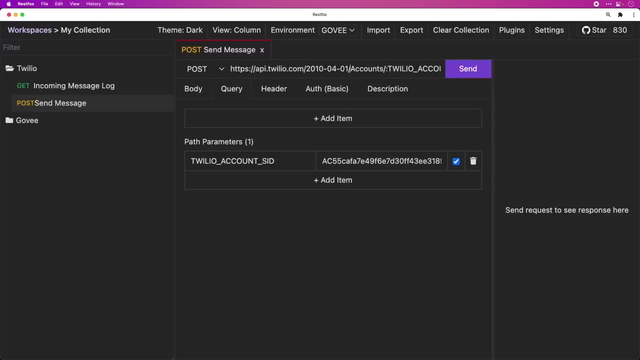 So we're going to do- uh, we're gonna do a post to that same URL. Twilio account slash uh account said messages dot JSON And we're going to make a post to it. instead of making a list and retrieving, we're going to create. 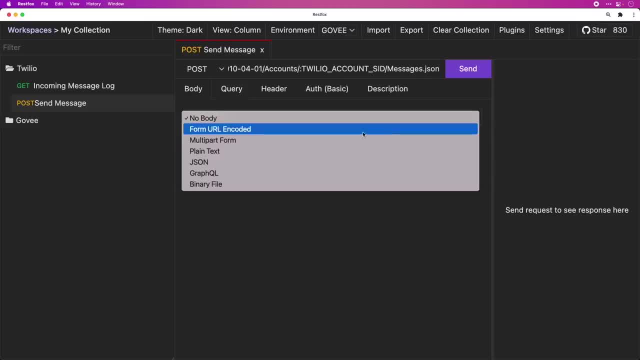 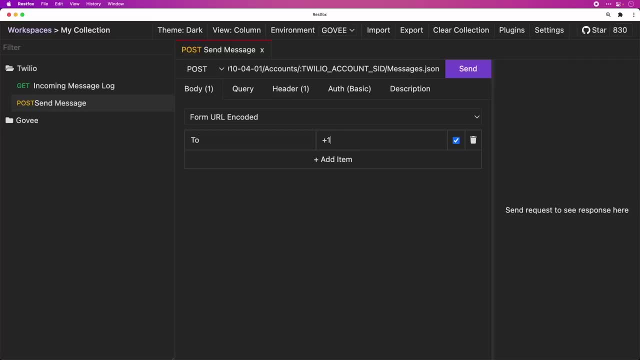 So, uh, we're going to go under body and for the body, we're going to make it form URL encoded, Uh, and what we want to do there is we want to send it to. so I'm going to send this to my number again. 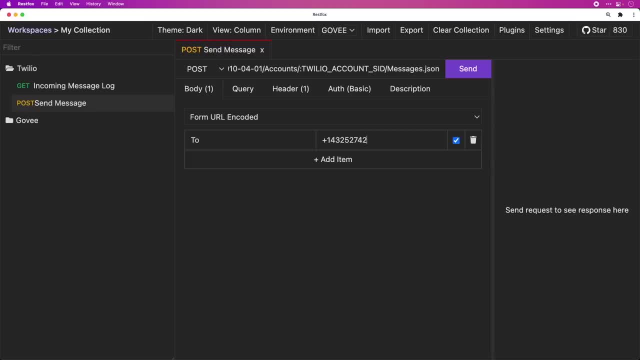 Don't call too late. Five, two, seven, Okay, Uh, four two, seven, four, Um, no, really, uh, if you want to call and get feedback, that's fine. Um, I'll, I'd love to chat. 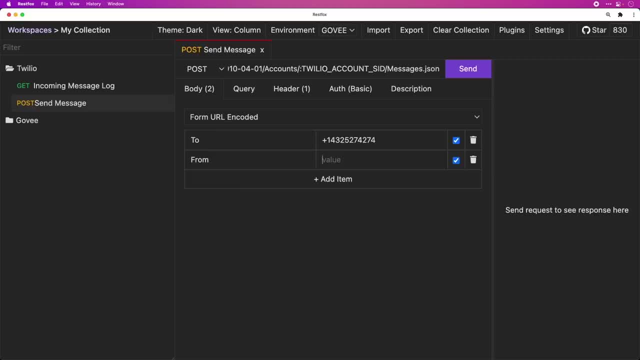 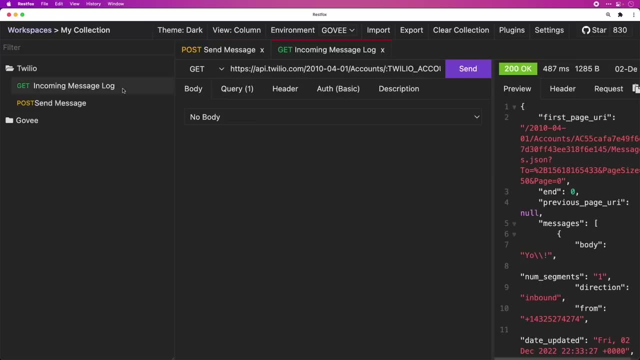 Um, so we'll do from and that is, uh, my number. again, this is my number And uh, what was that number? So we can come here into the message log. We can go pull that number from the query string. 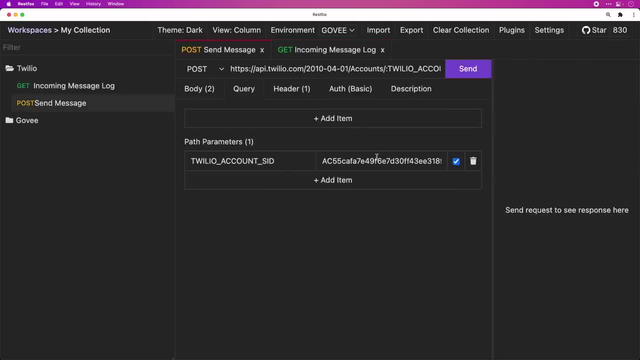 So this is my uh Twilio number there. Um, uh, from. is this value there? Yeah, And we are going to add uh the body. the body will say: uh, sent from, rest Fox, and let's add our media URL. 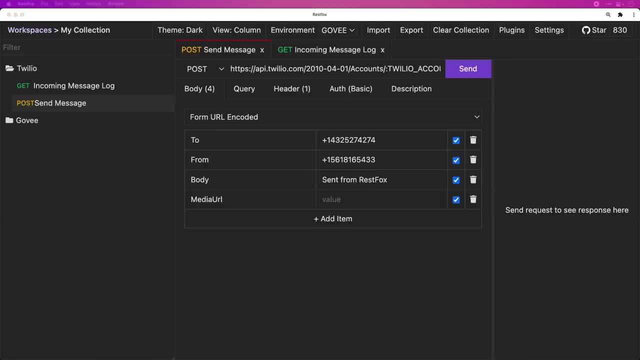 And I just happened to have one of my favorite photos, which you will have to um uh check out for yourself, um to know what it is, but it is a photo that uh I pick, if you will, that I'm going to uh send to myself. 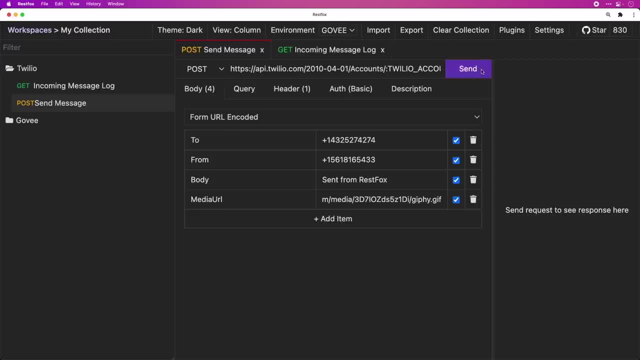 Um, it's also in The notes, if you want to do this as well, if you want to copy that and paste that. So here we go. I am going to do a send Now. remember, I'm also authenticated with my, my username and password, because that copied across when I did it. 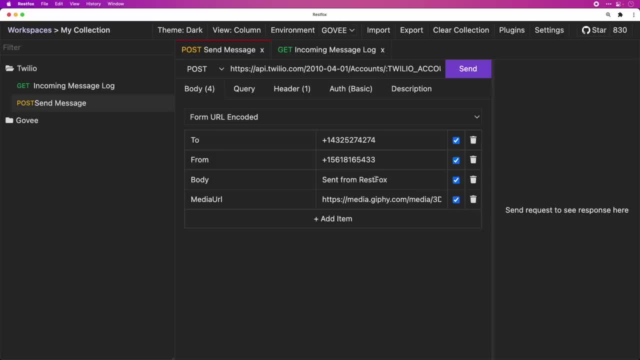 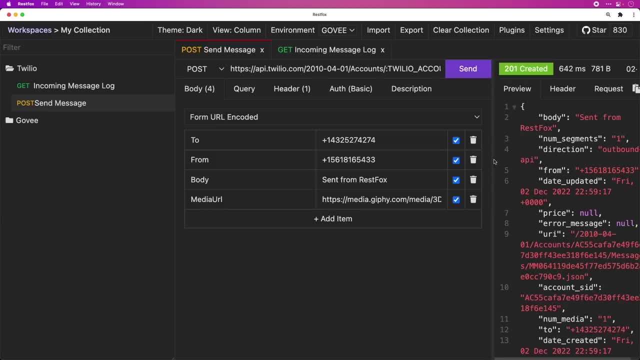 So I'm going to do a two from a body and a media URL. So now I'm going to go ahead and click send and boom, we got our message back Right. So the response: we got a two. Oh, one created right. 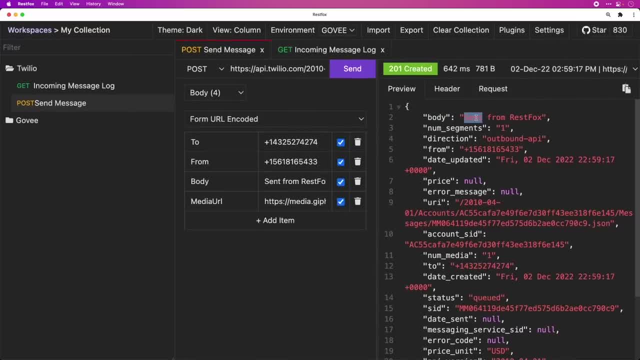 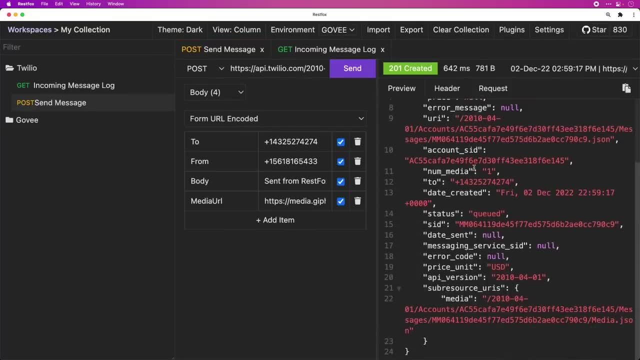 So it was created. uh, in the body We could see the body of our message. The key is sent from rest Fox. Uh, it's got some information. We can go ahead and uh get access to that uh message if we wanted to. 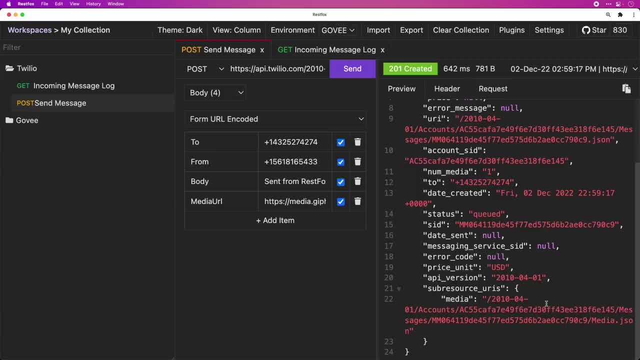 And it's got these actual uh media resources down here which we can also take a look at- And we could, if we wanted to open up a whole nother one of these and explore and see what that looked like. But let's take a look at that in a new tool before we do go to look at that new tool. 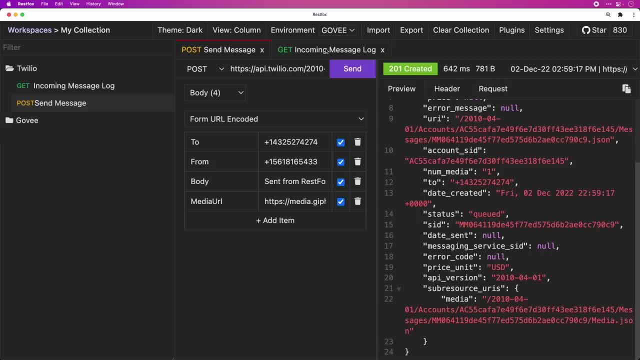 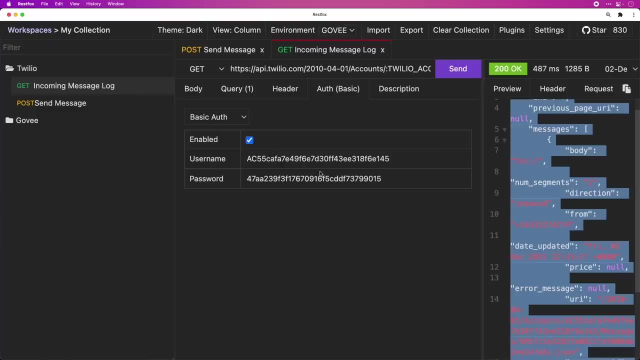 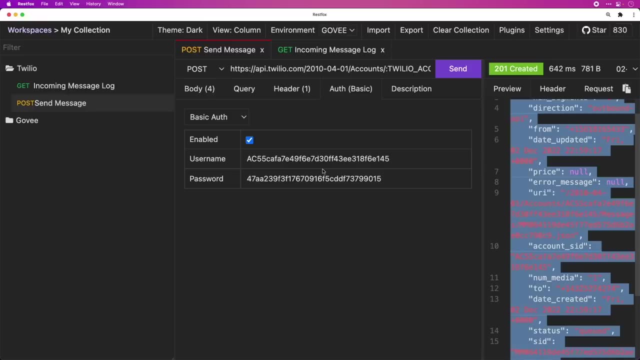 One thing that I don't love about what we just did are, um, in my, in these requests and these separate requests, these, these, uh, these, These are duplicated, right, I've got this username and password. If I go to my post, uh send message, I've got this username and password and they're duplicated there, which is a great right. 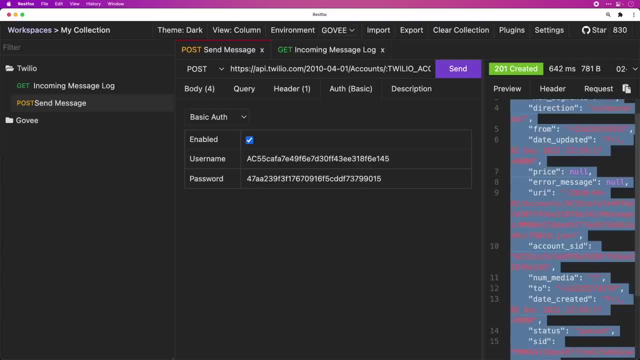 That's not, that's not excellent. Um, uh, one of the things and one of the tools that most of these uh rest clients provide is a thing called an environment, And let's set that up really quick, real quick for this. 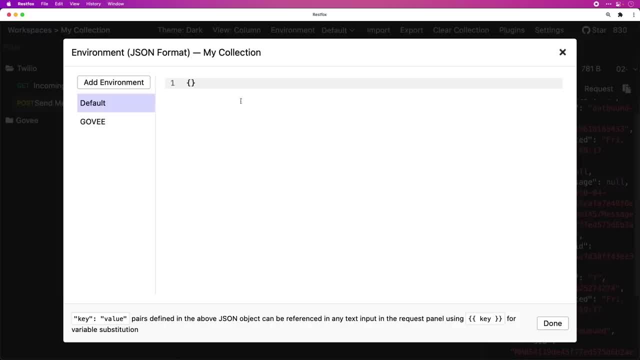 Um, so, if I come here under this environment, here is my default uh collection and I can add a new environment. I'm going to add one. I'm going to add one for Twilio. now, the way that these work, uh are they are JSON based. 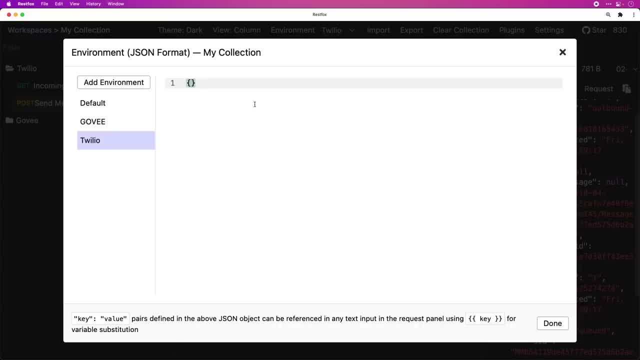 So, uh, this is remember. this is the start of an object. Now, if you've never written written JSON before, take your time, use some patience. Uh, one of the things that you could do is you could come in and you can put in: uh, account Twilio, account Sid, and uh, you do the key and then you do a colon and you can see that I'm- uh, this is unexpected JSON down here. 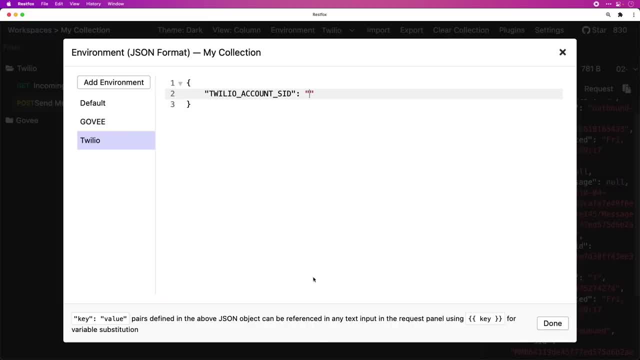 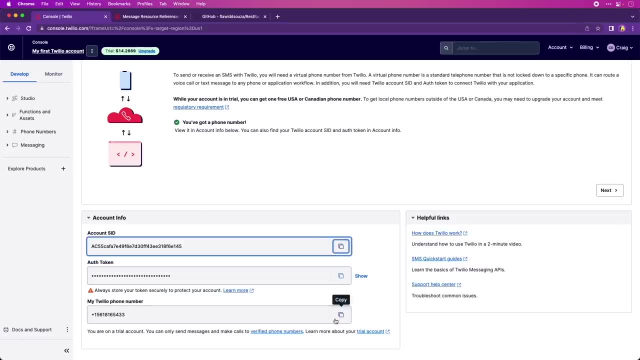 It's helping me out. Um, uh, and now. Uh, I'm going to put in my account, Sid, and again, let me go copy that one more time and I don't have to copy this anymore, because it will be part of my environment. 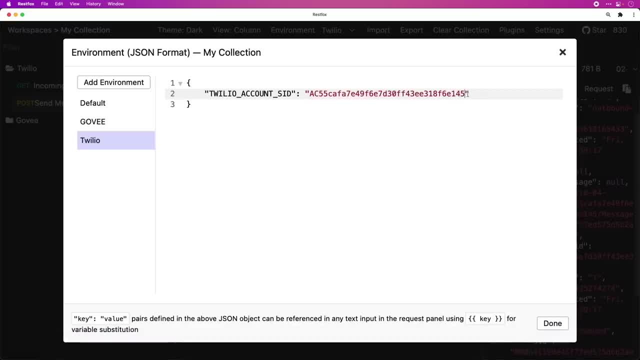 It will be here with me, which is really nice. So come over here, I'm going to paste that, And now I want to add a new key. So the way JSON works is you put a comma after that, right, And I'm going to put a new uh, the new key here, and we'll do a Twilio uh account or uh off again. 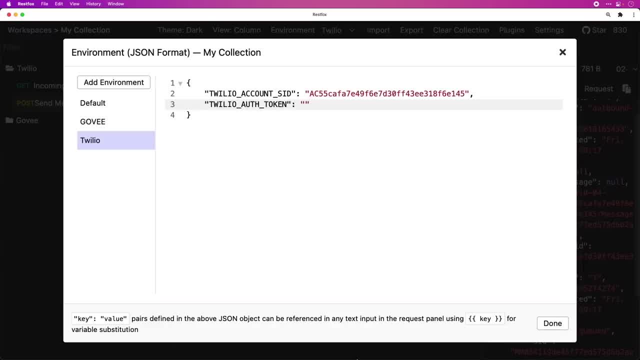 And again, this is: uh, that can be that key, can be whatever you want it to be, And we'll be able to reference It. So I'm going to come and grab my auth token. I'm going to change this right. 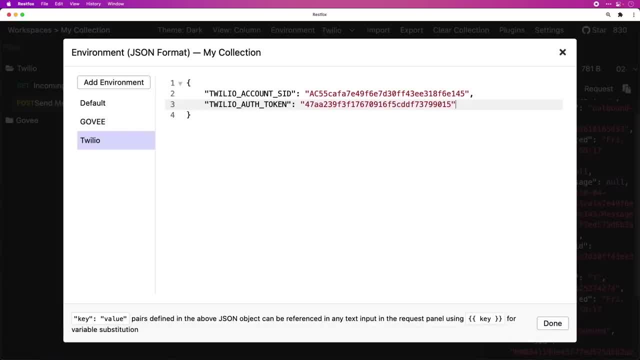 So, uh, that that's a great use case of this is. I don't want you to be able to. uh, I am going to change this right. So, as soon as this, as soon as I'm done recording this, I'm going to change my auth token. 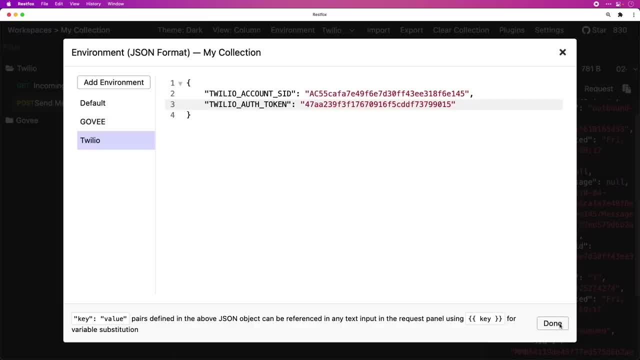 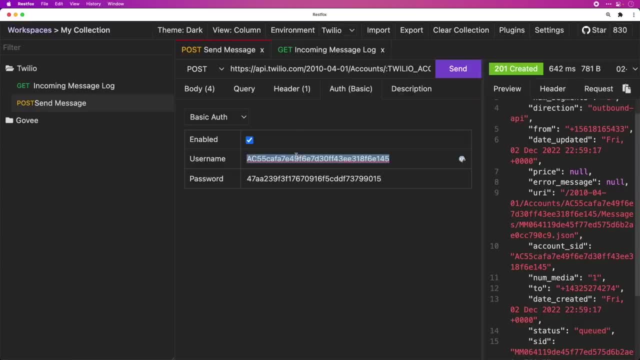 And that would mean that I'd have to go change each one of them. But now I have one place where it's defined. I have one place in my environment that's defined. So I have this environment here that says Twilio. Now, instead of username, I can do this. mustache, mustache. 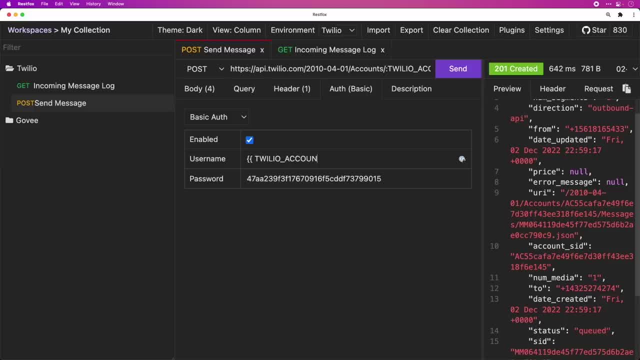 And I Can say Twilio, uh account said, and uh, th, th. that's the way the templating language works here, And then most of these rest clients, um, and you can do uh Twilio, uh token. 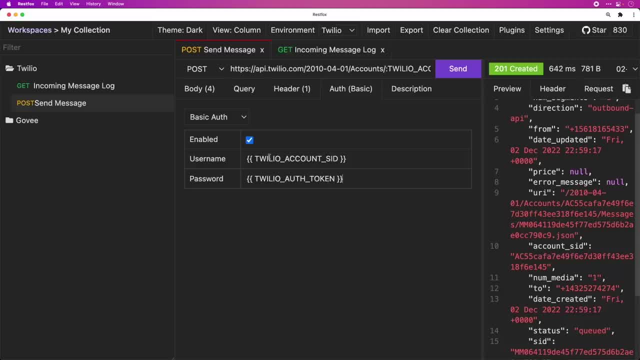 So when you see that that's what's happening, that is, the environment is using the environment variables. I'm going to go do that for here And also I'm going to copy my auth token for here, And so now I only need to change that in one place in my environment. 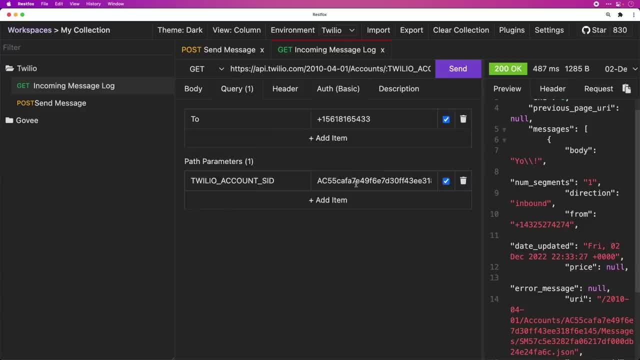 Um and uh, you can also use it here. So, like, no like, before I can, I can also put my account said here, Um, so that will also make this so that it's shareable, right? So, um, if I don't specify my information in here, I can share it. 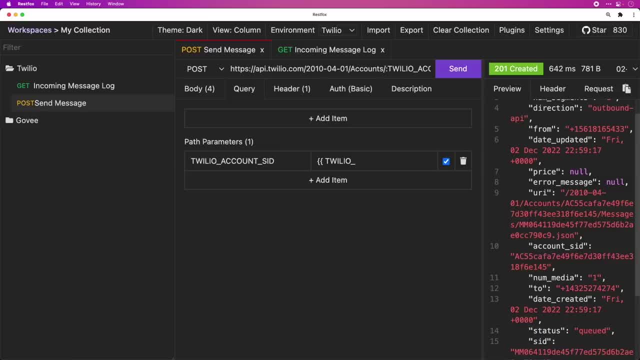 So you what you could do, and actually why don't you try to do it? Why don't you try to add your Twilio phone number? and uh see if you can figure out how to add to your JSON there: uh, your Twilio phone number. 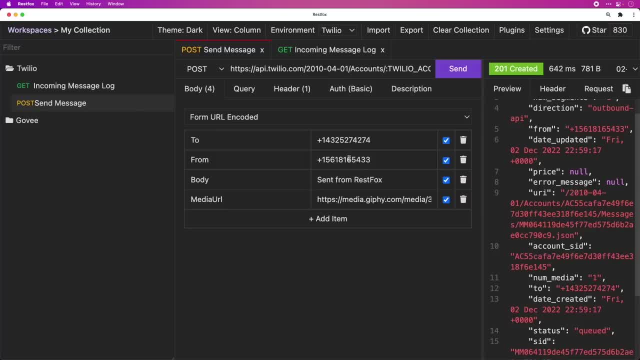 And then you could replace it. right, You could replace it here with your uh, with your from, from your Twilio phone number. Uh, pretty neat, right. So that's a good, that's a good little trick that you could do in here. 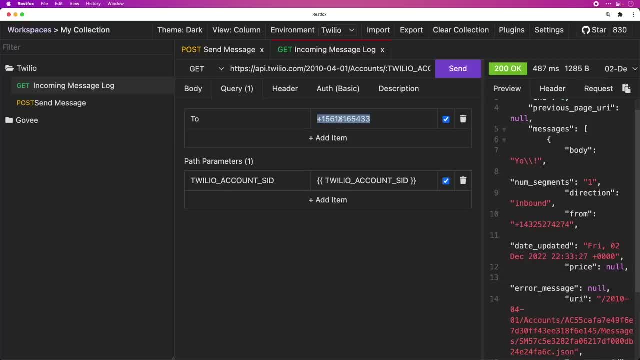 You could do your Twilio phone number. You could use it there too. So anything that you're using is something that you can kind of store there in your environment, And what's nice about that? let's make sure that it still works. 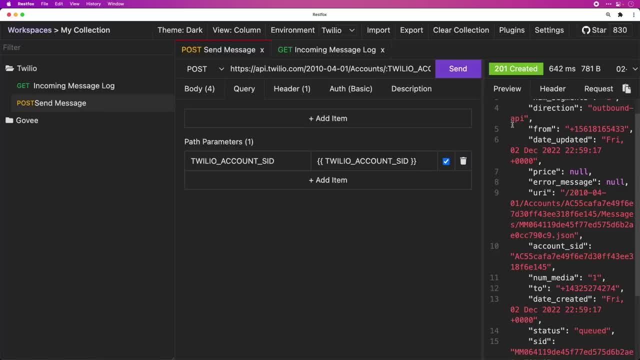 Yep, It's still working and let's make sure my oh, I'm not going to send another picture to myself, That's fine, Uh. so, uh, we know that this uh environment is now working And it's here, and I don't need to go back and get those every single time. uh, really handy. 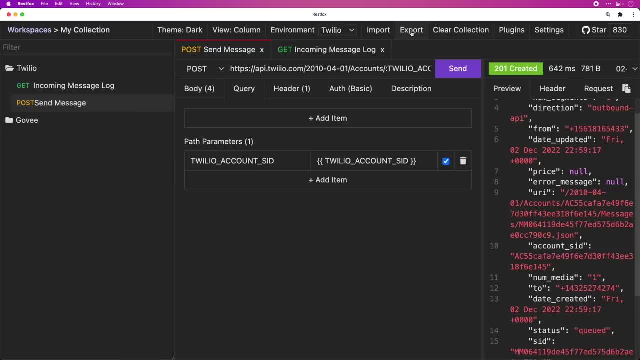 And what's nice is you can do these imports and exports and we'll take a look at that here in a bit. So, uh, when we get back, we're going to take a look in a different tool, uh, cause this is rest box. 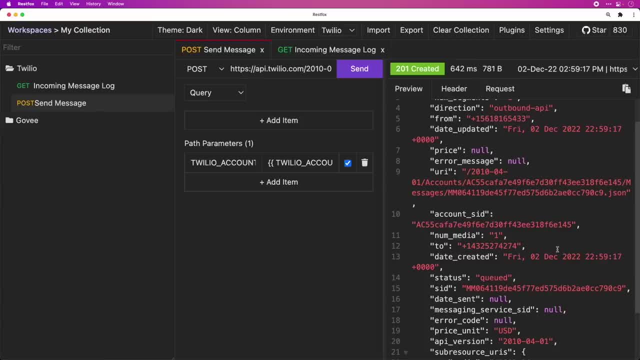 And I know that you're probably getting ready for a rest, So let's take a quick break, Um, and then let's see if we can't retrieve that pit that I sent myself via this API. but let's do that in another postman, Naney, uh, their rest client, uh, right after a quick break. 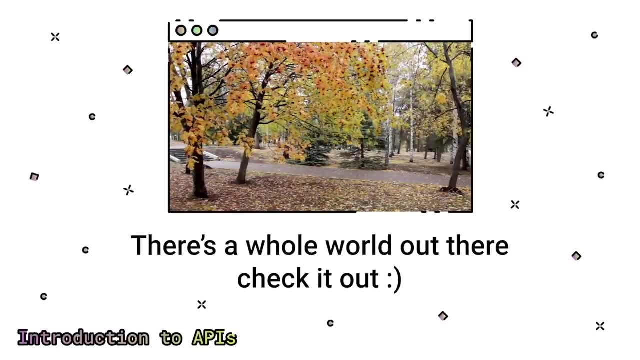 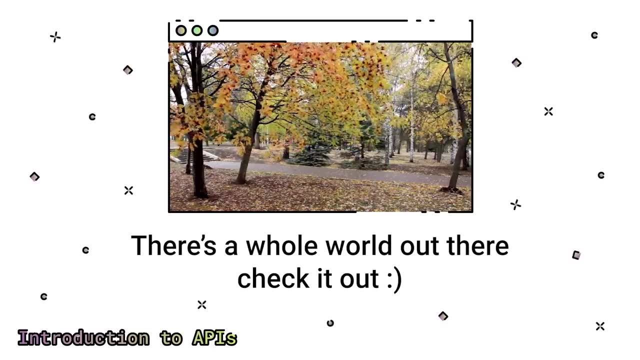 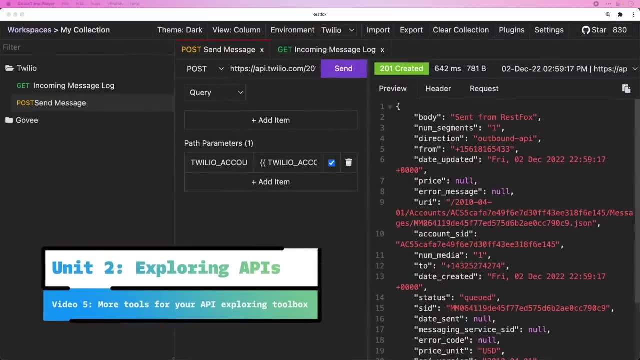 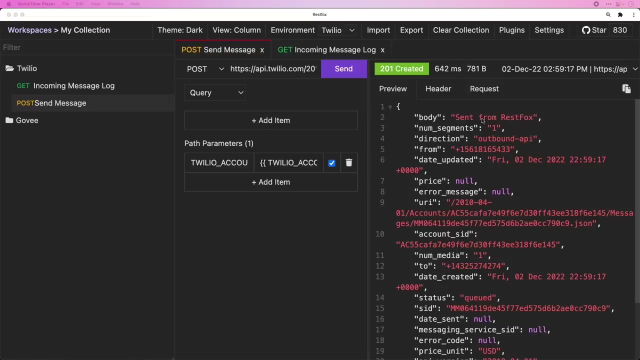 That is All right. Quick refresher. We had just sent a message from rest Fox, a rest API client. Uh, here's the body of the message we did sent from rest Fox And we actually sent across, uh, some media with it. 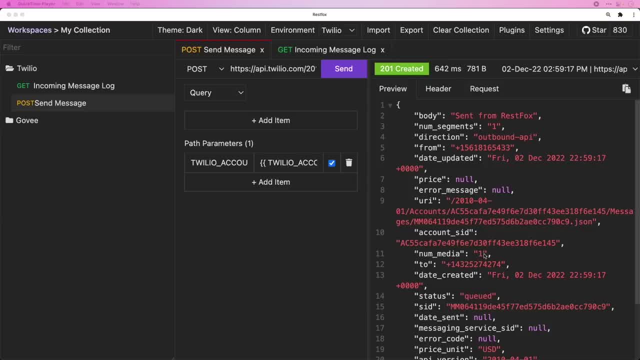 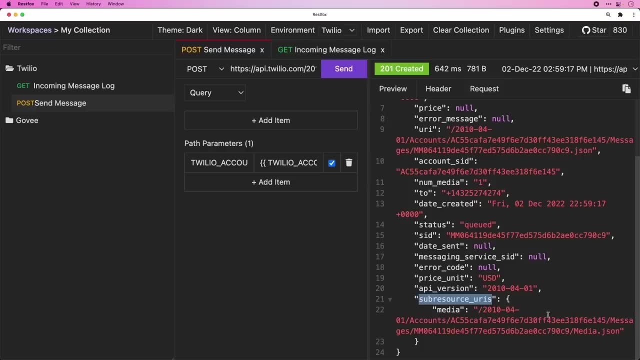 You can see here it has this numb media, One cause: uh. each text message can have multiple uh uh media is attached And if you scroll down here, you'll can see that there is this uh key of sub resource URIs and it has a list of um, an object here. 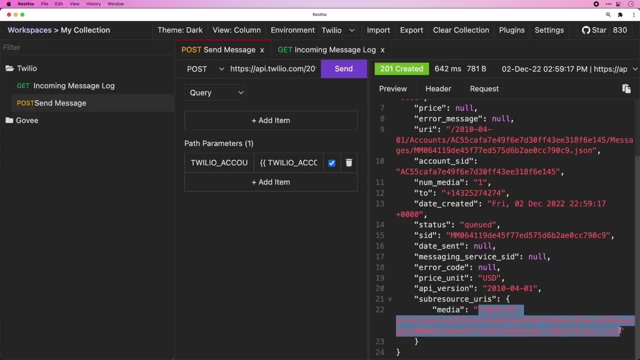 And one of the objects is for media, And what this will do is this: will allow whatever's at this URL, will give us the uh accounts. uh, for this account, for this message specifically, it'll give us all of the media that is listed now. 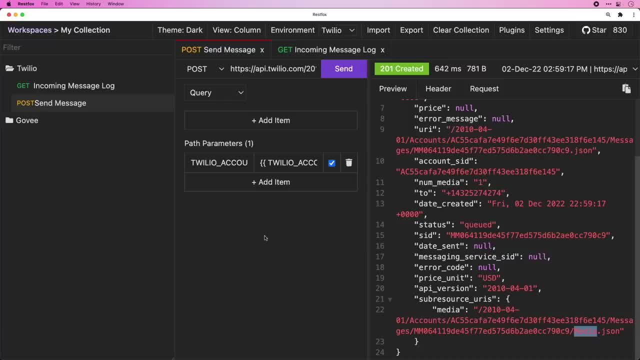 Um, typically, When I have something that's: uh, this far out. we could actually add another one here, but I thought I'd show you a little bit of how my process normally works, in case you wanted to, to see what that felt like. 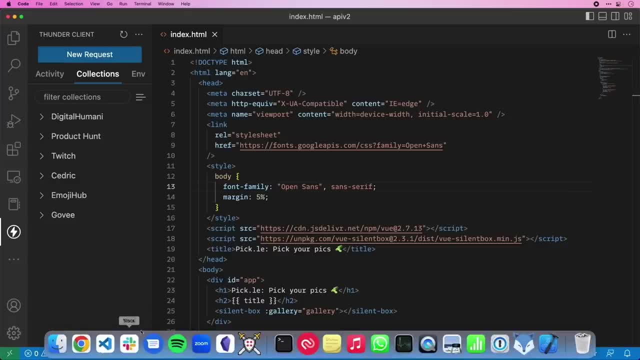 So I use an editor called visual studio code. It's free, It's available And this is where I do my coding from. So I start, I start here, I start working on my coding. I would love for you to go ahead and download this um, because I want to show you a tool that's inside of here that will allow us to do a rest client as well. 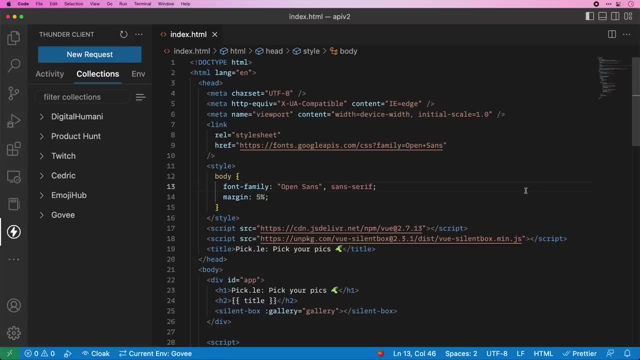 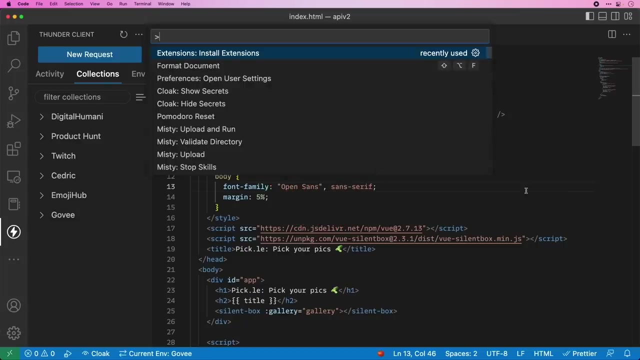 So go ahead And pause Me, get visual studio code, uh- installed, And when she do come back and uh, I'll show you something. Okay, So, uh, once you get visual studio code up and running, if you press a command, shift, P, there is a thing called extensions. 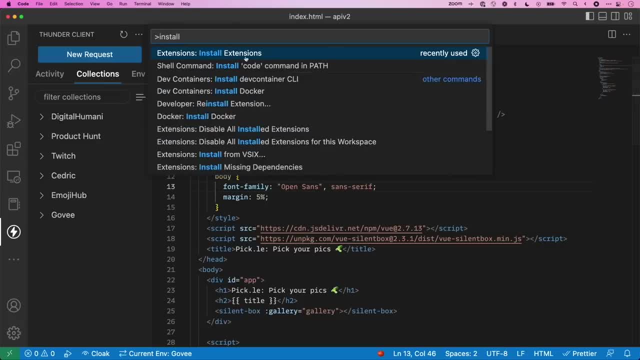 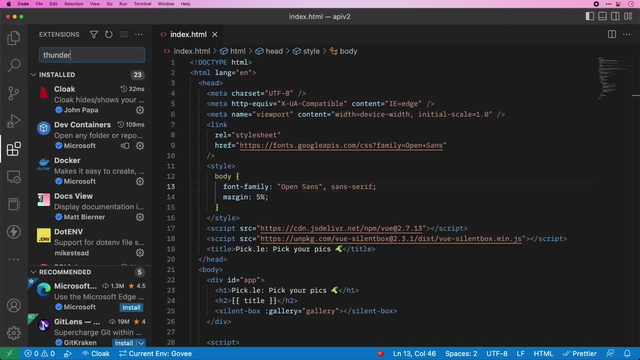 And this will do a little. if you type in install extensions, you can come here and you can see different things that are available. What I want you to install is a thing called thunder. We're going to do install a thing. It's called thunder client. 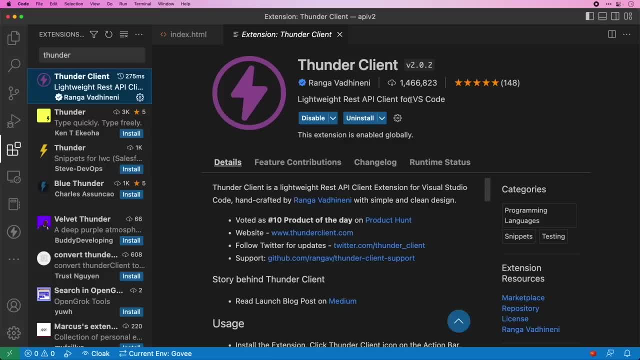 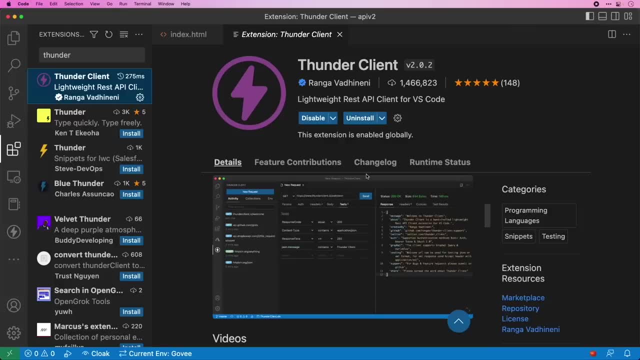 And it's this one here. It's a lightweight rest API client, uh for Vs code. It's really powerful And the good news is is it is post-man ask. you are going to feel very familiar when you take a look at this. 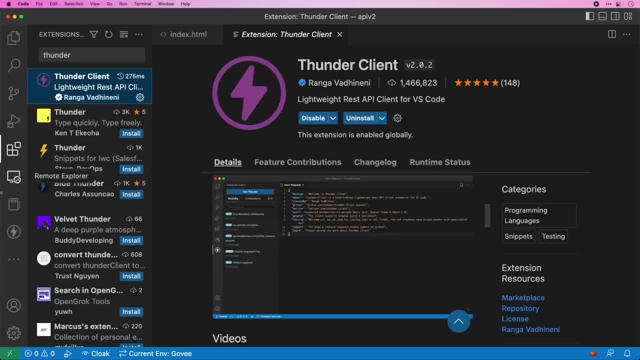 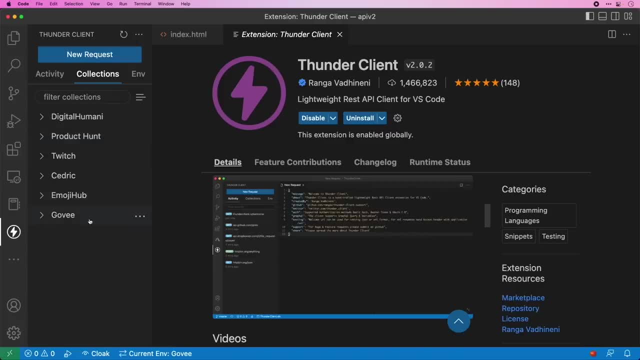 So uh. if you do it, you can go ahead and click install Uh, and what will happen is there'll be a little thunder client that will install over here like so uh, and just like you've seen before, there are these, this concept of uh collections, and we can make a new one. 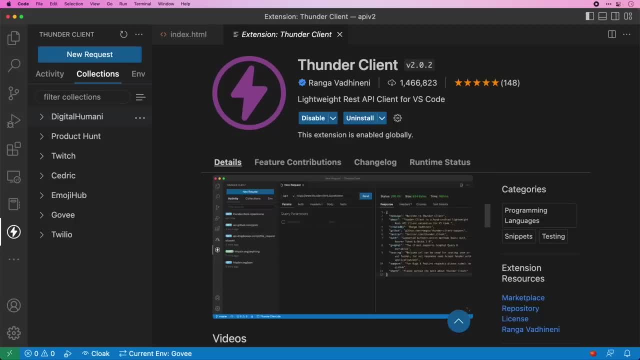 So I'll make a new collection, uh, for Twilio. Uh, and typically what I'm doing is I'm coding and I run into this API and I'm like, Ooh, I wonder what this is. Uh, I've been to go, uh, explore it a little bit and I'll explore it right from my editor. 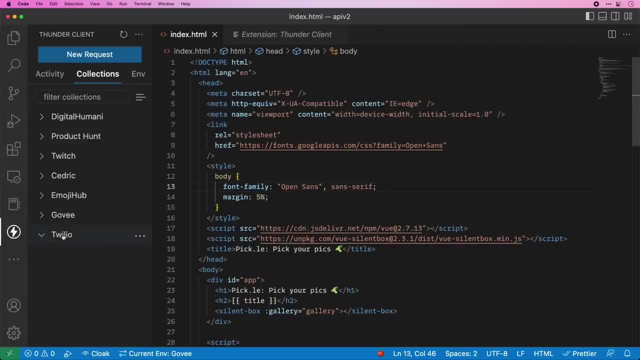 Right, So I'm writing my code here, and then I could come over here and just take a look at, uh, what was there? And so, uh, let's go back to rest Fox, and I'm going to grab that rest Fox that we had here. 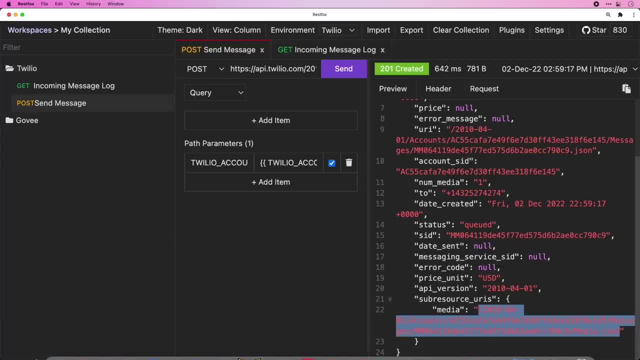 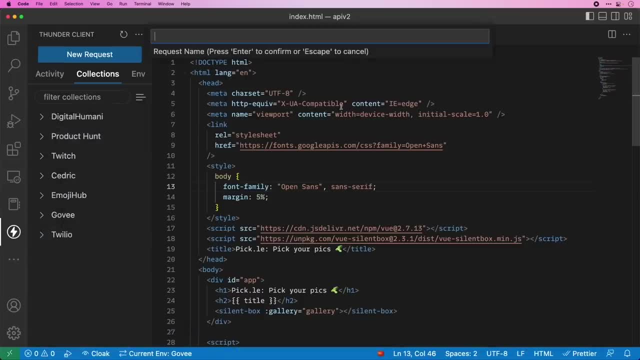 Right, So we're going to do that And I grab that and I'm going to come back over here to uh Twilio. I'm gonna make a new request, I get to name it, And this was the media check. 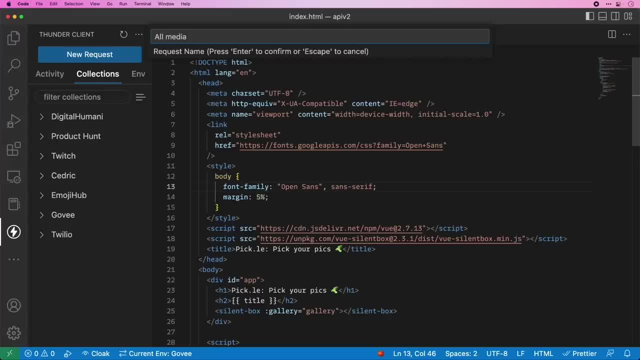 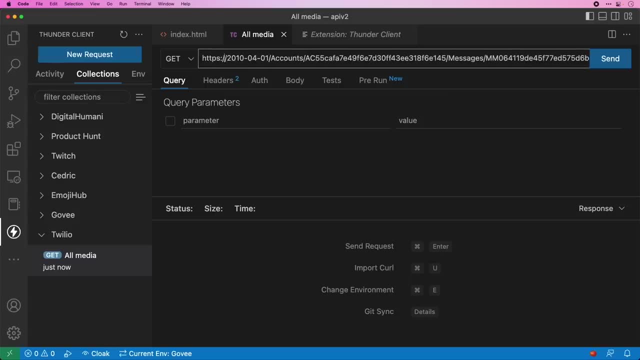 Uh, let's know, we're gonna do all media, all media for a specific message, right, Uh? so here we go. I'm going to paste that URL in here And of course it's missing that first part, which was: uh, apitwiliocom. 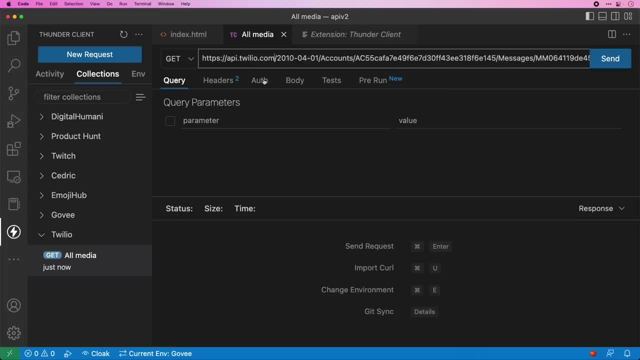 Uh, so again, this is the going for that account. to those messages: Um, I'm going to look here at where it says off. So it says inherit authentication values from parent. This is a very nice thing. This is something that postman has to. uh, that rest Fox doesn't necessarily have. 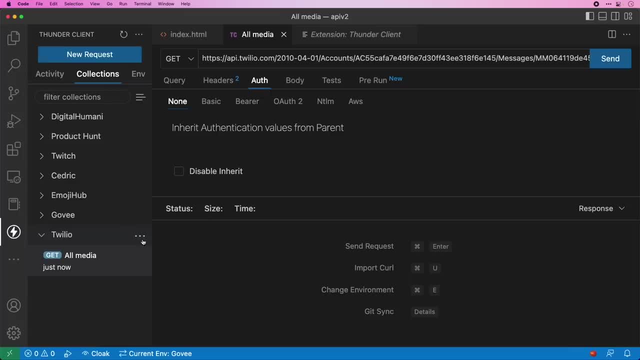 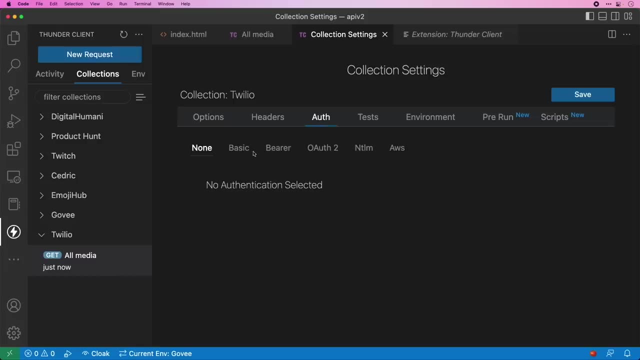 Uh, we put this in. It's kind of similar, uh, but you can make for this collection that we built, we can actually do the settings for the collection And if I come in here I can set the auth up here. so I could do this basic auth here. 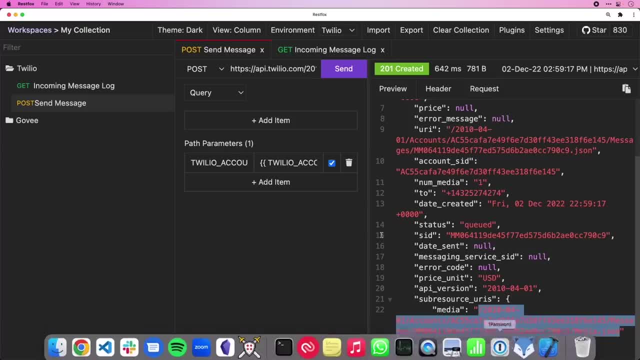 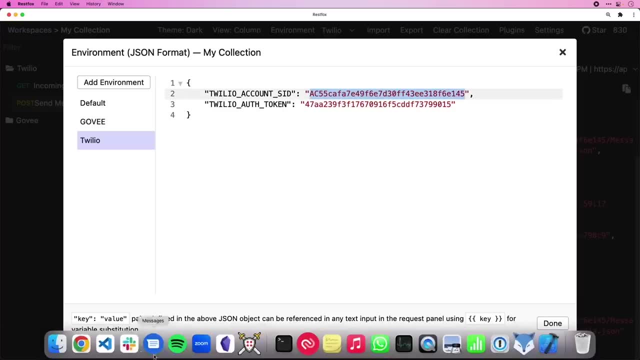 and uh, go grab my stuff. And so just a reminder, in rest, Fox, uh, when we did that before, we were in the environment of Twilio and I was able to grab, uh, the Twilio account Sid, right, So let's go. uh, let's go back to our code here, and the Twilio account Sid is the username. 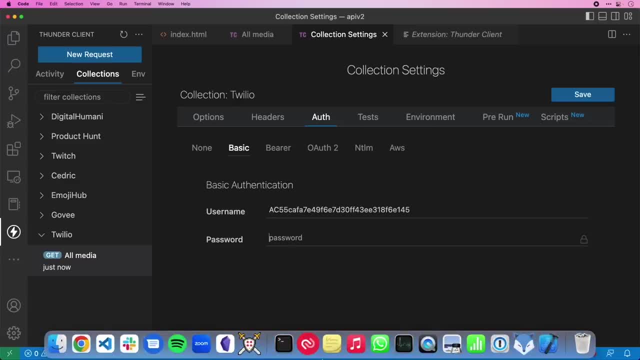 and the password. Let's go back to uh that environment and rest Fox, Uh, the password. is that off? Okay, There we go. We'll paste that there. Perfect, So I'm going to click save on this. And so now this all media should work. 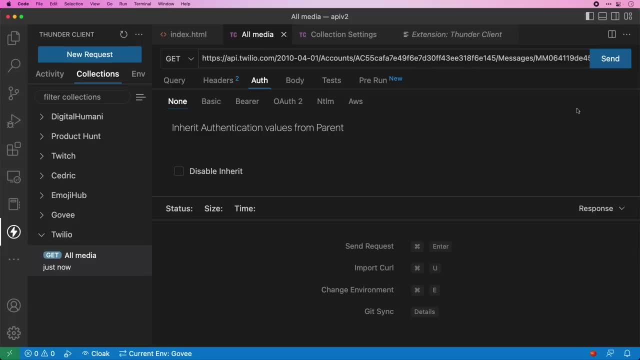 So I'm going to go ahead, I'm going to do a send to this and there we go, We got it back and we can see: uh, um, there's a media list, is the key here, And again, it's an array of those. 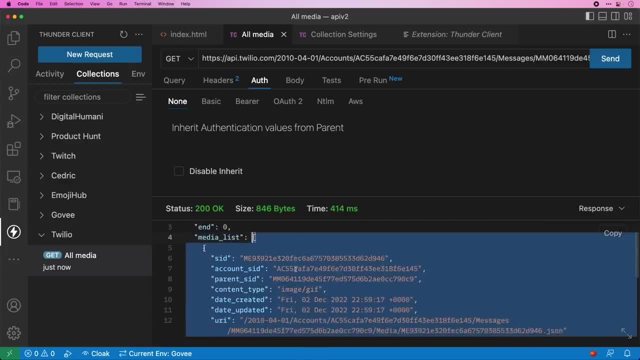 And this is the list of all of the media that's available. And so now look at this. This is the list of all of the media that's available. Okay, Look at this collection. So we have a collection of accounts and here's a specific account. 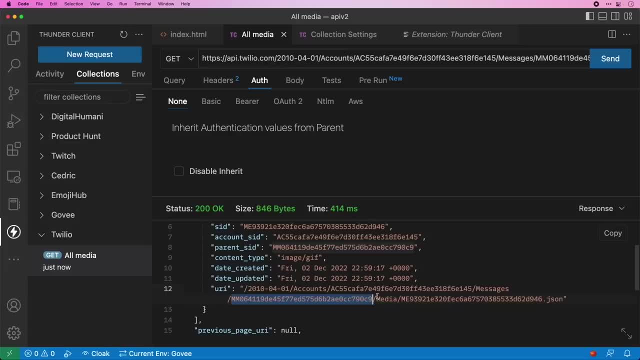 We have a collection of that account has messages. Uh, that uh message has media, and that media has an entry, a media entry, and that's it. This is what we're looking at right here, So something that's pretty cool. the way that this works is: if I get this, I can get some metadata. 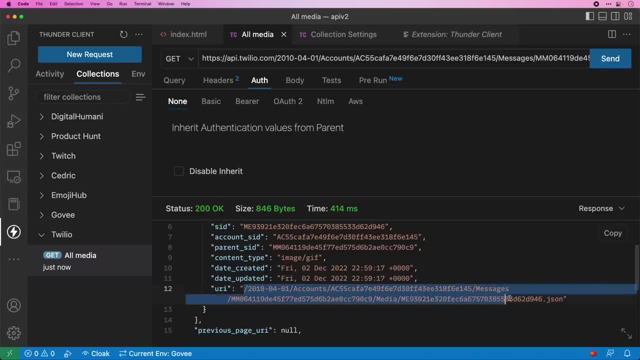 information about it. but if I get just a little bit of it, if I just go ahead and take this the way that, the way that Twilio works and not not all API APIs do this- but if I do this without the extension here, I'll actually get. 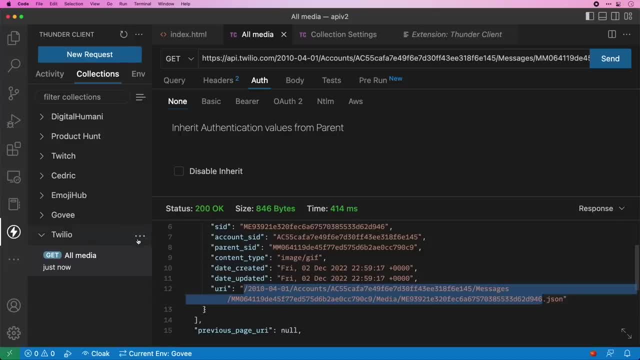 Back the picture that I sent. So I'm going to do that. I'm gonna make a new, a new little request here. So a new request And uh, we're going to call this. uh, get the pick right. 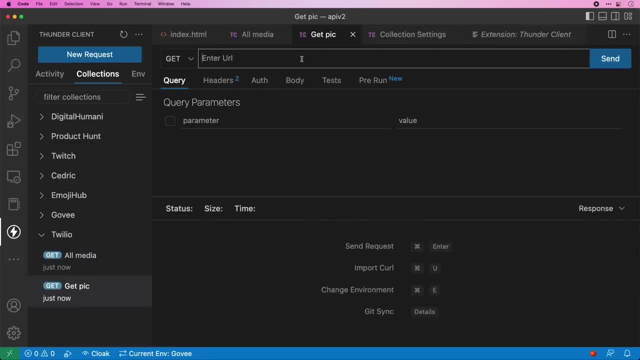 We're going to get that pick that I sent, Cause we don't still don't know what that pick was. What was it? Let's go take a look. So, um, so, again at the end of this: uh, oops, sorry. 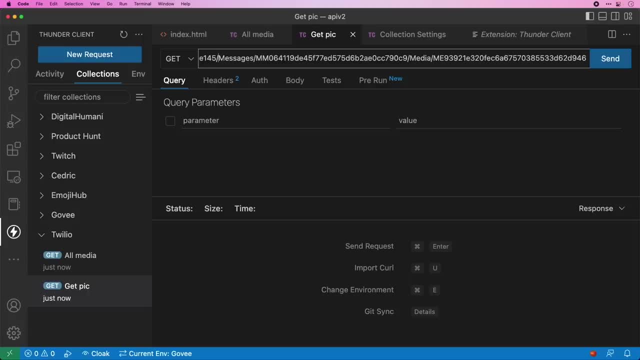 At the at the end of this there is no extension right, So I got rid of the dot JSON extension. I'm going to put at the front here: HPS, uh, API, Twiliocom and uh. the interesting thing about this is this pick is not authenticated. 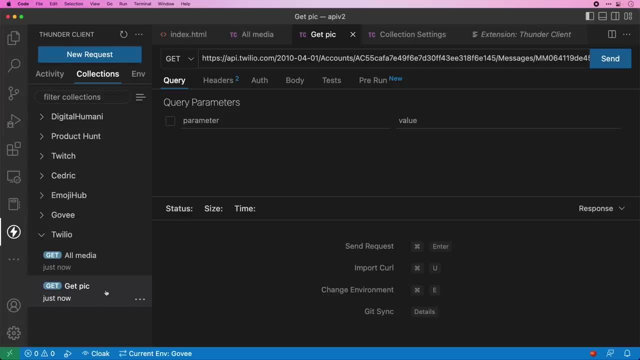 And if you do authenticate, you end up actually having some problems. So I'm going to tell this request specifically to not inherit values. So I'm going to disable this so that it's not authenticated. So when I click this, if all goes well, we should see the pick that I submitted. 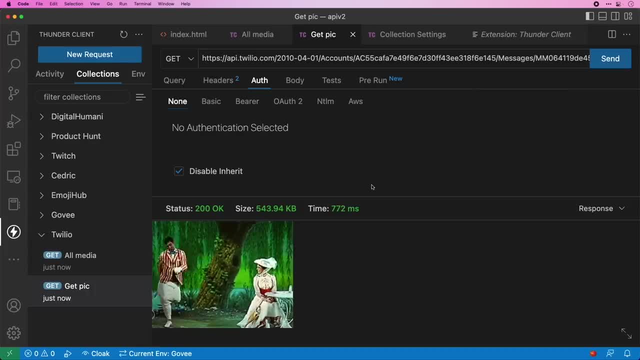 Awesome And we do uh, cool. So, um, it's a little big. it's a little big of a pick. um, that was sent here. Um and uh, we could take a look at some stuff here. 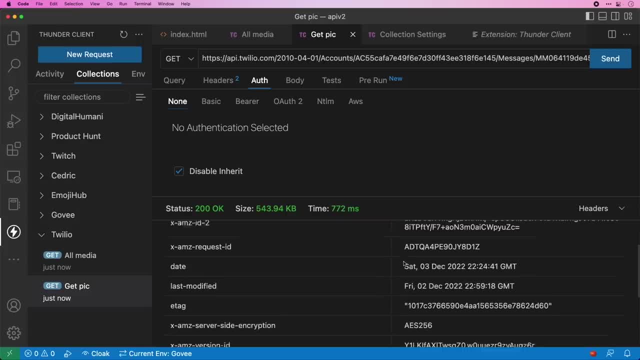 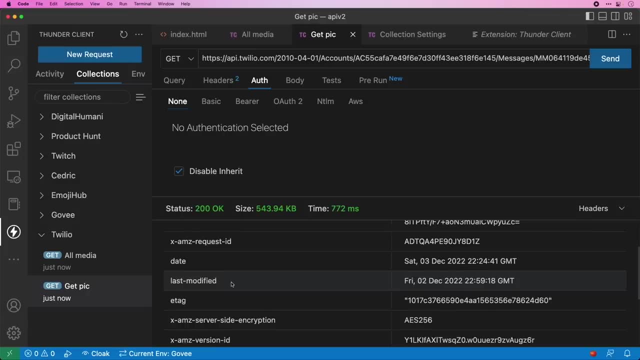 We could look at the headers that were sent, So we can see a couple of things. One of the things that I think is really interesting is when it says last modified, So, uh, the last modified date. if you have a request that has this on it, it means that you can use caching. 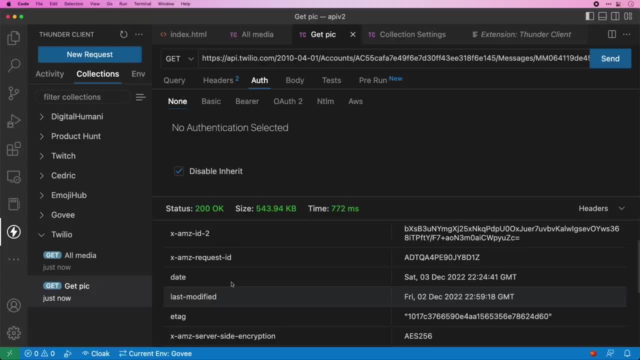 So you can uh, when you make the request, you can actually say if it's been modified since this time, uh, do it. So I'm going to do that, I'm going to grab this Let's. let's just take a look and see what that does. 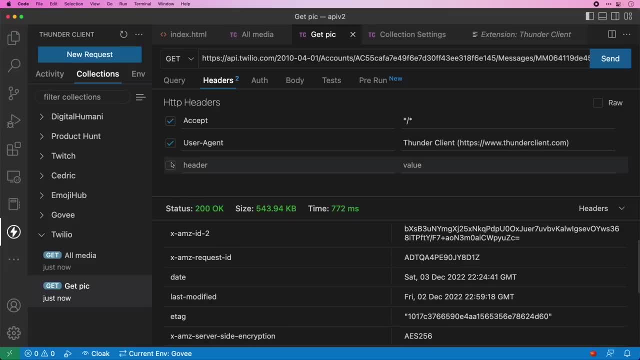 So I'm going to go to headers here and I'm going to put a new header in here Of uh, if, and you can see that there's auto-complete, So it's if modified since. so, again, this is the request that I am making. 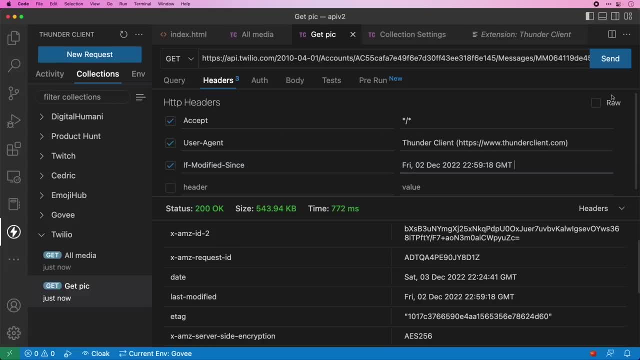 I'm making this request and I'm going to say if it's been modified since then, uh, uh, give me an, otherwise, uh, let me know. And so the way that it lets you know, um is three Oh four, not modified. 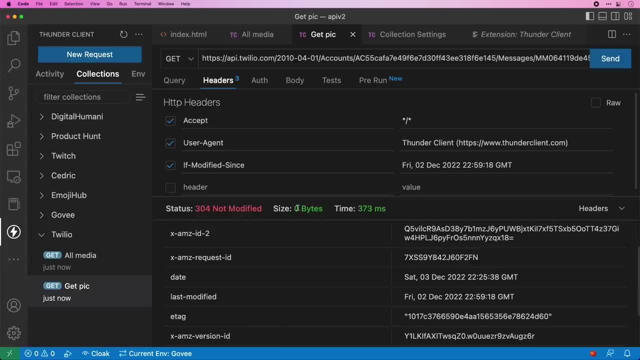 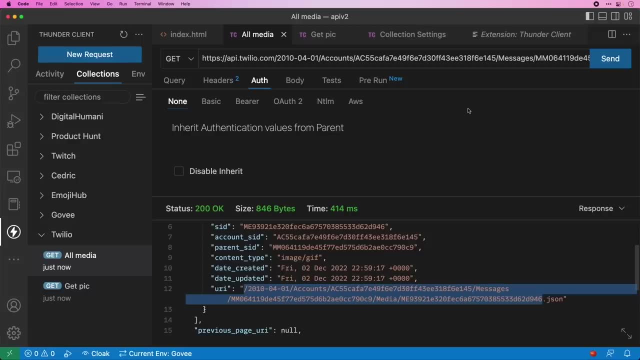 So that's a status, and you'll see that I got zero bites back. So that is how caching works, um, and what you can do to to send this across. So so this is really powerful, Right. I didn't need to set up all the other things and it's kind of really a quick little. uh, look at this. 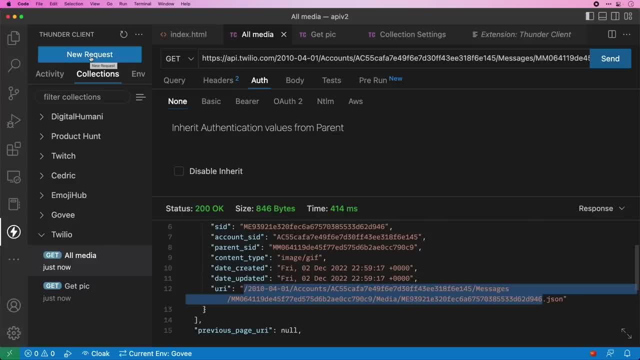 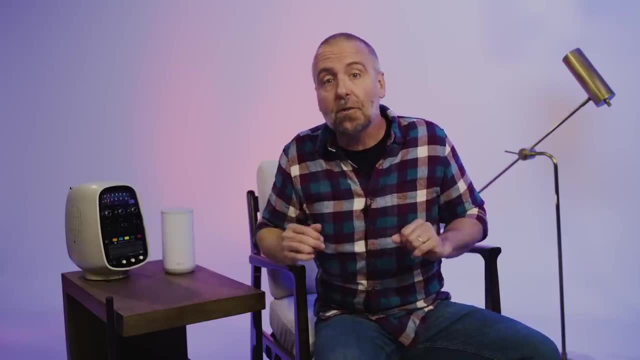 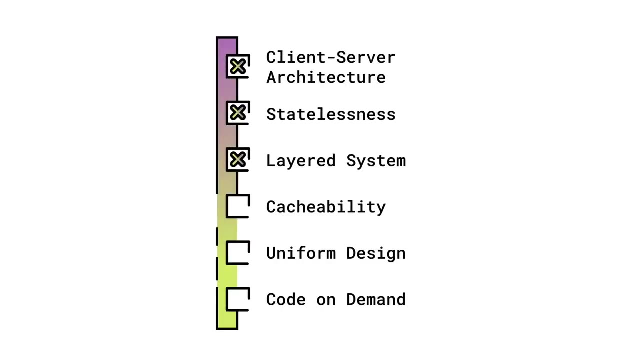 I don't actually even need to do a collection. I can just do a new request outside of it And I kind of explore through and see how these things are working, which ding ding ding means we covered another part of a restful API constraint scavenger hunt using standard HTTP caching mechanisms like last modified and e-tags. a restful API should support caching. 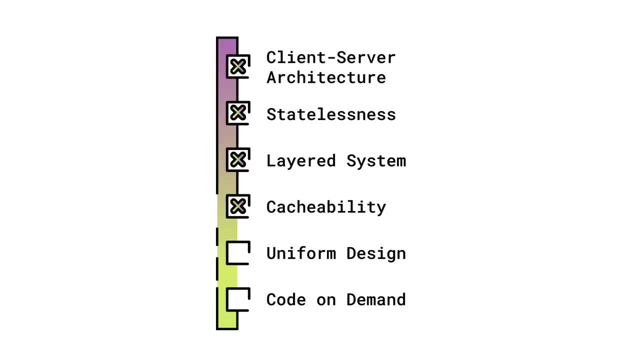 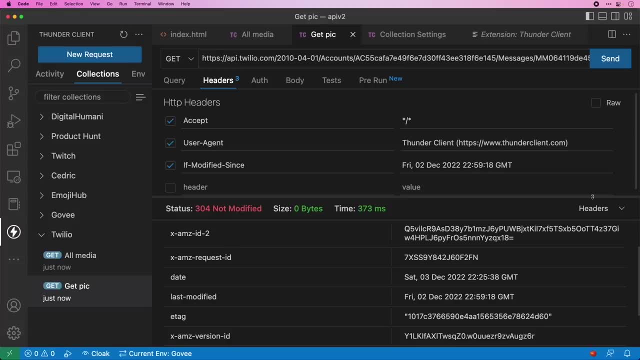 It's up to you to maintain the cache on your client and decorate your crests, but this can come in Really handy to avoid making unneeded requests. And those are the postman ask things I wanted you to see. they wanted you to be able to do that without diving in necessarily to do all of the postman enterprise, uh, things that you want to do. but I think it's time. 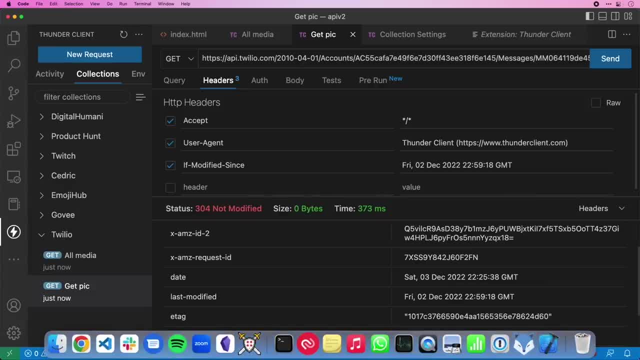 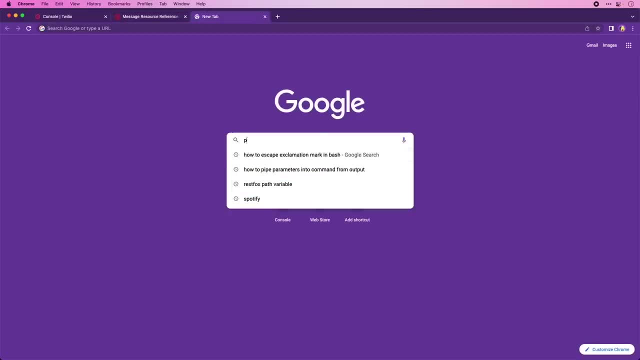 I think you should feel comfortable enough that we can now look at postman and see what we've already learned there. So I'm going to go, uh here and I'm going to just do a quick, quick little Google search for postman. 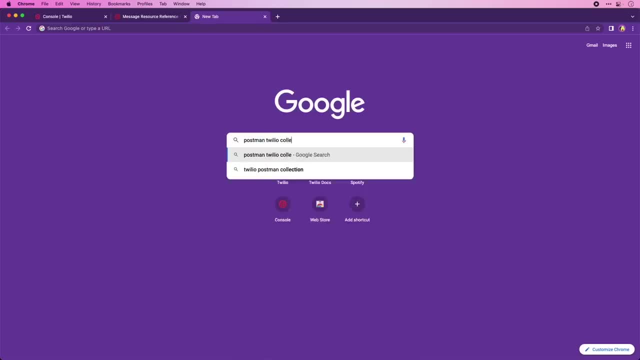 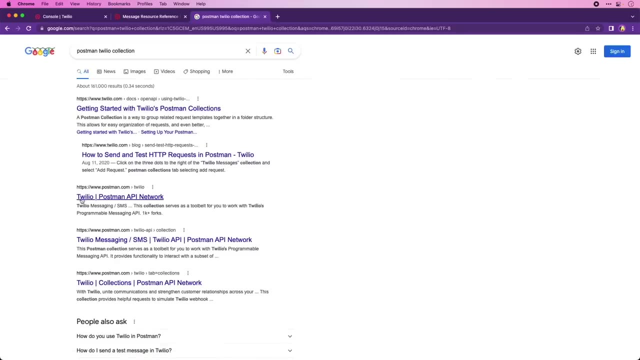 Um, and this is really nice. You can do this for Whatever API you're working with, And since we're working with polio, I'm going to search for the postman Twilio collection, Um, so there's some docs on Twilio about it, but if you look here, there's this Twilio postman on the API network. 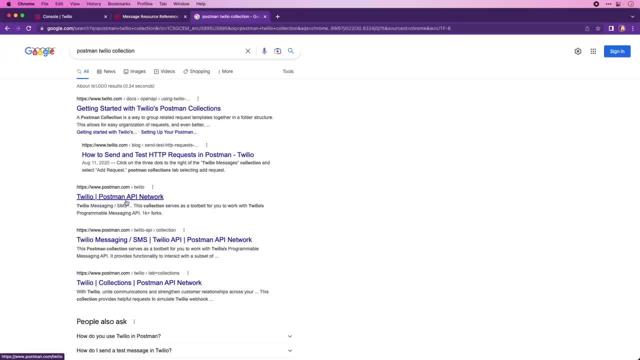 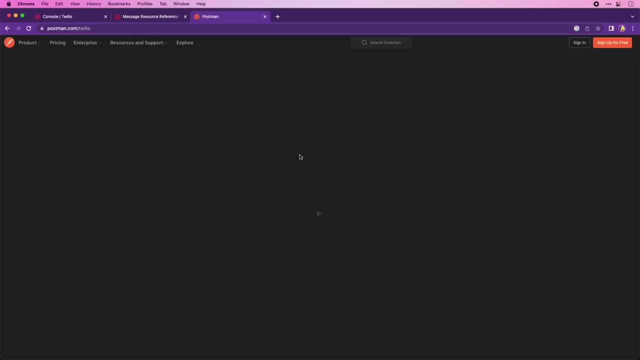 So this is important to know. There's a lot of uh uh things on this API network where they've built uh APIs for you to go and share, So I'm going to click this and now note I'm inside of a web browser. 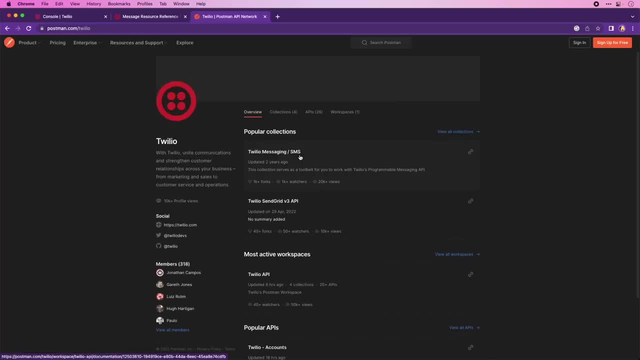 Postman has done a really gorgeous job of uh of letting you run inside of your browser. You also can run it locally, like we did with rest box, Um, but I'm going to run this from my browser, So I'm going to go into this messaging SMS, uh, and you can see there's all sorts of different things, uh in here. 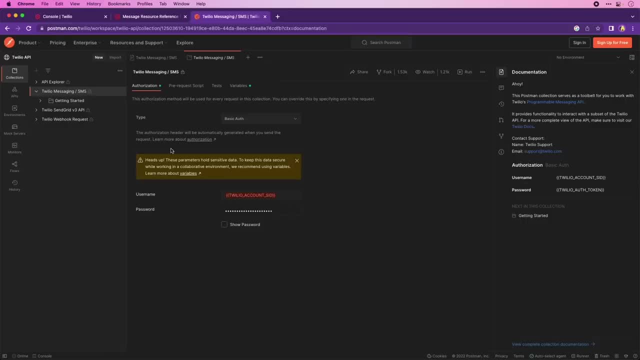 Uh, it's a little bit hard to get to here, but you could change things, put in your account, sit and and all sorts of things like we saw. Look, here's the double mustaches, right, And here's a thing to send an SMS. 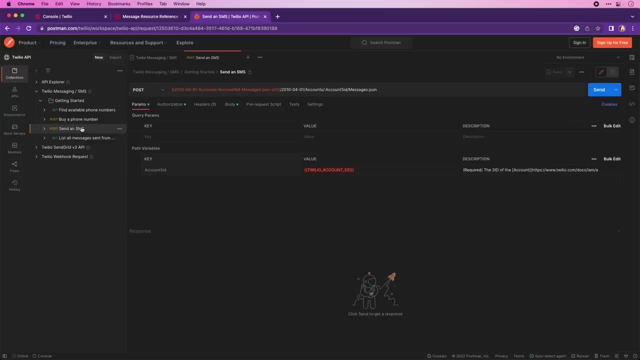 Um, and it's, it's super cool, Um, it, it's, it's neat, right? And so you've seen this. here's your authorization: the headers, the body, there's collections and, uh, what's cool. 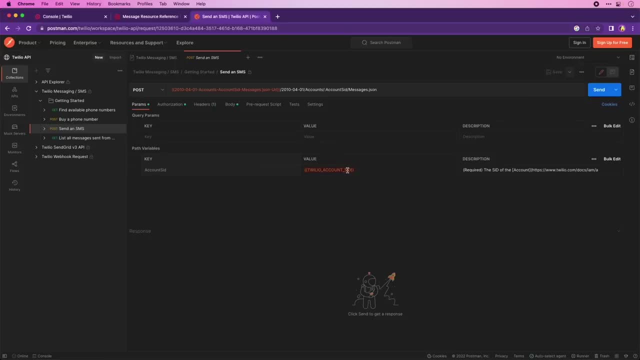 If somebody's already built these collections for you and they're sharing your stuff this way, right, So that's kind of. that's kind of nice. So there again, there's path variables, right, And the path variables coming up. here there's the. the colon account said that you saw uh from before. here somebody is using this as the start, uh, the HTTPS, uh, API, Twiliocom, and it's doing a post, right. 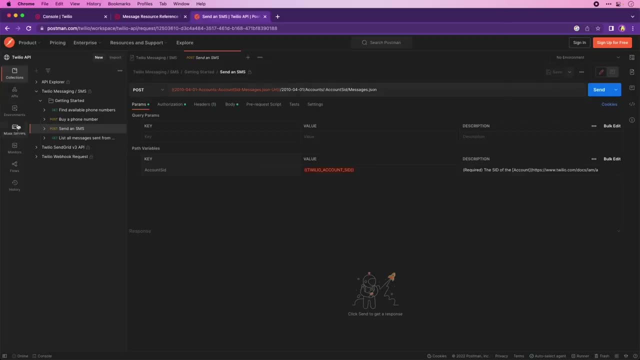 So it feels very similar. So you're you're familiar with this. There's also a bunch of other things over here that it can do that could get a little bit distracting, And that's what I was trying to kind of avoid. Uh um, cause I wanted you to to get. 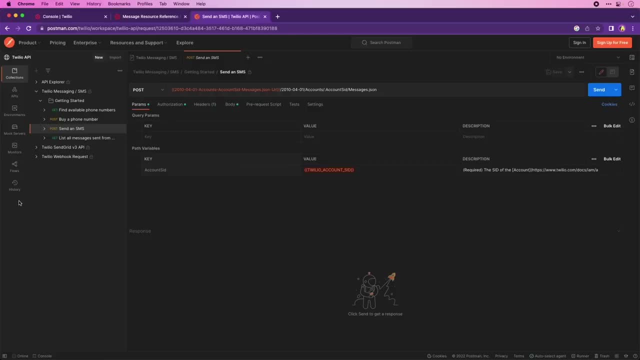 Get familiar with it but know that this exists. Um, one of the really cool things that postman does is if you click over here, on this far right over here, there's this little uh code. it's like open and close tag. 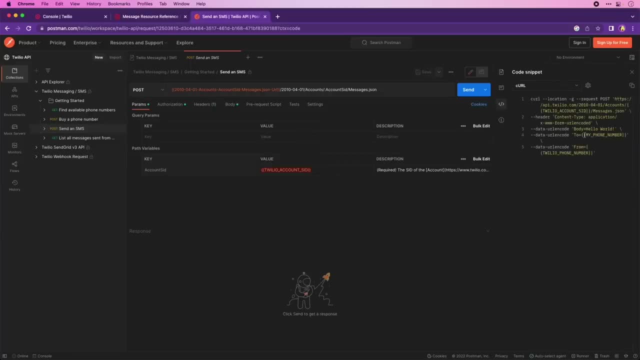 This is really neat. So, um, we have curl right, So we could see, this is how I would go ahead and do this And this. this feels familiar, right? This is how what we actually did, We did this curl statement, but check this out. 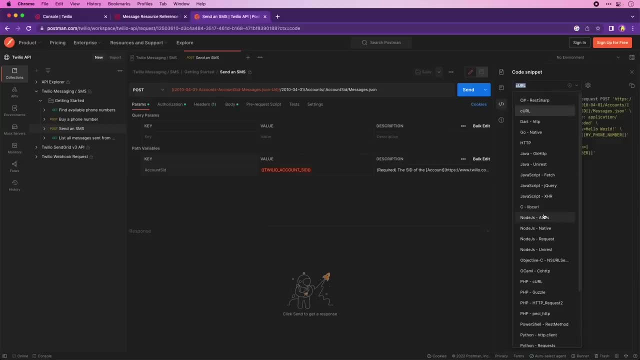 You can do this in any programming language. So the trick here, the trick to remember, is that any programming language that can make an HTTP request Like it has a client built. It has an API built into it, because these are all standard, the rest API right. 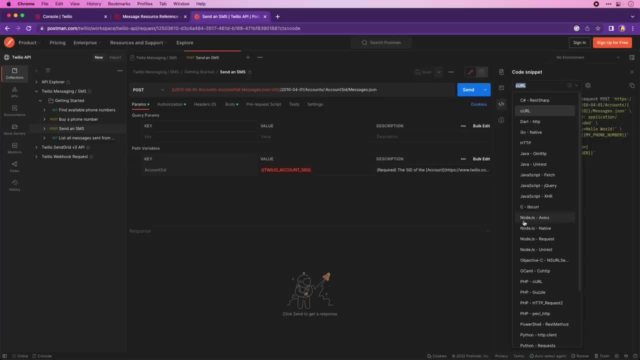 We're following these constraints that have been defined. It can generate code for you. So here's no JS using a package called Axios. So Axios allows you to fetch things. So this is what it would look like if you tried to write that using Axios. 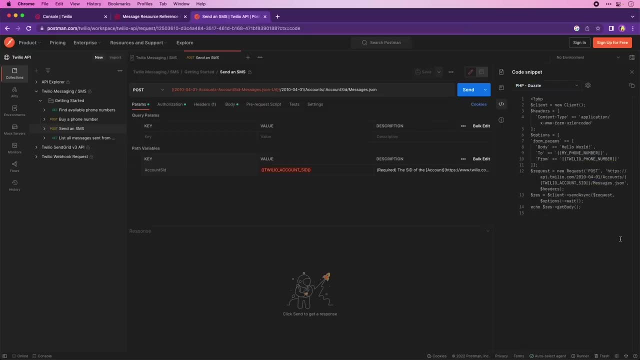 Um, and if you look in here, you come down here. here it is in a PHP with with guzzle. I don't. I don't know what guzzle is. I like that, though I. that's why I chose it. 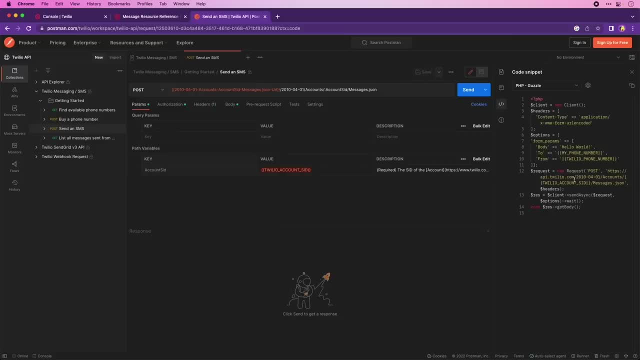 Um, so you can see that it's generating this code for you, And If I pasted it into my PHP code or my Python code or my Java code, it would just work, And that's really handy. That is, the company that's providing the API doesn't have a helper library or an SDK, a software development kit, which we haven't looked at yet, but we're about ready to um. Twilio does have one of those. 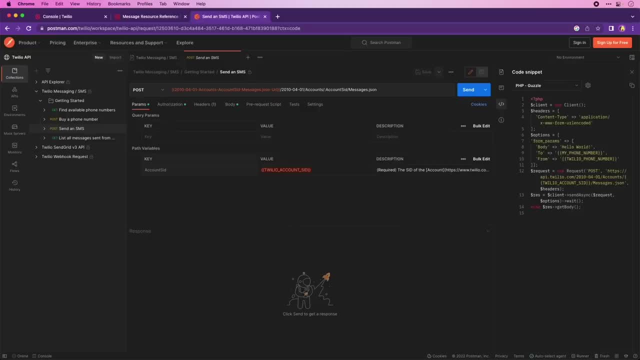 But if you were looking at one of these that that didn't, this is a great way to get that code. Um, so, again, check out the API network. uh, this Postman API network. It's cool. I think you're ready now, uh, to use this if you want to, but also feel free to use 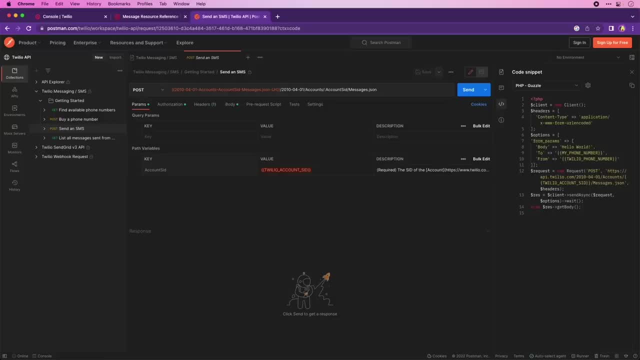 The other tools. explore the APIs in the in a in a comfortable way, wherever you might be uh uh most comfortable with Cause there's all sorts of really fancy uh tools here on Postman And, like I said, there are courses on how to take full use of all of the things that are available. 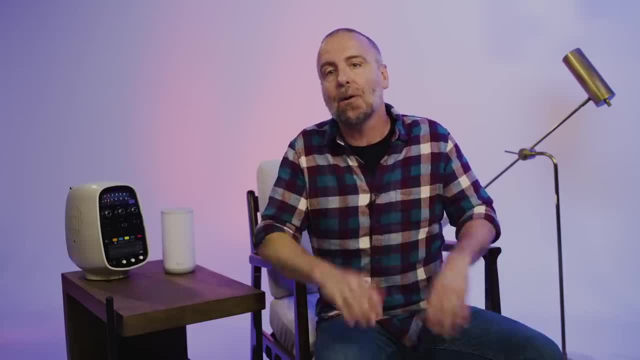 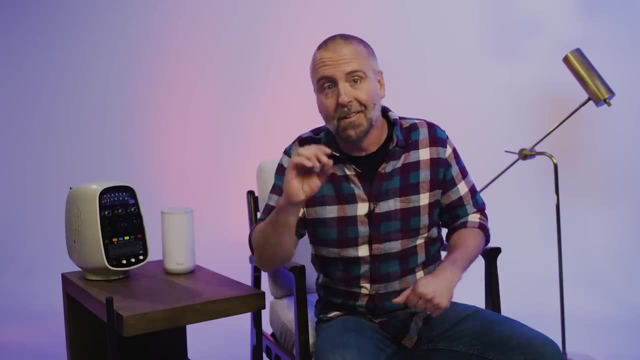 Awesome job diving into all those tools. Postman is a super powerful tool and it keeps getting better every day. There are so many features that we didn't cover. We barely even scratched the surface. There's an entire course out there on it. 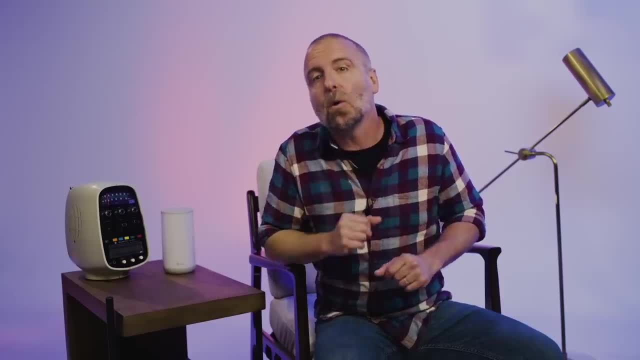 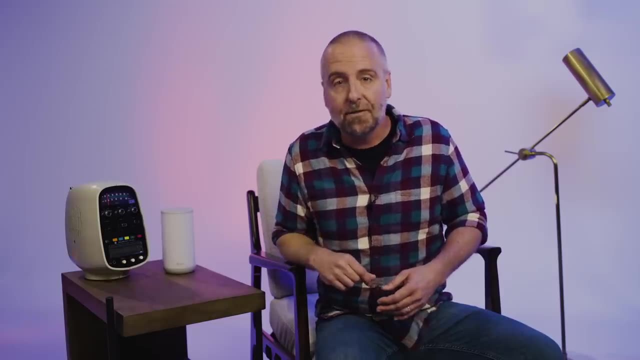 Check the notes for where to see that We saw how to organize our requests together into collections, as well as share common and secure values by using variables. We learned how to add different values to requests, both in form values, query strings and headers. 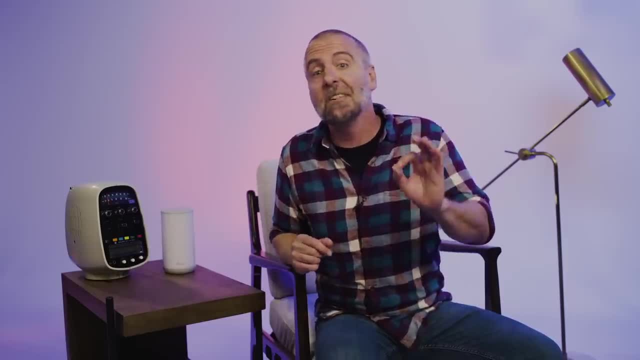 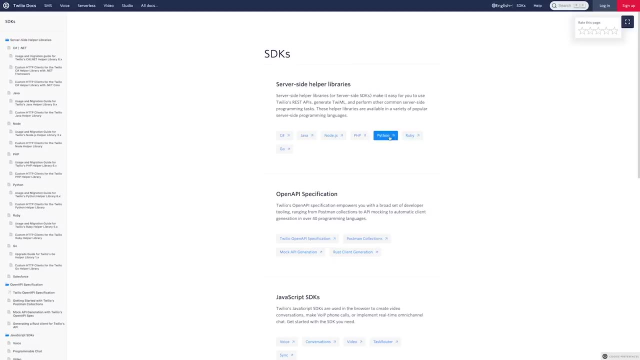 And we also saw how to navigate through various sub resources via clicking URLs. We even saw how to create actual runnable code from your request. While we were in the Twilio documentation, you might've noticed the code examples on the screen. On that page, it's possible to tab between various language implementations. 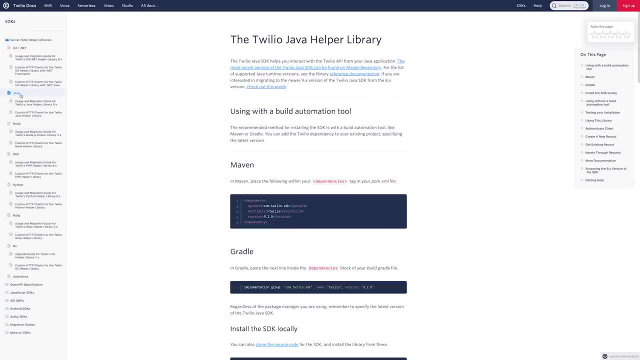 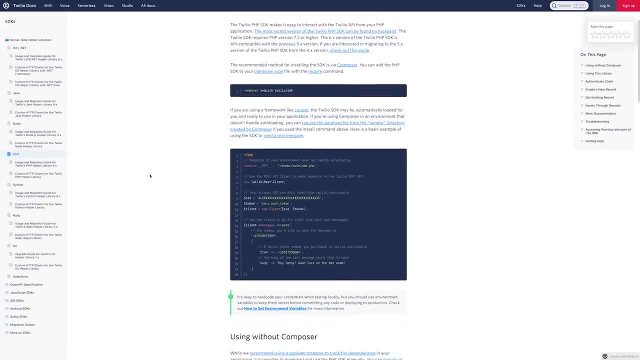 Many products offer what is known as an SDK or software development kit or helper library. that allows you to interact with their product in your native language. As you can see, it abstracts away the REST API completely. Let's take a look at the Twilio Helper Library next. 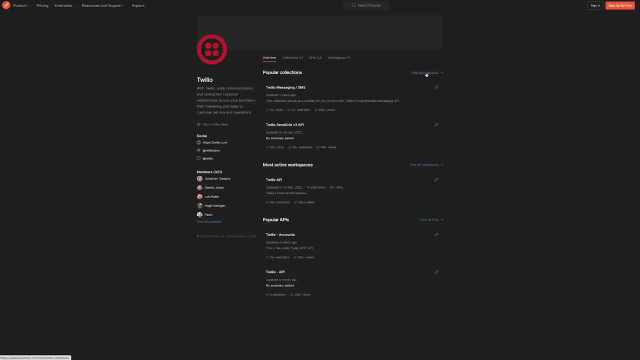 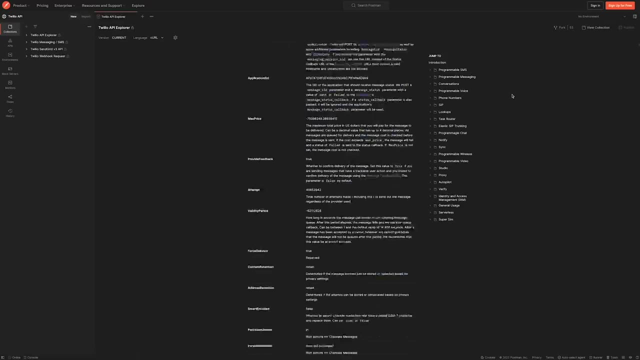 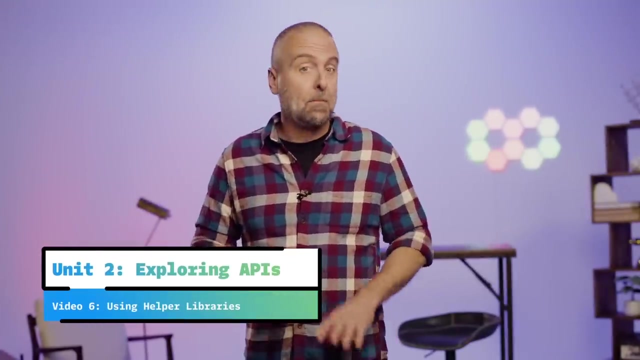 Before that, though, just a quick reminder to make sure that you check the notes on this video. There's a link to a repository of built out collections that are ready for you to use. There are lots of great APIs to practice with. All the tools that we just looked at are great for accessing and exploring APIs. 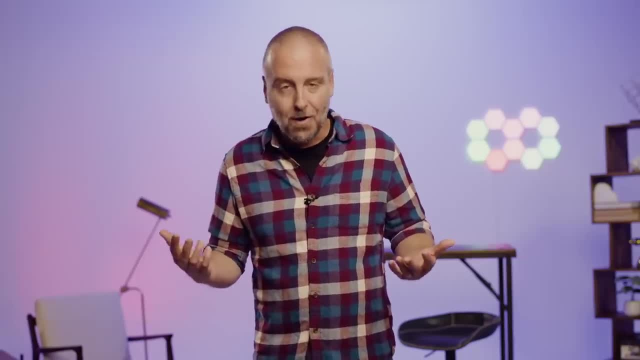 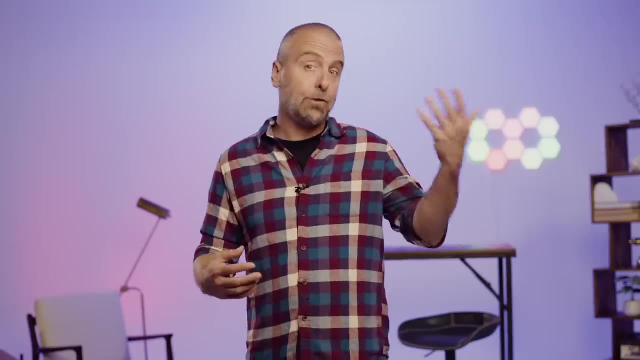 However, when it comes time, you're most likely going to want to write some code. Now, as we saw in Postman, you can actually generate code. All programming languages have some sort of way of making HTTP requests And, as you know, HTTP requests are all we really need to interact with REST APIs. 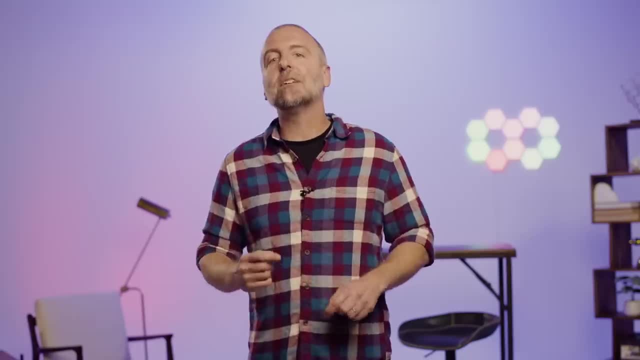 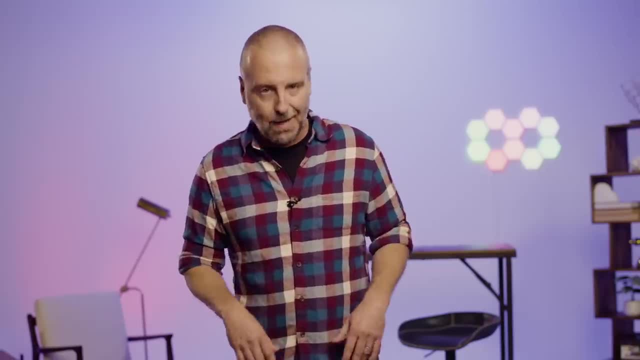 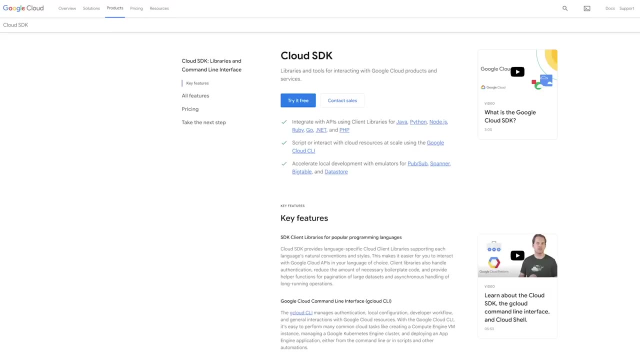 And that's a code that is repetitive and almost always the same, just with a few tweaks. Many products and services have created a solution to help you avoid this problem. They're often called helper libraries or SDKs- software development kits. They'll be specific to your programming language. 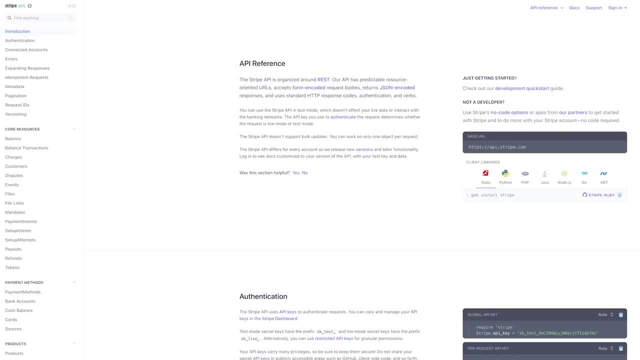 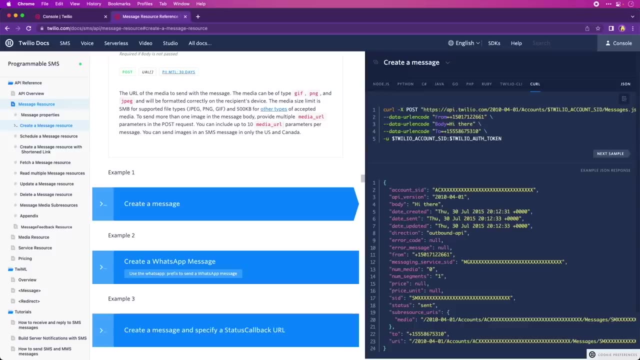 These libraries help make your code more concise and legible. They usually also provide additional documentation for your editor, which I find super handy. Let's go check out some of these helper libraries. Okay, so let's take a look at one of these helper libraries. 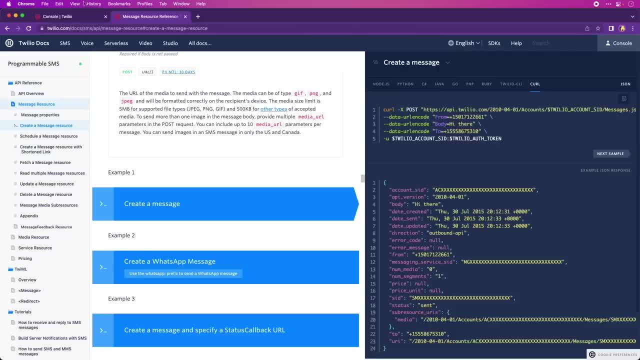 Let's take a look at the first one That's here. So again I'm in the docs: SMS: create a message resource. I'm here under the cURL tab currently. Remember, we did this, We went and we saw how to do this. 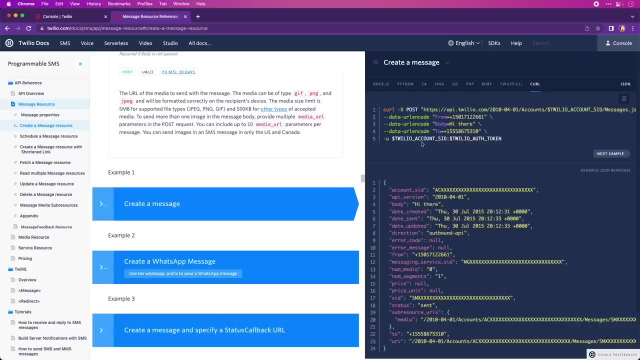 We passed the from the body and the to. We passed in these environment variables. That's what this dollar is And this dollar or Twilio auth token. they're environment variables And it's also used here in the URL, So we had done that. 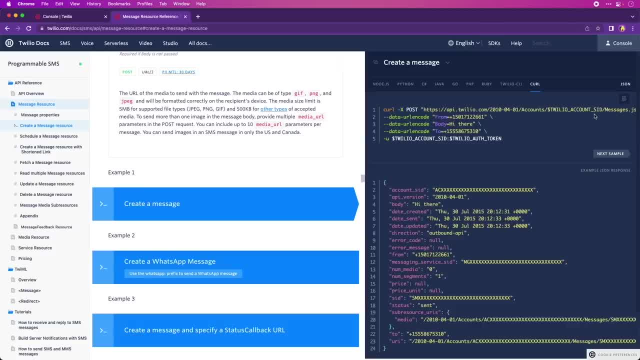 We had done that with cURL. Now, one of the really nice things about these helper libraries is they look very similar, but it's taken away this whole notion, So let's go here. I'm going to go to this nodejs. 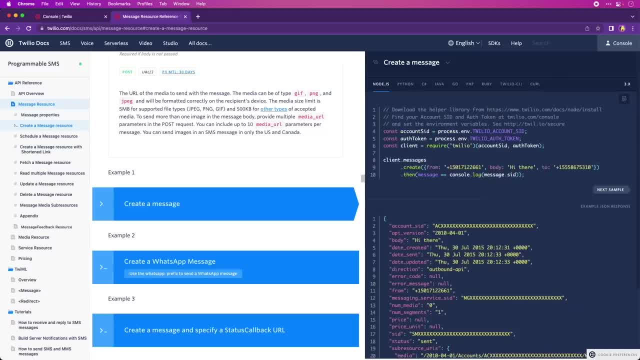 Now quick word of warning: If JavaScript is new to you, there is some stuff here that might be a little confusing, And I want this to just kind of wash over you. I want you to more feel what it feels like as I explain it. 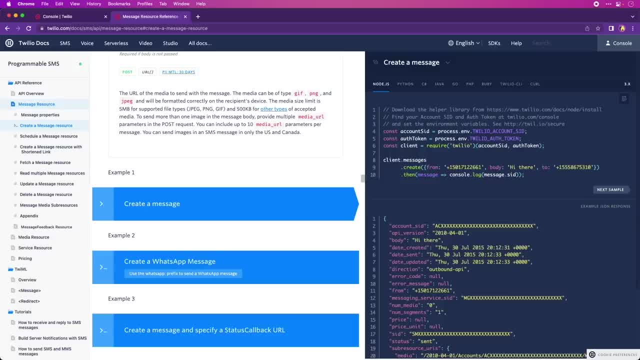 And don't be too concerned with not exactly understanding all of the things that can happen, especially if you're one of the folks who has the hello world requirement. Please don't feel like you need to fully understand all this. I will walk through this. 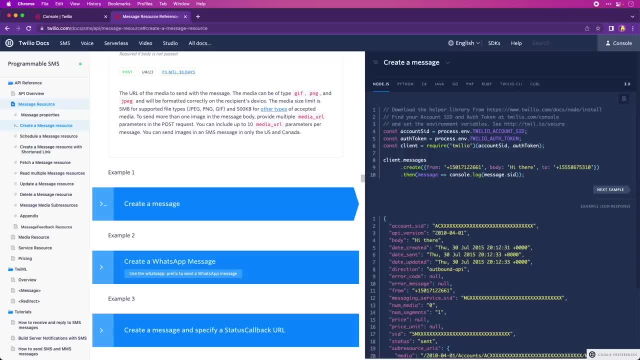 This code, line by line, and tell you what it's doing, And it will be familiar to what we've been doing, just in a programming language that you might not yet be familiar with. So I'll take my time and you take your time. Give yourself some patience. 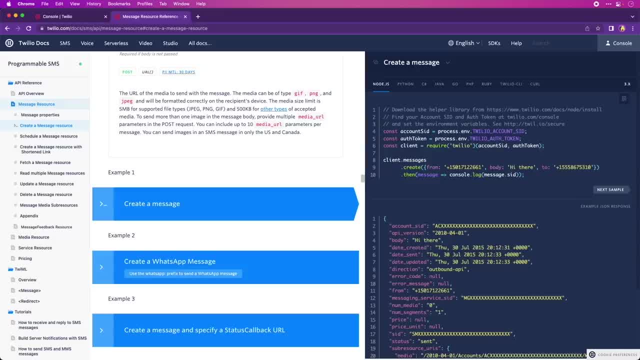 In fact, I'd like to suggest that if you are in the boat where you have not written code like this before that, you watch me first and then come back and do it later. We're going to take advantage of the fact that we're in a video, right? 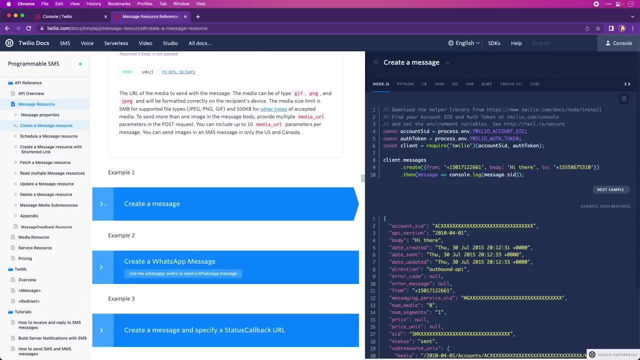 You can take me right back to right here. Take me back to right here. Let me get started. So one of the things that I love about Twilio's documentation is that you can just copy it and it should work. So this is what was happening. 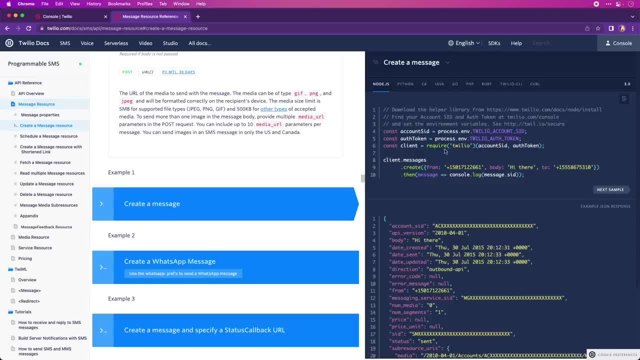 when we created something here, right, So we created a message. So this is: you get this authenticated client right. We know what that is. We authenticate with our client with our account SID and our auth token, like we've been doing. 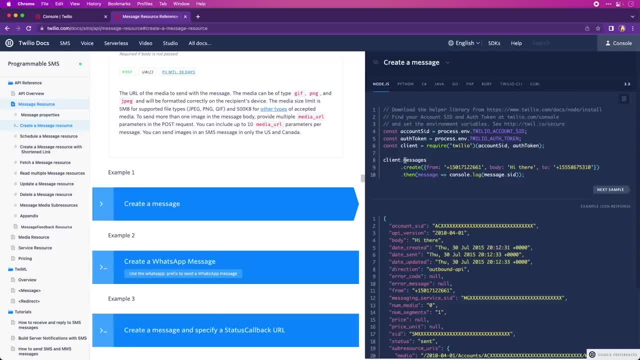 And then we're going to do this: messages a client, so clientmessages. There's our rest clientmessagescreate And we're going to pass in the from the body and the to, and it's got all the information that we know. 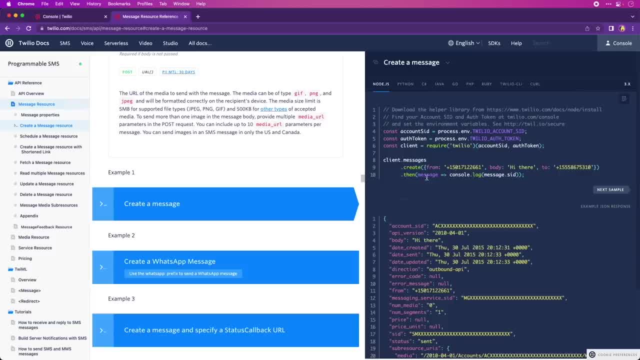 And then there's doing some of this JavaScript stuff. So then we're going to get a promise back and then we're going to get access to the message And this console log is going to print out to the screen. I don't think we should send a message. 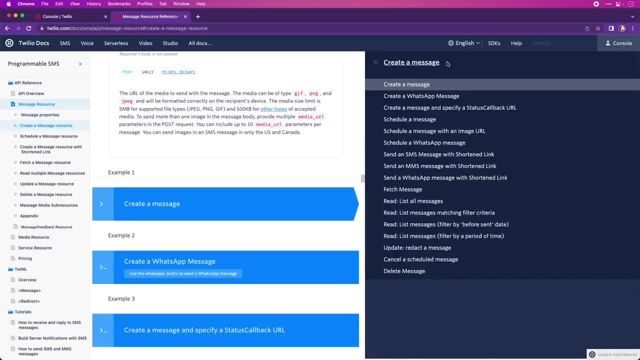 Why don't we look at the messages that we've done? Let's do that. So I'm going to go to that example. So I'm going to choose down here this list: all messages, Awesome. So we'll take a look at all of the messages. 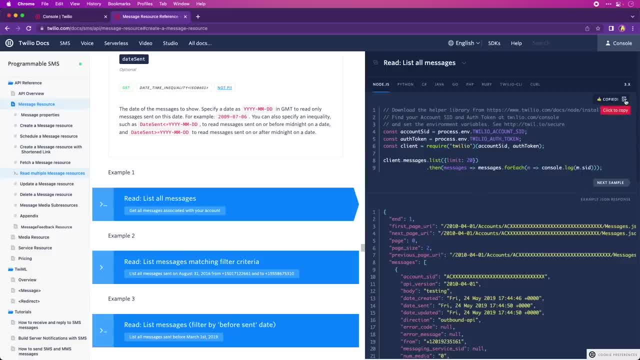 that are in the account. Now what I can do is I can just copy this. So I'm going to copy this and I'm going to run it on my local machine. Now I'm just exploring, and this probably happens as you're looking at APIs. 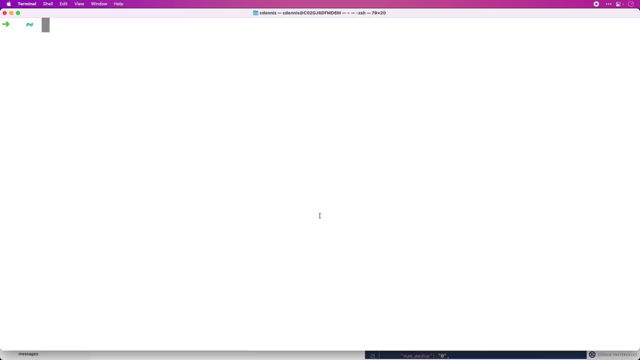 So typically I have a folder on my computer called Scratch, And if you want to make one, you do mkdir, scratch, Just kind of put this wherever you want to and then you get into that directory. If you're doing this in a terminal on Windows, 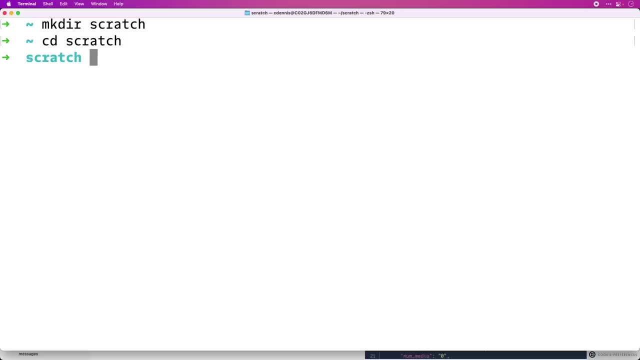 there are some instructions in the notes on how to do exactly that. So now I've got this directory named Scratch. Now I told you before I was using Visual Studio Code, which I hope that you have installed, And so I'm going to do code dot. 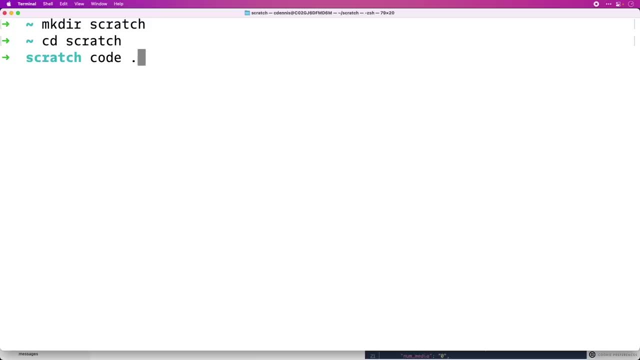 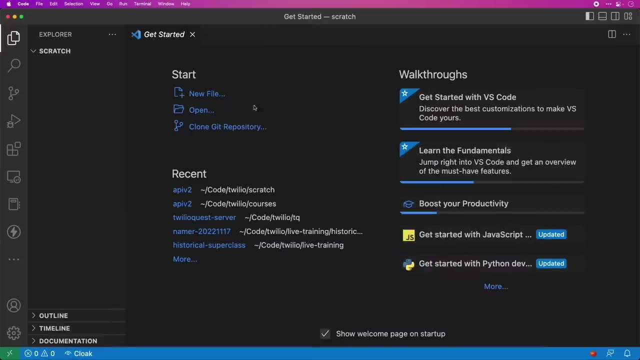 And if this doesn't work for you, there are instructions on how to get this installed properly on your machine. What it should do is pop open my Visual Studio Code directly in that directory. So I'm in this directory here and I'm going to make a new file here. 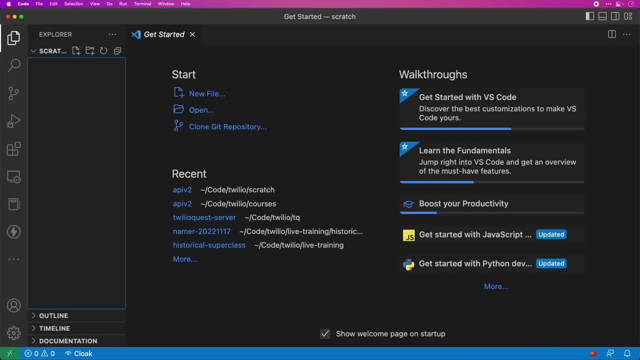 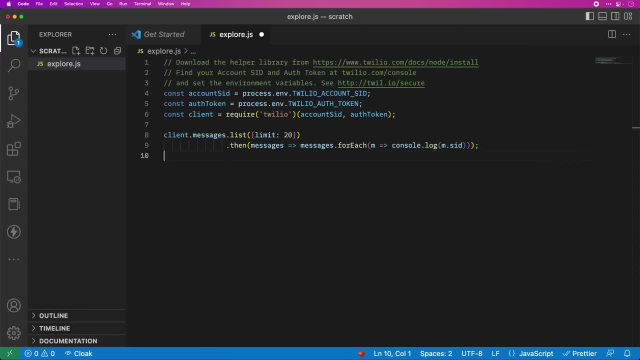 I'm going to call it explorerjs, because this is typically what I do. So I'm going to come in here and I am going to paste that code- Awesome. So now I have this code here and the code is on my local machine. 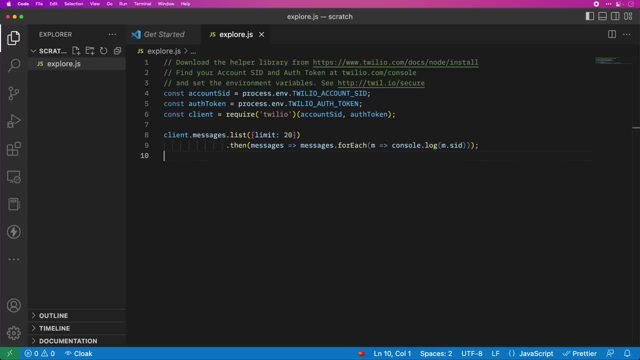 which is awesome. So now I'm going to try to make this code run. Now, one thing that I know for sure that I need to do is I need to download the helper library. So if I wanted to go here, I could go to this node install. 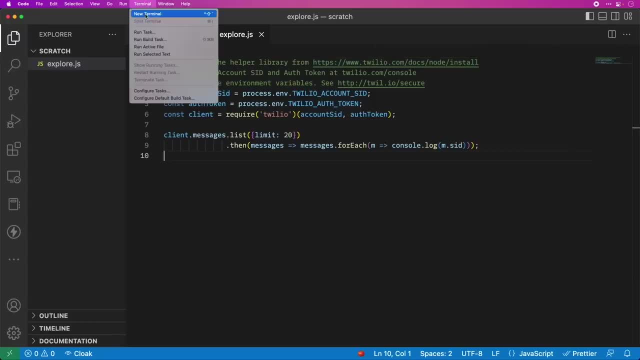 I happen to know how to do that, So I'm going to go up here under terminal and I'm going to do new terminal And in Visual Studio Code. this was really nice: My terminal can actually run the same terminal that I used to open it. 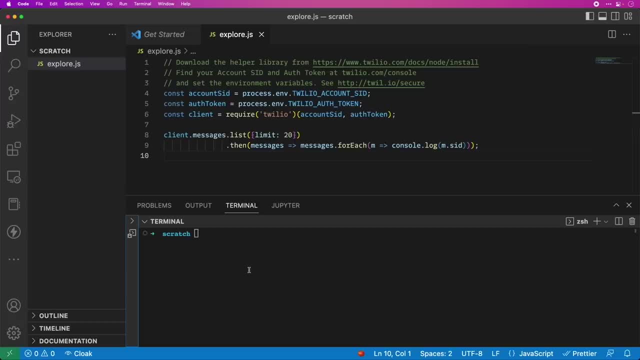 is running down here in the bottom, And what I'm going to do is I'm going to use package manager to install the Twilio helper library. So I'm going to say: npm, install Twilio. So npm is node package manager, And if you do not have this, if this does not work, 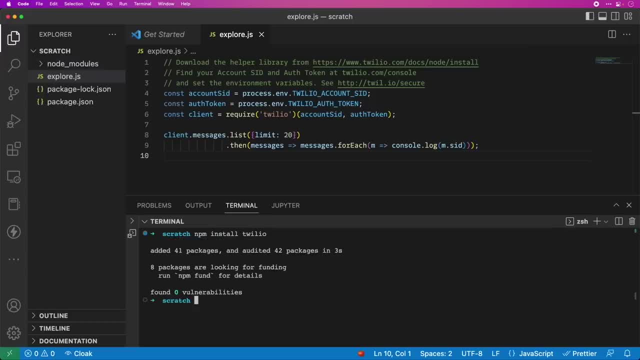 check the notes, because it means that node is probably not installed on your computer. And if node is not installed on your computer, there's a great walkthrough in the notes on how to get node installed. So I now have Twilio, a helper library, installed. 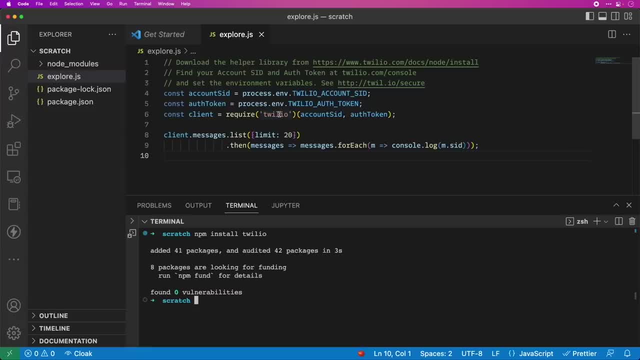 which means this require Twilio statement here is requiring that library. Remember in RestFox how there was an environment and we stored the account, SID and the auth token. we can do the same thing on our local machine. We can set up a little environment here. 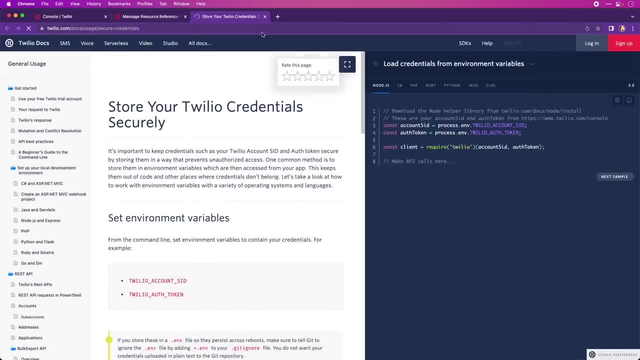 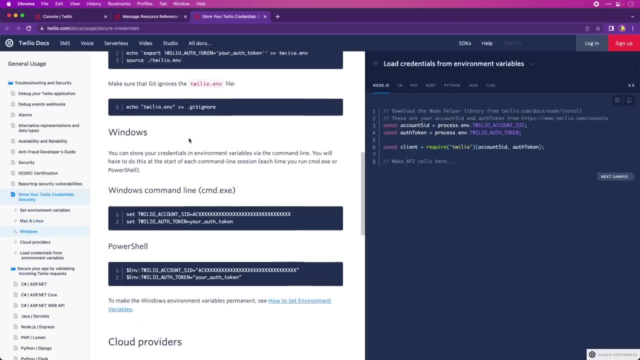 And actually, if we go ahead and we click this Twilio secure, there's some great examples in here and how you could do that. So one of the things that this is just doing, you can see it's for Mac and Linux, and different shells do different things. 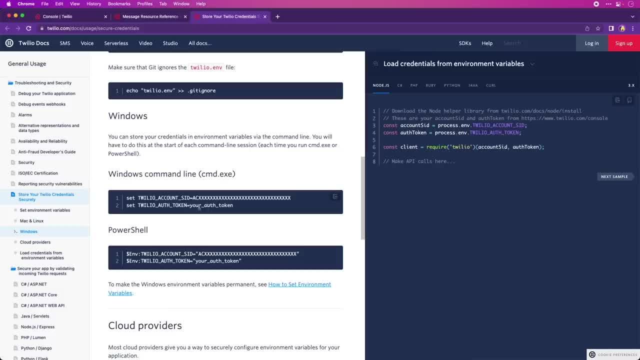 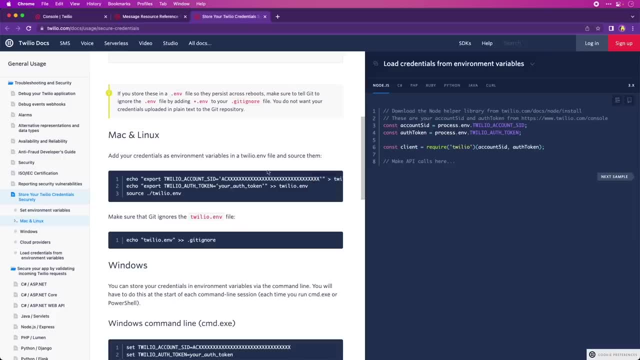 If you run this in your command line, you can set your environment variables, And then when you run node, it will work. I'm gonna do this one, So I'm gonna copy this here And I am going to just paste this. 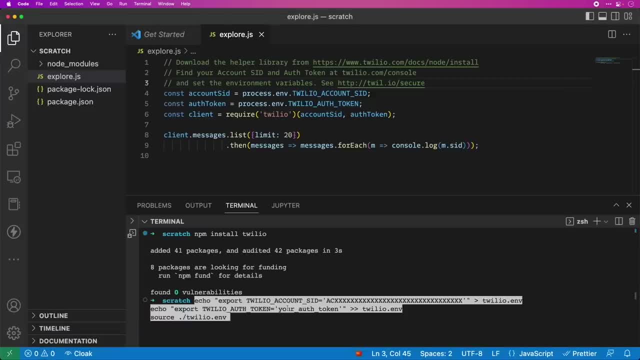 We'll paste this. I'll show you what it does. So it's saying we wanna export my account, SID and my auth token, which we're very familiar with these days. So we're gonna. We're gonna do that. Let's do this real quick. 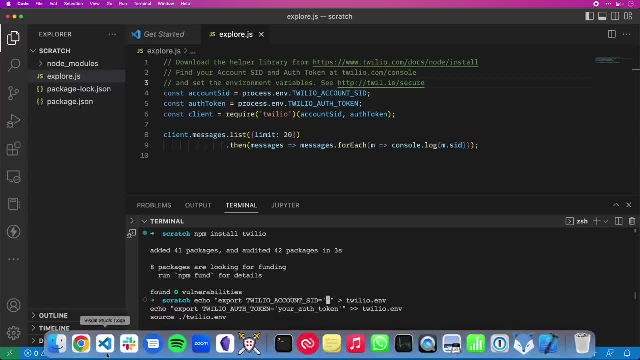 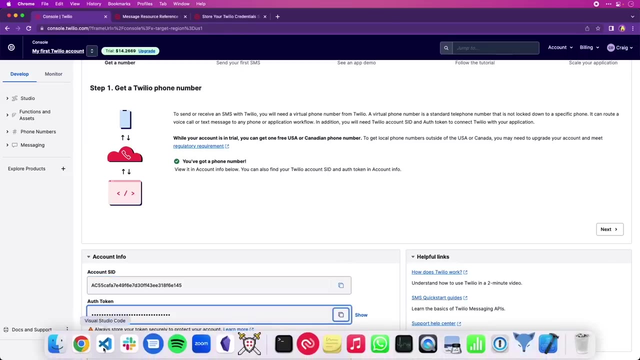 So I pop in my account token there, I'm gonna go back over to my console, scroll down and grab my account here, and then I'm gonna paste that. And I am gonna go and grab my auth token and I am going to paste that. 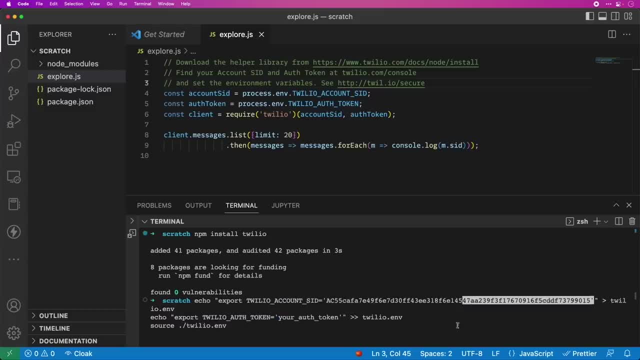 So again I got to that I accidentally pasted my auth token in the wrong way but wrong line there, so i know that it started with a four and i'm going to paste it down here. it says your auth token. so basically, what this is doing is this is writing a new file that will have this: 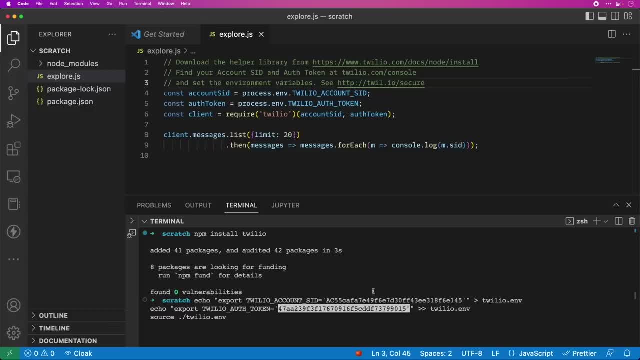 information. i'll show you that here in a second. so there's, there's my um. it's going to write these two lines. i'll show you. i'll show you what that looks like. so i'm going to- uh, it's going to create a new file called twilio inv and it's going to append that. that's what this double dash, dash. 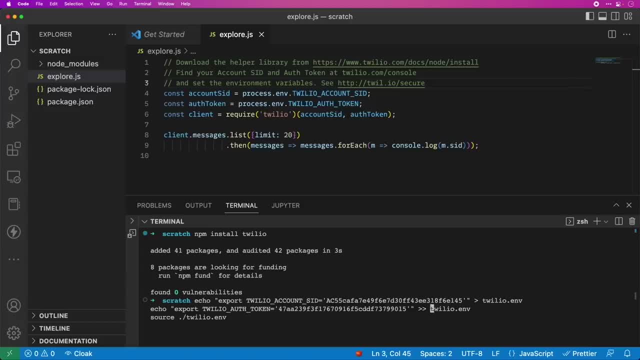 and then i'm going to source that, which means uh, put run that, uh environment variable. so uh, if all is working well now, if i say, uh, echo, and i can do twilio account sid, um, we can see that i have that available and that created this file here called twilio inv, and you can see, there is my. 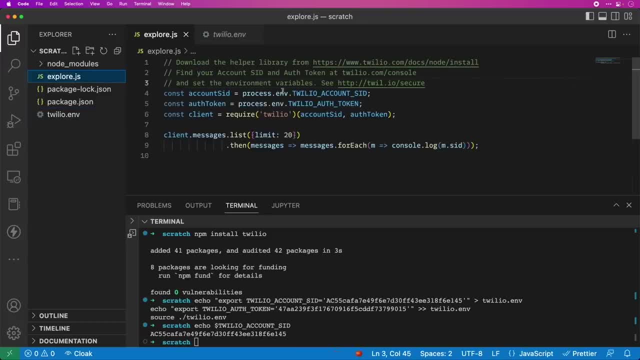 account, said in my token, which is nice, because now this code uh works, it should be working, and using this, and in fact, if all is going right, so i've. i've got node installed, i inst, i installed the helper library, um, i put my account sid from the console into this twilio inv and then i did this final command. here the source: 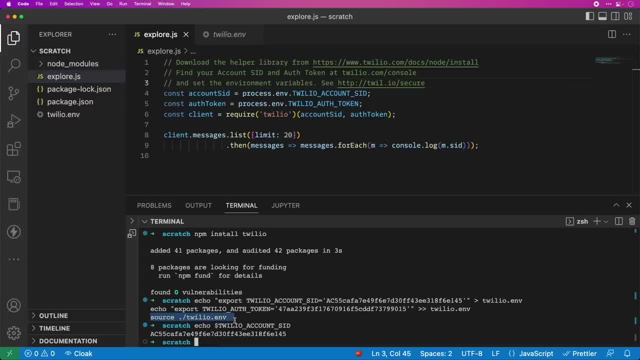 twilio inv, which will run that file and put those uh variables into my environment variables, uh, and as i showed you that they were working, so, so let's go ahead, let's do node explore. so what's going to happen? let's take a look really quick. i'll show you. let's see, let's make sure we got. 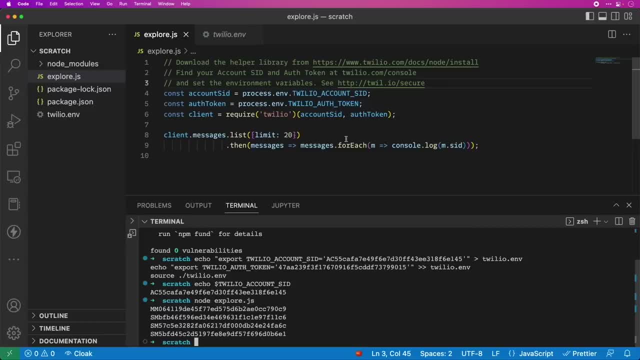 it working cool. we did so. so, uh, let's walk the code really quick. so this is pasted straight from the uh, straight from those docs, so we're getting a client back, um, from this required twilio. this is a twilio library and when you get the twilio library, if you pass it in account, sid and an off token, it'll. 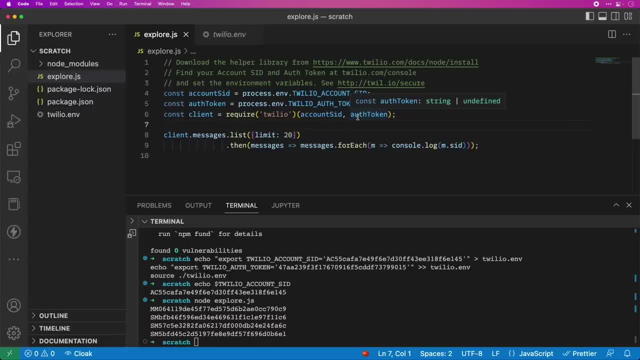 automatically create a brand new rest client for you, right? so this is a client that you're able to use to hit the rest api at twilio and, because it knows who you are, it's able to access stuff on your behalf. so very similar to what we were doing with the curl, but this client we can use. 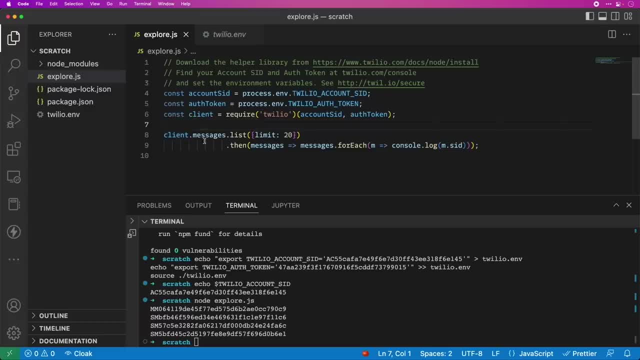 us multiple times, it will always be authenticated. so we're saying: of all of the messages, we want to list them, right? so we want to get a list of all of the messages. actually not all of them, only 20 of those. so let's go ahead, i'm going to just we know that we haven't sent 20, i'm going to get rid of. 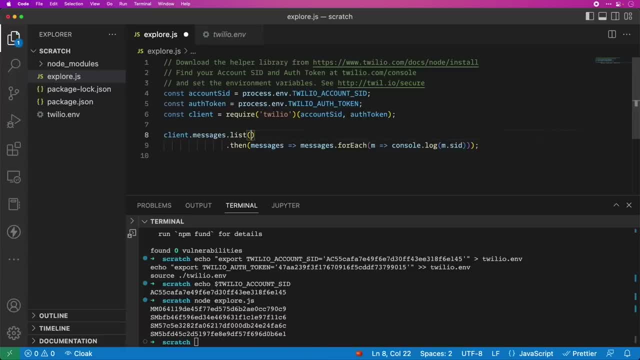 this, so you can kind of just see this other style here. so we're going to say, of those we're going to do this list, and then i'm going to bring this back a little bit here. so you can kind of see, let's change the structure of this a little bit. so we'll say client. 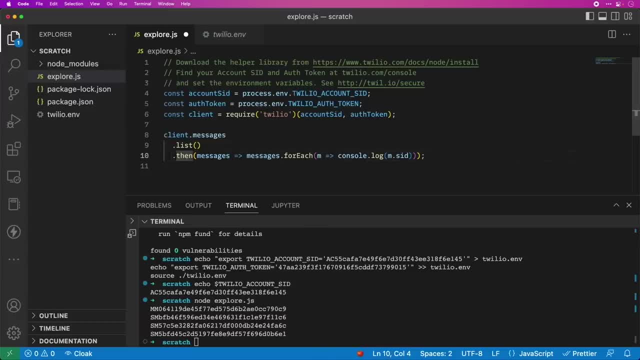 messages, and then we're going to do a list on those. now, the way that, the way that this works is: um, this is asynchronous, so javascript is asynchronous, and if javascript is new to you, you probably haven't encountered its asynchronous behavior. what we're going to go over here might 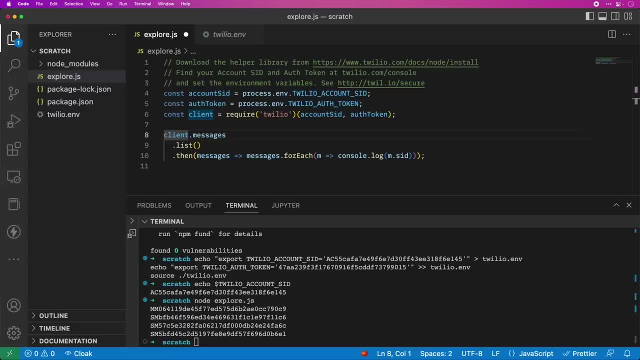 very well be overwhelming, but it'll make sense someday if you stick with it, i promise you. now i've added notes. but really, please, please, please, please, do not let this stress you out. i just want this to go over your mind about what's happening here and it's important to understand. 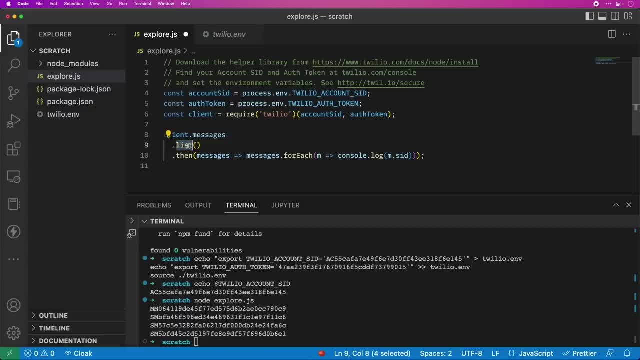 because our client here this late. these list methods are asynchronous, that which means that it's going to go and run off and do some things and then it's going to come back. when that comes back, it's going to run this code. so this is how a promise works. so it's: it's going to. 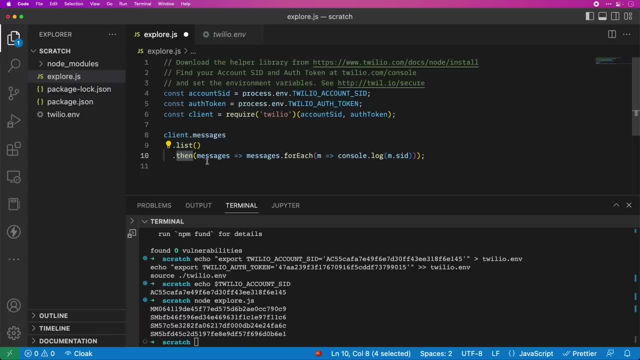 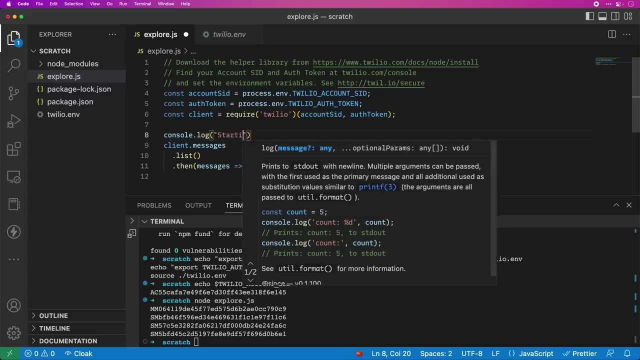 say then, after you go and make that request, then give me the messages, and just so you what's, what's kind of strange about that is if you're probably used to code, uh, working like this. so i'm going to write out to the screen that's this console log. i'm going to say starting, starting program and. 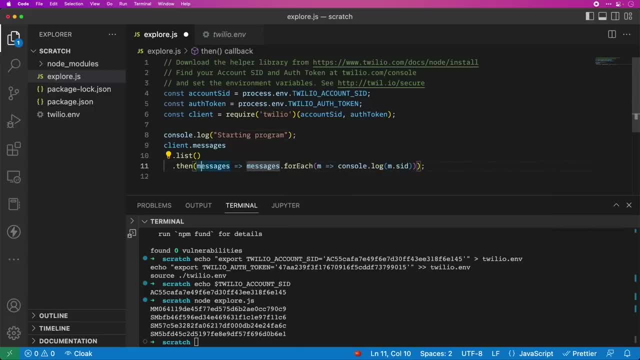 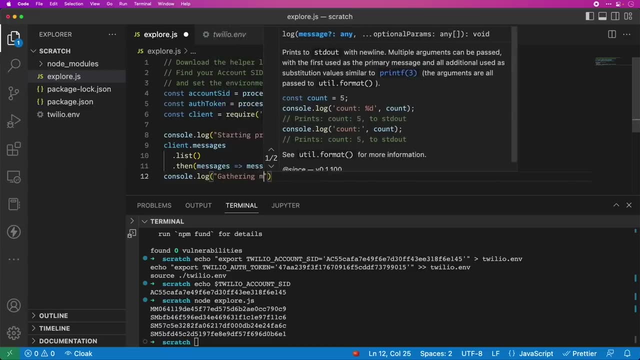 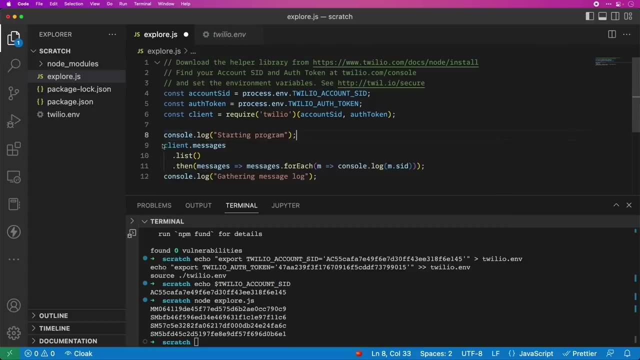 we should see that line print. now you might think that this is going to print: um, it's going to run this and then go. but if you, i'll show you here. if i do this console log and i say, uh, gathering message log, um what? what you'll see is it's going to say this: this line's going to start. 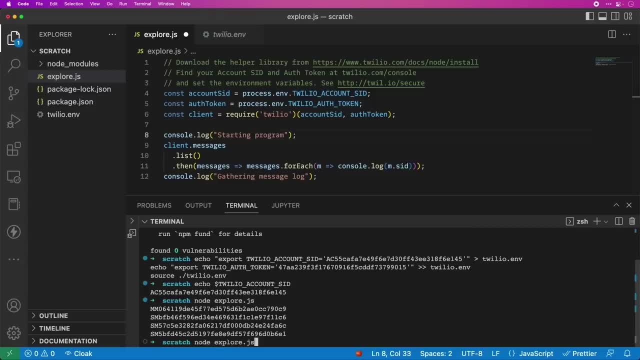 but immediately it's going to go to the next line. so let's do that. let's run that one more time. i didn't save it, so of course it won't do anything. so you can see this little dot here in visual studio. it didn't save, so i'm going to save that. run that one more time. here we go. 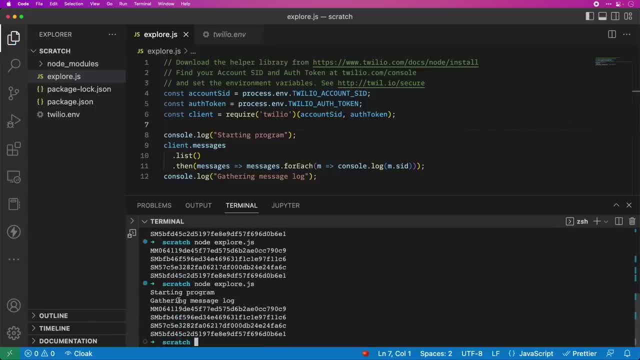 and you'll see right away. it's a starting program gathering message log, so it it ran this, but then it went down to here, so it did not wait, because this is asynchronous. what's happening here is asynchronous and what's happening is: client message list returns a promise. 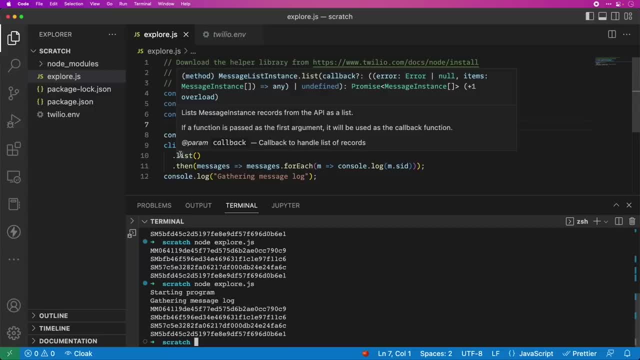 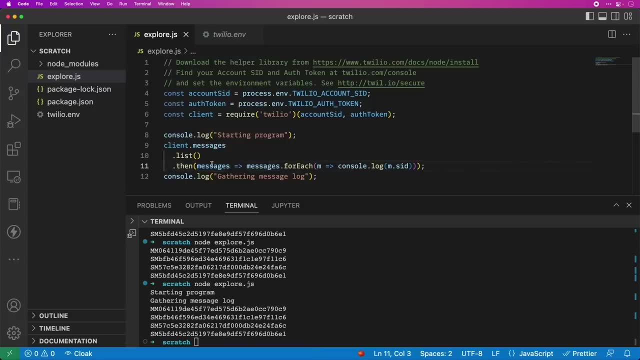 now. it's a promise that in the future there will be a value, and that value is messages, and so the way that you write that code is this: then waits, it defines a function here, and as soon as this is done, it will run this function. as soon as they come back, it will run the function. so that's what. 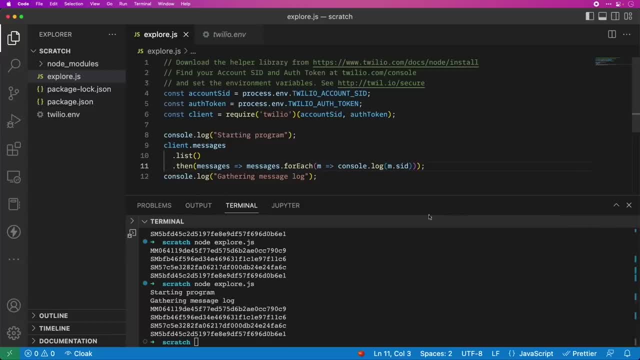 happened right. so it came, it started, it then ran the function. and when i say function, you might not have seen this before, but in javascript you can uh, make a function, uh, i'm going to put parentheses here so it's a little bit more clear. these are the 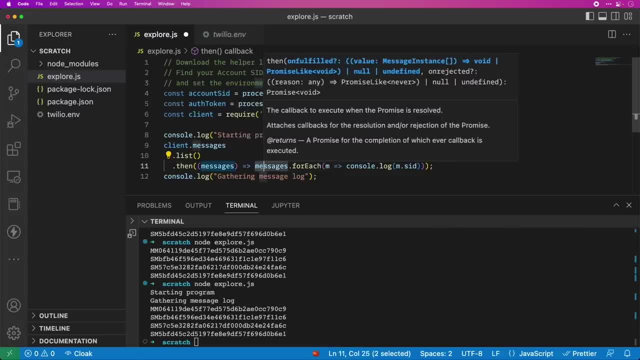 parameters for the function, and this fat arrow is saying: this is what happens when the function runs this like little. they call it the fat arrow. it's kind of cute, right? so it's an equal sign and then a greater than it's a. it's called a fat arrow and that's a way of quickly defining a. 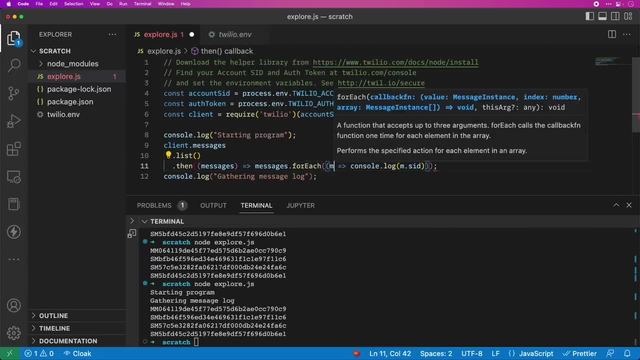 function, and so you can see here: um, there's another one here that's doing it as well- um, so it could be a little bit, uh, it could be a little bit uh, it could be a little bit, uh, it could be a, um, uh, messy. as you're looking at all these parens that we're looking at, it's kind of kind of hard to 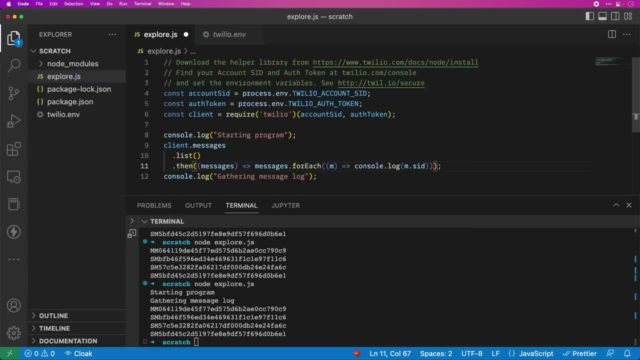 understand and read. if this is your first time looking at that, i totally feel for you, and so this messages that comes through here is an array. so so what was very nice is it came across this messages list. this is an array. it was a javascript array by itself. they have this method. 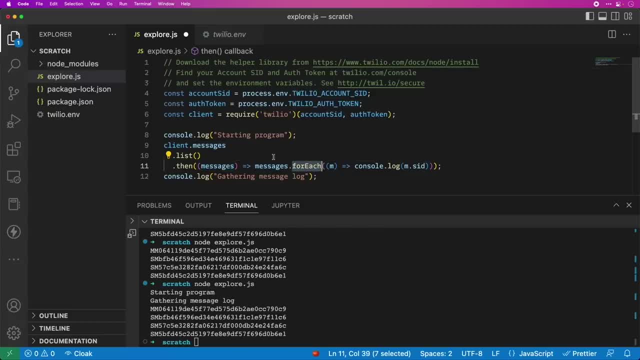 called for each on it and it will let you loop through each of the values that are in an array um and you'll notice that the object that was inside of that array has some properties. so what happened was the client went and made the request, made the http request. it got back that json that we saw. 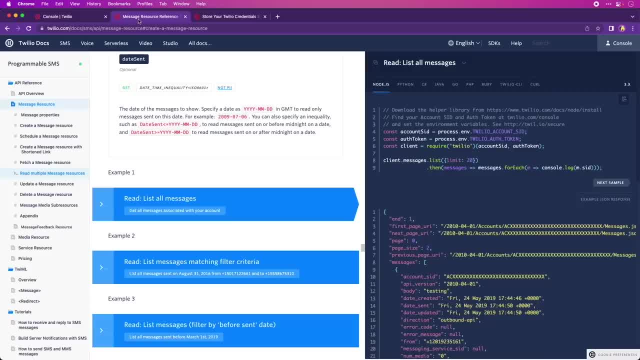 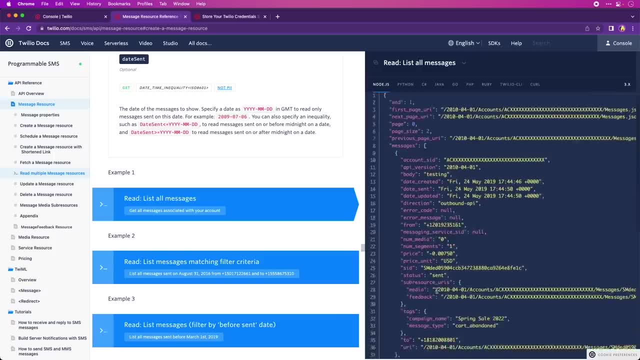 let me, let me just go show you one more time. uh, let's make sure that we're looking at the right thing here. so so we, we, we. this is the same code that we just saw. this json was returned, right, this json was returned. but what the client did for us was it inflated these into messages, right? so 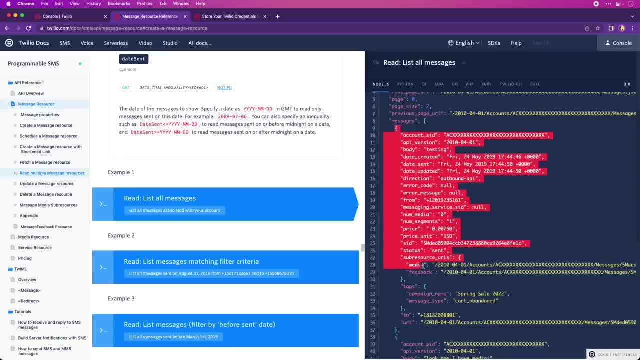 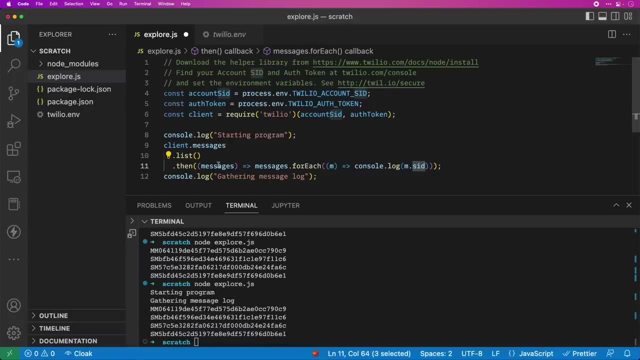 these are. this is this. this is a string of things, and it came back json. but i'm able to actually work with each of these messages as if they're an object, so let's look look at that again. so, uh, list returned this object, this array of messages, and each one of those um in that array. i'm able to use an array method for each and. 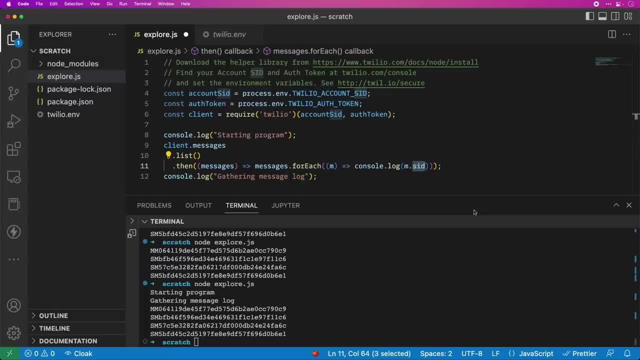 this message is an actual object that has a property called sid. um. so again, if that is all new javascript terms to you, don't forget to subscribe to my channel and i'll see you in the next video. don't worry too much about it. basically, we went and got the messages and we showed the messages. 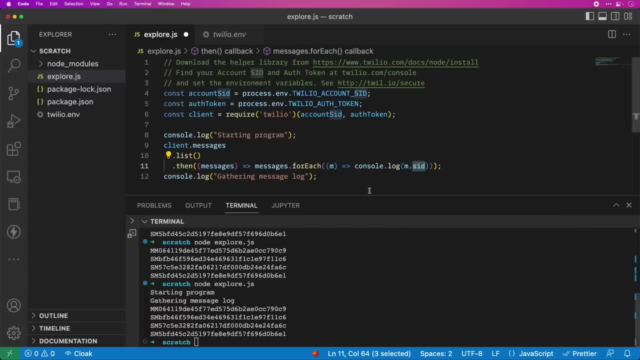 that we got. that's what this is saying, one of the things that i want you to be careful of as you're looking at promises- and you might see this sometimes as you work with apis, because oftentimes apis that you hit are going to be asynchronous like this- you might see that, uh, you need to be. 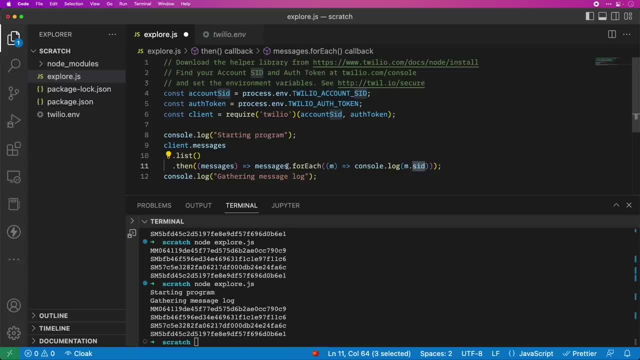 able to. you might run into an error, and what's good. what might happen is it might get swallowed. in fact, let me cause one to happen. so i here- it's supposed to say off token, i'm just going to put in, uh, um, my luggage, the password to my luggage: one, two, three, four, five, six. so that is not. 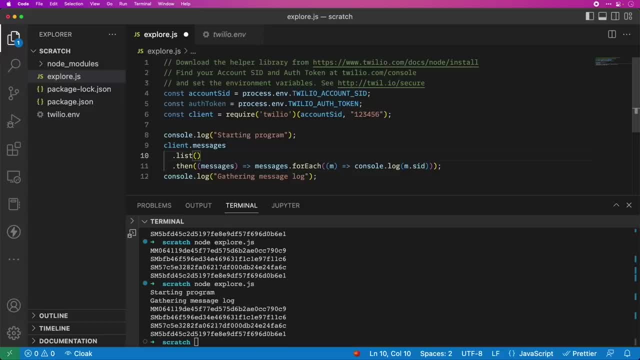 my account said: um, that is going in there, so i have the wrong account said. so i'm gonna say that, hey, this is the client, this is what how i want you to authenticate, and it's going to go to try to make this and it's going to fail. let's see what happens when it fails. 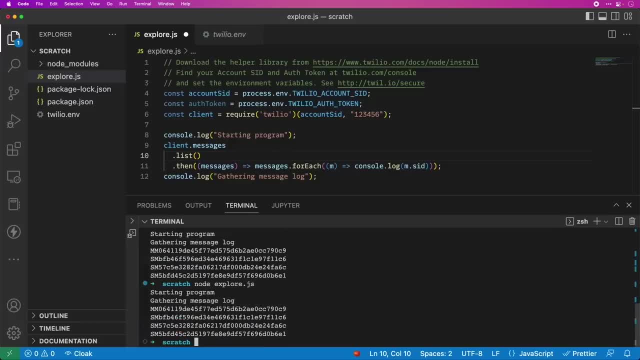 well, i didn't save it, so let's save it again. boy, that's a lesson that i really didn't know. you got to make sure you save your file or the code doesn't run, so let's do it again, um, and you'll notice that i didn't get any error at all. you know that can be confusing, that that. 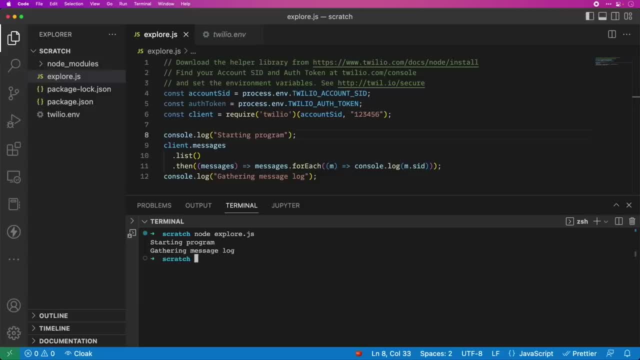 is something that is very strange, because obviously something wrong happened. i didn't get any of the messages back, but it doesn't look like i did. i had any problem. so what's happening? because this is running asynchronously. this then never runs right. we never get a chance to run this. 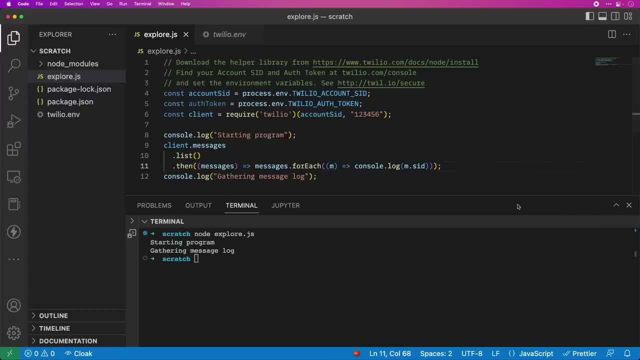 because this list method method didn't actually, uh, finish working. so one of the things you always want to make sure that you do is to every promise you can catch. and you can catch an error, and i'm going to make a fat arrow because i'm going to have a function happen here that says: 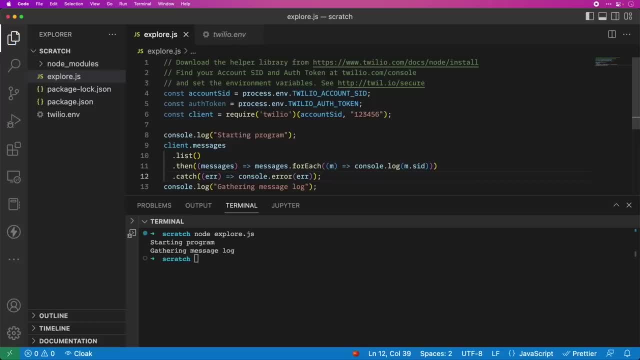 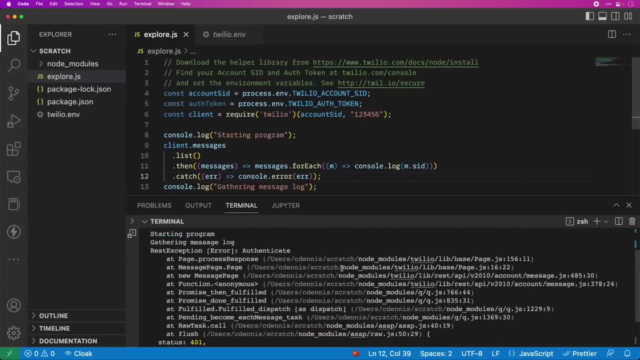 consoleerror err. okay, so now i'm going to print that out. i'm going to print out the error. let's run that again. let's see what happens. ah, now we see the error and you'll see that sometimes, uh, this is uh. what comes back is there was an authentication error, right, and we got a very 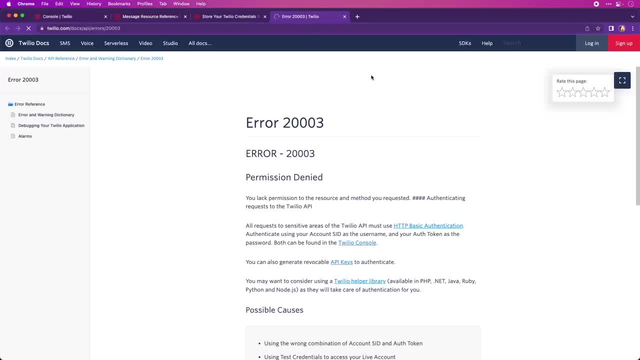 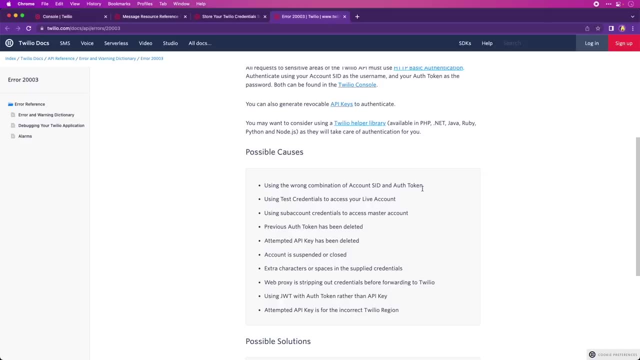 specific error on this 2003 and it will help us kind of look at what's happening. oh here, great, this is right. my off token is wrong. the wrong combination of accounts said an off token. exactly that is what has happened. um, so cool use of uh things there. i'm gonna put this back so that 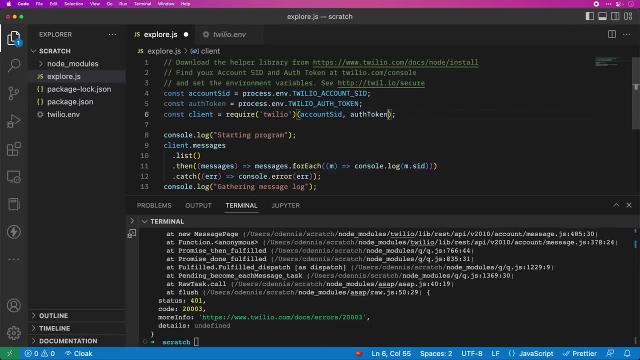 we have uh things working, uh. so this was off the token, um, and i can still leave my error in there. i'm not gonna hit an error, so it's not gonna happen. so a promise has a then and it also has a catch, right? so, uh, let's do that. so i'm gonna run that one more time and save it. wow, y'all, i. 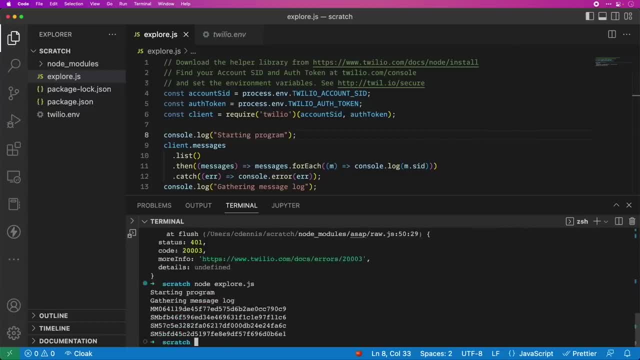 gotta get better at saving. here we go, there we go, so now we're back to working again. awesome, all right, i'm gonna show you a little bit of a different way that javascript can work. uh, asynchronously- that you might also see. um, and this is really syntactical sugar, it's called async a weight. 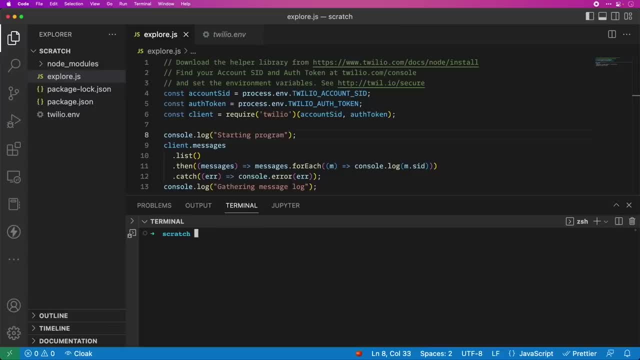 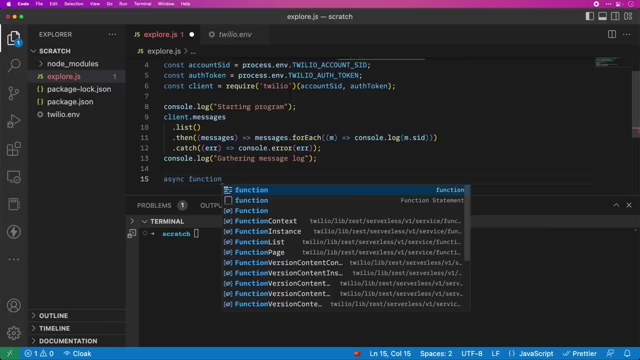 and if you just, uh, wait a bit, it will all sink in. i promise that's a. there was three jokes in that one. that was a. that was a hat trick of a joke. all right, so here we go. so, um, the way that it works, the way that this works is you can say that if a function is going to be asynchronous and 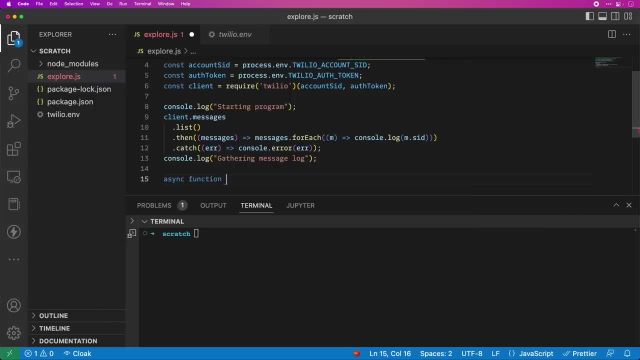 we want this to run, um, uh, asynchronously. so i was thinking we're getting ready to start using our number in an application and to get there, we need to clean it up. we have a bunch of weird messages in there that aren't going to be relevant to the messages that we have, so i'm going to make a new. 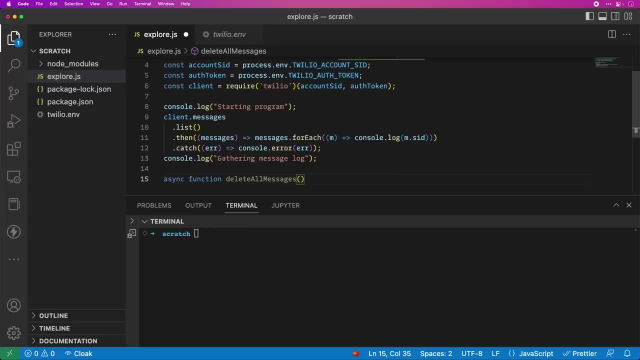 function and i'm going to call it: delete all messages. okay, when you define a function, you can kind of put: uh, the this is the parameters that it takes. we're going to say that there are no parameters and then i'm going to run this function. so, um, 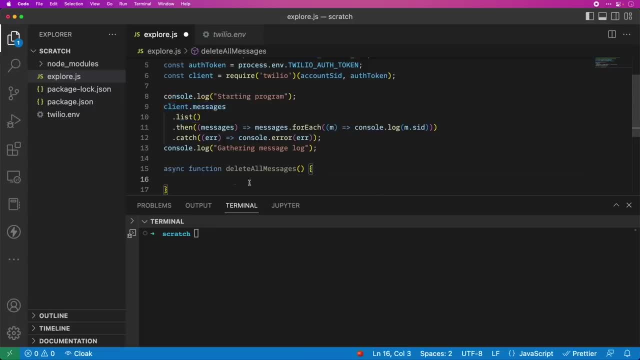 while this is an asynchronous function, i can actually make it look more, uh, like it is in line, so it can kind of run the way that we want it to. so i'm going to say: const messages equals await. so now i have, because the function itself is asynchronous, because i've used this here, i can. 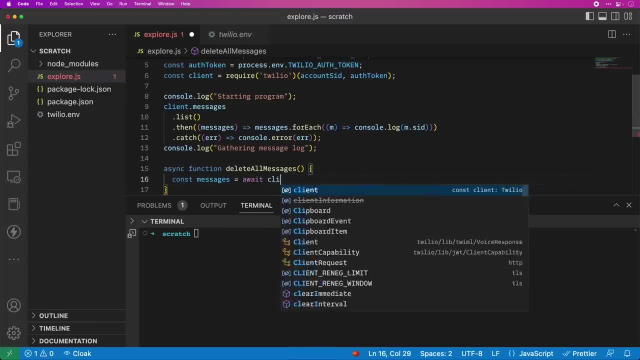 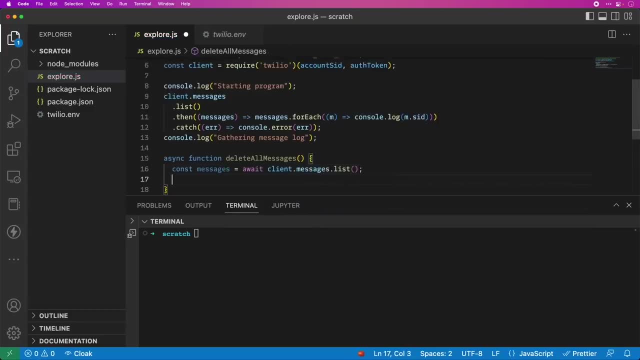 use this keyword, await, and i'm going to say client dot messages, dot list, and so now i think this is a little bit more clear, right? so this is basically doing the same thing, right, these messages are the same messages that were coming into this, this function, but now it's out on this side. so i 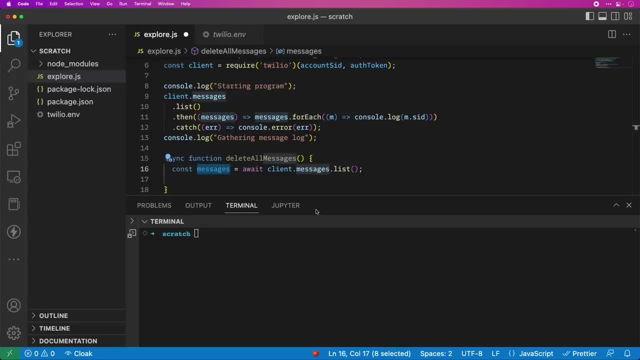 have this variable that's called messages. so, um, and that's an array, right and it's, and i could do, i could do this exact same thing here and i could list that, uh, the same way, but let's, let's go a little bit farther. so i'm going to say, for each of the messages, for each message, that is of the message. 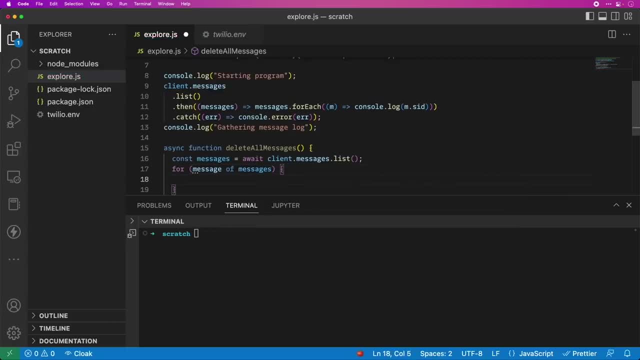 is array. so these are those uh inflated messages that we saw. uh, one of the cool things, um, that you're able to do with the client is the the. the object that's returned back has actually has some properties on them, and one of those properties that it has is called delete. uh, before we do that, 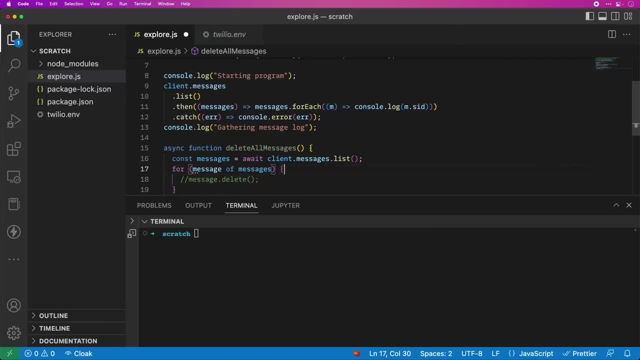 i'm going to make sure that let's do a warning uh here real quick. so i'm going to say console dot warn. we're going to say would have deleted. i'm actually going to use, if you use, these back ticks. this is kind of a neat trick. 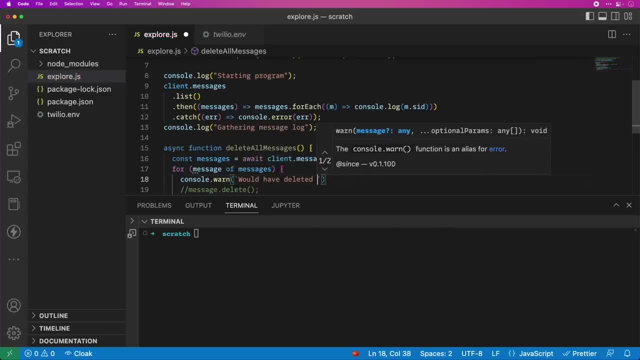 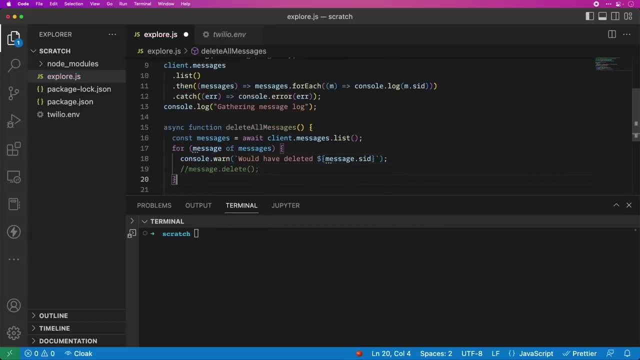 you can use this back tick to do string interpolation. so we'll say: would have deleted message dot sid. so again, that's the string identifier of that. so i would have deleted message dot sid. so, and uh, we will close that function out. all right, and now i'm going to call. 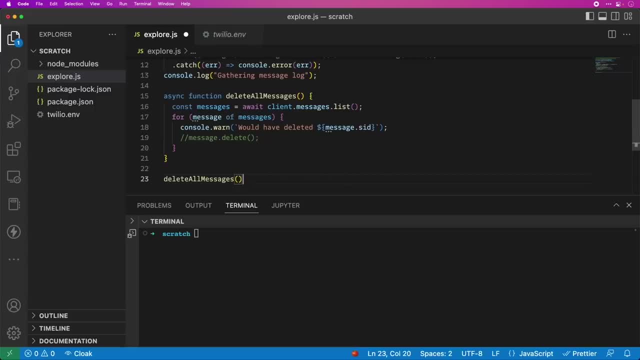 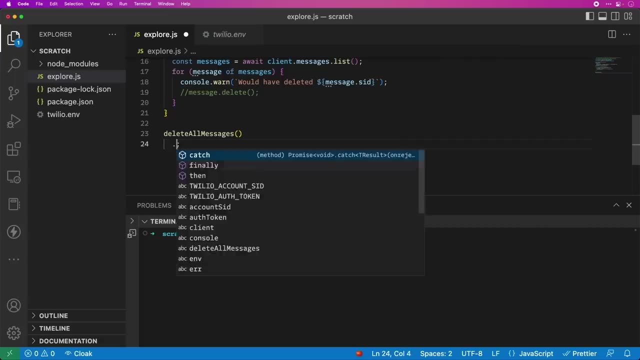 that function in this- you know, of course, that's how we call it and this is- would actually be a promise. so this would be a very similar. so we could do this, we could do a then. uh, in fact, let's do it. we'll say then and uh, if you, 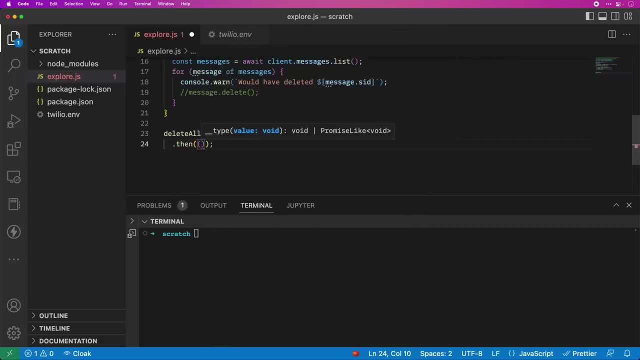 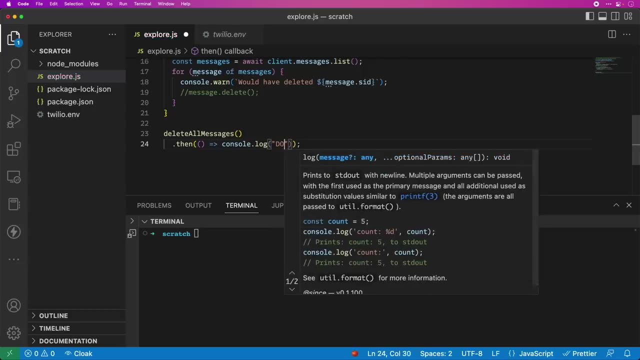 wanted to call a, make a function that has no parameters, because i'm not returning anything. right, i'm not returning anything from that function. i'm just going to say consolelog and i'm going to write done, and i will put all of these, this code, into the notes, so you. 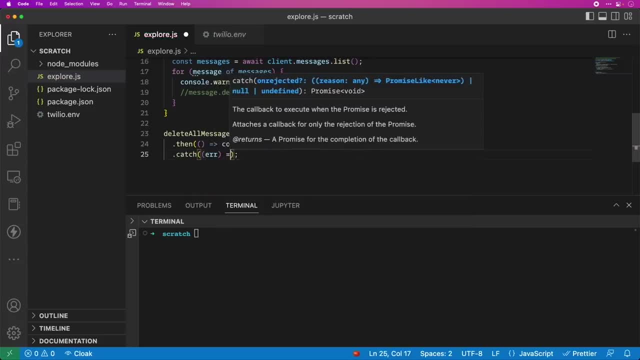 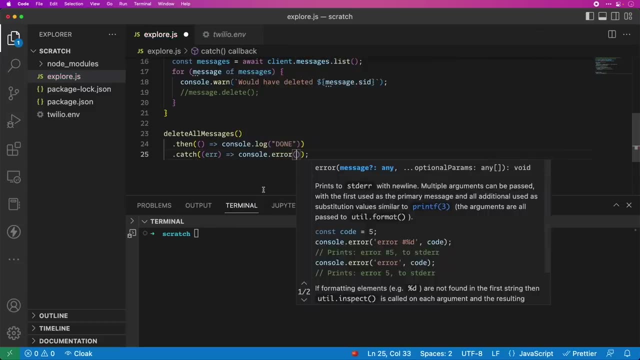 can also copy and paste it if you want to, and i'm gonna do the same thing that i did before: catch the error and i'll do. we'll do consoleerror. and now, if you use the console is you know, of course, what's running when the program runs is running out to the screen. 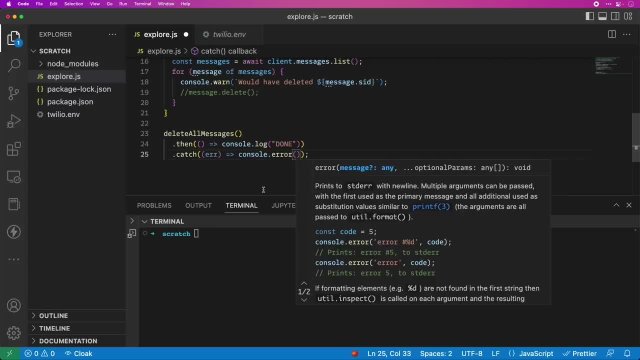 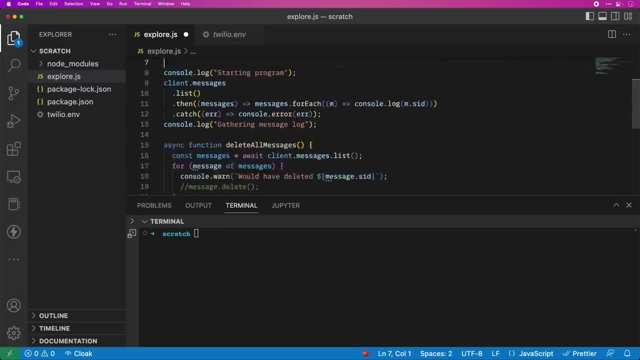 and there's different levels that you can do, and error is one of those, and if i just pass the error, that happened there. so, um, i'm going to warn that we're going to would have deleted the message, but let's, let's take a look at what happened. so i'm going to get rid, i'm going to keep the starting. 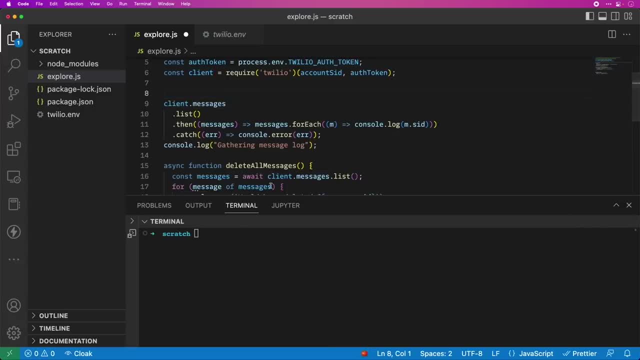 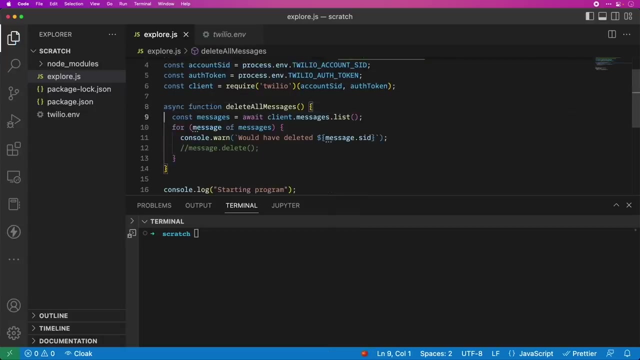 program here, right so, where we can do a starting program, and then it's going to do: delete all messages. it's going to call that and then, when it's all done, it will say: done, i'm going to get rid of what we had here. okay, so we have, delete all messages. it's going to go and it's going to get a. 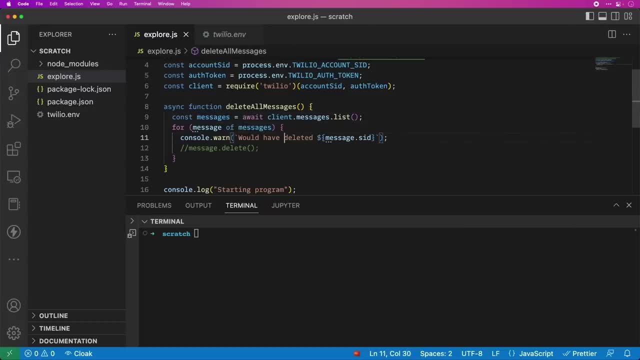 list of all the messages. it's going to loop through each one of those messages and, uh, when it is done, it's good. we're just right now we're going to warn that it's uh, would have deleted it, and this is, uh what we're eventually going to do, because there's a function that's available. 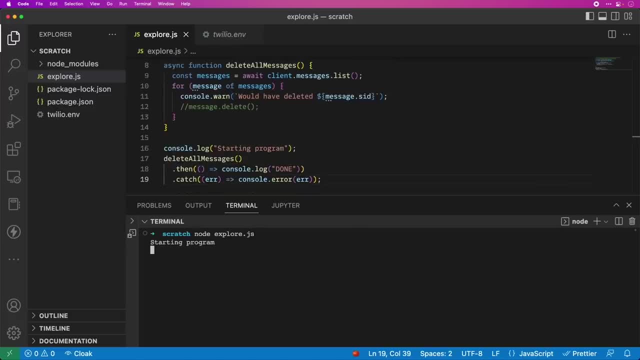 to it. all right, so i'm going to save that, i'm going to run it, let's see what happens. okay, so it would have deleted some of our sids. and again, this is the mm, this is the. the mm means it was the mms, which is the one with the picture and the rest of the sms that we have. so 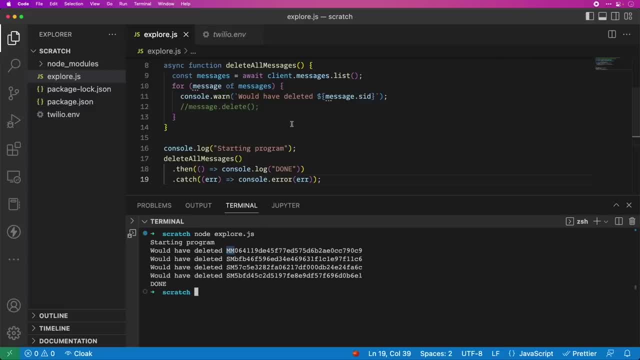 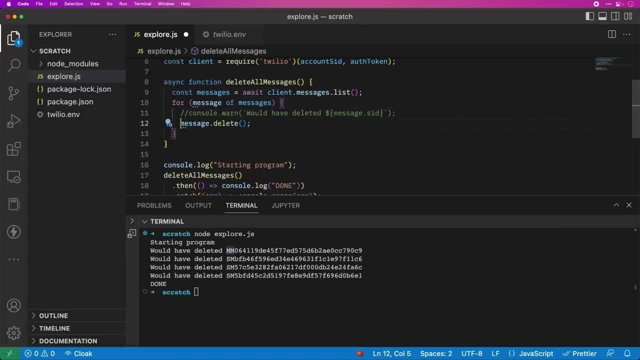 i think i am ready to do this. i hope that you are ready to do this as well. again, this code, should you want, it is available in the repo. because you want to run this, because you want to delete these messages, um, so, let's, let's, i'm going to say it would have deleted. 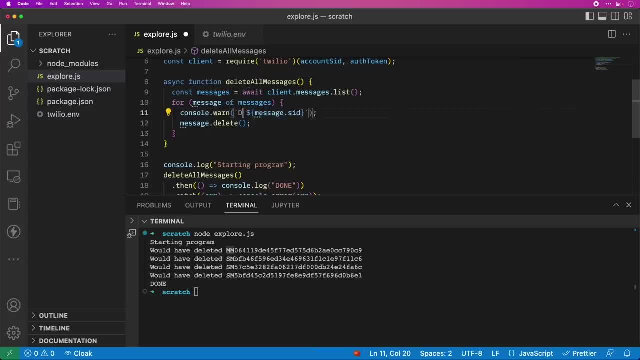 i'm going to say deleting, and then, uh, here we go, i'm going to save that, i'm going to run it, and so so message: the message object that's coming back from this client is really has enough information to make another api call to delete itself. right? because? um, because the object itself knows how to do that. 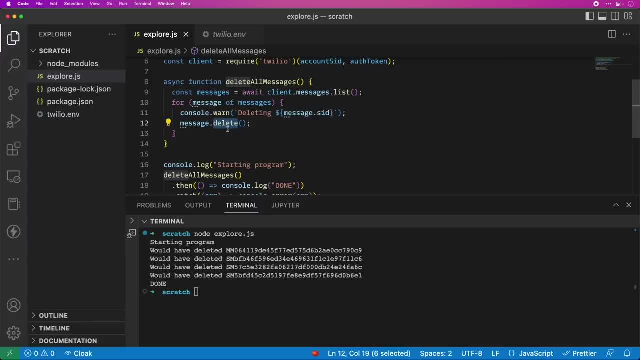 the library has made an object that is smart enough to be able to call delete on it and it feels like, um, it's just working that way, but it's really making a rest api call to make a delete request. it's pretty cool, right here we go. messagedelete is not a function. uh, what i meant. 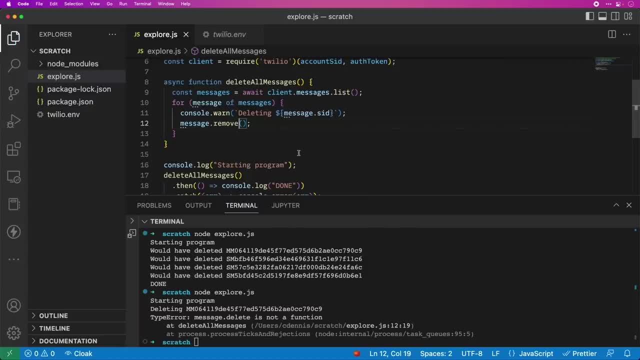 was actually remove. uh, so the function name is remove on the message. so here we go. so, um, and you saw that there was an error. right, that was the error that just happened. a good thing i put that catch in there, otherwise we would have thought it worked. uh, so here we go. so note, explore, move. 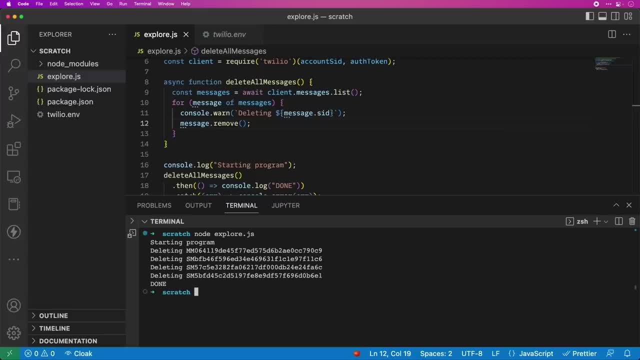 instead of deleting, deleting, deleting- we deleted all of those um. so remove is the name of the function that's there, but it is doing a delete, making a delete call, cool. so we have now cleaned out and if we try to run it again, you'll see that there's no messages left for it to delete. awesome, now, if you. 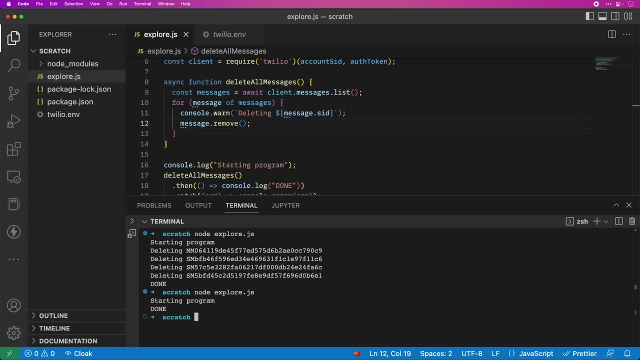 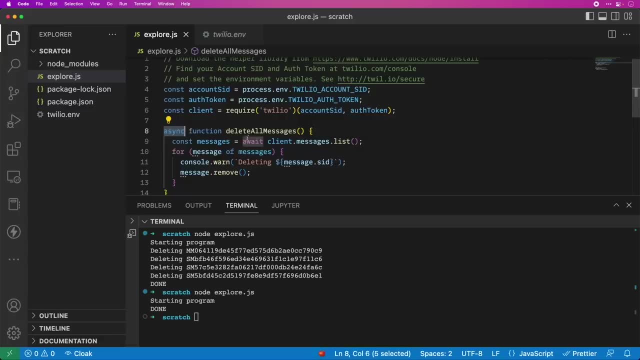 have just watched that and we're very confused. let's walk this last bit and then i want you to rewind it one more time. so i've made a function that is asynchronous and that function is called delete all messages, and because it's asynchronous, i'm able to use this await, which will return this: this clientmessageslist. 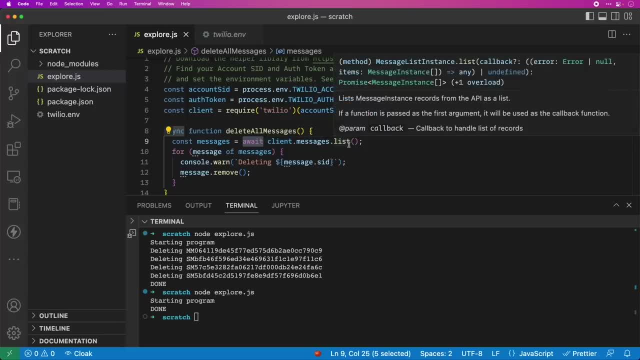 returns a promise, okay, but, um, a promise of the future, but because it's being awaited, it's going to return it right here in line. then i'm going to loop through each of those messages. and because that message came back from the api and an object was created thanks to our helper library here. 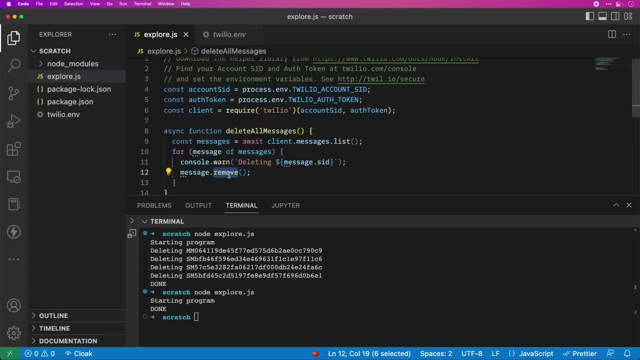 i have a, i have a method on that message called remove, and it will actually go and do the next level, the next level of delete there for me. so it's it's really nice. this object feels like it would uh feel like if you were writing javascript code. it would feel. 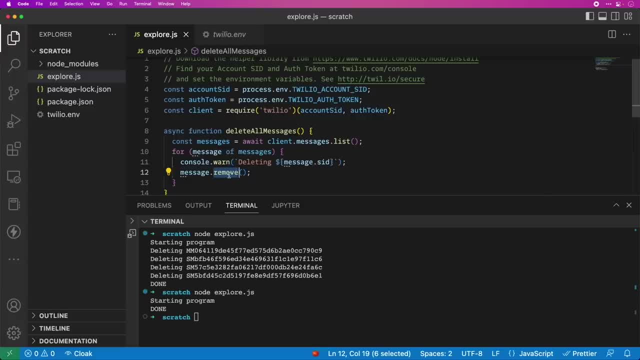 this way. uh, but behind the scenes we know that it's doing this. api calls and the client library has abstracted all of that away from us. uh, and if now, if you go and you take a look, let's go back really quick, let's take a look. there's other helper libraries, so if python happens to be your, 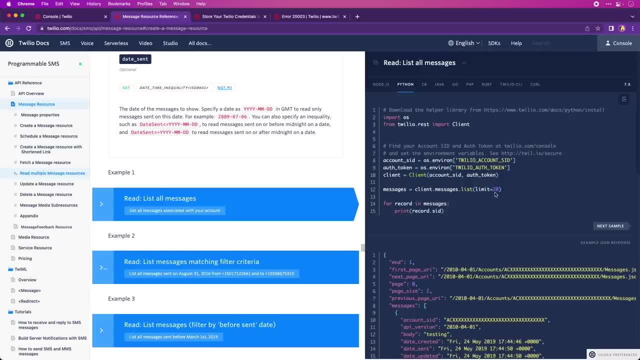 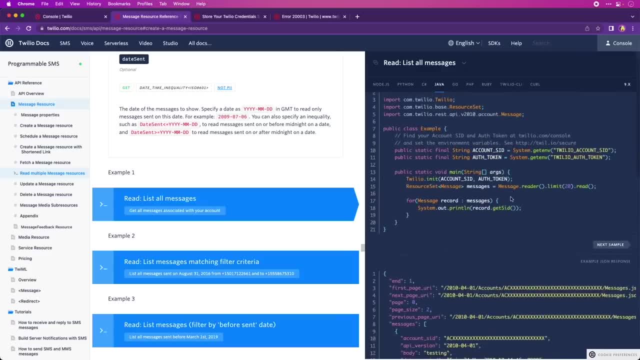 your language. there's how you do it. so it's: clientmessageslist returns a promise. so if you go to clientmessageslist and for record and messages and you print the record set and you can see that the code looks a little bit different in all the languages that you go through, but it's. 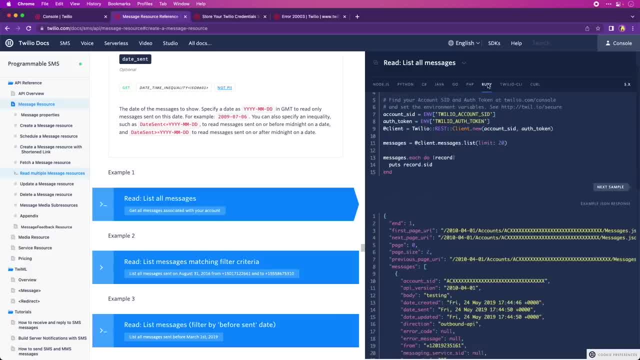 also kind of similar and so that's really nice about the standardness of a rest api is that the helper library is producing code that feels the same uh in each way, because the library is kind of the same and you'll you'll find that as you use other apis, um, and they have helper libraries. 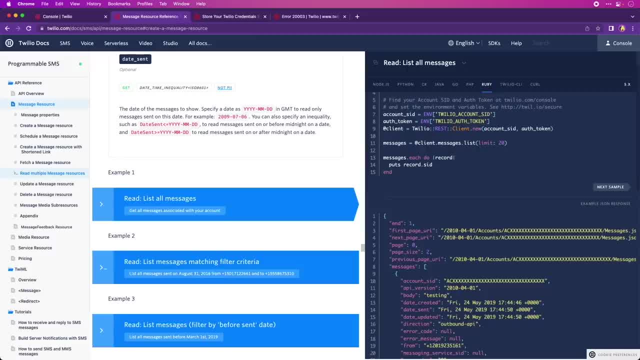 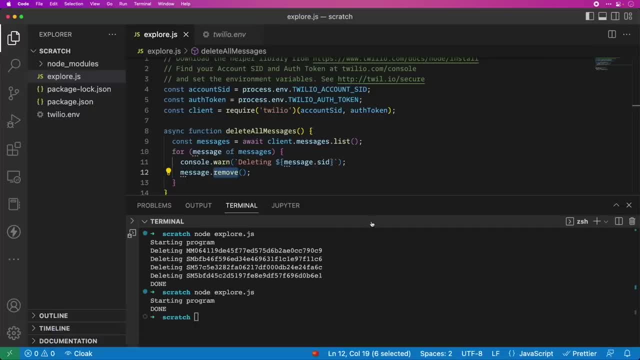 they will. they will mimic the way that the rest api looks. so i realized that was a lot. i don't want you to get hung up if you feel like you can't completely understand what that is. uh, in the next unit, what we're going to do is we're going to go. 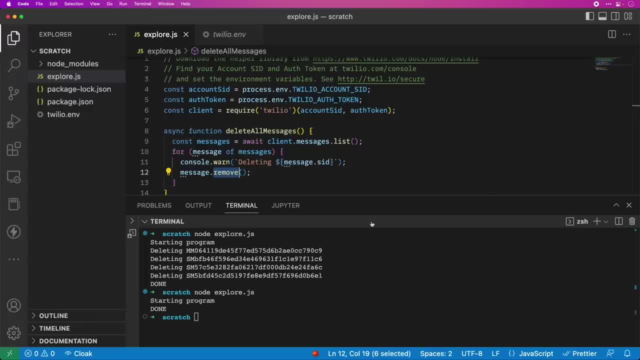 into more deep things, and i know you can do this. so, so there, this code is there. and also, if you feel like you want me to go back and explain that again, please, please, please, please, pause me, slow me down. let me walk through those, uh, different things, but don't feel like you need to be able. 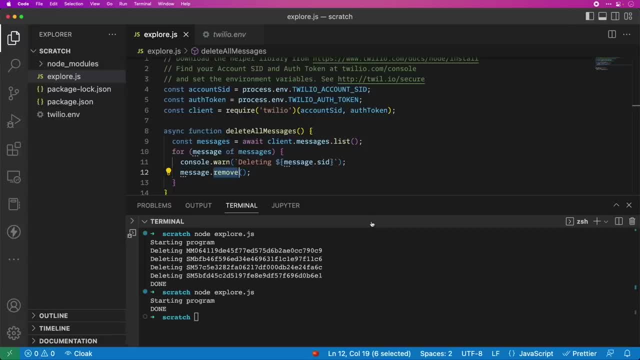 to read this. i want you to just conceptually understand what's going on, and i'm going to understand that you're using a helper library that's abstracting away all of the http api things that we were doing with curl and we were doing with rest fox. this is just doing it in code and 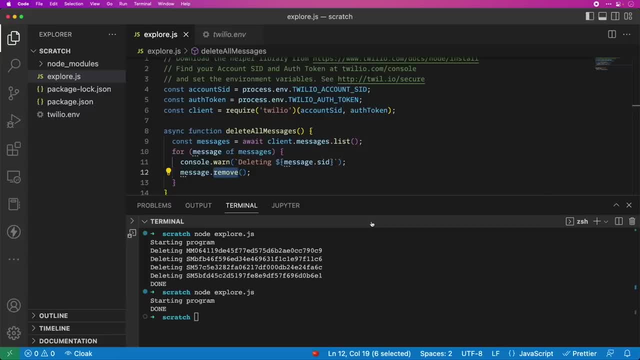 it's doing it for you. a lot of the magic is gone, uh, and hidden and tucked away and it just feels like you're actually working with these objects. that's the power of the subtraction- awesome. did you see how the helper libraries are all similar, yet match the development and the? 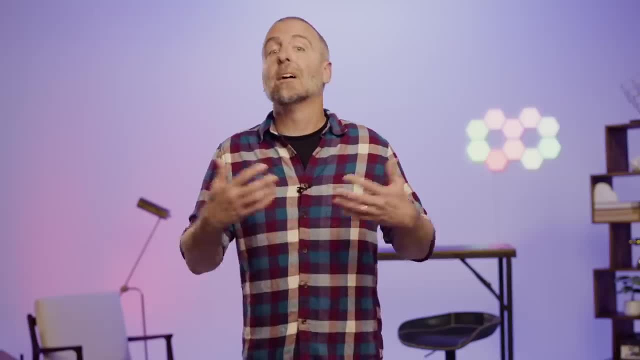 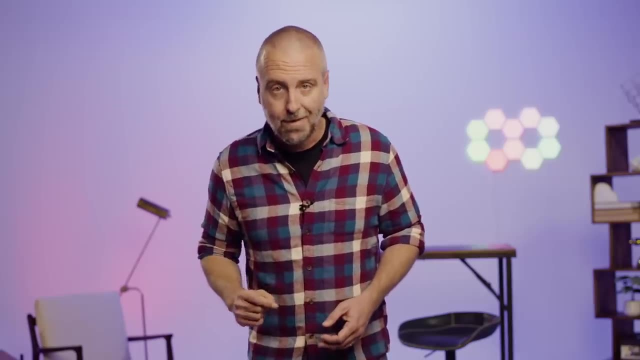 workflow and style of each language. this is one of the benefits of helper libraries in general. they abstract away the http client connection and the boilerplate necessary to make rest api calls. they also behave as you expect them to behave. it feels natural. the way that we were able to 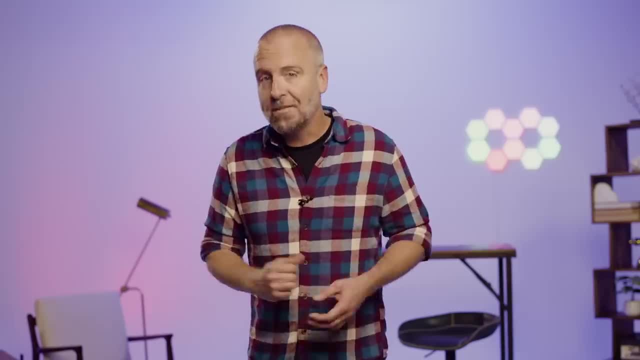 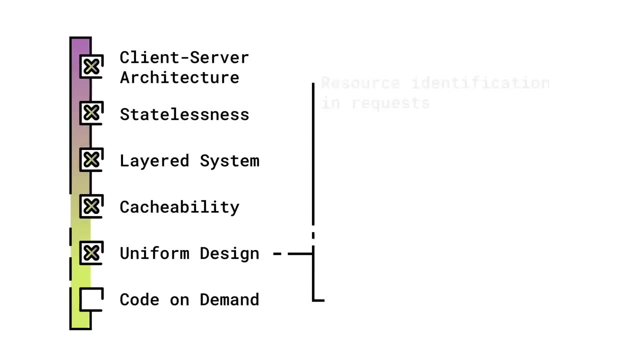 delete from the resource itself helps to unlock another rest api constraint, scavenger hunt item, and that one is uniform design. now this constraint has four subsections, one of which we just discussed: resource manipulation through representations. because enough information was included in the response, it was clear for us how we could modify and delete the resource. another subsection in here: 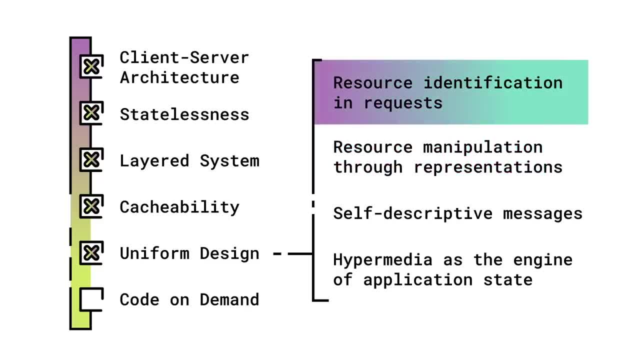 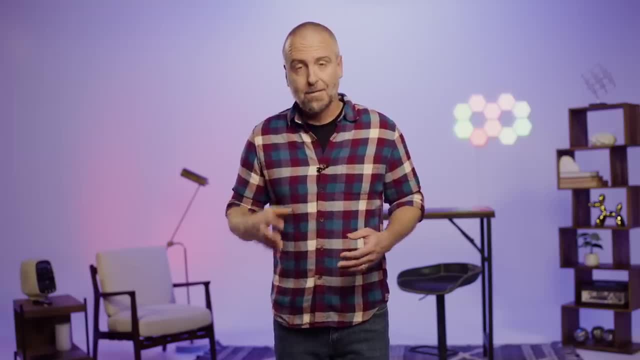 is resource identification and requests. that's the uris that are included and we've seen that. but because the uris are included, we know how to get and manipulate specific resources. uniform use of the http verbs is pretty powerful. we just wrote some scripts that make use of helper libraries. 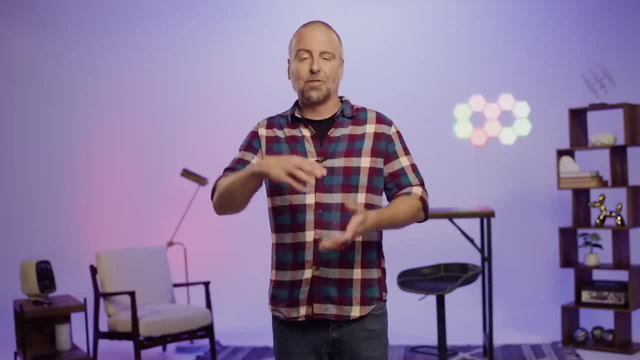 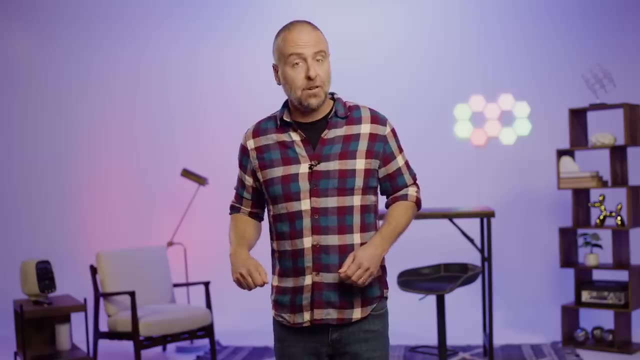 libraries are super handy for automation-based tasks or batch scripting, which is like making a whole bunch of calls at once. Now, while we're talking about this, we should cover another common tool for talking to external APIs, and that one is CLI Command Line Interface. 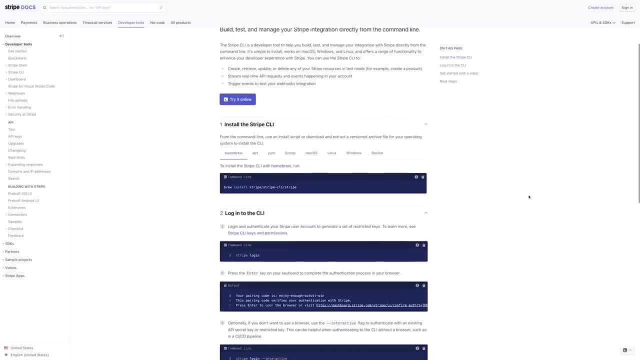 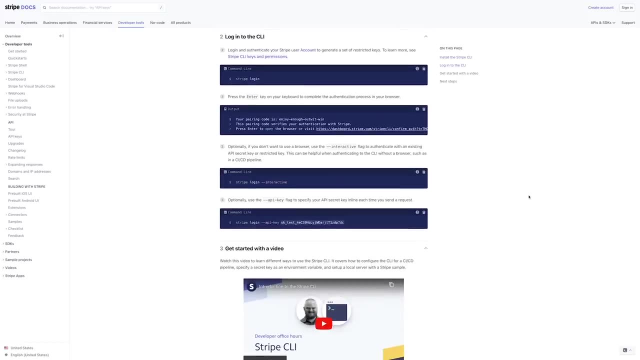 There it is again. Command Line Interfaces can be used to make API calls from an executable on your machine. More and more these are showing up for tools that require authentication and do a bunch of different services. This concept is popular amongst cloud providers, where setting something up needs to be done quickly from the command line. 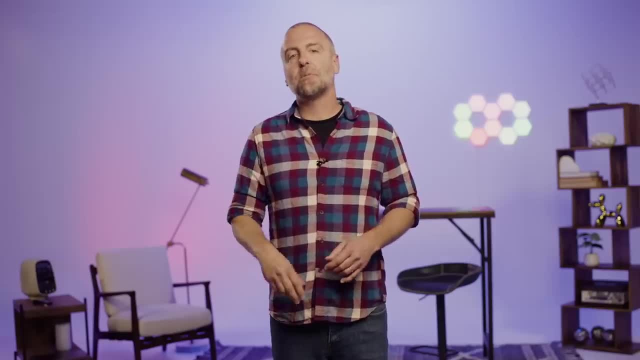 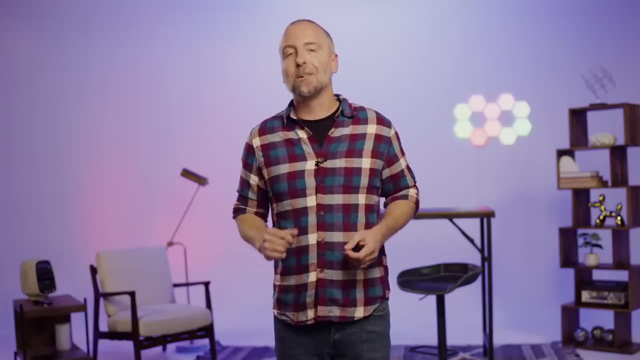 Check the notes for more. Another common place where you'll use helper libraries is from within applications that you're building. Let's get to the final unit of this course and implement an external API into an existing web application. You've got this? Ooh, we're here. I love this part, the building part. 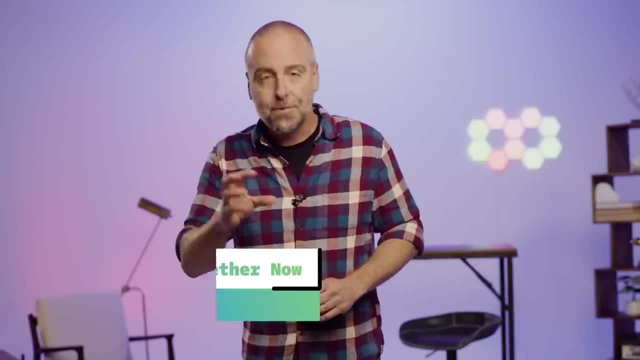 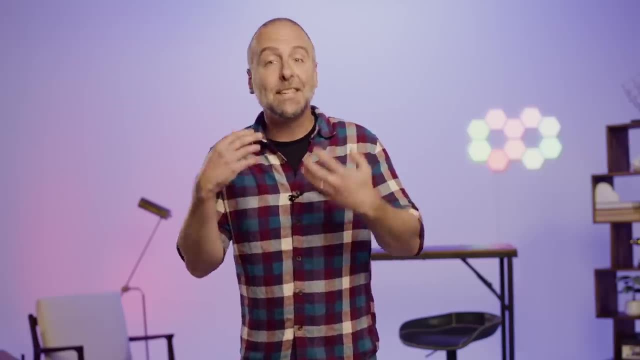 We're going to build a web application that shows off a set of user-submitted photos for a specific prompt. But here's where our app is going to stick out from all the rest. We're going to let our users submit their photos and captions via a text message. 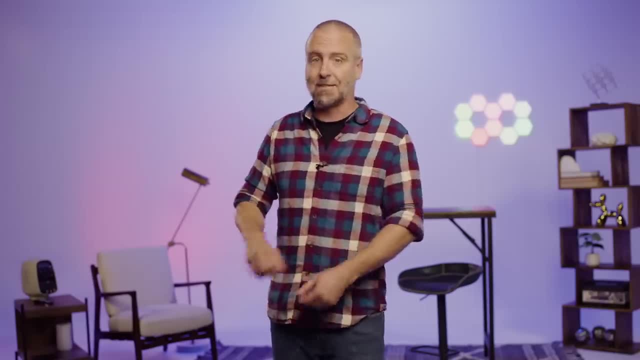 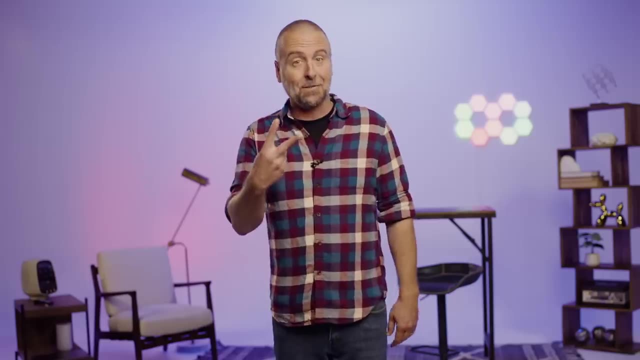 What this will enable us to do is put up signs and billboards and physical spaces that says text, a photo to this number, And then our site will gather those on a web page and display them. Now you're probably wondering two things right now. 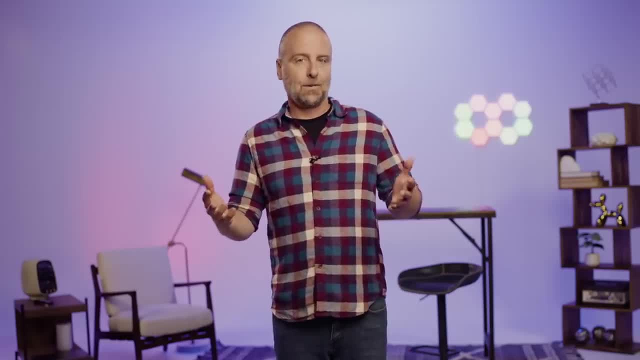 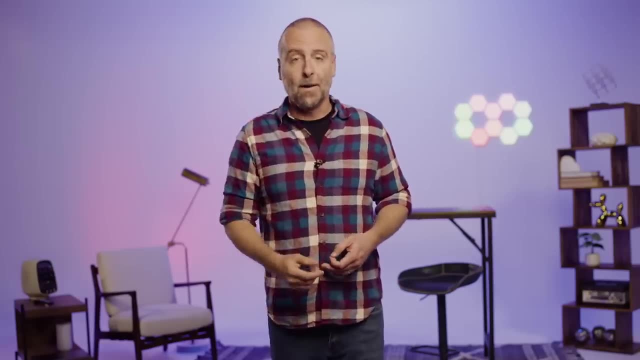 The first one is probably: wait, what are those photos? they're going to be texting, And that's a great question. We're going to be building this application so it can be dynamic, so you can define whatever you want Like text me a photo of your dog. 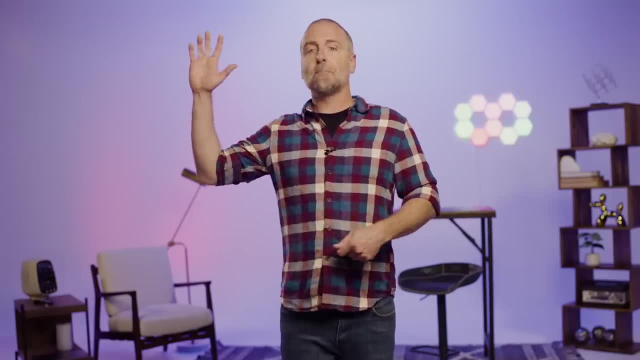 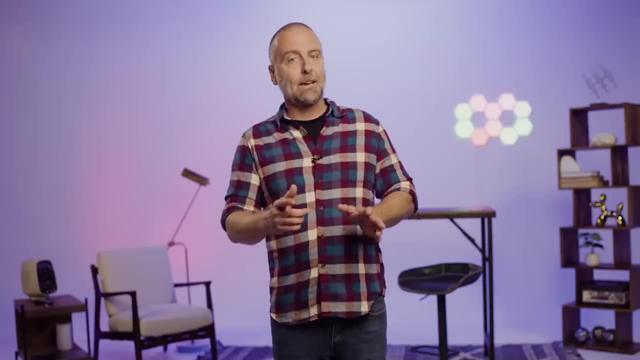 Send us a photo of the view out your window. Snap me a picture. Pick up the best impersonation of me. I don't know Anything along those lines Now. secondly, you're probably wondering: wait a second. you said I didn't need to know how to code. 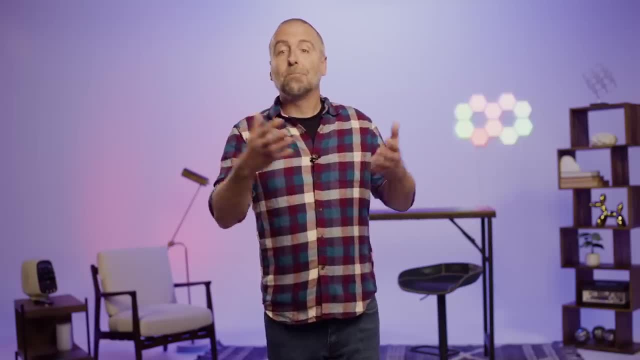 If you already know how to make a website, this part might not have fazed you. But if building a website is outside of your learning journey thus far, no sweat. I've got it set up and we're going to take our time. 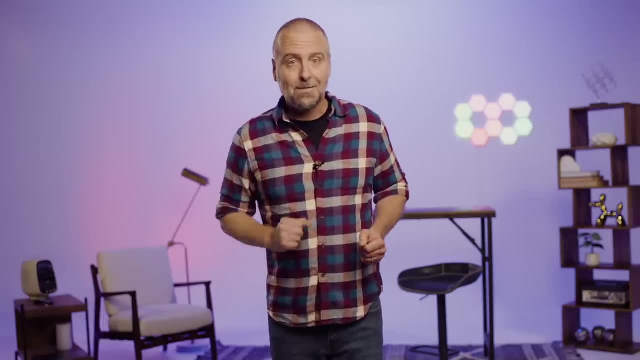 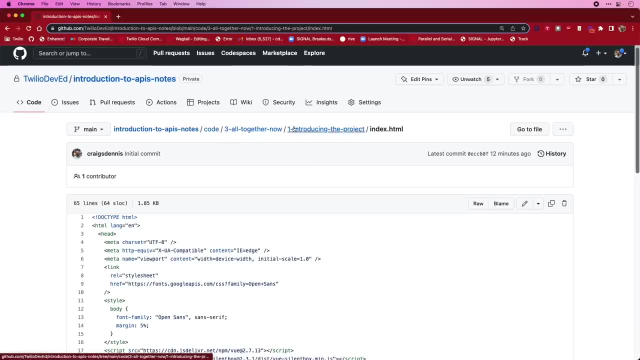 We're going to focus on making things work using this API. All right, Let's do this. OK, So I have a template here in the notes in the unit three, video one, We have this indexhtml, which is our web application. 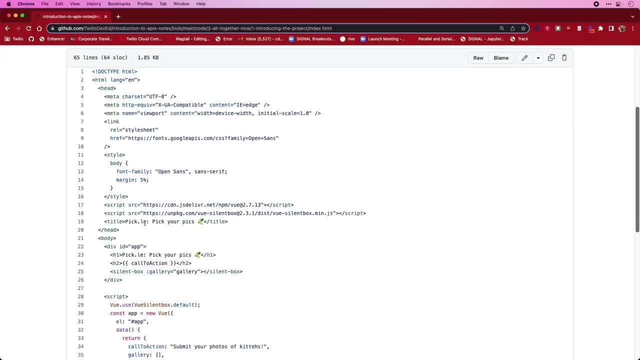 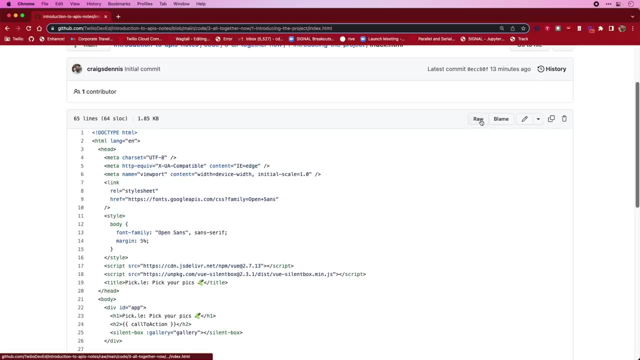 If you come in here you can scroll, You can kind of see things here. The app is called Pickle, where you get to pick your picks. Peter picked a pickle pickle- That sort of fun joke there. And then we're going to click this raw button right here. 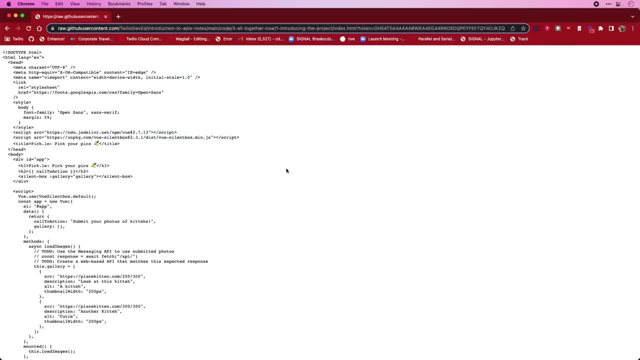 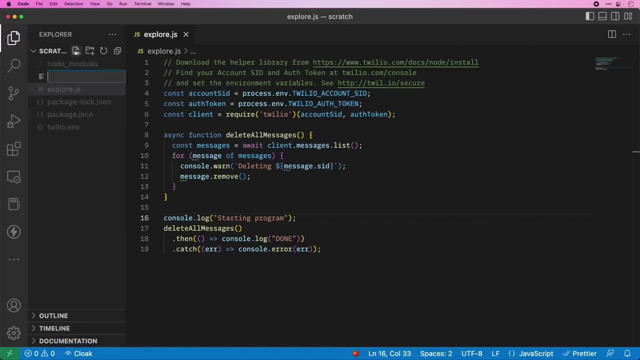 We're going to get a hold of this raw And I am going to highlight everything and use the magical developer command C copy. and then I'm going to come over to back to my scratch on my Visual Studio code. I'm going to make a new file. 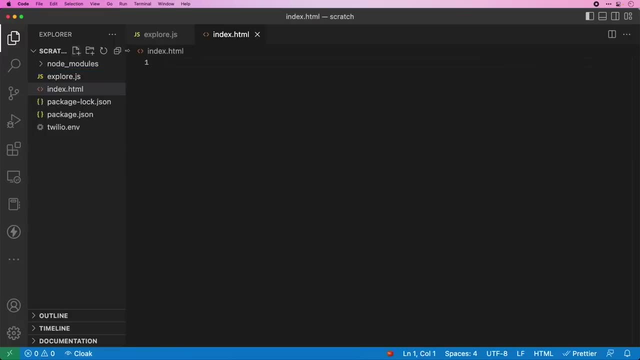 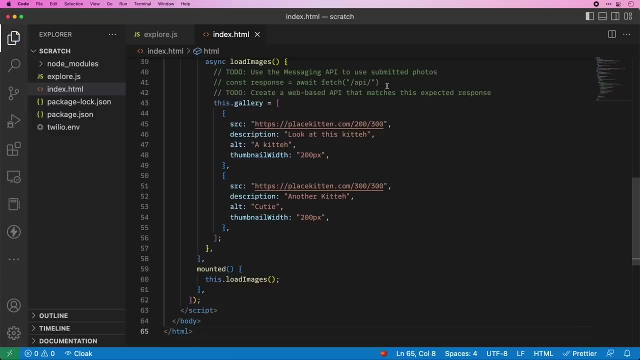 I'm going to call that indexhtml hypertext markup language right, And I'm going to paste that right here. So now I have that code locally on my machine. If you are a Git user, you could definitely check this out and have your own version of this if you wanted to. 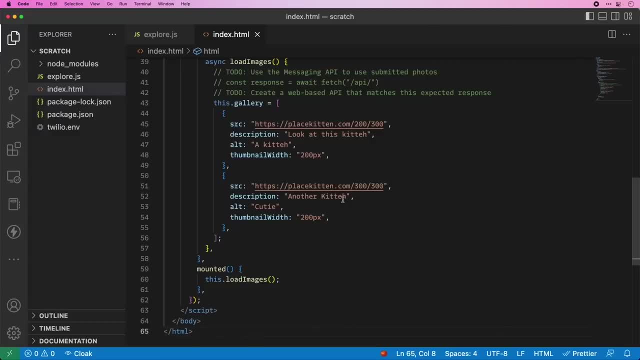 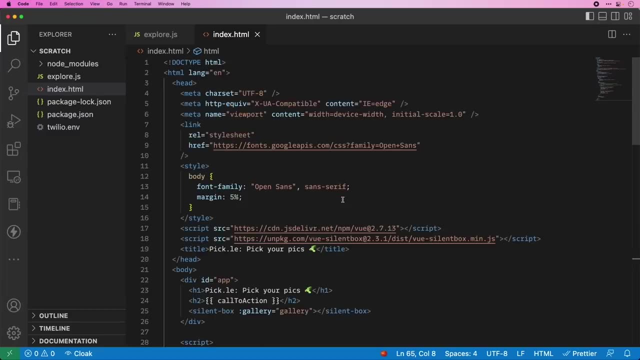 But that's a good way to get this here locally, because we're just going to explore around here just for a little bit. Let's take a look at this file as it exists. This is something that might happen to you as a developer who knows now about APIs. 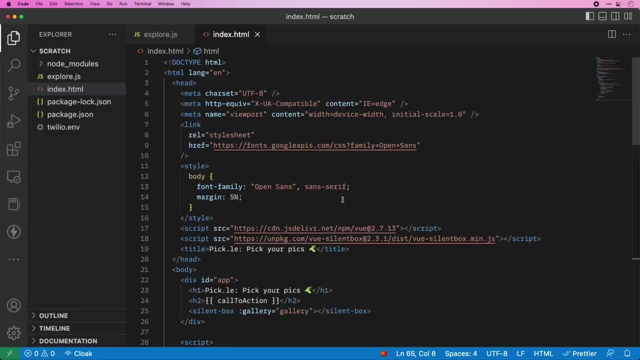 They might say, hey, I've got this template and I would love for you to be able to set it up to make the API work. So the first thing to do if you want to look at an index file locally on your computer. 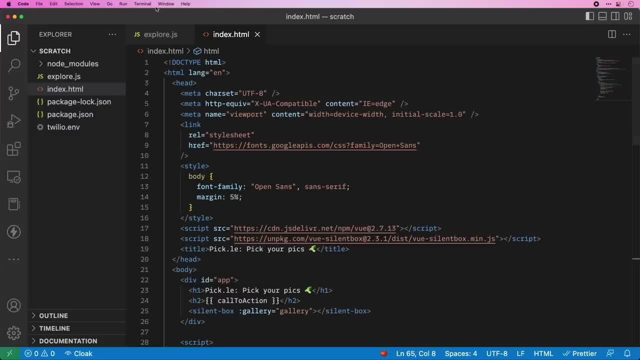 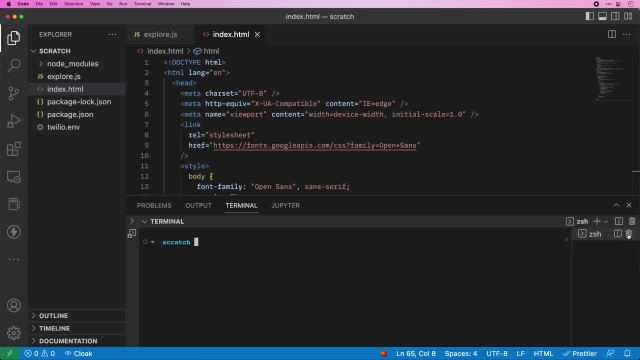 you could set up a web server. I've made it so we don't need to have a web server, So we can just go ahead. I'm going to go to my terminal. I'm going to do a new terminal here. I'm going to open that up. 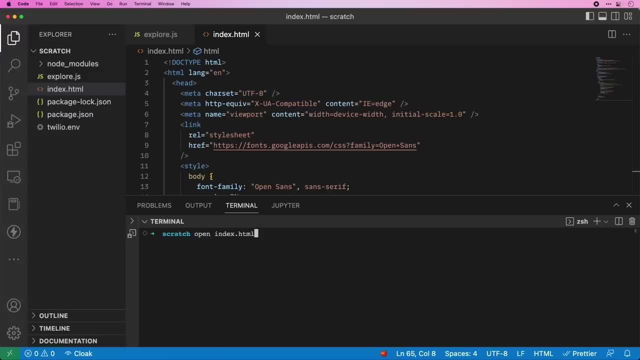 And I'm going to say- I'm just going to say- openindexhtml. Now, what that's going to do in my Mac is going to open this up For Windows. take a look and see how to do this exactly. But what this will do, it will update my pickle here. 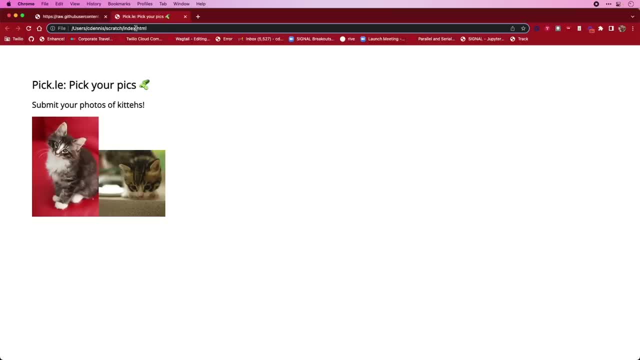 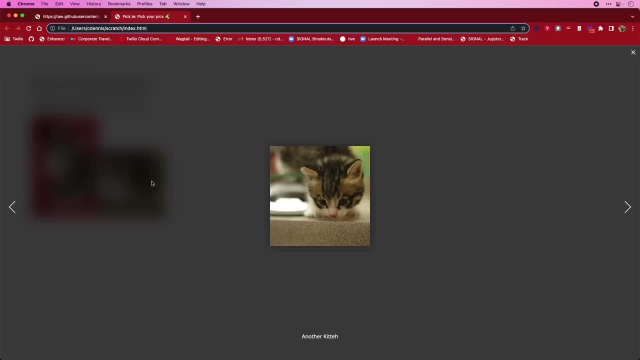 So you can see, this is this user scratch, And then, whatever it is, it's in my directory there And this is what's happening. There's some nice kiddie photos there. I'll show you how that's working And if you click into one of them you get a nice little gallery here. 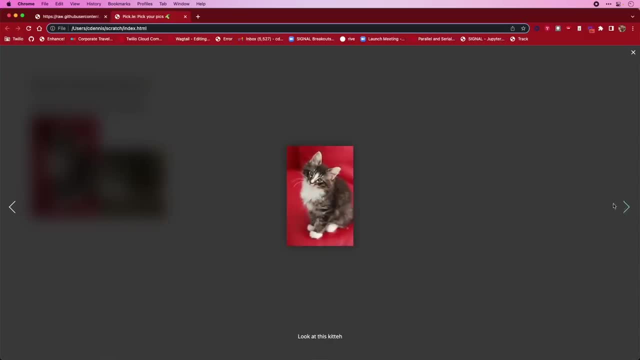 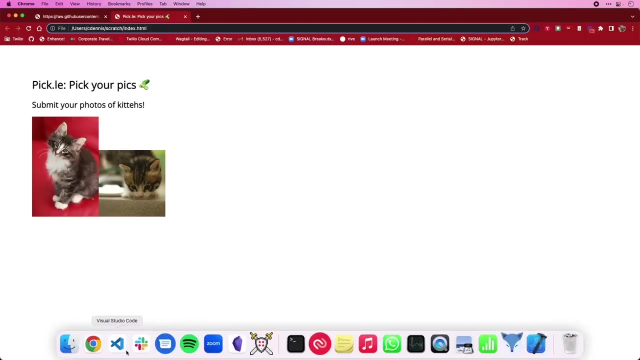 And you can switch between the different kiddies And you can see the text that the user submitted. That's kind of where we're going with this. That's what we're planning on doing. Very nice setup, Simple, one little pager application. 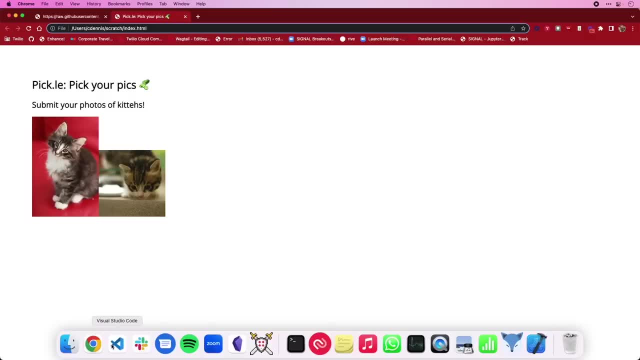 Because I'm using some APIs to be able to do that here locally. I'm using remember APIs, not web APIs, but I'm using Vue as the framework that I'm using. I'm using a framework called Vue And it has an API. 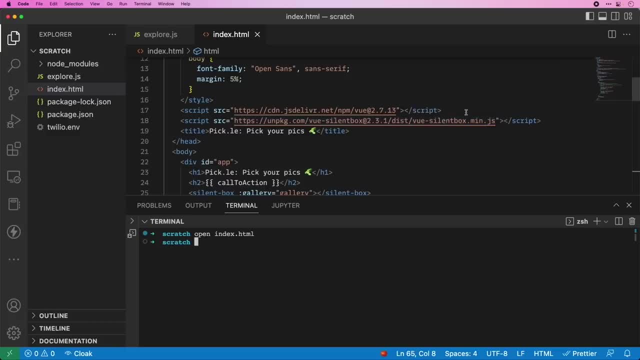 And I'm also using this site. It has silent box, which is allowing us to do that pop-up. It also has an API. Let's take a little bit of a look here. So I'm going to move a little bit slow through this. 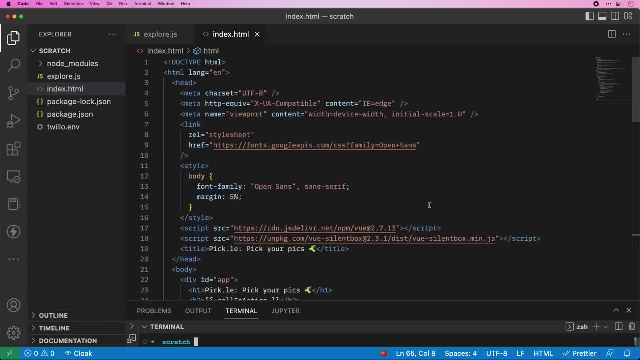 just so in case it's your first time seeing something like this. I've got some setup here. in this head tag You can see this HTML. This is the head tag. There's some setup, So I'm using Vue And I'm also using silent box. 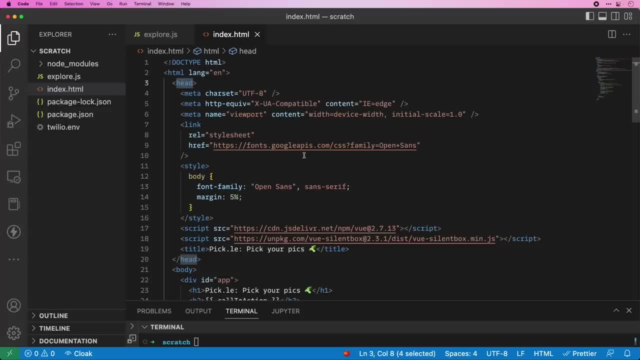 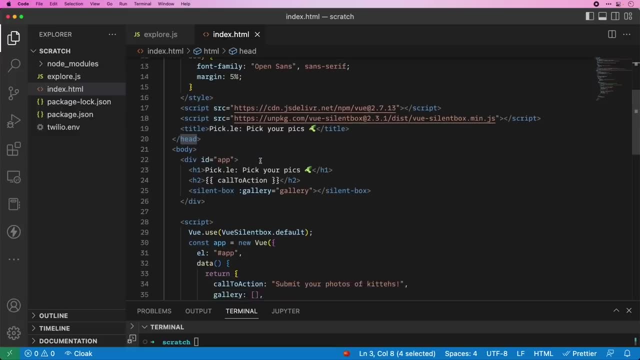 And I've got some very minimal styling. It's not my forte And oftentimes you're given a template Like this So you're given: hey, here's a working thing. I would love for you to get some APIs in there. 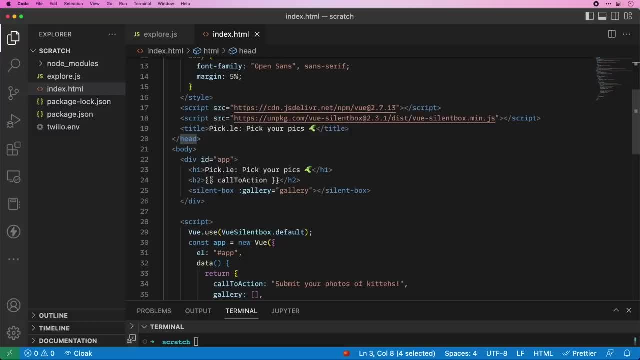 So the body of the app has this. You'll notice this little mustache, mustache And it says call to action. So in Vue- this is part of their API- is if you use this for a template, it will be replaced with something from the Vue object's data. 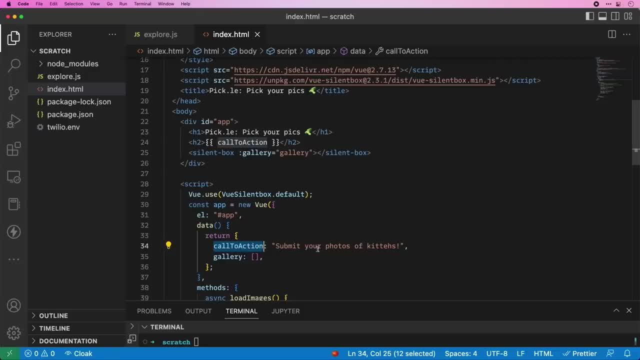 So you can see, here there's this call to action And that's what this is, And this is why I could change this and make this say whatever I wanted to say, it would be here. So whatever we decide to do with our apps, whatever kind of 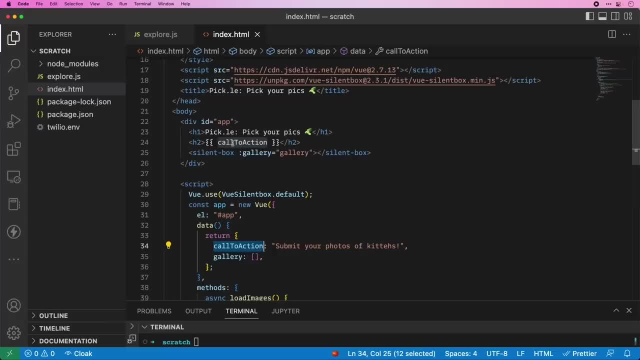 picks that we're trying to collect. that would be where we would change that. And then you'll also see: here there's this silent box and it's doing a gallery And the way that that works is we pass in this gallery from again, from this Vue objects gallery. 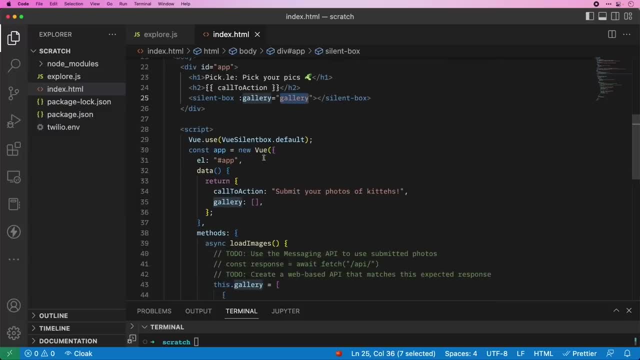 You don't necessarily need to worry too much about this, but I wanted to show you that there is. this is how Vue works. It's a front end framework and it provides an API where, if I give it a function called data and whatever's in here will get returned to it. 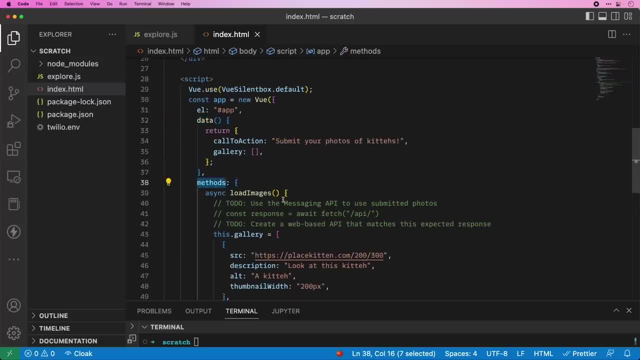 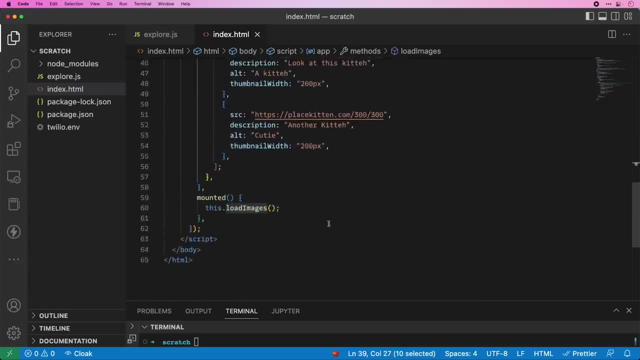 And then there's some more. I can define some methods on the Vue object. One of those methods that I've defined is called load images. Part of the API that Vue creates is there is a lifecycle method called mounted, which means that when the application is ready, 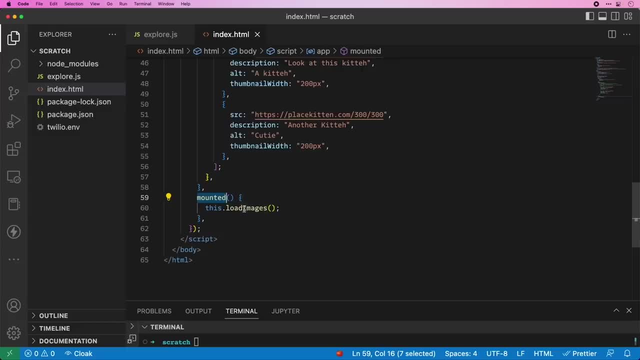 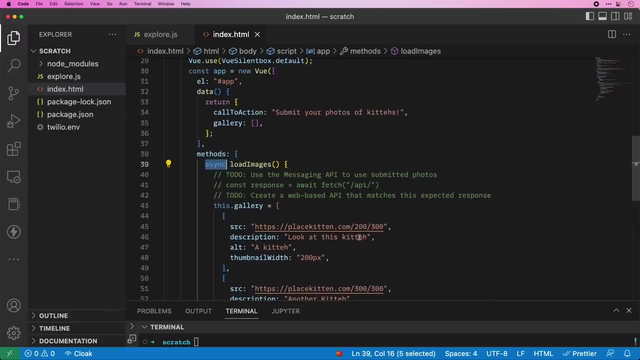 and it has been mounted onto your HTML through the JavaScript it will call this function. So it's going to call this load images function And this load images function. you'll notice it's an async image And I've got some to do's in here. 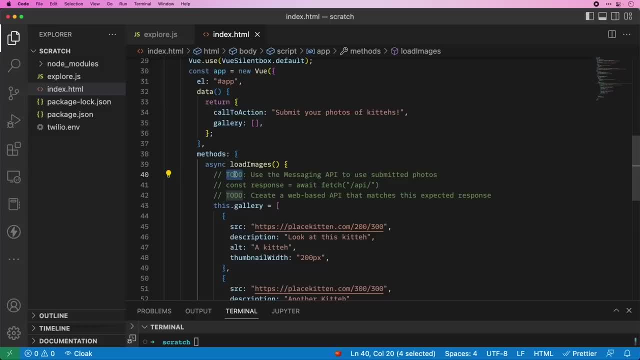 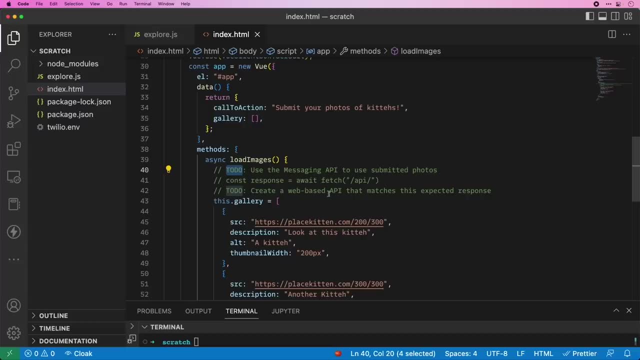 This is someplace where you might be communicating back and forth with people as you're working together on a project. So use the messaging API to use submitted photos and also create a web-based API that matches this expected response. So that's what we're going to do. 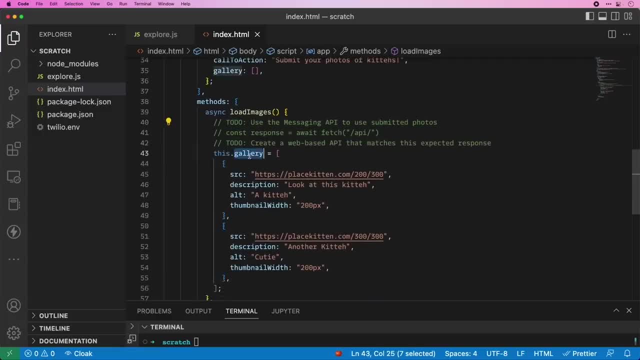 over the next couple of videos here. So what we see in the start here is there's this gallery and it is an array and it's got some stuff from this. There's a website called place kitten that I used here So you can get different versions of kit kitties here. 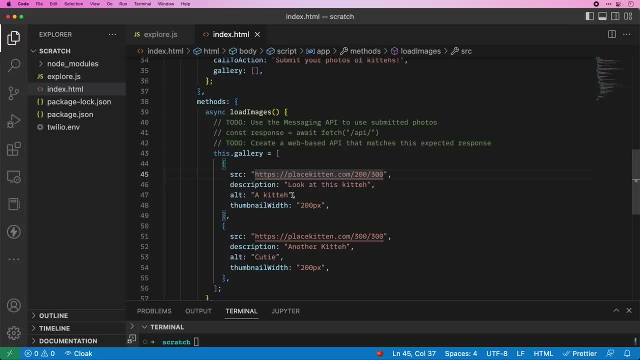 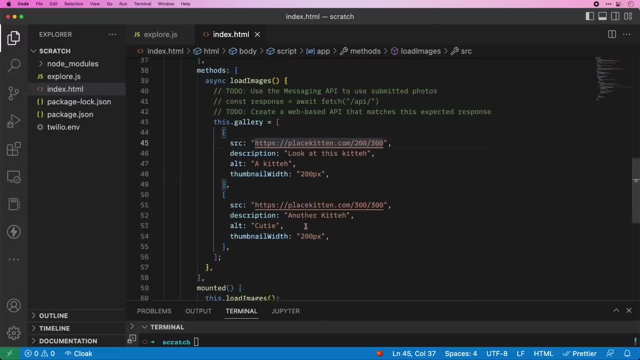 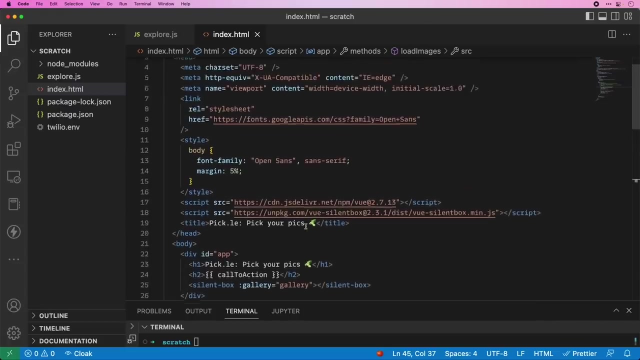 And there's a description and there's an alt tag, which is important because, for accessibility reasons, this is what it will say on the picture. So that is what is happening to be able to make that work. So we now have our app here locally and we can change things. 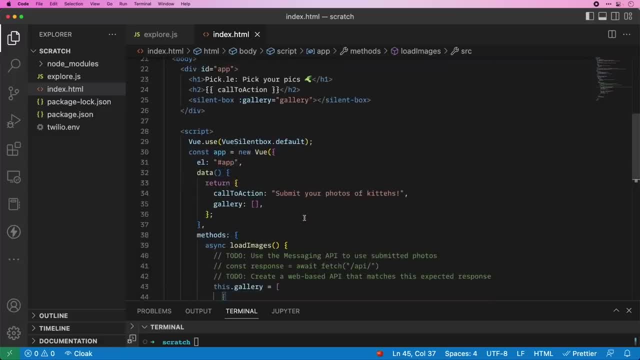 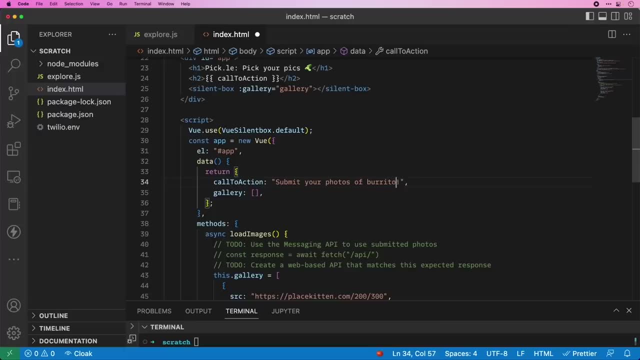 So one of the things, one of the photos that I want to do, I love to get photos of burritos from around town, So I'm going to change this. I'm gonna say, submit me a photo of your burritos and I'm going to save that file. 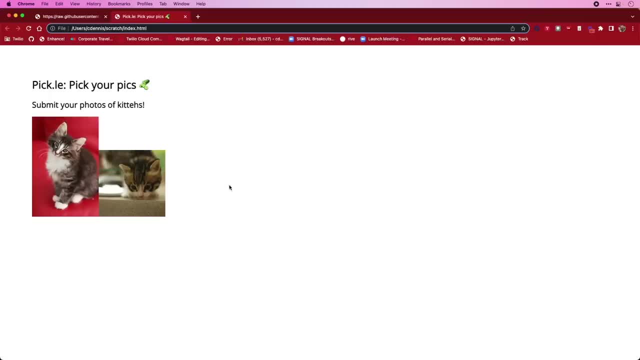 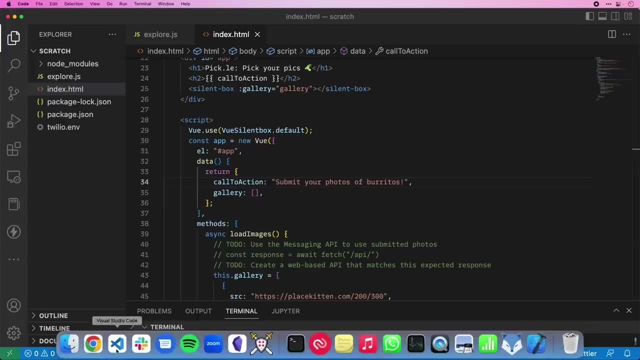 So see, it's not saved. I'm going to save it When I go back to my file there, when I refresh it, you can see that it says burritos. What are you going to want to gather? Why don't you go ahead and change that? 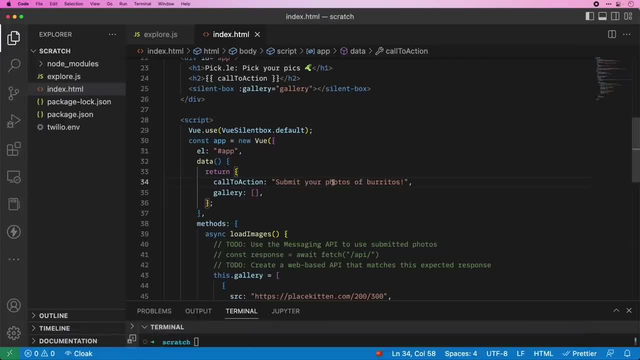 change that to whatever it is that you're wanting to gather as we build this project through, And, of course, you know, you see that you can change that, however, so make sure that it's downloaded and make sure that you can change that. 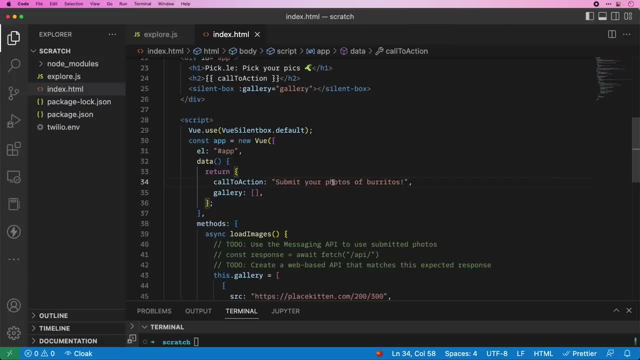 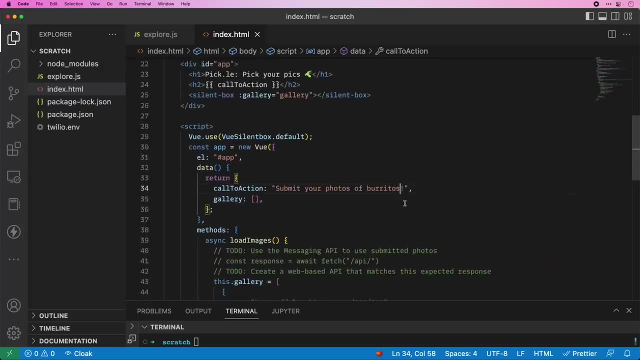 that you can change this file and it opens locally on your machine. Cool, And so now we have a little smattering of APIs here already. So we have a web, we have HTML working here, We have this view, and this view API has a very specific API. 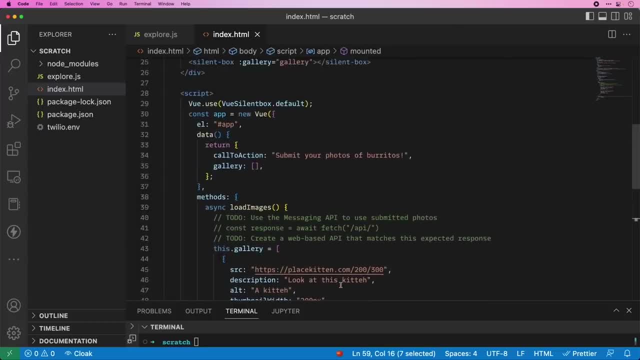 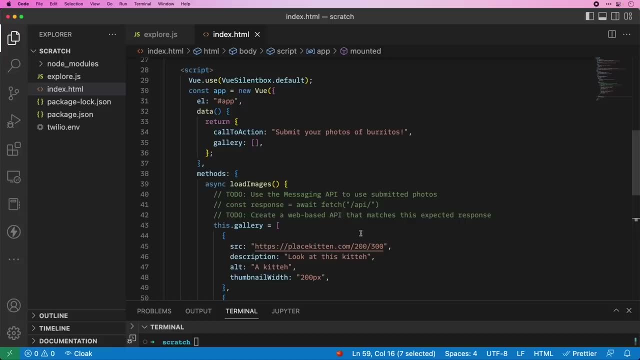 that's doing this mounted here, but remember, it is actually an API and we're going to use a web-based API to be able to to get this information, And we're going to do that here in just a bit. Now that we got our file all working, let's deploy it. 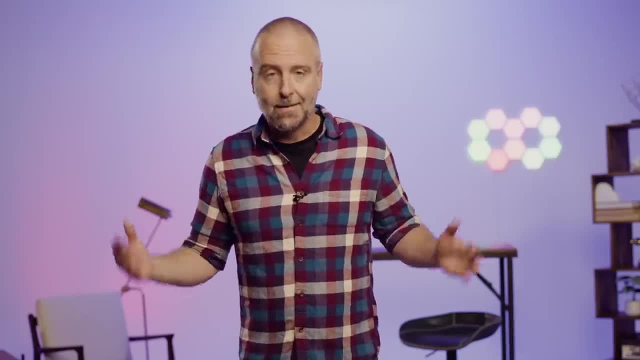 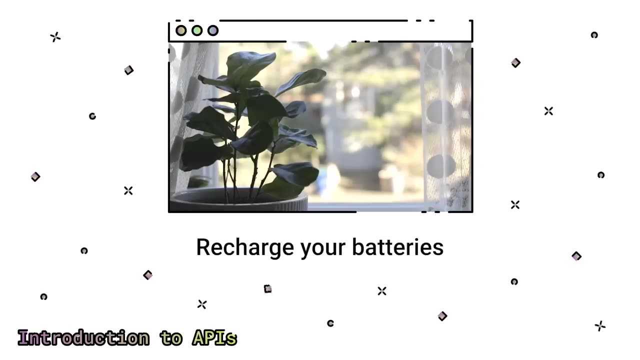 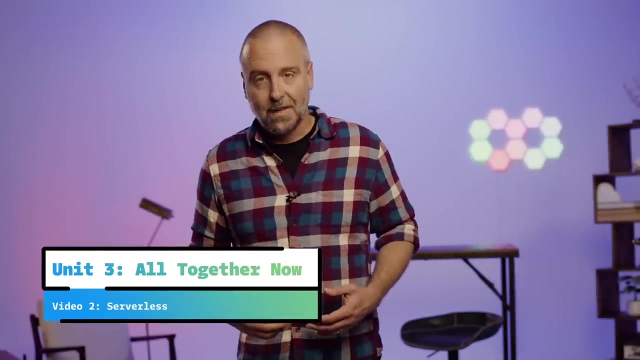 And by that I mean: let's get it up on the public internet so everyone can see it. That is, of course, after you take a quick break. We're going to get our webpage up on the internet so others can see it. 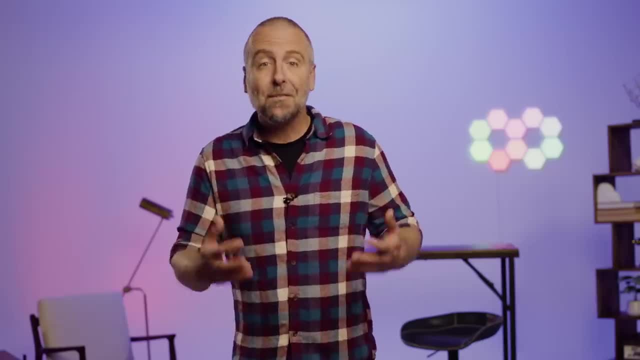 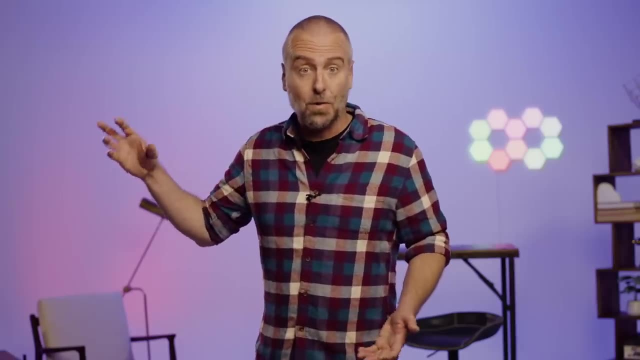 And this has gotten much easier as time has progressed. You used to have to set up a server like a physical computer, buy a domain name and configure it to point to your machine. You had to figure out where to host, like where to locate your server so that it was always on. And arguably the hardest part, after it was live. you used to have to watch over it in case too many people came to it. You didn't want it to get overloaded. You wanted it to scale up and be able to handle the traffic. Those servers are still around. 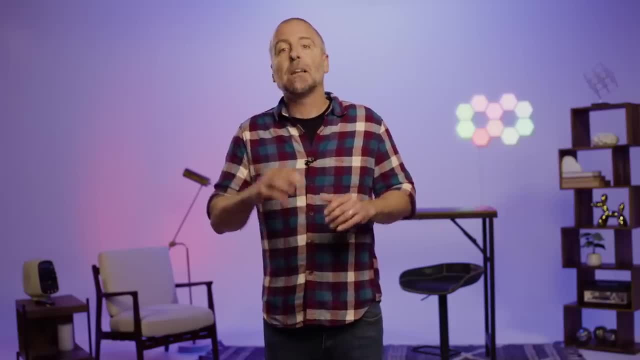 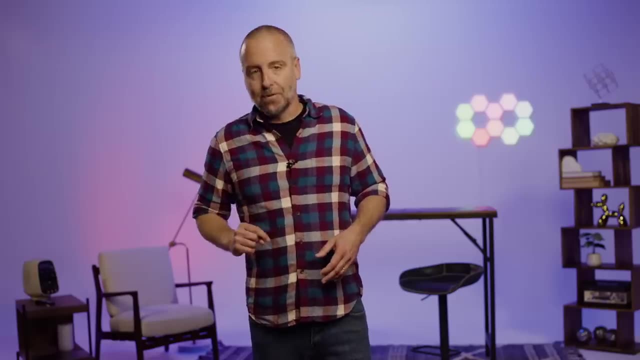 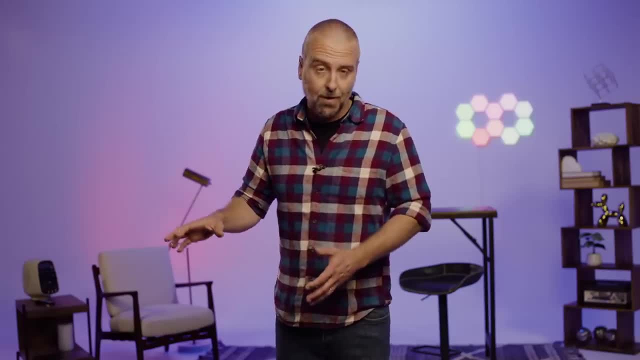 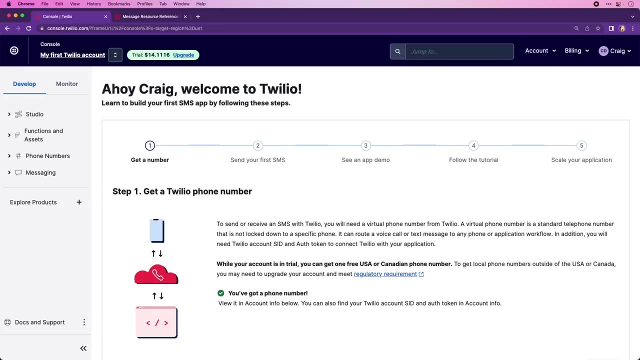 it removes all those previous things that we had to worry about and it offloads your concerns. I can tell by the look on your face that it's probably better if I just show you: let's get this application hosted. So we're going to have Twilio host our code for us. 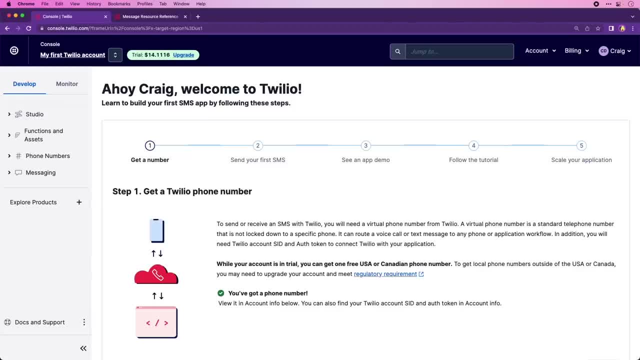 And that is to say we are going to have Twilio be our web server that will be used to serve our HTML. Our project will be serverless. Now, the way you do that is by using Twilio serverless environment, which is here under functions and assets. 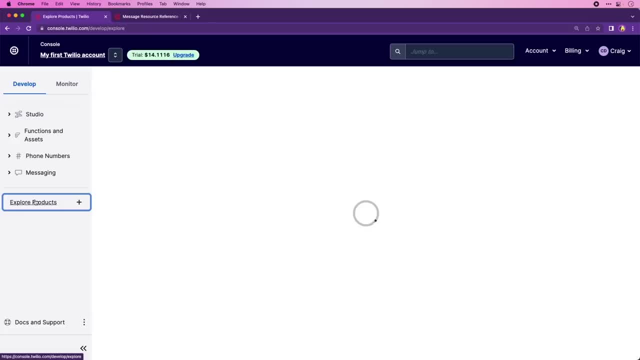 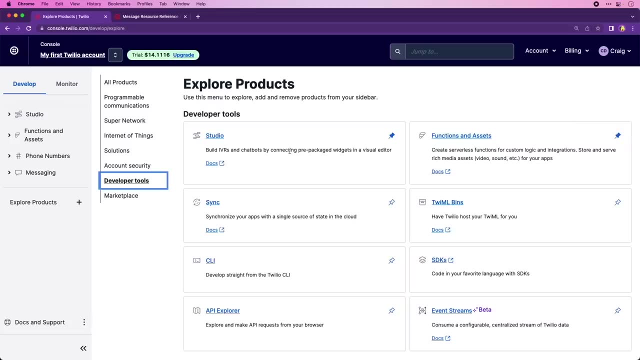 I'm going to select this Now if you don't have that here. if you click explore products and you come to developer tools and you come over to functions and assets, you can click this little pin icon and that will make it show up here. 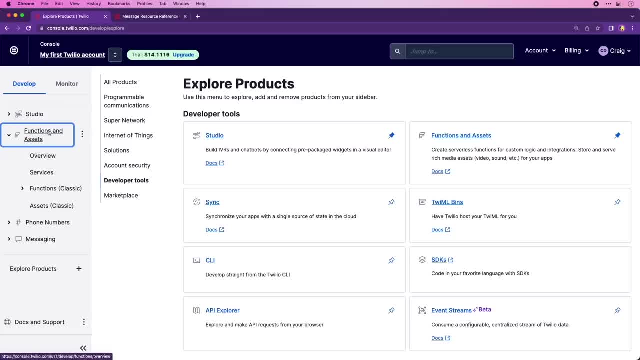 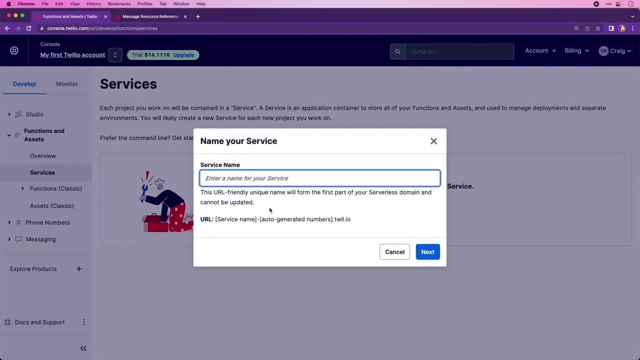 So I am going to create a new service. So I'm going to go functions and assets, services and I'm going to say create service. It could be whatever you want. I'm going to call it pickle like. pick your picks with pickle. Peter services allow us. 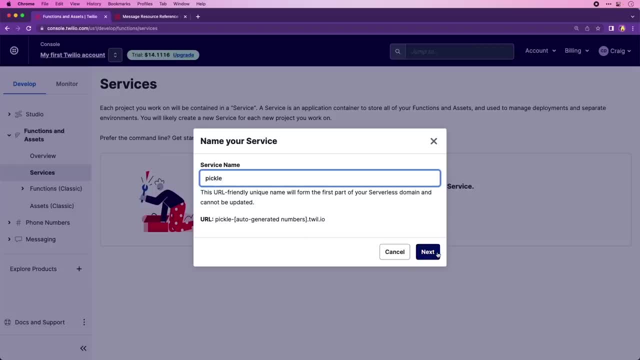 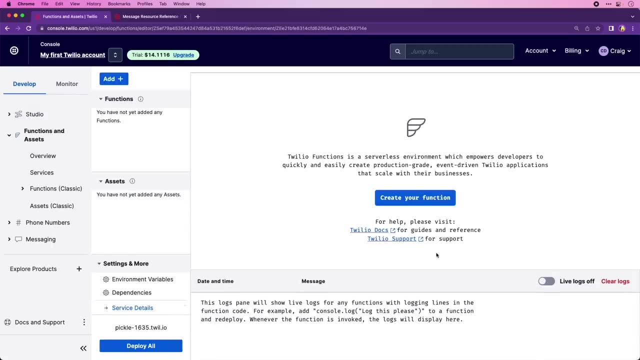 to group our functions and assets together for our application. So I'm going to click next And what's going to happen is we're going to open up to a very nice IDE that will allow us to edit our code. Now a friendly reminder, if you're having a hard time following along, because my screen 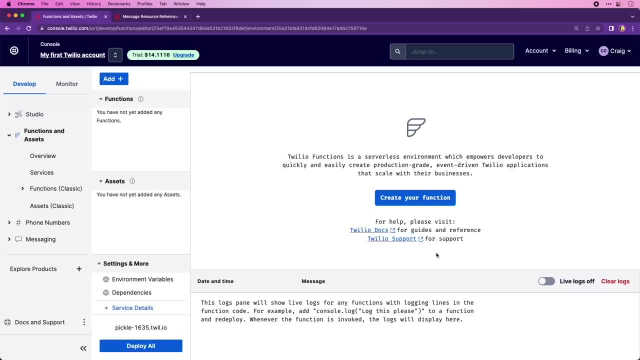 looks different than yours. you are using a new and improved experience, So check the notes for what might be different Now. traditionally, these services here are used to power Twilio based applications. Remember how I said You could respond programmatically to an incoming message. 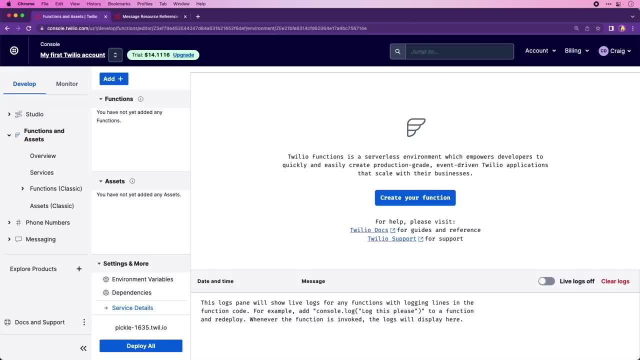 Well, functions are a great way to do just that. In fact, our current number has a default response, and we might as well fix it while we're here. But before we do that, let's get our HTML code up and running. So what I'm going to do is I'm going to grab code from my local machine. 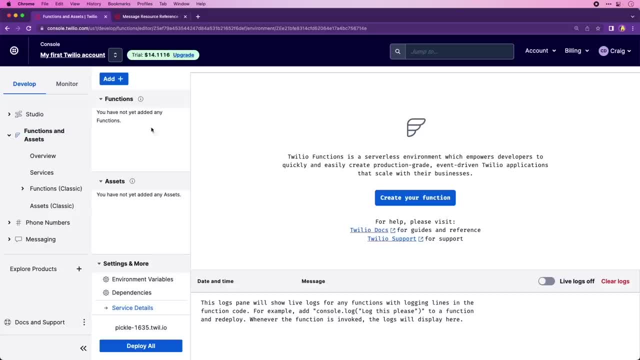 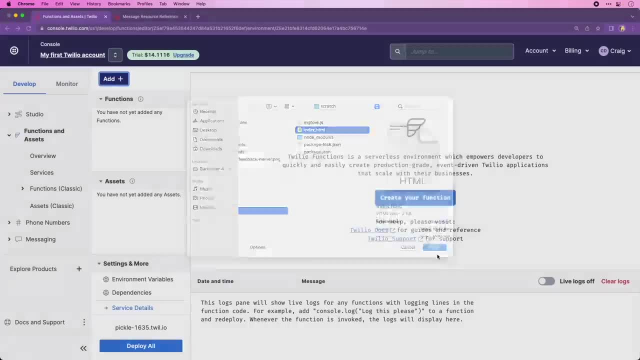 And if you want to, you can just grab it from GitHub. but check the notes for more on that. But I'm going to go add, I'm going to choose upload file, I'm going to find my file, my indexhtml, and I'm going to choose open. 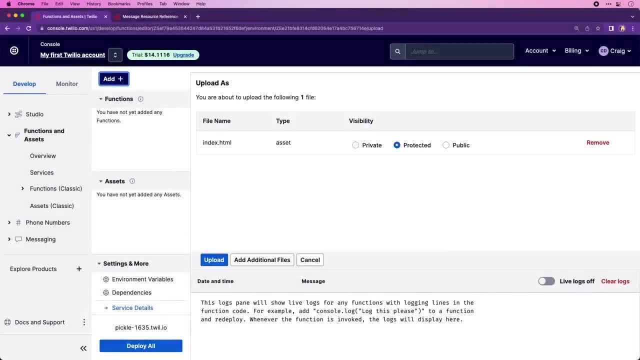 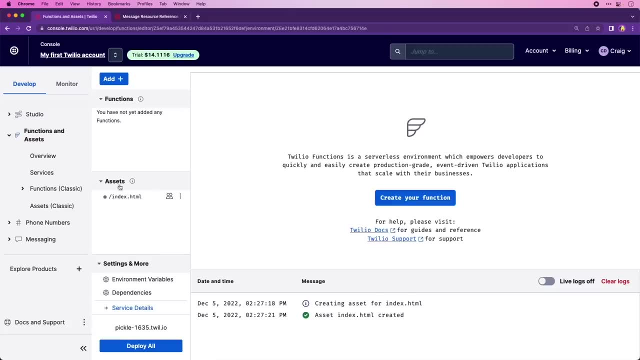 Now what we're uploading. we'd like the world to be able to see it, So I'm going to choose public and then I'm going to choose upload. So now this file's over here, you'll notice this little green dot, and this means that 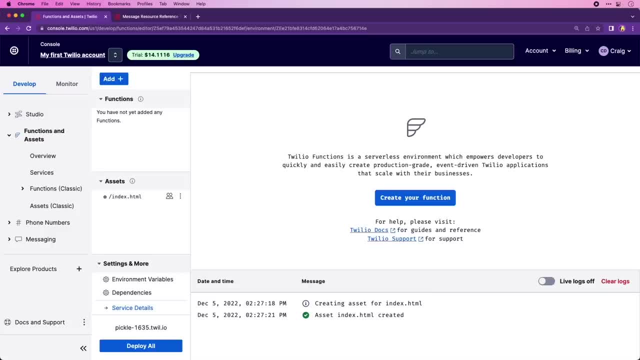 it is not yet deployed, and then that is, it's not yet available on the internet in this current state. So let's do that. I'm gonna do that by clicking this, deploy all button down here. And now we see that it's green and I'm going to go ahead and choose copy URL and I'm going 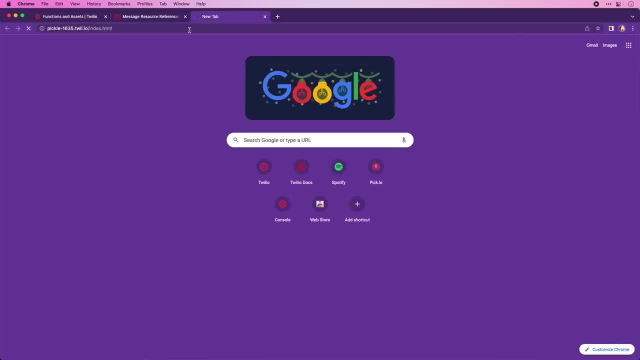 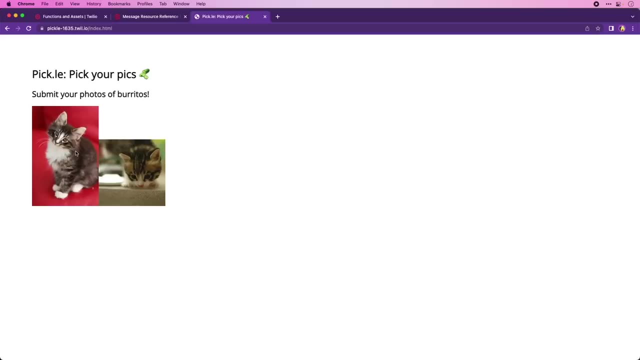 to open up a new tab with that there And we will see that our site is live, except it says burritos and these are kittens. but we're getting there, So, uh, it's working, It's up, It's on the internet. 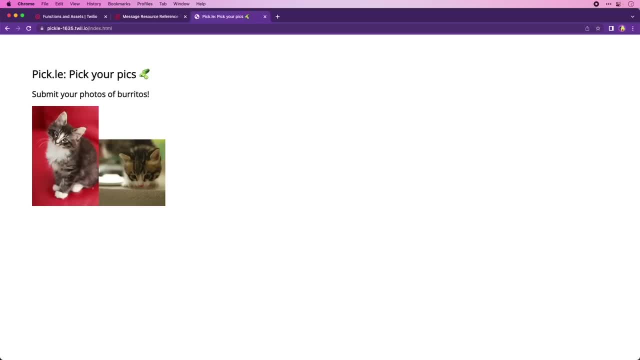 I could share this with people. The pickle site is up and running on Twilio's servers. One of the things that I used to have to worry about was scale Like what. There's a whole bunch of requests to the site. Would it fall over? 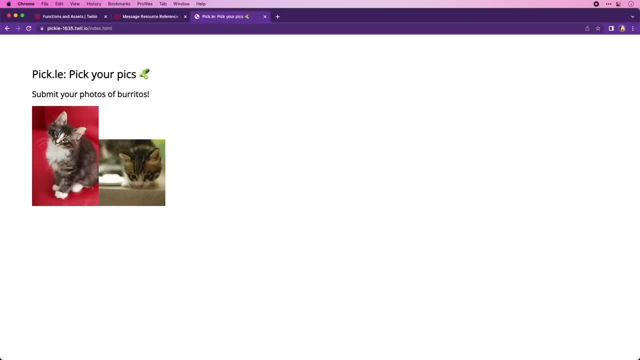 What the serverless solution is doing is allowing me to not need to worry about any of that anymore. Twilio is handling all those concerns for me, which is great because now I can focus on what I was building, which, by the way, we need to handle that reply programmatically. 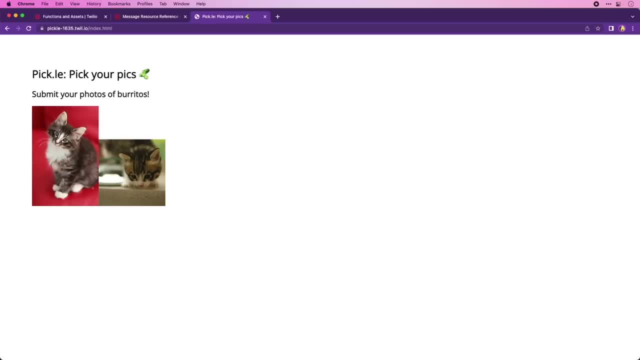 right. So the way that Twilio does things is with web hooks. Now, if you haven't encountered web hooks before, I have an entire course on them that I linked to in the notes. Web hooks are sometimes called a reverse API. That is, instead of you calling the API, the API calls you. 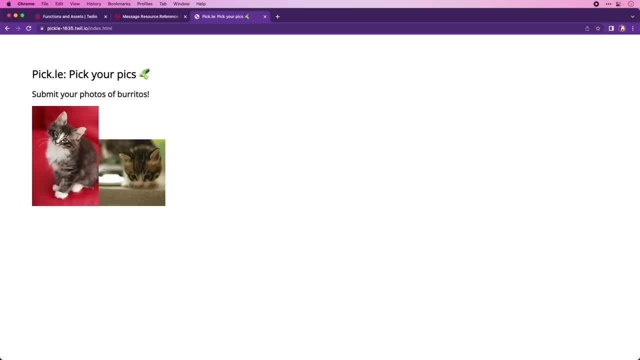 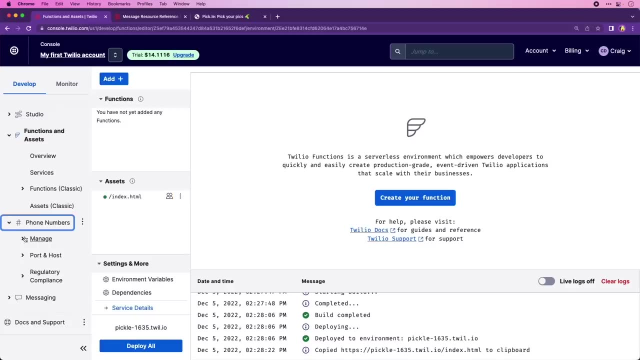 So let's configure our number to make use of the right web hook. So I'm going to go back to my number, uh over here. If I look under phone numbers- and I do manage, I'm going to hold down a command or control. 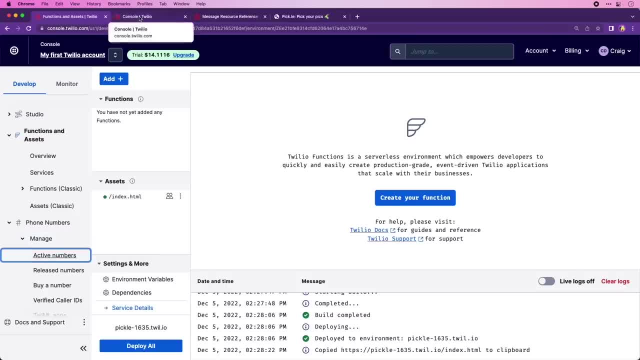 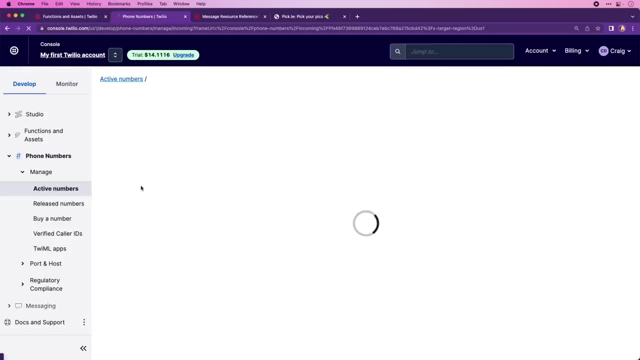 and click active numbers, I'll open up a new tab. nice little hack to keep your screen open here. Uh, so I've got my numbers here and if I come in here to configure it, What happens is I'm going to scroll down. 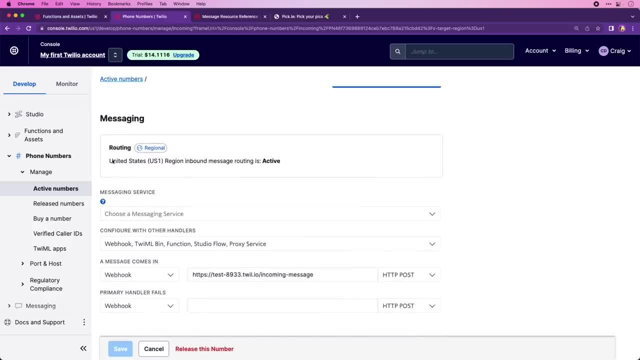 So here's the voice section and then here's the messaging section and it says: when a message comes in to this web hook and it sends to this URL here, does a post to this URL here. So the way that Twilio makes use of web hooks can be thought of like this. 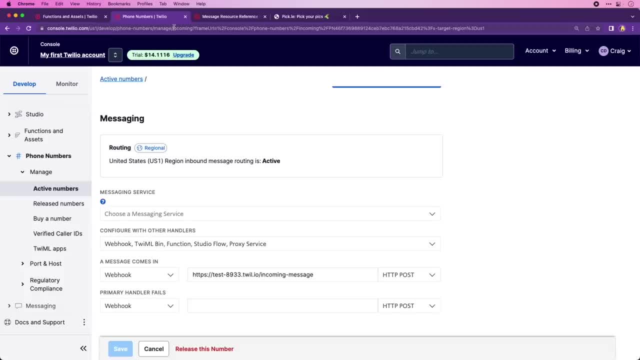 You know, when I hit this URL- right this URL- in my browser, my browser doesn't care about what's happening At that end point. it could have been anything, any web server, like express, Django or Java server, It doesn't matter. 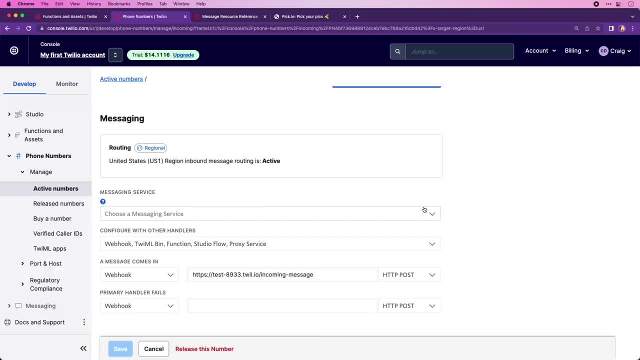 What matters is that what was returned from my server was HTML or hypertext markup language. My server responds with HTML and my browser renders the page. Now, the same is true with Twilio. Someone is going to text our Twilio number and Twilio is going to send a request to an. 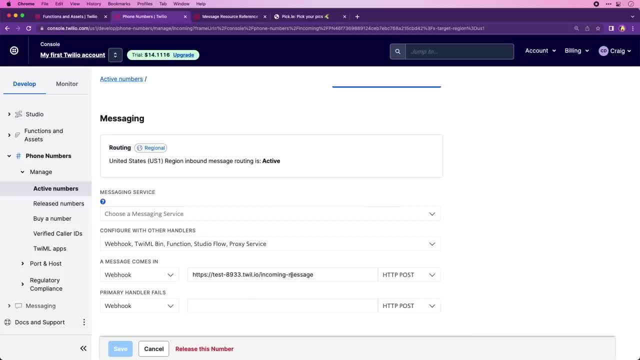 end point, In this case this end point. here it doesn't matter What is happening on the other side, as long as it returns Twiml or Twilio markup language. they look very similar: HTML and Twiml Twilio will be able to render your application. 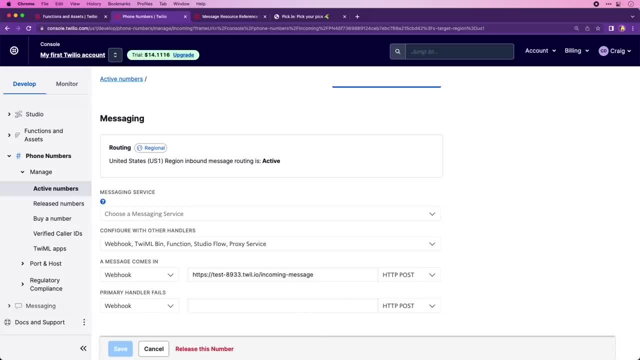 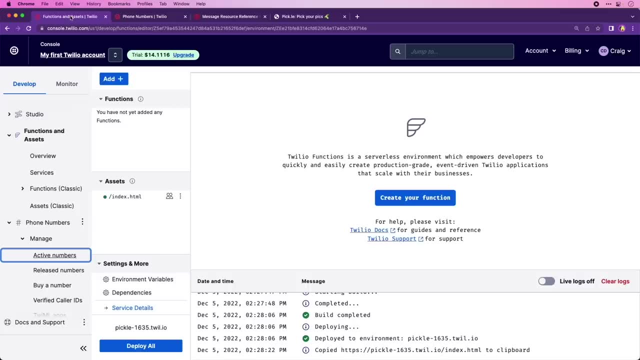 So we could set up a new web server to host this application that returns Twiml, or we could just use a Twilio function, And, like I said earlier, that is what these are commonly used for. So let's let's pop back to our service. 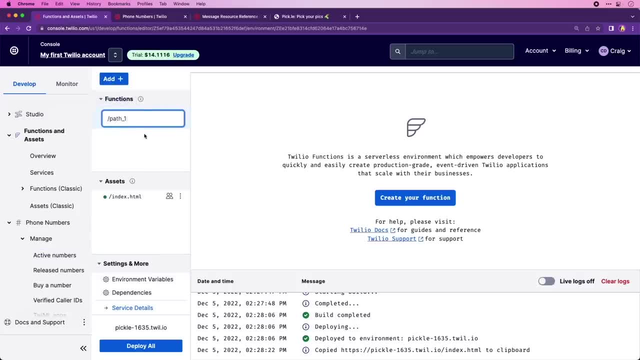 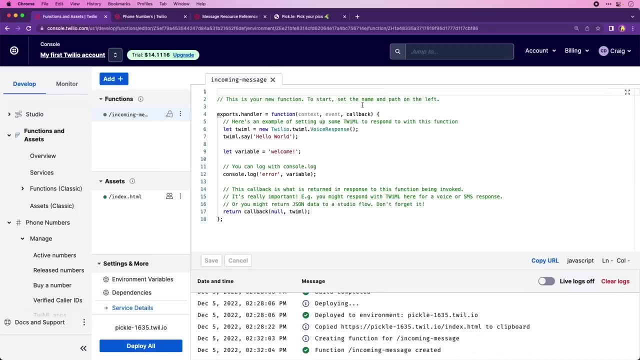 So I'm going to come here, I'm going to add a new function And I'm going to name this function incoming message. That's what we're going to do. We're going to handle an incoming message And there is some very nice default boilerplate that is commented, that comes through. 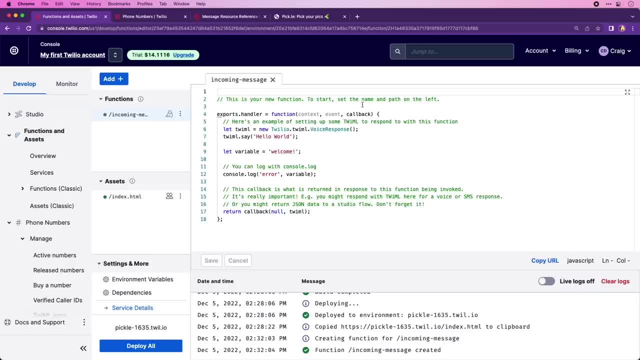 So boilerplate is code that's provided. That's usually the most common thing that you're going to be doing, And in this case it is. it's boilerplate for how to respond to an incoming phone call. It's kind of like the hello world of 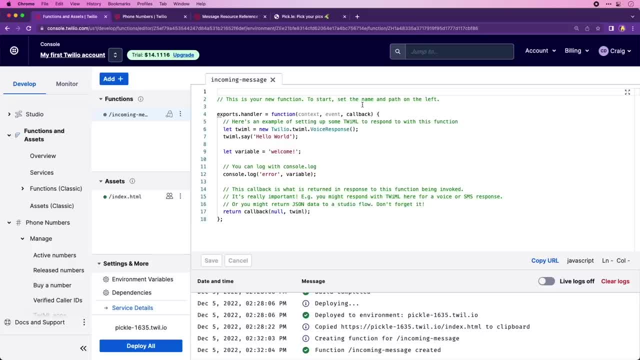 Uh, voice applications, but we're going to be building a messaging application, So we'll need to tweak this just a bit. Now I've put this code, I'm about to show you into the notes, So I don't want you to feel like you have to type this all out, or even fully understand. 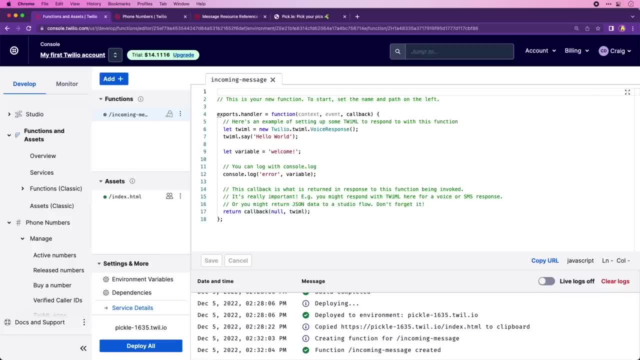 every line. I will step you through it. first, though, Let me walk you through this function just a bit. So Twilio functions all export a, a thing called a handler, and that handler takes a function that takes some parameters: context, events and callback. 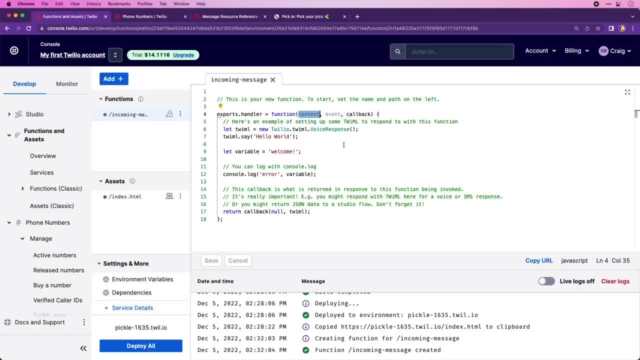 So context here is an object that holds information about the function that's running Like. it knows the domain, It knows the name of the function and the event. here You can kind of think of this like a web request in in most frameworks. 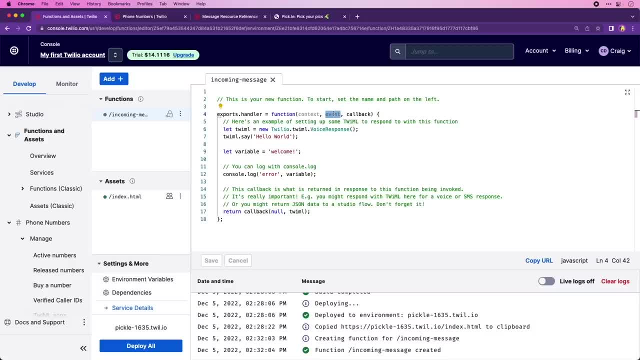 And if you haven't seen a framework before, this is kind of the way that information is passed into your web application. Uh, so, so this is the event will hold everything about the text message that was incoming, because that's what Twilio does. 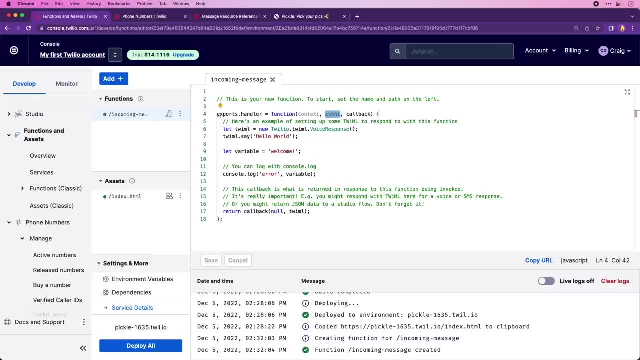 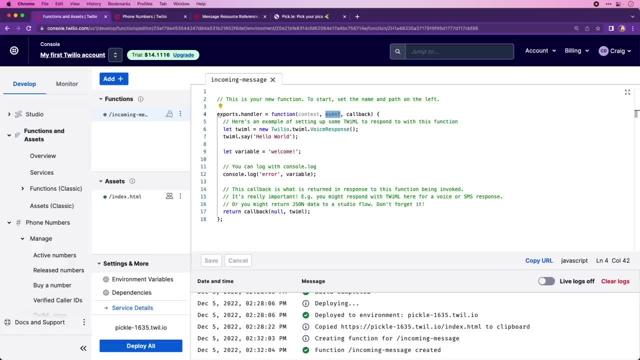 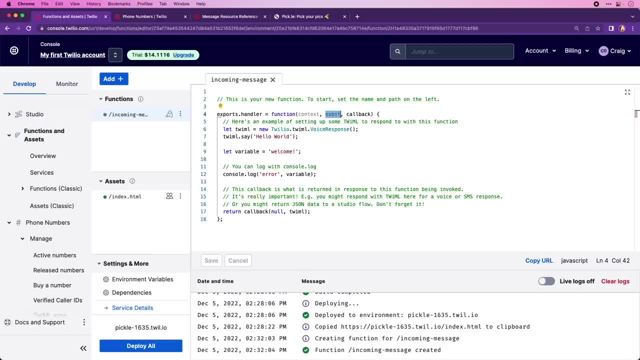 to this function. So Twilio will post the information here. It will call our function instead of us writing code, that checks if a new message was added over and over again. Twilio is going to call us. The API is going to call us via a webhook. 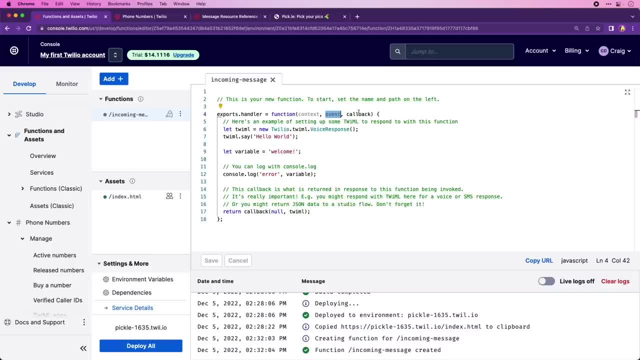 Webhooks are pretty cool. Uh, check the notes. And then, finally, there's this callback object here, which is how we send information out of the function. It's actually a function, So we have this callback. This is the errors that might've happened. 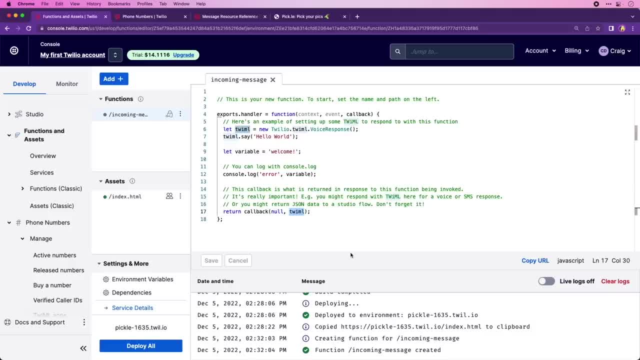 And then this is what gets returned. And here's that TwiML, Twilio markup language. So I'm gonna get rid of a couple of these lines here. These are sort of demo lines. I'm gonna get rid of that And I want you to be able to see. 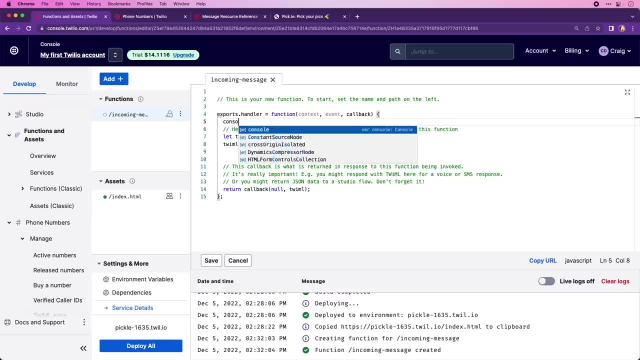 what's coming into the message. So I'm gonna start up here, I'm gonna do a consolelog And what this does is when the function runs. if we want to, we can see the message that will show up down here. So let's say that we got an incoming message. 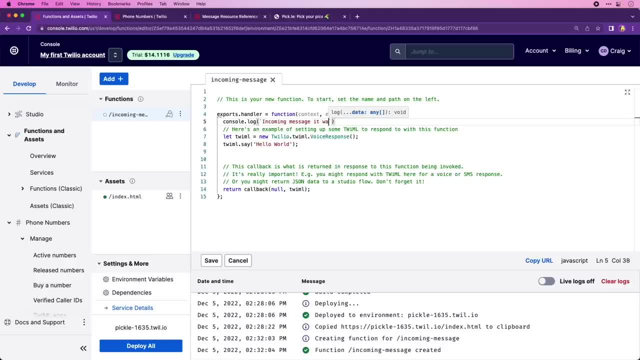 and it was incoming message and we'll just do a colon And then I'm gonna use this dollar, this style of a string interpolation. So I have the event object and on it there is a property called body with a capital B. So that's being passed in there. 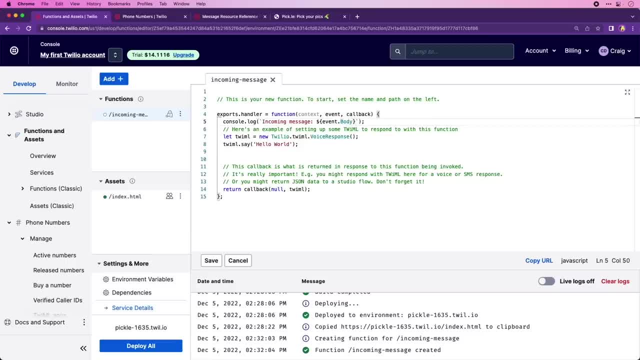 So when the function runs we will see that the message came in, because Twilio is gonna pass that message and we'll see it there And we're just gonna say thanks when somebody sends us in. So we don't really need to do anything with this message. 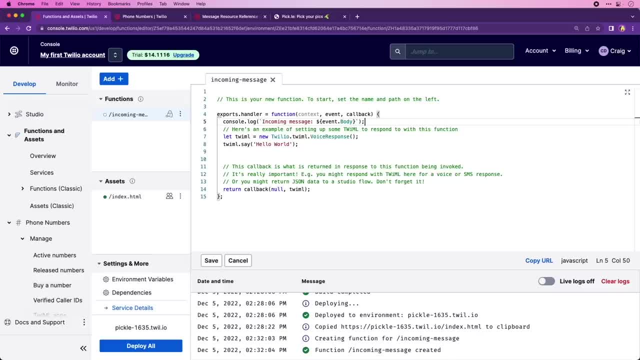 but you might want to filter it or handle things differently based on what they said in the message, And you totally could do that. But you'd probably also want to check the photo that came in and was actually a burrito or something not in a probes. 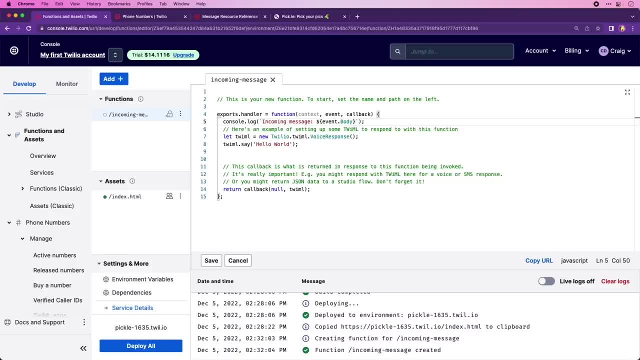 You could do that, And there are APIs for that, but that's a little out of scope. So, instead of a voice response, we're actually going to return a messaging response, and there's a little helper library here, right? So a little helper library for TwiML. 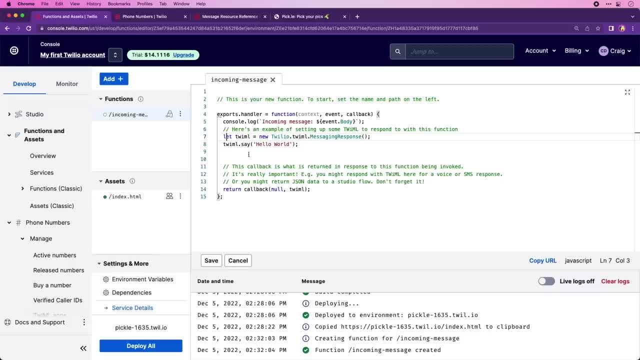 and it has this TwiML object And, before it was doing, say which is text to speech. So if you wired this up it would say hello world. And like a computery but actually pretty good sounding voice these days. 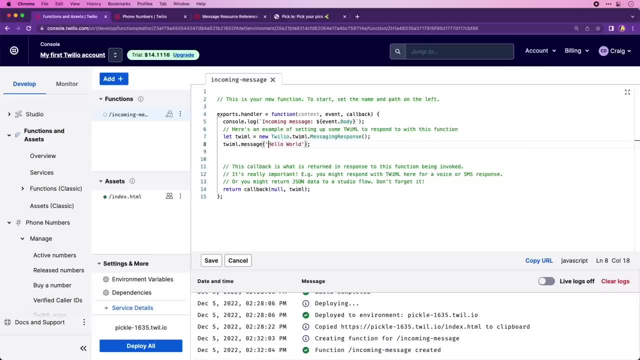 But I'm gonna change this to be a message, because that's what we want to return. We want to return a message and we want to say thanks for your submission. right, We want to want to thank them there And we can also send any sort of emoji here. 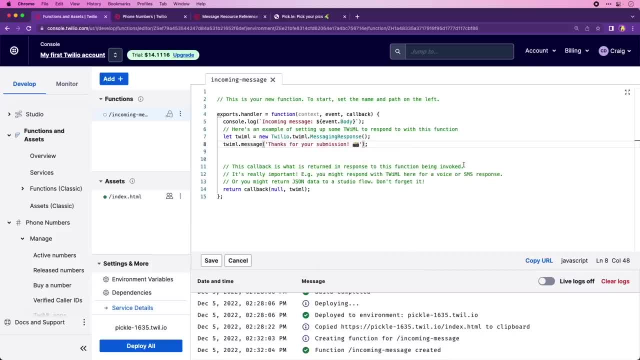 Let's see if maybe that sounds. yeah, that's nice. Thanks for your submission. And so what's happening here is this object. it's a fluid API, It means that it doesn't return anything. You kind of tweak it and it builds as things go on it. 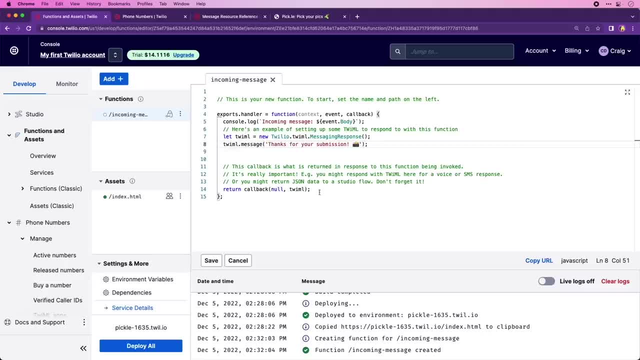 So you'll notice that this isn't returning anything. I'm modifying this object And then, when I send it out, at the end, that's how it goes out. So let me- let's just let me- show you what that object looks like. 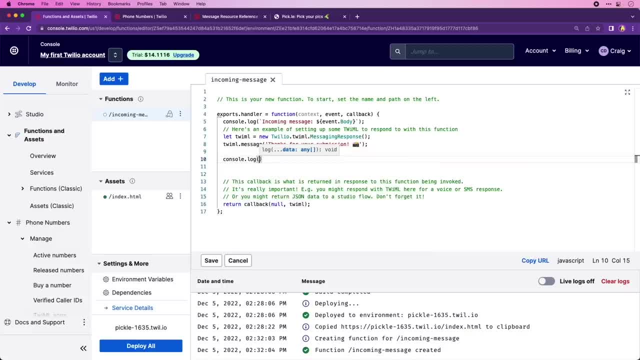 So again, I'll do one of these Consolelog and use the back tick and we'll say TwiML. So Twilio markup language was TwiML And you'll see that it looks a lot like HTML. There are some rules to it. 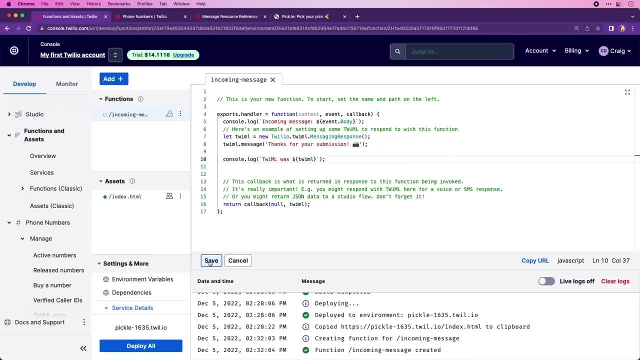 but we don't need to learn them all right now, So I'm gonna save this And, just like before, you'll notice that this is gray. It hasn't been deployed. So I'm gonna click deploy all, And while that's building, 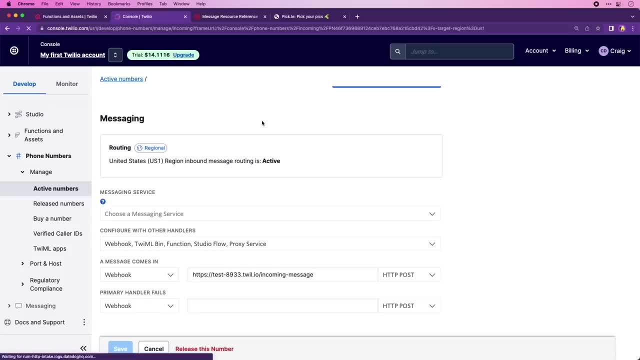 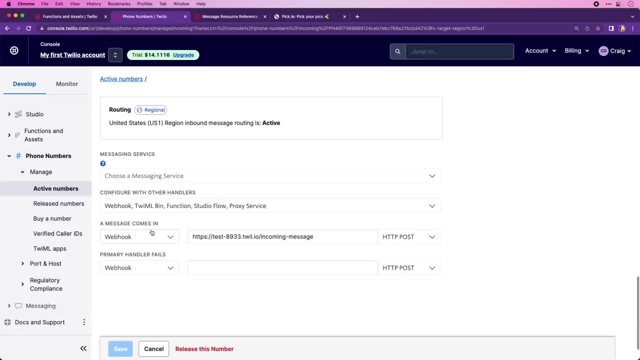 I'm gonna head back to my phone number page and I'm gonna refresh it. So on my phone number page I need to change my message down here. It says when a when a message comes in. we want it to be a function that is in the pickle service. 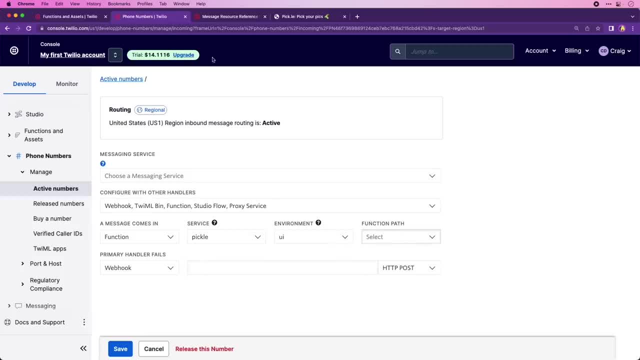 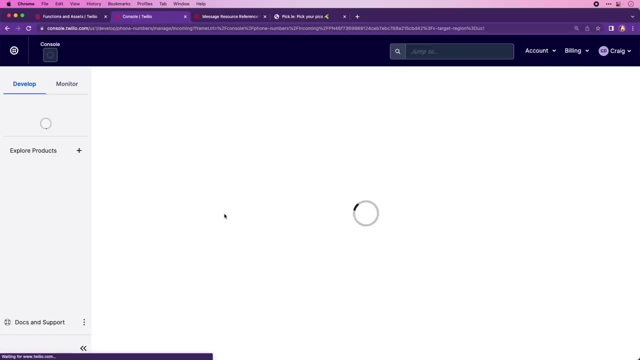 that's done in the UI And we wanna choose incoming message which it hasn't finished deploying yet, Just finished deploying One more time. let me refresh that page So that shows up for us We're going to go to when a message comes in. 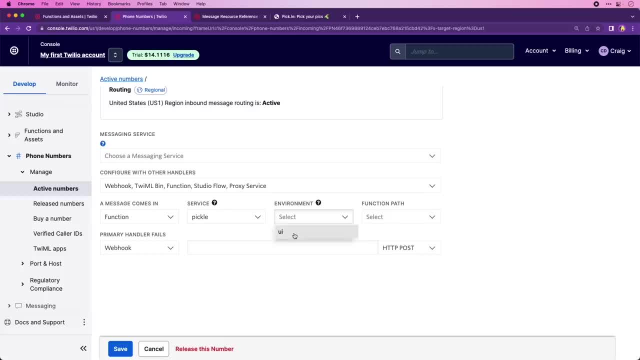 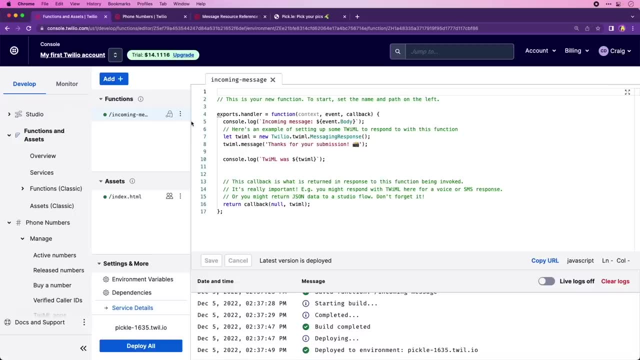 it's going to be a function And it's on the pickle service for this UI And we wanna do incoming message And if we do save, all right, So we should be all wired up. I'm gonna click clear logs here and I'm gonna turn live logs on. 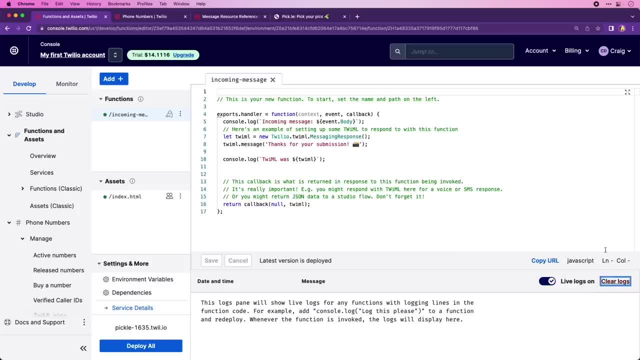 You can see that this says live logs on. when it's ready, I'm gonna clear the logs one more time And what I'm gonna do now is I'm going to send a message in And we should see this. We should see what I send in. 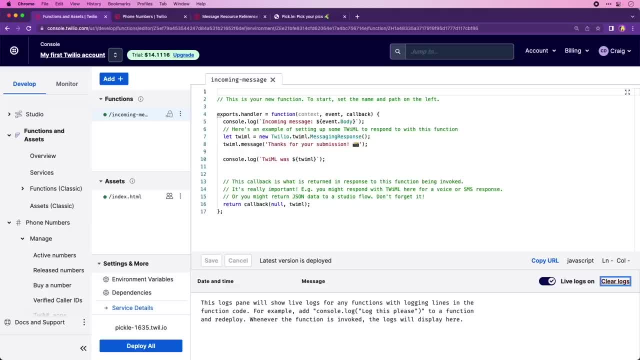 And we should see the TwiML that was sent back And we should get a response back. So let me send that message here, Let me send this text, All right. so, oh, check out this. I have this beautiful picture of a burrito. 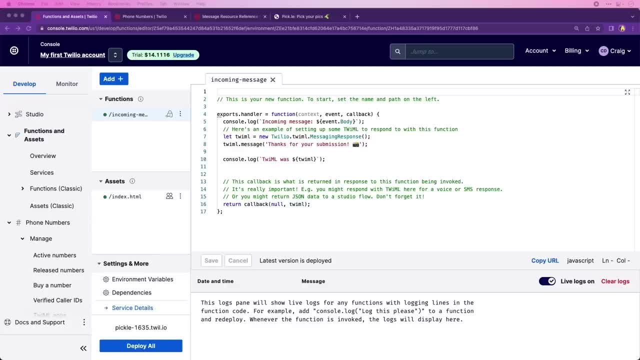 I love when burritos can stand up by themselves, And this is an awesome one. I'm gonna send this in. So check out this beautiful burrito little emoji. I'm gonna send that through And we should see here in the live logs. 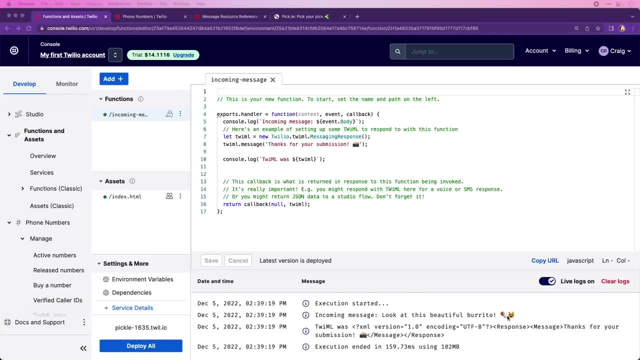 we should see the message come through. There we go. So look at this beautiful burrito. And this is the TwiML that was generated. So, as you can see, it's like 10 times faster. It's like a tag base. 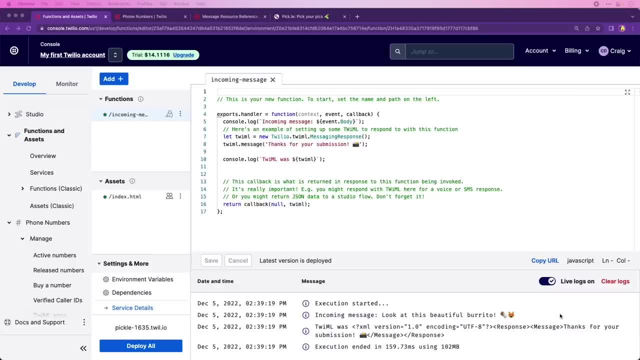 So there's a response and there's a closing response, And there's an opening message and a closing message. Thanks for your submission. I don't want you to feel like you need to learn TwiML. You could do that later if you need to, but this works. 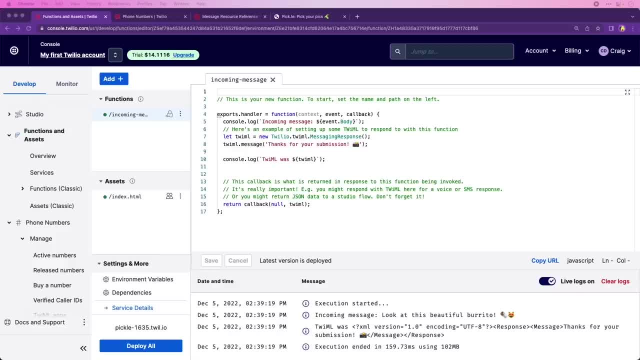 So I got my message back. Now, remember, since we are in trial mode, if somebody else sends in a message to your phone number, they're only gonna get a message back if they're a verified sender. So that is a limit of the trial API. 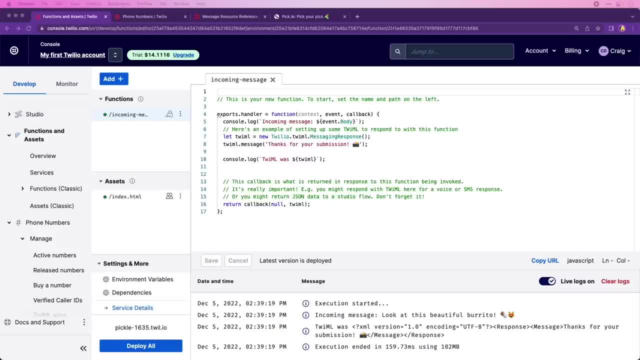 that we're using currently. Now, most APIs have limits. There's only so many calls you can make. There's you can only send to verified numbers. There's just different sort of limits, And that's what we're working with here right now. 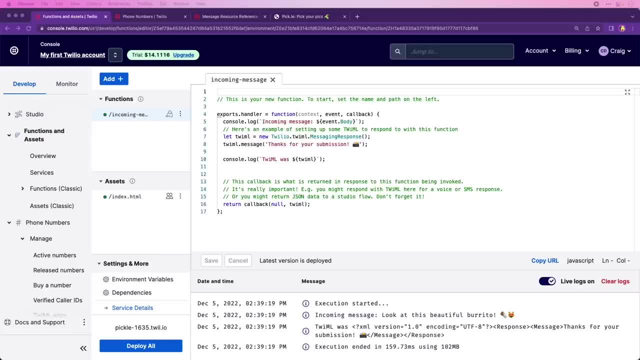 The limit is that you can only send to verified numbers. They can still submit, They just won't get this. thanks for your submission, So your phone number should. So when you submit from your phone number, you should get it, just like I did. 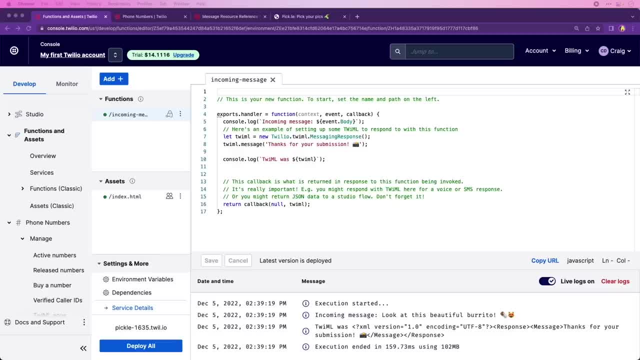 All right, so we're looking good, We have our site hosted and we're handling submissions by thanking them. Let's get to some more cooking Now. if you're interested in learning more about applications like this over the phone, check out the notes for more resources. 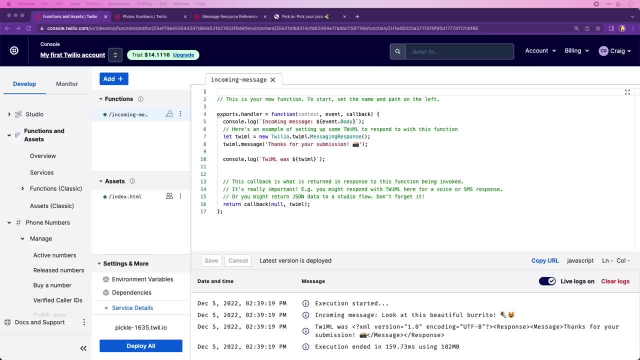 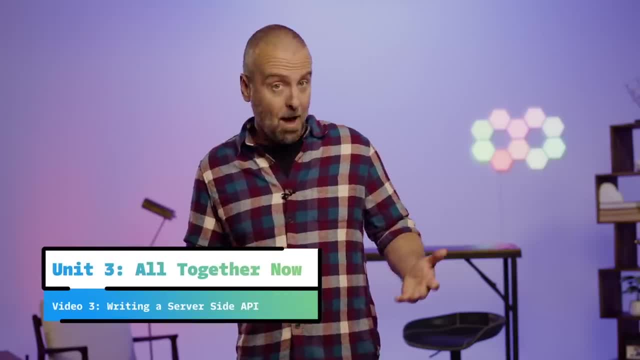 I have an entire course on this if this piqued your interest. But for now, let's get back to our API. Now, with our ability to host our own application, we can focus on designing our own API. Now the great news is that Twilio Functions. 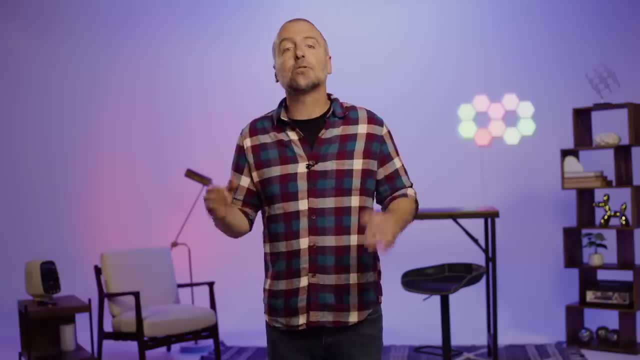 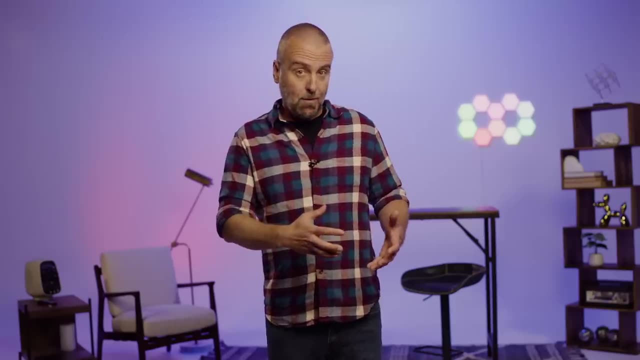 makes it really straightforward to return JSON. Remember that's JavaScript Object Notation, the lingua franca of the web. Let's design our web-based API to return the expected format And we can make use of Twilio's message API to get a hold of all of the messages that we received. 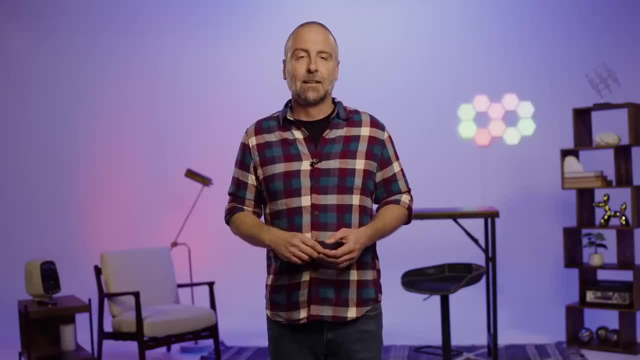 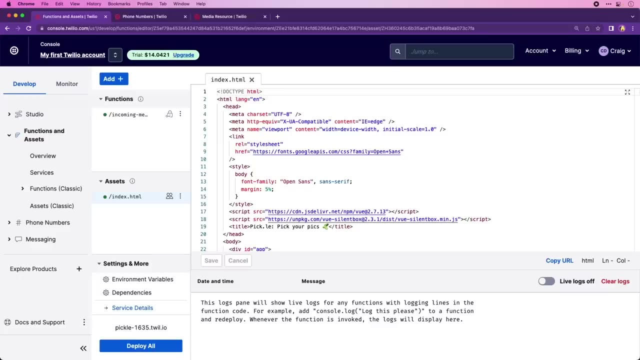 Do you see what I did there? Get, get it. All right, I'm gonna get out of here. I can't stop. All right, let's do this. Okay, so we're gonna actually write an API and we already have a spec or a specification, right? 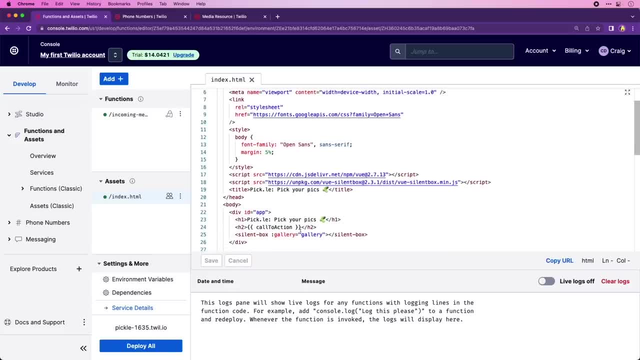 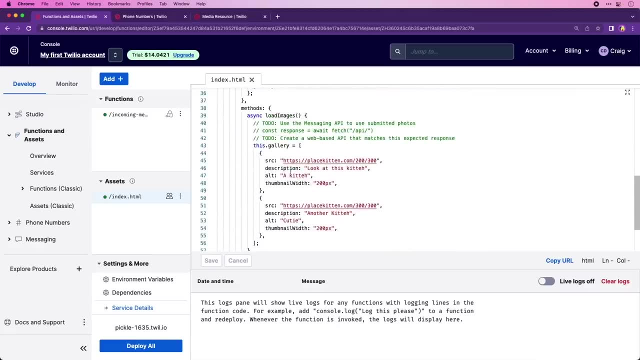 We need to provide for the specific plugin. This silent box has this gallery plugin and it has a specific API that it defines, And that API has a specific API that it defines And that API looks like this, right? So remember that we're setting this gallery. 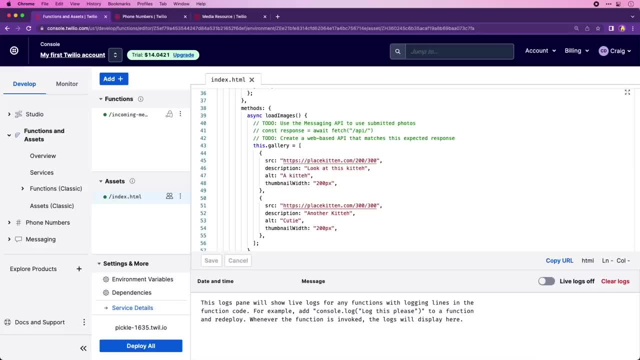 and we're setting an array and we're setting this information here. So I think we should start by creating an endpoint that returns exactly what we have here. We should return an endpoint that does this, that returns this, And then we'll move forward from there. 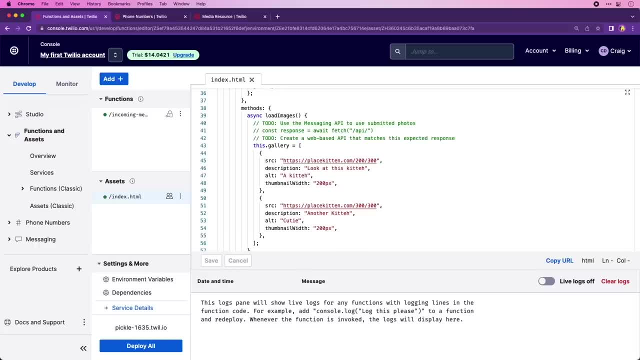 This is what I do when I find myself in a situation, when I'm working on a project with a team of people. I take what they expect in a template and I return it from an API. This way, they can keep working and I can keep working too. 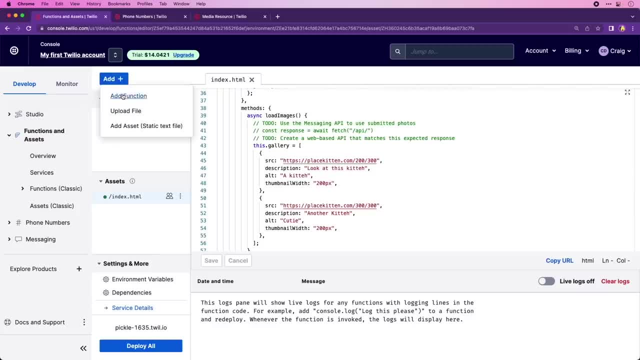 So let's do that. I'm gonna create a new function, So I'm gonna choose add, add, function, and I can name this whatever I want, And I suppose we should be clear, right, We're gonna make an API. We're actually gonna make one. 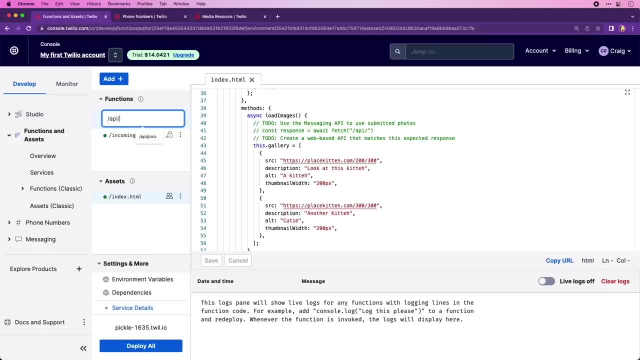 So slash API, And then I suppose we should probably just say what it's gonna be. So we'll do a PIX API here, right, And I'm going to press enter and that will get me my boilerplate code, of which I am going to get rid of. 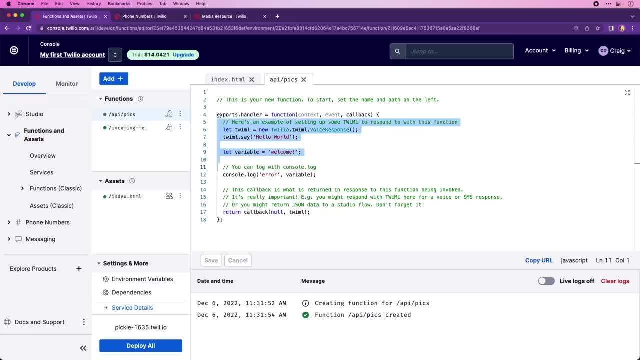 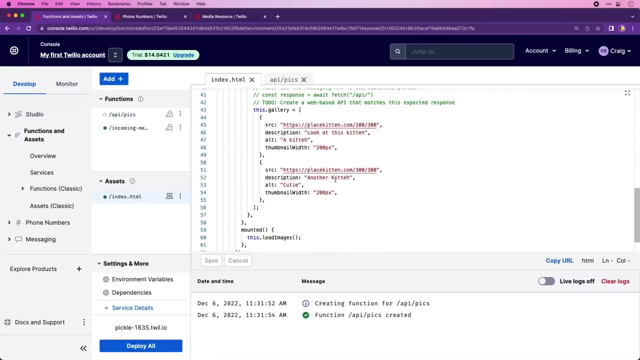 Get rid of everything. So thank you for the help. We're not actually returning TwiML this time. We're actually gonna return an object And what I'll do is I'll copy the hard-coded array from this index file here, I'll come in here and I'll copy this hard-coded. 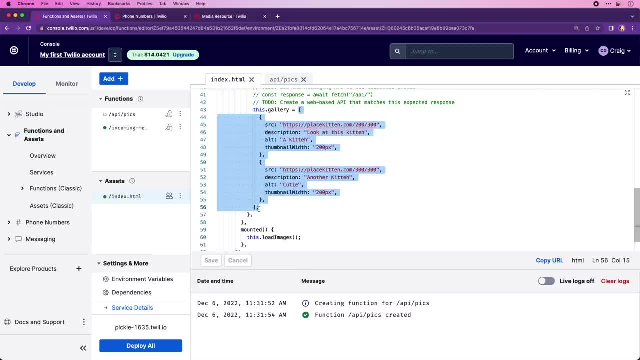 Now, hard-coded means it is just like in the code. this way, right? There's no way that this is going to be dynamic. I'm gonna change that here. I'm gonna paste that in here. I'm gonna name it the same thing. 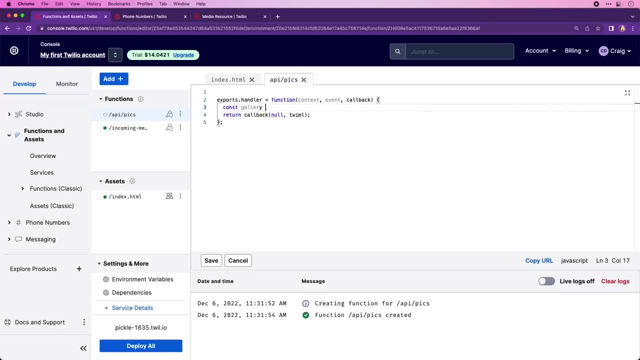 So I'm gonna create a new variable called gallery and I am going to just paste that hard-coded code there. There we go, And then I'm gonna call this gallery. So again, I have an array. That's what this bracket here is. 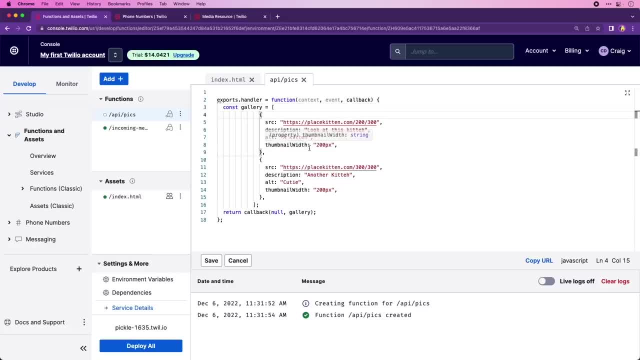 is array of these objects. That's what these objects are: These mustaches they open up and the objects have these properties here And these are representing the PIX That plugin requires, And now I'm gonna use this callback function to return that gallery array. 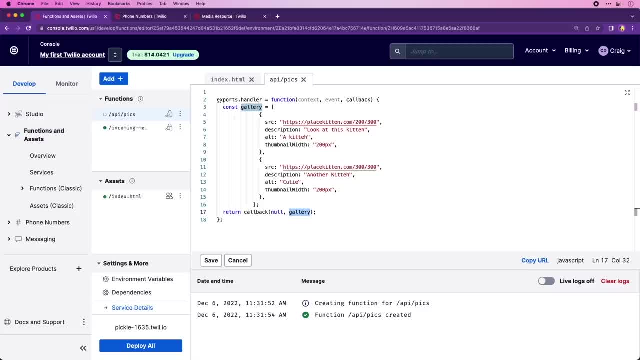 One really nice thing about this Twilio function is that if I pass it an object, like I did, it'll automatically return JSON to anybody who requests the URL. So let's do that. So I'm gonna go ahead. I'm gonna save this. 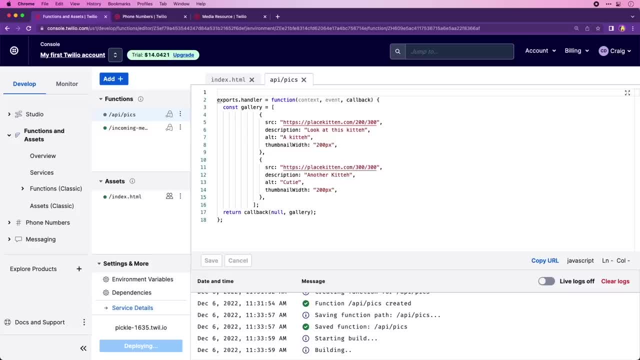 and I'm gonna deploy it. Now one thing to note: by default: it was actually protected. Now one thing to note: by default, it was actually protected. Now one thing to note: by default, it was actually protected. That's what this little key lock thing means here. 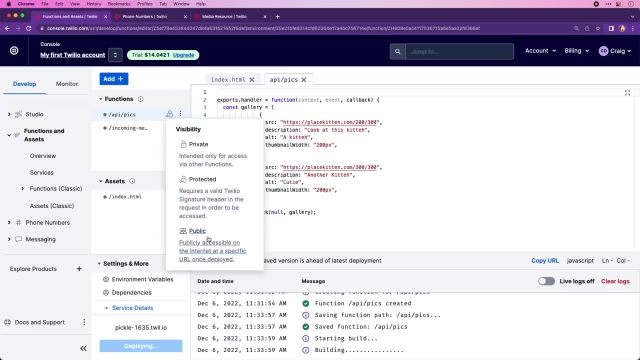 So I'm gonna click this and I'm gonna change this to be public, cause we actually want anybody to be able to see it, not just Twilio. So this is what we're gonna do: I'm gonna change this to be public, and then I'm going to choose: deploy all. 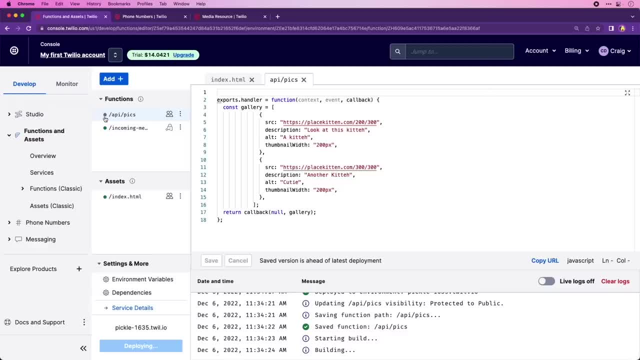 And you'll see that it's gray, And when it's ready, it will turn green for us, And so I'm gonna go ahead, I'm gonna copy this URL, So I have this URL ready And when it's green, when this goes to be deployed. 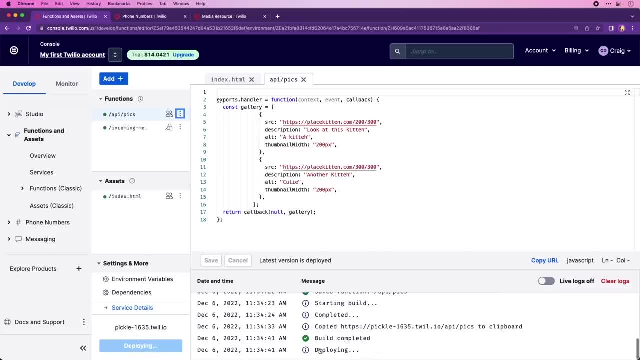 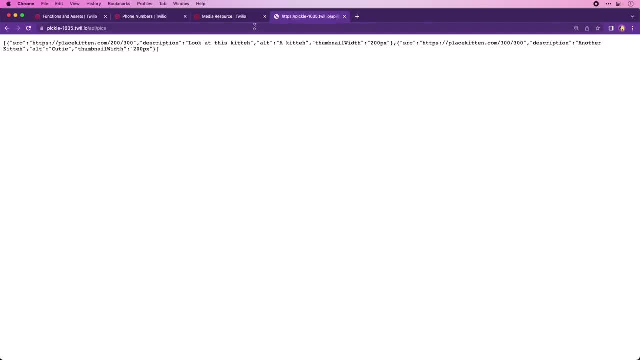 so it's still deploying. you can see it's deploying And you'll know. down here it'll say build completed and it'll say deployed, So it's deployed. So I copied that URL. I am gonna go hit that URL and let's see what we get back. 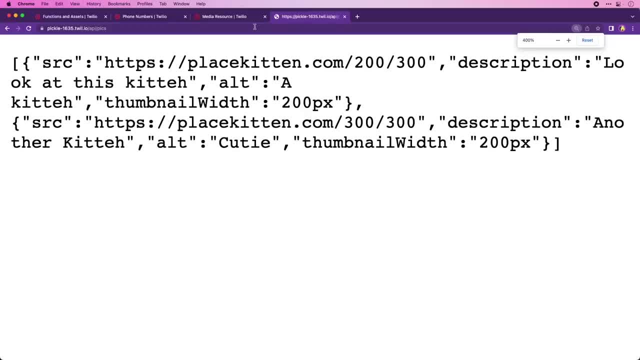 Awesome, we got it. So we got the kitty descriptions and blow this up a little bit here. This is JSON. it automatically built this for us, right? It put the it's in the right format, which is very nice. In fact, we could probably take this, and why don't we? 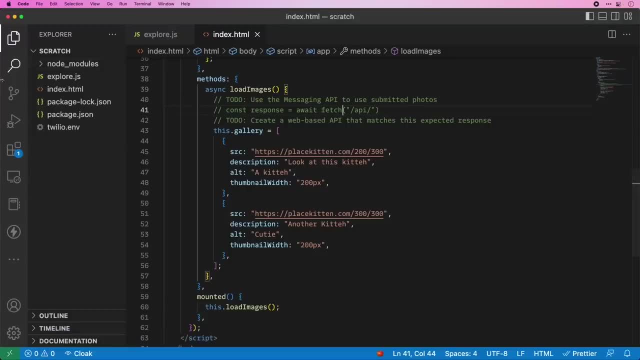 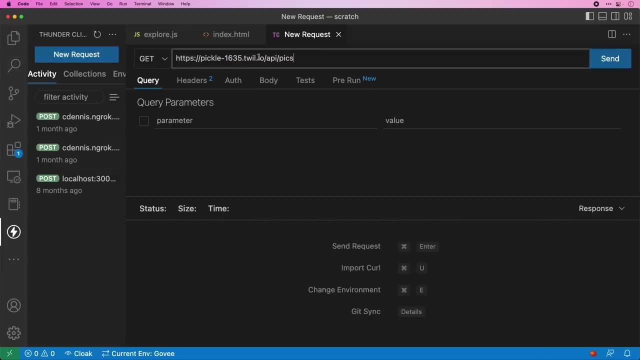 We'll go over to the Thunder client and take a look at what's going on over there. So I'm gonna come back to my Thunder client, I'm gonna make a new request and I'm gonna hit the do and get to this API that we just built and check it out. 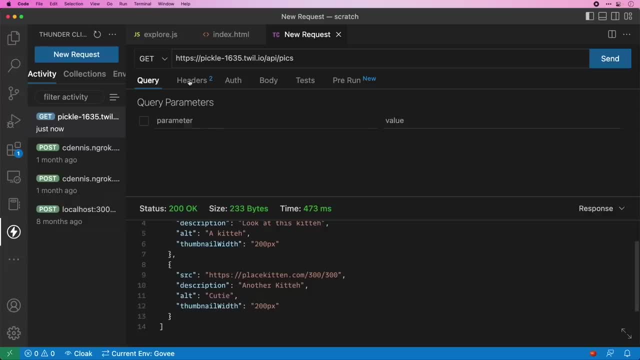 It comes back. it comes back with 200, okay, And here's the stuff that's coming back. There's even some headers in here. Oh, sorry, some. if we look at the response, we can look at the response headers over here. 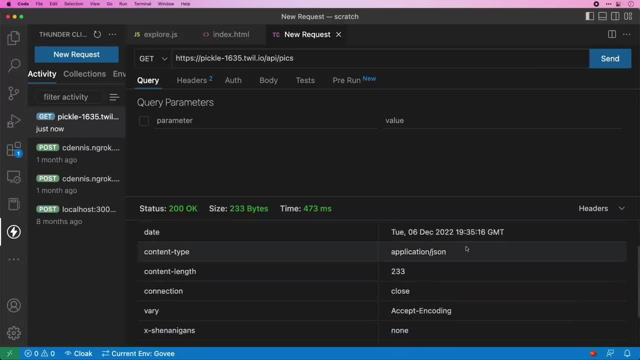 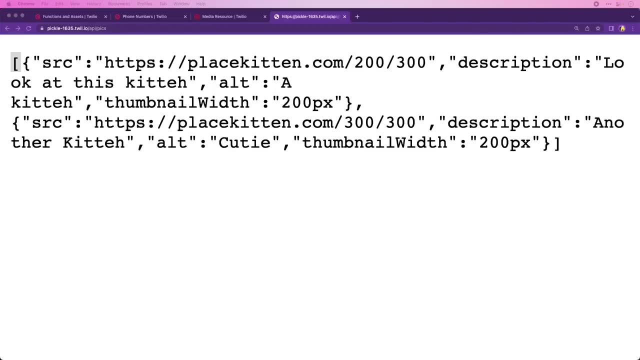 and we can see that the content type was set to application JSON. Twilio always sends back the shenanigans none which I love, So now what we can do is we can give this URL to the team that's working on making the front end. 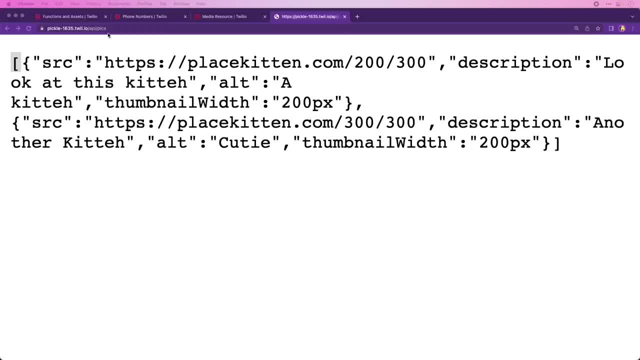 that view application. they could wire it up, They could take this, and as long as we match the same format and what we return, that is, as long as our API maintains the same contract, everything should just work. So that's pretty awesome right. 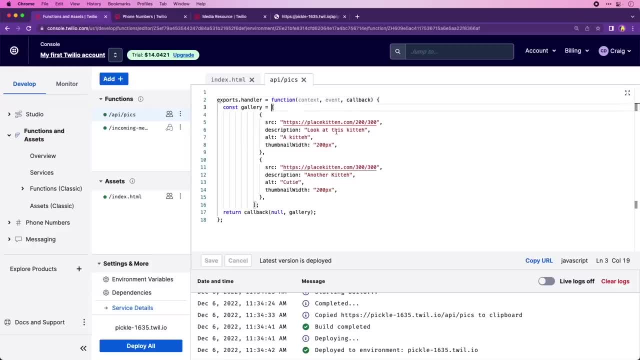 So let's move on to the next part. I'm gonna comment out this bit. So let's go ahead, let's give it a. we're gonna go ahead and make this an empty array, right? So that's how you make an empty array. 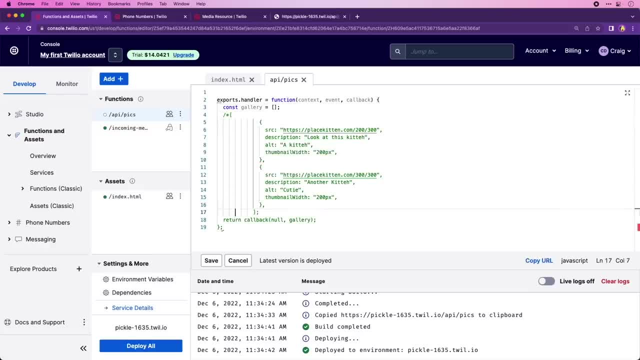 And I'm gonna comment this out so that we have it, so that we can kind of look at what the format is as we build stuff here. So I'm gonna comment that out And in fact I don't think I need the second one. 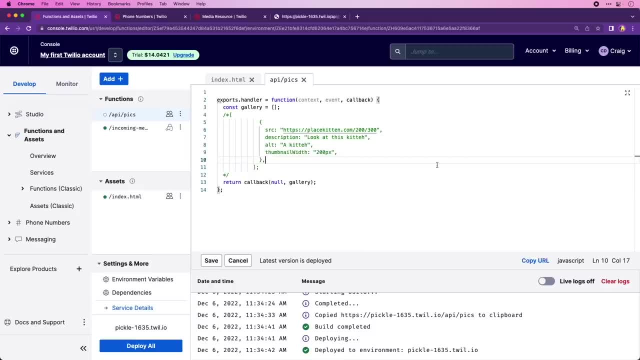 I'll just get that first one there. Give us some space there. Awesome. So now let's use the text messages that were sent in our incoming messages. So we're gonna write some JavaScript code Now. if you aren't quite fluent yet in JavaScript, remember. 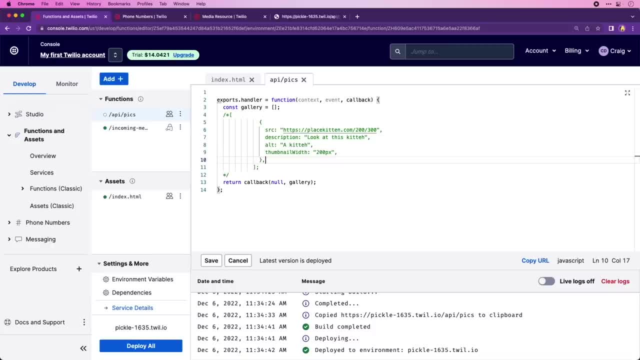 that is okay And we've all been there and we all, all of us. I guarantee you everybody watching this understands that what you're going through can be challenging. It's a new language. I want you to try to follow along conceptually. 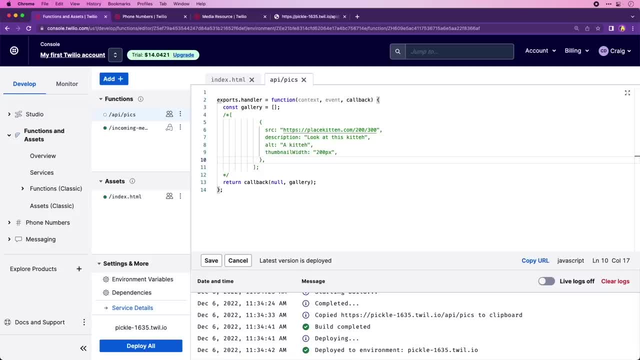 and I want you to take your time and I want you to take advantage of being in a video-based course. This code that we are going to write will be available in the notes and I will walk us through it And then I'll go over it again. 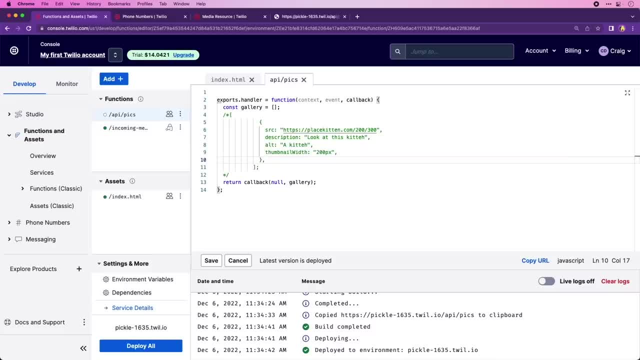 translating it into the concepts that we've covered. Okay, are you ready? Let's do this. So Twilio functions have another great feature: I can get access to a REST client. So the Twilio REST client authenticated. a Twilio REST client. 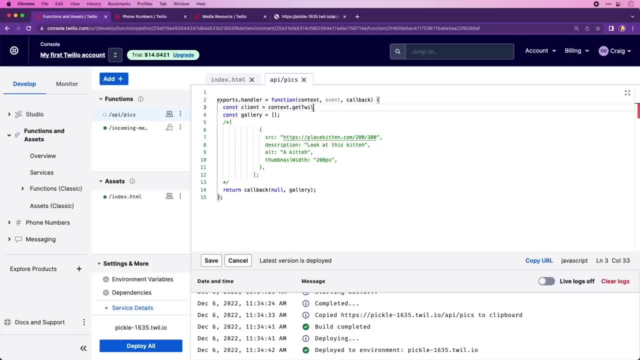 from the context object. So context: get Twilio client. Now, remember that is going to be using my auth token and my account SID and it's on this context. It just automatically is authenticated, which is really powerful Cause now I can get access to my thing. 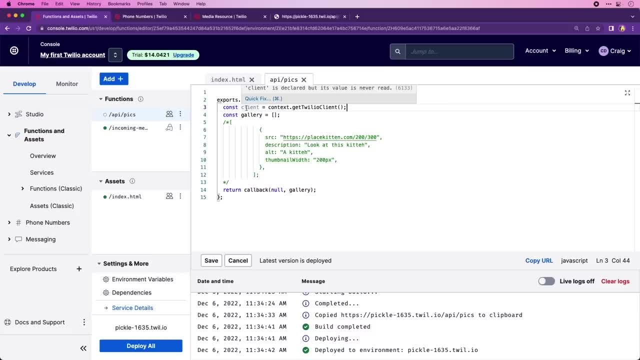 this function is running as me, right, So that's why it has access to that information. So, remember, we want to get a hold of all of the messages that were sent in, So we're going to use the API to do that. 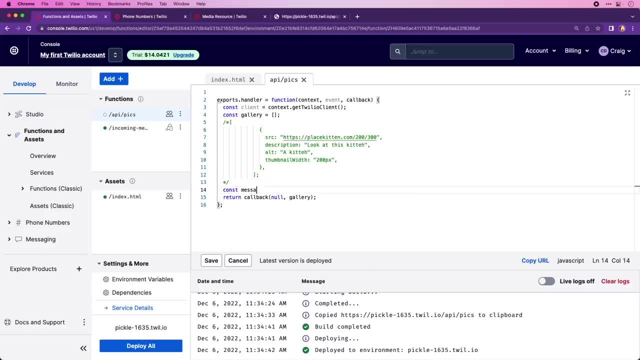 And remember we could have multiple phone numbers. So I'm going to get the messages that were just sent to this phone number, So I'm going to await, cause remember it returns a promise. So, clientmessageslist, and I need to do the ones that are specifically. 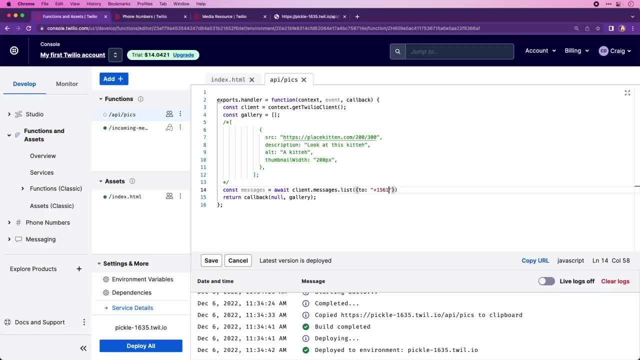 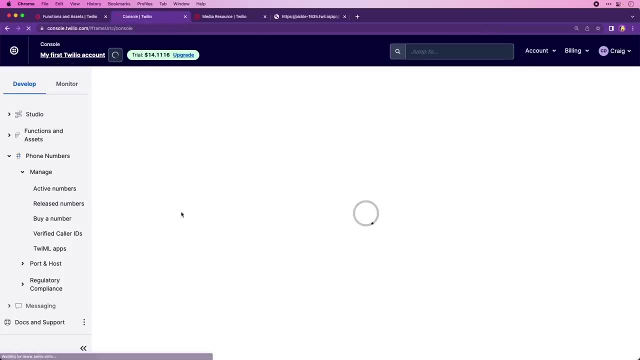 to my Twilio number, So that's 561-816-5433.. And I'm pretty sure that's right. I'm going to look one more time at my. oh, there it is. Yeah, that's it. So that's my phone number there: 516-854-33.. 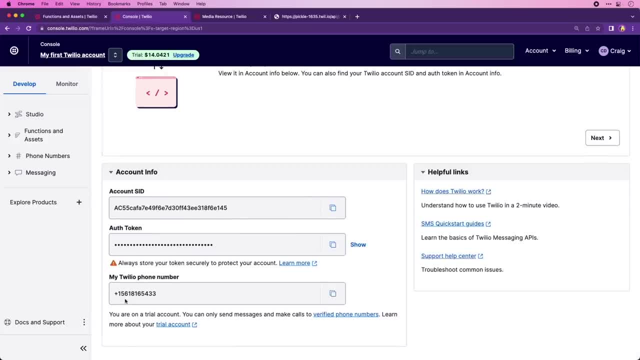 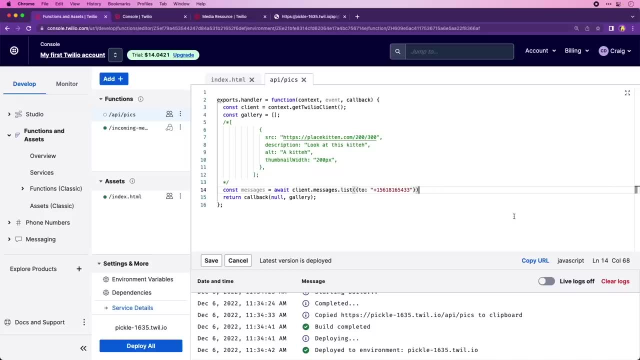 You could go there. it's also on your console, Remember, down here at the bottom, 561-816-5433.. That's what I wanted. I put that there. In fact, you know that's something. you can have: multiple numbers. 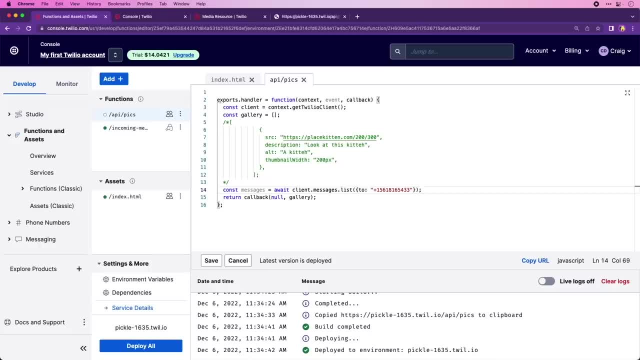 and that might be something that you want to store, possibly in an environment variable. So I think we should probably do that. Let's do that. So I'm going to take this number here and I'm going to store that here. You can see it in the functions and the services here. 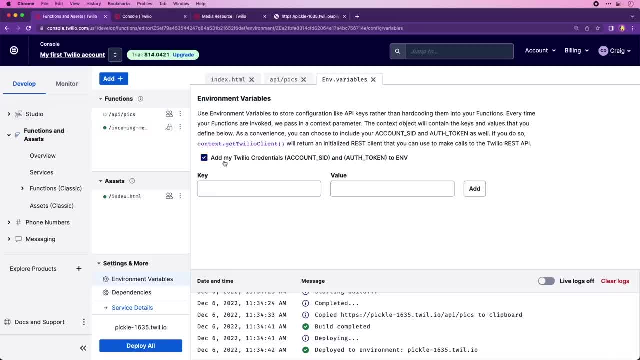 We have this environment variables. Let's add to that And you'll see here: actually, add my Twilio credentials. my account said my auth token to end. So that's why a context- get Twilio client works is because we've checked this. 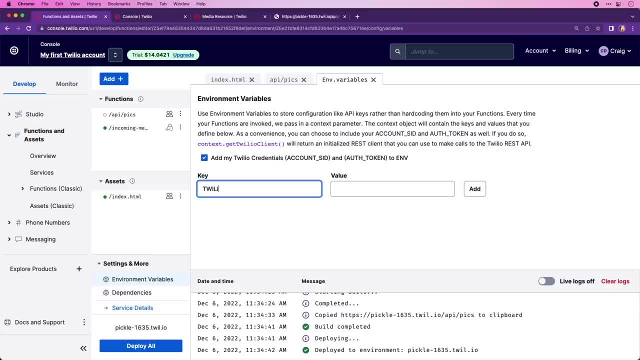 check this. If not, it won't work, So but it's checked by default. So we're going to do Twilio number and that value is going to be that, And now I'm in my code. What's rad is I can use that. 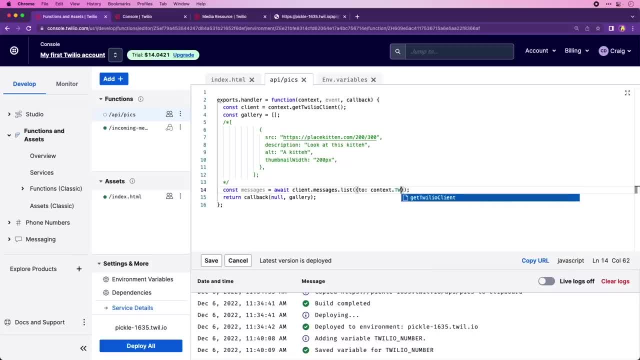 like, so I can say context: dot Twilio number. I can access anything that is in those environment variables that way, And it's now, it's in this code, And now, when I share this code, you won't need to do that. You will need to set your environment variable, though. 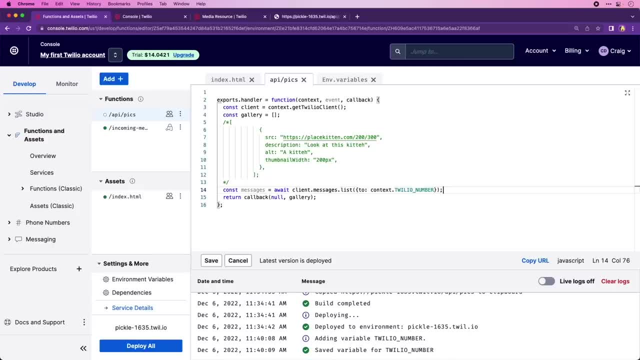 Awesome. So, and now, what we've got to access to? well, actually, first we set a weight and we need to make sure that this function is marked a sync, So that's required, right, In order to make this work. So now it's going to get the messages, It's going to return the messages, And now we're going. 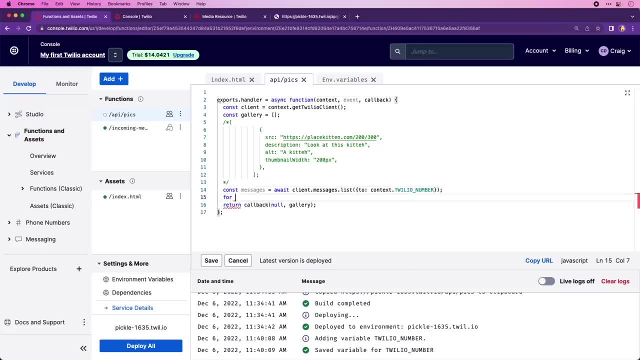 to loop through those messages. One of my favorite ways of doing that is this: for of loop. So we're going to say for message of messages And for each one of those messages, we're going to go through them And we're going to say for message of messages And for each one of those messages: 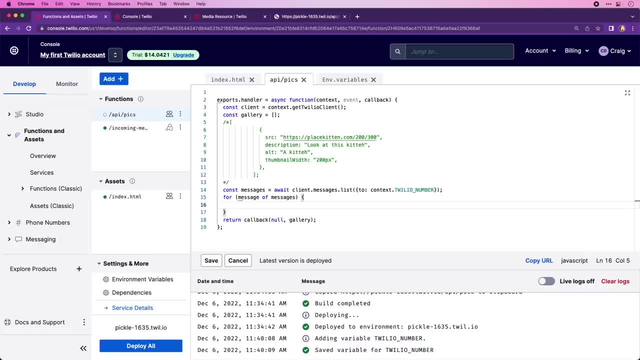 we're going to go through some things. So one thing you might not have thought about before is that when you send a message, you can put multiple photos. I think typically whenever I send one, I just send one, or then I send another message and another message you can. 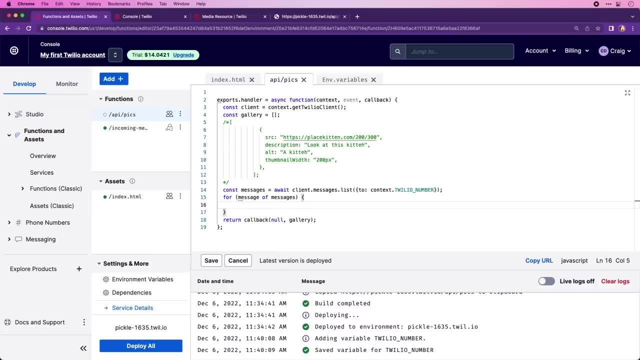 actually add multiple pictures before you send it. So let me, let's do that, Let's get a hold of all of the pictures that are available. So we'll say comp pics, We'll call, we'll call our variable called pics, right For picture, short for picture, And we'll say, oh wait. 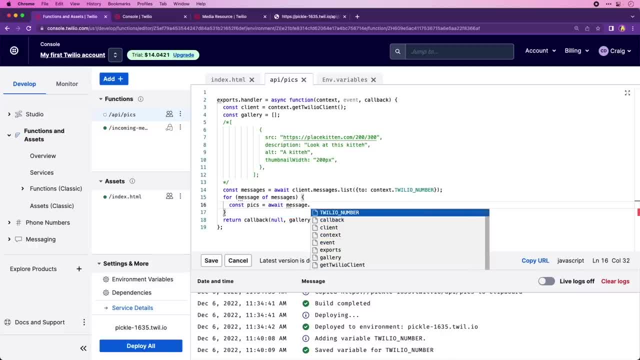 message. Now the message object that came back from this, this API. Now, we know that this was an API call, but it is an object and that object actually has access to the sub resources, which was media, which we we walk through this before. Remember there was the media URL and we grabbed. 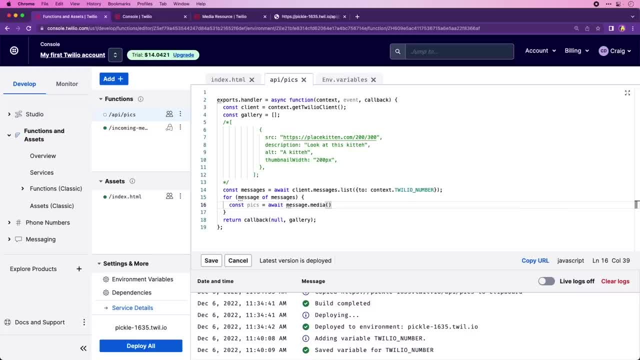 that media URL. we looked at all of them that were available. This is basically doing that same thing And we're going to get all of the media that is available, All right, so we have that. we have the message, we have all of the pictures of that message, And so for each of those pictures, 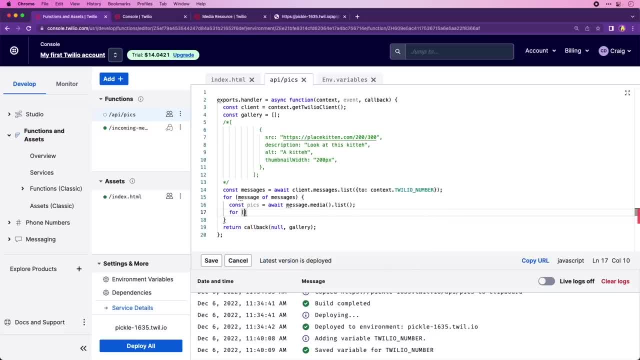 right, so each of the pictures we need to actually need to declare the variable, just to be better there. So we'll say for const pick of pics, right, so we're gonna make a new variable called pic, looping through each one of these that came back from from this array, right? 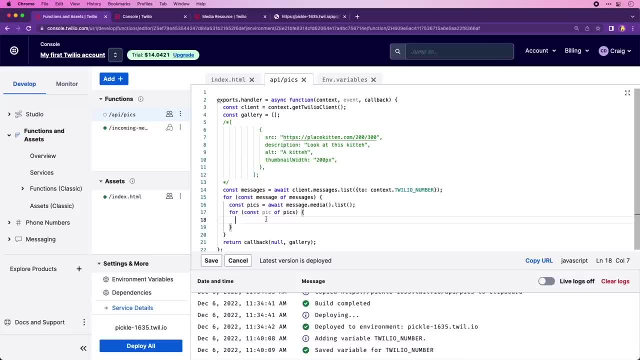 So, So, for all of the messages, for all of the pictures in the messages, now what we're going to do is we're going to add that to this gallery. So this is an empty array, but we're going to dynamically add to it. And the way that you add to an array, of course, is with gallery dot push. 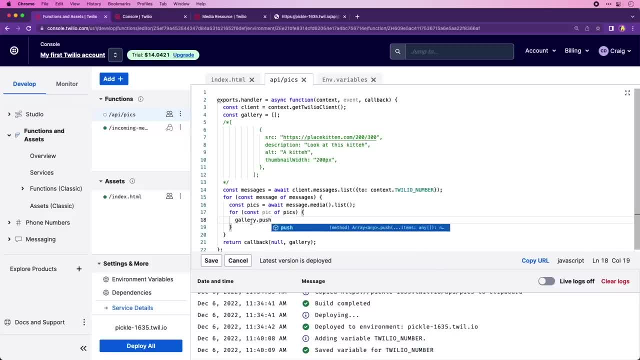 we're going to push a value onto the end of that array And we know what this is supposed to look like. right, It looks like this. it looks we have the source, right. So source here SRC is short for source. And then we have the source, And then we have the source, And then we have the source. 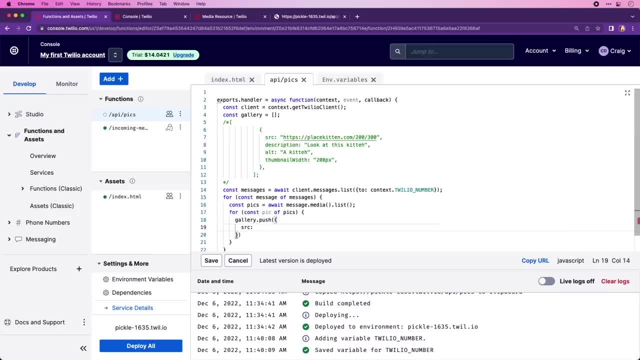 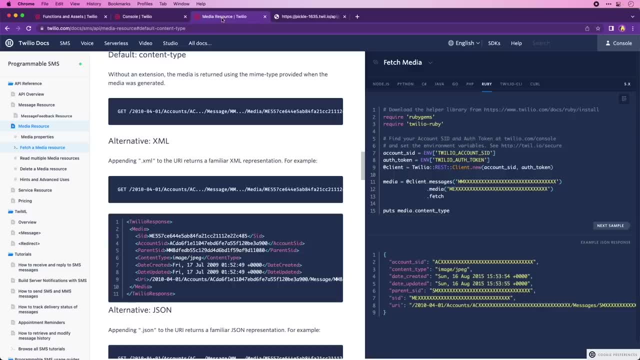 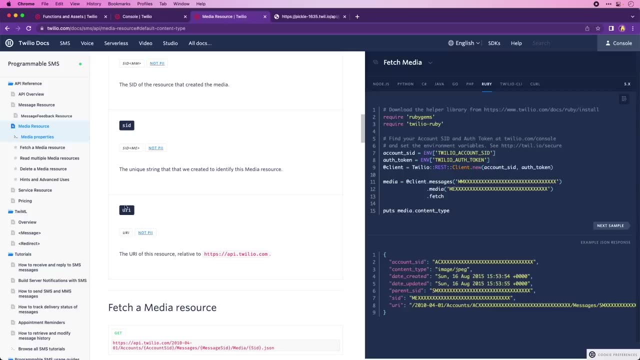 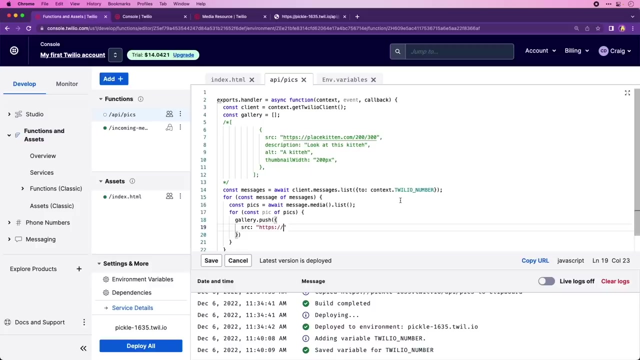 Source just from forever in the internet. So image source: SRC. And I know from from my, my notes, and I'm gonna pop over here real quick, that that this, this has the media resource, has this thing called a URI on it And it's relative to this HTTPS Twiliocom. So let's paste that. So 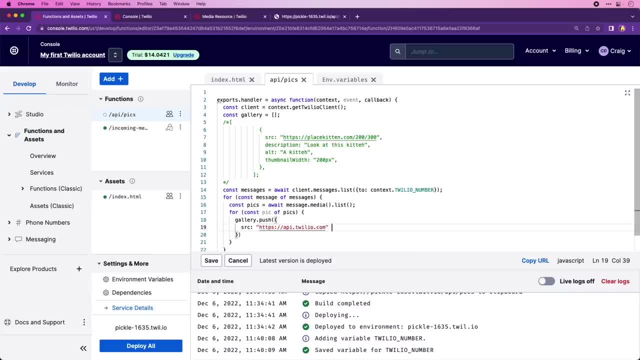 it's relative to that, which means that if I'm going to paste that, then I'm going to paste that here, So I'm going to display it. I need to let our people know. I'm going to give it a full URL. 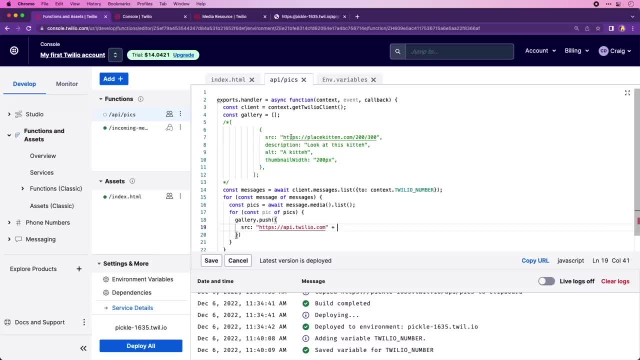 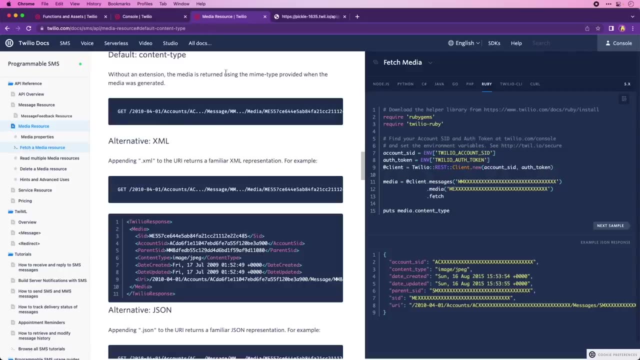 which it requires. right requires this full URL. So it's got the front part of it And then I'm going to use. the pic has a property called URI, which we saw And remember. what happens is it has this content type: if we want to, without an extension, the media is returned. Now I know. 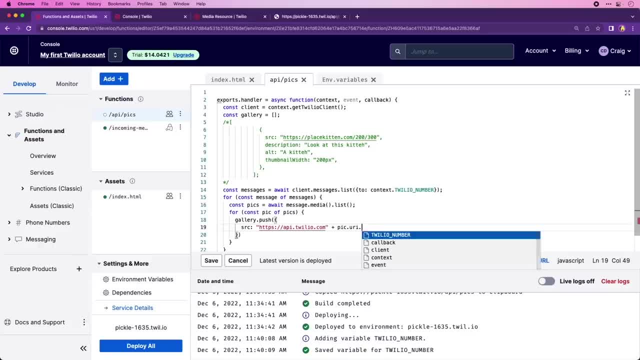 that by default. this is going to give me this pic: dot URI is going to end in dot JSON, So I'm going to replace that. I'm going to use the string method to replace the dot JSON. right, I don't. I don't want that dot JSON, I want it to be no extension at all, So I'm going to use this empty. 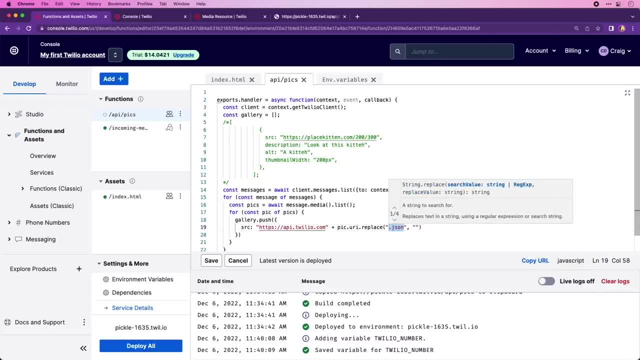 string. So I'm going to replace the end of what this pic was with dot JSON. I'm going to replace that with an empty string which will remove it. essentially, right. that's what we're going to do Now. I'm going to do a comma because I want to do more. I want to have the description. 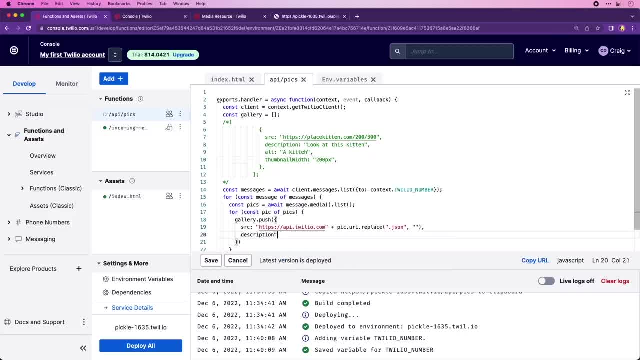 I want to put the description here is required Because that's what the little text is at the end, And I have a text that says: and that's whatever they texted in in their message, right? So I'm in this loop, I'm looping through each one of the pics, But I'm also. I have access to this. 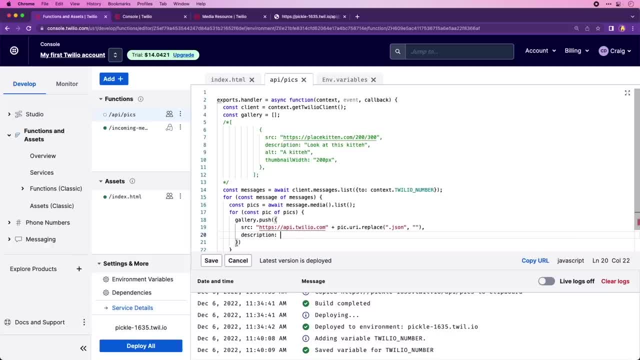 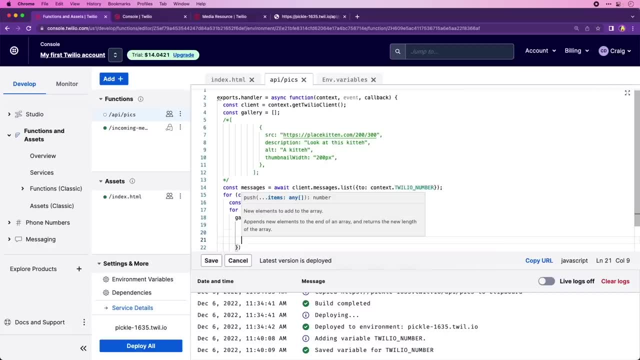 message, because I'm in this inner loop here, right? So I still have access to the outer loop, which is message dot body, right? So those are inflated. So that's whatever the text was that somebody sent it in And we should also. we'll make that the alt text too, So alt tags are handy for. 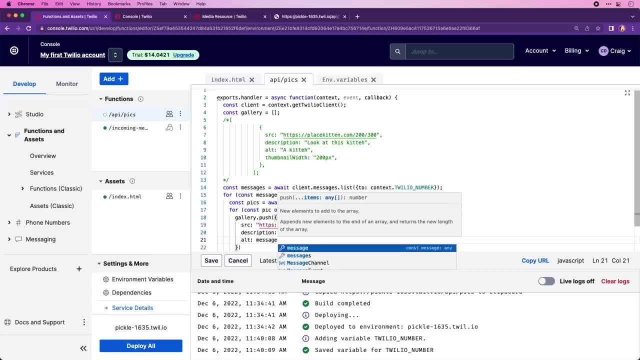 accessibility reasons. There there are people you might not think about this, But there are people who are going to use your application that are using it without being able to see some. So people are vision impaired and they have screen readers and alt tags are. 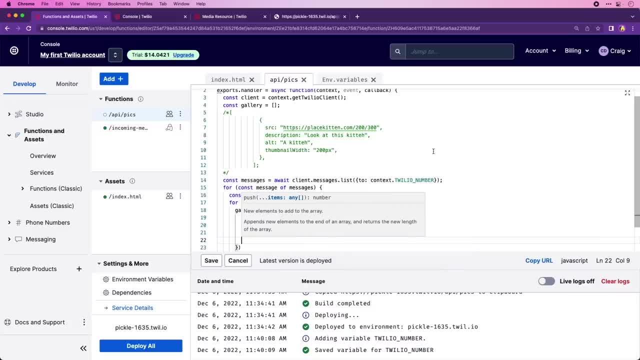 awesome for that. You always want to make sure that you make things accessible for people who can't see what it is that you're providing, And alt tags are an excellent way of doing that. That's just one way that you can make your application more accessible and everybody. 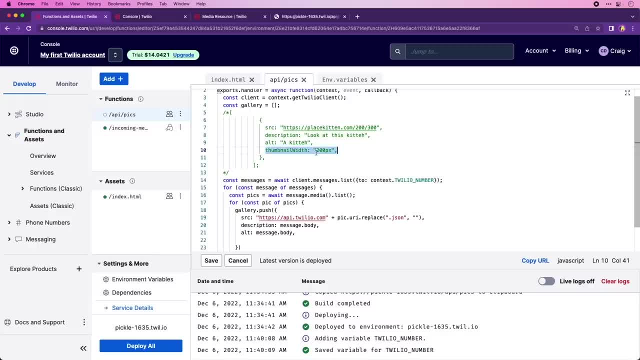 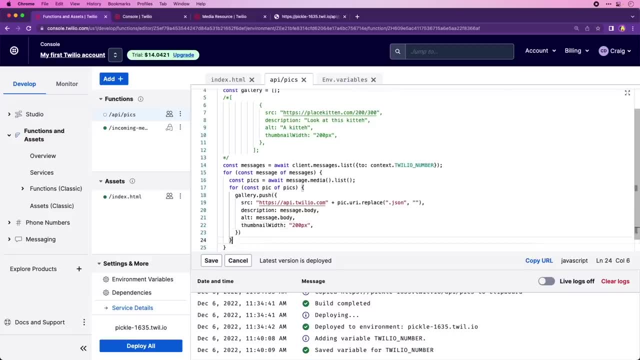 wins by it. And then, finally, I'm just going to grab this last thumbnail, width here, 200 pixels. We can see later if people want something different than that, what to do. So our gallery array for each one of those pictures it's going to add to it, right, So it's going to go and it's. 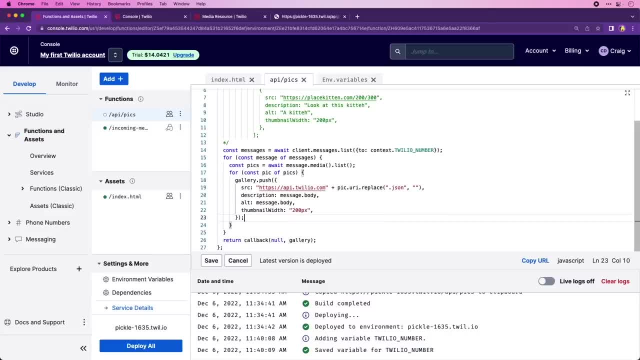 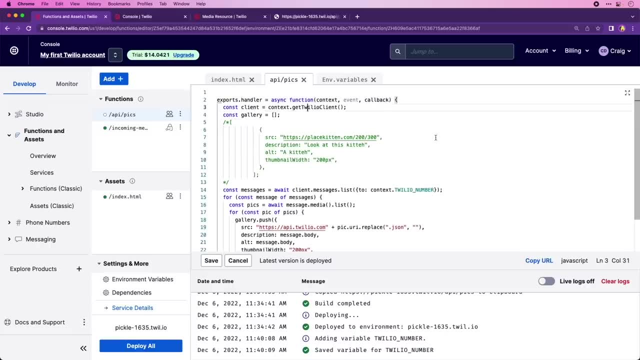 going to add each one of those and we're still going to return that gallery And I think y'all, I think we got it. Let's walk it one more time, Okay, so we're going to come in here and we are going to use the context that was passed in to this function when it was called. So when somebody 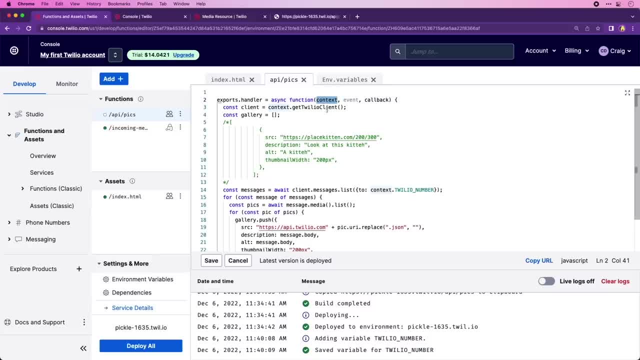 hits this URL, this function is going to run and it's going to know, it's going to have access to those environment variables that we saw. It's going to get access to an authenticated client And that client is logged in with my account, Sid, and my off token, And we're going to create an empty array, this gallery. 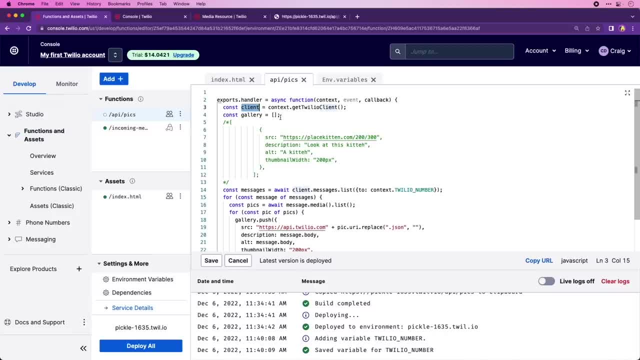 thing here. we're going to create an empty array. it's a list that we're going to populate. we're going to take our messages and we're going to push them into this array so that it has the format that is expected, which is right. here we're going to turn what our messages look like into. 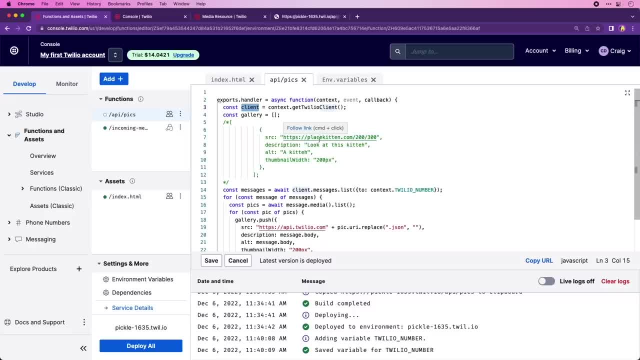 this so that later we can use them that way. So the way that we do that is: we use this client. this client is a rest client and it's going to hit the messages endpoint And we know that it's going to do a get. 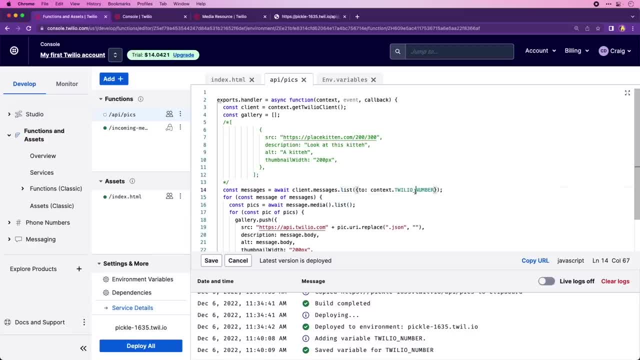 but it's been abstracted for us. So just we're just say: hey, list all of the numbers that were sent to this Twilio number. And those are this, this context, here Again, this is passed in in the Twilio number is set in my environment variables over here. So we're saying: because, because you 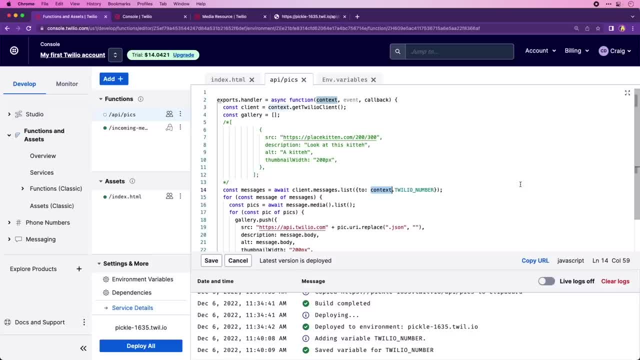 could have multiple, right, you could have multiple Twilio phone number. So we want to say only the ones that were sent to this Twilio number. So we're very, very specific. we're querying messages that were sent to this number, not from this. 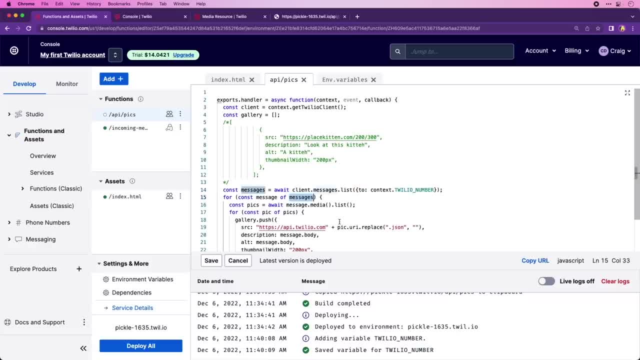 number, but to this number And we're going to loop through each one of those messages, And for each one of those messages, the object that's returned from this has this property called media, which lets us get to a sub resource, And 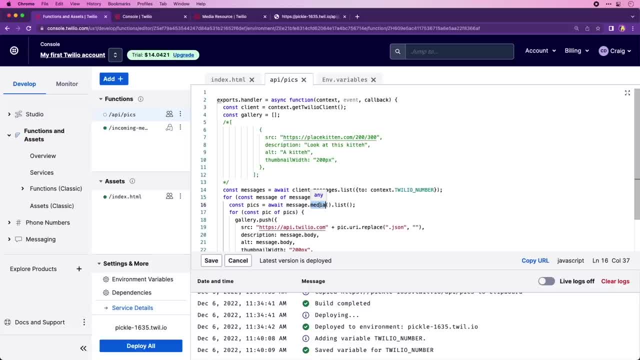 you'll remember, in the JSON there was a. there's a link to this and we could go and query this ourselves. but we don't need to because the API has wrapped that for us. It's very nice. It's nice, nice abstraction And we're we're. 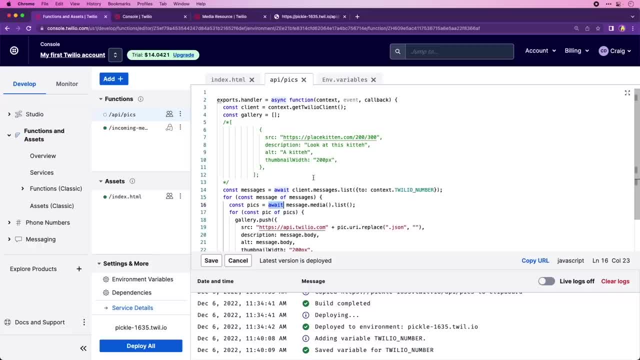 going to get the list Of those pics And again, this is asynchronous. we're using this, we're waiting for it to come back. we're waiting for these values to come back. So, once we have these pics, we're going to look through each of the pic And we are going to push out a source that has this. we 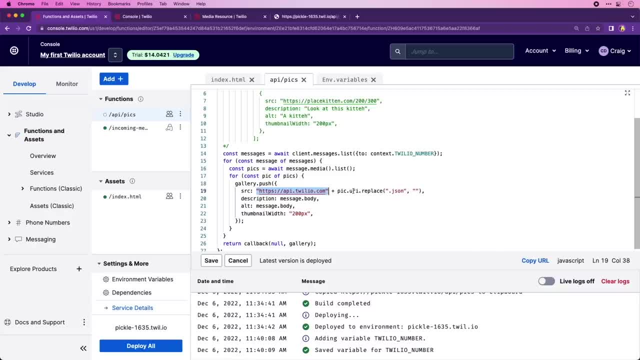 know that they all need to start with API Twiliocom, Because the URI itself, this URI here, is relative meaning, it doesn't contain the forward slash of this. So we're going to say: this is where it lives, This is the API call that we want you to do. 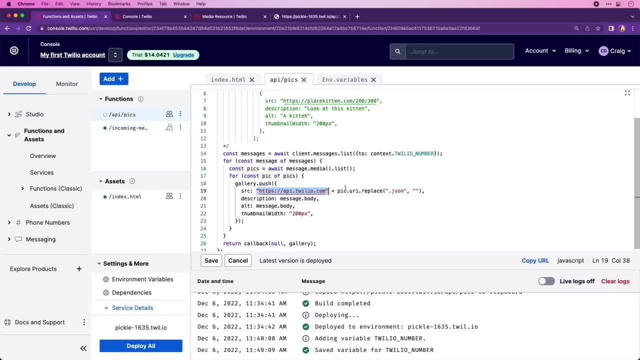 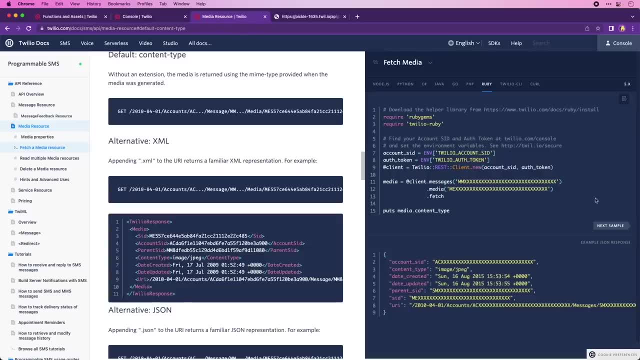 to get this content is apitwillycom- whatever is in the pic- URI, because that's unique to each one of the pictures And that URI comes with a JSON at the end of it. So if you look here, let's see: 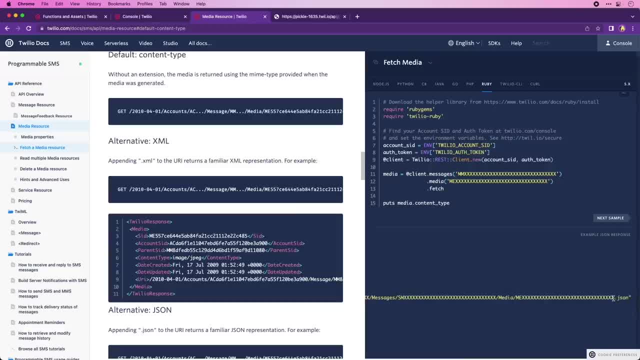 if we look here, we can see that it ends in this json right, And we want to get rid of that, because when you do get rid of it, what happens is it returns the actual picture. We did that. I don't know if you remember that earlier we did that. 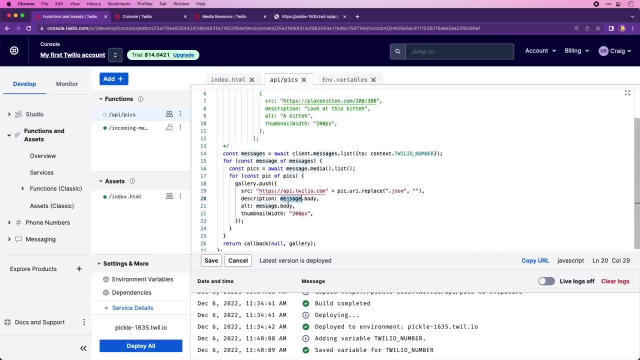 So, so that will be removed And then we're going to use the message and the messages coming from here, right? So the message for each of these messages, we're going to get the messagebody and the description and the alt tag for it. 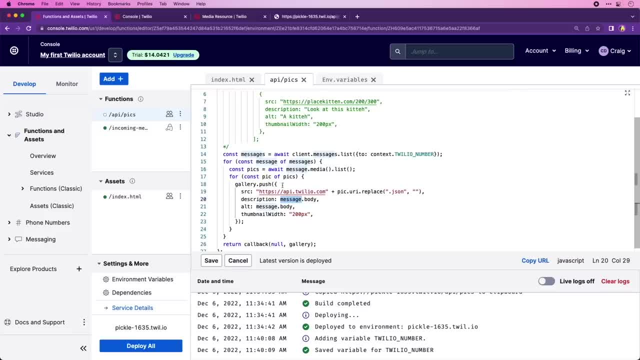 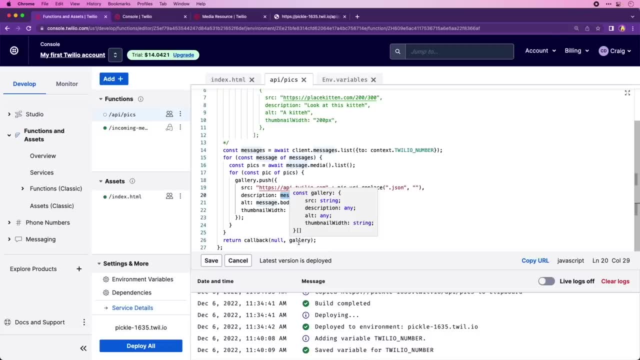 the alternate text we're going to set And that's from that. This is the required for remember. this looks exactly like what happened here, So we are returning that here and it should return JSON. I'm going to save it, We are going to deploy it and we are going. 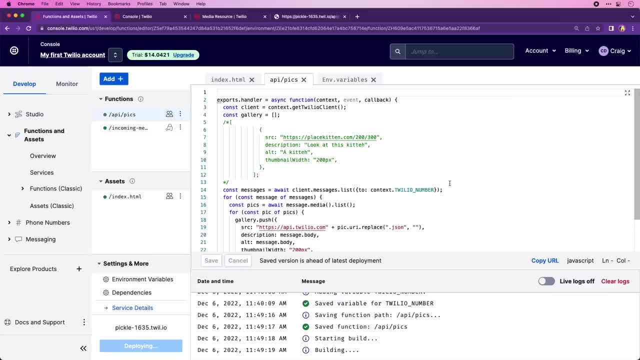 to cross our fingers because this we are at that point where we hope that the code that we wrote works, And if it didn't, it is okay. If it didn't work, we are going to work through it. We might get an error. 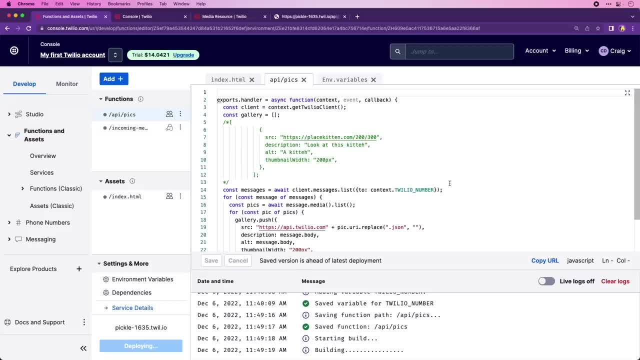 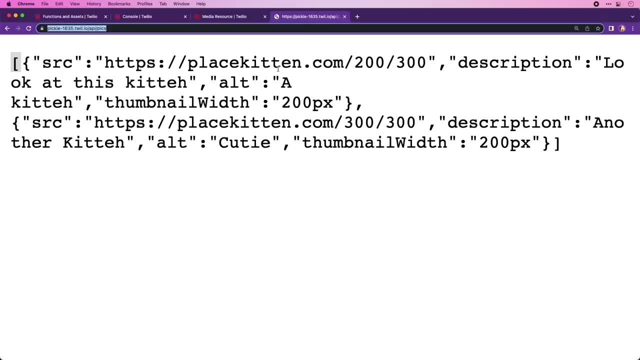 We might not understand exactly what that error is and we're going to work through it, but I am going to save this and deploy it Now. I let's assume that I gave this out. I gave this out, So now, if somebody hits this API, here we go. 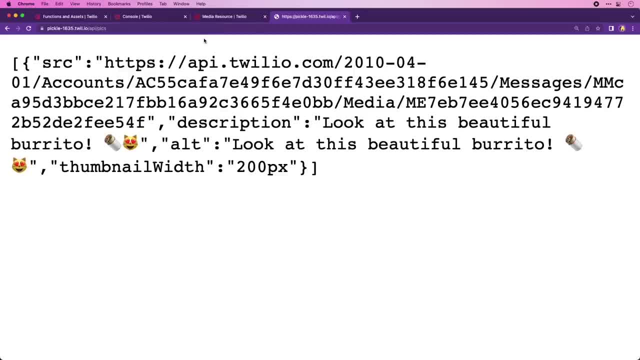 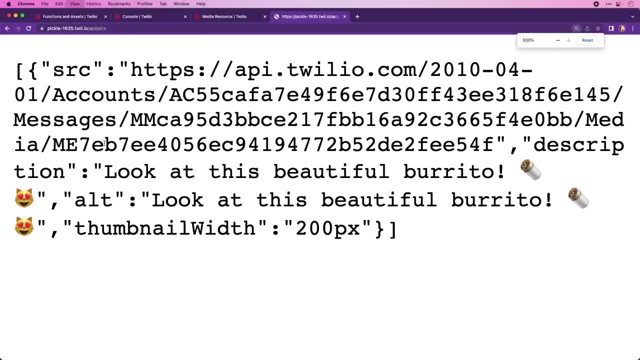 So that's what it was before. If we hit it, we should see burritos. We got it. So it says: look at this beautiful burrito. I texted that hit Wow. look at the clarity of the burrito. 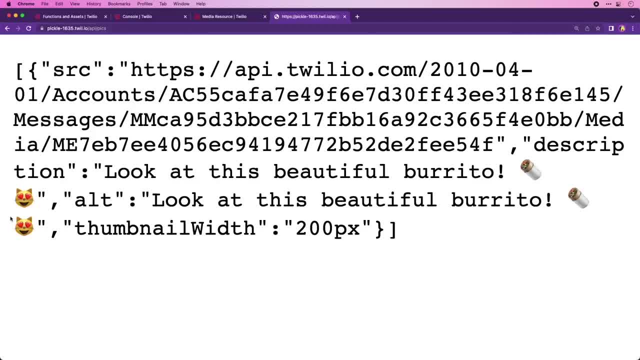 Oh my gosh, you can see the rice in the burrito emoji. That's impressive. I didn't know that. Look at that cat. All right, so in fact let's go hit it with our let's hit that same request I wrote before. 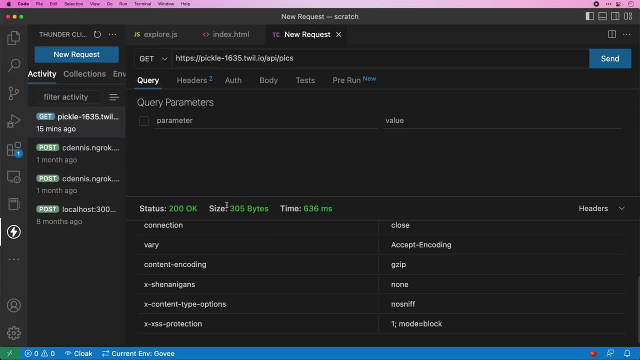 It should be a little bit different. now It's coming across here and I want to look at the response and the response. I'm going to go, I'm going to grab this URL and make sure that it works. So the source right. 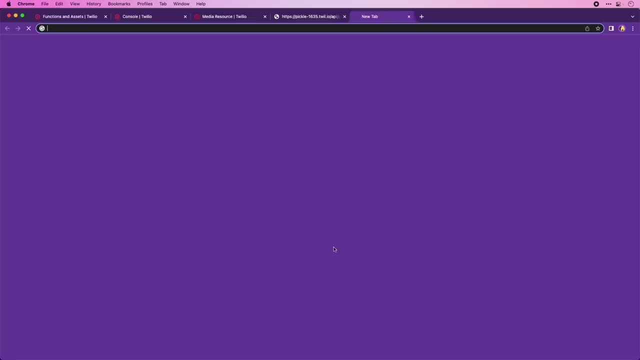 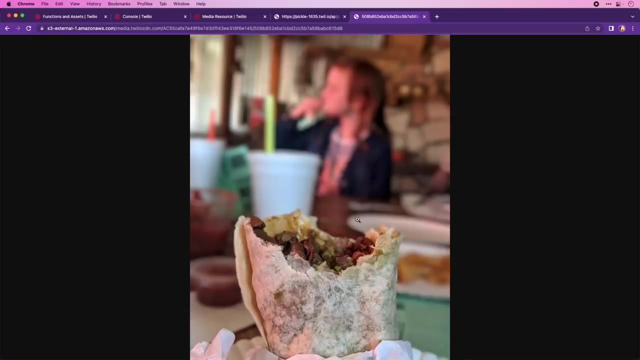 The source that came back here is should be the picture of it, And if I look at it, I should see my beautiful burrito. Oh, look at this thing. I believe that burritos when they can stand up by themselves. 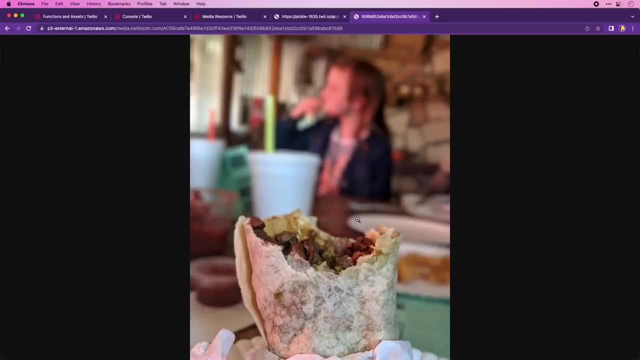 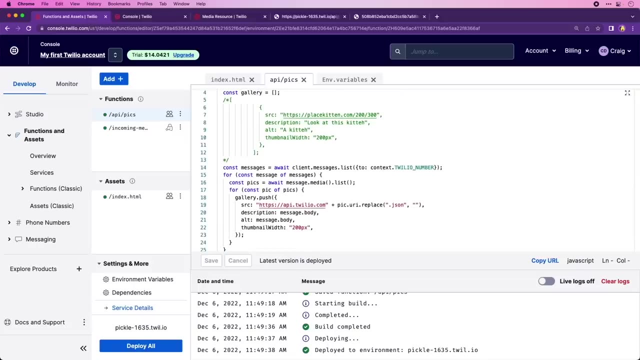 that's a sign of a good burrito. Look at that burrito. I got that in Arizona. Oh man, And what we did with this code is actually pretty common. Now, in an app like the one that we're building, probably eventually, what you're going to do is you're going. 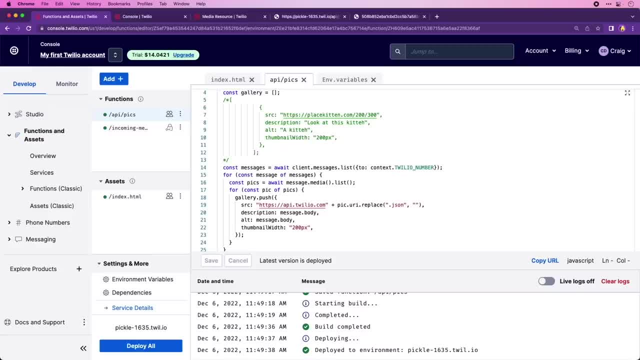 to store those photos That were submitted into a database, right, And you're going to do that from this incoming message function. You're going to get it, You're going to store it If it's valid, if it's a valid picture. 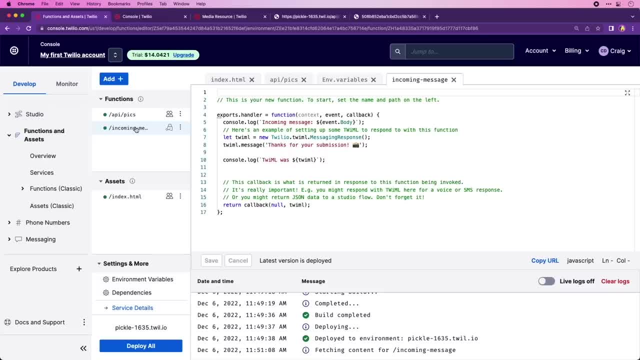 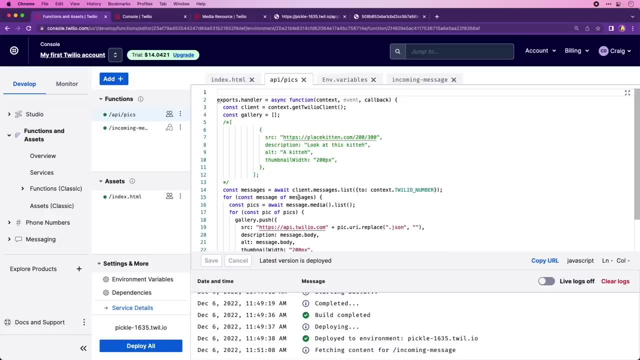 you don't want to show pictures, that aren't? you're going to store it in a database And then you're going to format it for whatever your client is, You're going to get that from a database. So maybe, instead of coming back from this API, 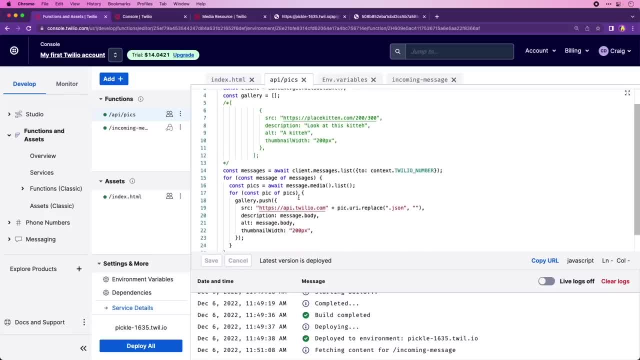 you're going to come from a database API and you're going to pull back your information and then you're going to push it through And that database is going to be in its own format, but you're going to make it match whatever it is. 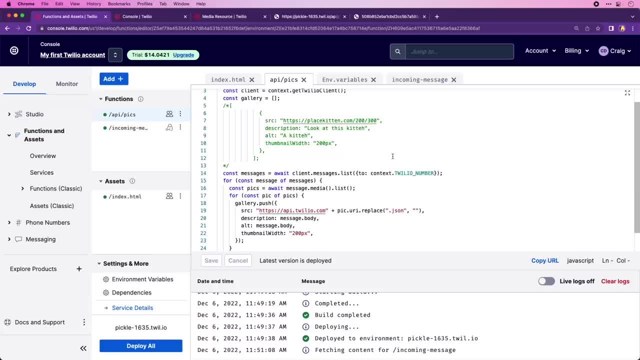 that you are trying to push out there. You're not going to. it's not going to look exactly like the message, right? I'm not going to send back one of these messages and make my API look like that. I'm going to shape the data. 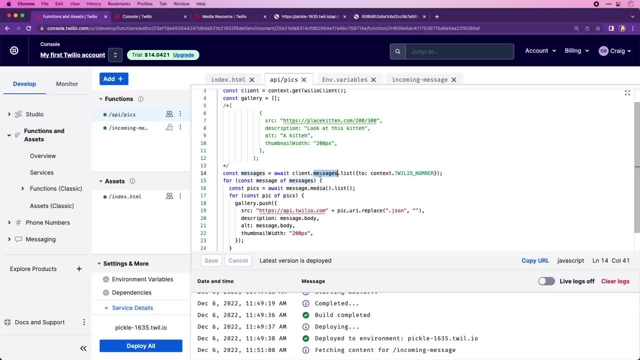 That's what that's called. I'm going to shape my data in the way that I want it to be used, And we came with the spec. This is the shape of the data. So we took the data and we shaped it. We formed it into what was expected. 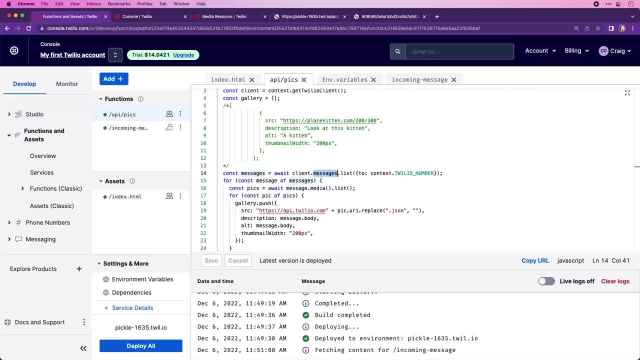 All these burritos are making me hungry. I think I'm going to go fetch one from my favorite taqueria. I'll make sure to snap a pic. You should get one too. actually, You deserve it. You deserve a burrito. 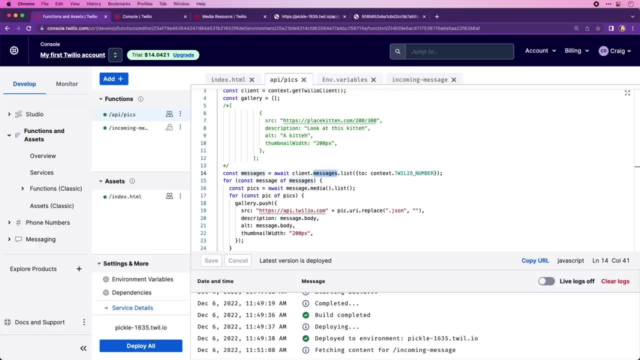 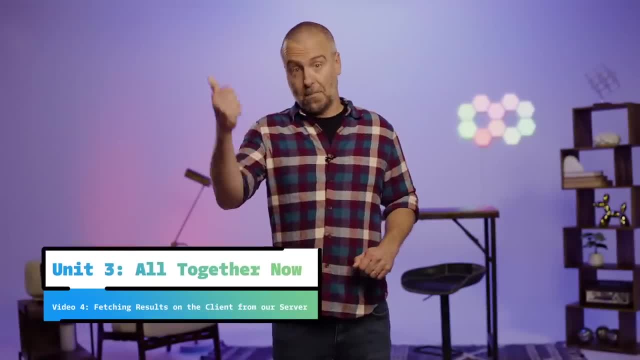 And when we get back, we'll look at how to fetch this data that we just generated in our client app. So we've coded our external public API and it's ready to be consumed. Now our API uses an external API- Twilio. 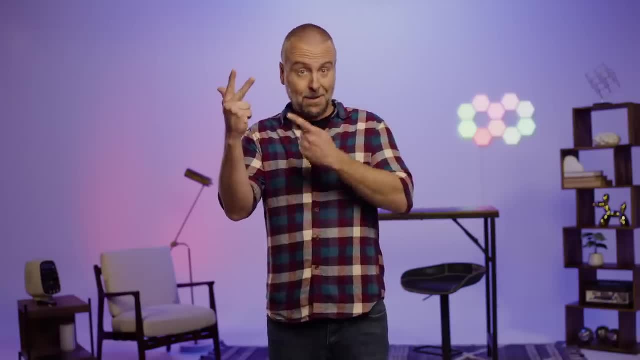 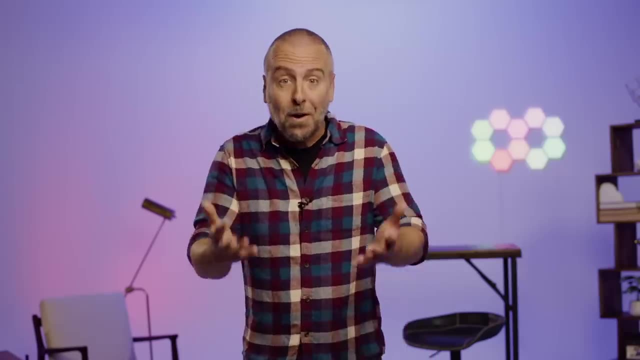 and we're going to need to use our web framework views API to retrieve the data, And to do that, we're going to need to use the web API. fetch APIs are everywhere, No wonder you came looking for this course. All right. 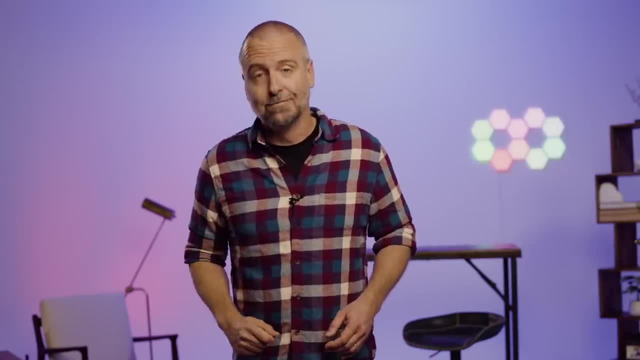 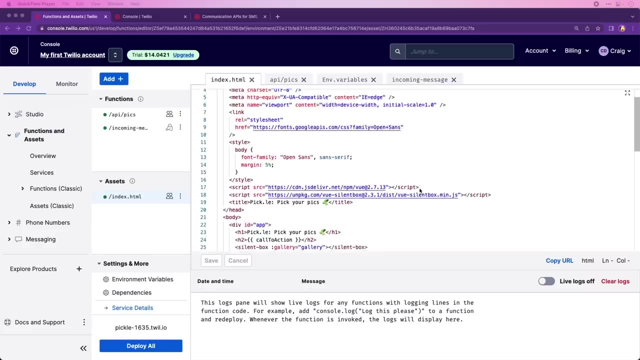 Let's make use of our server-based API and our client side application, All right, So just like I just consumed my burrito, we are going to consume that API that we just created. So if I scroll down here, remember we're passing in this gallery here. 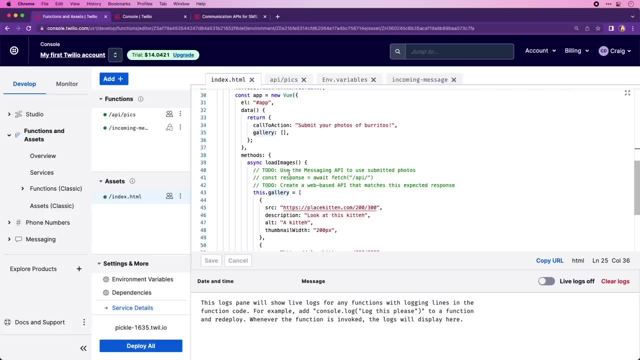 and we scroll down here into this load images and this load images gets kicked off from the API of Vue, right? So Vue has these lifecycle APIs And when the thing's mounted, it's going to call this load images. We're going to come into load images. 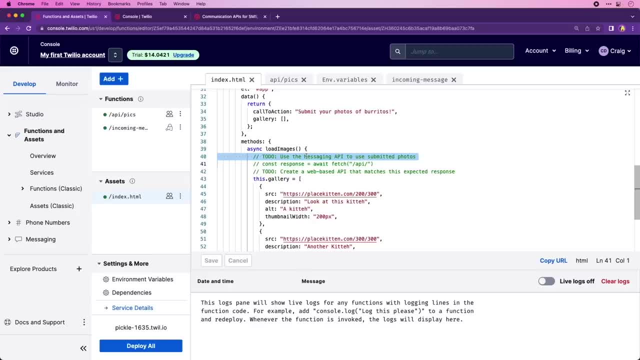 And now we have some to-dos that we have already to done. So we are going to use the messaging API to use submitted photos. We did that, We did that in our API, And then we are going to create a web-based API. 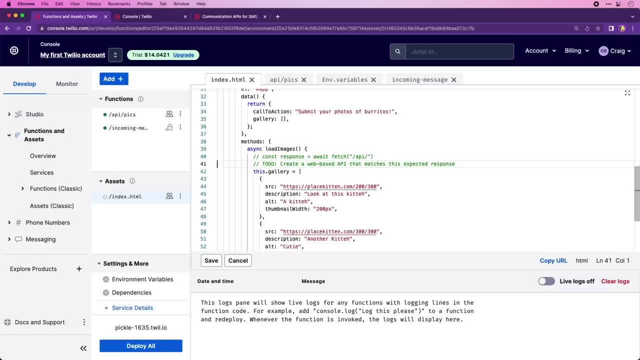 that matches this expected response. We also did that, didn't we? We did that, So let's get rid of that. All right, So here we go. So this has got a suggestion here of what to start doing here, So I'm going to uncomment this. 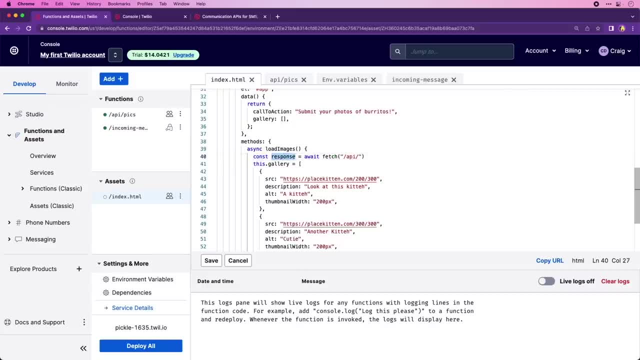 So We're going to create a new response object and we are going to await And we are going to use fetch, And fetch here is part of the web API that browsers must implement to do exactly what we're trying to do, right. 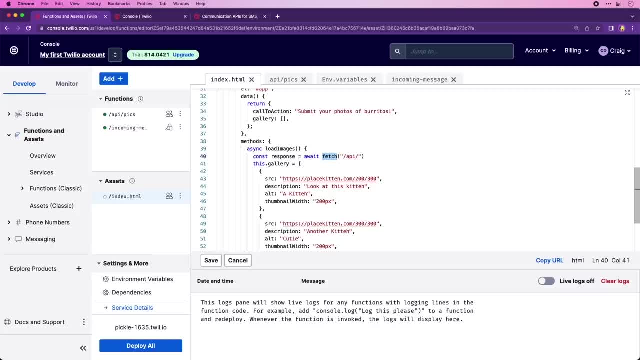 We want to fetch data from our API. Now this happens to be on the same server, So we can use a relative link like this slash API. here We don't need to specify the server, right? It's assumed So our API. we called that right. 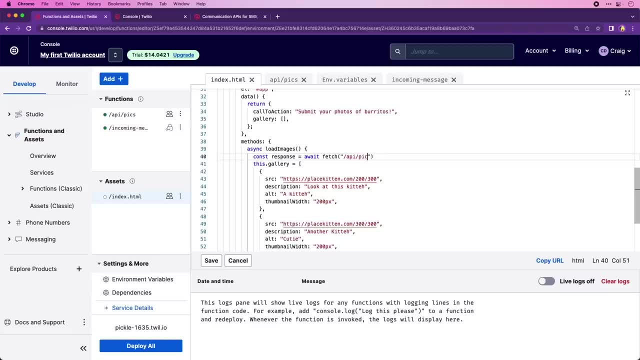 We called it API slash picks. So slash picks is what we are going to hit there. And you notice that it's using await, because this is an async function. So fetch returns a promise and it's going to return that response, And that response has a method on it called JSON. 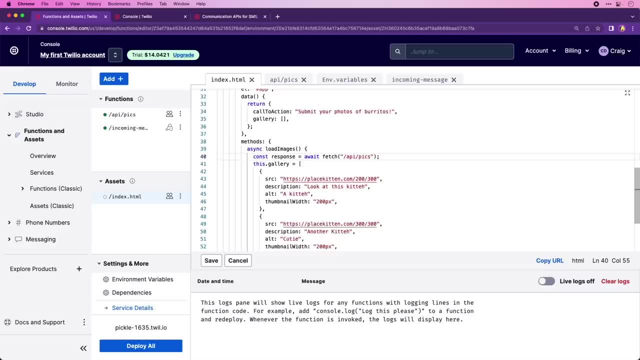 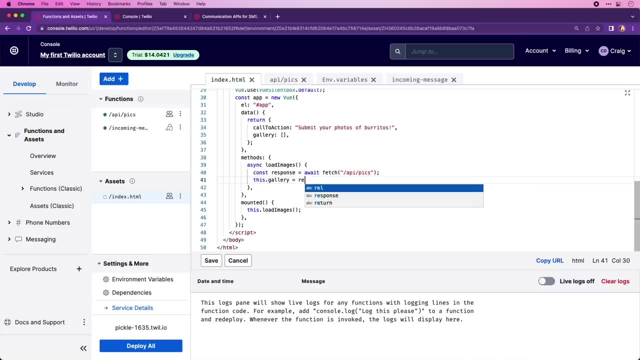 that will actually return the JSON representation of whatever came back. So what I'm going to do is I'm going to get rid of this gallery, this hard-coded gallery that is gone, And I am going to say await, We are going to await. 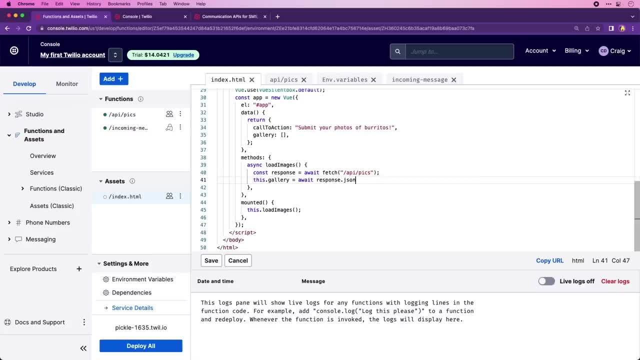 because this method is also asynchronous responsejson, So that's going to get back whatever is in this response that came back. This response has all sorts of metadata about it, but we just want to get the data out of it And that's by using this json. 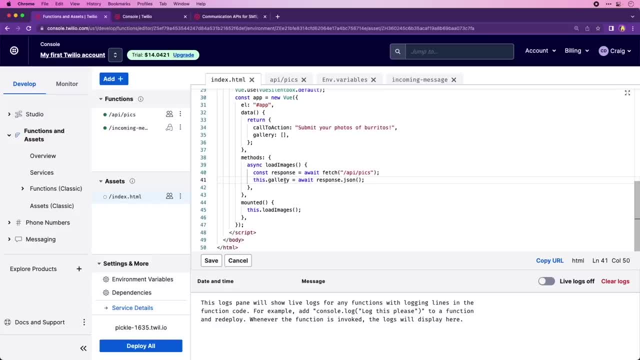 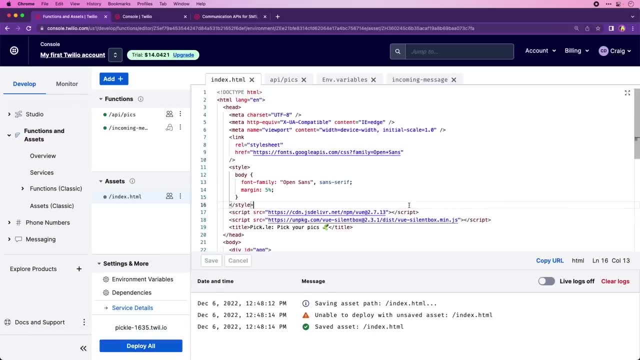 And because our API is JSON enabled, it's just going to come out. All right, let's deploy it. I cannot stop. Oops, this is not unable to deploy because I didn't save it, So I need to save it. So I need to save it first. 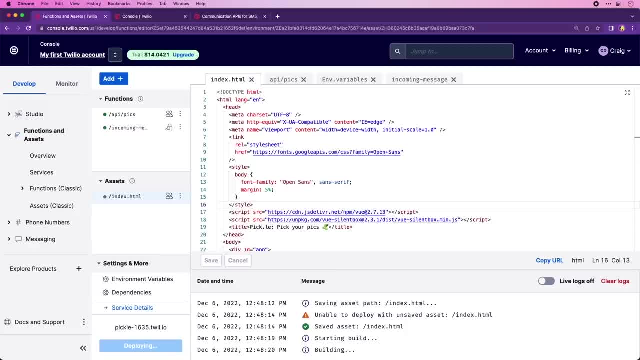 I cannot stop thinking about that burrito. It was so good. I submitted a selfie of myself and I texted it to my Twilio number And I got a reply back from my Twilio trial account right, And it says thanks for submitting it. 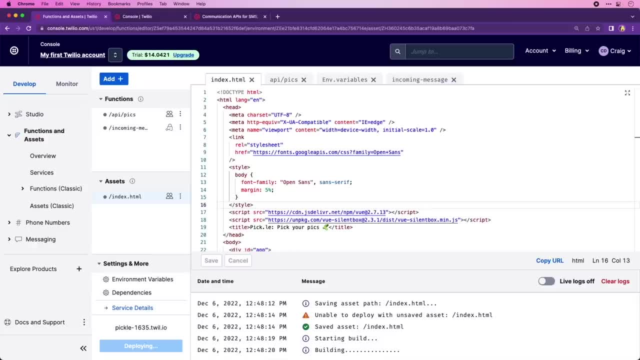 So, if all goes well, when we look here, I'll be able to show you the burrito that I texted to my number. So it's been deployed and I'm going to come in here under this assets and I'm going to copy this URL. 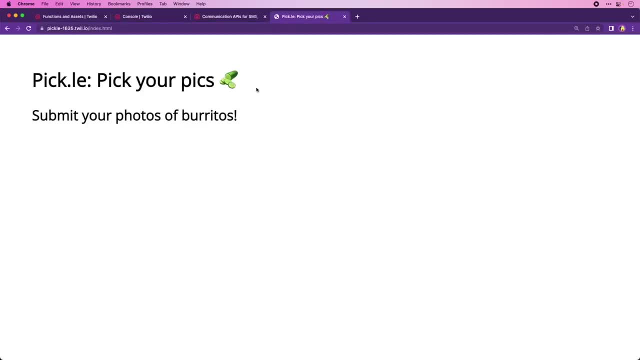 And I am going to paste it here, And this view application is going to go and it's going to hit my API and it's going to bring back some photos into this gallery. And here it is. Look at the size of this thing. 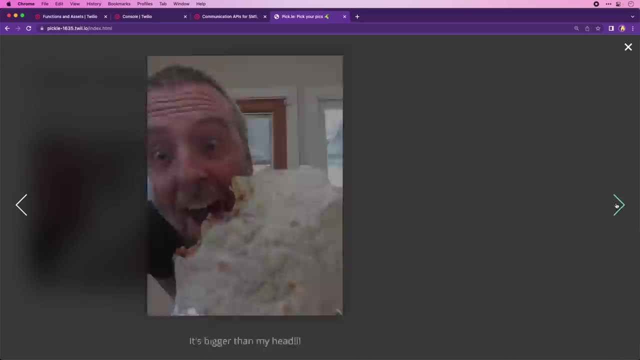 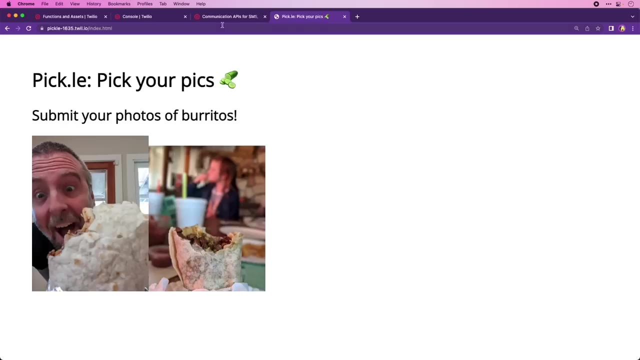 It was truly bigger than my head, So if we click that we could go. we could see my other beautiful burrito there as well. Now let's look again back here at the client side of things and just take a look at how beautiful this is. 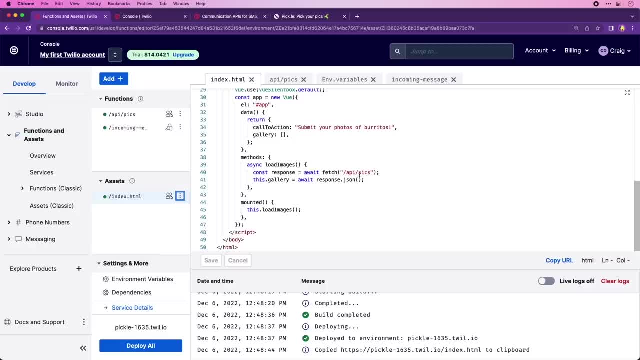 It's just two lines and it's hitting our API. So that's the power. We were able to hit an API and get users submitted text messages, text photos, right, And it only took two lines And really it only took one line actually, you know. 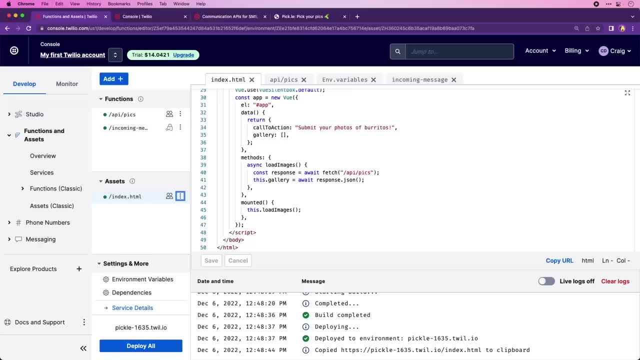 like if we could have, like, chained some stuff on top of this, Awesome. Now, one thing that I do want to note is that there's no authentication at all to this API. right, I could, I didn't supply any authentication information at all. 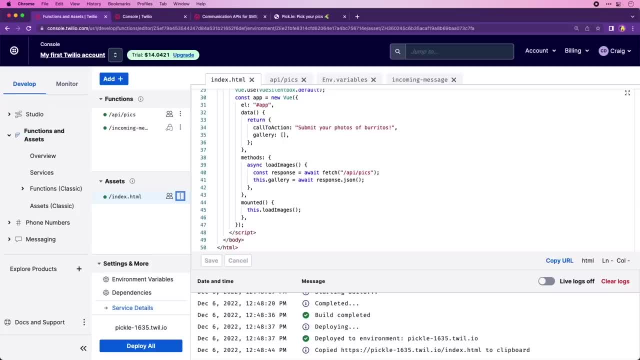 It's open to everyone And that's kind of a good thing. If you are working on a client side application, you don't want to pass your keys around Like I would not want to put my Twilio keys here on this page because I don't know if you know this. 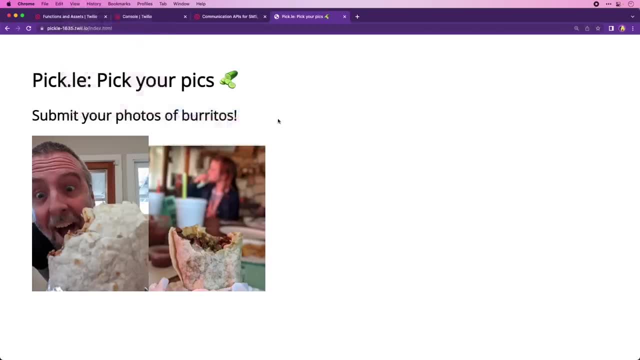 but you can actually see everything that comes down. So I'm going to view the source of this and you can see. here's the source that we're looking at, And if I had to use any sort of API keys, I would see them right here. 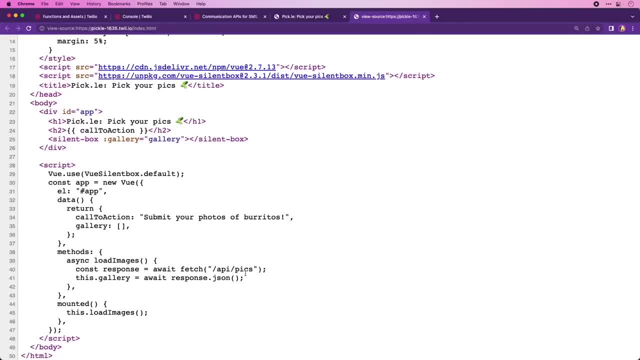 You don't want to leak your keys that way. Check the notes for more information on how to get around this. But typically this is what you do is you write a server that then the server keeps track of all the keys And you connect to the server. 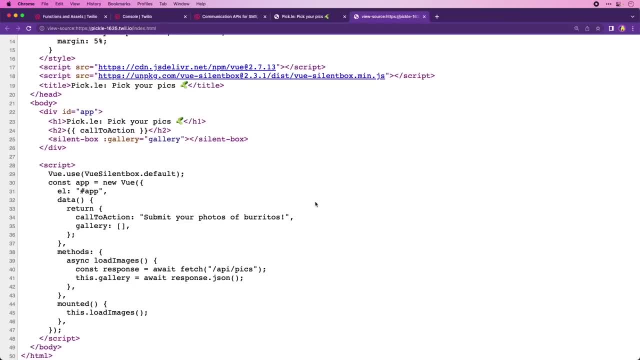 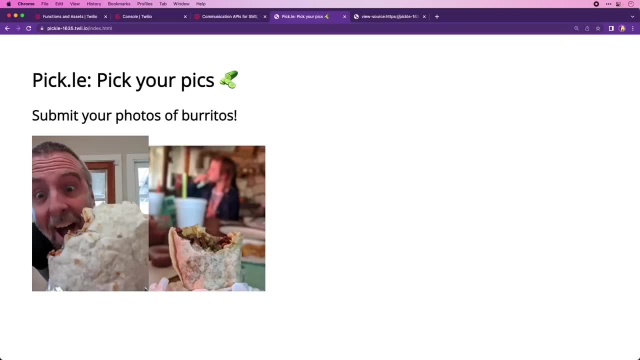 But if you do need to provide some authentication locally on the client, there are ways to do that. Check the notes. but look at this, look at this. You did this. you have designed a new interface, a text messaging interface. right, 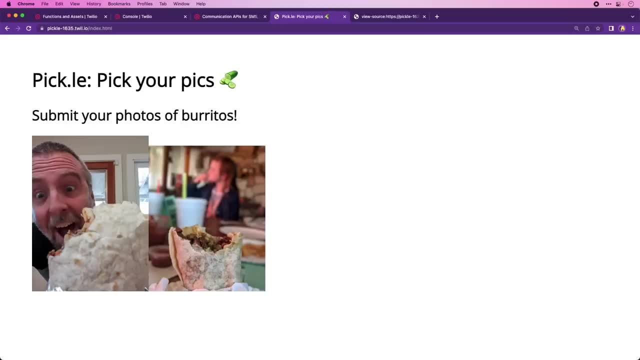 A TMI. well, I hope this wasn't TMI, or also known as too much information for you. You learned a whole lot about APIs, and not just the web-based ones. You saw them in practice and you even built your own one. 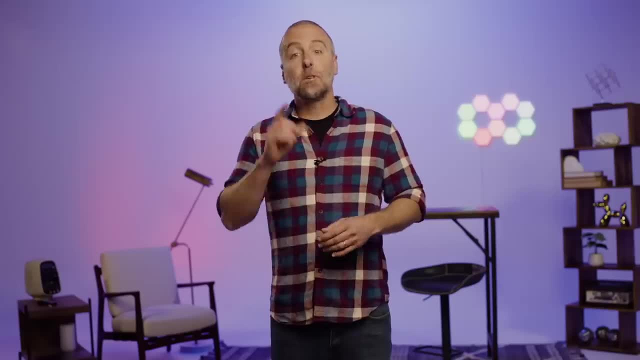 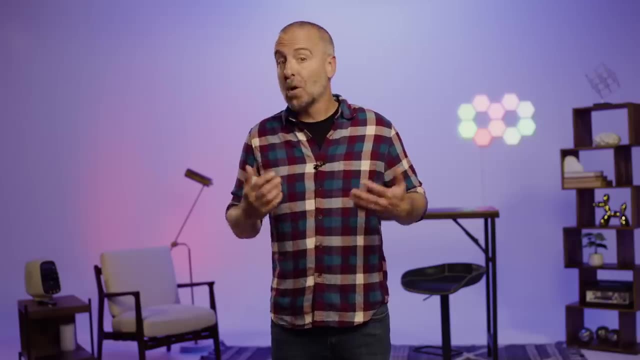 You really deserved that burrito. Awesome job: You've just built and consumed your own API. Now here's my question to you: Do you think that the API code that we wrote together should be considered RESTful? Why don't we take a look? 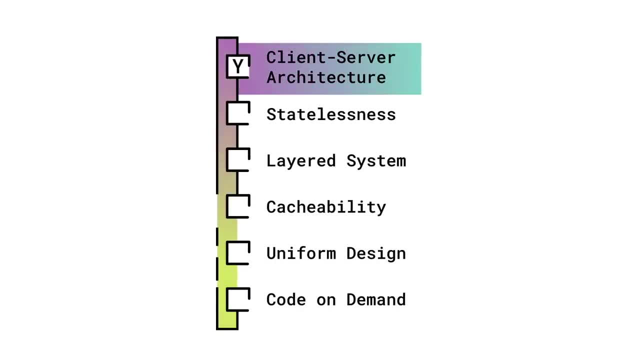 at our weathered scavenger hunt card. So it's definitely a client server architecture. Our client happens to be, in this case, a Vue application running in the browser and our server is a serverless node application, but any client could connect and use this. 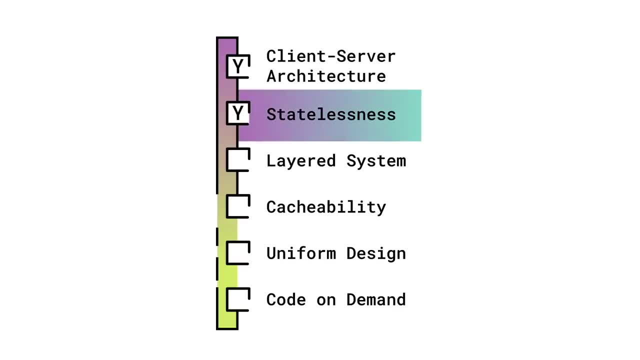 Statelessness. it's definitely stateless, right? We aren't requiring any prior knowledge about the client Cacheability. hmm Well, at the moment we aren't providing any caching information, though we could right. We could fairly easily pay attention. 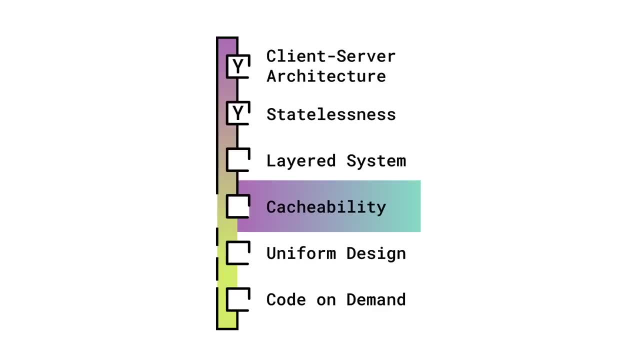 to those headers coming in and we could respond appropriately. It would require us writing some additional code and thinking through some of the edge cases, but we could do it. Let's put that in the maybe column Layered system. yeah for sure, right? Connect" let's액tyoucom to sportscomicaddressnet. Launch Vuecom D. certain should be working in. your Mitxo app Is Chess Same. Stay on the same level at any time we able includes us, and you'll also use the serverless license to accessicitize us as they want- much less or the same. 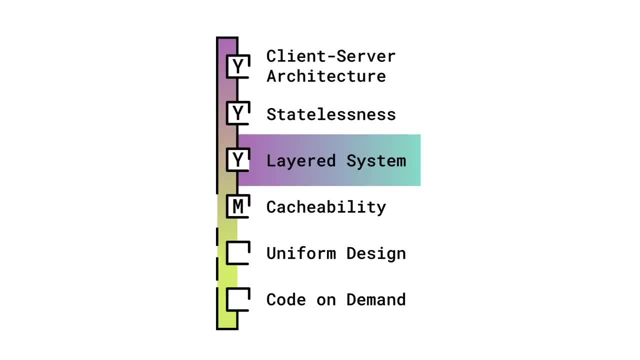 right. In fact, it's a little layered already. Our API is calling another API, but our client doesn't need to know that. We can also add additional functionality and the contract wouldn't change Code on demand. We haven't even talked about this one yet, and it's the only. 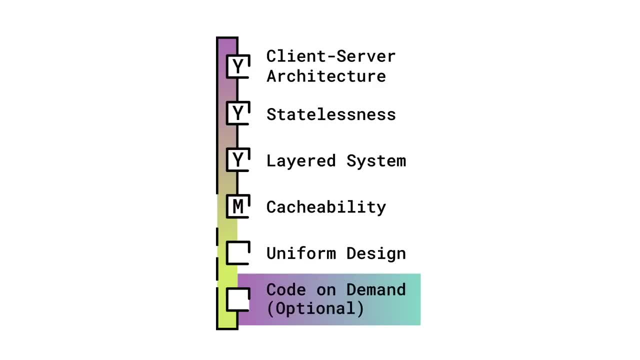 optional requirement. Basically, this means that your API returns code that is runnable, Like maybe it returns an embeddable widget or some actual JavaScript code. This doesn't make any sense in our use case and that's totally okay, So we're going to drop this one into the 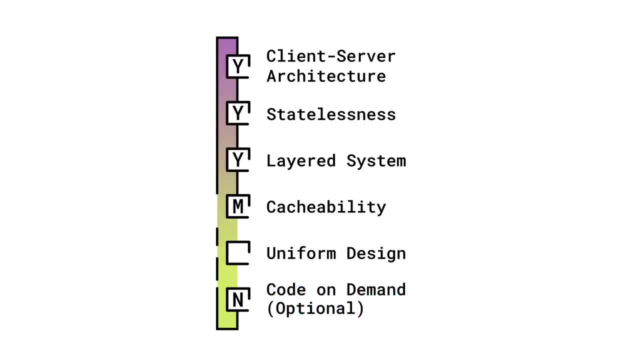 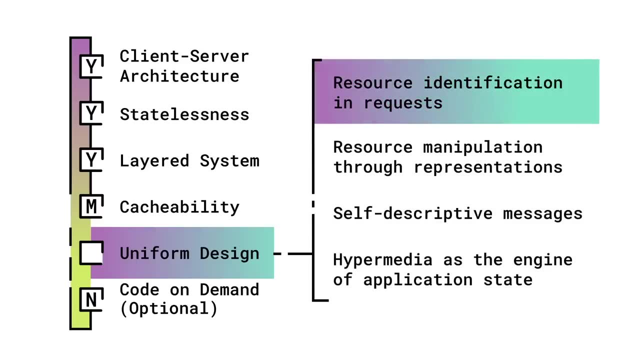 no column. So we're looking good so far. but here comes the doozy Uniform interface. So remember this one has four subsections: Resource identification and requests. Currently, we're just representing all the messages as objects and absolutely no way to identify them. 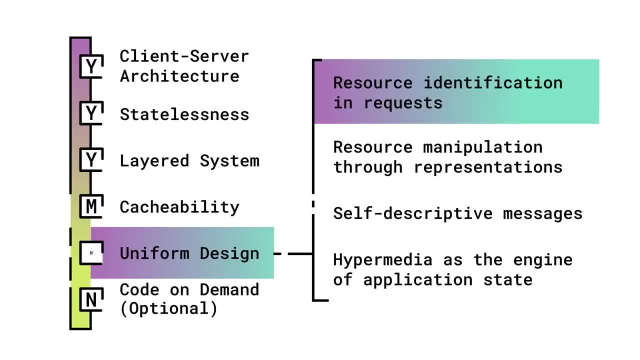 So we failed this sub requirement and therefore this is a no. But let's keep going through the rest of these, Pun intended, Sorry. Resource manipulation through representations: We definitely do not allow any sort of manipulation of the images, so this is another fail. 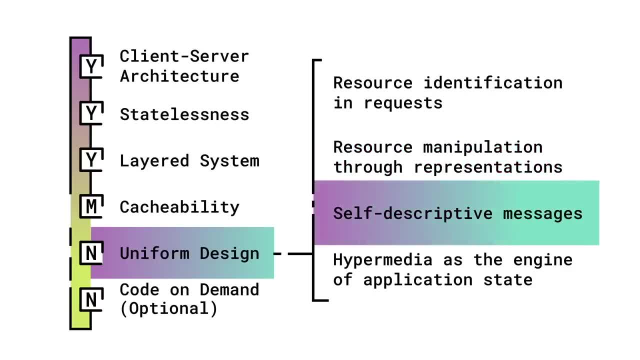 Self-descriptive messages. We haven't gone over this yet, but by using headers we can tell that this is JSON. The message sent down has a type and it's clear that it should be JSON decoded to be used. Hypermedia as the engine of application state And, last but certainly not least, 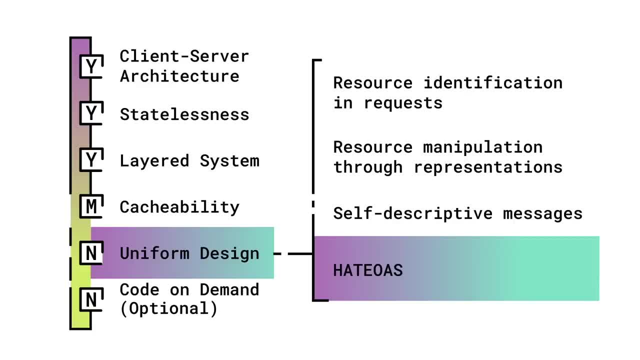 HATIOS or HATEOS. It's an often forgot about part of the RESTful constraint, And the idea here is that there are links to show off what more you could do with this and where you could find related resources. It provides URIs or links, and we did see this in both the Spotify and Twilio. 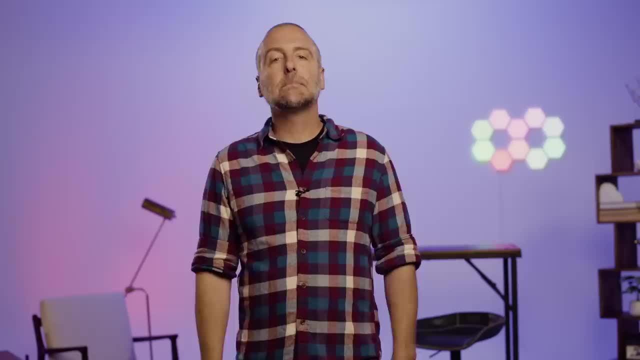 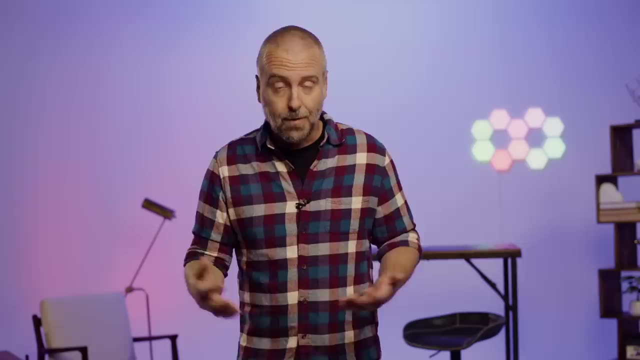 ones. However, ours doesn't provide links to other resources, So we don't have a RESTful API, and that's okay. It's going to suit our needs. It does look like we could get there pretty quickly if we wanted to. One thing I want you to gain from that exercise, though, is that you now 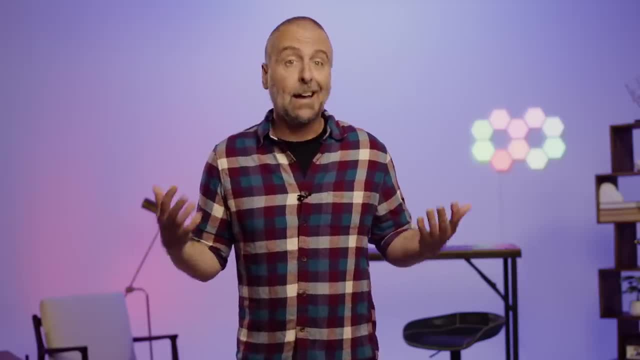 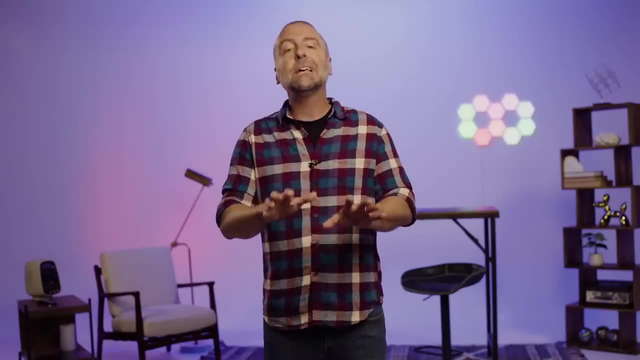 have the ability to identify whether or not an API is RESTful, and I hope that felt pretty good. We've now completed the scavenger hunt. We revealed all the constraints and I hope most of those are pretty clear. Please don't feel like you need to memorize those. You can find those. 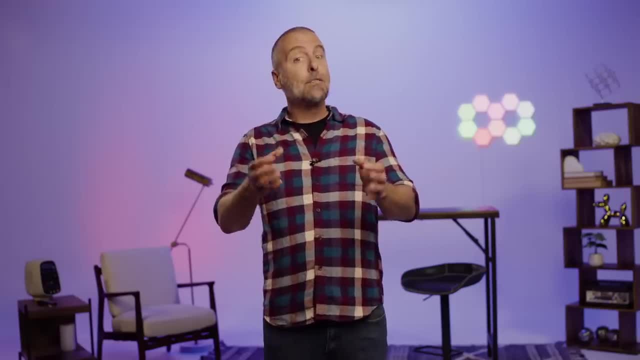 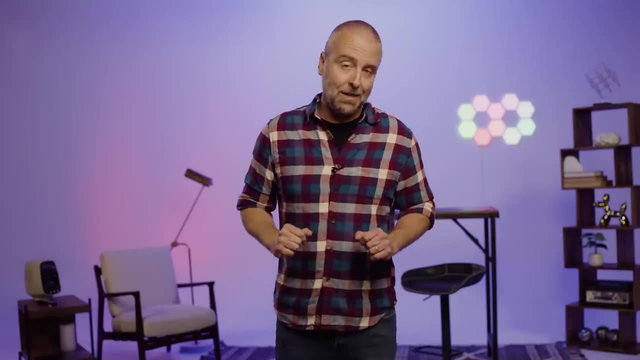 same constraints littered all over the internet. Now, as a prize for finishing the constraint scavenger hunt, I've dropped links to my favorite REST API constraint documentation for you to lean on, should you need to. I've also included links to the popular REST API frameworks that will help. 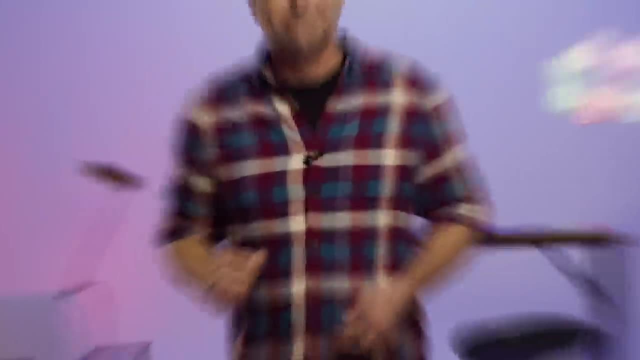 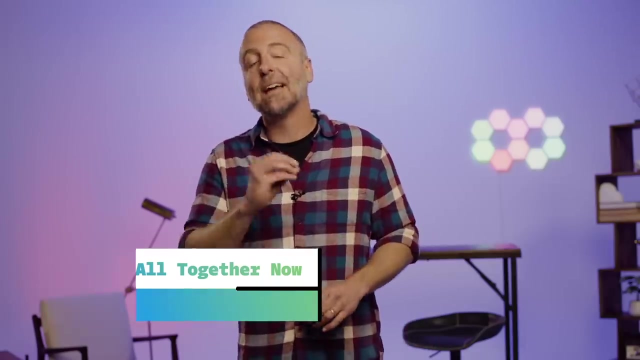 you design RESTful APIs, Make sure to check out the notes. You did it. You just completed a whirlwind of RESTful APIs and I hope that you can see how much more power they can add to your programming journey. By looking at interfaces in general, I hope you're more comfortable with the idea of not 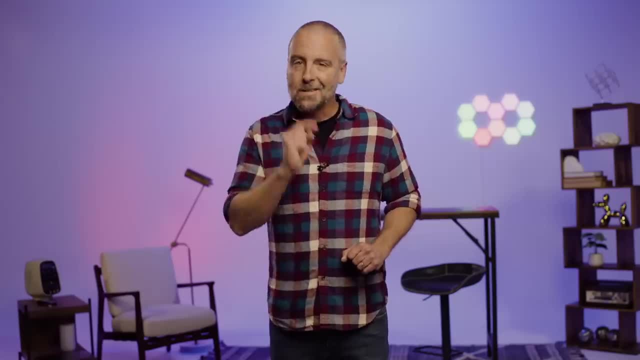 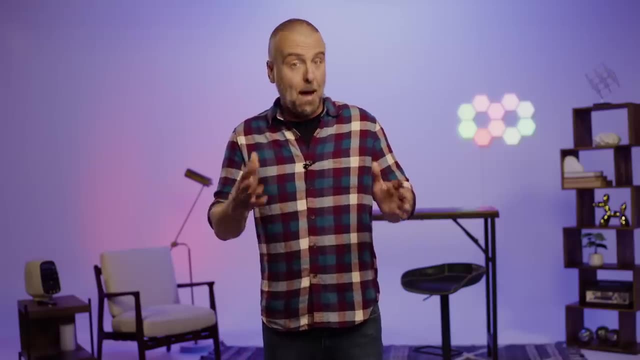 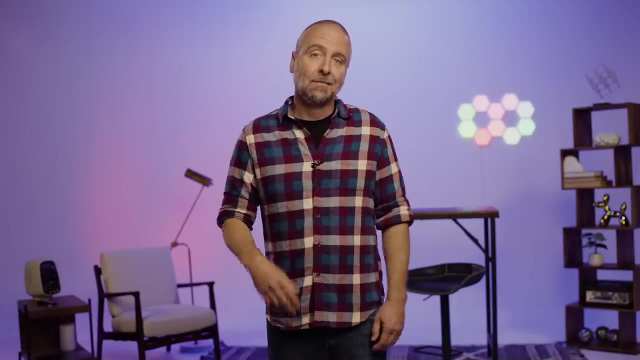 fully understanding exactly how something is working, but still leaning on that abstraction to build your tools and applications. Do this all the time with physical object interfaces and APIs or application programming interfaces. They aren't all that different. I hope you enjoyed taking this course. I know I had a lot of fun making it. If you think someone you know might benefit from this, 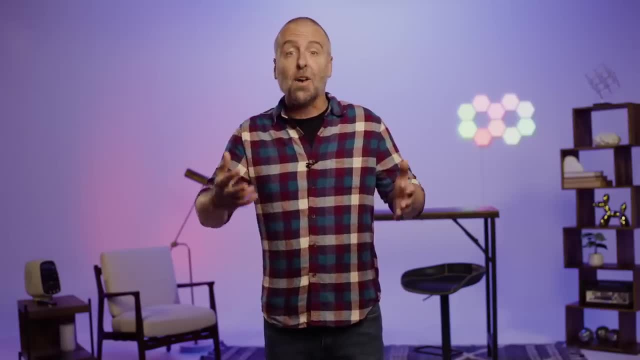 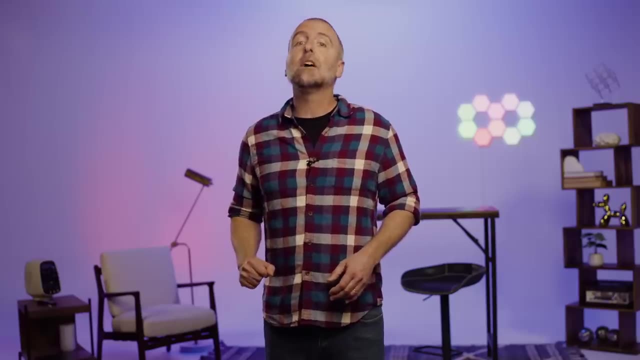 course, please share it with them. I'll see you next time. I'd love to hear your feelings, your thoughts, your dreams, So I threw together a little something, using a smattering of APIs to capture your feedback. If you've got the time, I'd love to have. 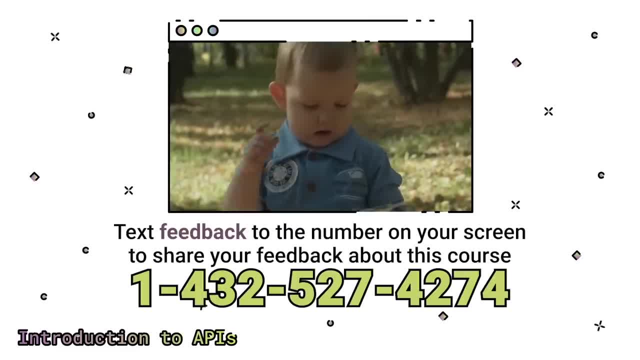 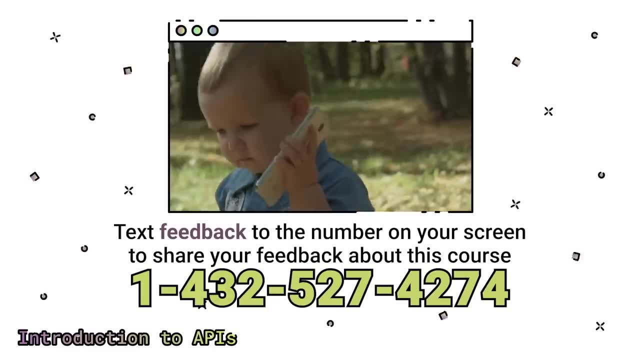 you answer a quick text-based survey: Text feedback to the number on your screen. Well, actually, you know what. If you want, you can also call and just leave me a message too. I use an API for that too. So please, please, please, keep me posted on your journey, and really I can't wait to see what you.